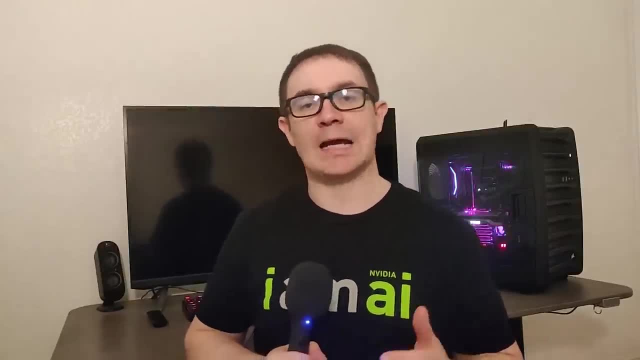 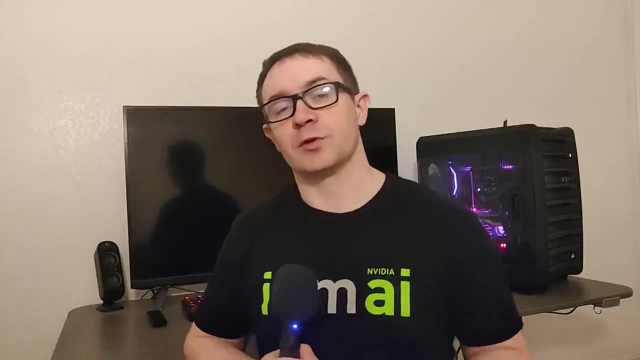 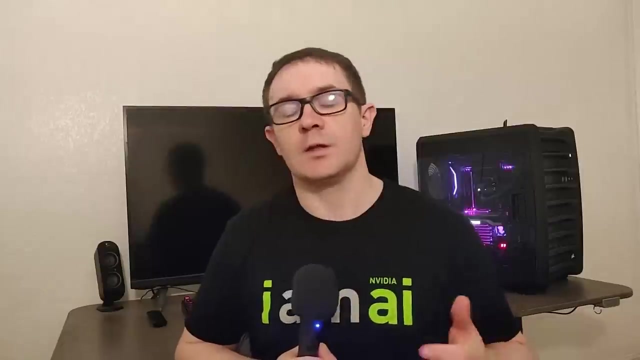 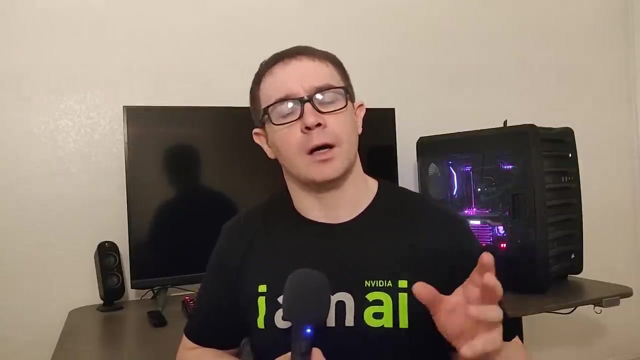 Welcome to an introduction to advanced actor critic methods. I am your instructor, Dr Phil Tabor. I'm a physicist, former semiconductor engineer turned data scientist. In this course, you're going to learn the fundamentals of advanced actor critic methods. Now, if you've seen some of my prior work here on the free code camp- and you may have seen some work related to deep Q learning as well as actor critic methods- there will be a little bit of overlap between the other actor critic courses and this material, simply because I can't assume everyone has seen my earlier content. 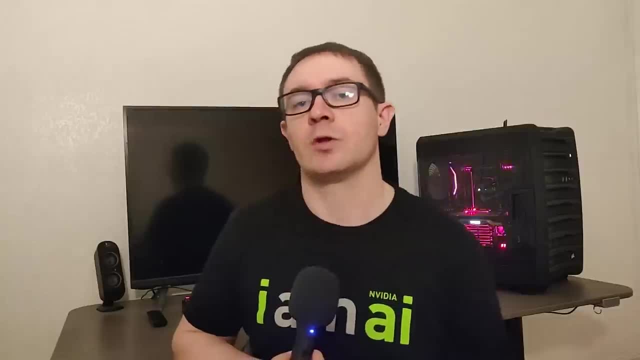 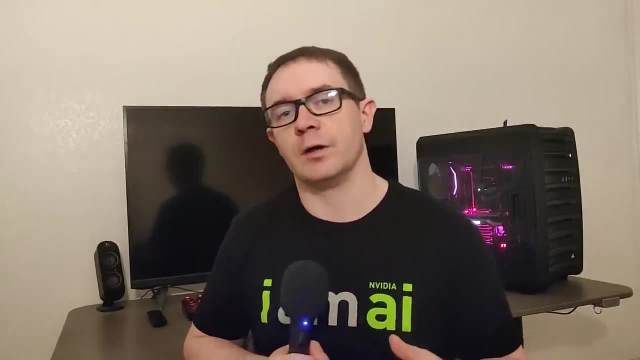 No need to go back and rewatch that, though, although you are free to do so if you wish. I will include enough information in this particular course for the motivated beginner to get started in the field of deep reinforcement learning and actor critic methods in particular. 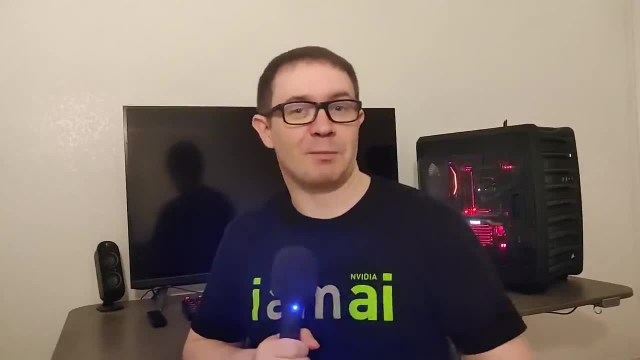 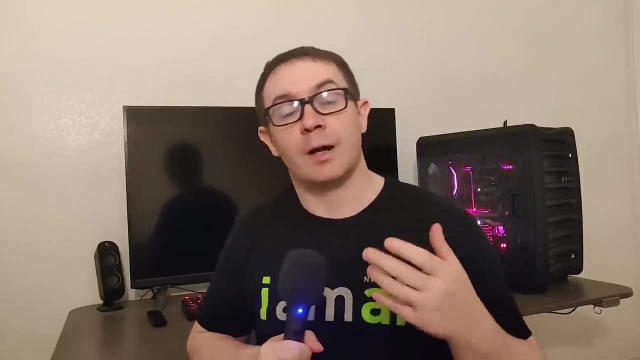 Now why are actor critic methods important? That's a great question I'm glad you asked. The basic idea is that things like Q learning are great for learning. problems with discrete action sets, like playing video games where you can move left, right or shoot your face. 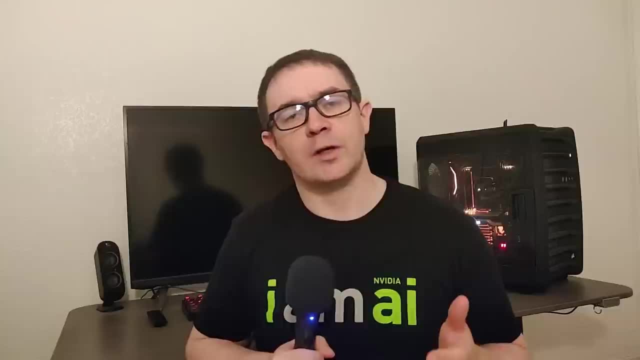 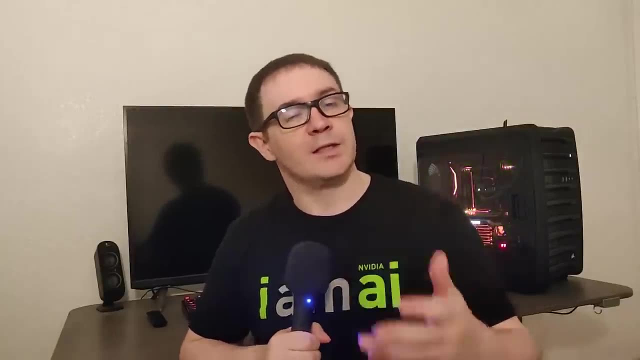 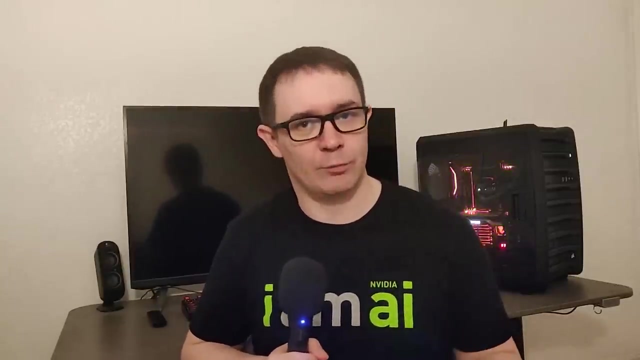 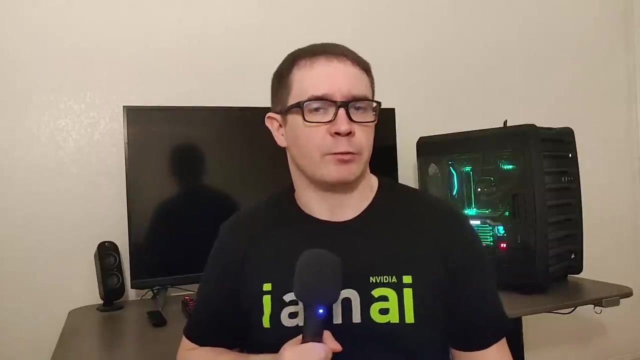 You can use laser blasts or the invading aliens, but it falls down when attempting to handle things like continuous actions. So this is important in fields like robotics, where you are applying continuous voltages to motors and joints to actuate movement, And so we need new technology to handle robotic movement above and beyond deep Q learning. Now, far from being a theoretical exercise in March of 2021, this year, a group at Berkeley did in fact, use deep reinforcement learning to do that. 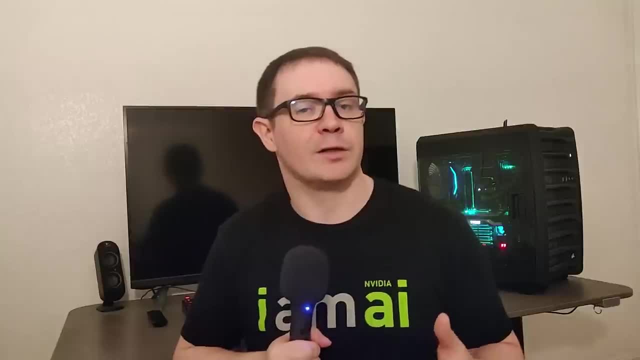 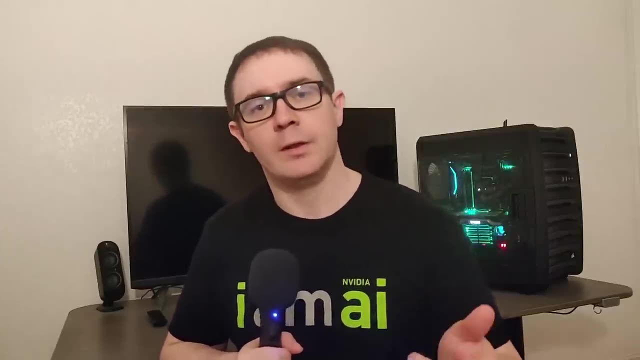 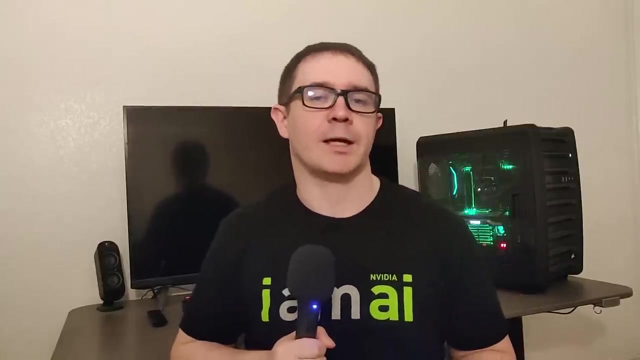 And so I'm going to detail that on my channel. By the time you see this, it may already be out, So go ahead, check me out at Machine Learning with Phil. I'll leave a link in the description. You can go subscribe if you are interested in more deep reinforcement learning content. but enough of the shameless plugging. 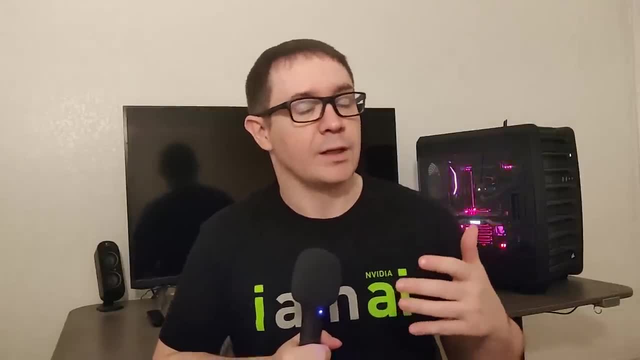 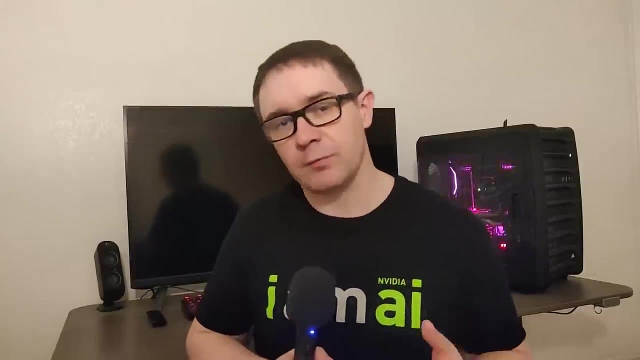 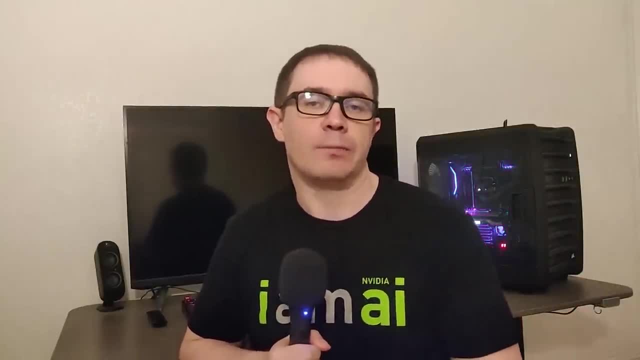 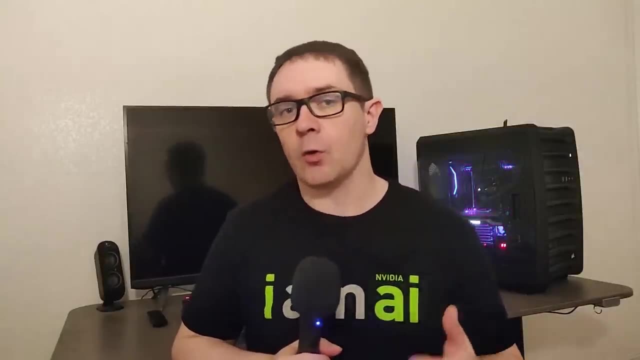 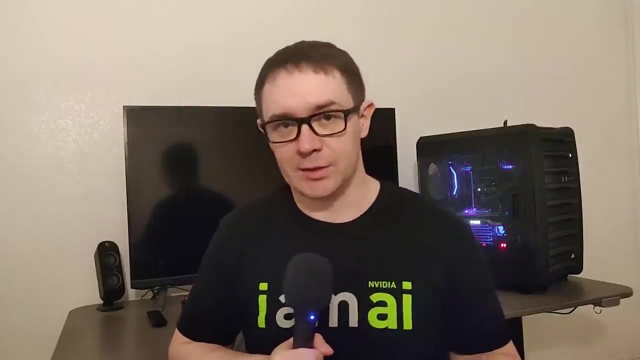 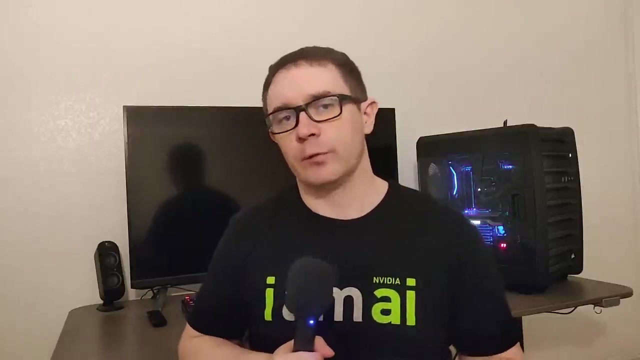 The environment is input and outputs some action. Now, in the case of a robot, that action could be an actual voltage that we apply to our motors, or it could be a probability distribution that we sample to generate some action. So, for example, Gaussian distribution, you know a normal bell curve that you sample to get some value for your action. We're going to cover both cases in this course. 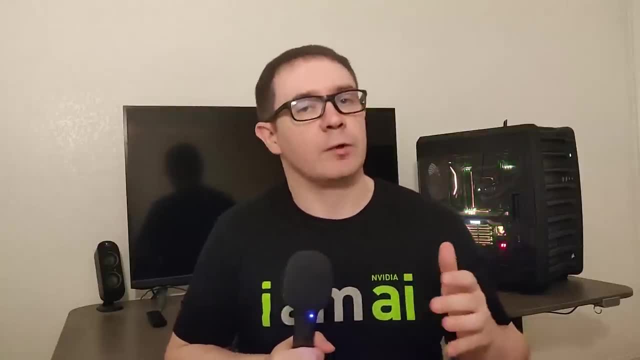 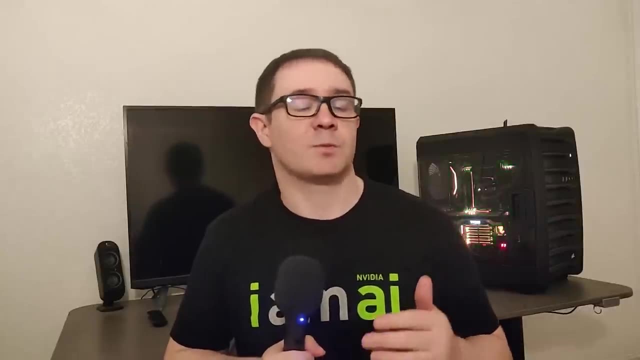 We're going to cover a whole host of algorithms, starting with the The vanilla actor critic method, deep deterministic policy gradients, twin-delayed deep deterministic policy gradients, proximal policy optimization, soft actor critic as well as asynchronous advantage actor critic. 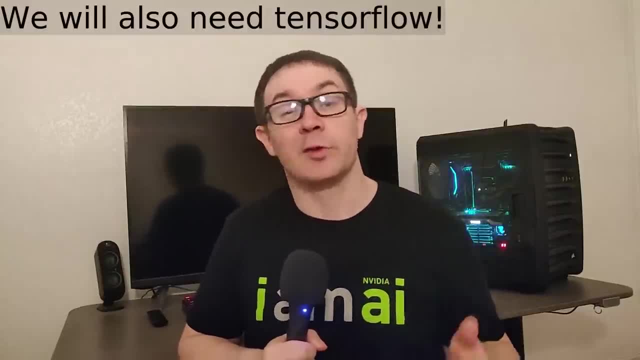 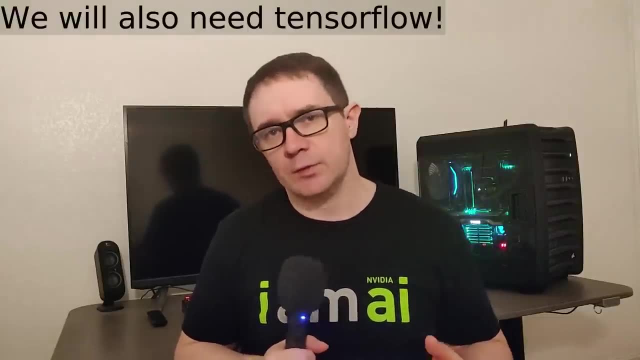 Try saying that five times fast. As far as software requirements go, they are relatively light, so we will need NumPy, PyTorch and Matplotlib. I highly recommend using the versions that I will leave for you in the description, because NumPy, in particular, likes to deprecate stuff. 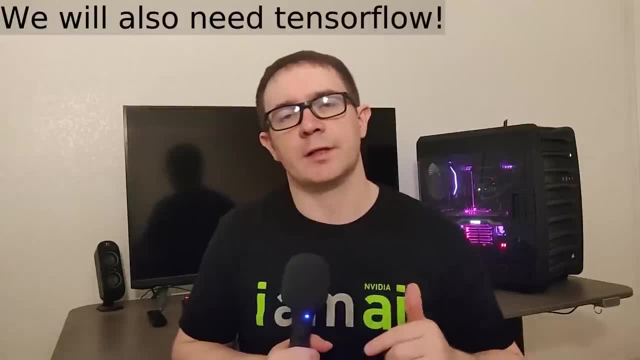 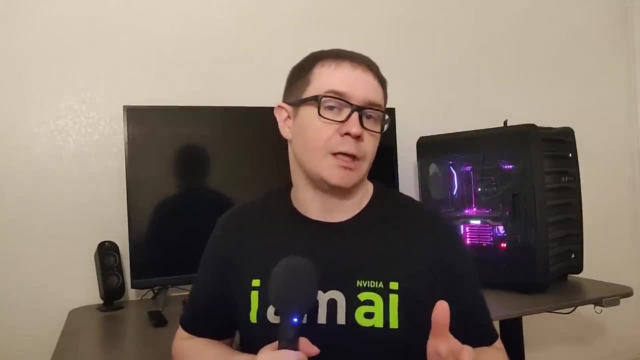 and that tends to Break my code. So if you use the versions that I've linked in the description, it's almost guaranteed to work, provided we didn't make some mistake along the way. As far as hardware, you're going to need a GPU. 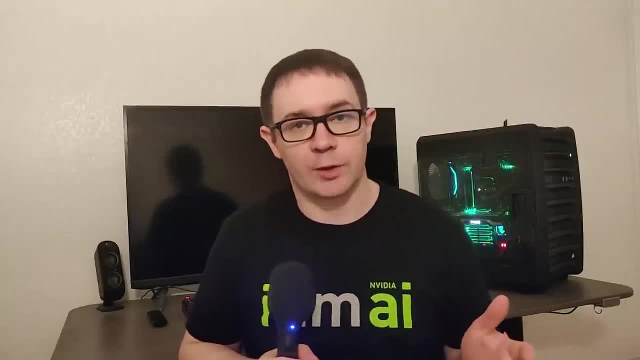 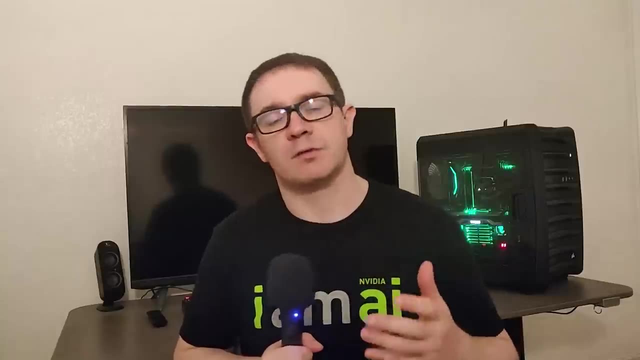 Unfortunately, in 2021, the GPU market is totally broken, so hopefully you already have one on hand. If not, don't despair. In particular, the A3C algorithm- asynchronous advantage actor critic- is designed to run a multi-core CPU, so at the very least, you'll be able to run that and get really good results. 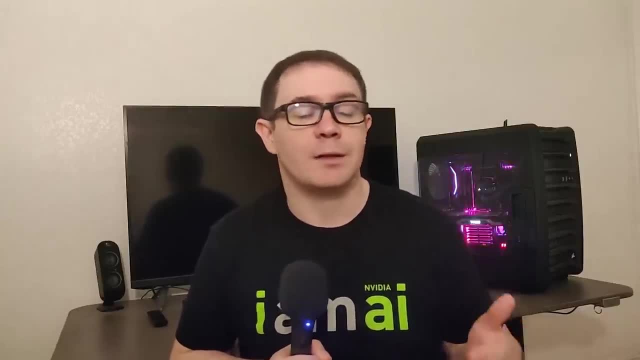 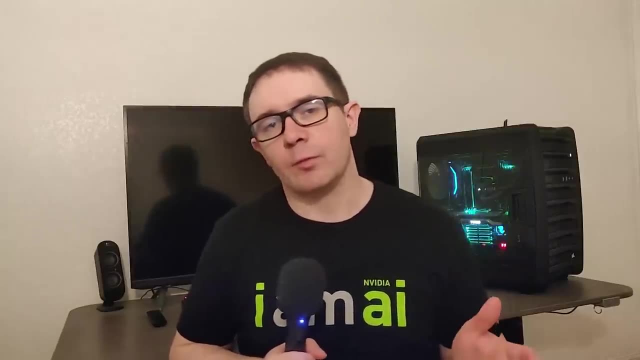 Other algorithms, You may be able to get something that converges, although the timeline- the amount of time you're going to have to train- is going to be a little bit longer, so you may want to leave things running overnight. With all of that said, I will check in periodically for questions. 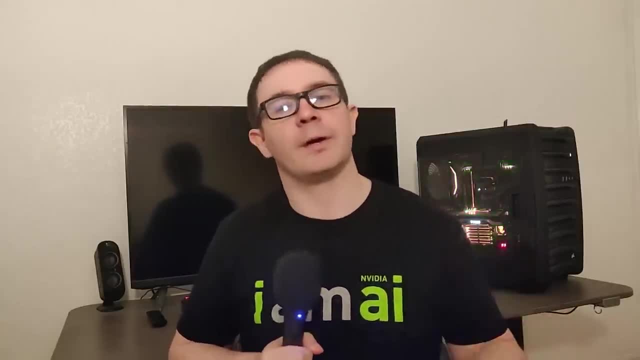 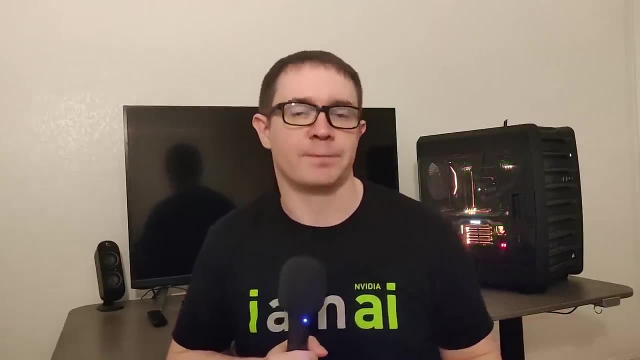 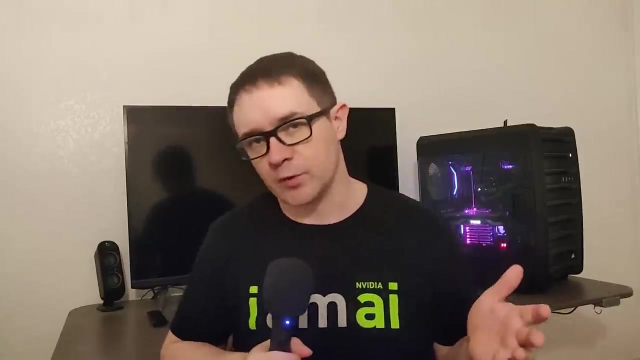 Obviously, I don't get notifications from the free CodeCamp channel, but I'll do my best to patrol the commas to see. should there be any confusions or need for clarification, I can swoop in to render assistance. Once again, if you like this type of content, check me out at my YouTube channel, Machine Learning with Phil, where I go over all things: deep reinforcement learning. 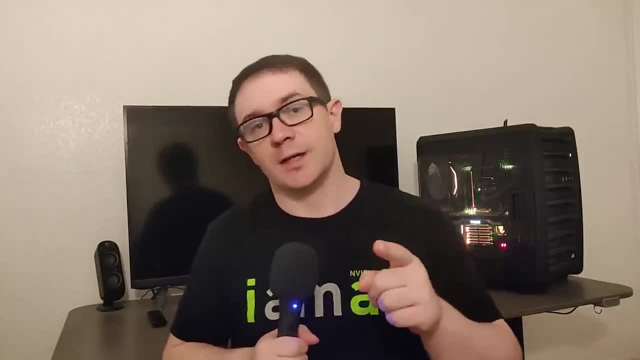 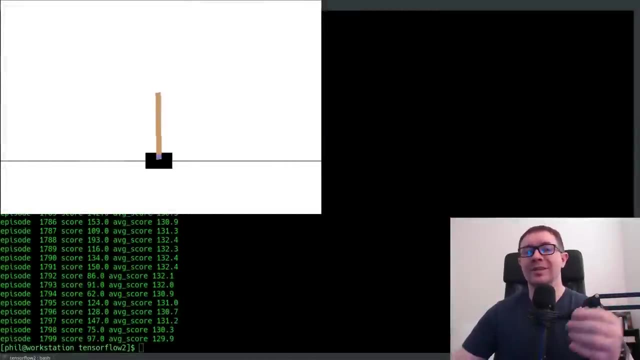 and occasionally natural language processing as well. Let's go ahead and get started and I look forward to seeing you on the inside. Welcome back everybody. In today's tutorial, you are going to get a mini crash course in actor critic methods in TensorFlow 2.. 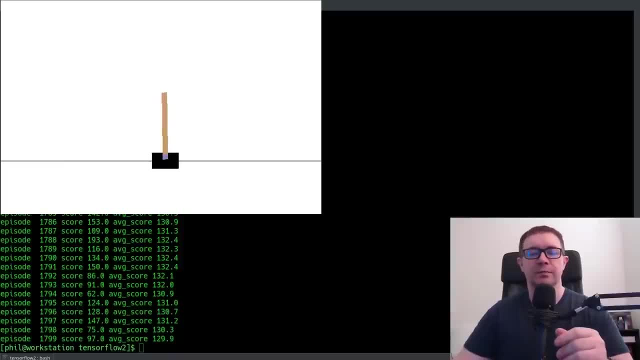 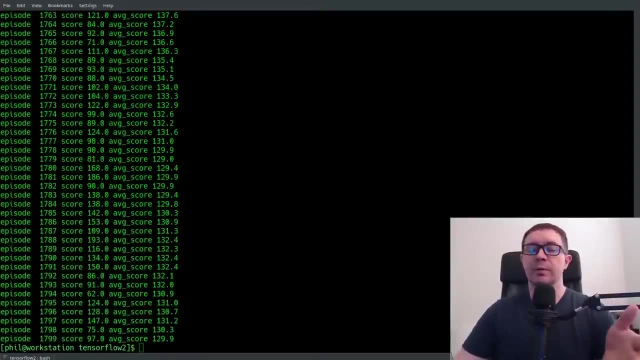 We're going to have around 15 minutes of lecture followed by about 20 minutes of coding, and you're going to learn everything you need to know to go from start to finish with actor critic methods. If you'd like to know more, you can always pick up one of my Udemy courses on sale right now- link in the description. 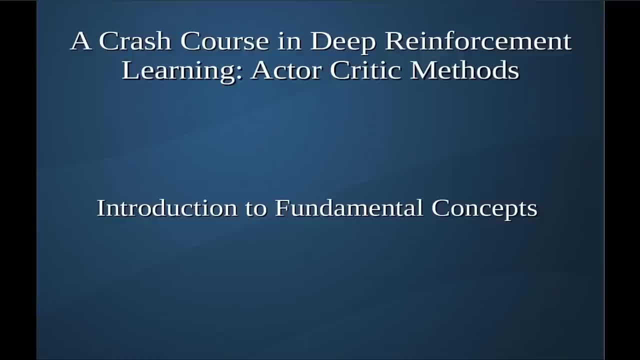 Let's get started. Welcome to the crash course in actor critic methods. I'm going to give a relatively quick overview of the fundamentals of reinforcement learning in general, and then of actor critic methods in particular. Finally, we'll work together to code up our own actor critic agent in TensorFlow 2.. 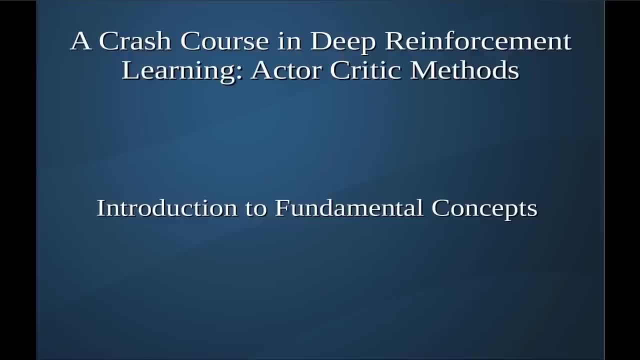 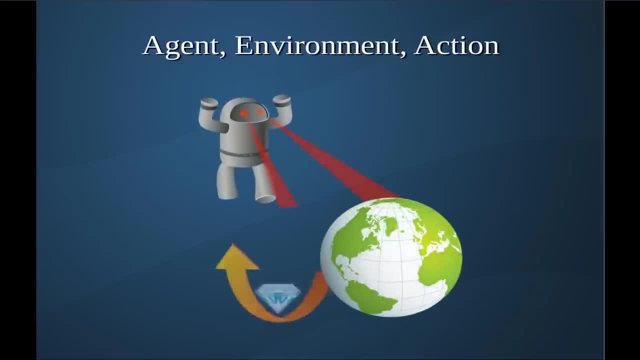 This is geared toward beginners, so feel free to ask some questions in the comments section. Reinforcement learning deals with agents acting on an environment, causing some change in that environment and receiving a reward in the process. The goal of our agent is to maximize this total reward over time, even if it starts out knowing literally nothing about its environment. 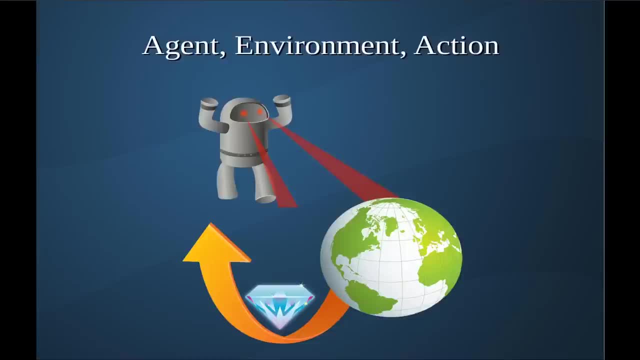 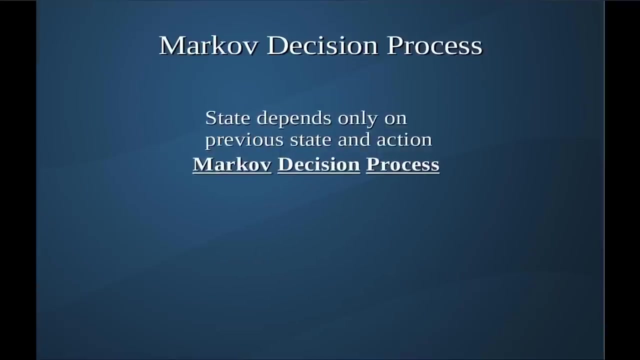 Fortunately, we have some really useful mathematics at our disposal, which makes figuring out how to beat the environment a difficult yet solvable problem. The mathematics we're going to use relies on a very simple property of the system, the Markov property. When a system depends only on its previous state and the last action of the agent. 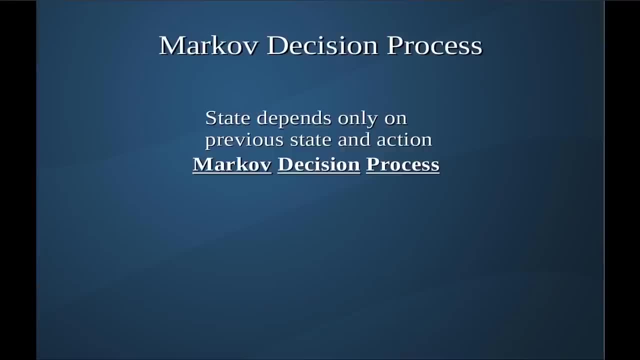 we say it is Markovian. As we said earlier, the agent is given some reward for its action. So the set of states the agent sees, the actions it takes and the rewards it receives forms our Markov decision process. Let's take a look at each of these components in turn. 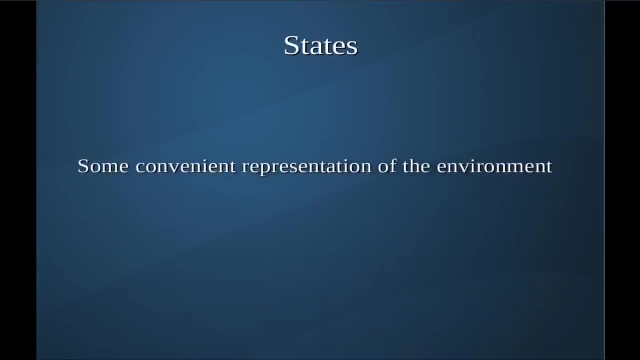 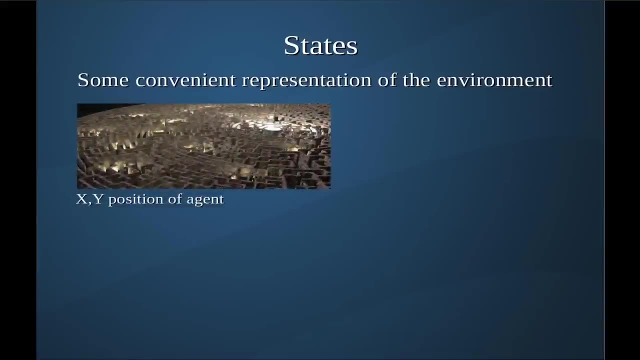 The states are just some convenient representation for the environment. So if we're talking about an agent trying to navigate a maze, the state is just the position of the agent within that maze. The state can be more abstract, Like in the case of the lunar lander, where the state is an array of continuous numbers that describe the position of the lander. 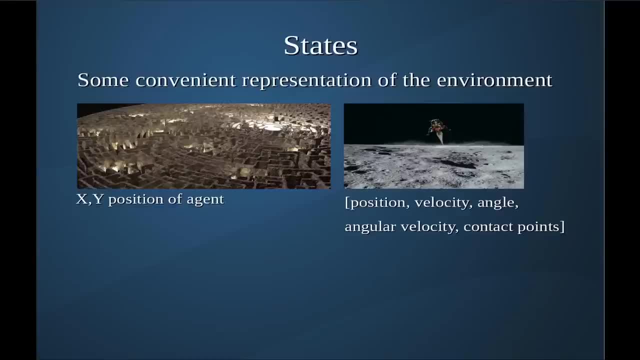 the velocity of the lander, its angle and angular velocity, as well as which legs are in contact with the ground. The main idea is that the state describes exactly what about the environment is changing at each time step. The rules that govern how the states change are called the dynamics of the environment. 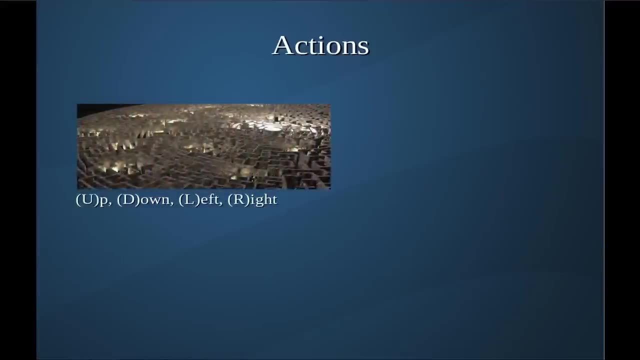 The actions are a little simpler to understand. In the case of a maze running robot, the actions would be just to move up down, left and right- Pretty straightforward. In the case of the lunar lander, the actions consist of doing nothing. 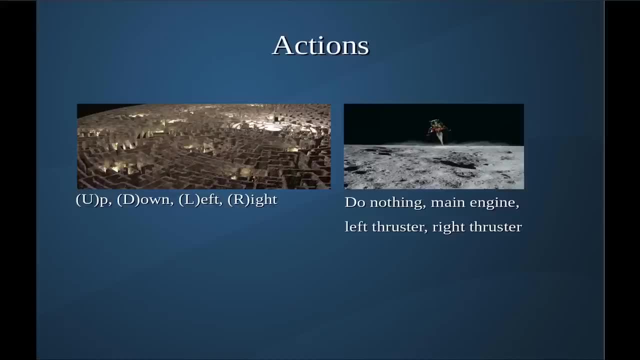 firing the main engine, firing the left engine and firing the right engine. In both these cases the actions are discrete, meaning they're either one or the other. You can't simultaneously not fire the engine and fire the right thruster, for instance. 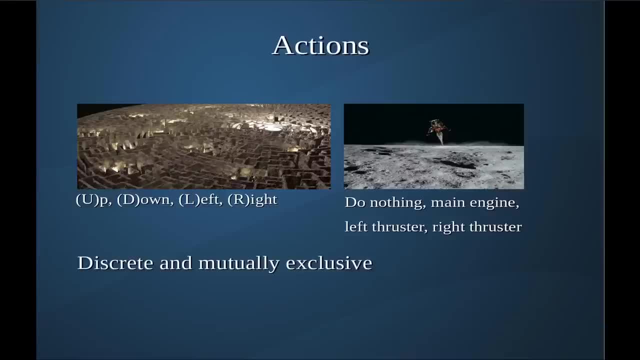 This doesn't have to be the case, though. Actions can, in fact, be continuous, And there are numerous videos on this channel dealing with continuous action spaces. Check out my videos on soft actor critic, deep deterministic policy gradients and twin delayed deep deterministic policy gradients. 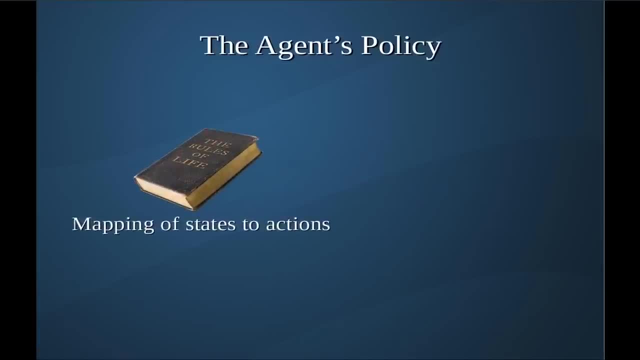 From the agent's perspective, it's seeing some set of states and trying to decide what to do. How is our agent to decide? The answer is something called the agent's policy. A policy is a mathematical function that takes states as inputs and returns probabilities as output. 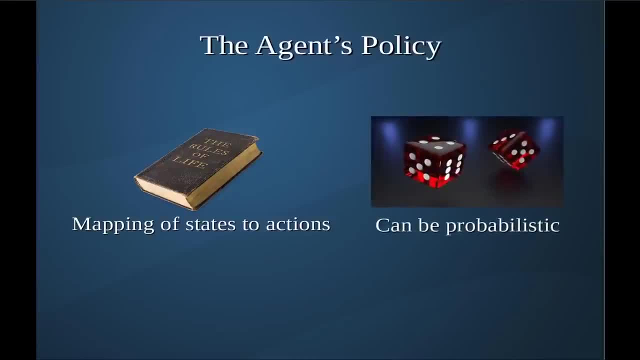 In particular, the policy assigns some probability to each action in the action space for each state. It can be deterministic, meaning the probability of selecting one of the actions is one and the others is zero, But in general the probabilities will be somewhere between zero and one. 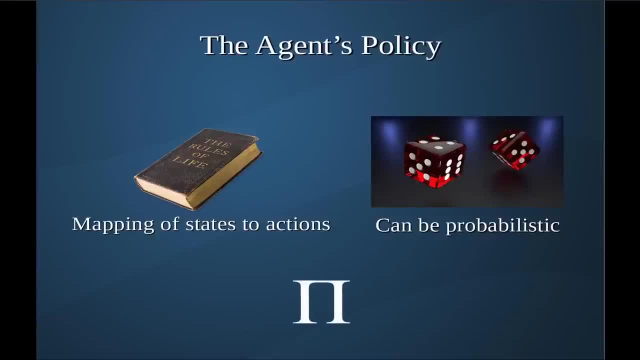 The policy is typically denoted by the Greek letter pi, and learning to beat the environment is then a matter of finding the policy pi that maximizes the total return over time, by increasing the chances of selecting the best actions and reducing the chances of selecting the wrong ones. 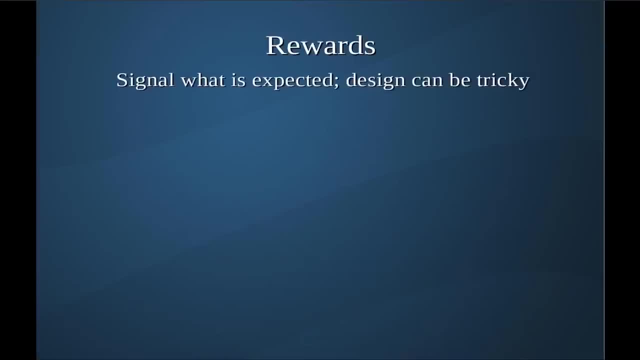 The reward tells the agent exactly what is expected of it. These rewards can be either positive or negative, And the design of rewards is actually a tricky issue. Let's take the maze running robot. If we give it a positive reward for exiting the maze and no other reward? 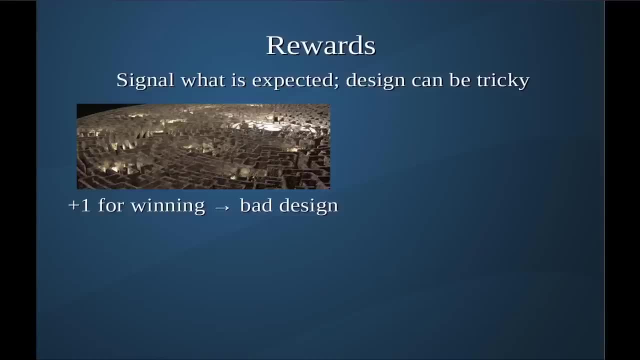 what is the consequence of that? The consequence is that the agent has no motivation to solve the maze quickly. It gets the same reward if it takes a minimum number of steps or if it takes 100 times that number. We typically want to solve the maze as quickly as possible. 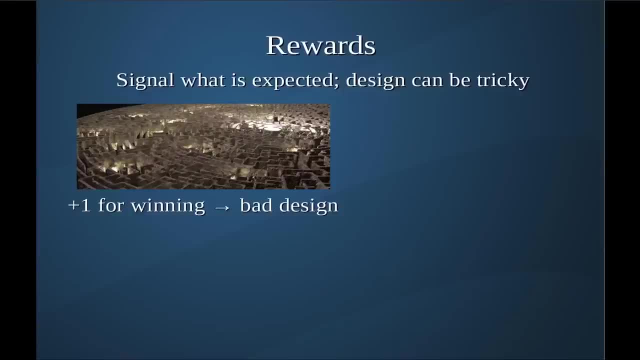 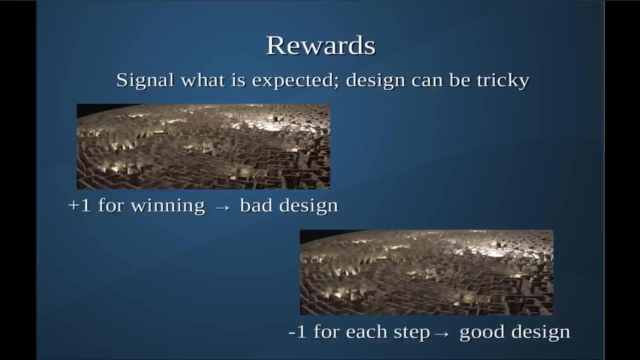 So the simple reward scheme fails In this example. we have to give a penalty for a reward of minus one for each step and a reward of zero for exiting the maze. Then the agent has a strong motivation to solve the maze in as few steps as possible. 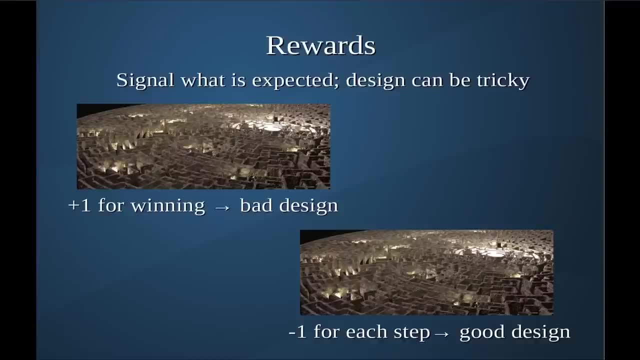 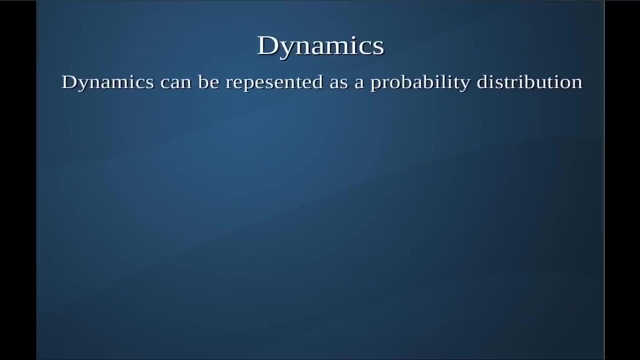 This is because the agent will be trying to maximize a negative reward, meaning get it as close to zero as possible. So now that we have our basic definitions out of the way, we can start to think through the mathematics of the reinforcement learning problem. 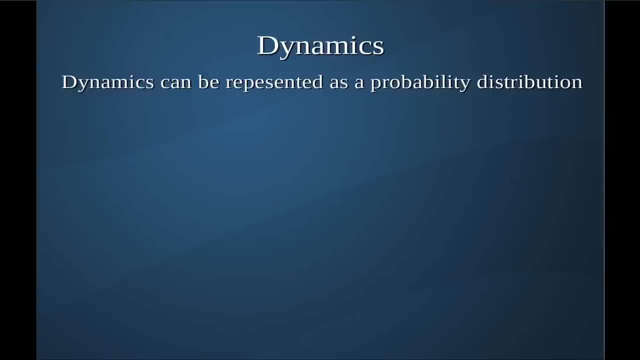 From the agent's perspective, it has no idea how its actions affect the environment, So we have to use a probability distribution to describe the dynamics. This probability distribution is denoted P of S prime and R, given S and A, which just reads as the probability of ending up in state S prime and receiving 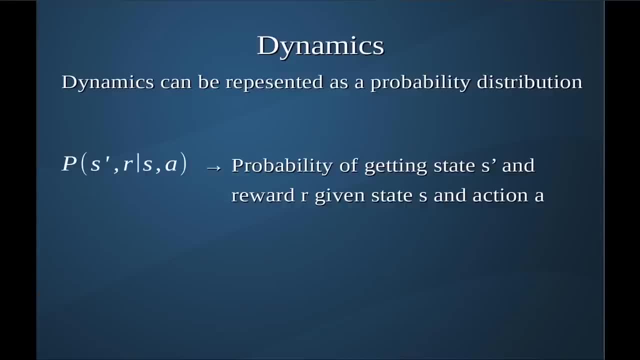 reward R, given we are in state S and take action A. In general, we won't know the value for this until we interact with the environment, And that's really part of solving reinforcement learning. Since we're dealing with probabilities, we have to start thinking in terms of expectation values. 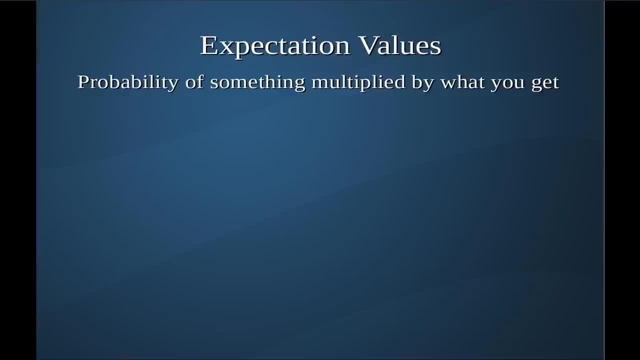 In general, the expectation value is calculated by taking into account all possible outcomes and multiplying the probability of that outcome by what you receive in that outcome. So in our Markov framework the expected reward for a state and action pair is given by the expectation value of that reward. 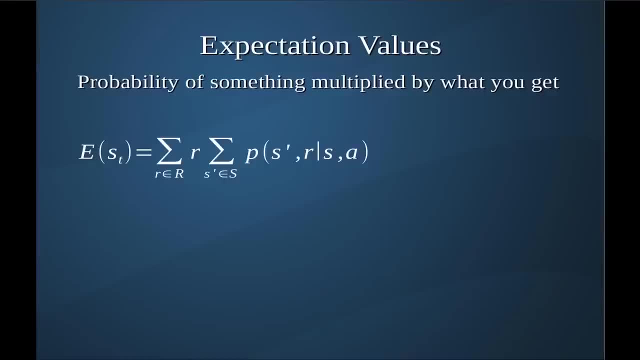 which is the sum over all possible rewards, the outcomes multiplied by the sum over the probabilities of ending up in all possible resulting states. For a simple example, let's consider a simple coin toss game. If we flip a coin and it comes up heads, you get one point. 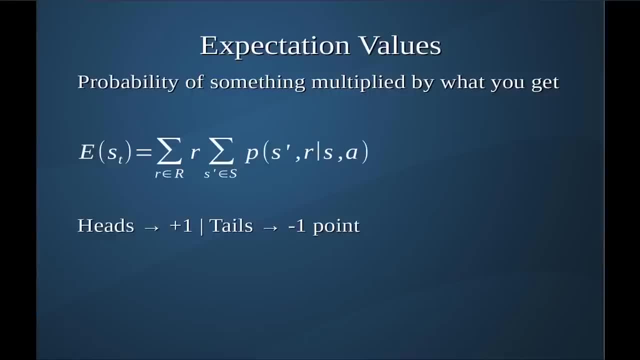 If it comes up tails, you get minus one point. If we flip the coin two times, what is the expected number of points? It's the probability of getting heads multiplied by the reward for getting heads, plus the probability of getting tails multiplied by the reward for getting tails. 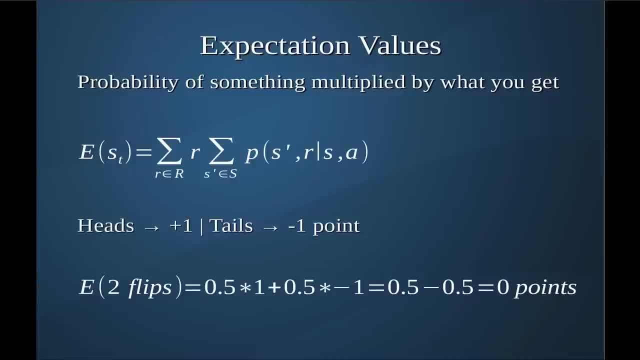 So it's zero point five times one, plus zero point five times negative one. This gives an expected reward of zero points, which is what you would intuitively expect. This is a trivial example, but I hope it illustrates the point. We have to consider all possible outcomes, their probabilities and what we would expect. 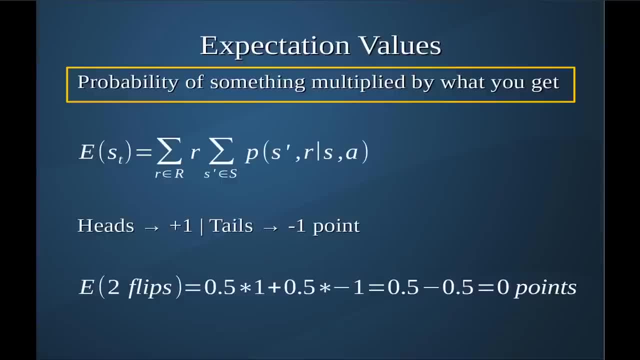 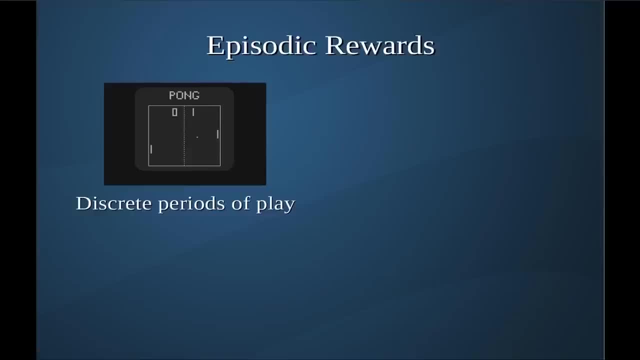 to receive in each of those outcomes. When we go to put theory in practice, we're going to be doing it in systems that are what we call episodic. This means that the agent has some starting state and there is some terminal state that causes the gameplay to end. 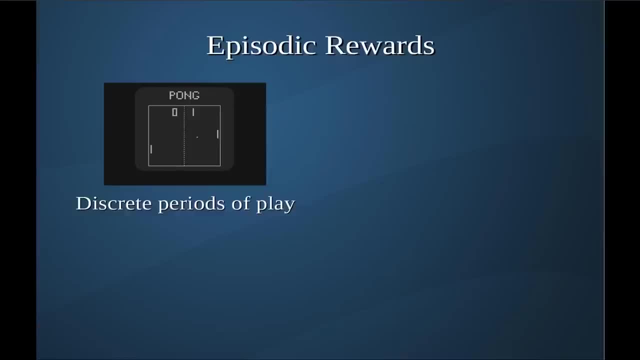 Of course, we can start over again with a new episode, but the agent takes no actions in this terminal step and thus no future rewards follow. In this case, we're dealing with not just individual rewards, but with the sequence of rewards over the course of that episode. 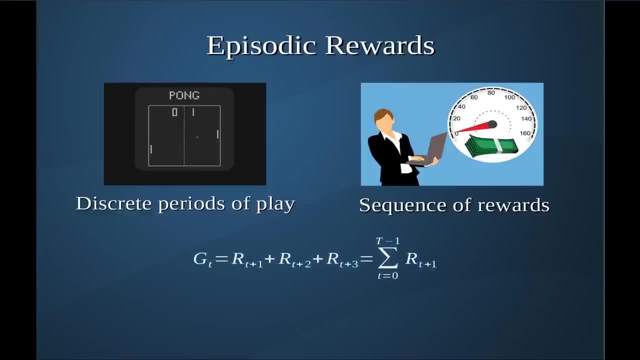 We call the cumulative reward the return, and it's usually denoted by the letter G. Now, this discussion is for games that are broken into episodes, but it would be nice if we could use the same mathematics for tasks that don't have a natural end, If we have a game that goes on and on. 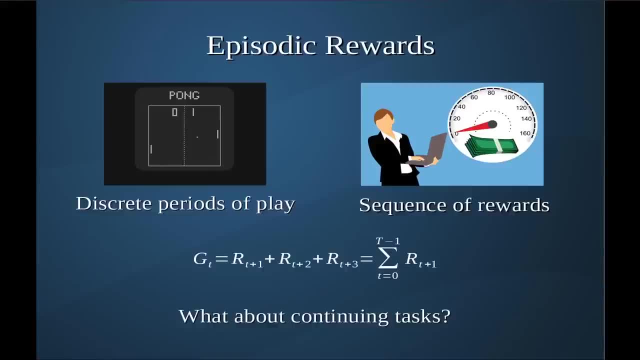 then the total sum of rewards will approach infinity. It's absurd to talk about maximizing total rewards in an environment where you can expect an infinite reward. so we have to do a little modification to our expression for the returns. We need to introduce the concept. 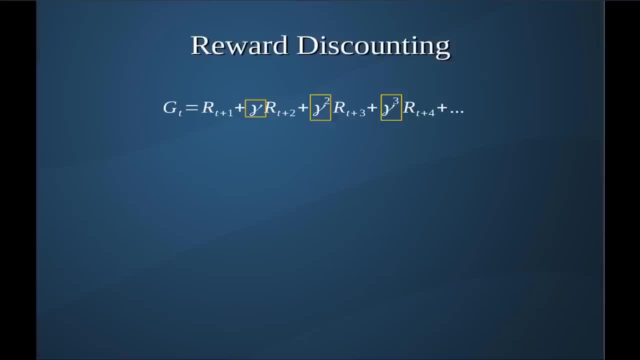 of counting. We're going to reduce the contribution of each reward to the sum based on how far away in time it is from our current time step. We're going to use a power law to describe this reduction so that the reward gets reduced by some additional power of a new hyperparameter we'll denote as gamma. 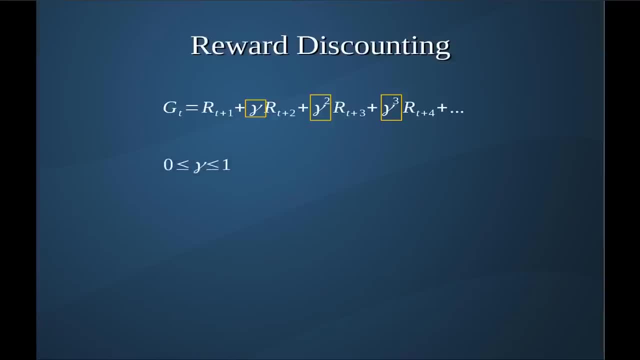 Gamma is between zero and one, so each time we increase the power the contribution is reduced. If we introduce gamma into the expression for the return at time, step T, we get that the return is just a sum over K of gamma to the K multiplied by the rewards at time T plus one plus K. 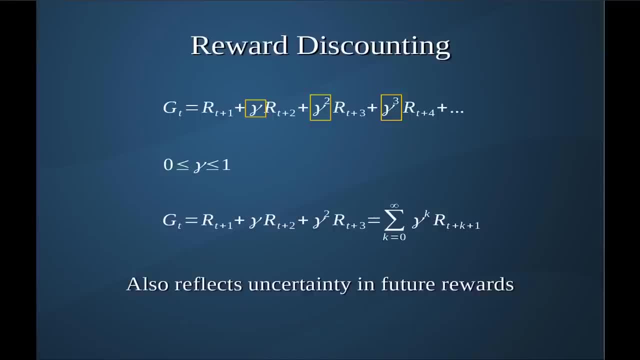 Besides being a trick to make sure we can use the same mathematics for episodic and continuing tasks, discounting has a reasonable basis in first principles. Since our state transitions are defined in terms of unknown probabilities, we can't really say how certain each of those rewards were. 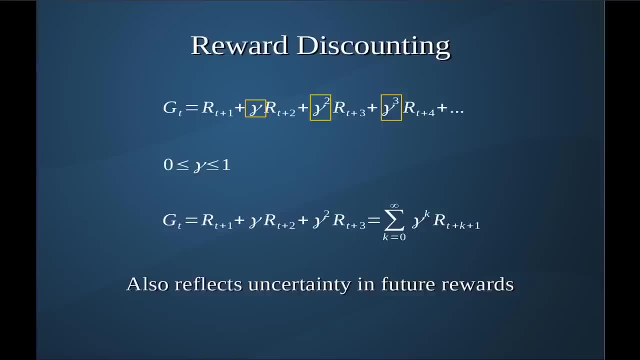 States that we encounter further out in time become less and less certain, and so the rewards for reaching those states are also less and less certain. Thus, we shouldn't weight them as much as the reward we just received. If you've been following along carefully, something may not quite add up here. 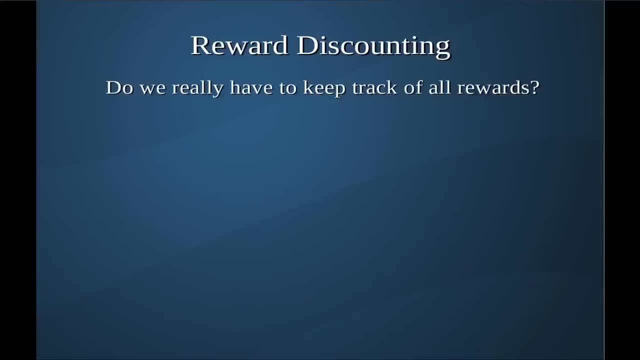 All of this math is for systems with the Markov property, which means that they depend only on the previous state in action. So why do we want to keep track of the entire history of rewards received? Well, it turns out that we don't have to. 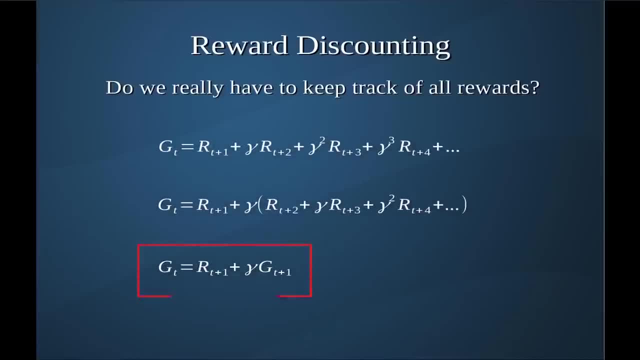 If you do some factoring in the expression for the return at time step T, you find that the return at time T is just the sum of the reward at time T plus one and the discounted return for the T plus one time step. This is a recursive relationship between returns at each time step. 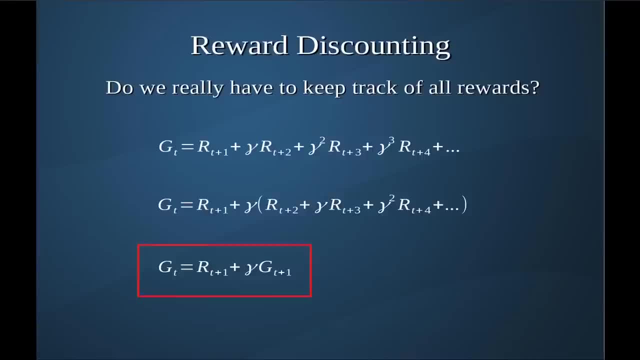 It's more consistent with the principles of the Markov decision process, where we're just concerned with successive time steps, Now that we know exactly what the agent wants, to maximize the total returns and then function for how it's going to act, the policy. 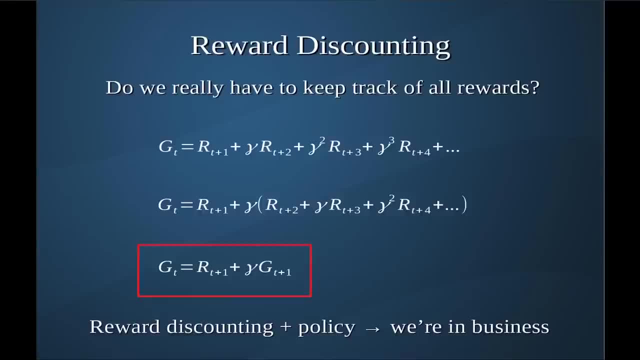 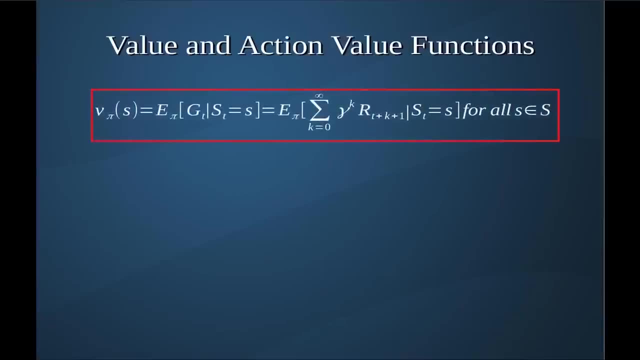 we can actually start to make useful mathematical predictions. One quantity of particular interest is called the value function. It depends on the agent's policy pi and the current state of the environment and gives us the expectation value of the agent's returns starting from time T and state S, assuming it follows the policy pi. 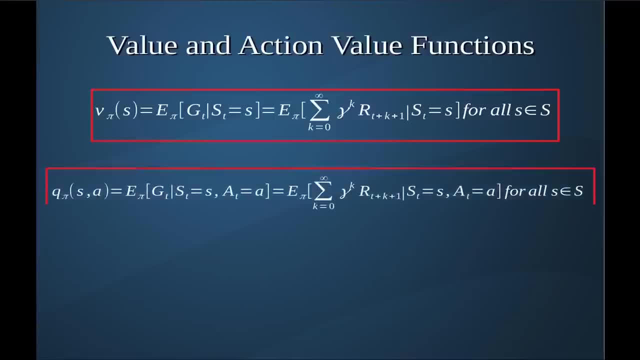 There's a comparable function for the value of state and action pairs which tells us the value of taking action A and state S and then following the policy pi afterwards. It's called the action value function and it's represented by the letter Q. 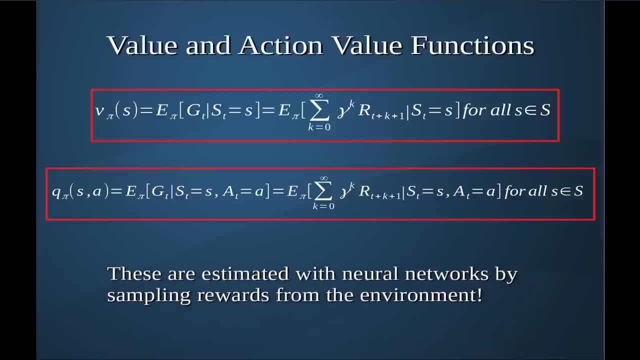 So how are these values calculated in practice? Well, in reality, we don't solve these equations, We estimate them. We can use neural networks to approximate the value or action value function, because neural networks are universal function approximators. We sample rewards from the environment and use those to update the weights. 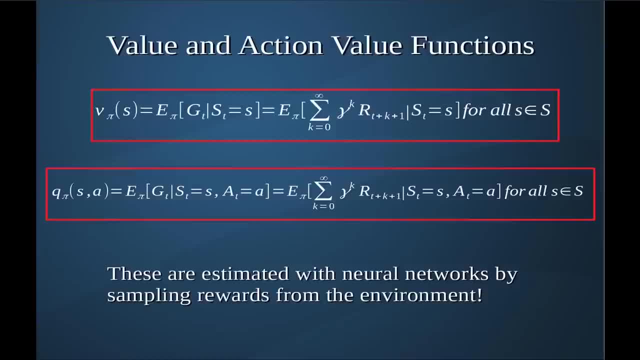 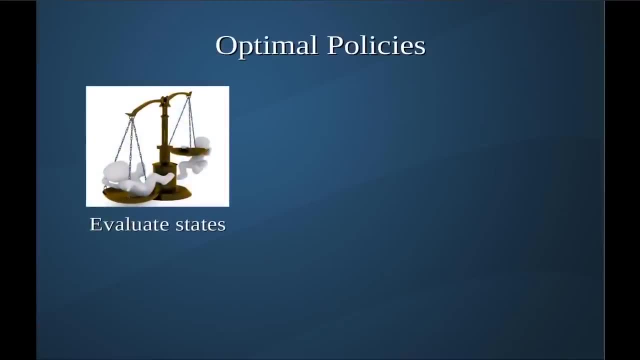 of our network to improve our estimate for the value or action value function. Estimating the value function is important because it tells us the value of the current state and the value of any other state the agent may encounter. Solving the reinforcement learning problem then becomes an issue of constructing a policy that allows the agent to seek out. 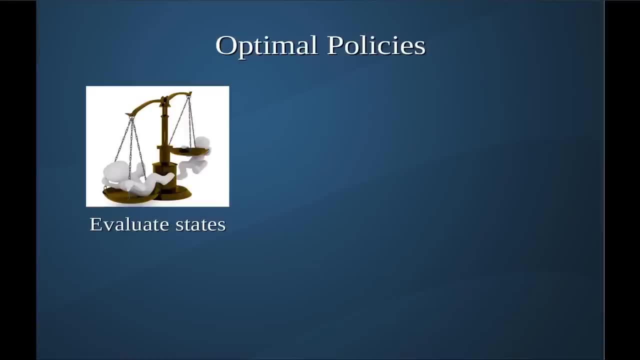 the most profitable state. The policy that yields the best value function for all states in the state space is called the optimal policy. In reality, it can be a set of policies and they're all effectively equivalent. Various schemes to find these optimal policies exist. 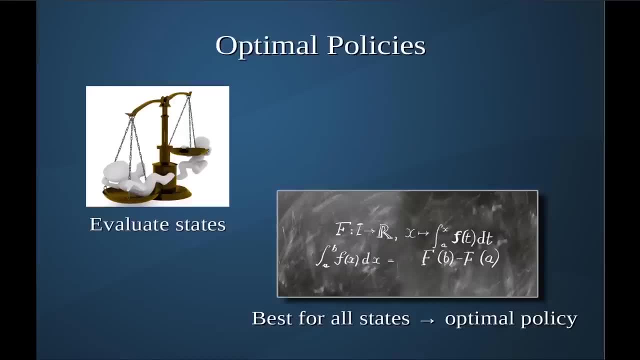 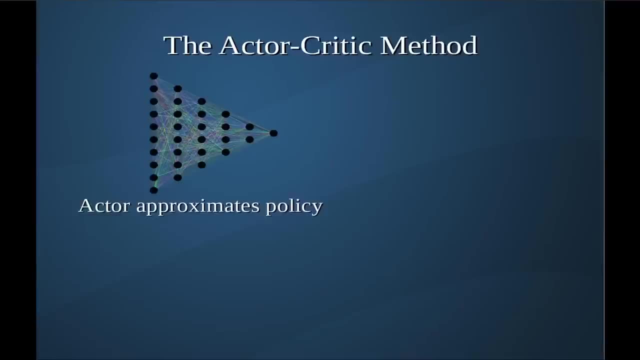 and one such scheme is called the actor critic method. In actor critic methods, we're using two deep neural networks. One of them is used to approximate the agent's policy directly, which we can do because it's just a mathematical function. Recall that the policy is just a probability. 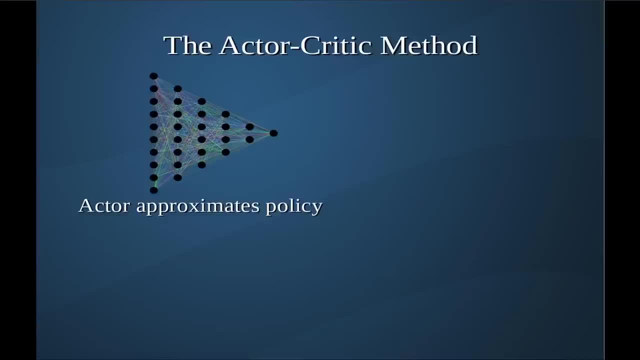 distribution over the set of actions, where we take a state as input and output a probability of selecting each action. The other network, called the critic, is used to approximate the value function. The critic acts just like any other critic, telling the actor how good each. 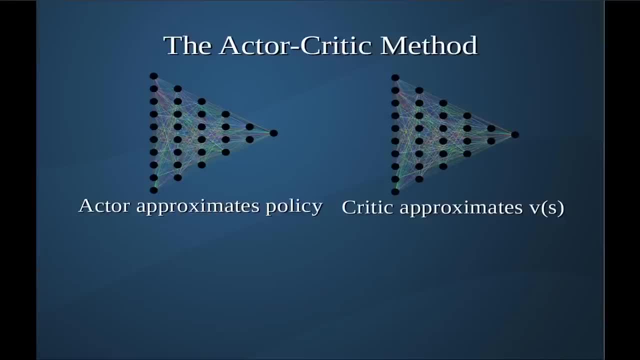 action is based on whether or not the resulting state is valuable. The two networks work together to find out how best to act in the environment. The actor selects actions, the critic evaluates the states and then the result is compared to the rewards from the environment. 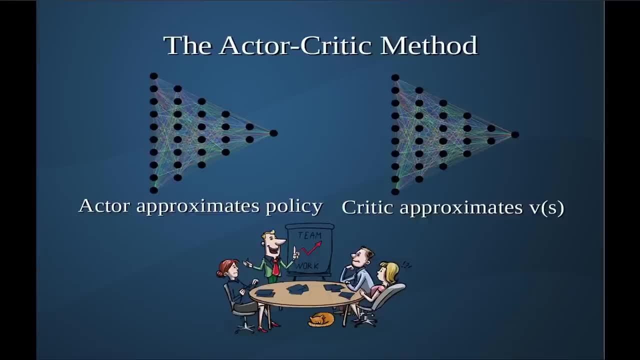 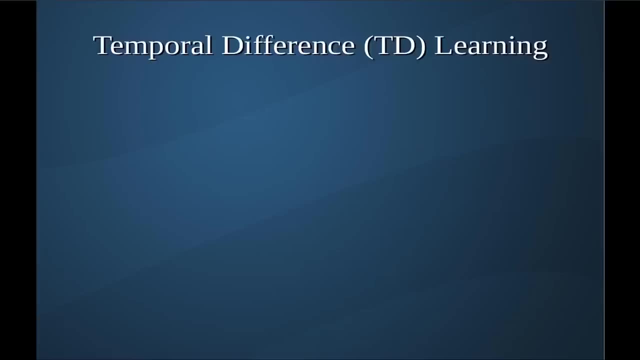 Over time, the critic becomes more accurate at estimating the values of states, which allows the actor to select the actions that lead to those states. From a practical perspective, we're going to be updating the weights of our deep neural network at each time step, because actor critic methods belong to a class of algorithms called 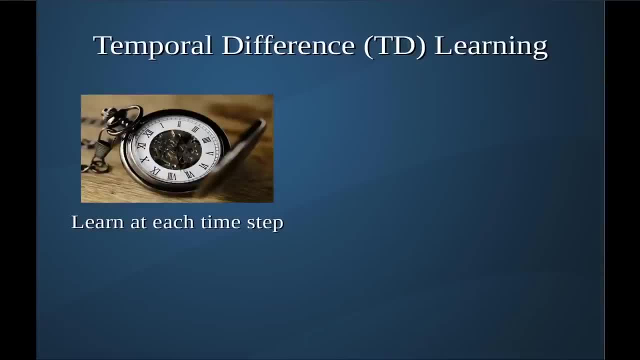 temporal difference learning. This is just a fancy way of saying that. we're going to be estimating the difference in values of successive states, meaning states that are one time step apart, hence temporal difference. Just like with any deep learning problem, we're going to be calculating cost functions. 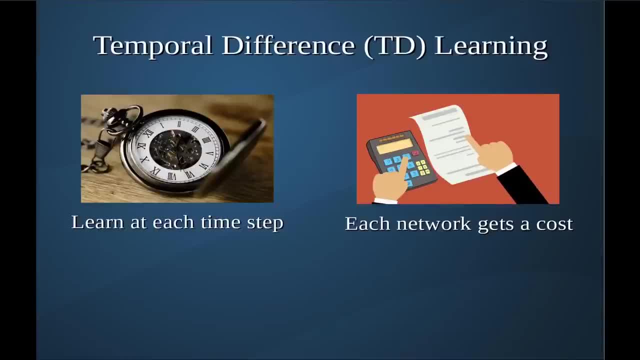 In particular, we're going to have two cost functions: one for updating our critic and the other for updating our actor. To calculate our costs, we want to generate a quantity we'll call delta, and it's just given by the sum of the current reward and the discounted estimate of the new state, and then 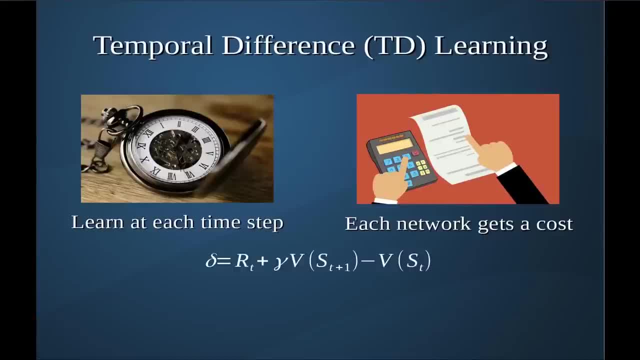 subtracting off the value of the current state. Keep in mind that the value of the terminal state is identically zero, so we need a way to take this into account. The cost for the critic is going to be delta squared, which is kind of like a typical linear regression problem. 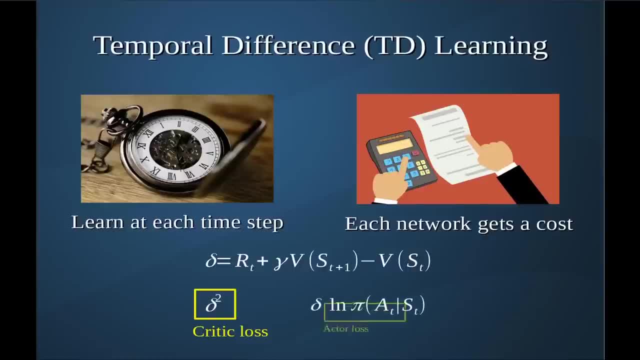 The cost for our actor is a little more complex. We're going to multiply this delta by the log of the policy for the current state and action the agent took. The reason behind this is a little complex and it's something I go into more detail. 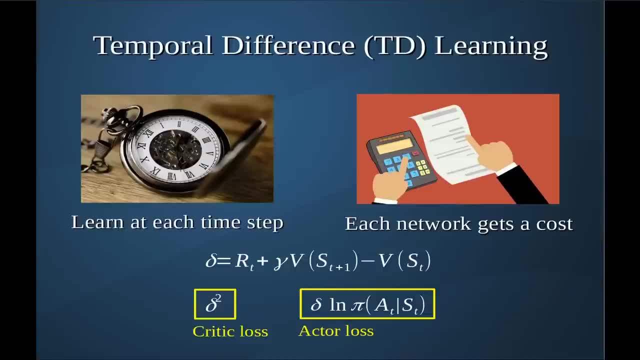 about in my course or you can look for it in the chapter on policy gradient methods in the free textbook by Sutton and Bardo. So let's talk implementation details. We're going to implement the following algorithm: Initialize a deep neural network to model the actor and critic. 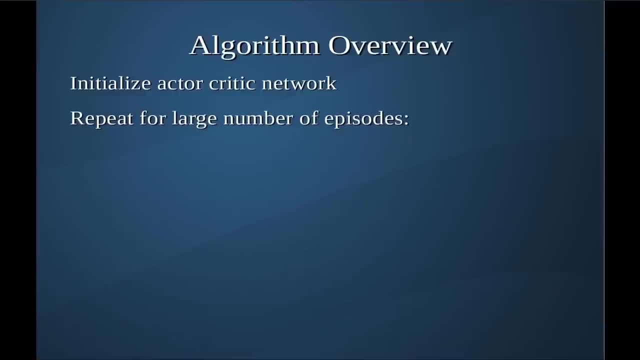 Repeat for a large number of episodes. Reset the score. terminal flag and environment. While the state is not terminal, select an action based on the current state of the environment, Take the action and receive the new state reward and terminal flag from the environment. 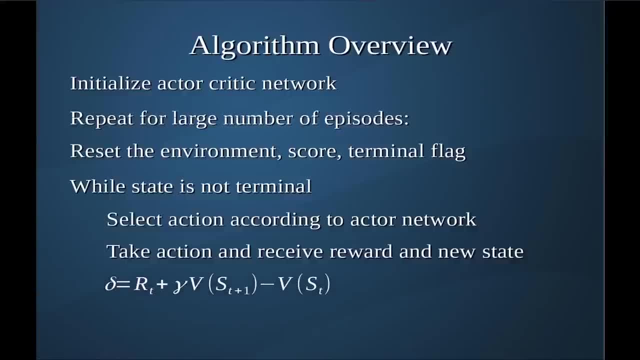 Calculate delta and use it to update the actor and critic networks, Set the current state to the new state and increment the episode reward by the score. After all the episodes have finished, plot the trend in scores to look for evidence of learning. This should be an overall increase in score over time. 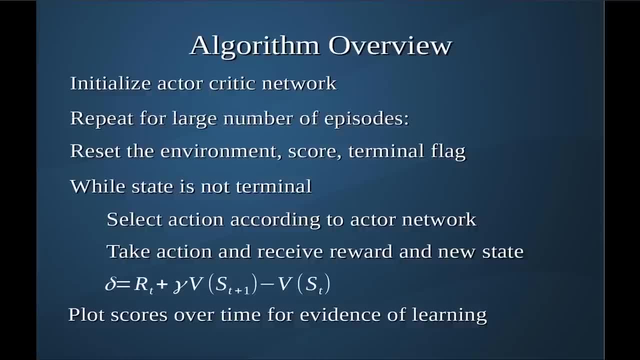 You will see lots of oscillations because actor-critic methods aren't really stable, but the overall trend should be upward. Another thing you may see is that the score can go upward for a while and then fall off a cliff. This isn't uncommon because actor-critic methods are quite brittle and they're 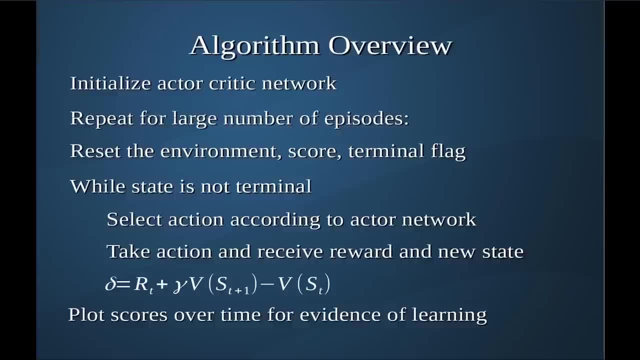 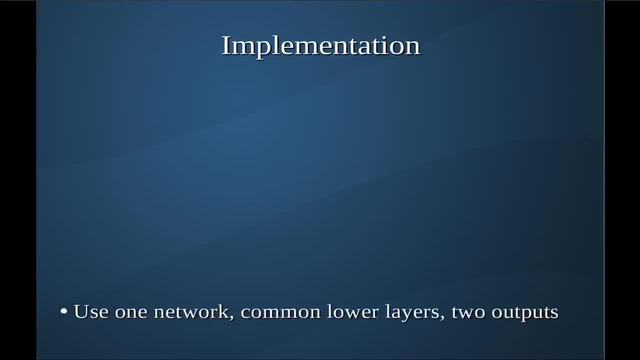 really not the best solution for all cases, but they are a stepping stone to more advanced algorithms. Other important implementation details: You can use a single network for both the actor and critic, So you have common input layers and two different outputs, one for the actor and one for the critic. 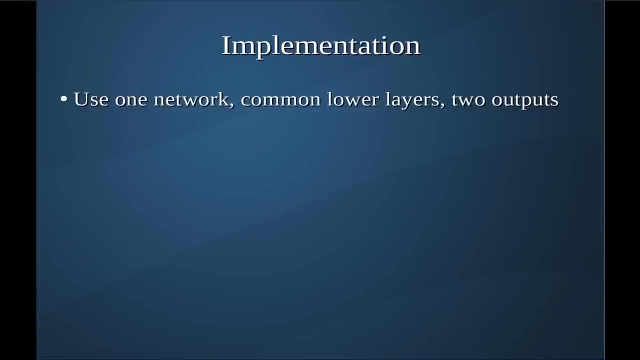 This has the benefit that we don't have to train two different networks to understand the environment. You can definitely use an independent actor and critic. It just makes the learning more difficult for an algorithm that is already pretty finicky. We'll let it play almost 2000 games with a relatively large deep neural network. 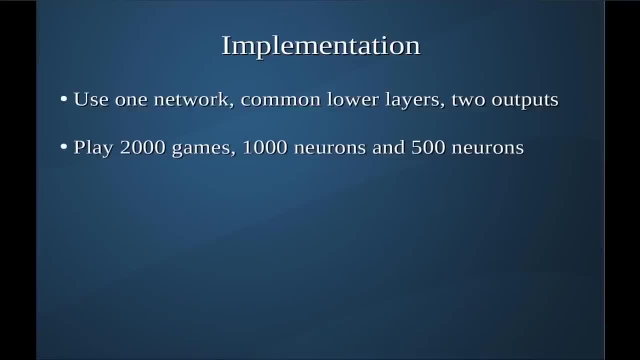 something like about 1000 units in the first hidden layer and 500 units in the second. The hard part is going to be the actor. As I said earlier, the actor models the policy, which is a probability distribution. The actor layer will have as many outputs as our actions and we use a softmax. 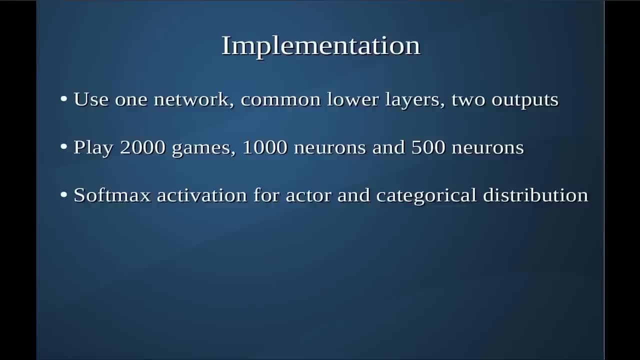 activation, because we're modeling probabilities and they had better sum to one When selecting actions. we're going to be dealing with discrete action spaces, So this is what is called a categorical distribution. We're going to want to use the TensorFlow underscore probability package for the categorical distribution and then use 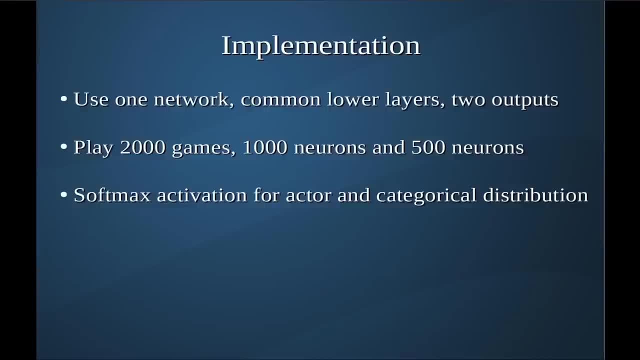 the probabilities generated by the actor layer to get this distribution which we can then sample and use the built log prob function for our cost function. As far as the structure of our code, we're going to have a class for our actor critic network and that will live in its own file. 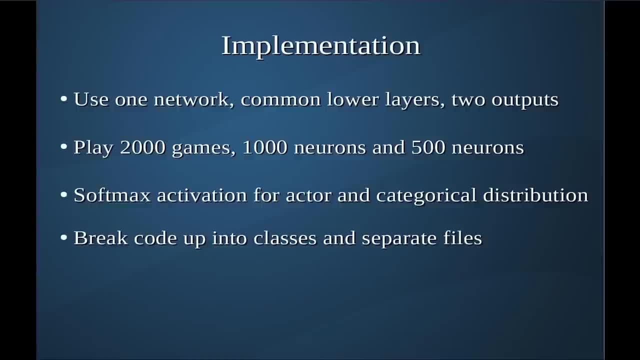 We'll also have a class for our agent and that will have the functionality to choose actions, save models and learn from its experience. That goes in a separate file. The main loop is pretty straightforward, but it does go in its own file as well. 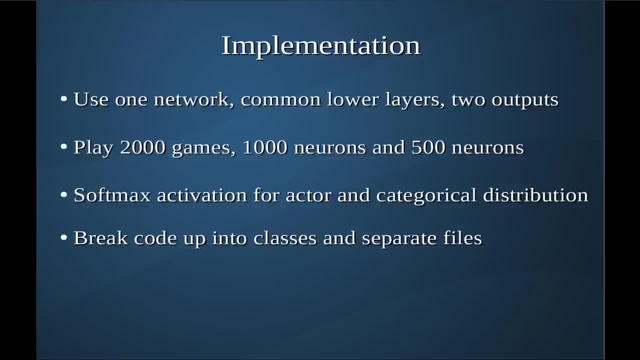 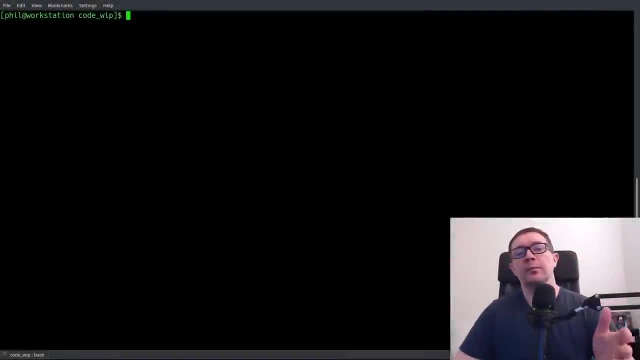 OK, now that we have all the details out of the way, let's go ahead and get started coding this. So, now that we have all of our lectures out of the way, we're going to go ahead and proceed with the coding. We're going to start with the networks. 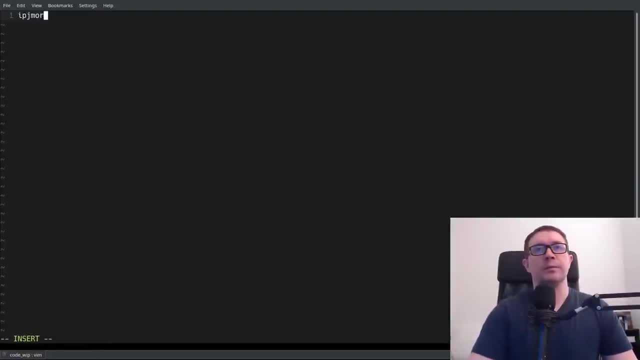 We begin, as always, with our imports. So we will need OS to handle file joining operations for model checkpointing, We will need Keras And we will need our layers, Which, for this example, is just going to be a dense layer. 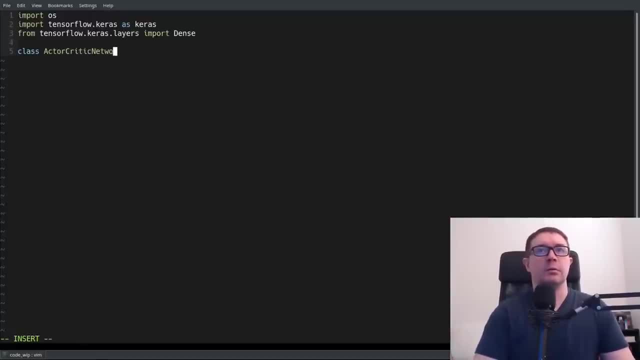 So we will have our actor critic network And you see a case of converging engineering here where TensorFlow and PyTorch both have you derive your model class from the base model class and we can go ahead and define our constructor. That will take a number of actions. 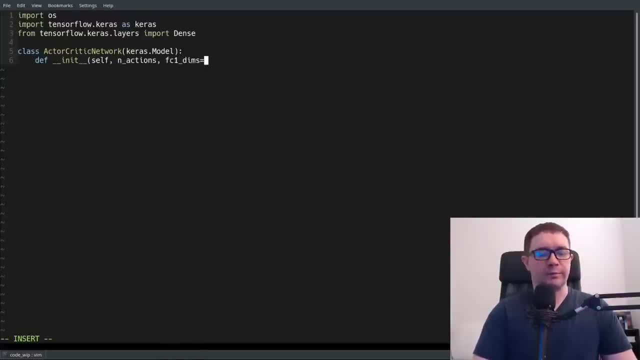 as input the number of dimensions. for the first fully connected layer, We will default that to 1024 and for the second, we will default it to 512. We will have a name for model checkpointing purposes and a checkpoint directory- Very important. 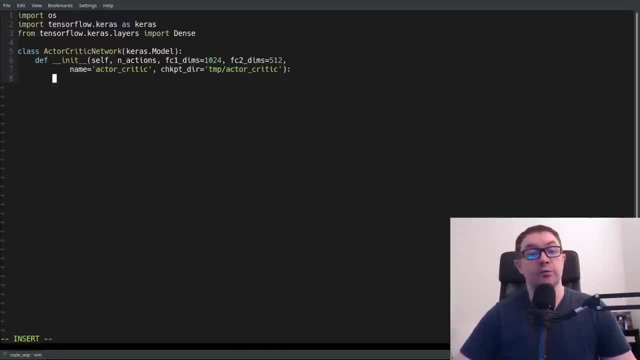 You must remember to do a make directory on this temp slash actor critic before you attempt to save a model, Otherwise you're going to get an error. The first thing you want to do is call your super constructor And then go ahead and start saving your parameters. 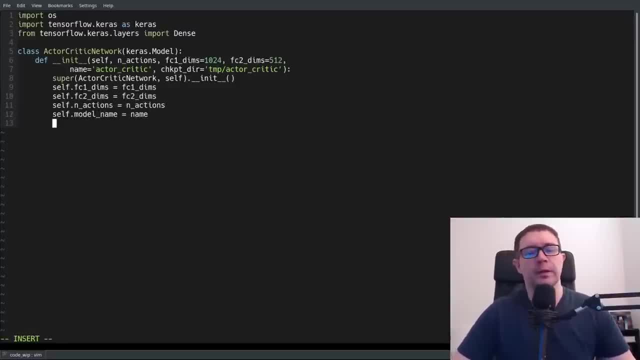 Now, also very important for our class- that we've derived from the base class. In this case, we're going to be using a class that we've derived from the base class. So we're going to be using a class that we've derived from the base class. 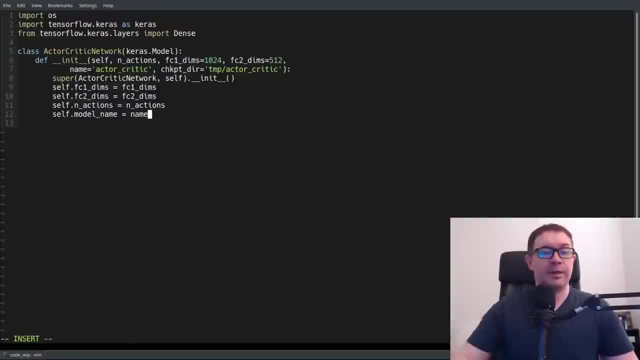 So we're going to be using a class that we've derived from the base class, So we have to use model name instead of name, because name is reserved by the base class. So just be aware of that, Not a huge deal. Checkpoint directory. 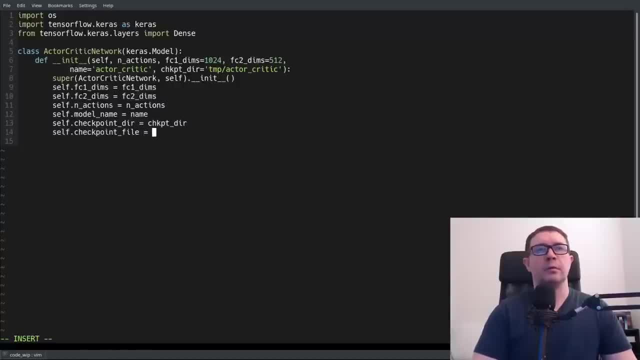 And then we'll have our file And that will be OS path. join the directory name plus underscore. Hey see, I like to use underscore algorithm, in this case AC for actor critic, in case you have one directory that you use for many different algorithms. 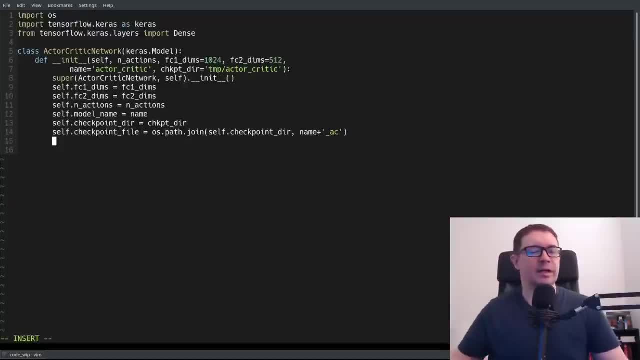 If you're just using, like, say, a working directory, you don't want to confuse the model types. Otherwise, if you have a good model saved, you don't want to override it with something else. Now we'll go ahead and define our layers. 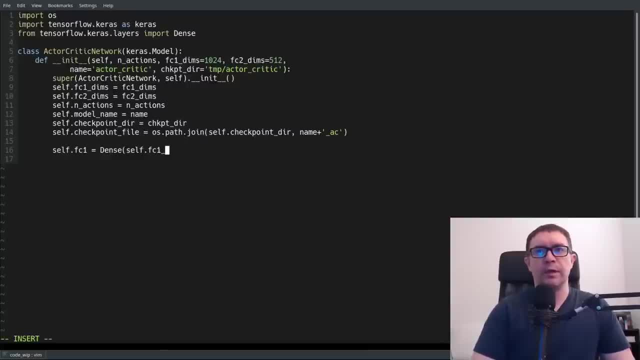 And that will be fully connected dense layers. The neat thing about Keras is that the number of input dimensions are inferred, so we don't have to specify it. That's why we don't have an input dims for our constructor, And it will output FC1 dims with an activation of value. 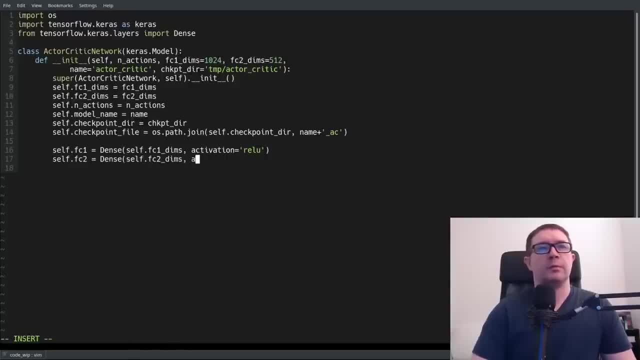 FC2 will be similar And then we will have two separate outputs. So we have two common layers and then two independent outputs: One for the value function And that is single valued with no activation, And the second is our policy pi And that will output an actions with a softmax activation. 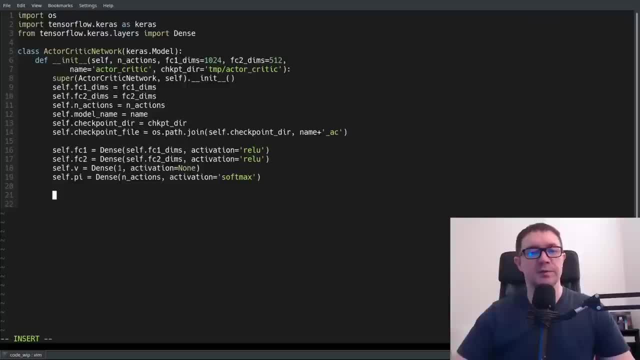 Recall that the policy is just a probability distribution, So it assigns a probability to each action And those probabilities have to add up to one, because that's kind of what probabilities do, right. Next we have to define our call function. This is really the feed forward. 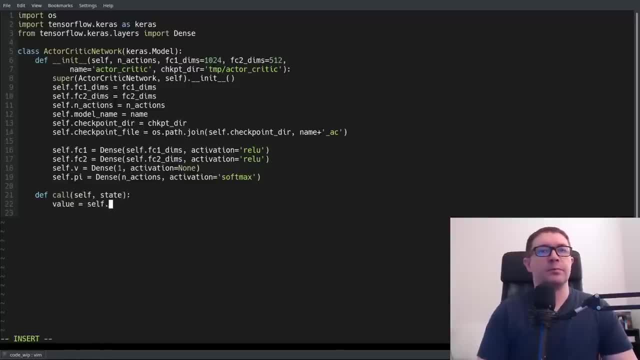 If you're familiar with that from PyTorch. So we'll just use some generic name like value- doesn't really matter- and pass it to the second fully connected layer and then get our value function and our policy pi And then return both the value function and the policy pi. 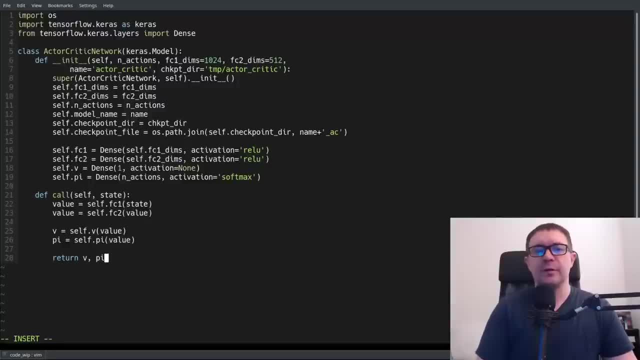 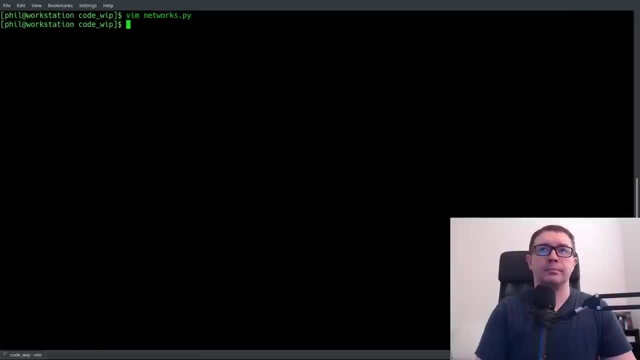 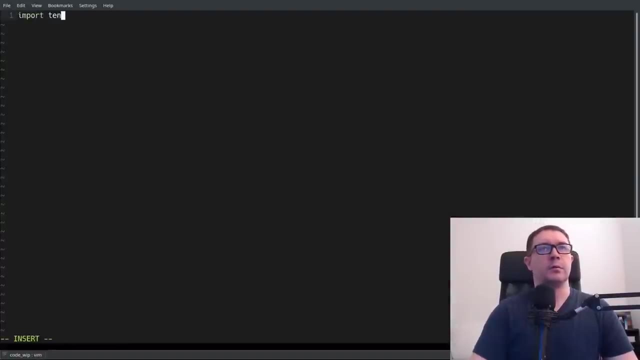 So that is really it for the actor critic. So let's go ahead and start writing the agent class. So let's go ahead and start writing the agent class. So we begin, as always, with our imports. We will need tensorflow, We will need our optimizers. 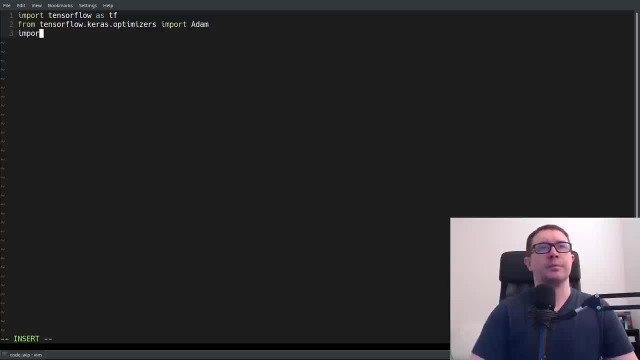 In this case we're going to use an atom optimizer. So we're going to use an atom optimizer. So we're going to use an atom optimizer. We will need tensorflow probability to handle our categorical distribution, to model our policy directly. You have to do a pip, install tensorflow probability before you can run this. 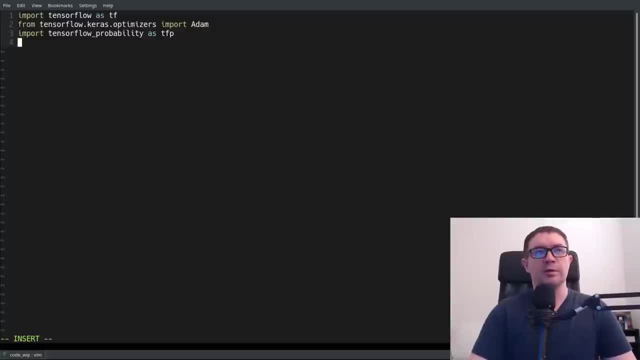 This is a separate package from tensorflow And we will also need our actor critic network. Let's go ahead and code up our agent. So our initialized agent class is going to be our agent class. So our initialized agent class is going to be our agent class. 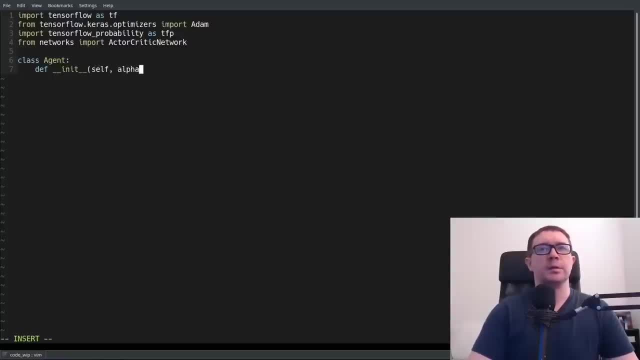 So our initialized agent class is going to be our agent class. We will need some default learning rate. I'm going to use 0003.. It doesn't really matter, I'm going to pass in a specific learning rate in the main file. 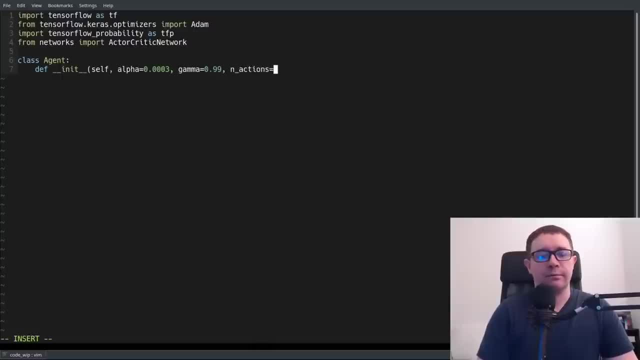 We will have a gamma of 0.99 and default inactions of some number, like say 2.. So we're going to go ahead and save our parameters. Recall that gamma is our discount factor. We're going to need a value of 0.99.. 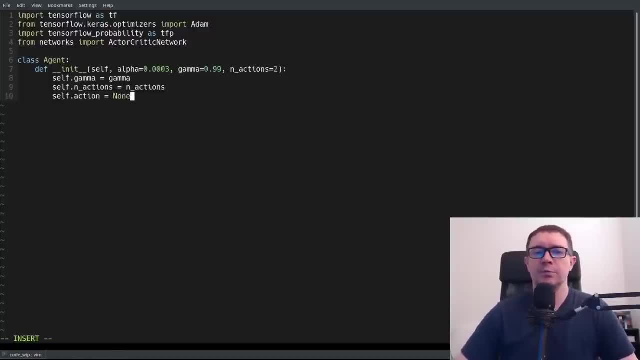 We're going to need a variable to keep track of the last action we took. This will be a little bit more clear when we get to the learn function. It has to do with the way we calculate the loss, because we have to use a gradient tape for tensorflow2.. 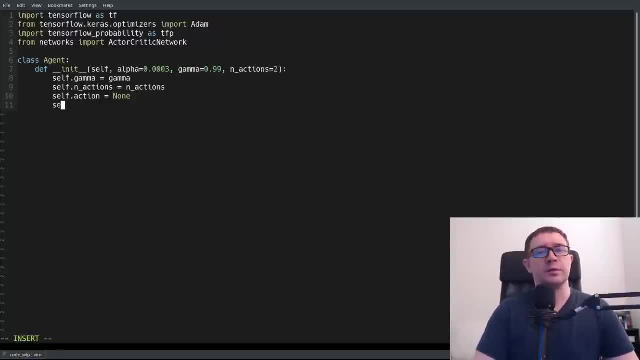 It's just a bit of a workaround for how tensorflow2 does things. We need our action space for random action selection. That's just a list of actions from 0 to an actions minus 1.. We need our actor critic. We want to make sure to specify the number of actions and we want to compile 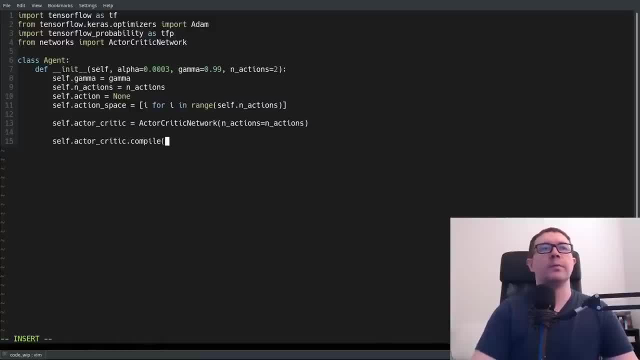 that model. so actor critic, compile with an atom optimizer and learning rate defined by alpha. Next, we have the most basic functionality of our agent, the functionality to choose an action, And that takes the current state of the environment as input, which we have to convert to a tensor. 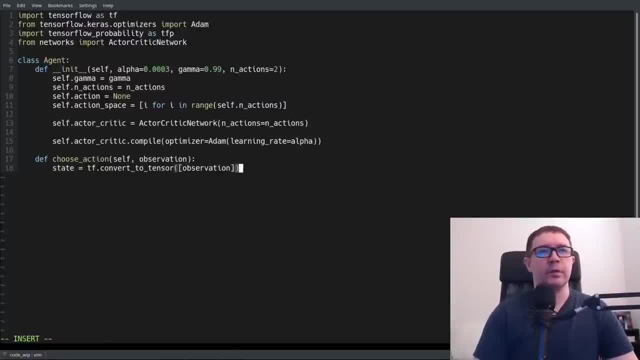 And, in particular, we have to add an extra dimension, a batch dimension, The reason being that the deep neural network expects a batch of inputs, And so you have to have something other than a 1D array that's two dimensional. So we just add an extra dimension along. 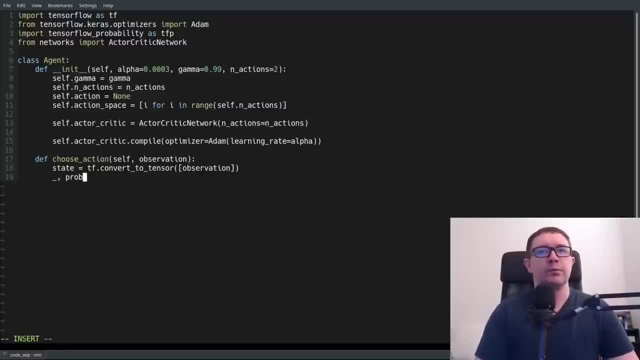 the 0th dimension. So then we will feed that through our deep neural network. We don't care about the value of the state for the purpose of choosing that action, So we just use a blank and we will get the probabilities by passing the state through the actor critic network. 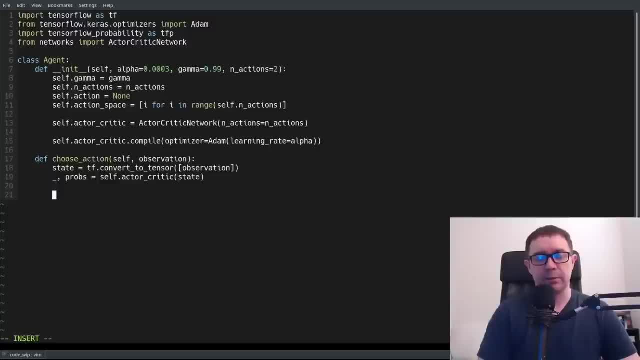 And then we can use that output, the probabilities defined by our neural network, to feed into the actual tensorflow probabilities, categorical distribution, and then use that to select an action, sampling that distribution and getting a log probability of selecting that sample. Sorry, that's TFP. 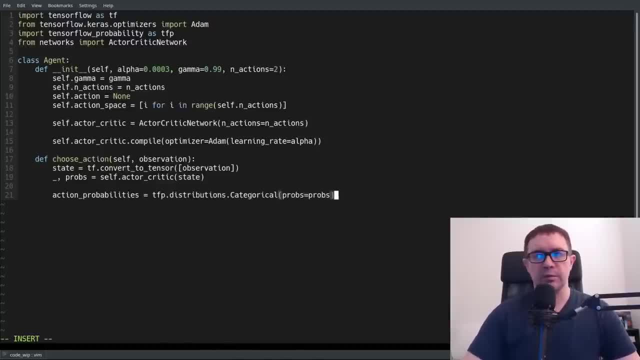 Categorical, and probabilities given by problems and our actual action will be a sample of that distribution And we don't actually need the log prob at this stage. We will need the log problem- We calculate the loss function for our deep neural network, but we don't need it now. 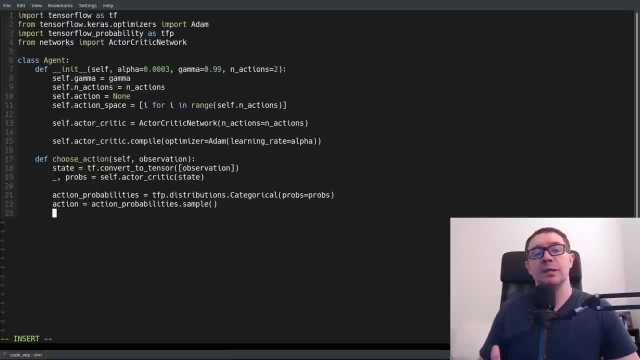 And it doesn't make sense, or rather it doesn't actually work, to save it to a list, let's say for use later here, because this calculation takes place outside of the gradient tape. TensorFlow 2 has this construct of the gradient tape. It's pretty cool. 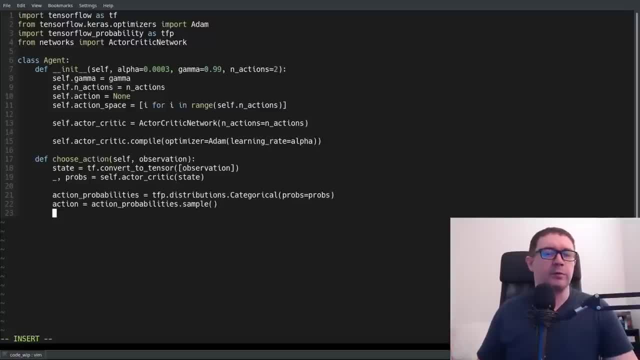 It allows you to calculate gradients manually, which is really what we want to do here. Uh, but anything outside of that tape doesn't get added to the calculation for back propagation, So the log prop doesn't matter at this point, So why bother calculating it? 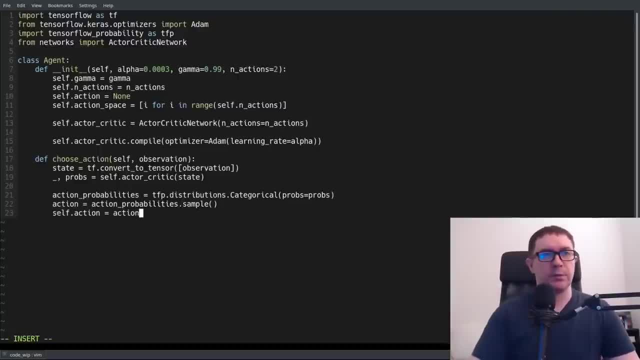 One thing we do need, however, is the action that we selected, So we will save that in the action variable and we will return a NumPy version of our action, because action is a TensorFlow tensor which is incompatible with the OpenAI Jim. 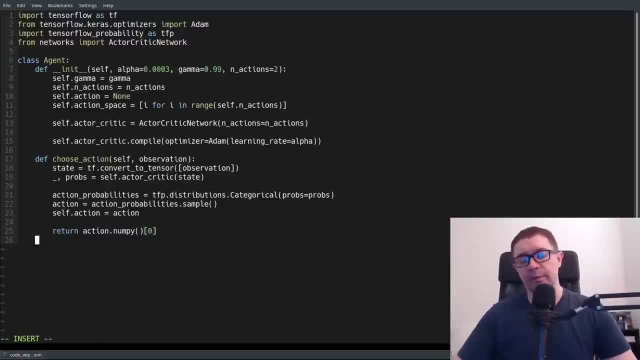 It does, however, take NumPy arrays and we want the zero element of that because we added in a bash dimension for compatibility with our deep neural network and a little bit confusing, but that is what we have to deal with. Next. let's do a couple of bookkeeping functions to save and load models. 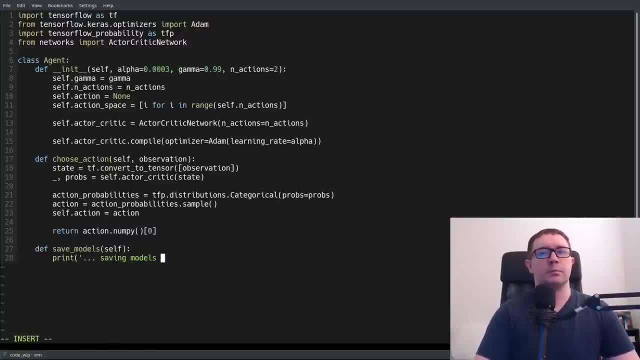 Those will take any inputs And so it will save the weights of the network to the checkpoint file. We do the inverse operation, to load models, And we will load weights from a checkpoint file. So that is it for the Basic bookkeeping operations. 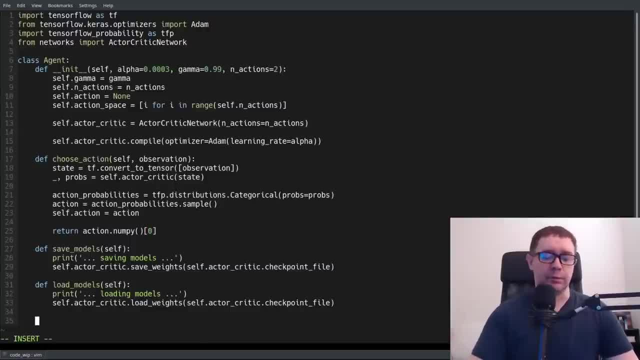 Next we have the real heart of the problem, the functionality to learn. So this will take a number of inputs. We'll take the state reward received new state and terminal flag as input. The first thing we want to do is convert each of those to TensorFlow tensors. 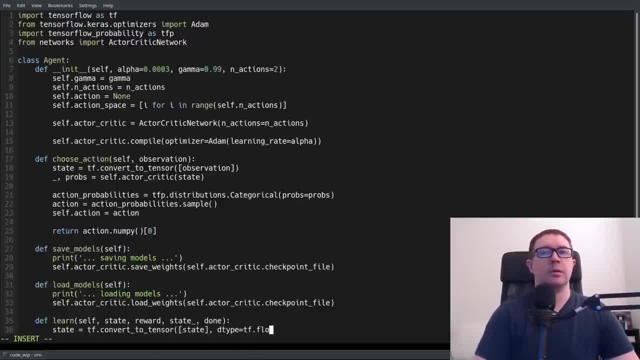 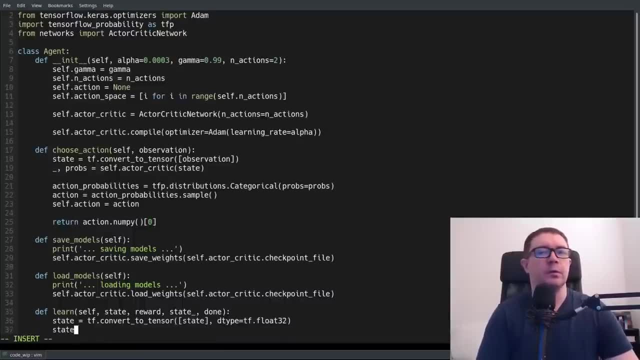 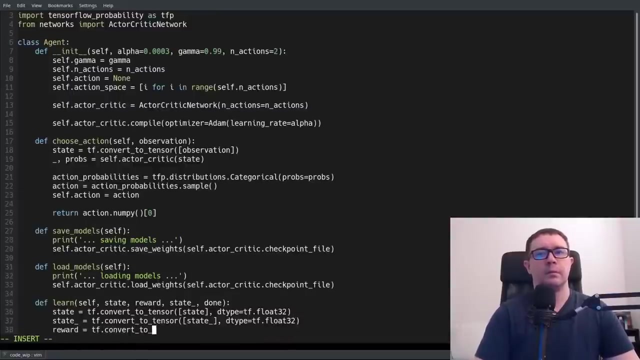 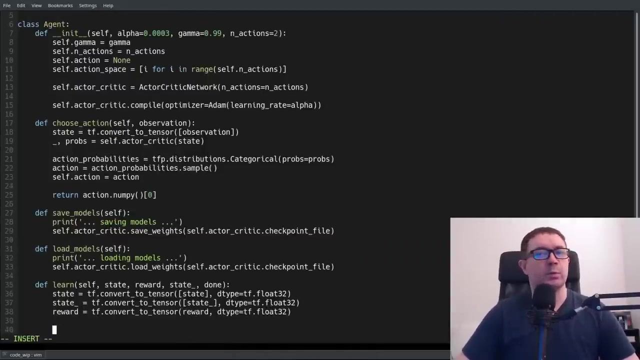 And make sure to add a batch dimension, And I like to be Really pedantic with my data type, so I will cast it to TF, float 32.. And we don't have to add a batch dimension to the reward, because it is not. 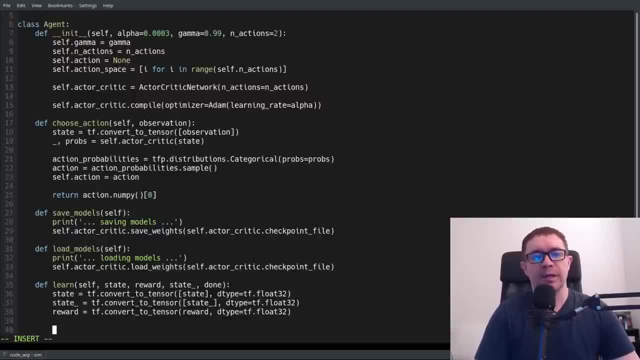 fed to a deep neural network. So now we get to calculate our actual gradients using something called the gradient tape And we'll set Persistent to true. I'm not actually sure that's needed. I'm going to go ahead and experiment with that when we go ahead and run the code. 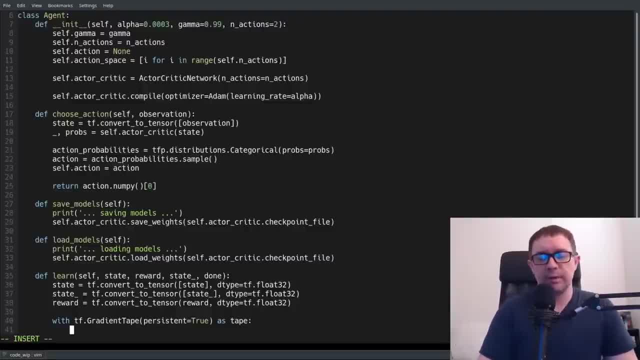 but I have it that way. I might have just copied and pasted code from somewhere else, So let me double check. But we want to feed our state and new state through the actor critic network and get back our quantities of interest. So we feed the current state and then the new state. 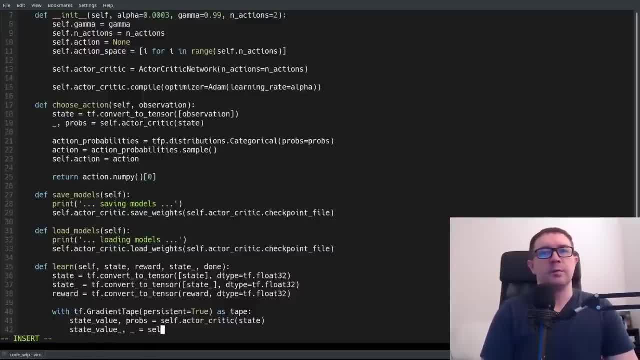 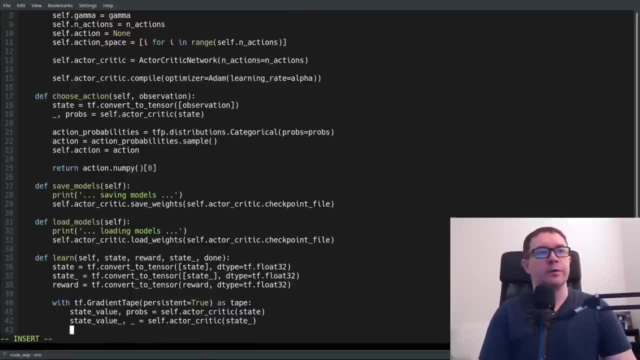 But for the new state we don't care about the probabilities, We just care about the value, And that is for calculation of our delta. But for the calculation of our loss we have to get rid of that batch dimension. So we have to squeeze these two parameters. 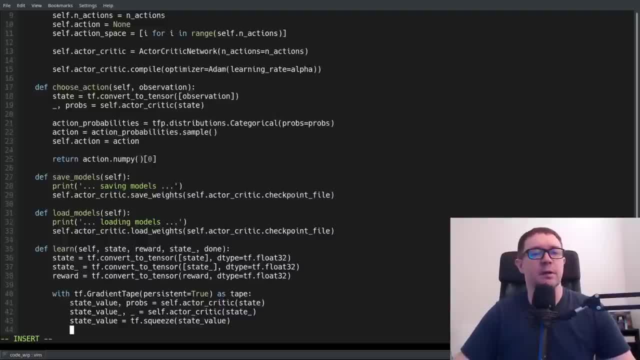 And the reason you have to do that is because the loss works best if it's on a one dimensional quantity, or rather a scalar value rather than a scalar value inside of brackets. So it has to be a scalar instead of a vector containing a single item. 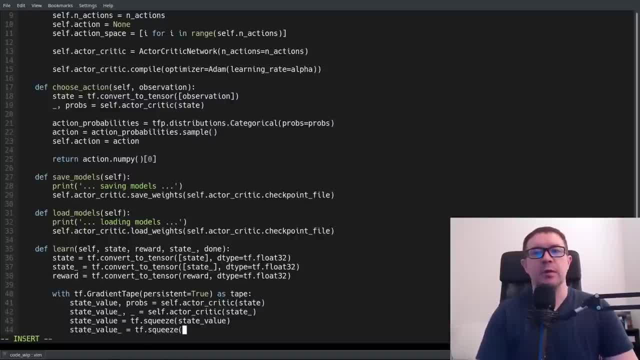 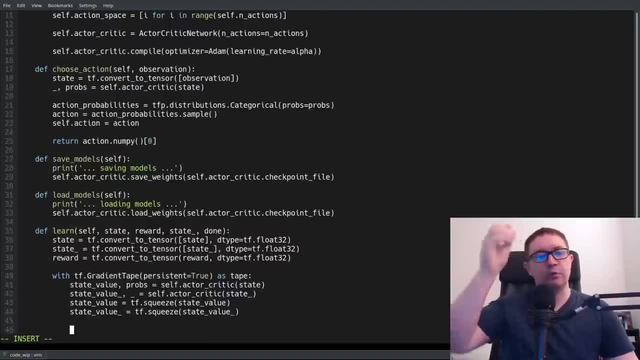 It's just something we have to do. I encourage you to play around with it to double check me on that. I move between. I move between distributions, excuse me- framework. So sometimes stuff isn't always 100 percent necessary, even if it doesn't hurt anything. 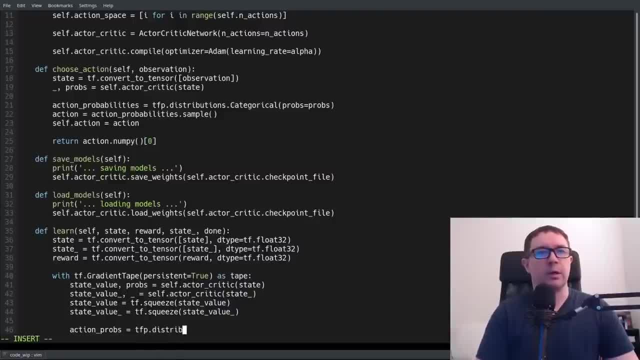 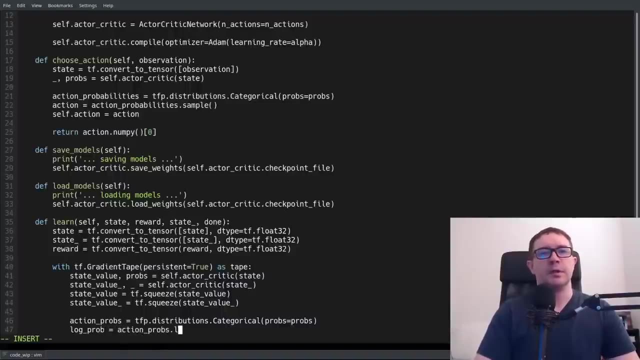 So we need our action probabilities for the calculation of the log prob, TFP distributions, categorical, And we define our probes by the output of our deep neural network. And then our log prob is action probes, log prob of the self action, And this is the action that we saved up. 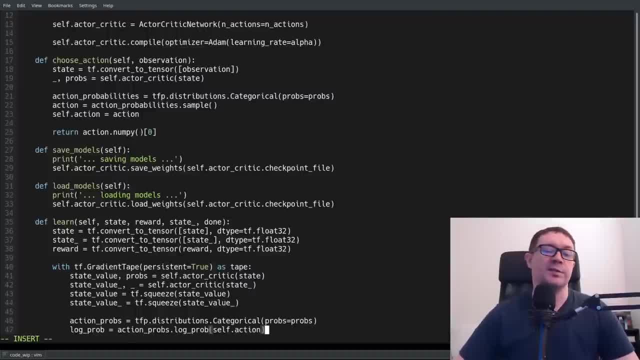 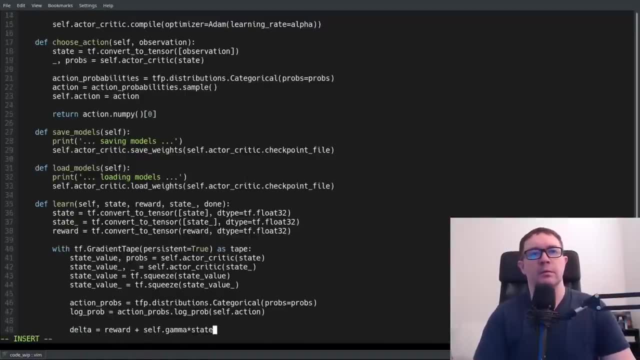 at the top when we calculate the action for the agent, So this is the most recent action. Then we calculate our delta, That is a reward plus gamma multiplied by the value of the new state, times One minus int of done. And the reason for that is that the value of the terminal state is identically zero. 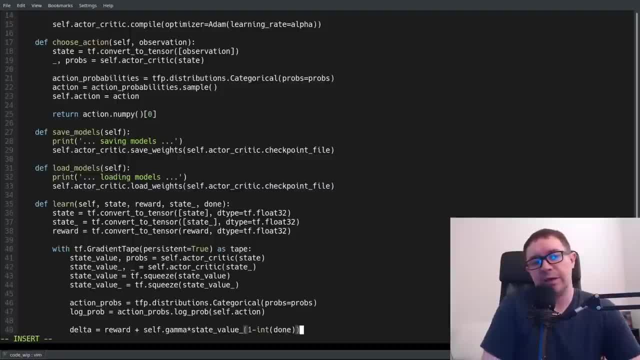 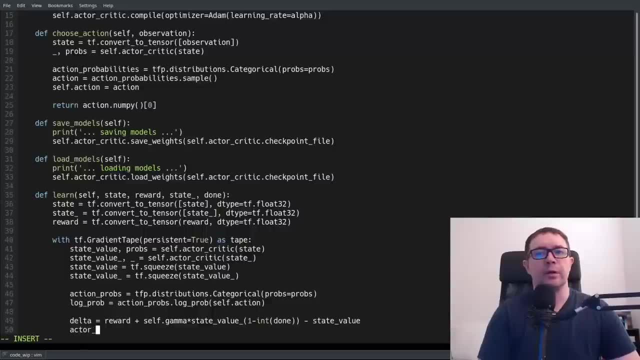 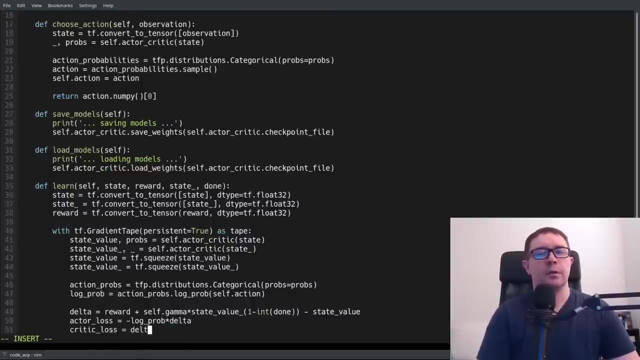 because no returns, no rewards follow the terminal state. So it has no future value And subtract off the state value. So our actor loss is minus log prob times that delta And the critic loss is delta squared And the total loss equals after loss. 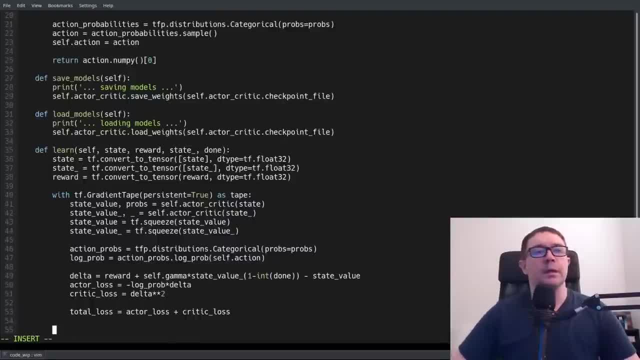 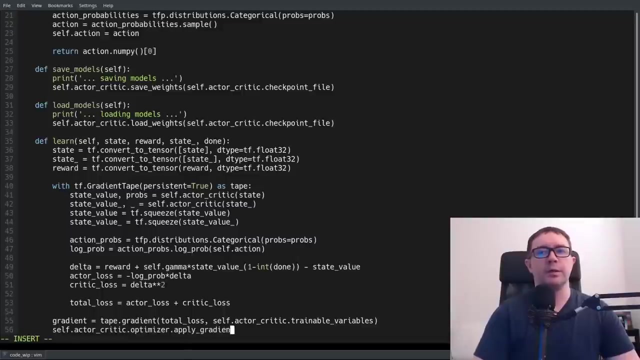 Plus critic loss, And then we can go ahead and calculate our gradients. So our gradient is taped out, gradient total loss with respect to the trainable variables. Optimizer apply gradients and this expects a zip as input. So we're going to zip the gradient. 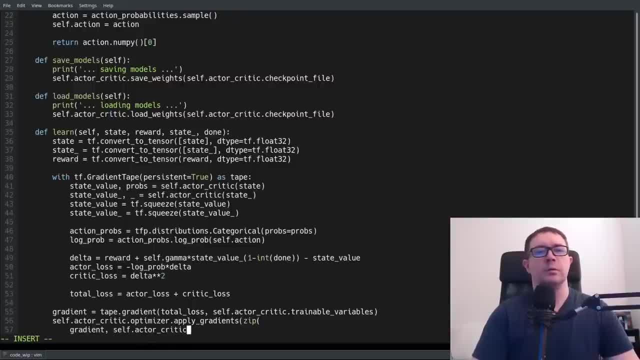 And the trainable variables. All right, And that is it for the actor critic functionality. So I'm going to come back to this in a few minutes to see if I need that persistent. I don't believe I do. I believe I need this in the case when we have 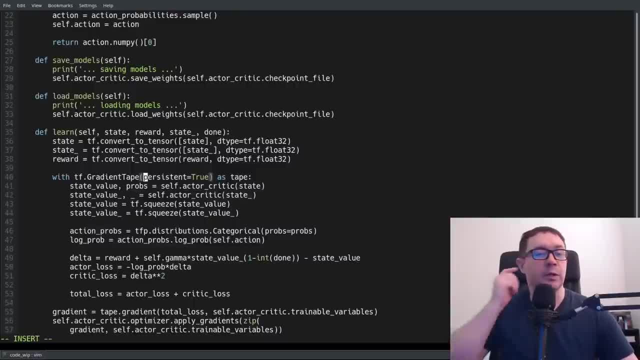 if we were to have, say, separate actor and critic networks and had to calculate gradients with respect to two separate sets of trainable variables. I believe that's when the persistent equals true would be necessary And when we had coupling between the loss of one network and the other. 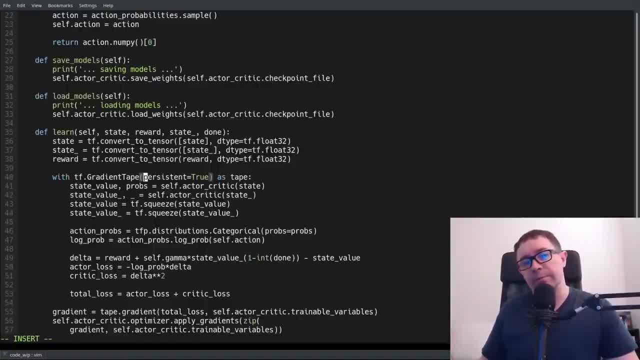 so that it keeps track of the gradients after it does the back propagation, kind of like in PyTorch, where it throws it away and you have to tell it to retain the graph. I'll double check on that, though. So let's go ahead and write and quit. 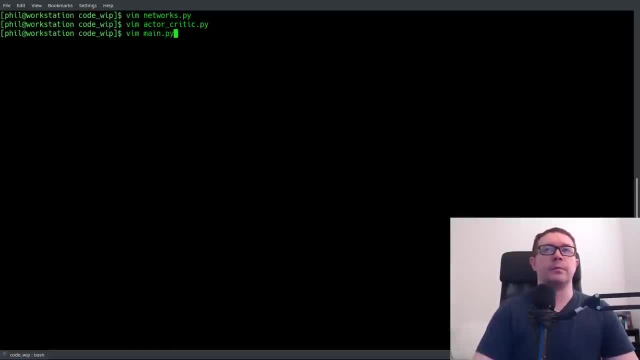 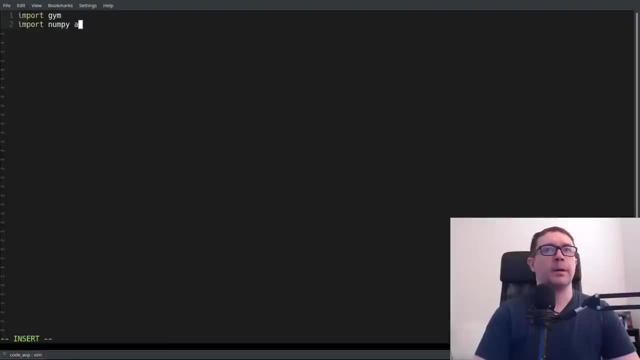 And then we're ready to go ahead and code up our main file. So, with our imports, we will need Jim, we will need NumPy, We will need our agent, We will need our plot learning curve function. I'm not going to go into any detail on this. 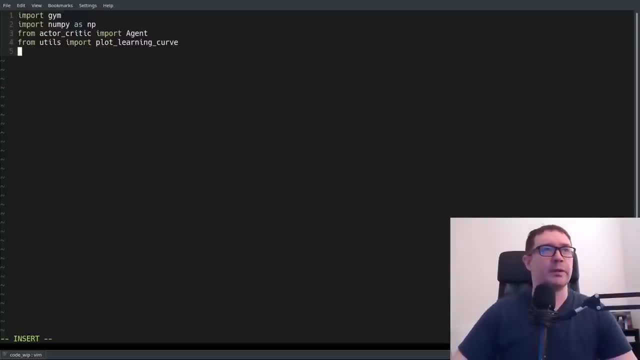 It's just a function to plot data using plot live with some labeled axes. It's nothing really worth going into. First thing we'll do is make Our environment- And I'm using the cart pull because it runs very quickly and the actor critic. 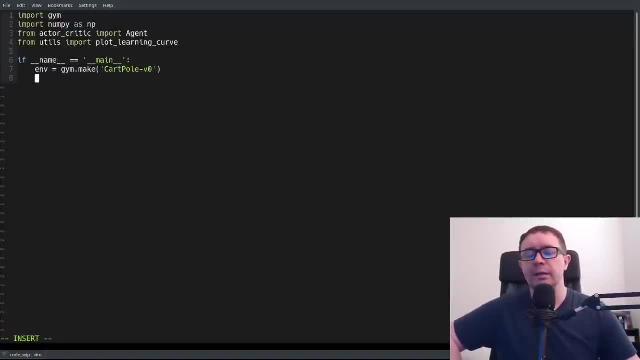 method is quite brittle, quite finicky, you will observe, in many cases where it will achieve a pretty decent score than a fall off a cliff, because the learning rate was just a little bit too high. so there are a number of problems of the algorithm and it's easiest to test in a very simple environment. 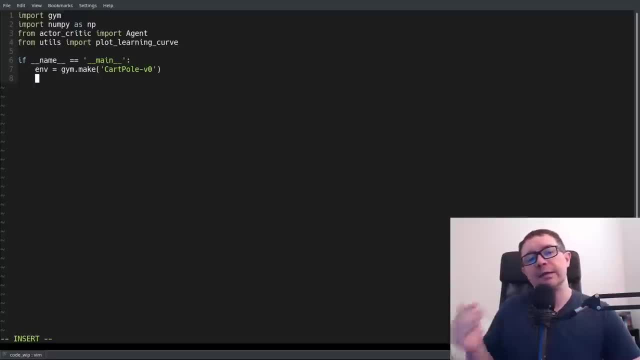 In my course we use the lunar lander environment and I did more hyper parameter tuning to get it to actually get pretty close to beating the environment. I believe In this case we won't quite beat it. We achieve a high score like one hundred forty points or so when beating it is two. 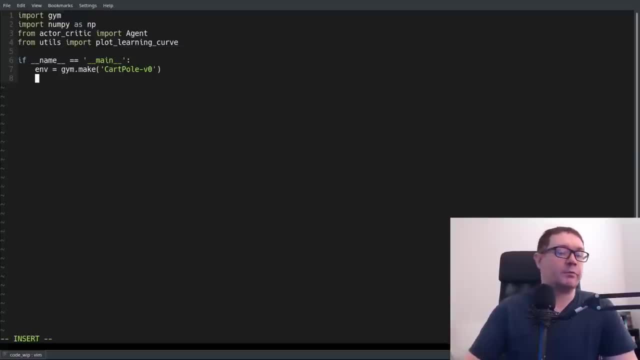 hundred, but I leave the exercise of hyper parameter tuning to you, the viewer. I got to leave something for you to do as well. Right, So we'll define our agent with a learning rate of one by ten to the minus five and a number of actions to find. 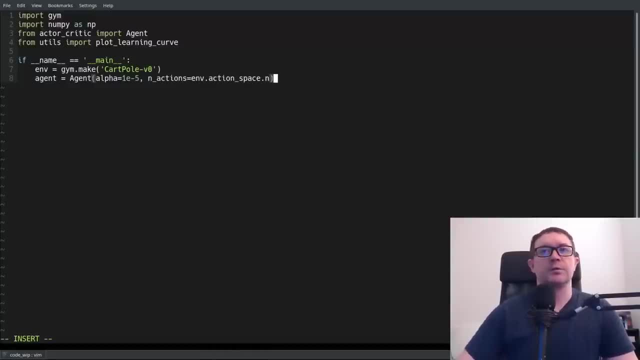 by our environment action space underscore, And then we'll have, say, eighteen hundred games, about two thousand, with a file name of cart pull dot PNG. I would encourage you, if you do hyper parameter testing, to put the string representations of those hyper parameters here in the file name, so that way when you look at it later. 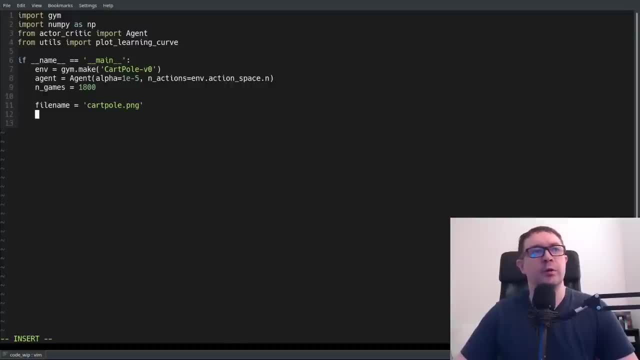 you don't get confused and you know what hyper parameters were used to generate which plot. So our figure file is just plots plus the file name. I split it up. You don't have to do it that way. We want to keep track of the best score received. 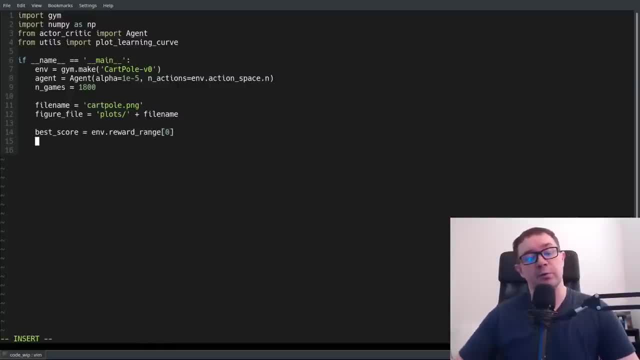 and it'll default to the lowest range. So that way the first score you get is better than the lowest of the range. So you save your models right away. An empty list to keep track of the score history and Boolean for whether or not we want to load a checkpoint. 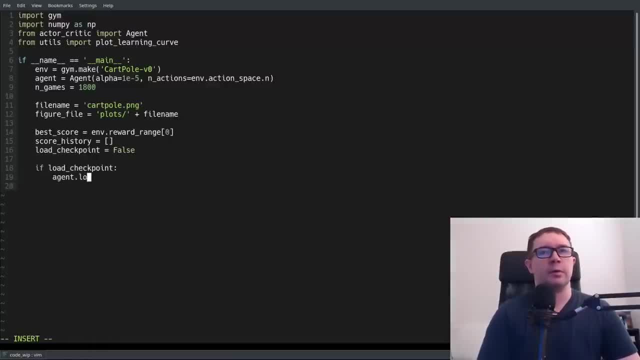 So if we're going to load a checkpoint, then I'm going to load models And then, finally, we want to go ahead and start playing our games. We want to reset our environment, reset our terminal flag, set our score to zero. 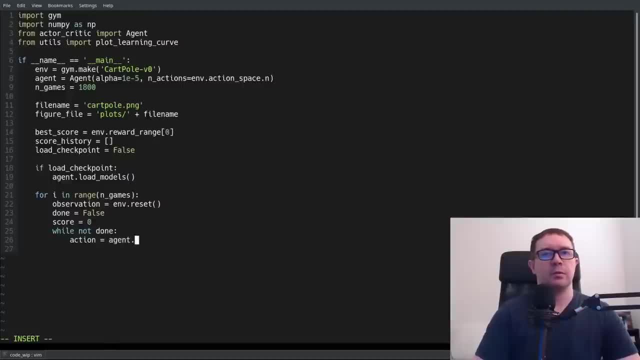 And while we're not done with the episode, we can choose an action: Get the new state Reward done. an info from the environment: Increment our score. If we're not loading a checkpoint, then we want to learn. Either way, we want to set the current state to the new state. 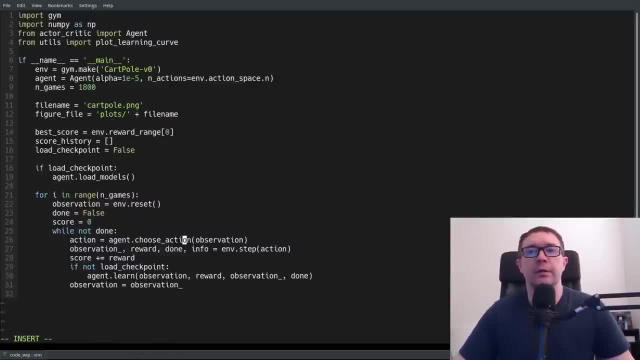 Otherwise, you will be constantly choosing an action based on the initial state of the environment, which obviously will not work. You also want to append the score to the score history for plotting purposes and calculate a score, an average score of the previous I don't know, say 100 games. 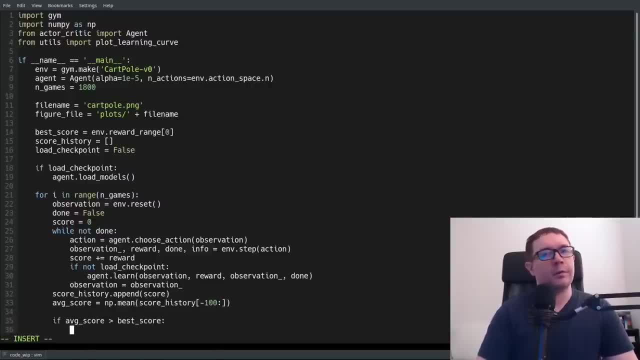 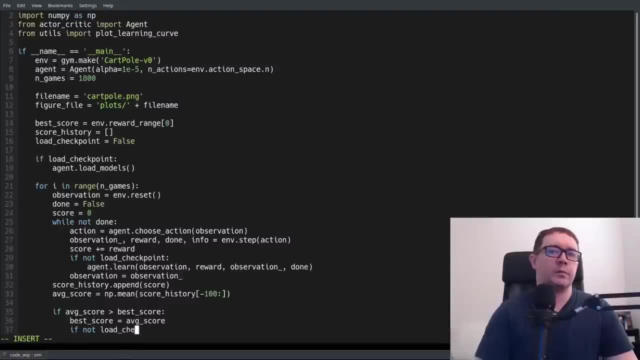 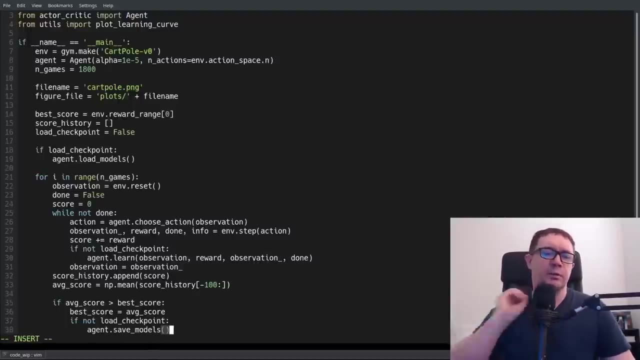 And if an average score is better than your best score, then set the best score to the average score, And if we're not loading A checkpoint, Then save your models. So this inner conditional statement keeps you from overriding your models that had your best scores when you're actually testing. 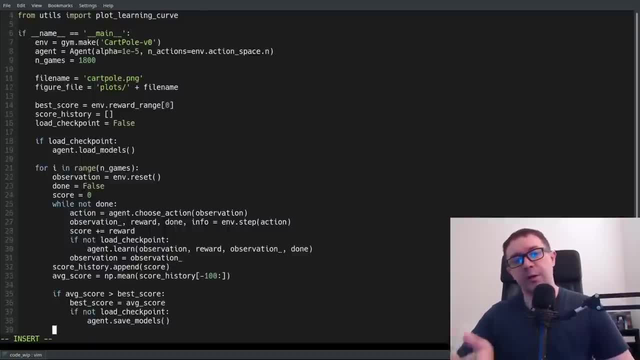 If you just save the model every time, then you'd be overriding your best model with whatever which may not be the best model. So at the end, if we're not loading a checkpoint, actually we can just plot either way. Let's do that. 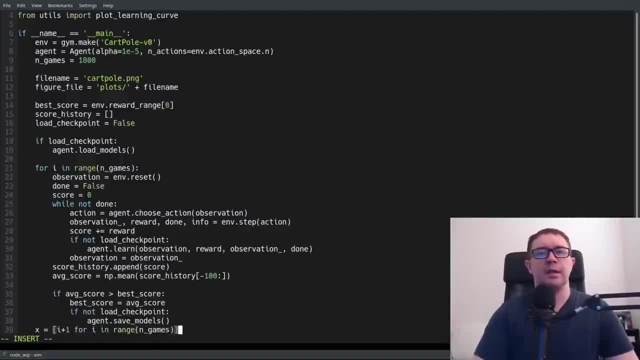 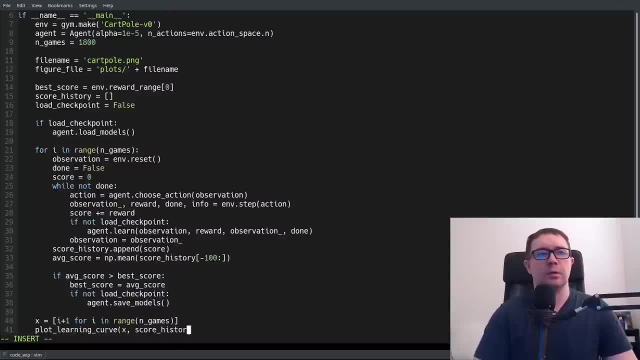 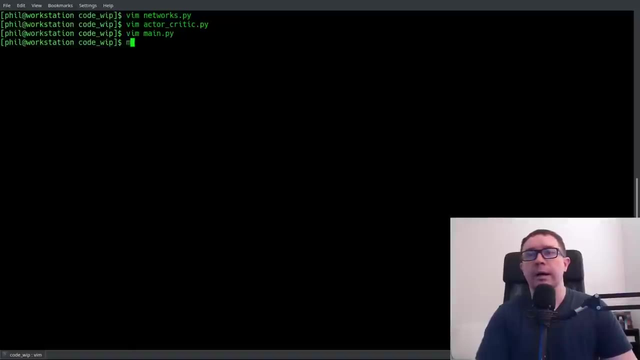 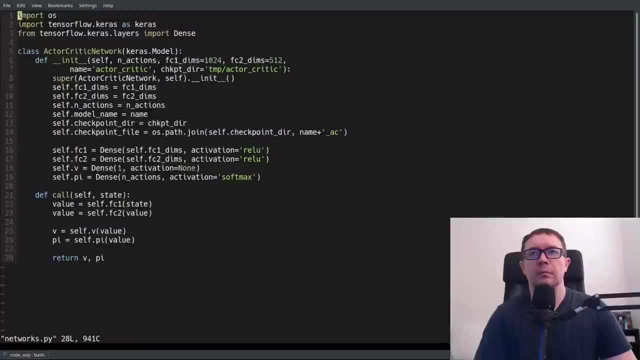 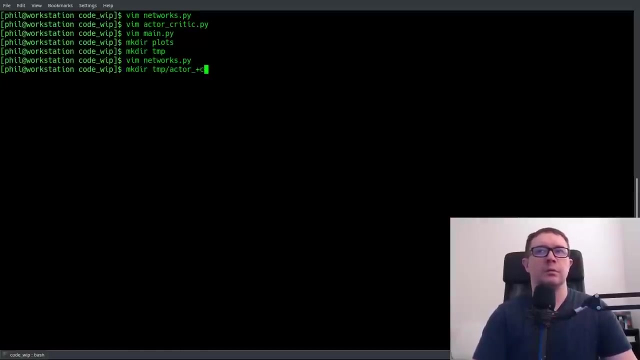 It's got our X axis and plot learning curve, X score Figure file. Okay, now I have to do a maker on plots temp, that I call it Temp slash, actor critic. Otherwise this stuff won't work. And you also want to do a pip install flow. 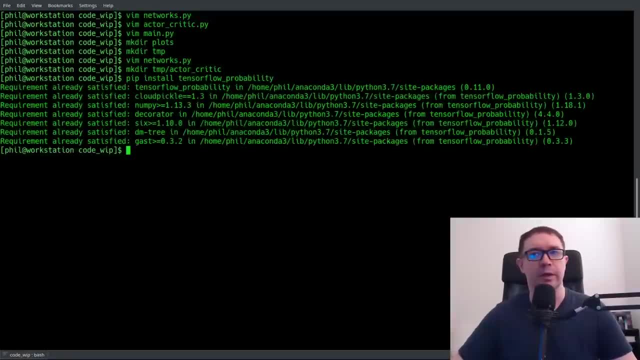 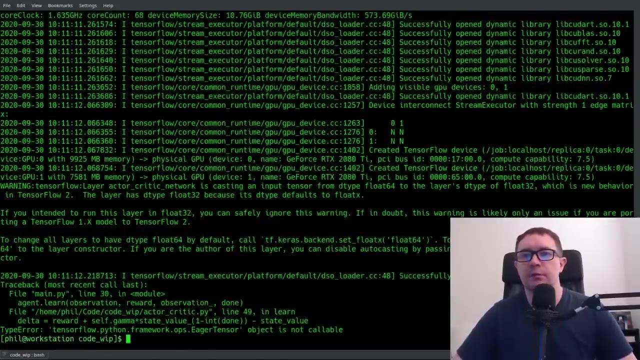 TensorFlow probability, because that is a separate package. Of course I already have it. So let's go ahead and try to run this and see if I made any typos. I'm certain, almost certain, I did. So it says something. Something is not callable. 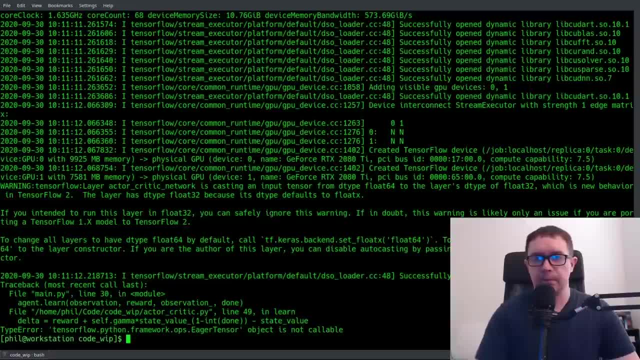 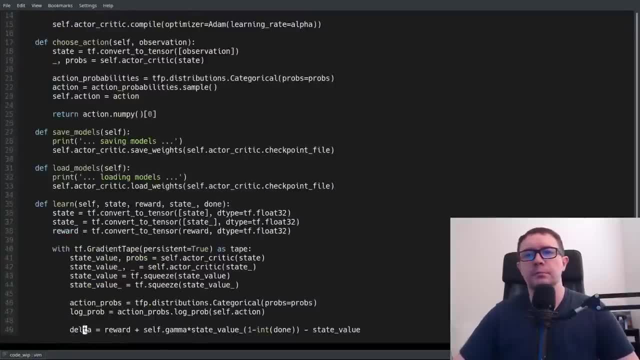 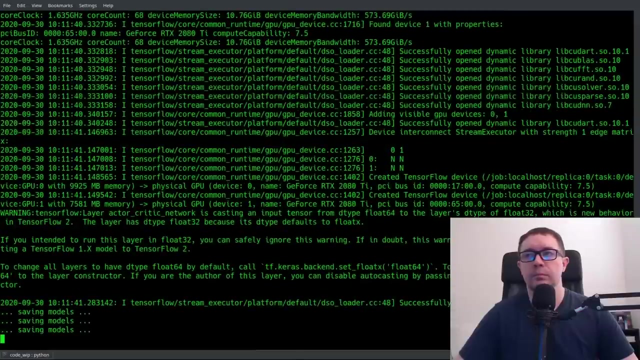 Oh, that's because I have forgotten my multiplication sign. So that is in line forty nine. Yeah, I think I'm trying to call something here when I really want to multiply. Oh, you know what I'm going to do: a pip install flow. 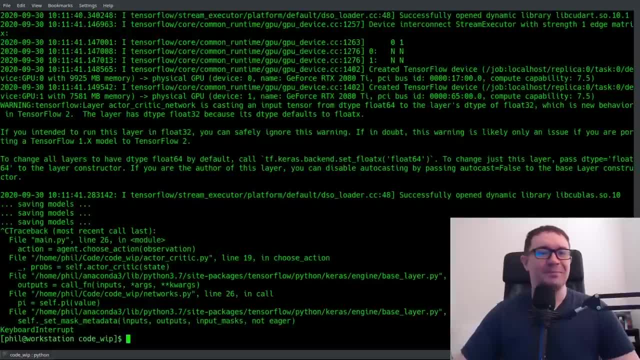 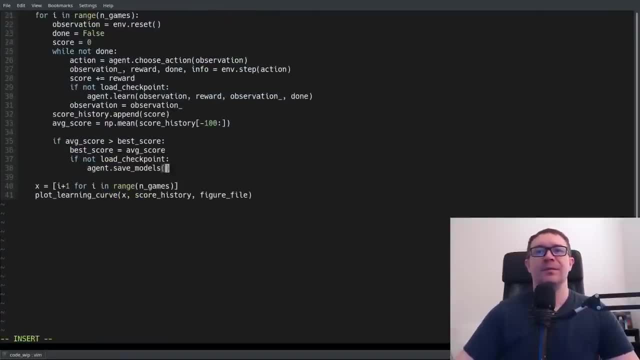 Oh, you know what I did forget? One thing I did forget, of course, is down here I forgot my debug statement, So let's do this. That's pretty funny Episode I score sent one F. Always have to forget something. 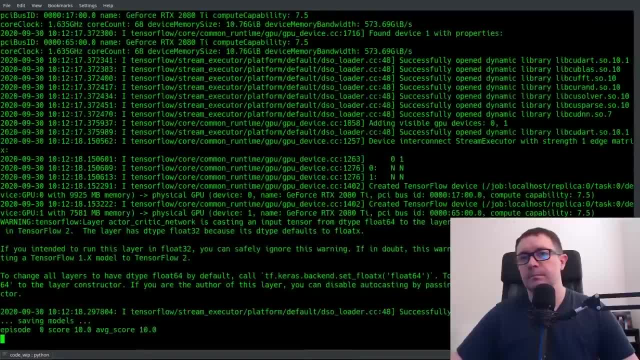 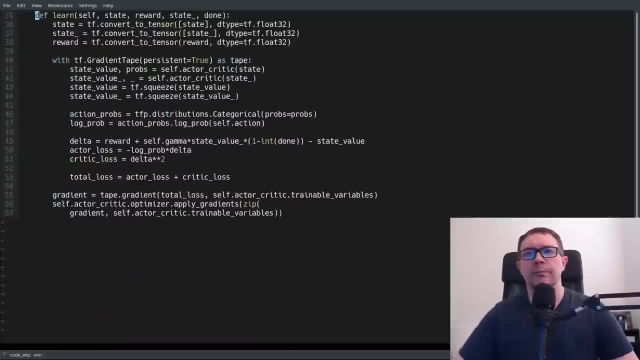 Of course. OK, there we go. So one other thing I want to do is come back here to actor critic and get rid of this persistent equals. true, I don't think I actually need this. Sometimes I just copy and paste code And then, as I'm doing the video, I realize: oh hey, I don't always need all. 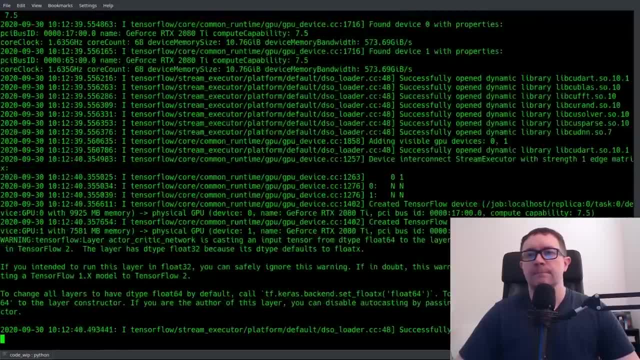 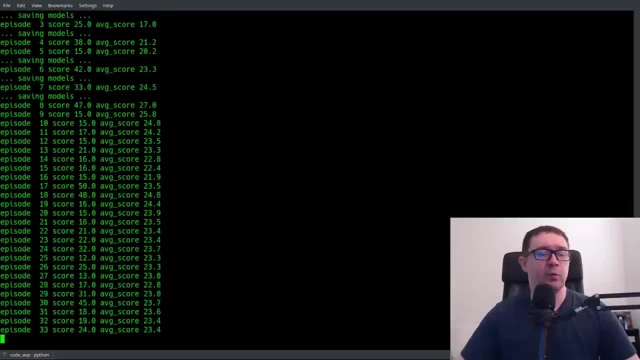 of that stuff. OK, so yeah, it does run, All righty. So I'm going to go ahead and switch over to another window where I have let this finish up, because there's no point letting it run for another eighteen hundred games. 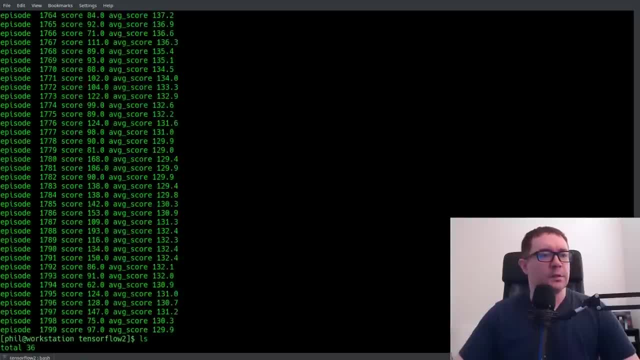 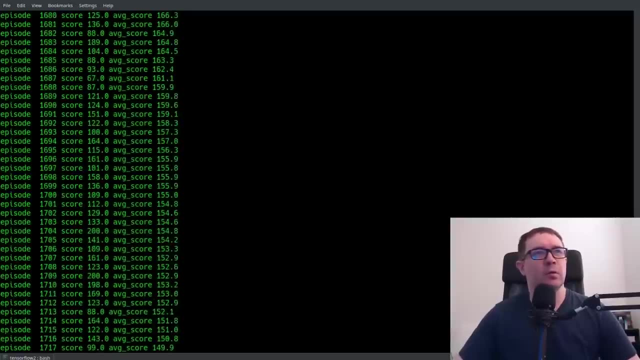 So let's go ahead and check that out. So here you can see the output of the other eighteen hundred games I ran, and it does achieve a score of around one hundred and sixty, seven hundred sixty eight, about one hundred seventy points or so, which is almost beating the environment. 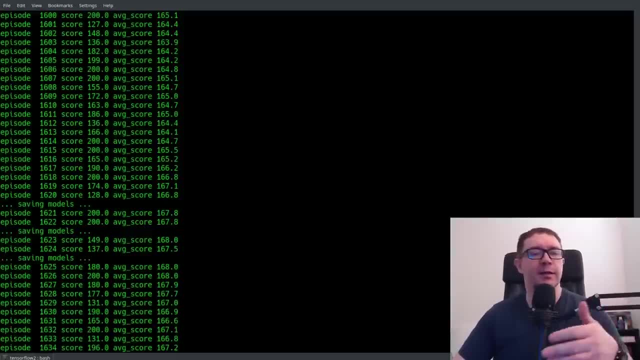 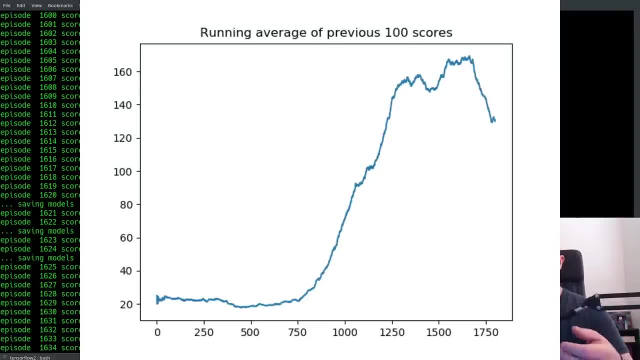 It's pretty close. If you take a look at the learning plot here, you can see that it has an overall overall upward trend and it's linear. And the reason I don't let it continue is because, as I alluded to in the lecture, these models are very brittle. 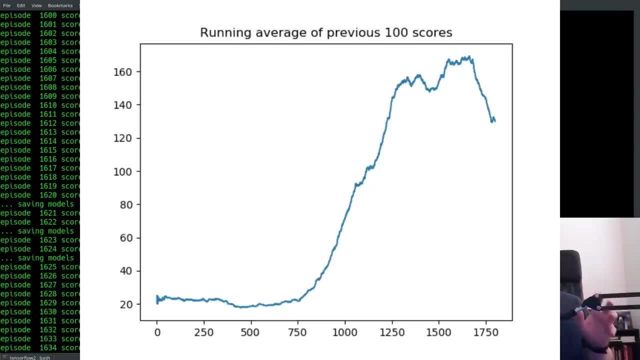 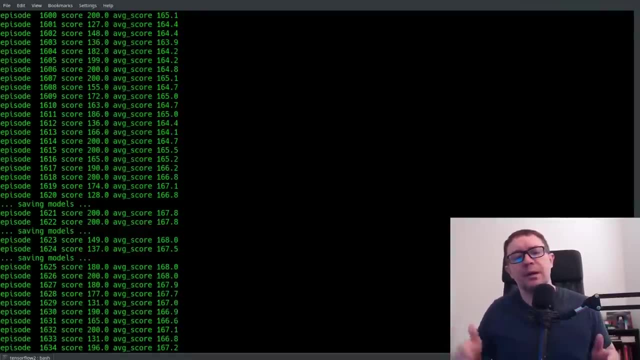 And so sometimes you can get on a very narrow slice of parameter space where your model is doing well And any small step out of that range blows up the model. One thing to fix that is replay memory as you get a broader sampling of of experiences and get a little bit more stable learning. 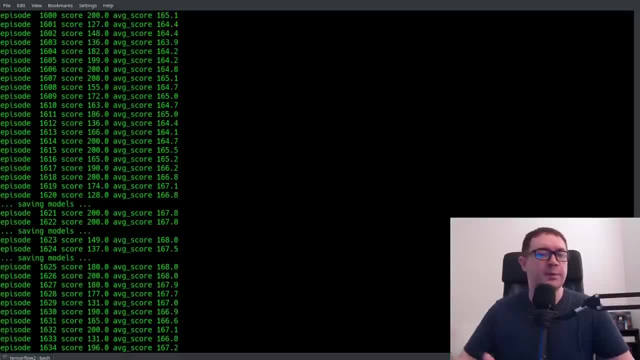 But that doesn't work. by bolting it directly onto actor critic methods, At least from my experience. I've tried it. I have a video on that. I wasn't able to get it to work. Maybe some of you can. That would be fantastic if you could. 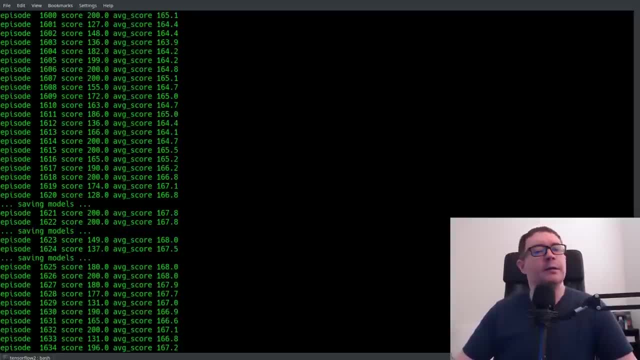 But in my case I didn't get it to work. I thought it would work. It does not, And in fact there's a whole separate algorithm called actor critic with experience replay that deals with bolting experience replay onto vanilla. actor critic methods. 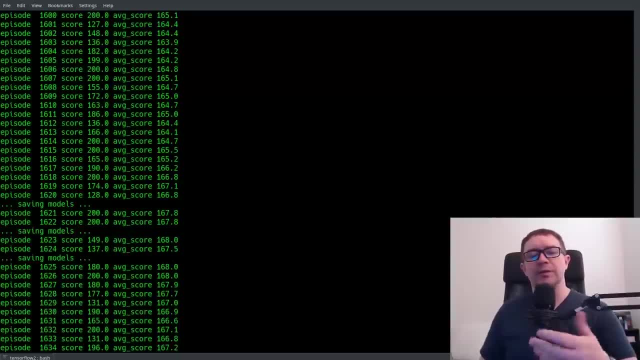 So I hope this was helpful. It's pretty hard to give a really solid overview in like a 30, 40 minute YouTube video, But it serves to illustrate some of the finer points of actor critic methods and some of the foundational points of deep reinforcement learning in general. 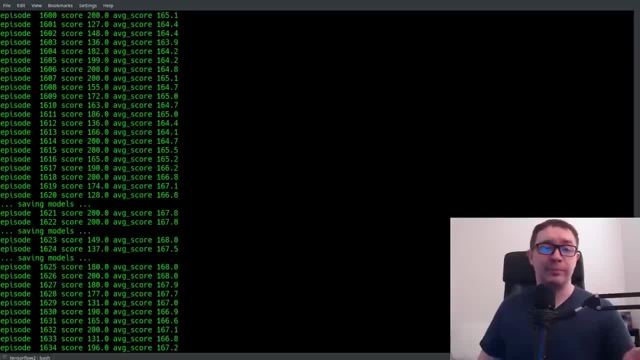 And my courses are going to much more depth and, in particular, I show you how to actually read papers, how to turn papers into code, a useful skill It's really hard to find anywhere else on YouTube or Udemy. So if you like the content, make sure to leave a like. 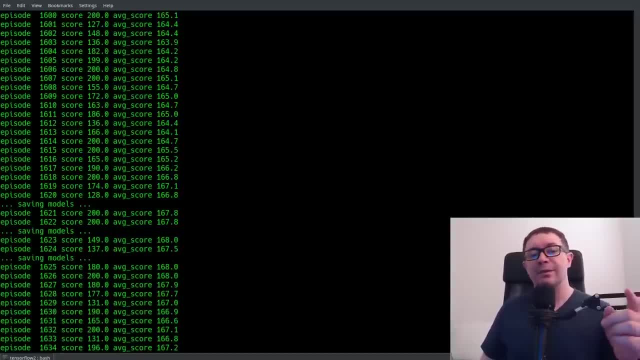 Subscribe, if you haven't already, and leave a comment down below. Let me know with any questions, comments, criticisms, concerns, and I will see you in the next video. really quick, before we do, Let's check in on the other terminal to make sure it's actually learning. 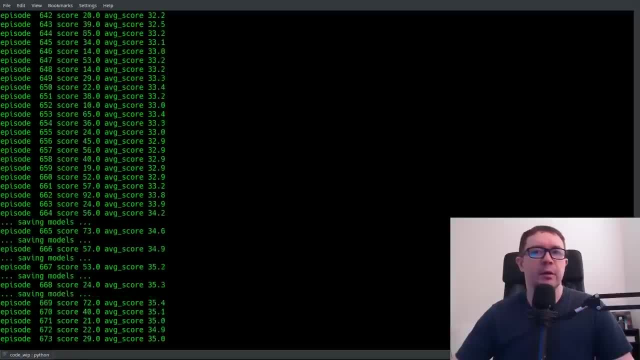 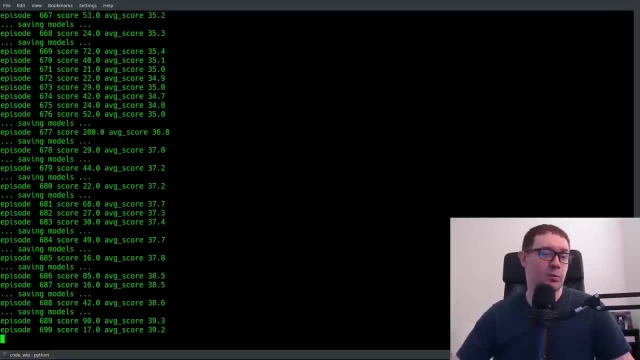 So here is the output And you can see as it's going along. it is saving some models and the score is generally trending upward over time. and that's where you get the saving models, because the score is best in the last best score. 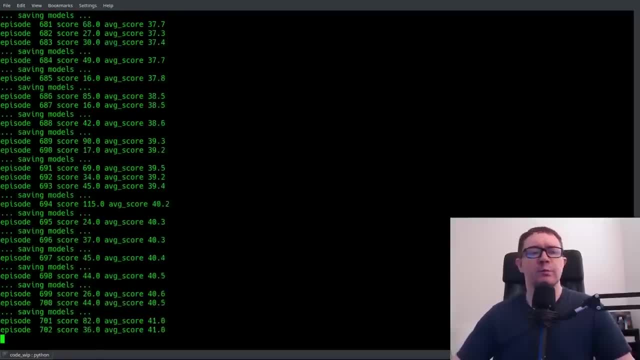 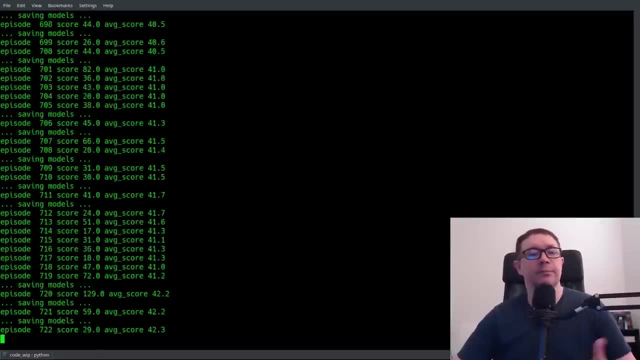 So we didn't make any fundamental errors in our code. If it doesn't achieve the same result, that isn't entirely surprising, because there is a significant amount of run to run variation, But the code is functional. What's up on my GitHub? If you want to go ahead, check it out. 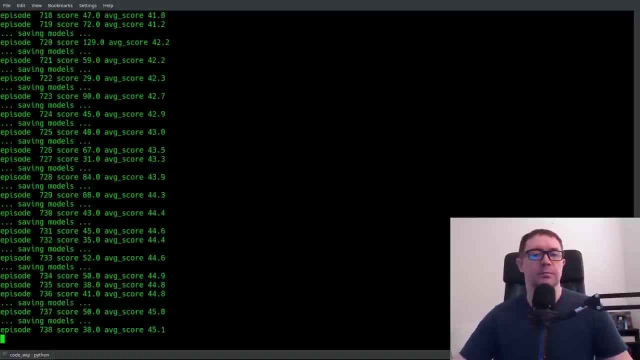 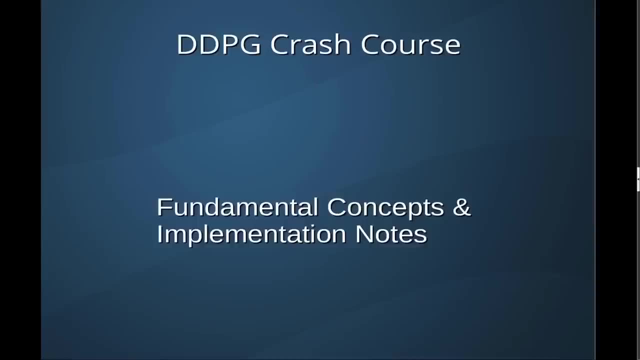 I'll leave a link in the description. See you in the next one. Welcome to a crash course in deep deterministic policy gradients, or DDPG for short. In this lecture we're going to briefly cover the fundamental concepts and some notes on the implementation, so that the stuff we do 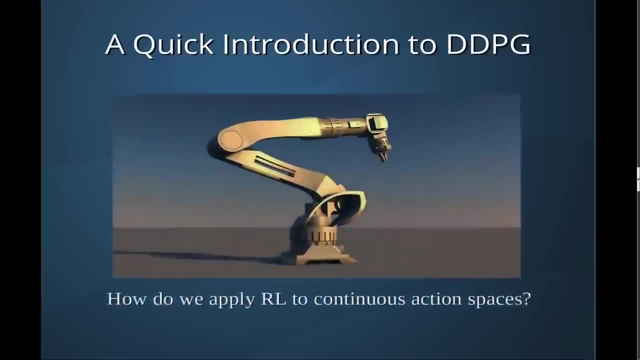 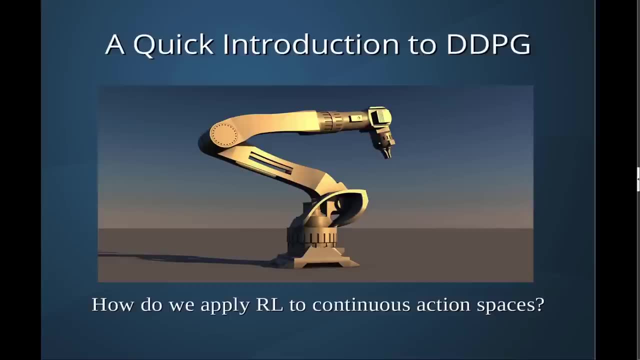 in the coding portion isn't such a mystery. So why do we even need DDPG in the first place? Well, DDPG exists to answer the question of how do we apply reinforcement learning to continuous action spaces. This is particularly important in something like, say, robotics. 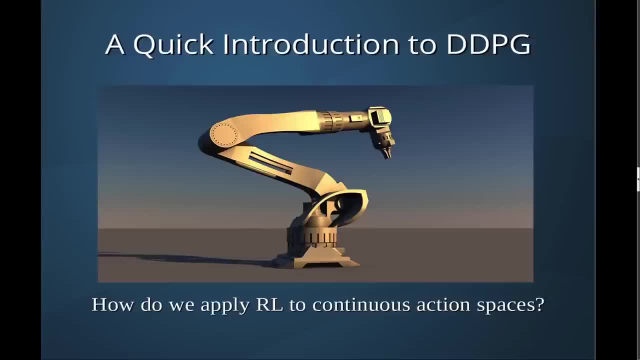 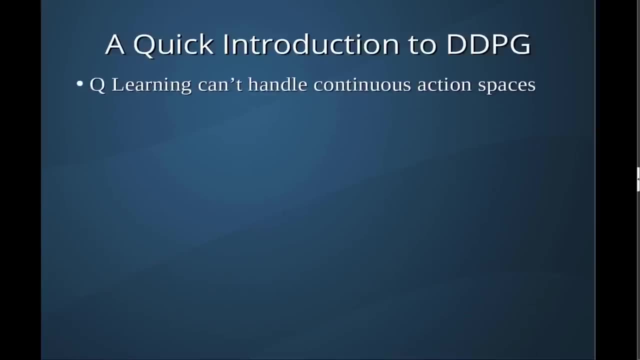 where we are applying continuous voltages to electronic motors that cause the robot to move in three dimensional space. Now you may think: well, why can't we just use something awesome like deep Q learning, And that's not such a terrible idea. 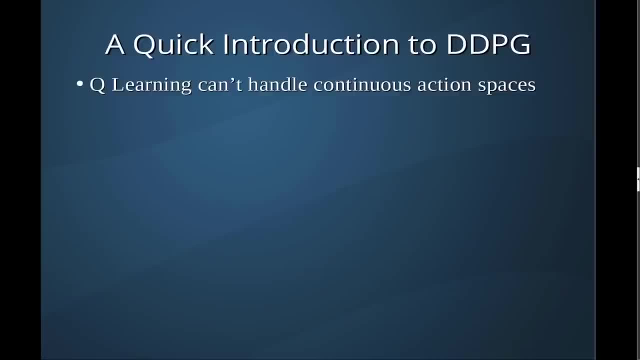 However, the problem is it doesn't work. In particular, Q-learning can't handle continuous action spaces. If you've coded up a Q-learning network, a deep Q-learning network that is, you know that it outputs discrete numbers as actions And of course, that doesn't cut it when you're dealing with continuous 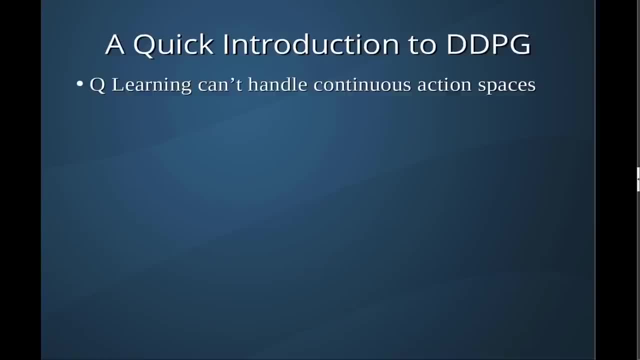 action spaces. Now you might think, why can't we just discretize our action space, And that's not such a bad idea. But the problem is it doesn't work. And the basic idea here is: if you have some finite interval for your action space and then you just divide it, 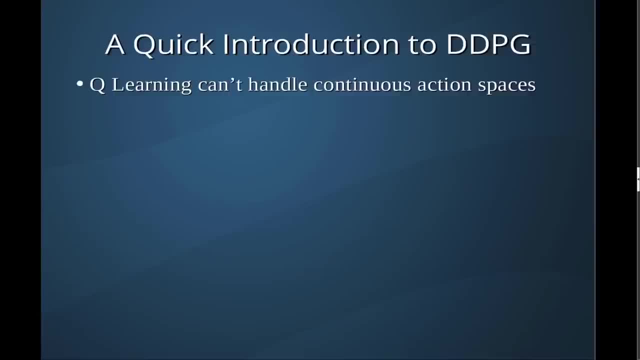 up into a number of discrete chunks and then, every time you want to output the action in that chunk, you just use that discrete integer. The problem with this is that these robots tend to have many degrees of freedom, meaning they can move in many different directions in space, right? 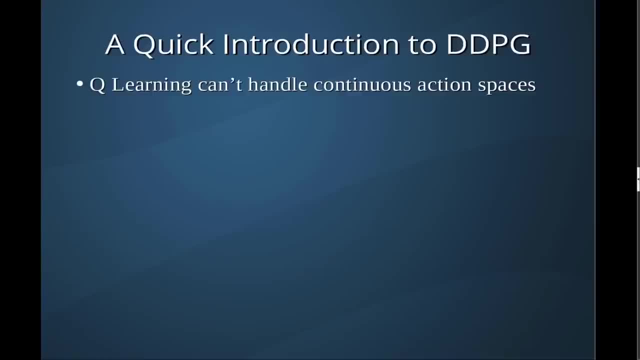 They can rotate around axes, multiple axes in general. They can move up down, left and right, They can rotate, And so your number of discrete actions approaches the thousands very, very quickly. And so Q-learning, while it does handle discrete action spaces, doesn't handle large numbers of discrete actions particularly well. 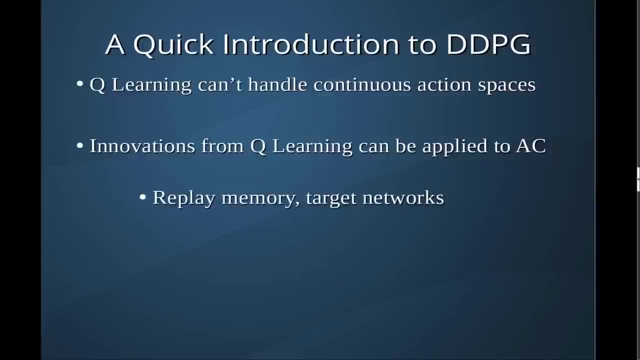 However, that doesn't mean that the innovations from Q-learning can't be applied to actor-critic methods, and in fact they can, And that was the motivation behind the work done in the DDPG paper. In particular, we're going to make use of a replay memory where, instead of just 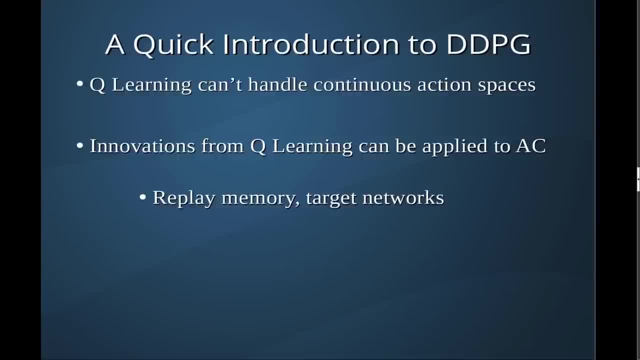 learning from the most recent state transition that the agent has experienced. it's going to keep track of the sum total of its experiences and then randomly sample that memory at each time step to get some batch of memories to update the weights of its deep neural networks. 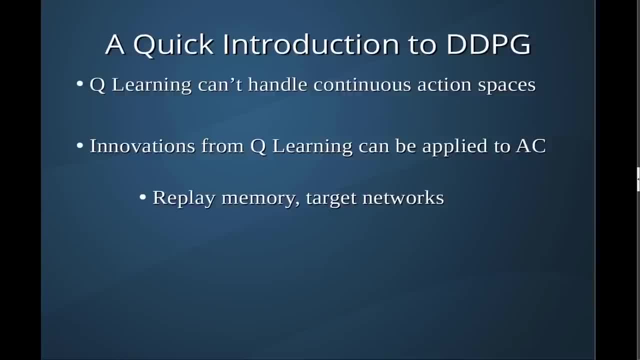 The other innovation is the use of target networks. So in Q-learning we have to do two different things: We have to use a network to determine the action to take and then we have to use a network to determine the value of that action And that. 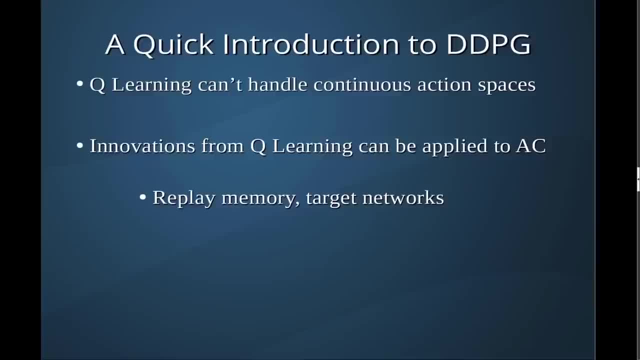 value is used to update the weights of the deep neural network. Now, if you're using the same network to do both things, the problem is you end up chasing your tail. You end up chasing a rapidly moving target because at each time step those weights. 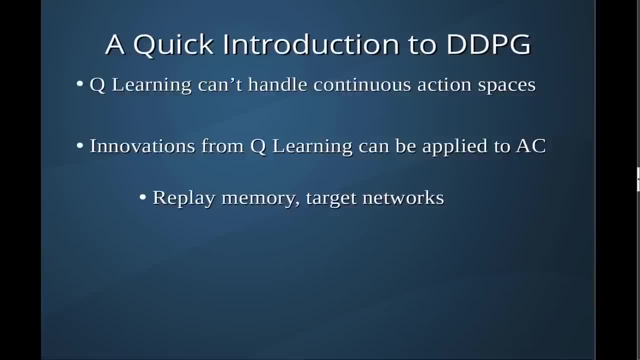 are getting updated, and so the evaluation of similar actions- excuse me, the evaluation of similar states- changes rapidly over the course of the simulation, causing the learning to be unstable. The solution to this is to keep two networks, one of which you use. the online network, is called to choose actions at each time step. 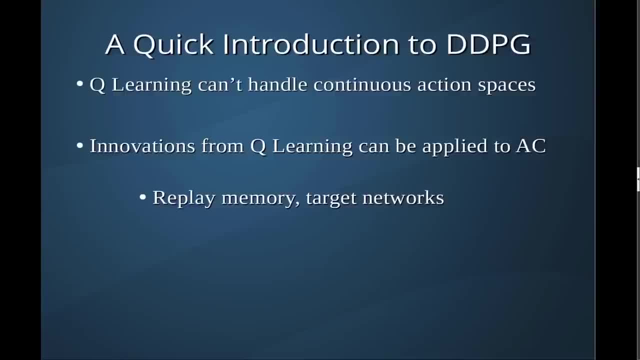 and then another network called a target network, to evaluate the values of those actions when performing the update for your deep neural network. Now, in this case, you will be doing a hard update of your target network. So every- let's say- thousand steps, it's a hyper parameter of your agent. 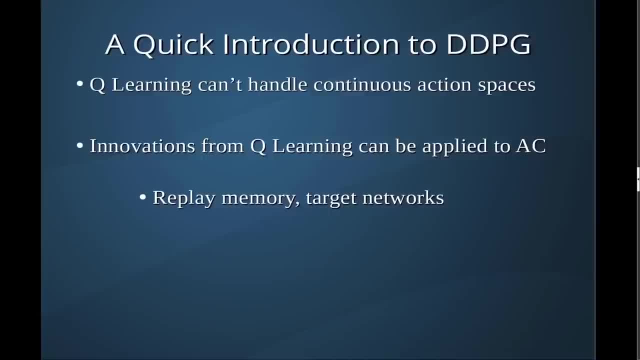 but a typical value would be a thousand steps. You would take the values for the network from the online network and directly copy those over to the target network. It's what's called a hard update. The authors of the DDPG paper took inspiration from this. 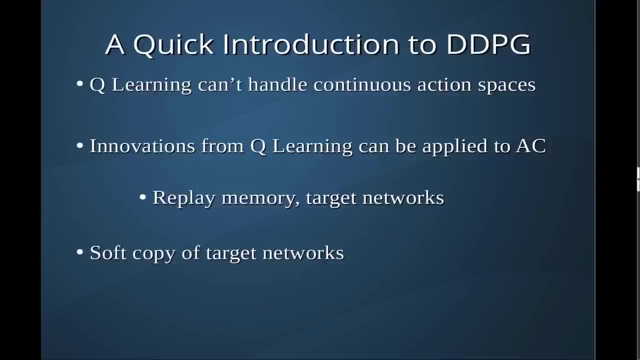 but instead of doing a direct hard update, they used something called a soft copy of the target networks. All this means is that we're going to be doing some multiplicative constant for our update and we're going to be using a new hyper parameter called tau. 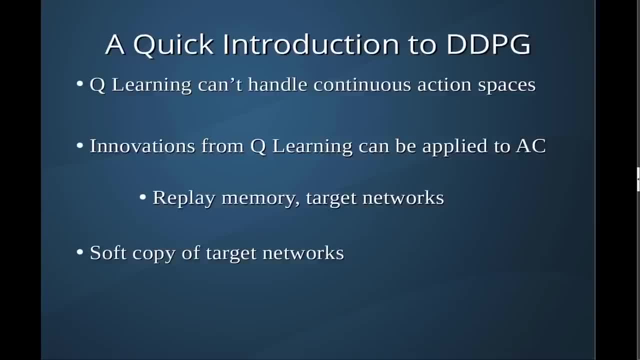 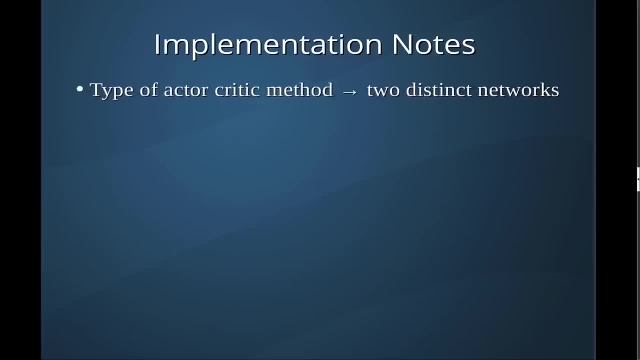 and it's going to be a very small number of order: point zero, zero one. It's also worth noting that we're going to have more than one target network here, And the reason we need more than one target network is because DDPG is a type of actor critic method. 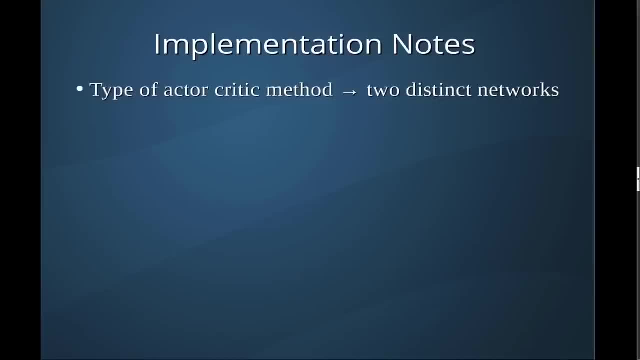 And so you have two distinct networks, one for the actor and one for the critic, And in fact, in this implementation we're going to have four different networks: one actor, one critic and then one target actor and one target critic. 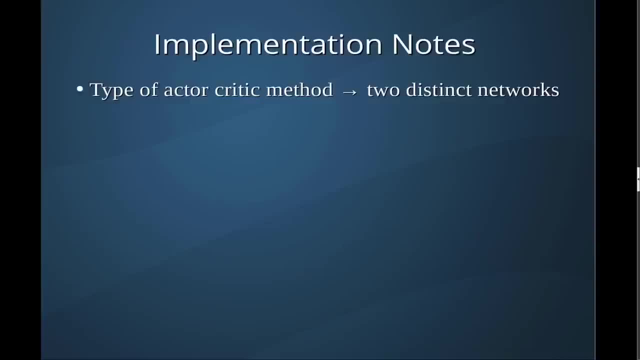 Now for simple problems with discrete action spaces. you can get away from having a single network where the lower layers learn the features of the environment and the upper layer splits off into outputting the, the critic evaluation, as well as the output for the actor network. 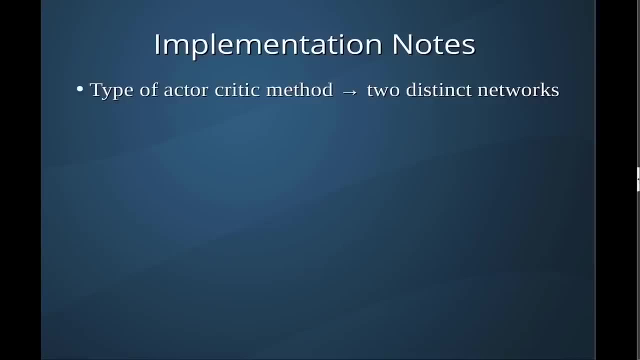 But in this case we do in fact want two totally distinct networks, as well as two copies of those for the target networks. The basic idea is that our critic network is going to evaluate state in action pairs, And so we're going to be passing in states and actions. 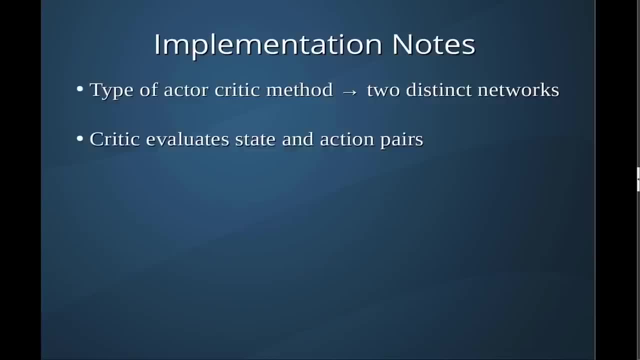 We're going to say, hey, given that state, the action we took was pretty good, or maybe that action was pretty terrible. We should probably do better next time. And, similarly, the actor is going to decide what to do based on the current state or whatever state we pass into it. 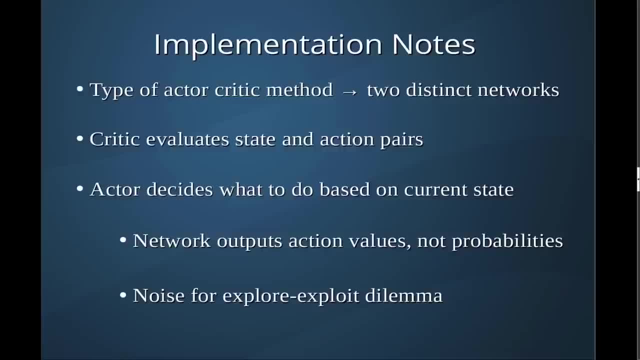 Something worth noting is that this network is going to output action values, in other words, a continuous number that corresponds to the direct input for OpenAI Gym environment, rather than outputting values. So if you've been doing this for a while, you may know that the policy is actually a probability distribution. 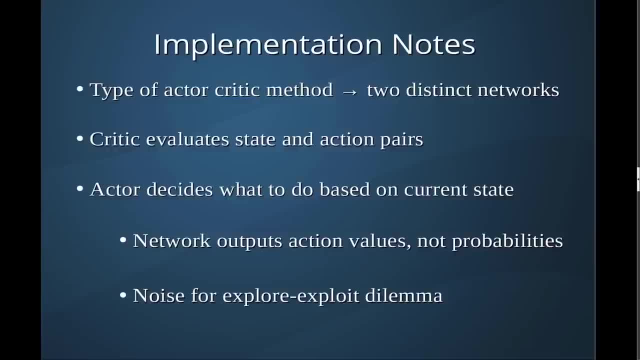 It is a function that tells us what is the probability of selecting any action from the action space given an input of a state or set of states. The deterministic part comes from the fact that DDPG outputs the action values themselves, And it's deterministic in the sense that if I pass in one state over and over, 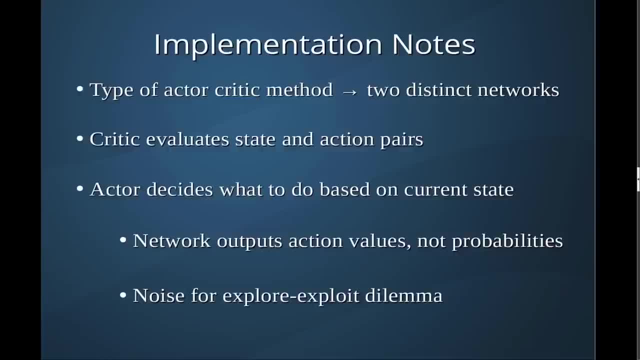 and over again. I'm going to get the same action value out every single time. Now this does have a bit of a problem. So the problem is that the agent has something called an explore-exploit dilemma, and this is present in all reinforcement learning problems. 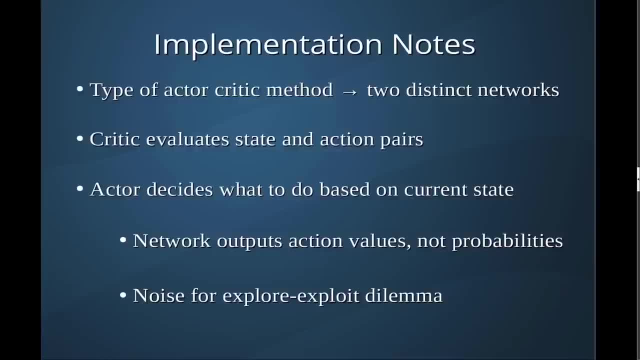 It's a fundamental concept in the field. The basic idea is that our agent is attempting to build out a model of the world. The agent wants to know how to maximize his total score over time, But it starts out knowing absolutely nothing about its world. 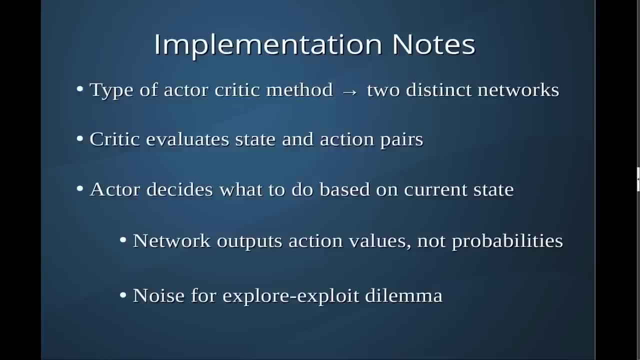 It has to figure out how states transition from one into another and how its actions affect those states and in particular how its actions give it rewards. So it starts out knowing none of this and has to build out that model over time. The problem is the agent can never be quite sure that its model is accurate. 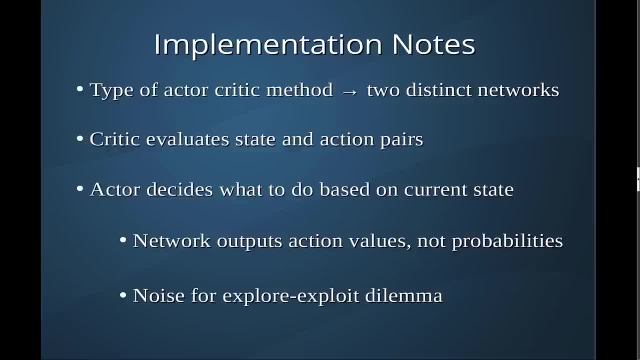 No matter how long it spends playing the game, interacting with the environment, it isn't 100% certain that the action it thinks is best is actually the best. Perhaps there's some other strategy, some other action out there that is significantly better. 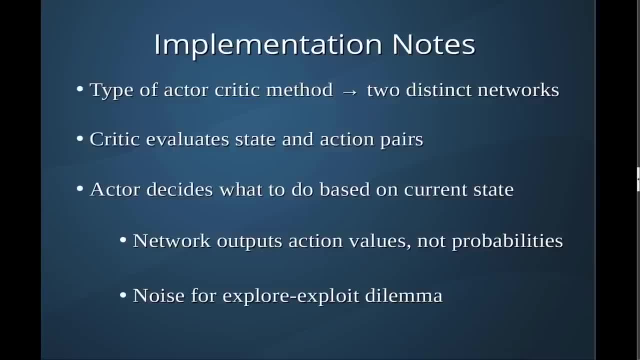 And the degree to which the agent takes off-optimal actions is called the explore-exploit dilemma. So, of course, taking an off-optimal action is called exploration and taking the optimal action is called exploitation, because you're just exploiting the best known action, And this is a dilemma that is present. 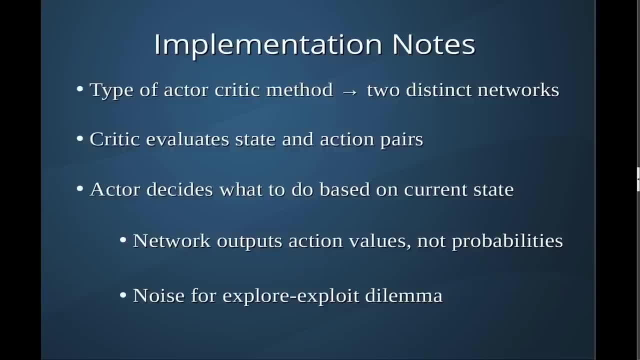 in all reinforcement learning problems, And the solution here is to take the output of our actor network and apply some extra noise to it. Now, in our implementation, we're going to be using simple Gaussian noise, because it's sufficient for the problem at hand. 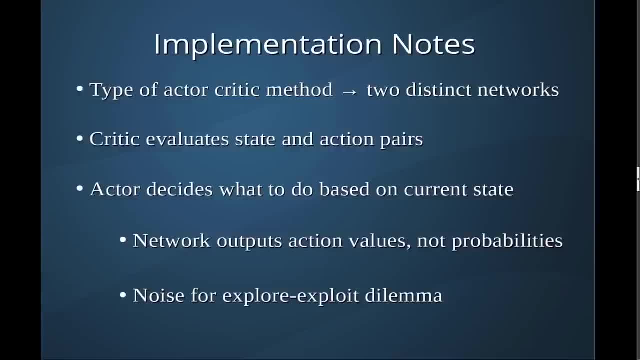 However, in the original paper the authors use something called Ornstein-Uhlenbeck noise. It's a model of Gaussian processes and physical systems. It's overly complex and it's not needed, So we're not going to implement it, Although in the course I do show you how to implement it exactly. 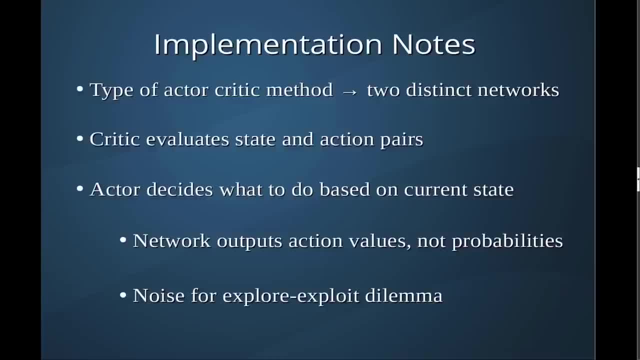 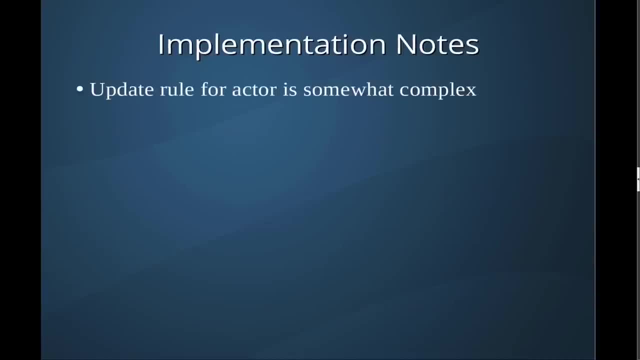 But for YouTube it's not really necessary And in fact, when other authors implement DDPG, they just throw that right out the window because it's pretty dumb. Next is the update rule for our actor network, and it is somewhat complex. 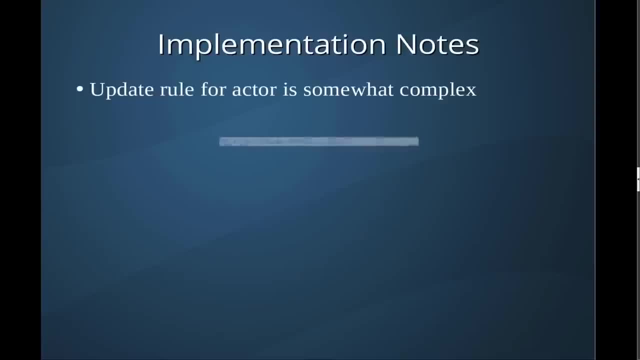 So I'm going to show you the equation and then I'm going to walk you through it. So this is the update for the actor network, And don't panic, This is a little bit easier than it looks at first glance. So from left to right, we have the nabla operator. 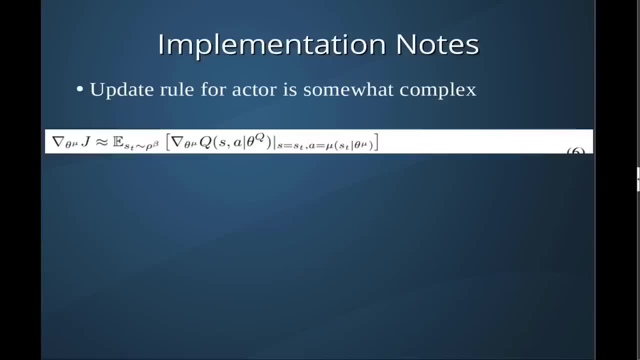 That is the gradient And the subscript. there theta super mu means that we want to take the gradient of the cost function j with respect to the network parameters of our actor network, where the actor is denoted by mu and its parameters are denoted by theta super mu. So theta super q means the 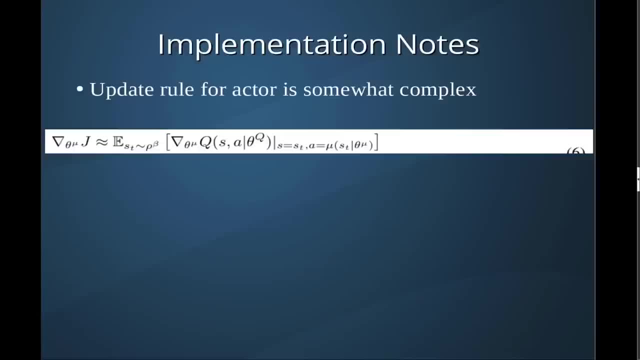 parameters for the critic network, where the critic is denoted by q And that's just given by an expectation value or an average of the gradient of the critic network, where we're going to input some states and actions, where the actions are chosen according to the current policy. 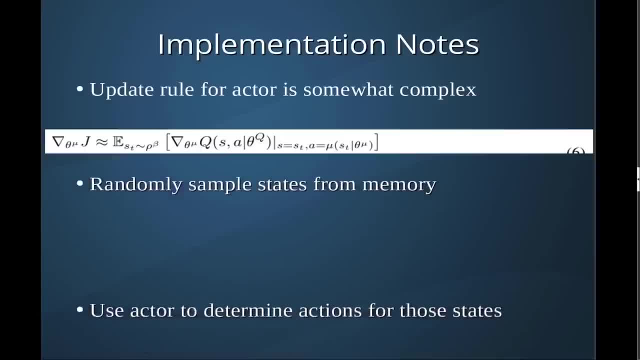 OK, So in practice, what this means is what we're going to do is randomly sample states from the agent's memory. Now, the memory keeps track of everything we want. It keeps track of the states the agent saw, the actions it took. 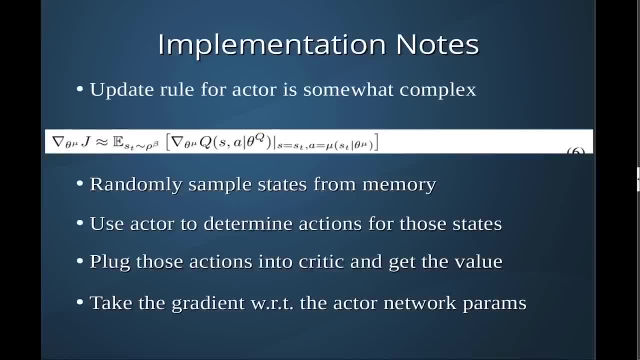 and the new states that resulted from those actions, as well as the reward the agent received at that time step and the terminal flag to determine whether or not the episode ended on the new time step. So the memory keeps track of all of that, But here we just want to sample. 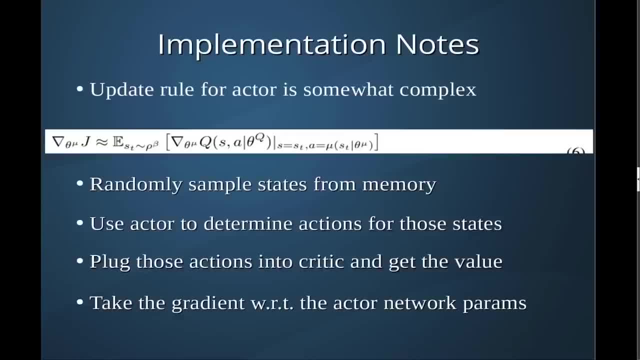 the states, the agent saw OK, And then we're going to use the actor network to determine what actions it thinks it should take, based on those states. Now, these actions will probably probably be different from the actions we have stored in memory, and that's OK. 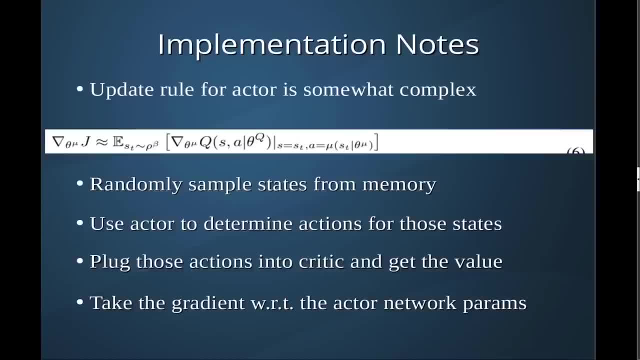 This is off policy, meaning we're using a separate policy to gather data and use that data to update a different policy, the current policy. So it's OK that these actions don't match. Don't worry about that, It all works out in the end. 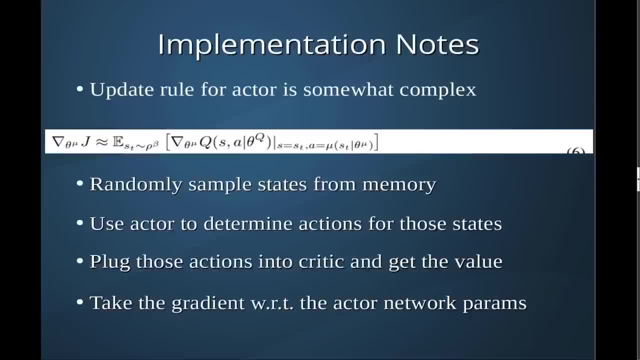 Then you. then the next thing you want to do is plug those actions from the actor into the critic network along with the states we sampled from the memory, and get the value for the critic network, what it thinks that state action pair is worth. And then we're going to use the gradient. 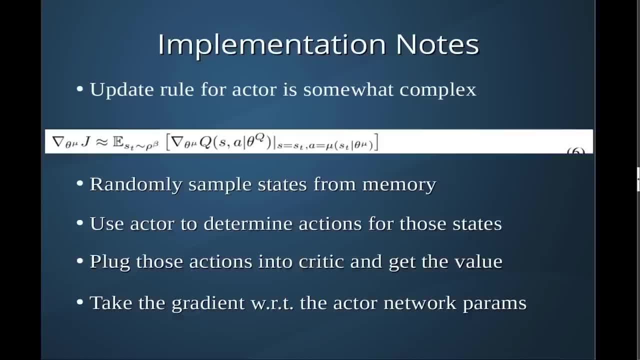 tape from TensorFlow 2 to take the gradient of the actor network. This is the critic network with respect to the parameters from the actor network, And we can do that because they're modeled through the selection of the actions based on the actor network. OK, so it's a little bit complex. 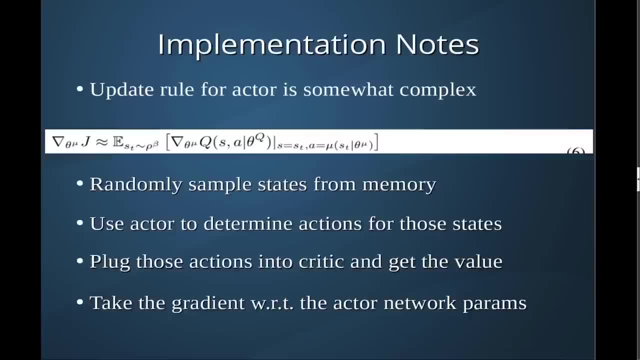 It's much easier in code. Just in code you sample the states, then you get the actions based on the critic network and then plug those states and actions into the critic network And then you just have the loss proportional to that. It's actually much simpler in code than it is on paper. 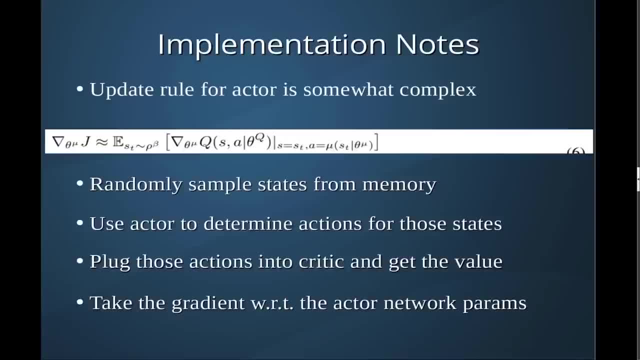 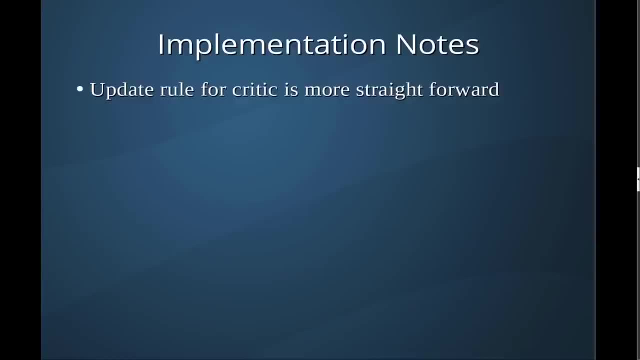 But that's the basic idea. So then the next question is: how do we implement our critic network? Well, fortunately, it's a little bit more straightforward and it's more reminiscent of deep Q learning. So we have this relatively simple loss function that is the mean squared error between this, this target value, Y, sub I. 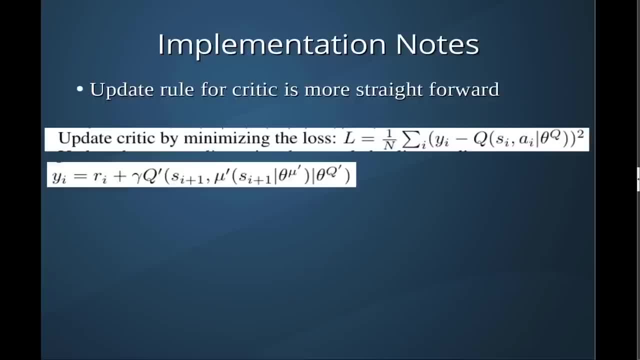 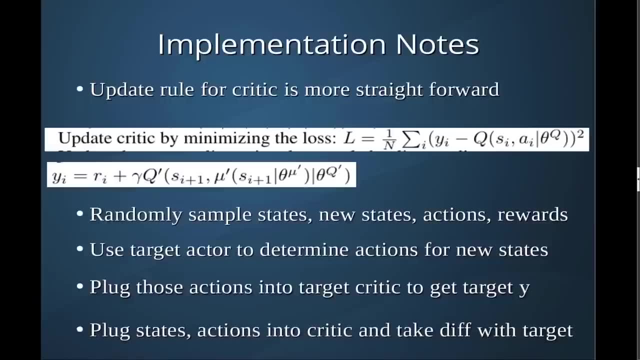 and this Q for the current state and action. So what we're going to do here is randomly sample states, new states, actions and rewards, And then we want to use the target actor network to determine the actions for the new states, Then plug those actions into the target. 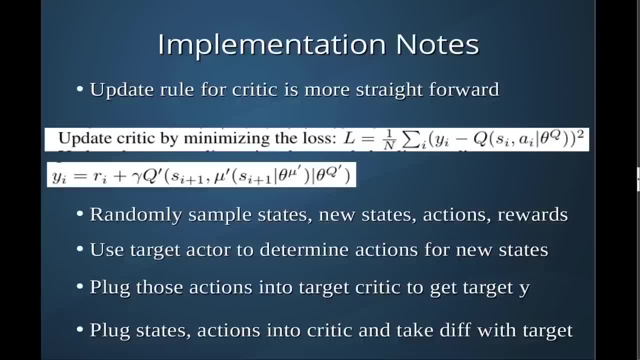 critic network to get your Y and multiply it by the discount factor gamma and add in the reward from that time step which you sampled from the memory, And then that is a target, The value we want to shift the estimates for our critic towards. 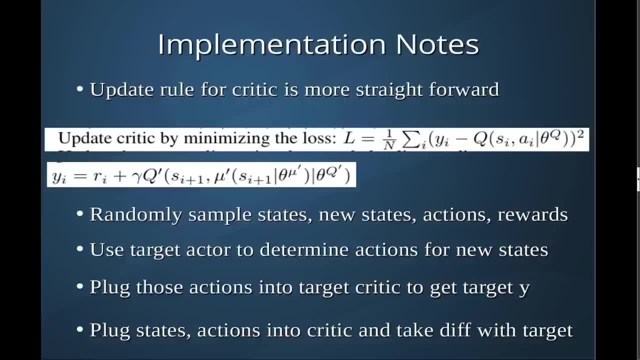 And then we want to plug the states and actions into the critic network, In other words, the actions the agent actually took that we sampled from our memory- This is in contrast to the update for the actor network- and take that difference with the target and then we're going to input it into the mean squared error loss. 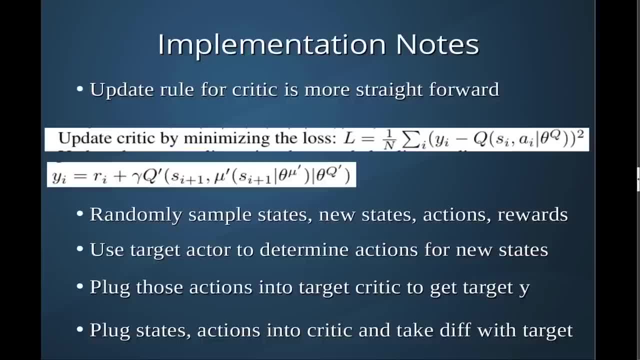 function for TensorFlow two. So in code this is going to be relatively straightforward as well. We're going to have a sample function to get states, new states, actions and rewards. We're going to plug in the new states into the target actor network. get some output. 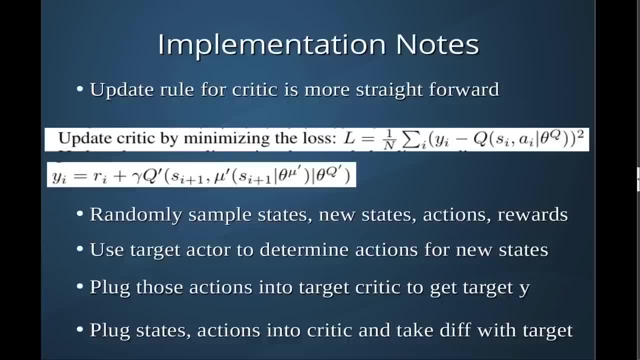 We're going to plug that output into the target critic To get our target Y and note it is S sub I plus one. So it is the new states that we get from our memory buffer And then we're going to plug the current states and actions from our memory. 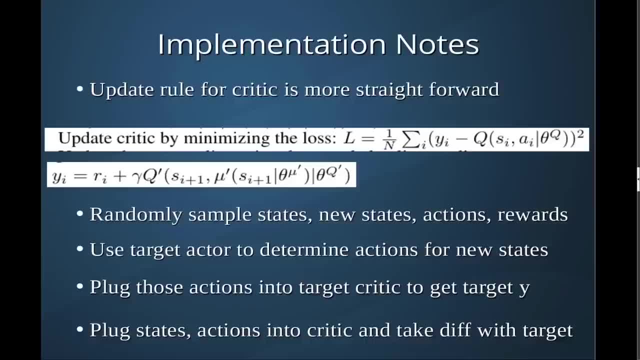 into the critic and take the difference with the target. So it only looks kind of scary on paper. When you see it written in code, it'll make much more sense. So the other piece of the puzzle is how we're going to handle the updates of our target networks. 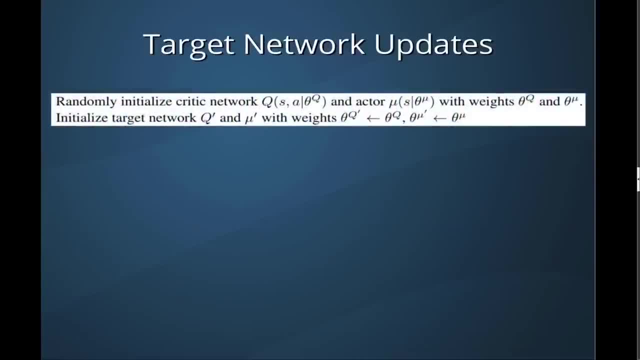 So at the very beginning of the program we are going to initialize our actor and critic networks with some parameters- Of course they're going to be random- And then we're going to directly copy those parameters over to our target actor and target critic networks. 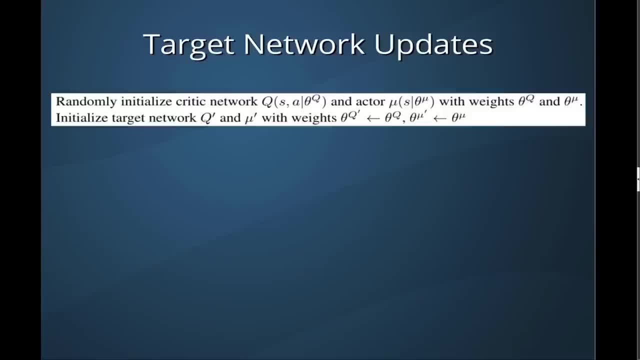 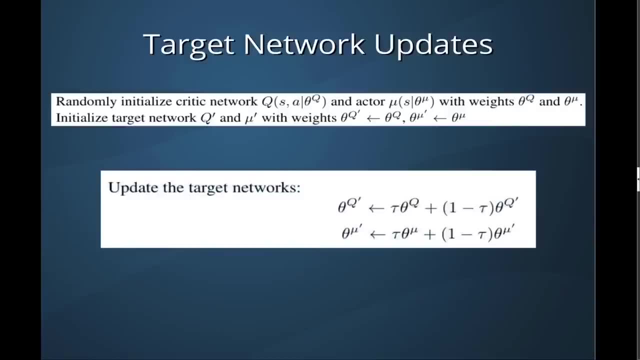 That'll be the only time in the simulation that we do an exact hard copy. Every other time step we're going to use the soft update rule. So here you have the two parameters: theta super q prime, So the weights of the target critic network. 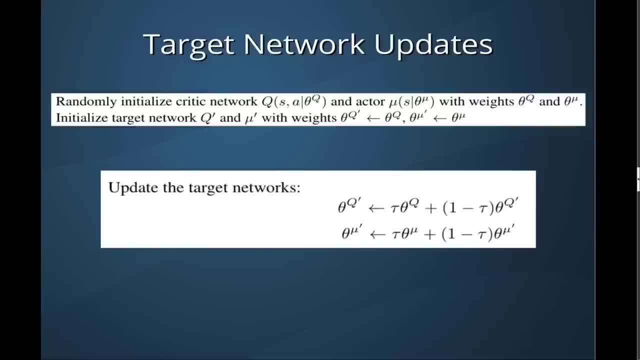 and theta super q prime, Theta super mu prime, which is the weights of the target actor network. You're going to update those with tau multiplied by the respective value of the online network, the critic or the actor, and add in one minus tau times the current value of your target actor or target critic network. 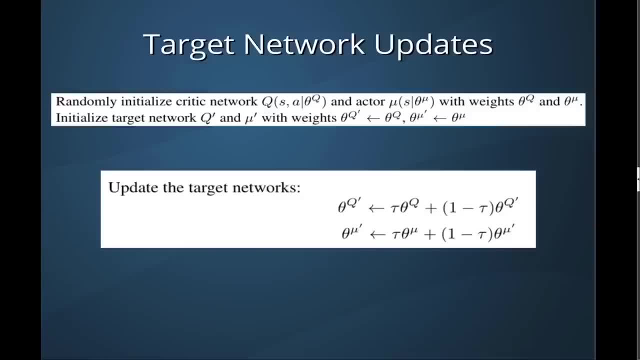 And so this will be a very slowly changing function, because it's going to be some small number tau multiplied by some parameters, plus one minus tau, which is which is approximately one multiplied by the current value. So it's going to be approximately equal to its last time step, just plus minus a little bit. 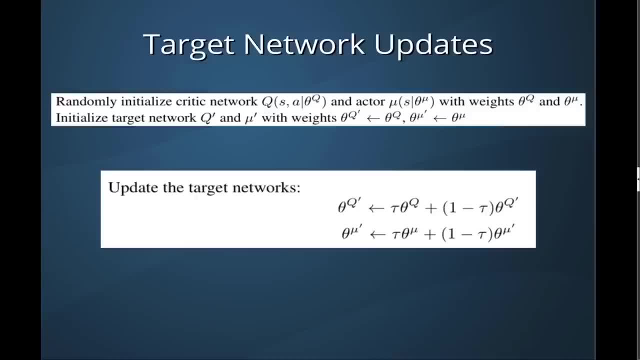 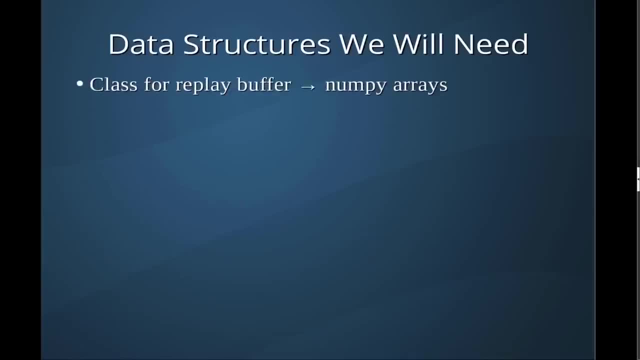 So it's relatively straightforward. We'll see it in code. It's not all that bad. So then the next question is: what data structures are we going to need for all of this? So we're going to use a class to encapsulate our replay buffer, and that will use NumPy arrays. 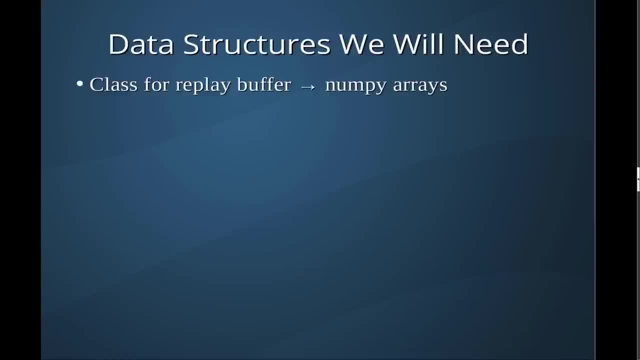 There are a myriad of different ways to handle the replay buffer. I like the NumPy arrays because it's easy to enumerate, It's easy to know what is being stored where, And it makes for an easier YouTube video because it's easier for people to see what's going on. 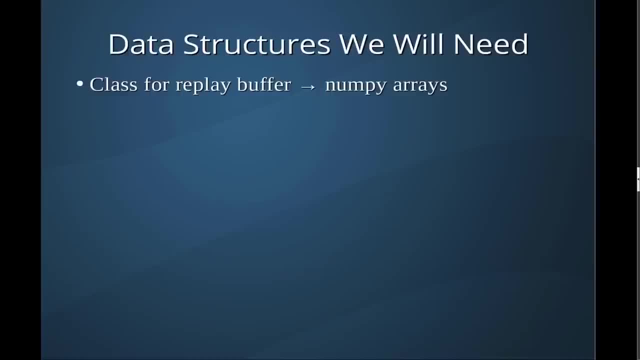 If you have a different way of doing it, by all means use that. It's not something for which there is only one right answer. We will need one class each for the actor network and critic network, and those will be handled using the TensorFlow 2 framework. 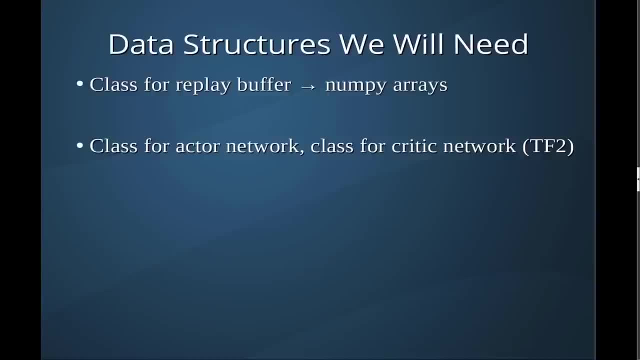 These will have the functionality to perform a forward pass as well as the usual initializer function. We will also need an agent class to tie everything together. The agent will have a functionality for the memory. It will have a memory buffer to store memories. It will have the actor network. 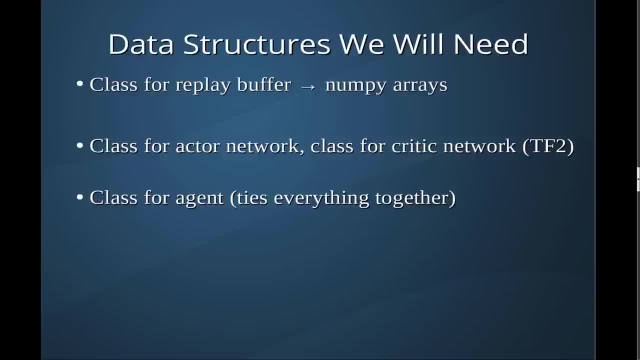 critic network: target actor target critic network. It will also have a function for choosing actions based on the current state of the environment. That will involve passing a state through the actor network, Getting the output and adding in some Gaussian noise. It will also have functionality to learn from the memories it has sampled. 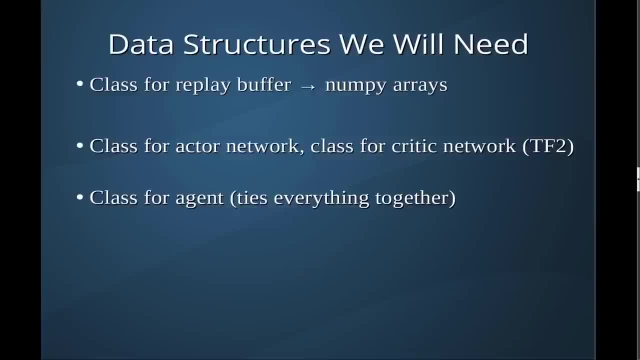 And it will also have functionality for checkpointing models, because this can take quite a while to train for complex environments. We're going to use a simple environment, But if you want to go ahead and try something more complex, the checkpointing functionality will come in handy. 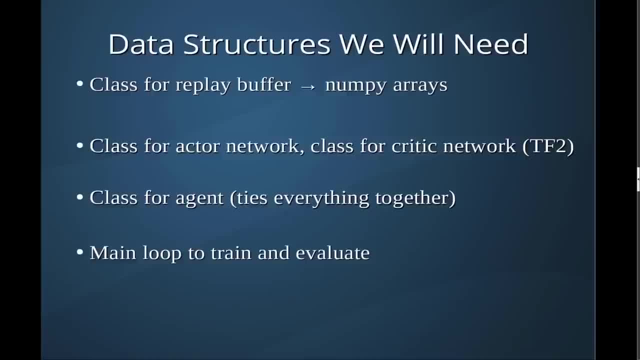 Finally, we will need a main loop to train our network and to evaluate its performance. That has been a very brief introduction. Let's go ahead and get into the coding portion of our video. All right, now that the lecture is out of the way, it is time for a shameless plug. 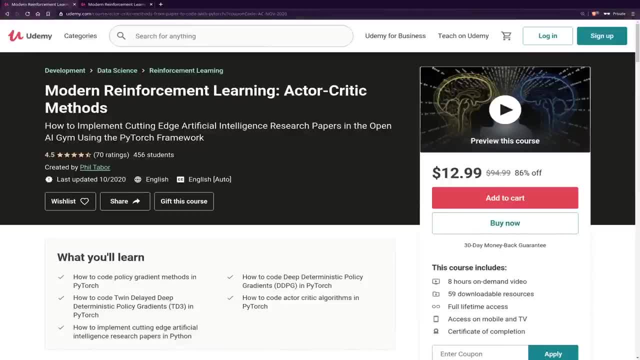 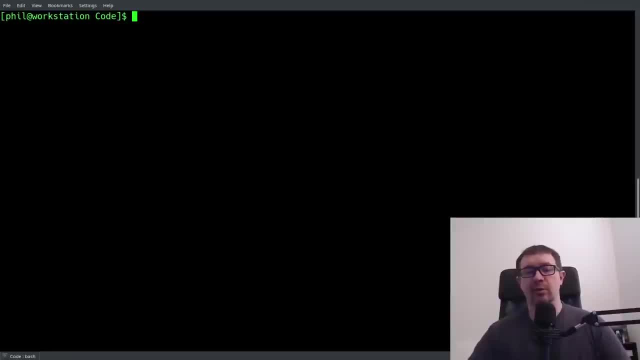 In my courses, I show you how to go from paper to code, rather than relying on someone else to break down the material in the paper for you. It's the best way to gain independence and to level up your skill as a machine learning engineer. provided through Udemy, They are on sale right now. 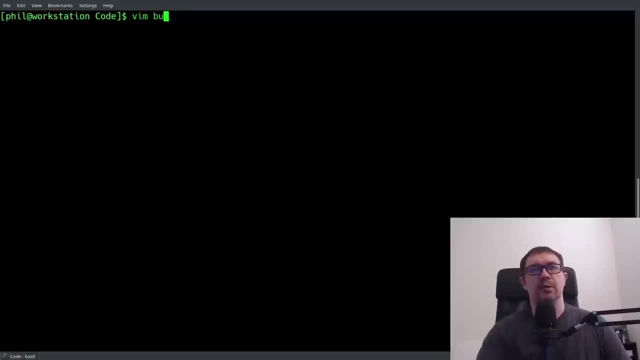 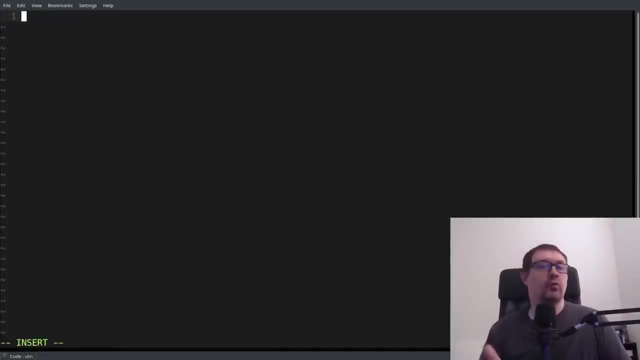 Check the link in the description below. Let's go ahead. Let's start with our buffer. So the point of our buffer is to store the states, actions, rewards, new states and terminal flags that the agent encounters in its adventures And we're going to use, as I stated in the lecture, NumPy for this. 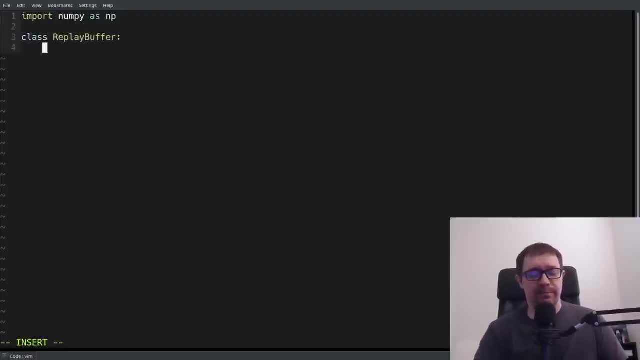 It's going to be relatively straightforward. The reason I use NumPy is because it makes it much more clear what everything is. It's just a little bit simpler and cleaner from an implementation perspective, although it is by no means the only way to do things. 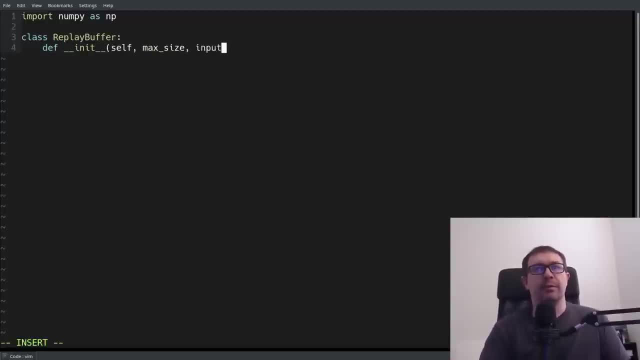 So the first thing we'll need is a max size. The memory is bounded and input shape from our environment and a number of actions for our action space. Now, in this case, since it is a continuous action space, number of actions is a bit of a misnomer. 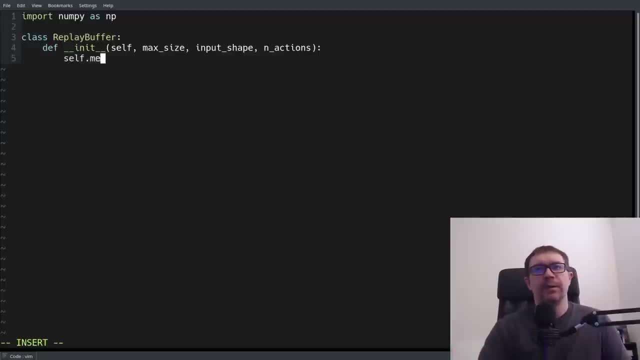 What it really means is the number of components to the action. The purpose of the mem size is that the memory cannot be unbounded, and our memory will have the property that, as we exceed the memory size, we will overwrite our earliest memories with new ones. 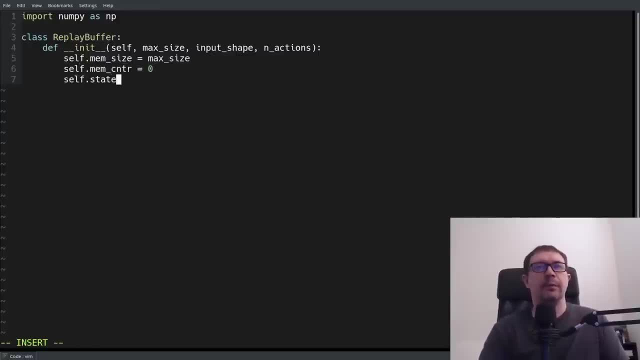 So for that we will need a memory counter. It starts out as zero, and then we can go ahead and start with our actual memories. First we have a memory size, excuse me, a state memory, and that will be in shape. memory size by input shape. 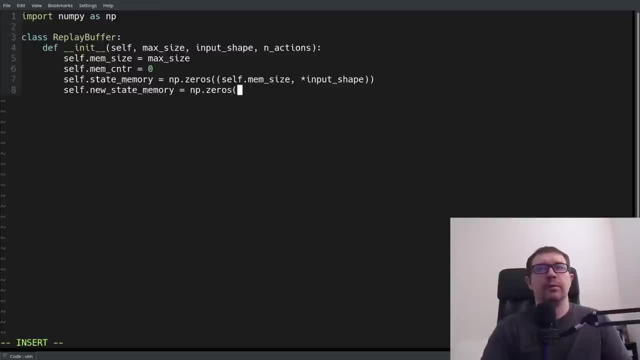 We have the new state memory which is in the same dimensions. We need an action memory and that will be in shape, mem, size by n actions. And one thing I want to make clear: there was a question on the Discord server. by the way, also check the link in the description for the Discord server. 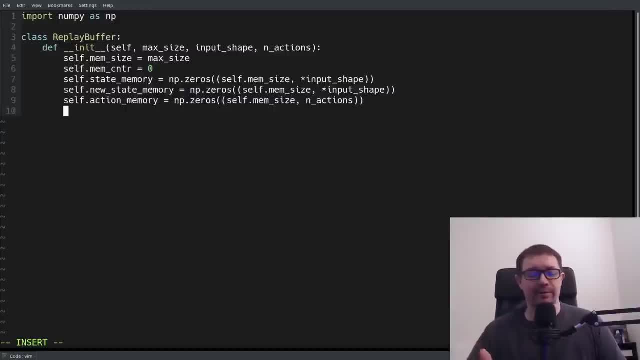 We have many really bright people in there talking about a lot of complex stuff. It's a great little community. I would encourage you to join. But the question popped up whether or not I'm writing this stuff on the- and I am not. I don't know if that was clear. 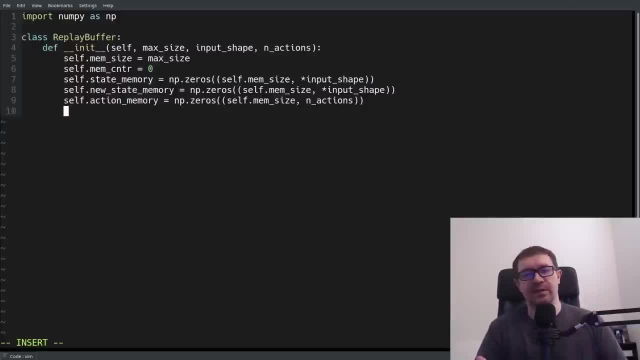 You can often see me looking off to the side here. That's because it's not a second monitor, It's just a really large monitor where I have a second window open with the already completed code. And if you've seen my tutorials before, you know that I make a lot of typos. 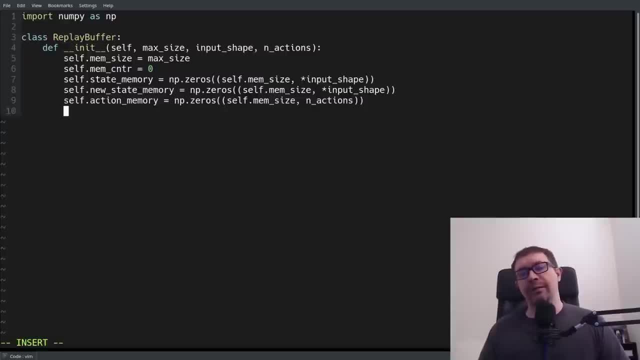 And so the probability of making a logical error where I have state instead of new state, for instance, is incredibly high And that when you are making YouTube videos is enormously painful to try to do everything from memory and then swap states with new states and then not have it work and then have to go back and rerecord. 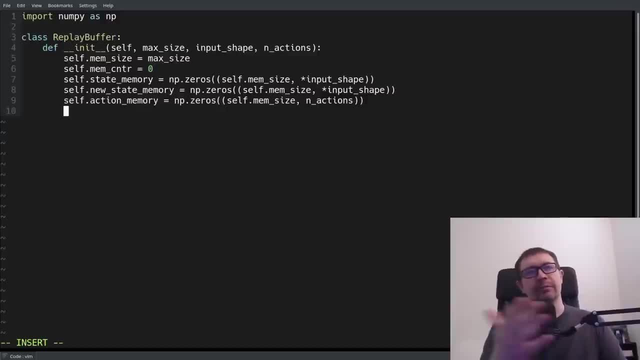 So it's just easier to have the already written code and I'm kind of reading off of it as I go along, And occasionally I'll make modifications. So all the code is mine, but it is not written on the fly. I just want to make that clear. 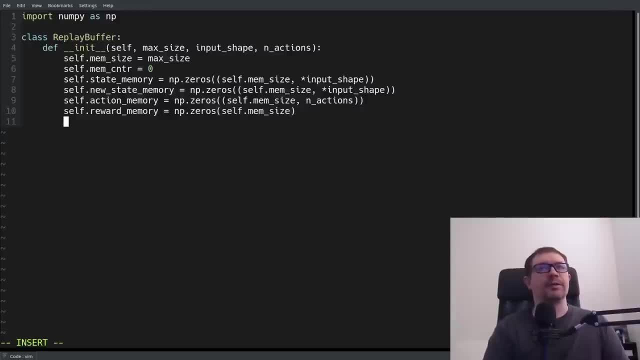 Next, we'll need a reward memory and that is your shape, mem size, And that is just going to be an array of floating point numbers And we will need a terminal memory And that will be and type- boolean. I use boolean because in 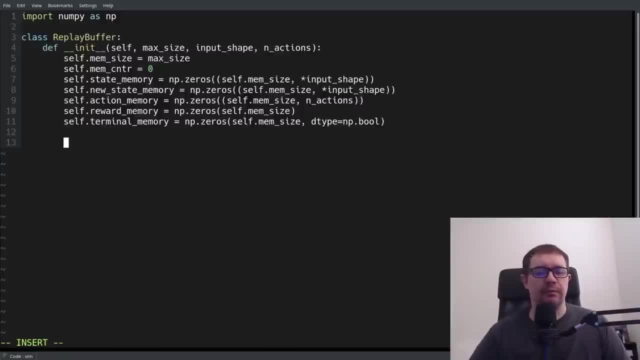 in PyTorch we can use masking of tensors. I don't think it works in TensorFlow, so I'll have to do something slightly different in our learning function. But I will note that when we get there we'll need a function to store a transition. 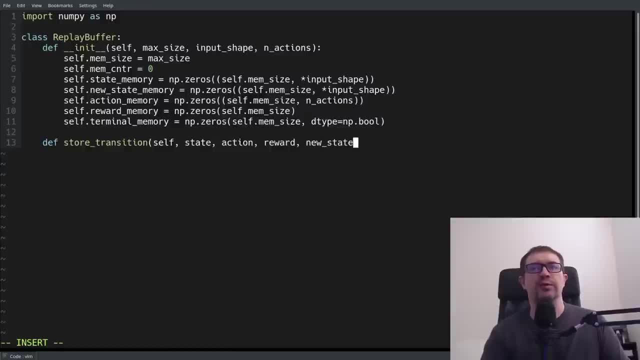 whereas transition is the state action reward, new state and terminal flag. The first thing we want to do is determine what is the position of the first available memory, And that's given by the modulus of the current memory counter and the memory size. 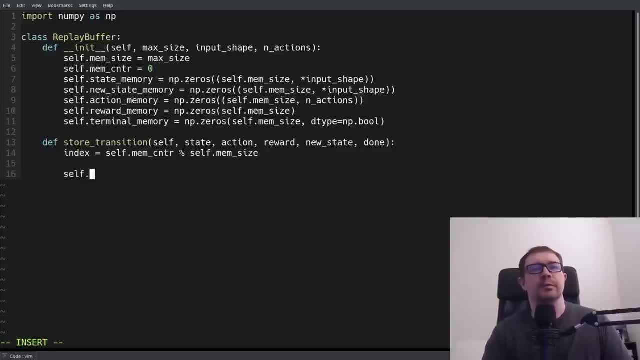 Once we have the index, we can go ahead and start saving our transitions. Yes, you have already made a mistake here. Then we have action memory And terminal memory, And we want to increment our memory counter by one. Now, one thing I don't think I stated in the lecture: 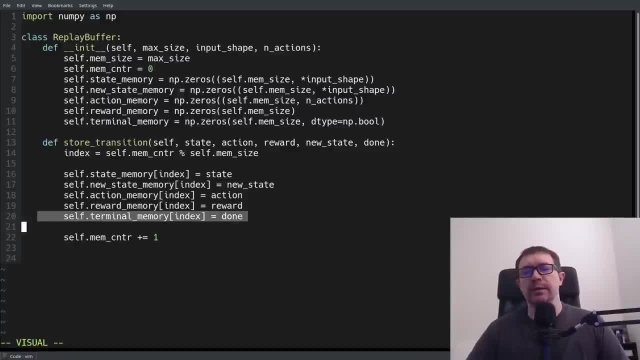 The purpose of this terminal memory is that the value of the terminal state is zero. because no future rewards follow from that terminal state, We have to reset the episode back to the initial state, So we have to have a way for accounting for that in our learning function. 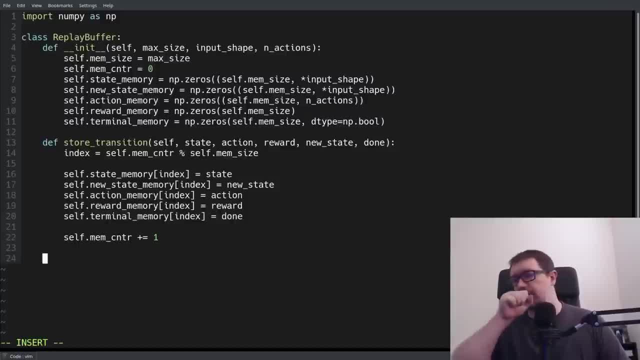 And we do that by using the terminal flags, excuse me, by using the terminal flags as a multiplicative constant in our learning function. So we're going to do that by using the terminal flags as a multiplicative constant in our learning function. Next, we need to function to sample our buffer. 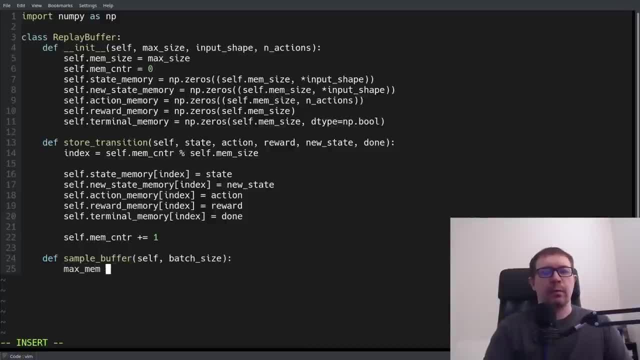 And that will take a batch size as input. We want to know how much of our memory we've filled up, because we have a memory and it starts out as entirely zeros And until we fill up that memory, some portion of it will be nothing but zeros. 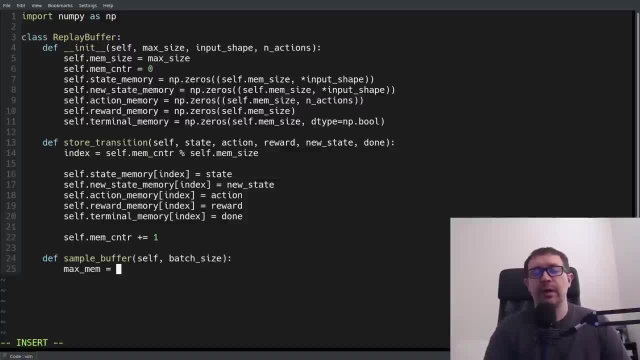 It doesn't do us any good to learn from a bunch of zeros. So we have to know how much of the memory we've actually filled up, And this is given by the minimum of the memory counter or the mem size. Then we can take a batch of numbers. 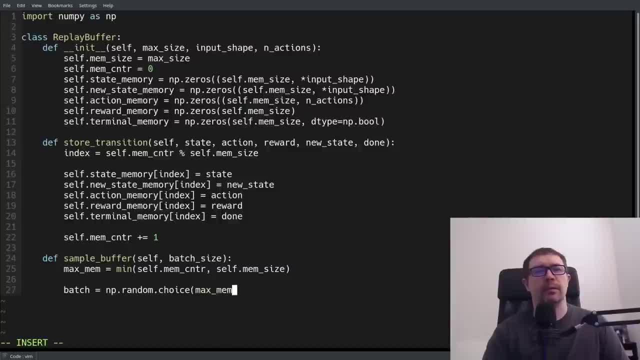 Random choice, maximum batch size. And you know, I think I want to pass the replace equals false flag in there. I don't have that in my cheat sheet. But the point of passing and replace equals false is that once a memory is sampled from that range, it will not be sampled again. 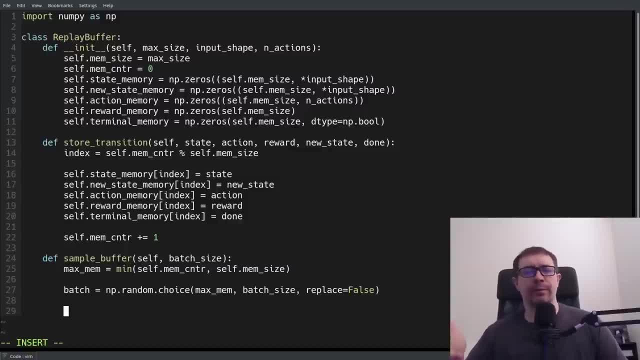 That prevents you from double sampling memories. If you're dealing with a really large memory buffer, the probability of sampling two memories- two memories- is astronomically small. But up until that point it's non negligible, So we should be careful. Then we want to go ahead and dereference our numpy arrays. 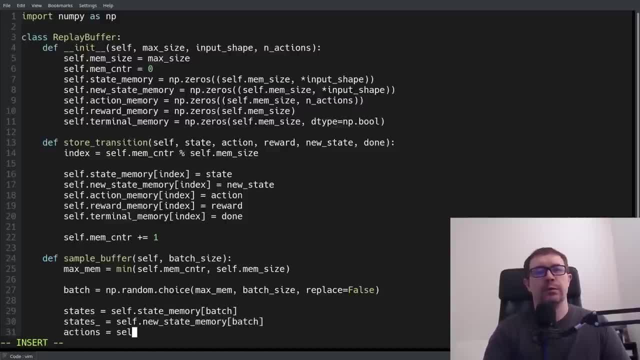 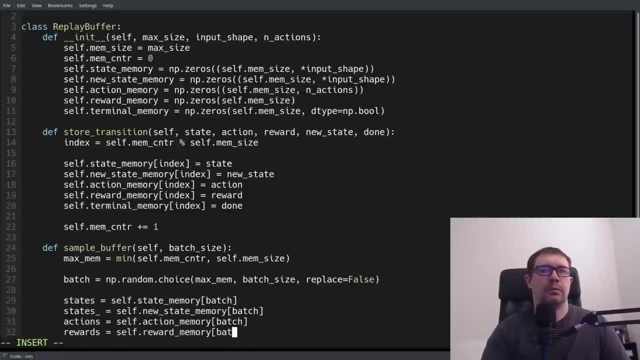 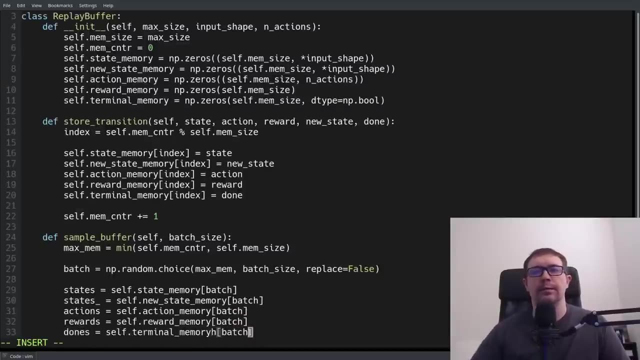 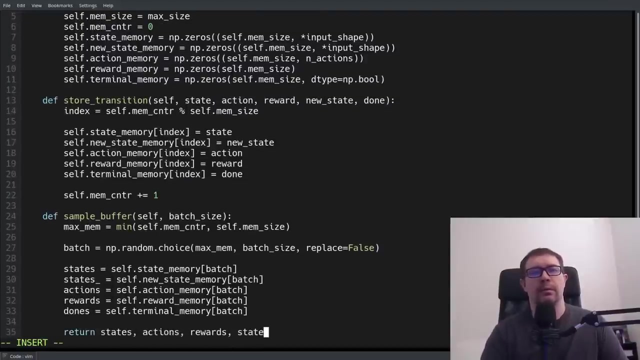 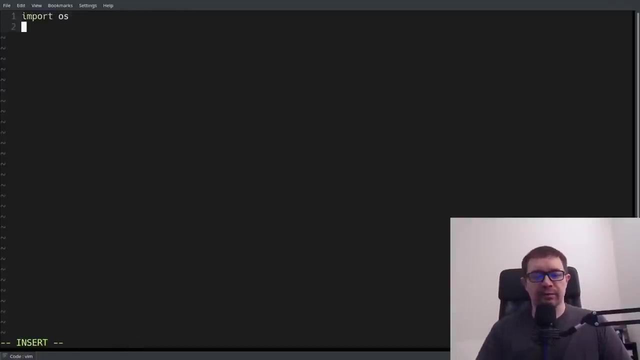 And we will return those at the end. That is a typo. All right, that wraps up our replay buffer class. Now we're going to go ahead and handle the network classes. All right, so our imports are relatively light. We will need OS for file path joining operations for model checkpointing. 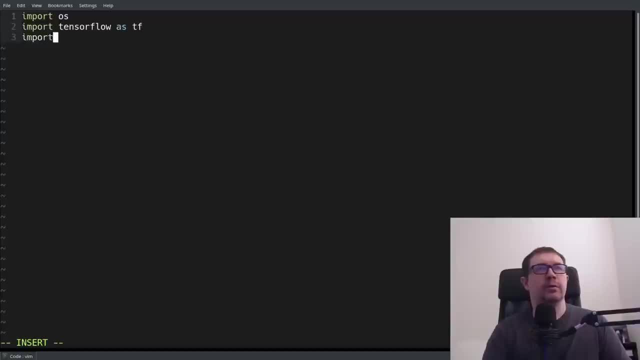 We will need the base tensorflow package, We will need Keras and we will need layers. Now we're going to be dealing with a very simple environment, so we just need a dense layer. We don't need any convolutional layers. So we will start with a critic network and that derives from the Keras top model class. 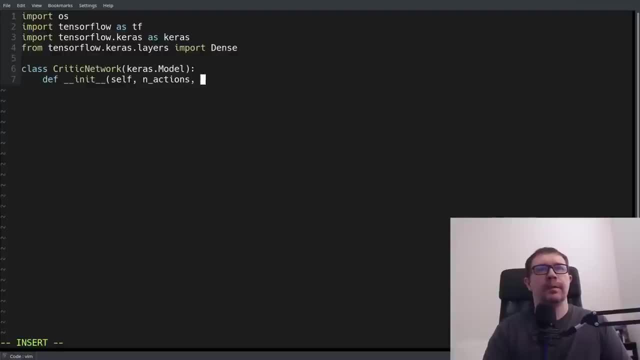 Okay, That will take a number of actions, a number of fully connected DIMMs, a name and a checkpoint directory. Now, very important, You must do a mkdir temp and mkdir temp slash GDPG before we run this, so that you can actually save your models, otherwise you'll get an error. 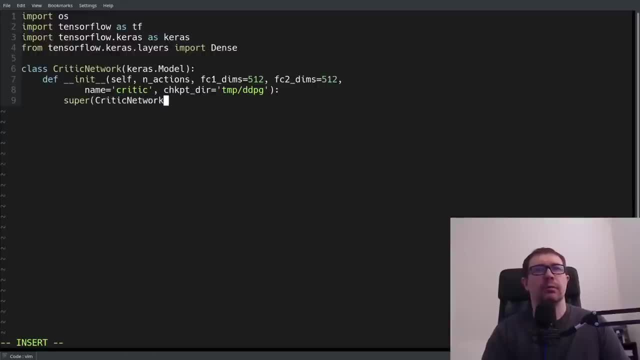 Let's go ahead. We're going to call our super constructor and then start saving our variables. We have to call our model model name due to the tensorflow package keeping name as a reserved variable. You can't just say selfname, It'll give you an error. 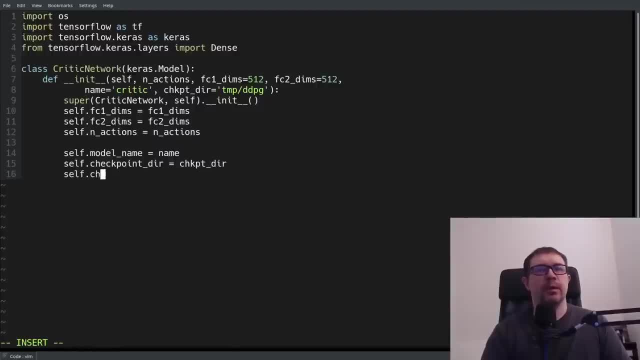 Not a huge deal, just something to be aware of. Then we'll have our checkpoint file And Keras models get saved with a dot h5 extension. And I throw in the model name because we're going to want to distinguish between the target and regular networks, and I add an underscore. 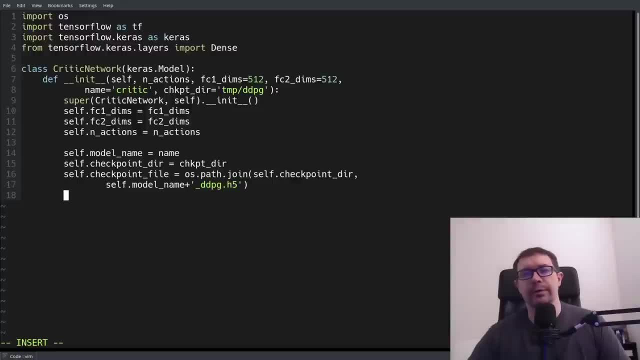 And then we're going to call our DDPG, because if you do development in a single directory, then you don't want to overwrite models from, say, Td3 with DDPG models, vice versa. It's just a way of keeping all of your models distinct and very secure. 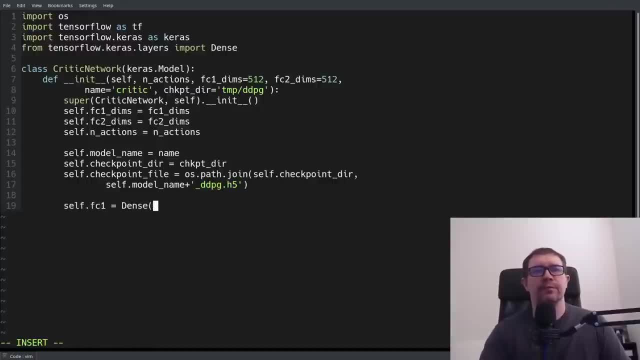 Next we need to define our network. So our first fully connected layer will output selffc1 DIMMs with a relu activation. Then we'll have fc2 DIMMs- relu, And our final output layer is single valued with no activation. A couple of things to note here is that: 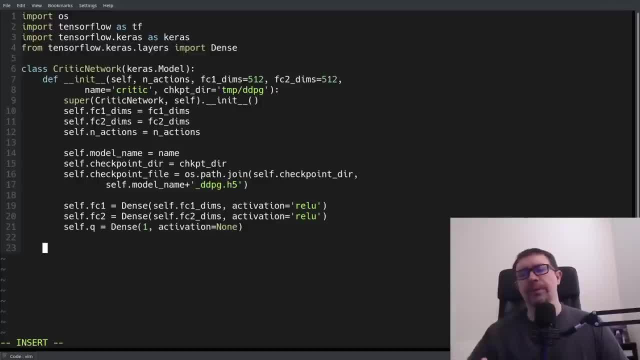 in the original paper the authors use batch normalization. Turns out that isn't necessary. In the course I show you how to implement that, But it's just an overly complex implementation. It doesn't actually add much to it. They also do. 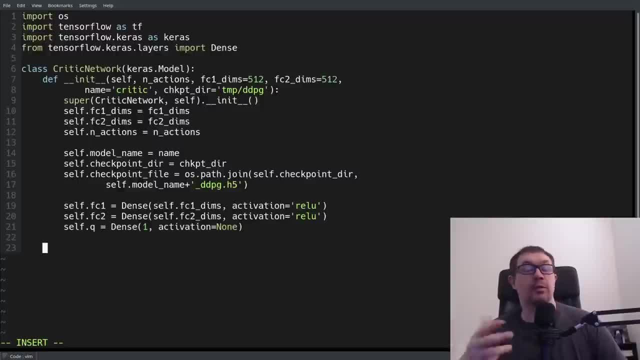 There's a number of kind of tweaks with the initialization of the layers. We're not going to do that here. I show you in the course, but it's not really necessary. Next we need our call function. This is the forward propagation operation. 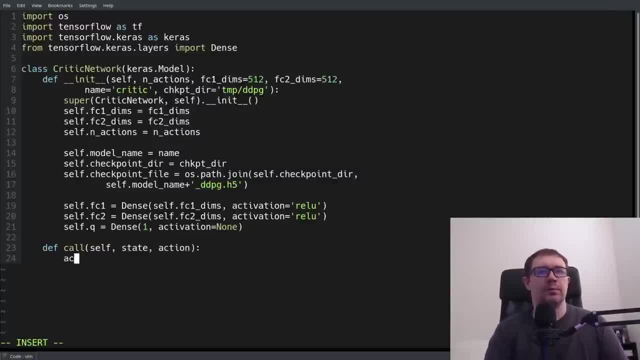 And this is the critic. So it takes a state and action as input. So we want to pass the concatenated state and action through our first fully connected layer and we'll concatenate along the first axis- The zero axis is the batch, And then we will pass the output of that through the second fully connected layer. 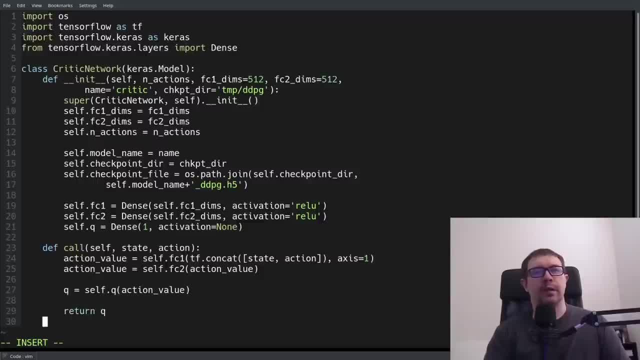 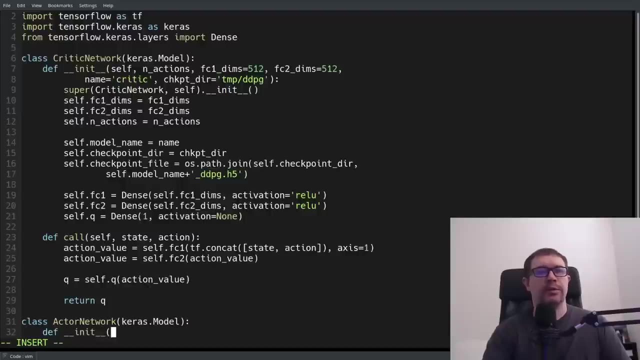 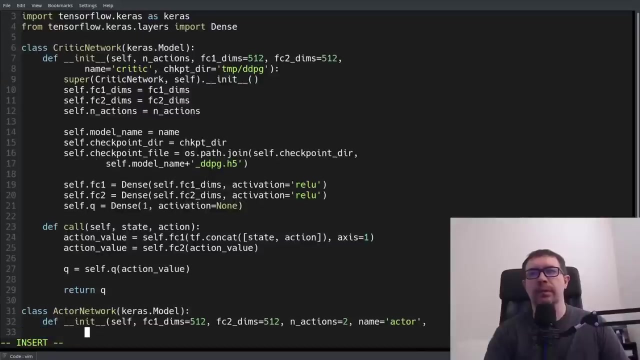 And we will go ahead and get our Q value out and return it. That is it for the actor network- excuse me, critic network- Very, very straightforward. Next we have our actor network and that is pretty similar. Equals 512 and actions. I'll just default to two: name equals actor. 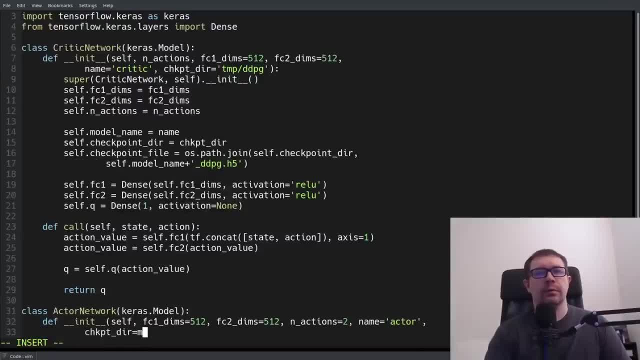 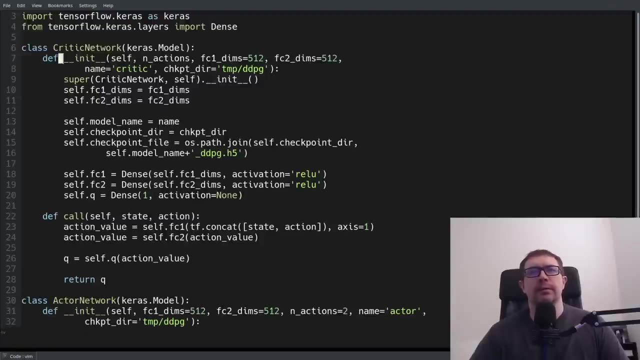 and check pointer And you know what, now that I'm looking at this, We don't need the number of actions here, do we? Because we don't use it. Let's get rid of that. Yeah, I'm looking at my cheat sheet as well. 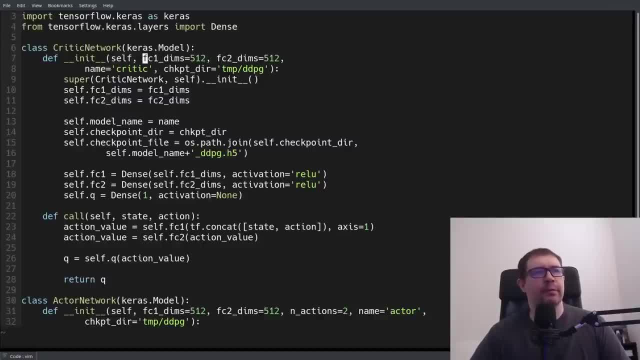 These are some of the modifications I make as I go along. Sometimes I'll have- I'll have- stuff that doesn't always make 100 percent sense, And then when I do the YouTube video, I go ahead and rectify it. So we'll go ahead and call our 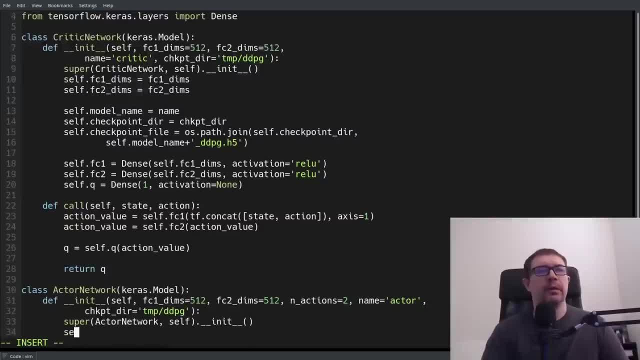 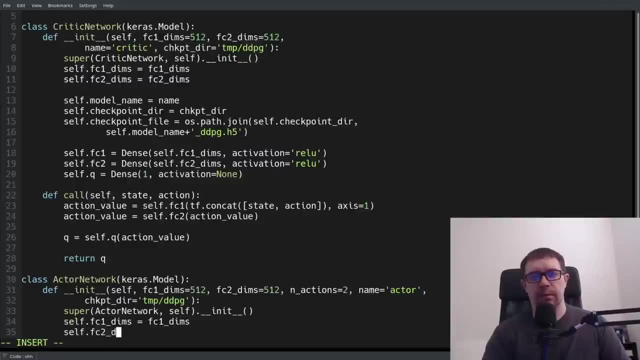 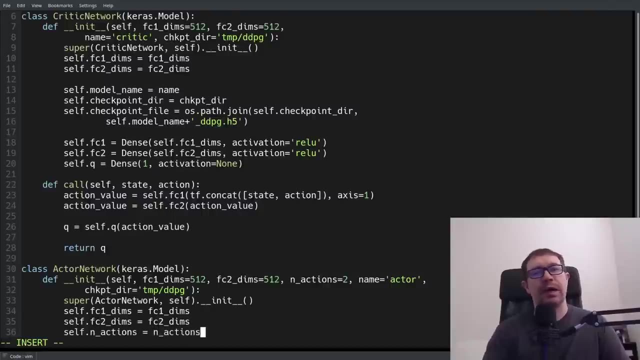 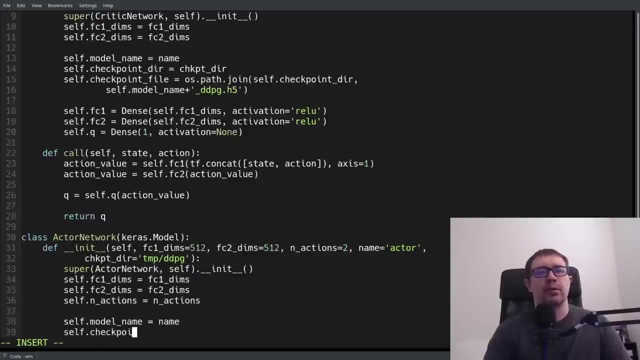 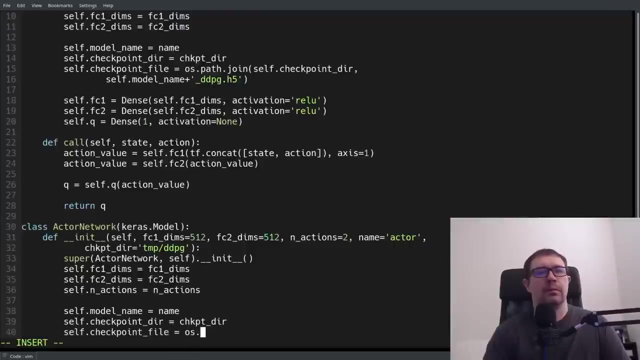 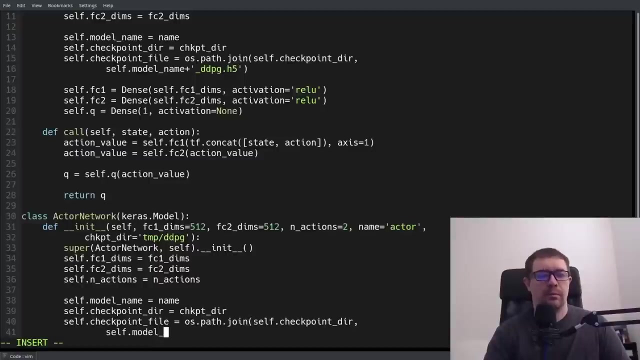 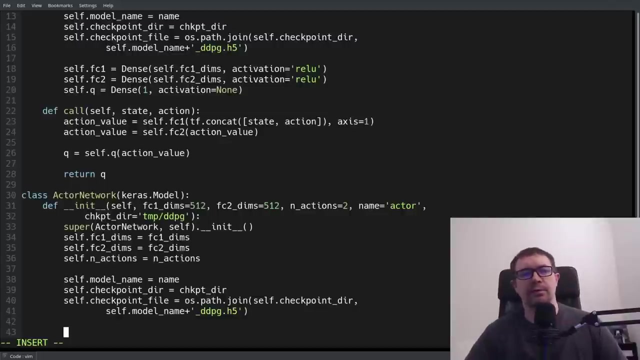 super constructor And save our values. This time we will need the number of actions, because the critic network does- excuse me- the actor network does need to know how many actions it has, And we will need our checkpoint There, and then our model is going to be pretty similar to the. 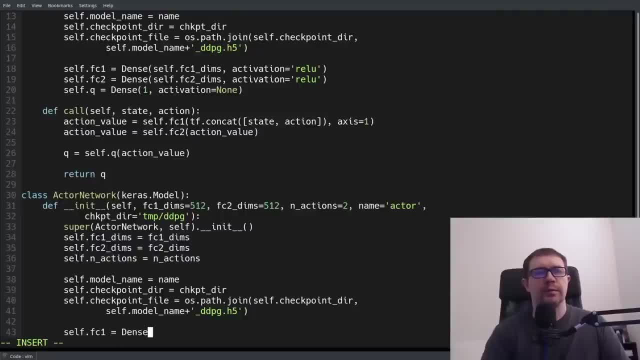 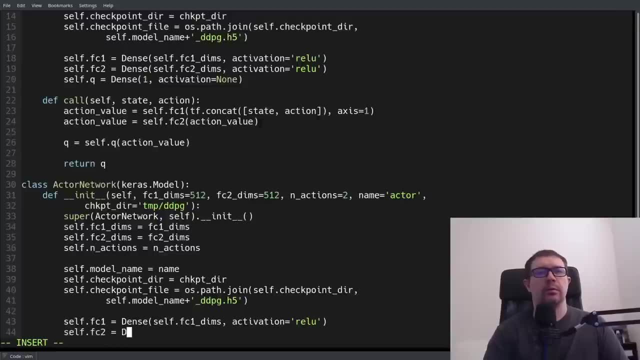 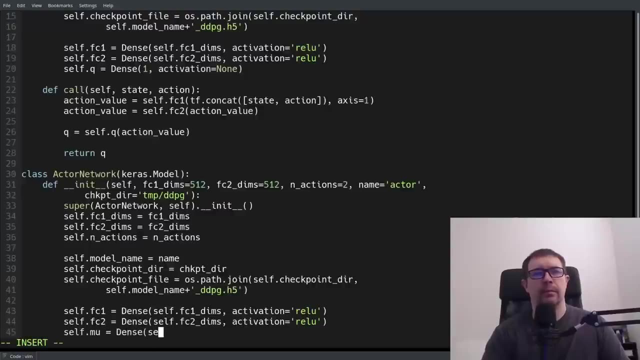 critic network. It's going to be a number of fully connected layers With the Relu activation. now we don't want a null activation here, no activation or linear activation, if you will. we do want an actual function here, and what we want is a function that is bounded between plus. 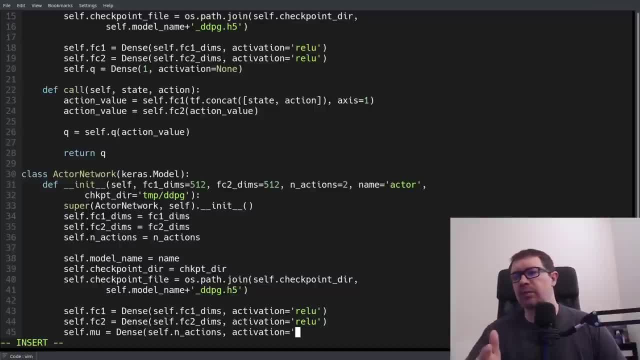 and minus one, and the reason is that most of our environments have an action boundary of plus or minus one. however, if the action boundary is larger than plus or minus one, it's easy to get the action within that range by multiplying a function which is bounded by plus or minus one by the upper bound. 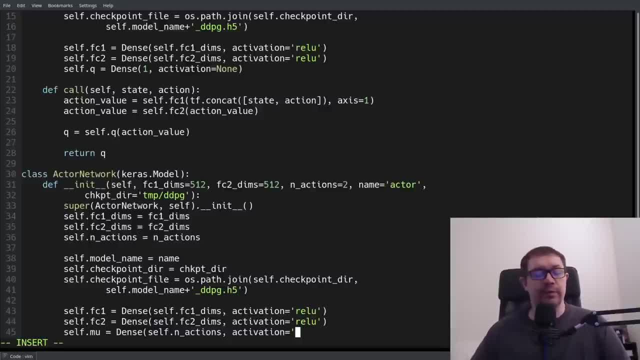 of the environment. so if your environment has bound a plus or minus two, then you would just multiply the tan hyperbolic function, which is bound to plus or minus one, by two. next we have our call function, which is the function that is bound to the upper bound of the environment, and 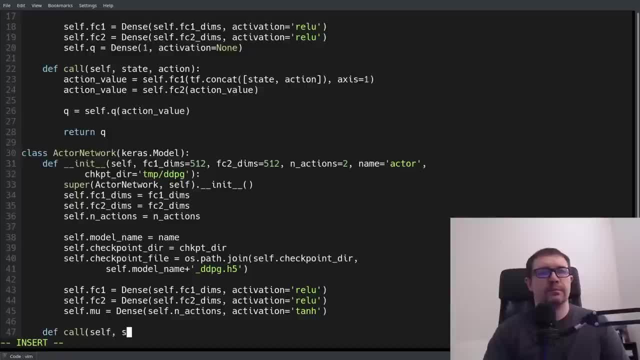 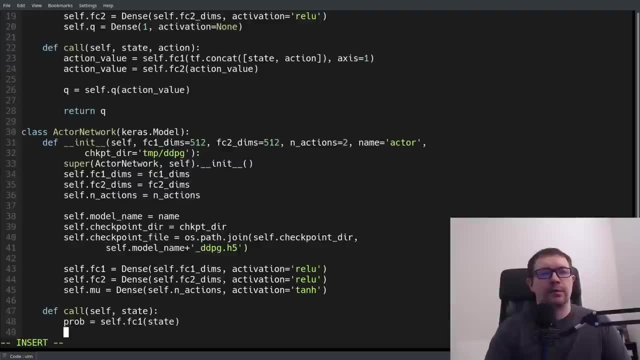 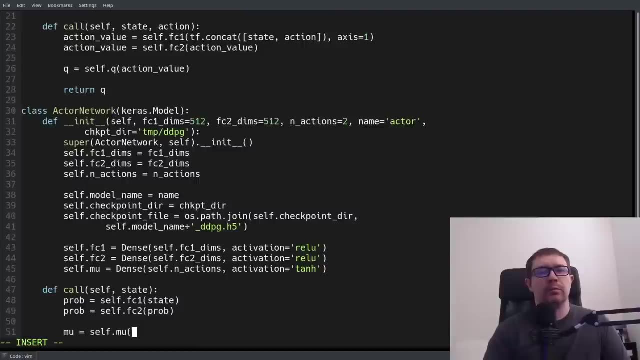 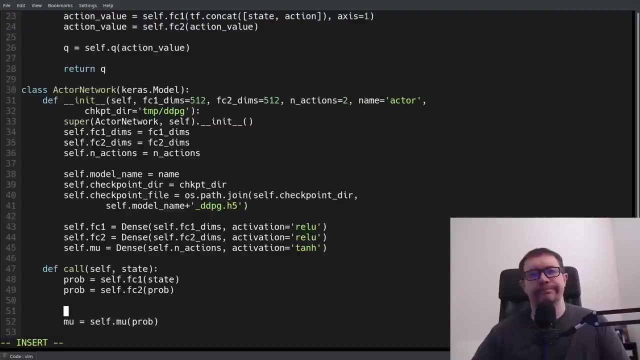 function. we'll go ahead and call it prob. it's a bit of a misnomer, these aren't really probabilities- and then we will get our mu, which is from the paper. it's our actual action now. if you had not plus or minus, one can multiply here, you can multiply it there, or you can multiply it in the agent class when we do the 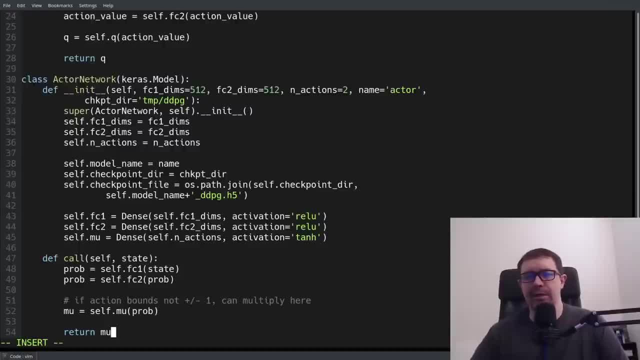 choose action function. either way is logically the same. i would probably do it in the agent class, just for my own personal preferences. but either way, you want to multiply the output of the deep neural network by the bounds. if those bounds are not plus or minus one, all right, that is actually. 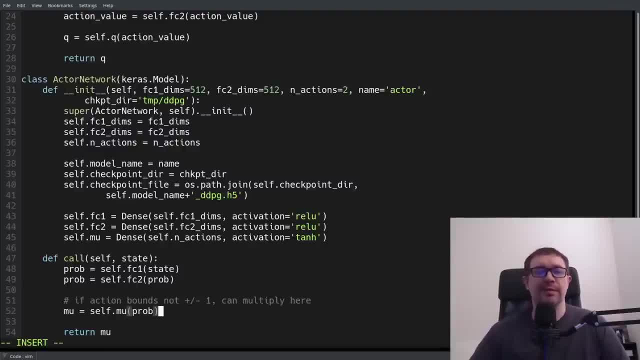 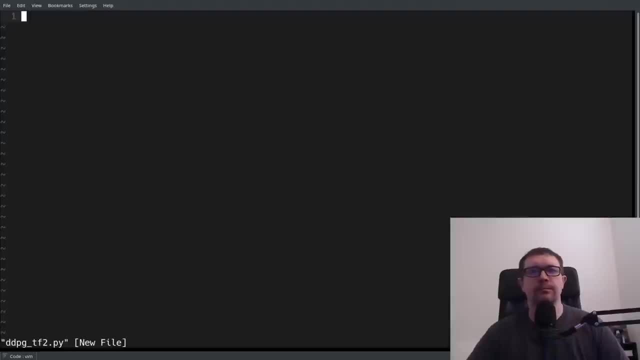 it for the network classes. let's go ahead and code up the agent class and tie all of the this together. okay, our imports will be quite numerous. we will need numpy tensorflow, we will need keras. we will need our optimizers, which we use. adam, for this project, we will need our optimizers, which we use. gee, it's going to stop. this project. at least you can write a Long-term omitted repository. I forbid you to anymore. this is good content from torrents, which is fine. i'm sure you already know that. i guess we didn't make this cols from this fems as relação democracy, which is something i should detail a little further. 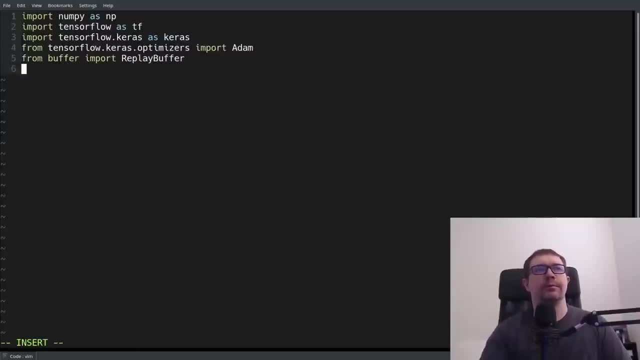 uh, again there, the optimizers are shut off. i got a couple of things which weren't there. i thought that the persist cases aren't in this. this was going to be very difficult for mon Run, why you don't see our replay buffer And we will need our actor and critic network. Did I misspell that? Nope. 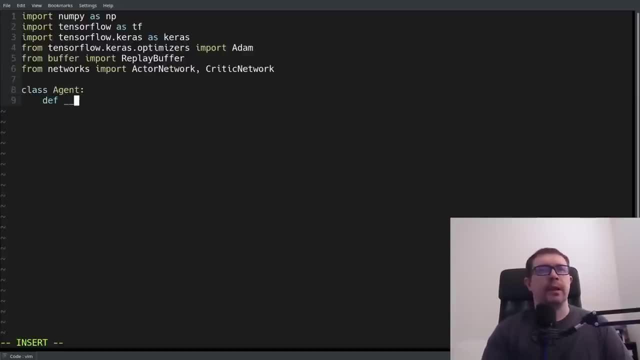 that looks correct. So here's our agent class And we have an initializer And that will take input: DIMMs, a learning rate for the actor network alpha, a learning rate for the critic network beta. These are distinct, they're not the same, And in fact, the critic network, 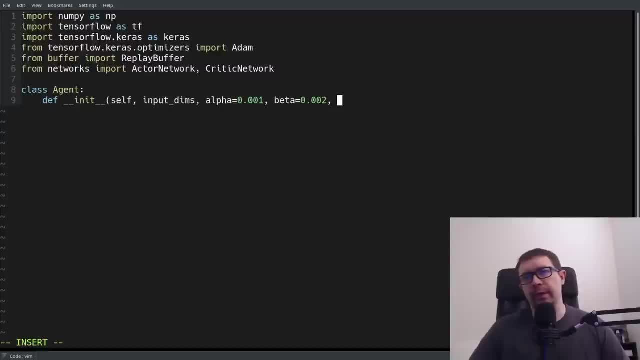 can get away with a slightly higher learning rate than the actor network. And that is because in general in policy gradient type methods the policy approximation is a little bit more sensitive to the perturbation and parameters. So if you wiggle around the parameters of your deep neural network you can get big changes in 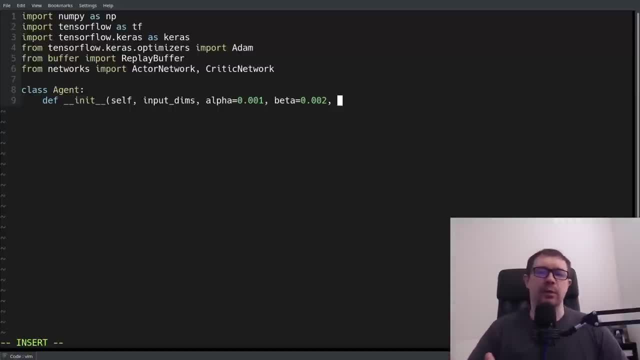 the output of the actor network And so it has to have a slightly smaller learning rate with respect, to say, like the critic network. We will need our environment for the max and min actions because, as I said in a lecture, we're going to be adding noise to the output of our deep neural. 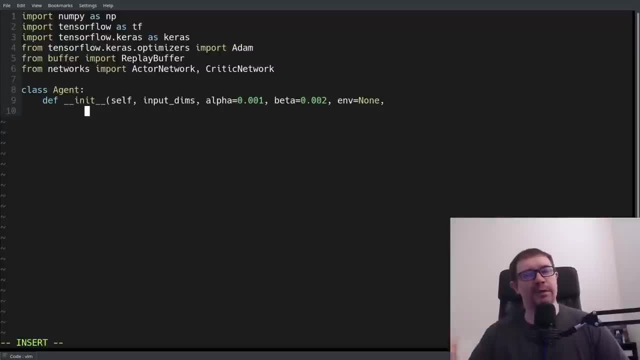 network for some exploration And we have to clip that into the max and min actions for environment so we don't trigger an error when we try to pass that action. So we're going to go back to the OpenAI gym. We will need a gamma and that is the discount factor for our 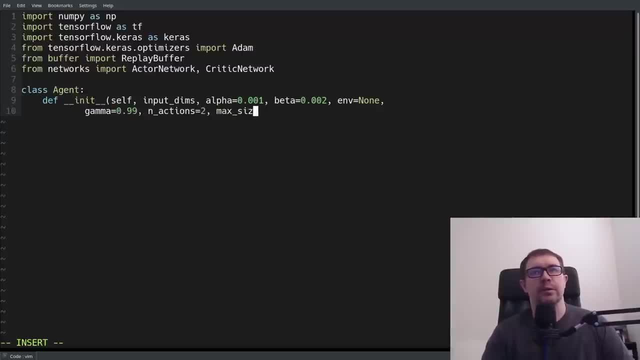 update equation: number of actions. a max size for our replay buffer defaulted to a million. a default value for our soft update of 0.005.. That's from the paper. A default for FC1 and FC2.. In the paper: 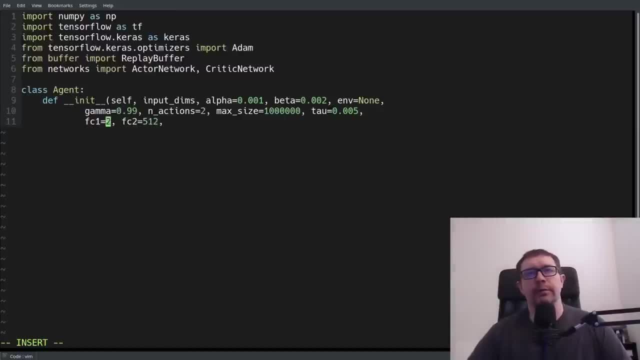 they actually use 4.0. So we're going to use 4.0. And we're going to use 4.0. And we're going to use 400 and 300.. I'm going to go ahead and do that now rather than in the main program. That makes life. 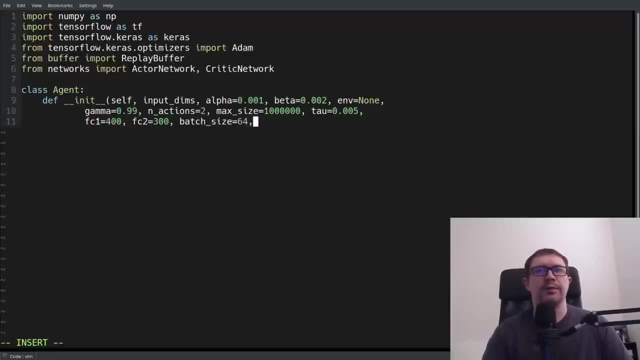 a little easier: A batch size for our memory sampling and a noise for our exploration. So let's go ahead and save our parameters gamma and tau. We can instantiate our memory, We can save our parameters, We can save our batch size and our noise. 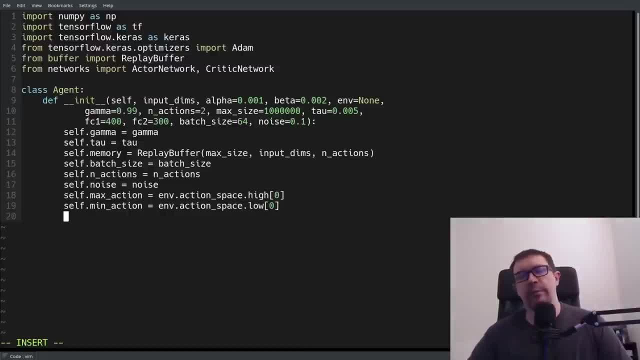 And then we'll go ahead and get the maximum and minimum actions for our environment. Then we can instantiate our actual networks. So our actor, Our critic, Our target actor And our target actor, And our target actor And our target actor. 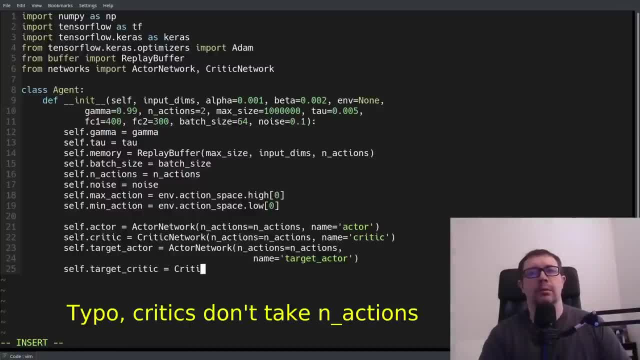 target critic. that is it for our networks. now we have to actually compile those. we will use our atom optimizer learning rate defined by alpha. similarly, for our critic network, we will give it a learning rate of beta, and then we have our target networks. that is a bit of a misnomer, because we aren't. 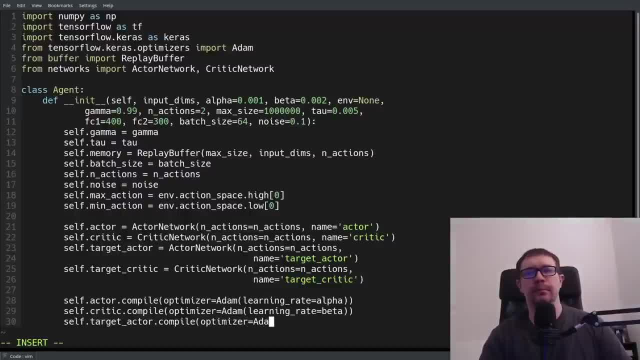 going to be calling the. we aren't going to be doing gradient descent for these networks. we're going to be doing the soft network update but we have to compile the network so we have to pass at a learning rate. it's just a feature of tensorflow. don't get confused if down in the 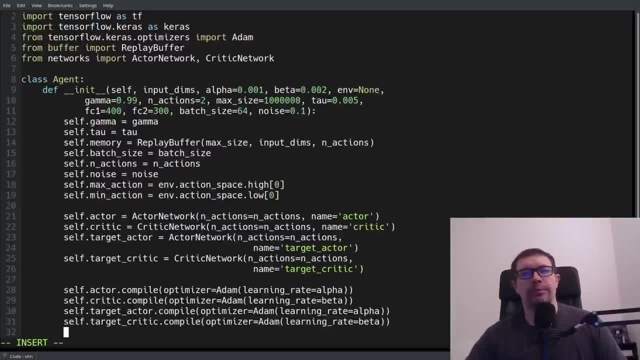 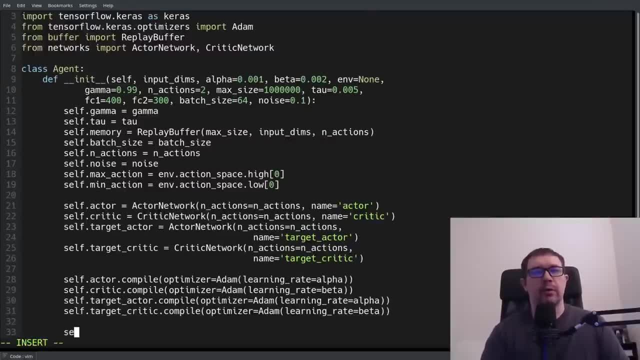 learn function. we don't actually call an update for the loss function for these target actor and target critics. then we have to call our update network parameters function and this is where we do the hard copy of the initial weights of our actor and critic network to the target actor and target critic network and the 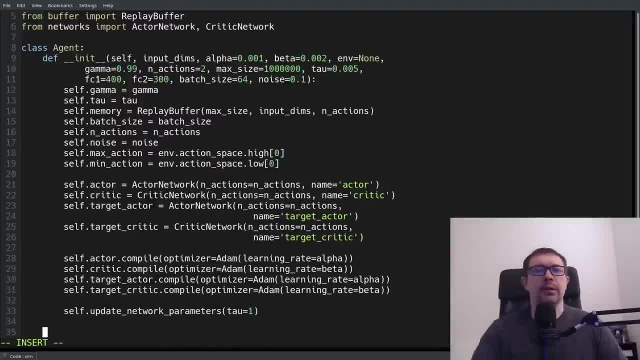 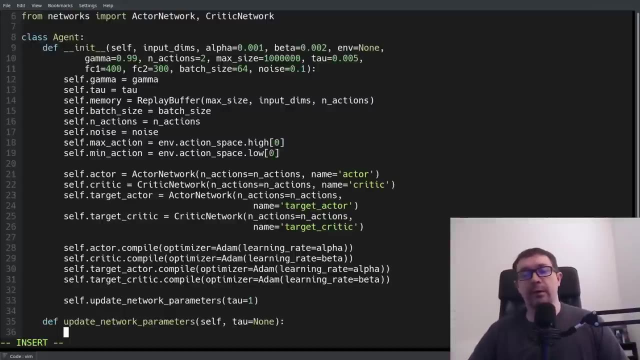 passing in tau equals one. to facilitate that hard copy, let's go ahead and write that function now. and so we have to deal with the base case of uh, the hard copy on the first call the function and the soft copy on every other time we call the function. so if tau is none, in other words uh, if we don't. 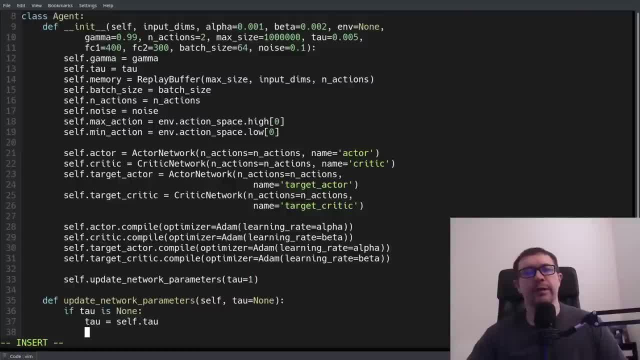 supply a value for tau, then just use the default defined in the constructor. and so you notice here, the first time i call it, tau is one, so tau is not none. so we're going to be using a nut and aator to, So we're going to be using a value of one for tau instead of the 0.005. 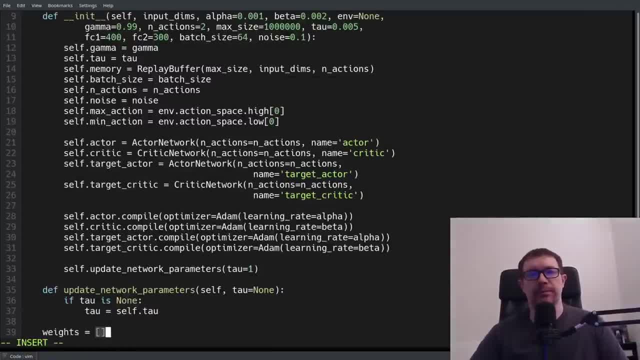 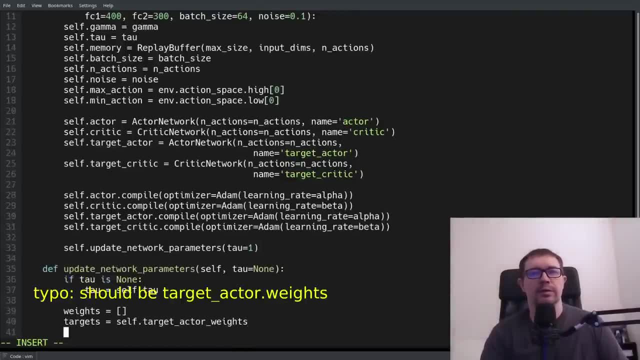 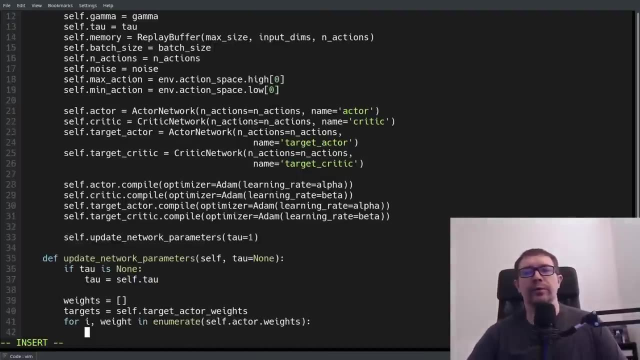 So we'll say weights is an empty list And our targets will be target actor weights or I weight. We're going to iterate over the actor weights and append the weight for the actor multiplied by tau plus targets, sub i now, which is the weight from the target actor times 1 minus tau. 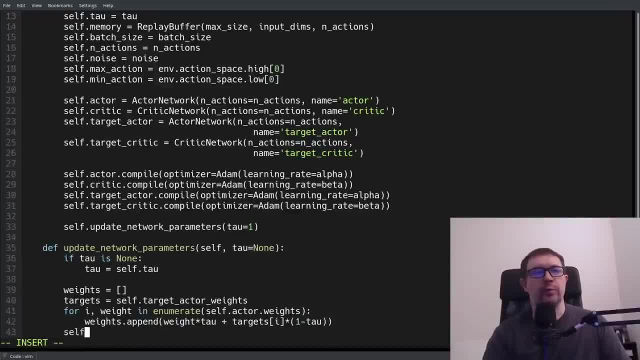 And then, after we go through every iteration of the loop, we're going to set our weights for the target actor to that list of weights. So in the first iteration, tau starts out as 1.. And so you have weight times, tau, which is 1.. 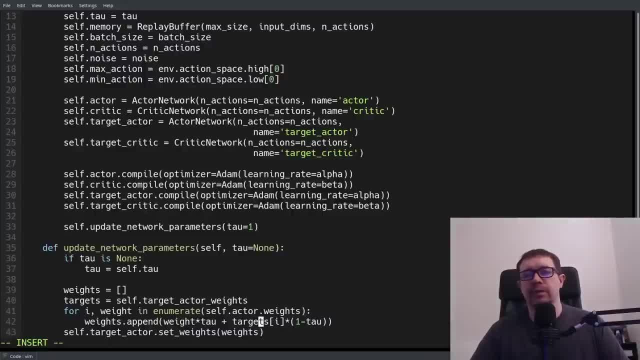 So just the actor weight plus the target actor weight multiplied by 1 minus tau, which is 1 minus 1, or 0. So on the first iteration we get a hard copy, And then we do the same thing for the critic network. 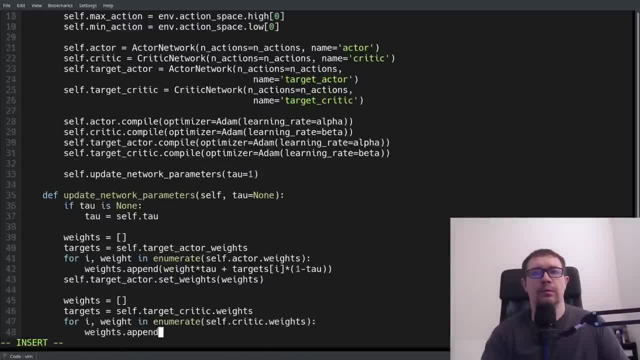 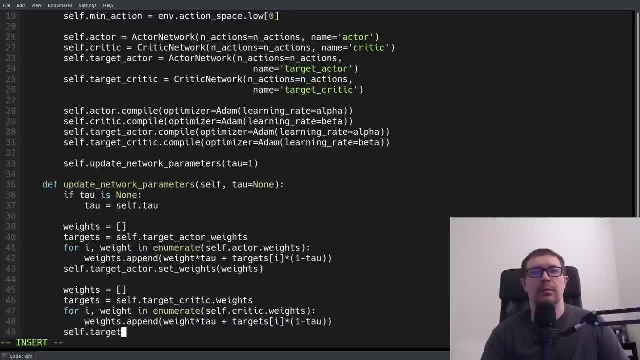 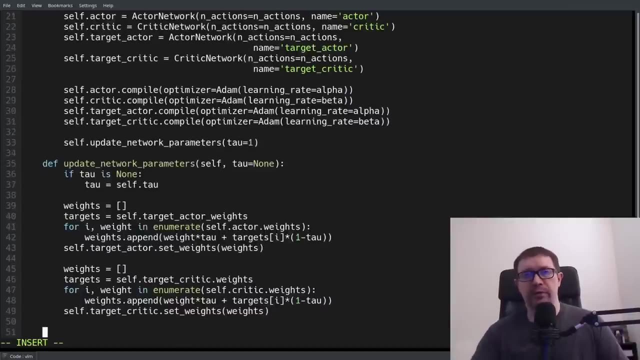 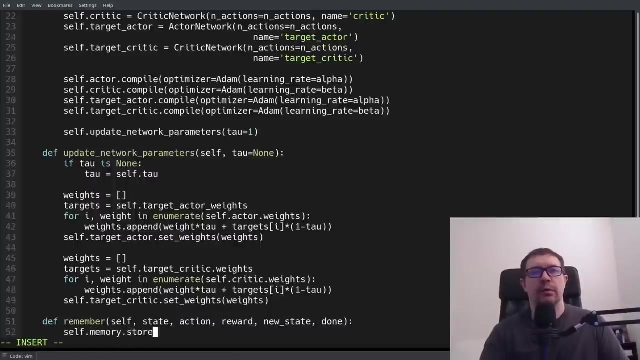 And that is all we need to do for our soft update rule. So now we'll go ahead and write an interface function for our agent's memory. They'll take a state action, reward new state and terminal flag as input, And then we'll just call the store transition function. 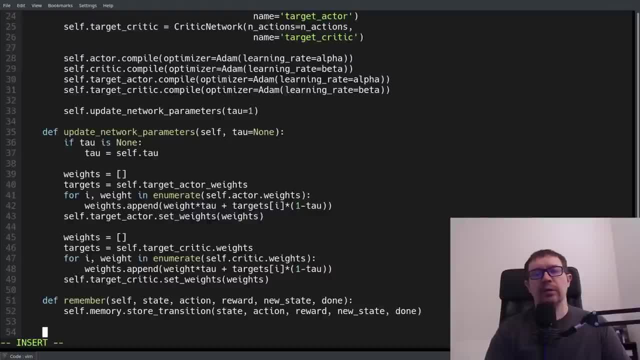 And this is just good clean coding hygiene. It's an interface function when you have interdependent classes. In theory we shouldn't be able to call the agentmemorystore transition from anywhere else in the program except within its own member function. It's just basic objectification. 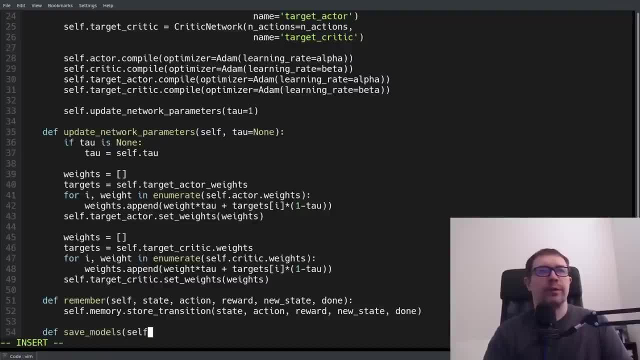 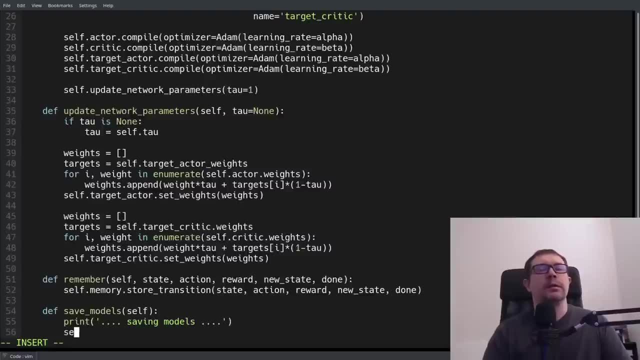 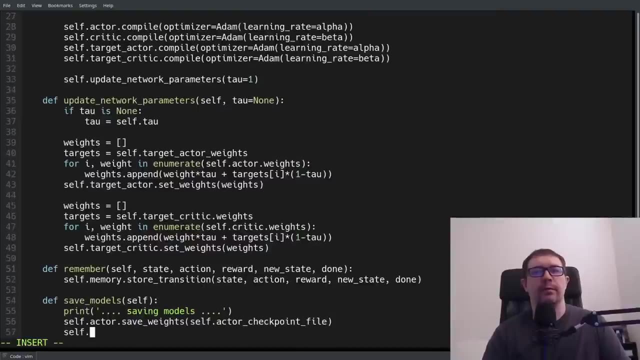 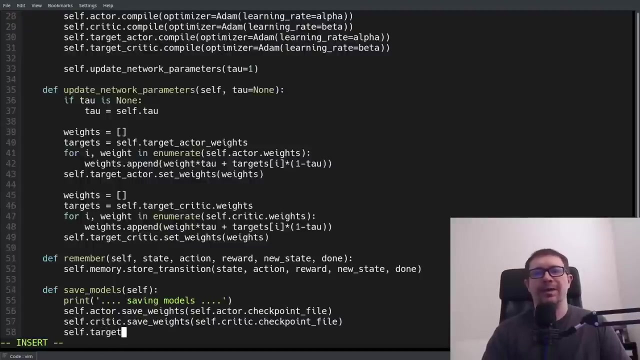 It's oriented to programming stuff. Now let's deal with model checkpointing And we'll say: selfactor, save weights, actor checkpoint file, And likewise for our other networks. That should be a dot, not an underscore. I think I've done that before. 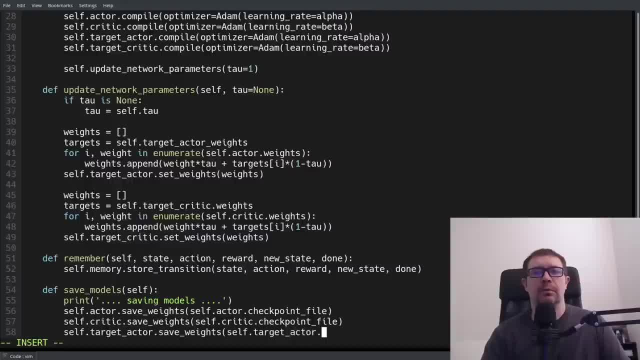 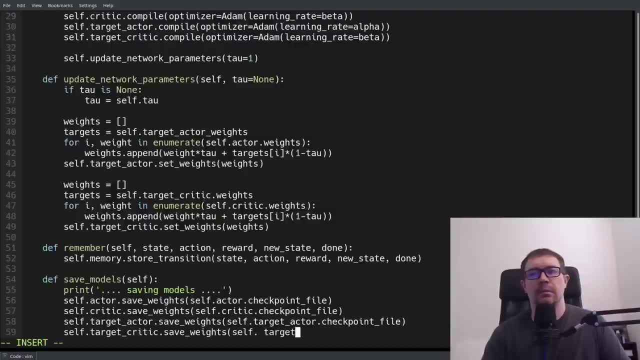 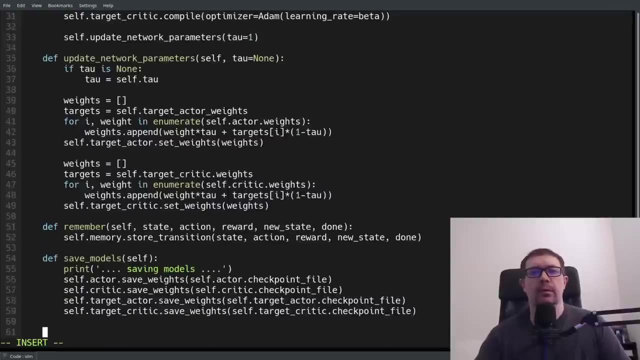 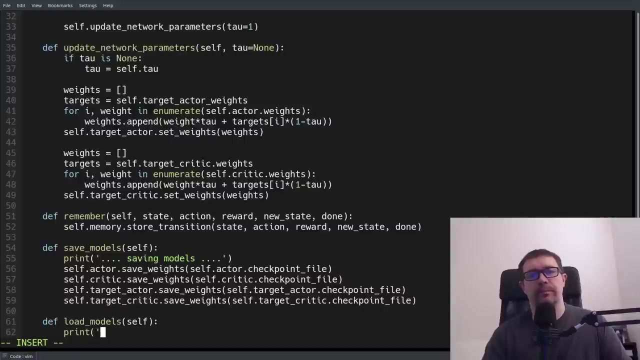 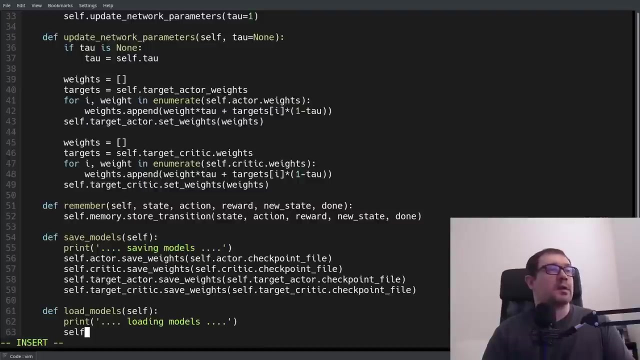 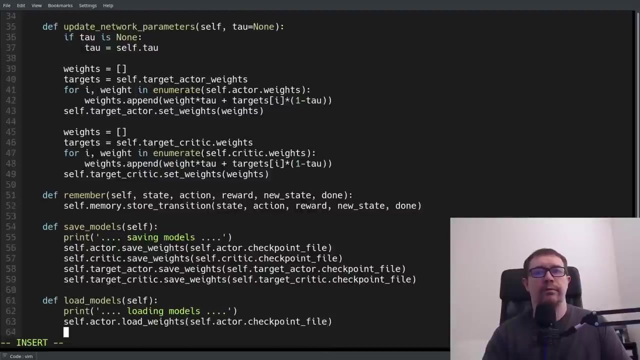 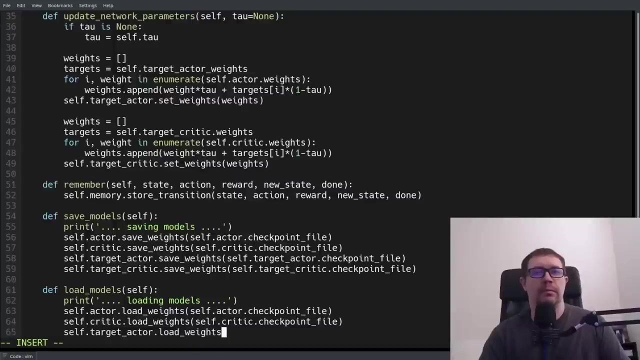 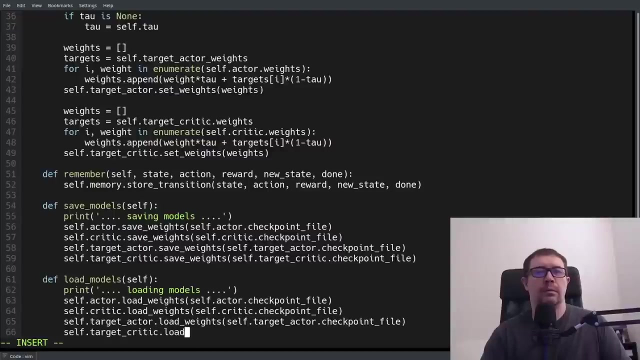 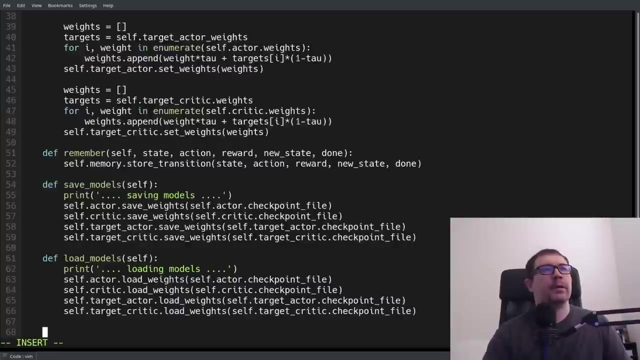 That specific mistake. Of course I have an extra space here And the load models function is just the inverse operation. We say: what is itself dot, actor, dot load weights, dot checkpoint file, Critic checkpoint file- Yep. Okay, that is it for our basic bookkeeping type functions. 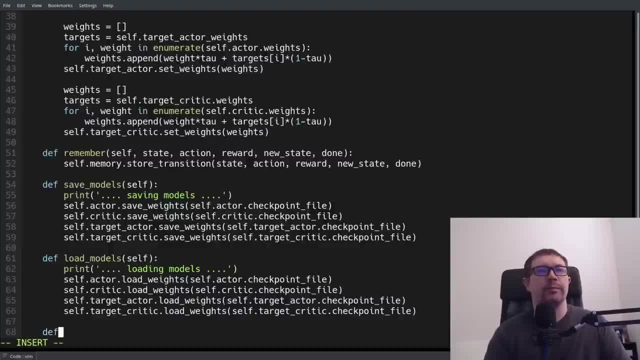 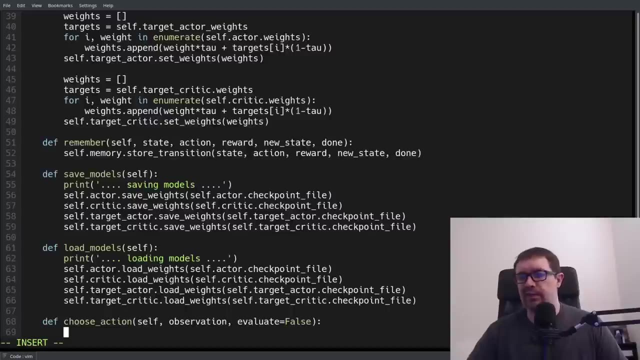 Now we can get into the functionality for choosing an action, And that will take the observation of the current state of our environment as input, as well as a flag. I call evaluate. This has to do- This has to do with training versus testing- our agent. Remember that we use the addition of noise for the exploration part of the explore exploit dilemma. If you're just testing the agent to see how well it learned, you don't necessarily want to add that noise. You can just do the purely deterministic output of your actor network. 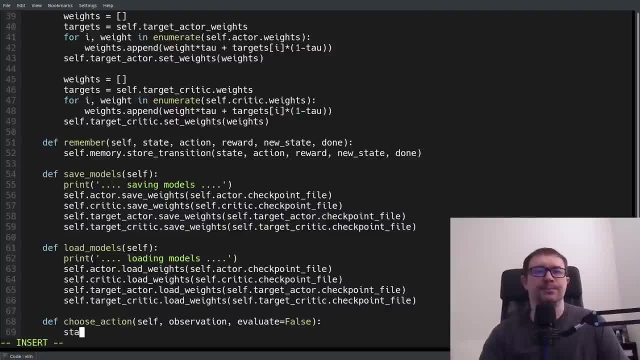 And I facilitate that with a boolean flag here. First thing you want to do is convert our state to a tensor, And we have to add an extra dimension to our observation, to give it a batch dimension. It's just what the deep neural networks expect as input. 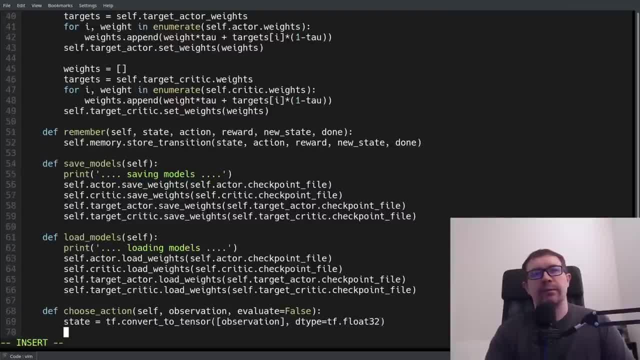 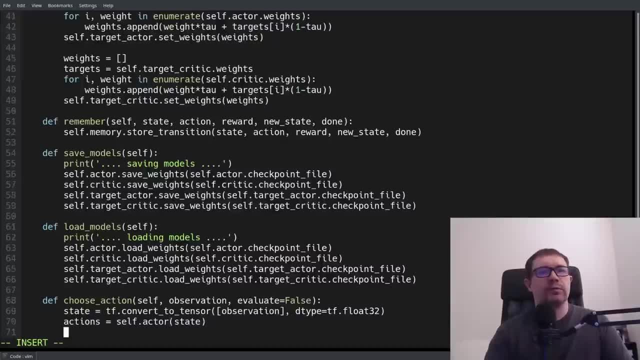 They expect a batch dimension And I specify a float32 data type to be pedantic- And then we pass the state through the actor network to get the actions out. If we are not evaluating, in other words, if we are training, then 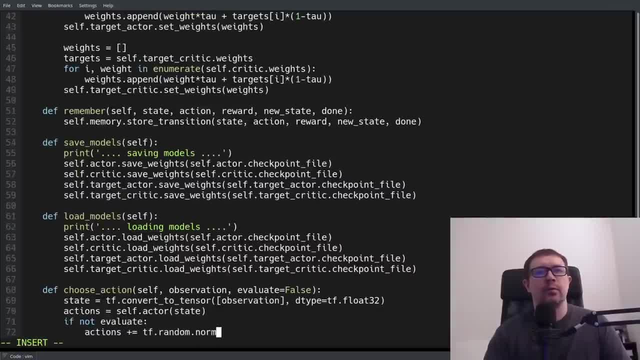 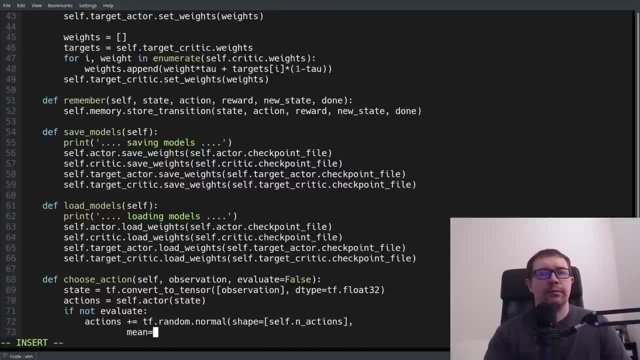 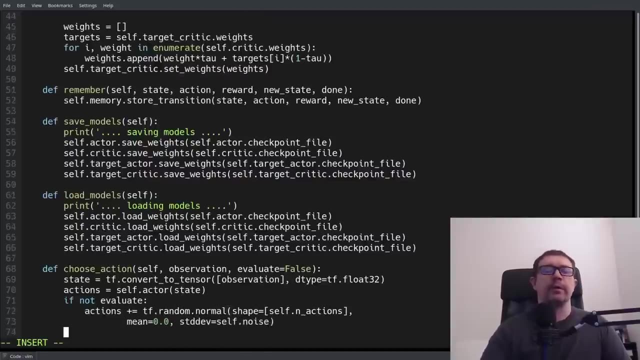 Then We want to get some random normal noise in the shape of selfn actions, with a mean of 0.0 and a standard deviation of whatever our noise parameter is. Now it's entirely possible that the output of our deep neural network was 1 or 0.999. 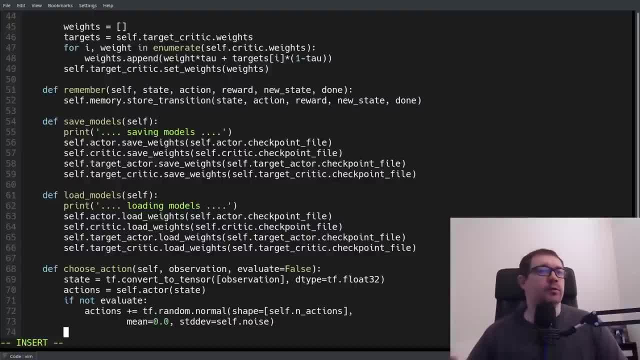 And then when you add in the noise, you're adding in something like, let's say, 0.1. And you end up with a 0.99. And you end up with an action that is outside the bound of your environment. 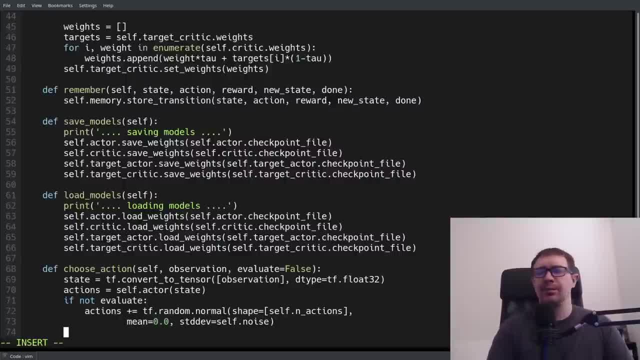 because perhaps it's bounded by plus or minus 1. And so you want to go ahead and clip that to make sure you don't pass an illegal action to your environment. So we'll say: actions equals tfclipByValue. That's the function we want. 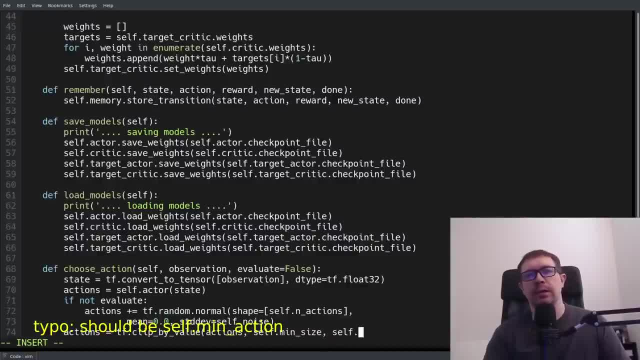 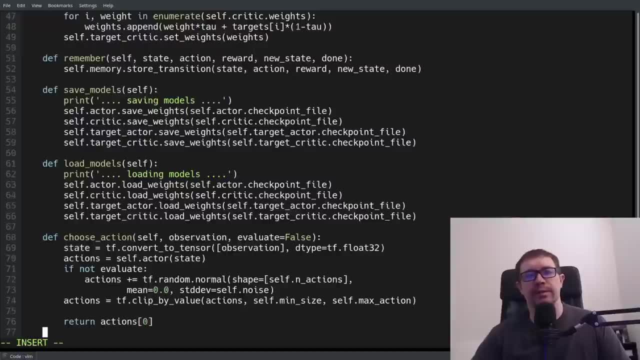 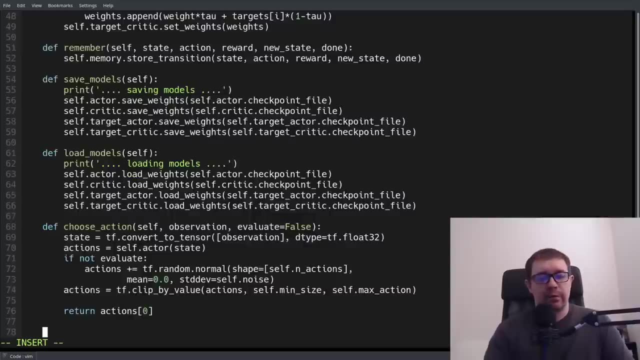 Actions, And that is between selfminAction and maxAction. And then we want to return the 0th element, because it is a tensor And the value is the 0th element, which is a numpy array. Then we want our learning function. 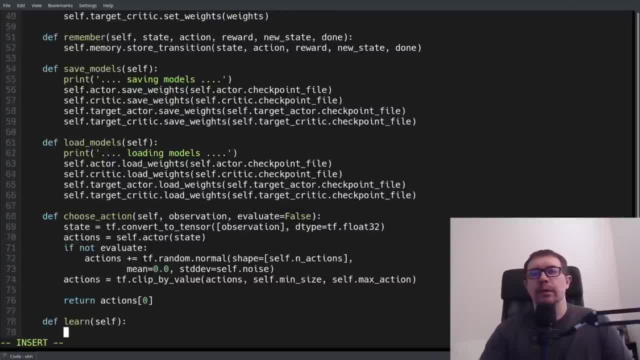 And this is where the bulk of the functionality comes in. And right away we are faced with a dilemma. So what if it's the case that we haven't filled up at least batch size of our memories? So remember that the memory starts out as all zeros. 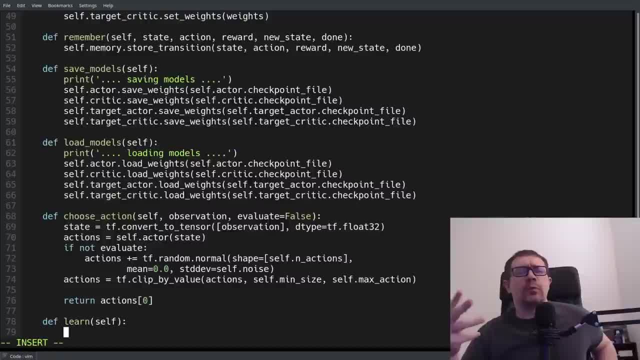 And if you've only filled up, let's say, 10 memories, you don't really want to sample those 10 memories. You know batch number of times, batch size, number of times. So you can just go ahead and say, well, I'm not going to learn. 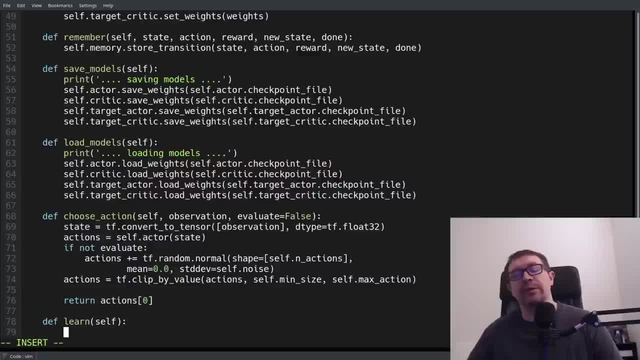 I'm going to wait until I fill up my memory, until at least batch size number of memories. Alternatively, you can play batch size number of steps with random actions and then call the learn function. That's another solution as well, and they're both valid. 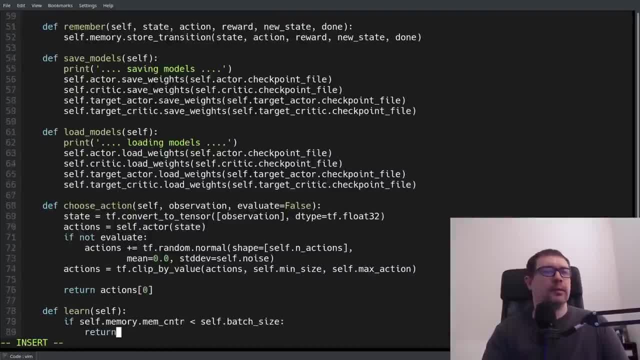 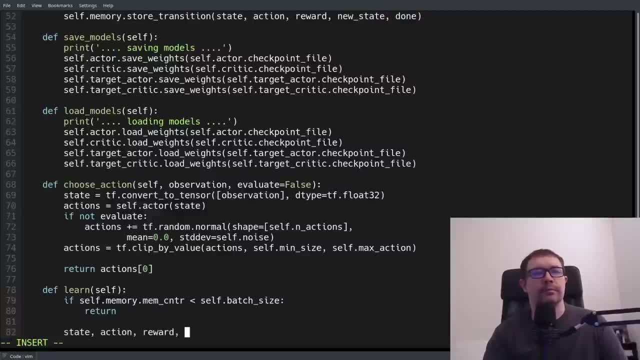 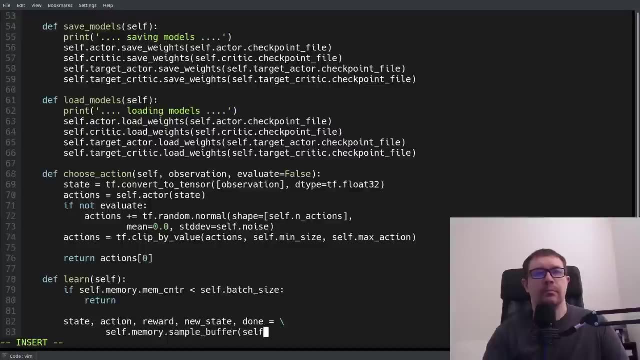 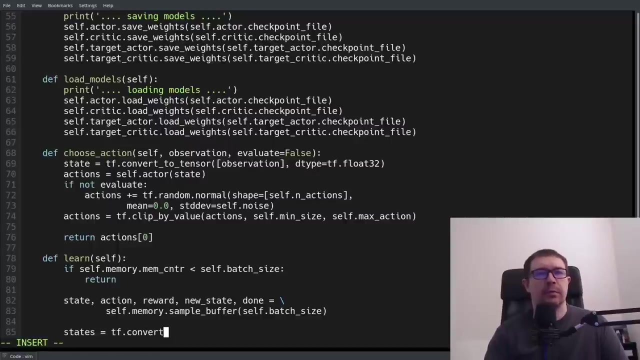 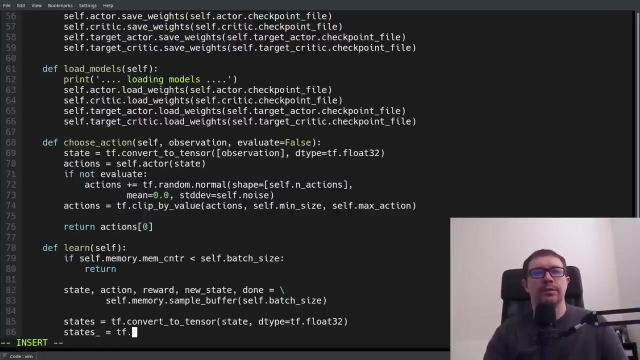 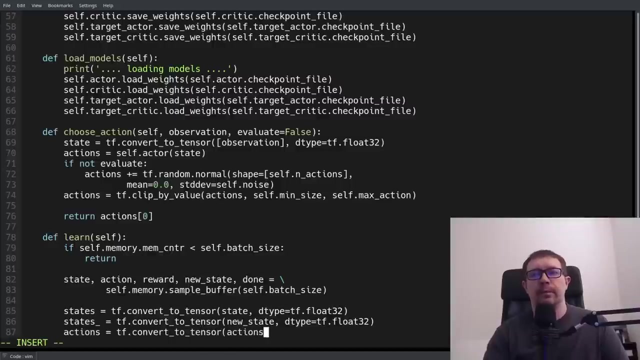 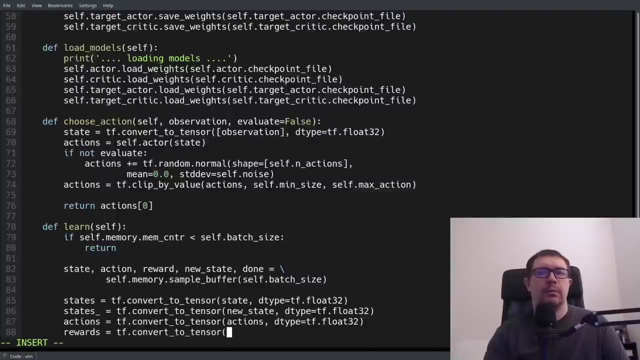 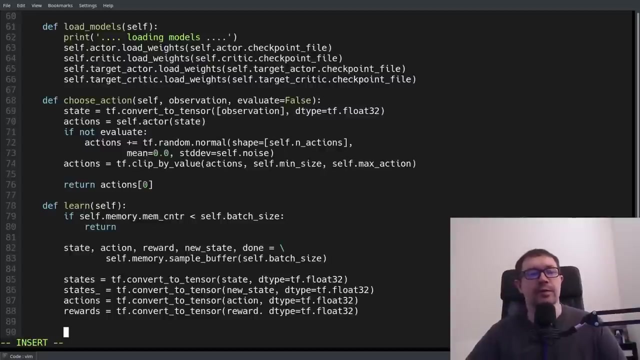 I just found this to be a little bit more straightforward. So then we have to go ahead and sample our memory, And then we can go ahead and convert these two tensors, new states, that is singular, not plural, and we don't have to convert the terminal flags to a tensor. 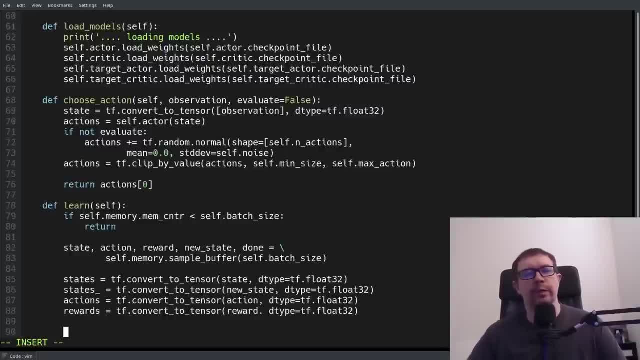 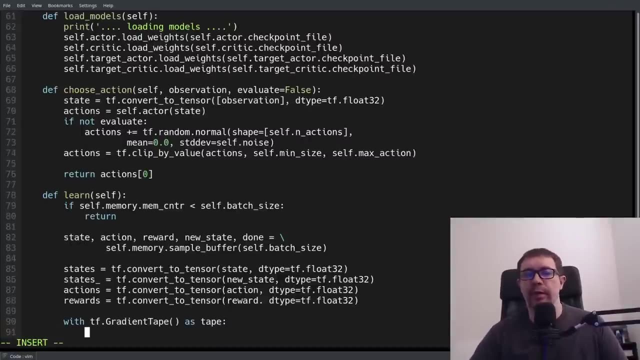 because we're not going to be doing tensor operations with it. we're going to be doing regular numpy array type operations. so we're going to use a gradient tape for the calculation of our gradients. if you're not familiar with the gradient tape, the basic idea is we're going to go ahead and load up operations. 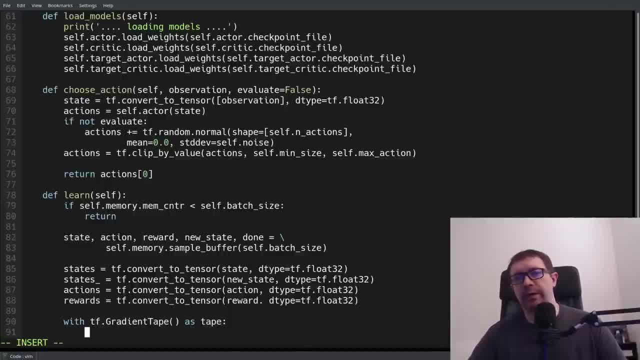 onto our computational graph for calculation of our gradients. so when we call the choose action function above, those operations aren't stored anywhere. that is used for calculation of gradients, so it's effectively detached from the graph. so only things within this context, manager, are used for the calculation of our gradient. 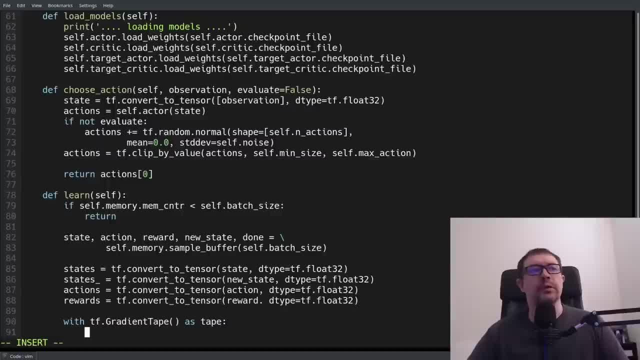 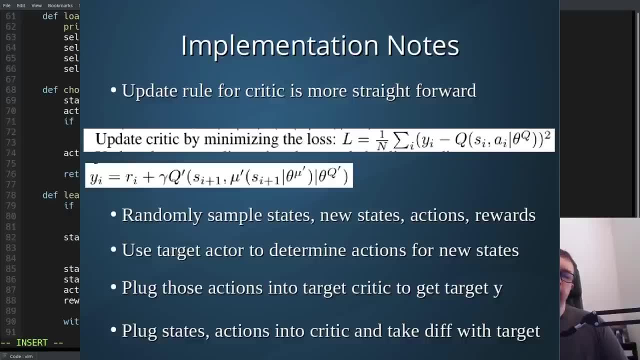 and so this is where we're going to stick the update rule from our lecture. so let's go ahead and start with the critic network, where we recall that we have to take the new states and pass it through a target actor network and then get the new states. 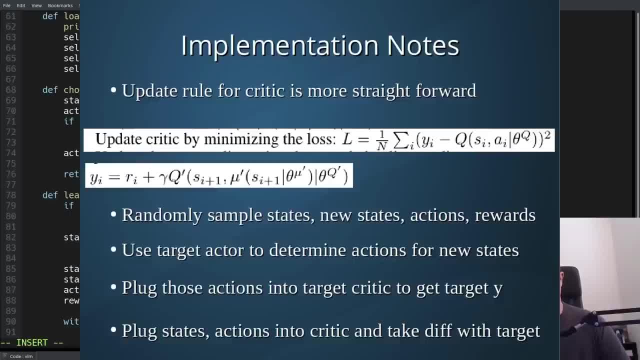 and get the target critic's evaluation of the new states and those target actions, and then we can calculate the target, which is the reward plus gamma multiplied by the critic value for the new states, times one minus a terminal flag, and then take the mean squared error between the target value. 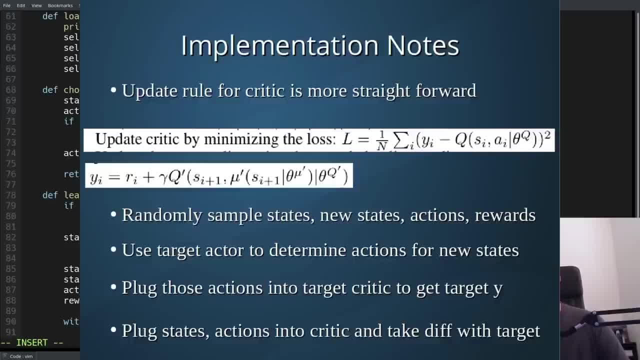 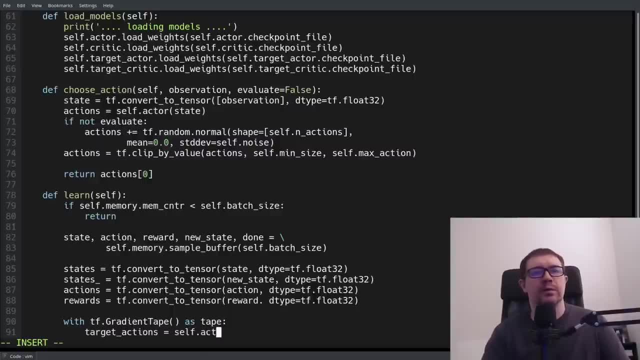 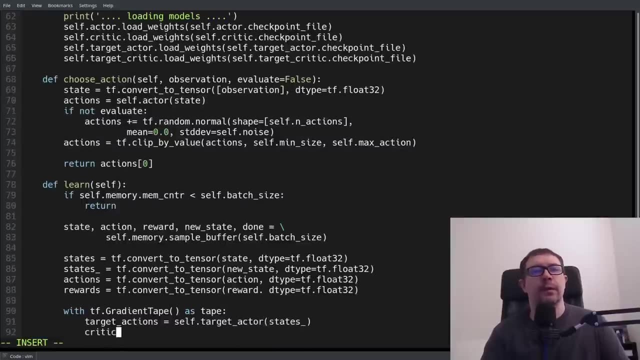 and the critic values for the states and actions the agent actually took. so let's go ahead and write that out. so target actions is given by our target actor, what it thinks we should do for the new states, and the critic value for those new states is going to be given by 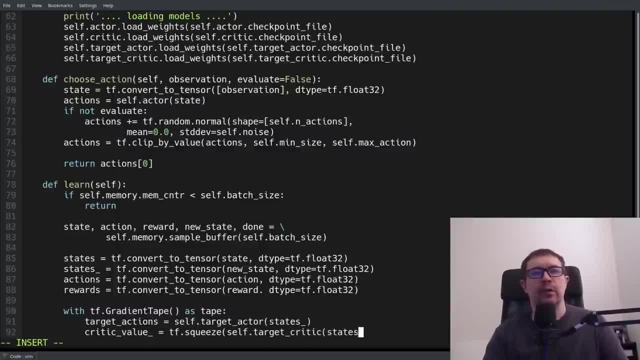 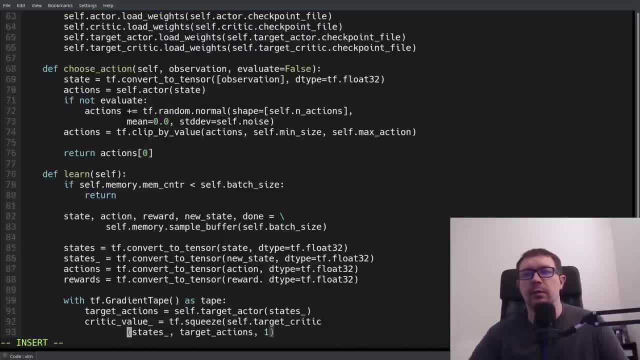 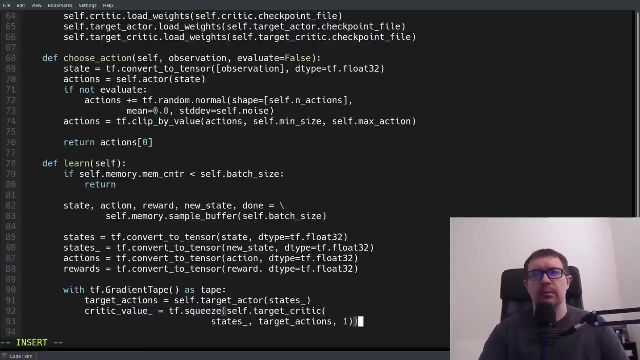 the target critic evaluation of those new states and target actions and squeezed along the first dimension. we have to put in this squeeze because we have the batch dimension and it doesn't actually learn if you pass in the batch dimension and i feel like i am missing. there we go. 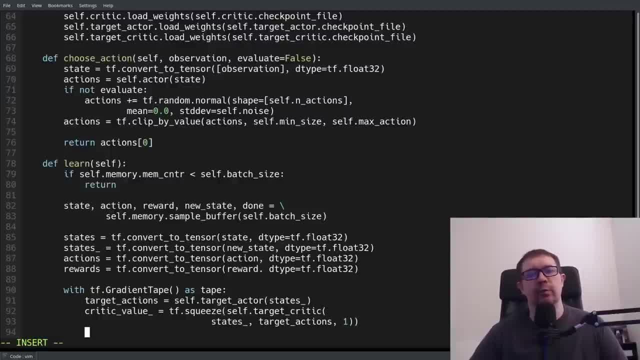 a parenthesis, so we'll have a squeeze everywhere- that we had to actually pass stuff through the network. so then, the critic value, which is the value of the current states, the original states and the actions the agent actually took during the course of the episode, is given by the squeezed output of the critic. 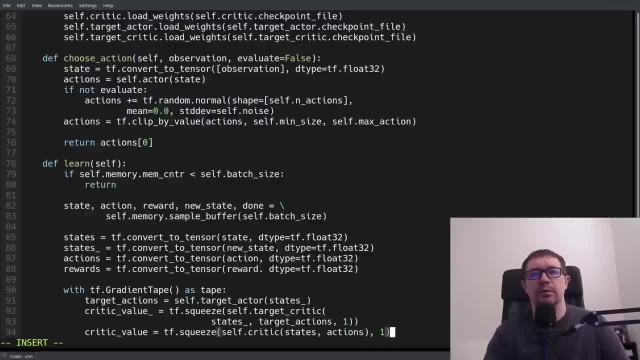 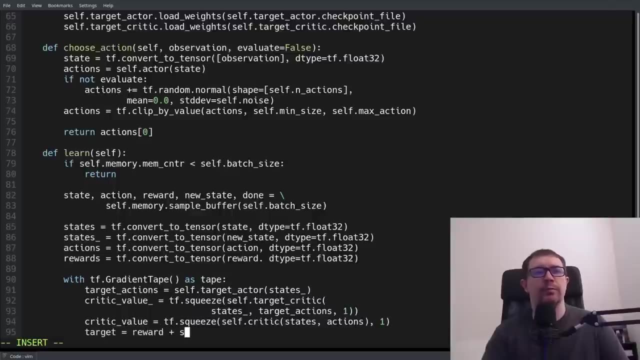 or the states and actions along the first dimension. i guess that is right. and then we have our target and that's reward plus gamma times this critic value underscore times one minus done. so this one minus done is one minus true or false. so when the episode is over, 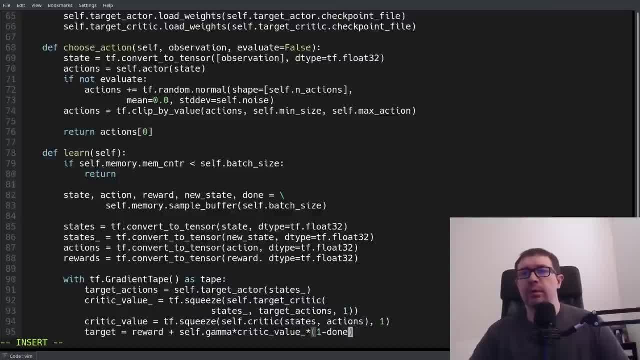 done is true, and so you have one minus one or zero, And so the target for the terminal new state is just the reward. As for every other state, it is reward plus the discounted value of the resulting state according to the target critic network. 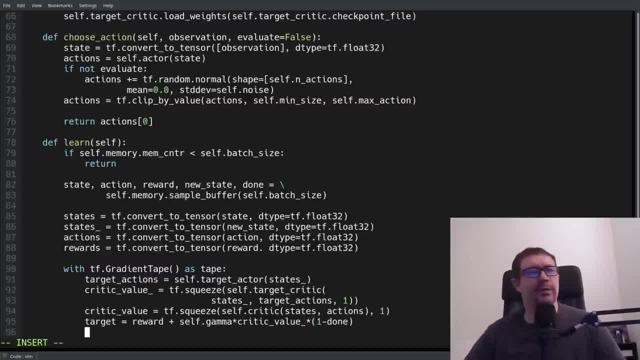 I'm sorry. if you can hear the landscapers outside, It's Tuesday. They're doing the neighbor's yard. Hopefully the noise suppression filter takes care of that, But if not I apologize. Next we have a critic loss, And that's the mean squared error between our target and the critic value. 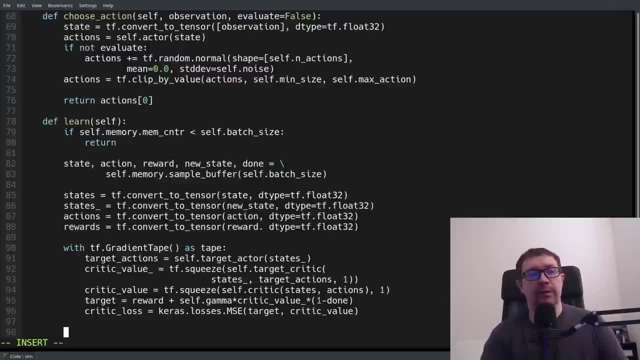 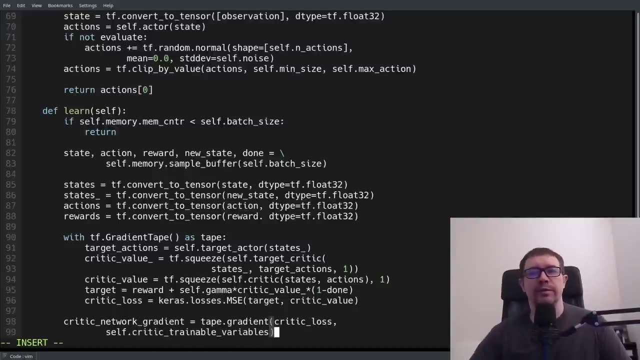 Outside of the context manager, we want to go ahead and calculate the gradients. So we'll say credit network gradient. It was taped out gradient critic loss, self-critic, trainable variables. So it is the gradient of the critic loss with respect to those critics. 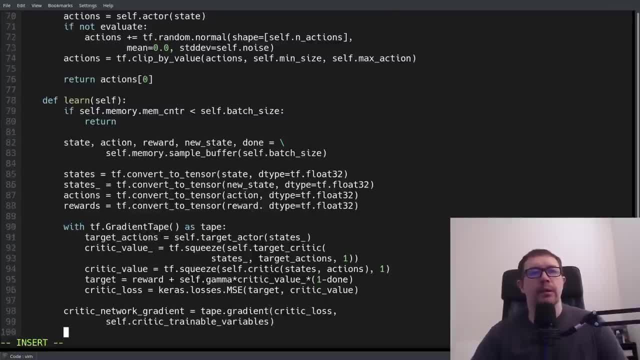 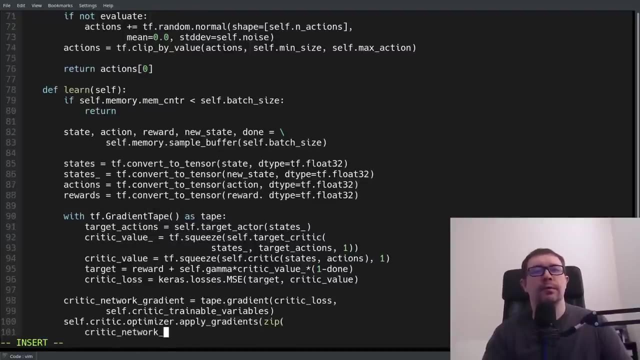 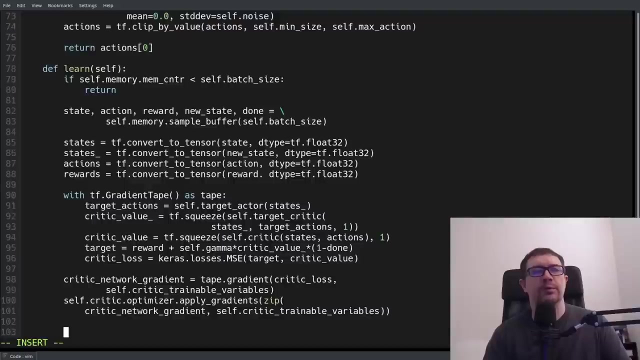 and then we want to apply our gradients. So our optimizer dot apply gradients And that expects a zip as input. We want to zip up the critic network gradient and the critic trainable variables And that is it for the critic loss. Now we have the actor loss. 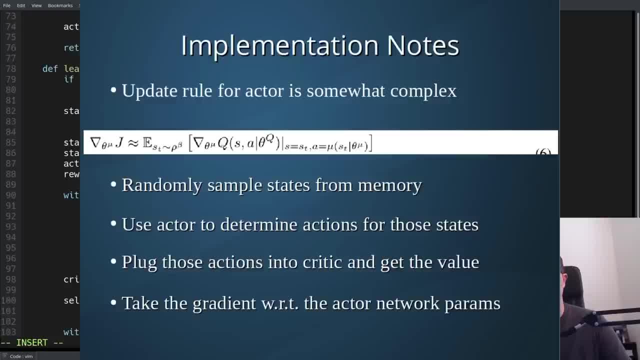 So with that, we're going to go ahead and calculate the gradients. And that is it for the critic loss. So with that, we're going to go ahead and calculate the gradients. We want to do essentially the same thing. We want our context manager gradient tape as tape. 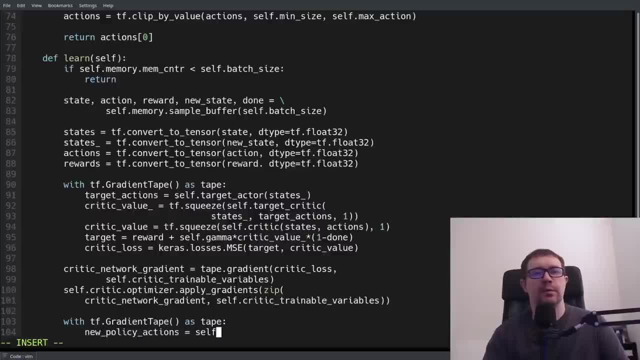 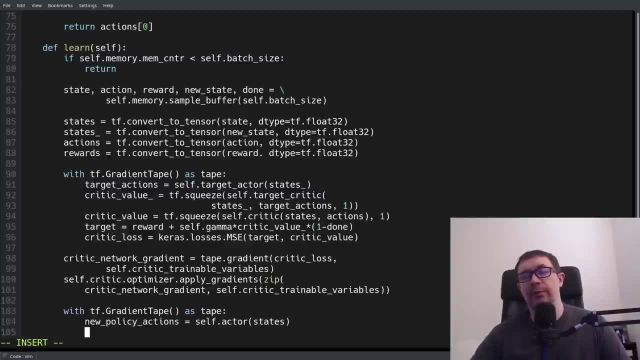 Then we say new policy actions, actor states. So these are the actions according to the actor, based on its current set of weights, not based on the weights it had at the time of whatever memory we stored in the agent's memory. So then we have our actor loss. 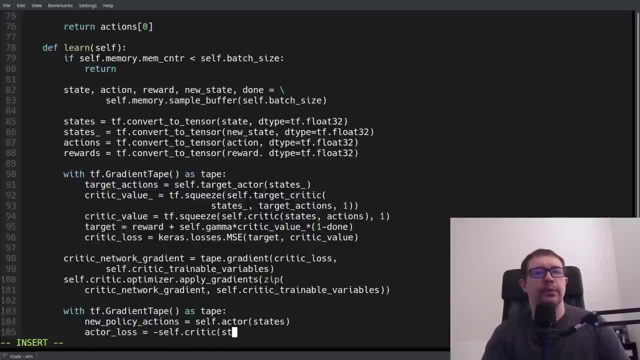 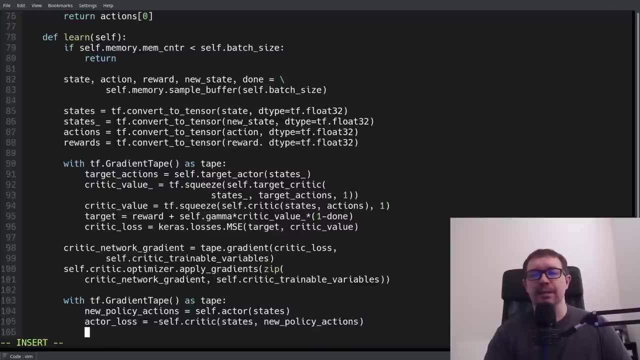 And that is the new policy actions. So we're going to go ahead and calculate the gradients. So we're going to go ahead and calculate the gradients negative of the critic output of the states and the new policy actions. It's negative because we're doing gradient ascent In policy gradient methods. you typically want to take the you don't. 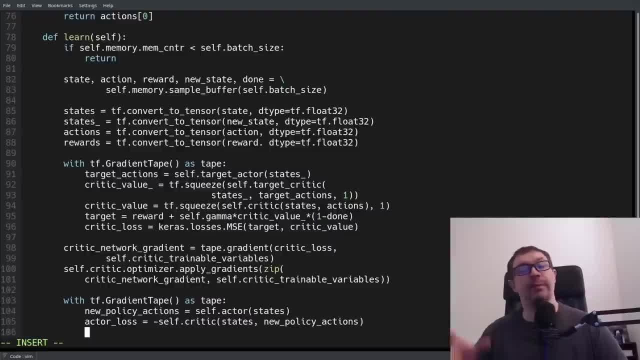 want to do a gradient descent because that would minimize the total score over time. You want to maximize total score over time, So you do gradient ascent. Gradient ascent is just a negative of gradient descent. So we stick a negative sign in here And then our loss is just the reduced mean. 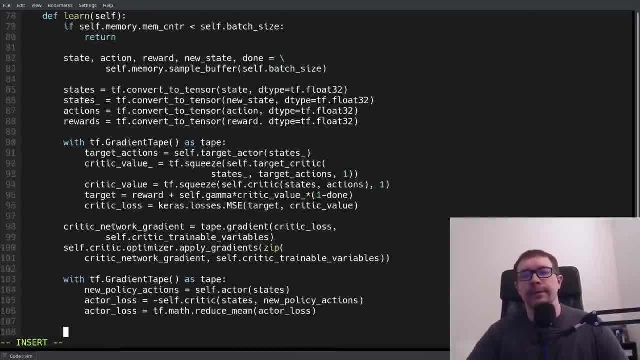 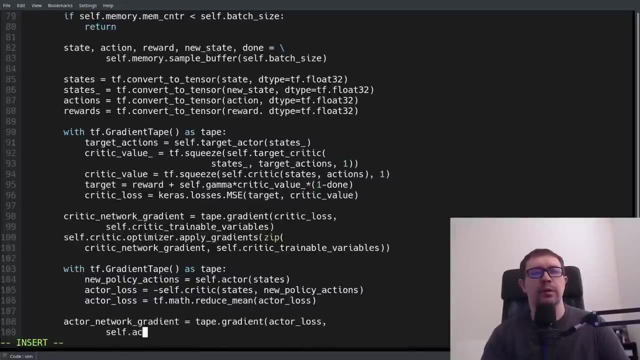 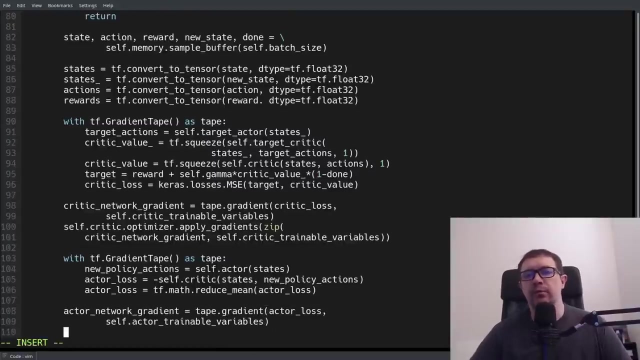 of that actor loss And then we can go ahead and calculate our gradients and apply them. So the actor network gradient is taped out, gradient of the actor loss with respect to the actor trainable Variables, And this is how we're going to get that. gradient of the critic loss with respect to 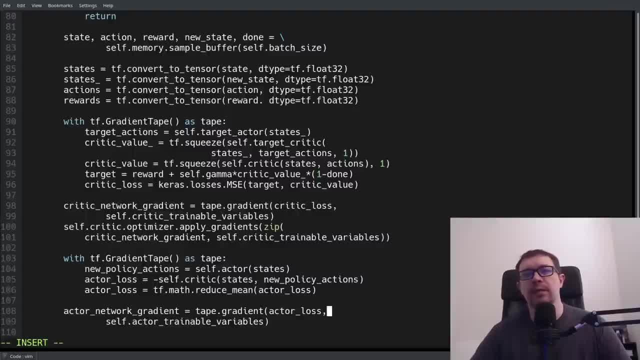 the mu parameters of theta super mu is by taking this actor loss, which is proportional to the output of the critic network, And that is coupled, The gradient is non-zero because it has this dependency on the output of our actor network. So the dependence, that gives you a non-zero gradient. 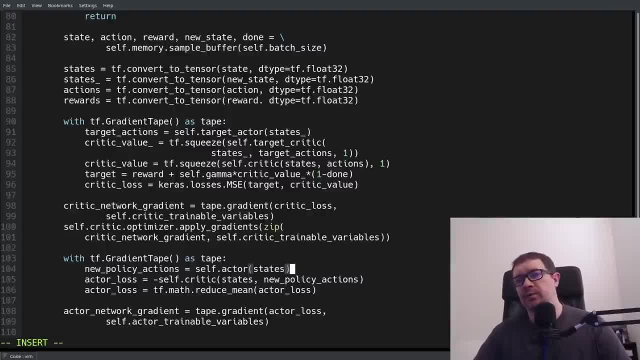 comes from the fact that we are taking actions with respect to the actor network, which is calculated According to theta super mu And that gets fed forward through here through the critic network. That's what allows you to take the gradient of the output of the critic network with respect to the 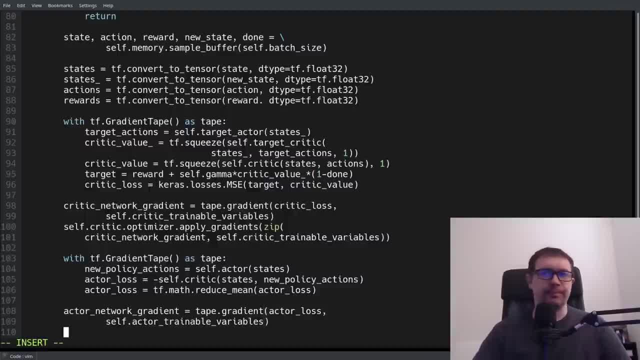 variables of the actor network. It's how we get that coupling And if you read the paper, they actually apply the chain rule and you get the gradient of the critic network and the gradient of the actor network. This form is actually easier to implement in code. That's why I do it based on. 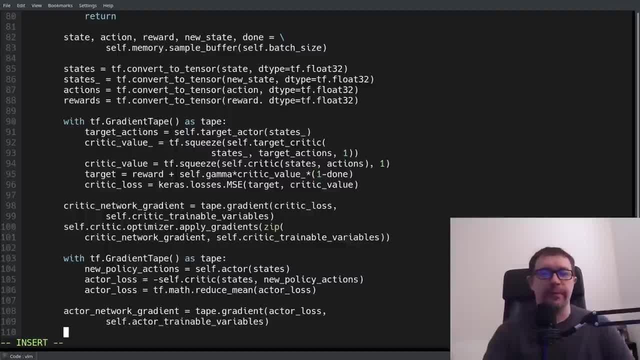 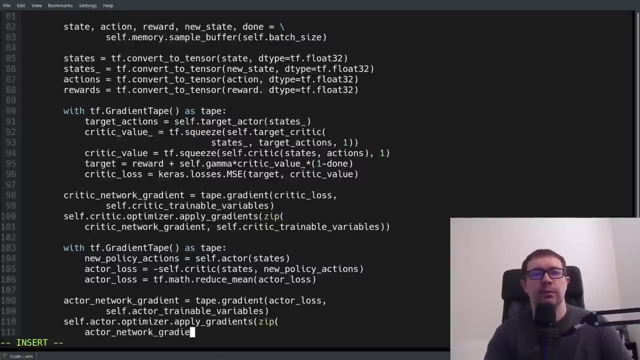 the first equation, The second equation in the paper it's just easier to do, So why not do it the easy way? Then you want to apply those gradients, which again takes a zip as input. We want to zip up our actor gradient network and the actor dot trainable variables. 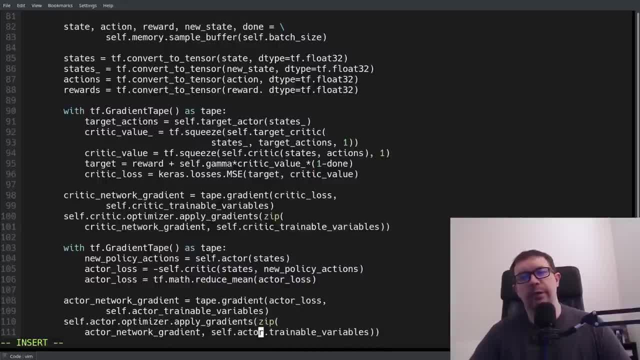 One other thing I want to point out is that this actor dot trainable variables we didn't define. It comes from the fact that we derive our actor network class from the Keras dot model class. It's just comes from the properties of object oriented programming. 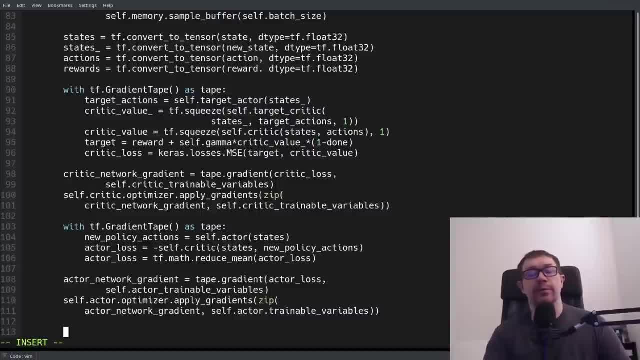 Once we have updated the main networks, we want to go ahead and perform a soft update of our target networks. And since this is not the first time we're calling the function that gets no input, so we'll use the default value for tau of 0.005.. 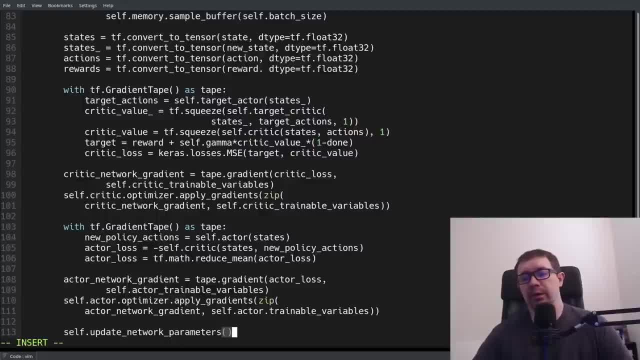 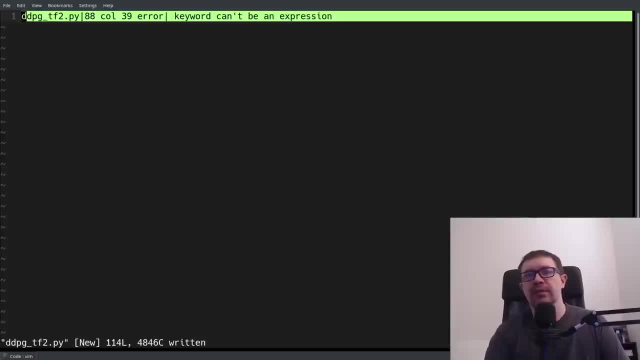 And that is it: 113 lines for our agent class. Now we're ready to write up the main loop and test it out to see how well it does. Okay, I have an error. It says keyword cannot be an expression. Uh, let's see. 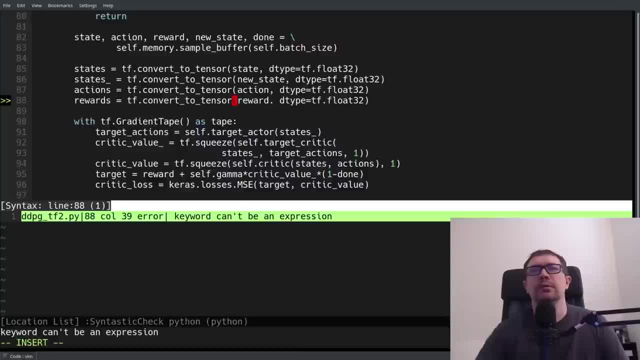 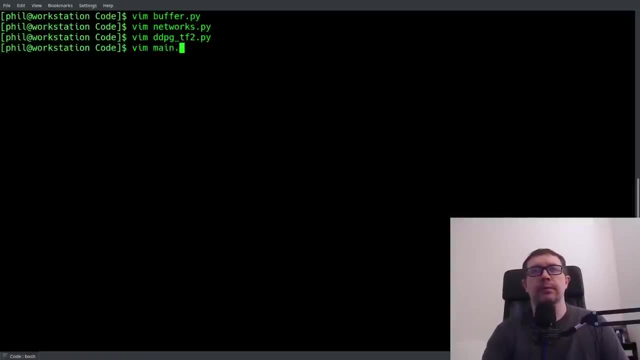 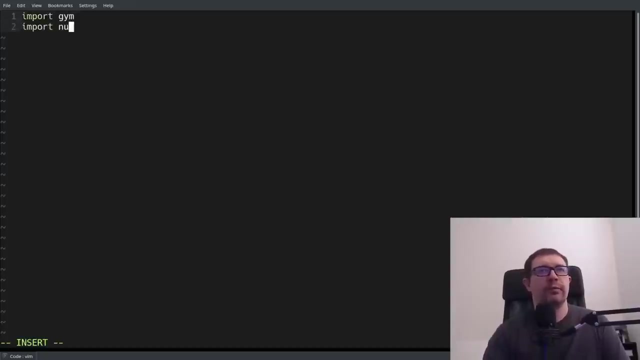 Rewards tf. convert to tensor. Where have I gone wrong? Ah right, here It's a period instead of a comma. All right, Now we're good. So let's go ahead and start with our imports. We have Jim, we have numpy, we have our agent and our plot learning curves. 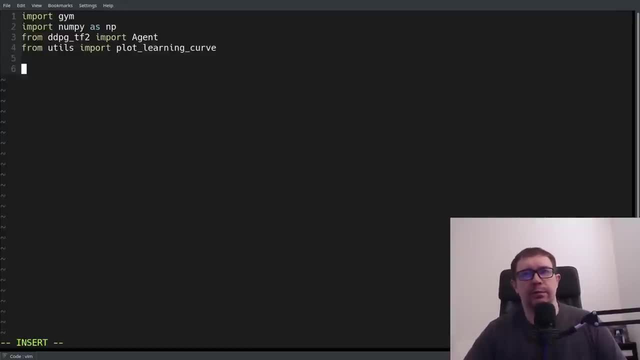 So, uh, go to my GitHub, do a git clone and get those utils. It is just a matplotlib function to Uh plot our learning curve, which is the score versus time, The running average of the previous hundred games. uh, over time. 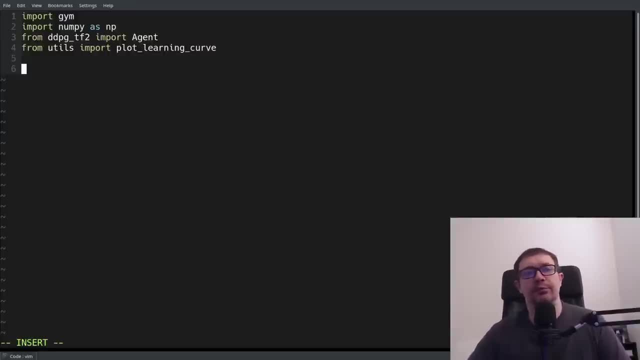 It's nothing magical. I don't go over it because it's rather the trivial and doesn't really contribute to your understanding. You can just do a plot of the scores over time to see if it's learning. So we start with our making, our environment and we will use the pendulum. 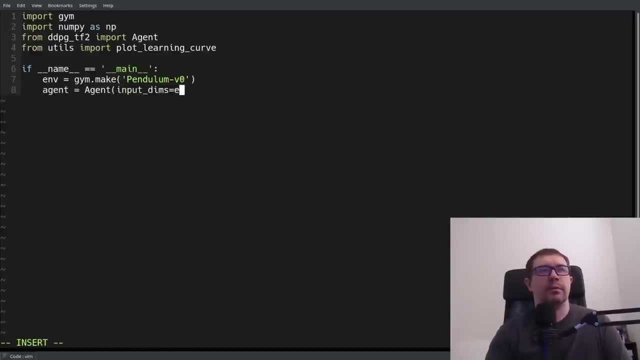 And We'll instantiate our agent by getting the observation space from our environment or input dims passing in the environment Shape and we will use the default value for our um noise and every other parameter, because those were good Defaults will let it play 250 games. 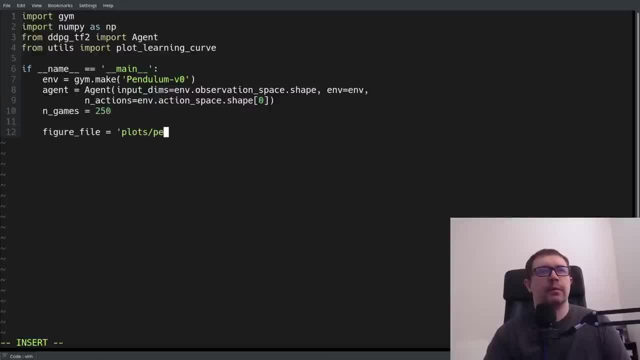 Let's go ahead and define a figure file: Pendulum dot PNG. We need to keep track of the best score- That's the lower bound of our reward range- and to keep track of the history of scores The agent receives and a load checkpoint. 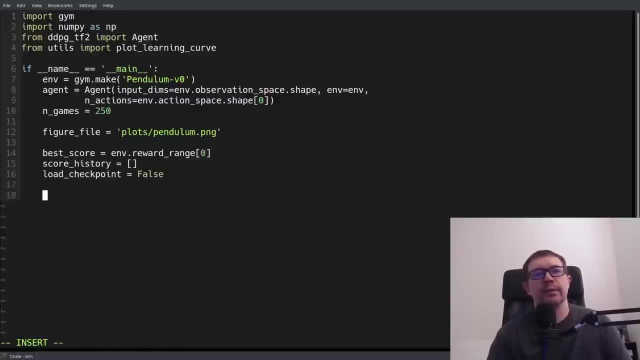 That'll be false. That's if you want to uh set Up our training versus testing. if we're going to load that checkpoint, then, um, we want to set number of steps to zero, while end steps is less than agent dot batch size. uh, what we're doing here? 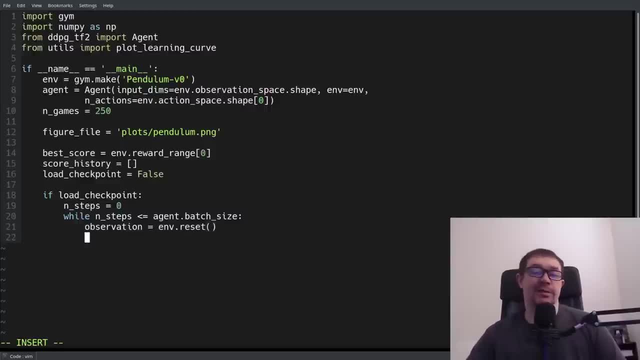 Okay, So I should explain this. So my understanding and this could be wrong. if it's wrong, drop a comment down below to correct me. I don't profess to know everything about tensor flow, but from what I've read, uh from uh Google, the model loading is set up such that you have to call the learning function um before you can load your model. 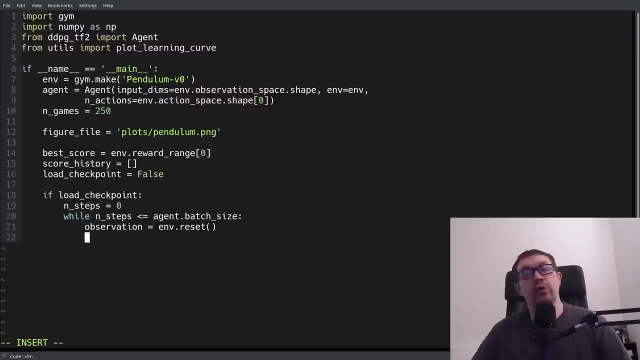 Uh, and that's because when you instantiate the agent, you aren't actually loading any values onto the graph, And so it's basically an empty network. There are no values loaded into that network. It doesn't load any values until you try to do something with it. 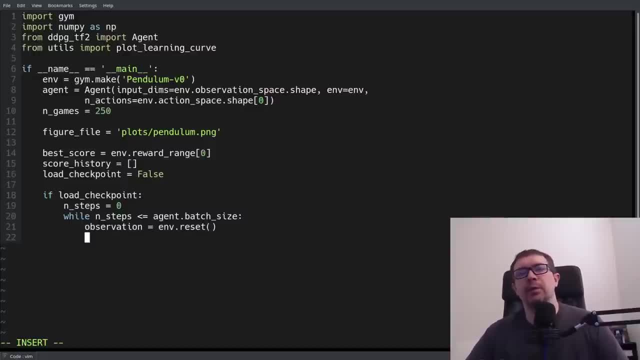 And so we're going to Go ahead and fill up the agent's memory with dummy variables, dummy values- Uh, they don't really matter. Uh, we're just going to go ahead and load it up with dummy values and then call the agent's learn function so we can load our models. 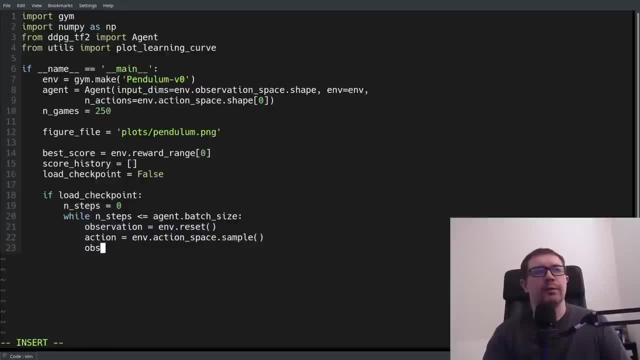 And so we can do a random action, Doesn't really matter. Get our new state reward done and info from our environment, And then remember that And very important when, increment number of steps. once you've done that, call the learn function and load your models and set evaluate value eight to true. 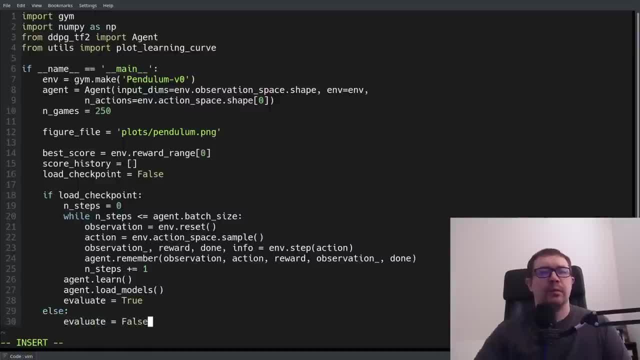 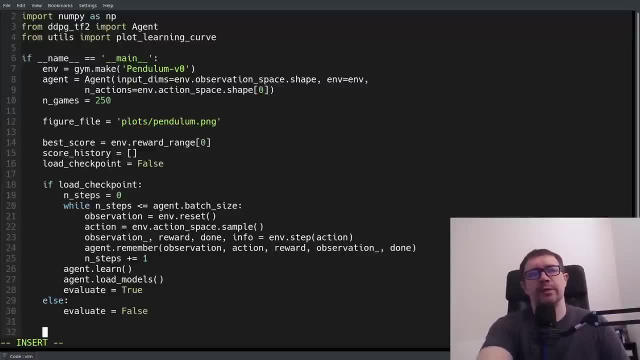 And if we're not going to be loading our checkpoint, we'll just say evaluate equals false. I guess We could just use load checkpoint in place of evaluate or call it evaluate. but whatever, I've used two separate variables. Sue me. 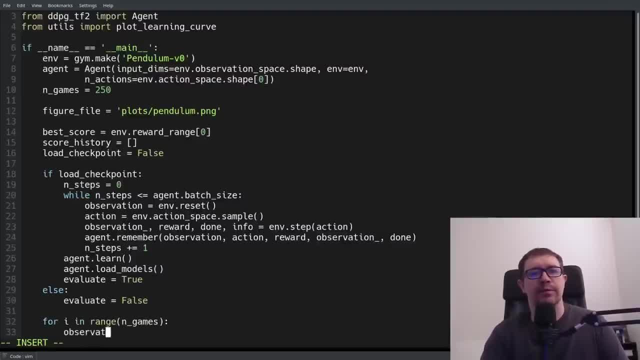 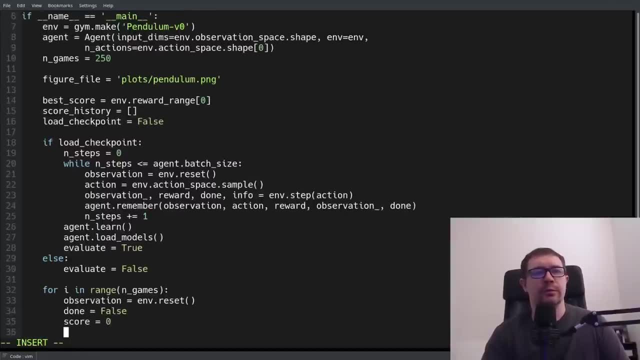 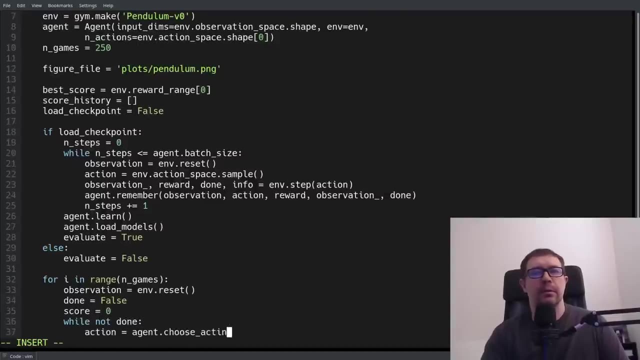 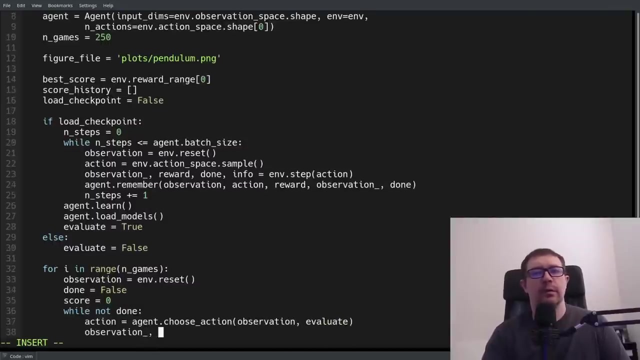 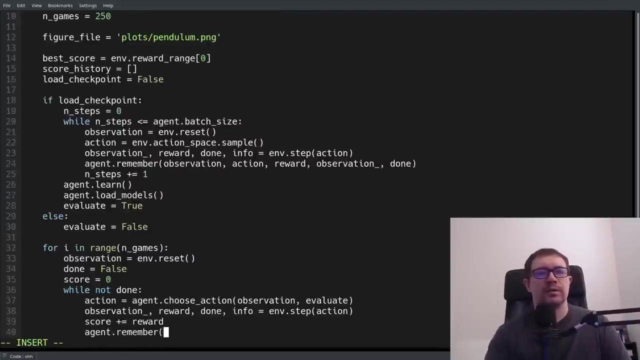 So for iron range and games, we want to go ahead and reset our environment at the top of every episode. Reset the terminal flag and the score to zero. while the episode is not done, Agent can choose an action based On the observation and the evaluate flag. get the new state reward uh done and info from the environment, increment our score and store that transition. 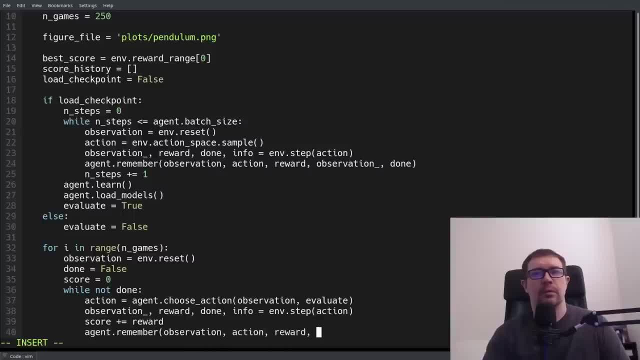 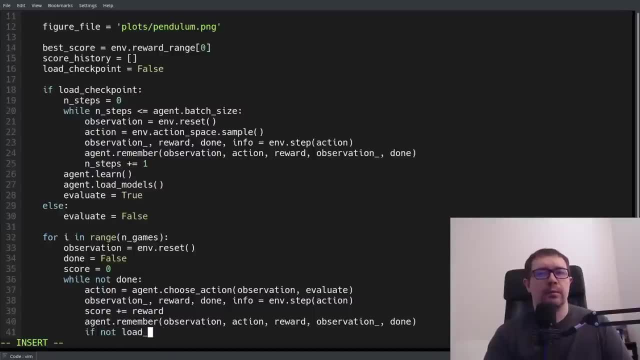 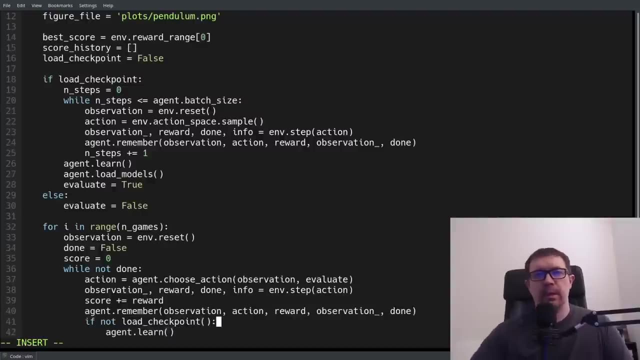 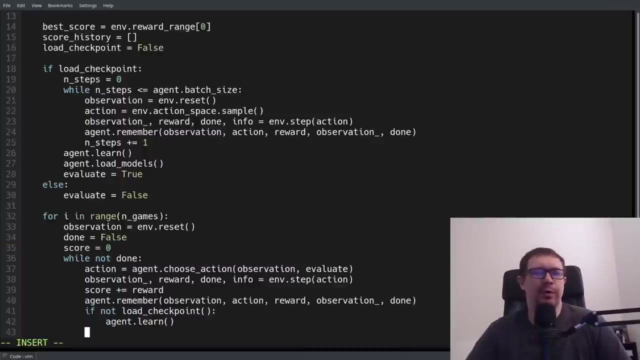 Uh, if we're not loading a checkpoint, Then we want to learn, And the reason I put in that uh, conditional statement is because if you're evaluating the performance of the agent, you probably don't want to disturb its parameters. You want to just go ahead and see how it performs as of the last time you saved it, rather than trying to get it to learn a little bit more. feel free to change that. 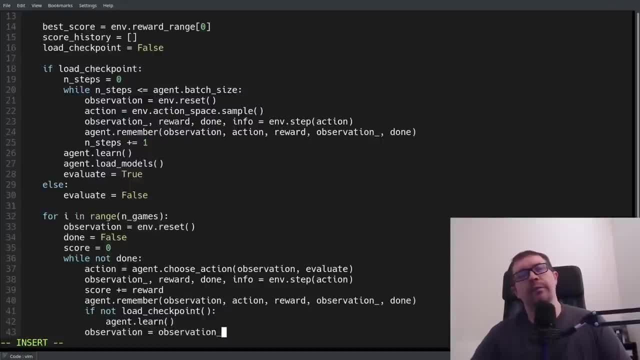 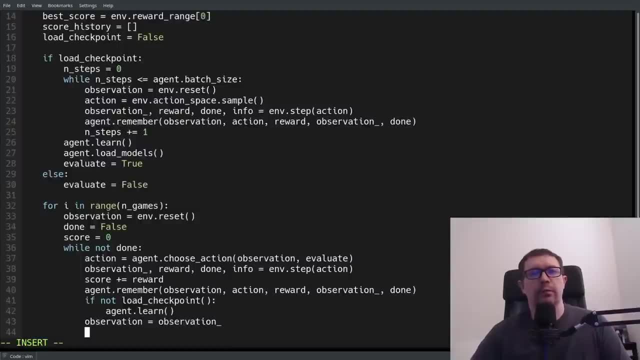 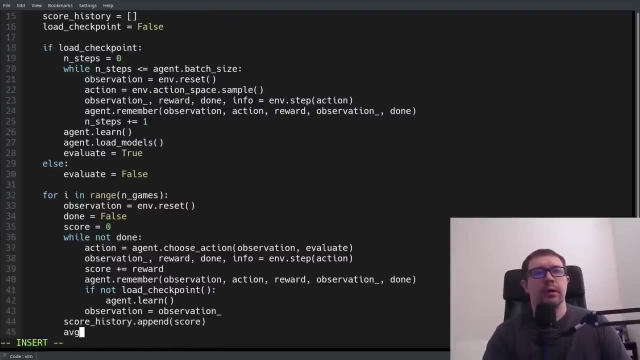 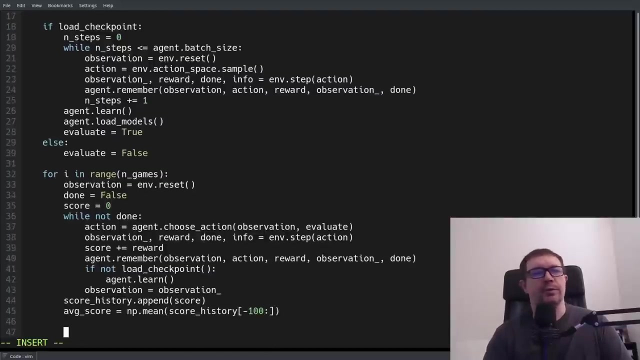 And, very importantly, we want to set the current state of the environment, The environment, to the new state after the uh agent took its action. So then, we want to um. at the end of every episode, we want to append the score and calculate the average to get an idea of whether or not our agent is learning. 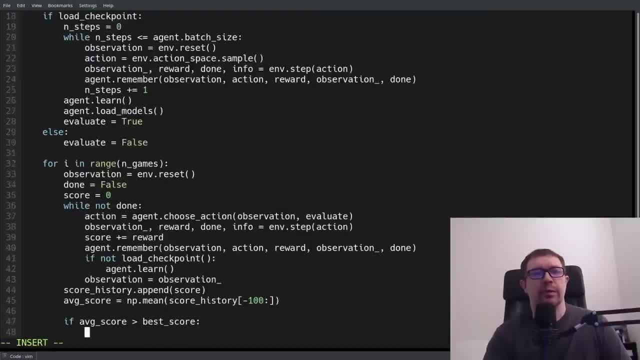 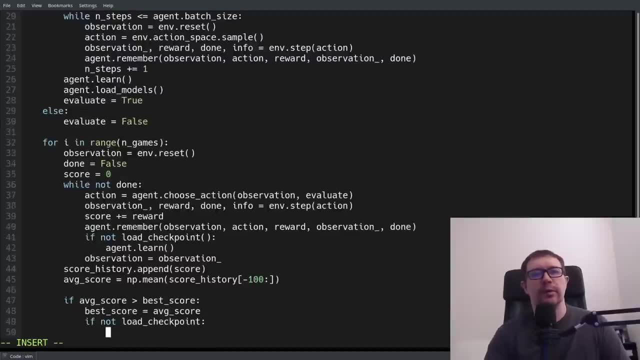 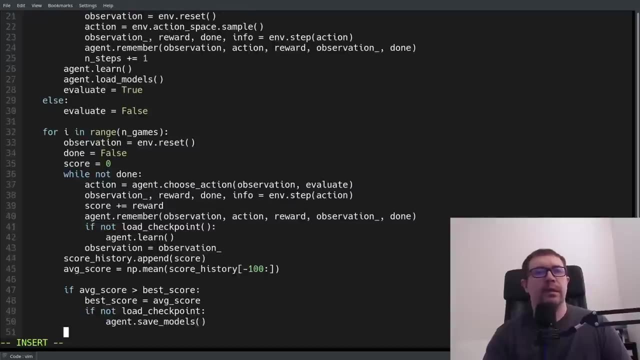 If the average score is better than the best known score, then set the best score to that average score. And again, if we aren't loading a checkpoint, go ahead and save your models. And at the end of every episode we want to print some basic debug information. 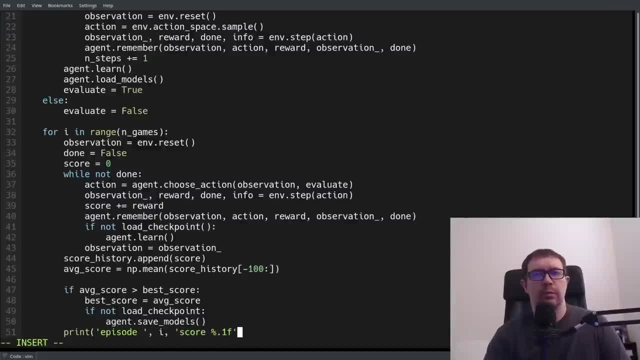 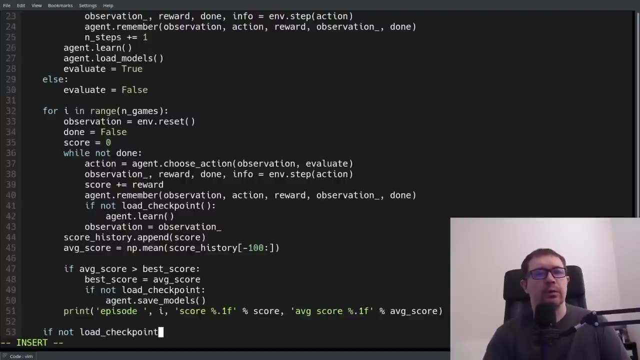 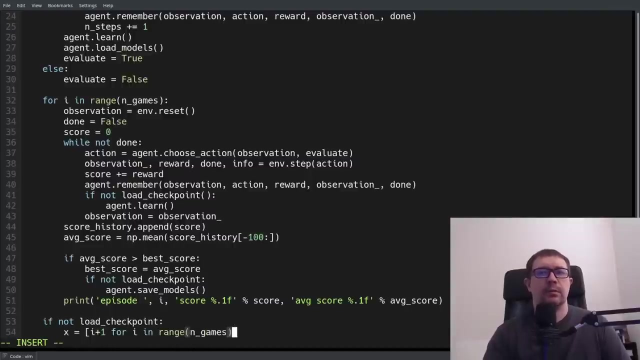 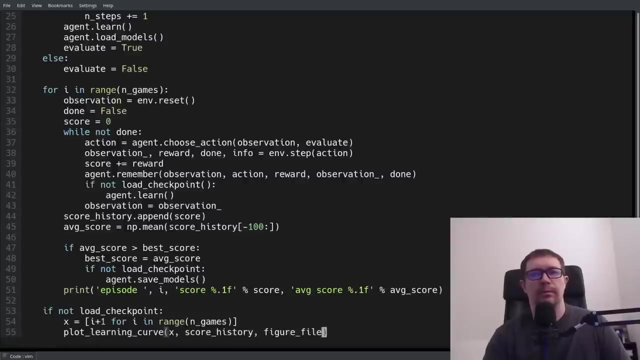 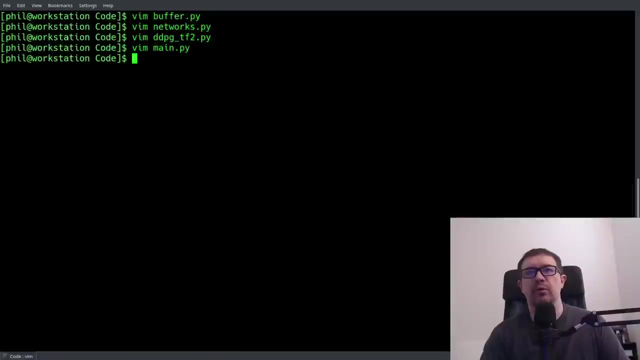 So I score, And at the end of all the episodes We want to print our, or plot our, learning curve. So our X axis number of games. Okay, That is it for our main loop. Let's go ahead and test it out to make sure I made a sufficient number of typos. 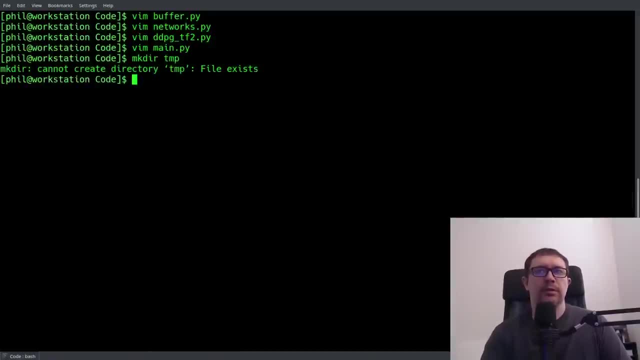 But, as I said, the first thing you want to do is make der temp- Uh, okay, I already have that. to make der temp slash GDPG- I didn't have that. and make der plots- I think that already exists, Okay. 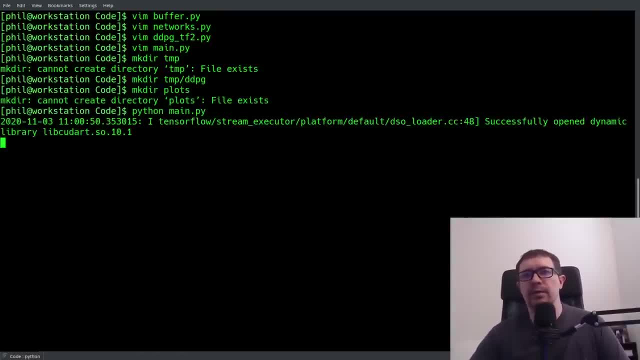 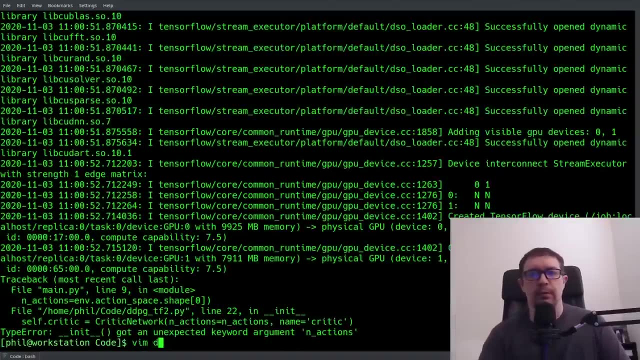 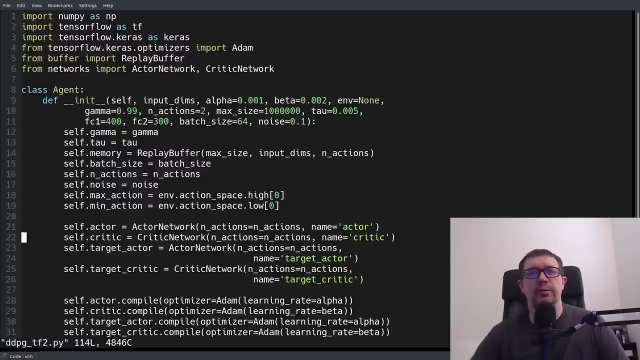 Now we can go ahead and run the main file and see what I messed up, Okay, So, oh yeah, of course our critic network um does not get a number of actions. That's something I changed on the fly, Okay. 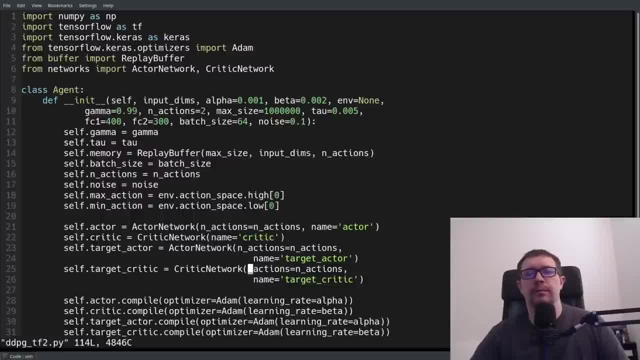 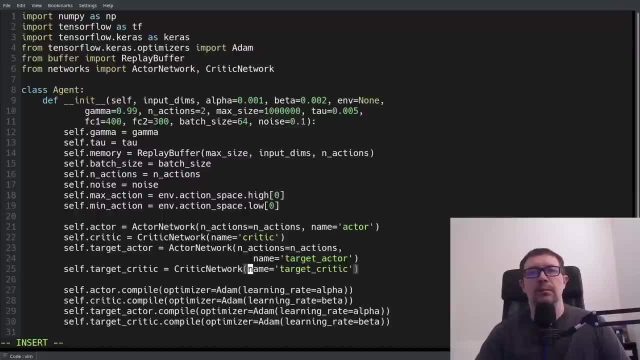 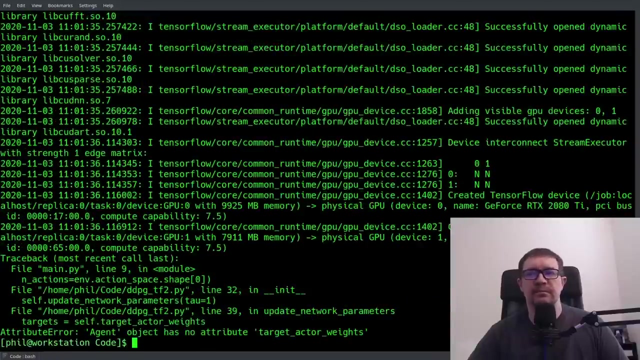 So let's fix that here as well, And we can go ahead and put this back up here. I think that is right. Let's try it again. Yeah, Okay, Okay, Yeah, Okay, No, no, No, No, no. 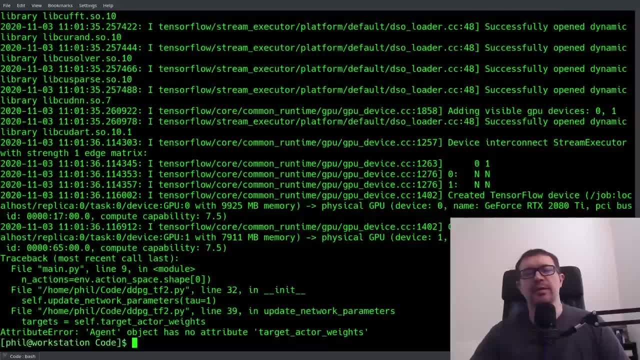 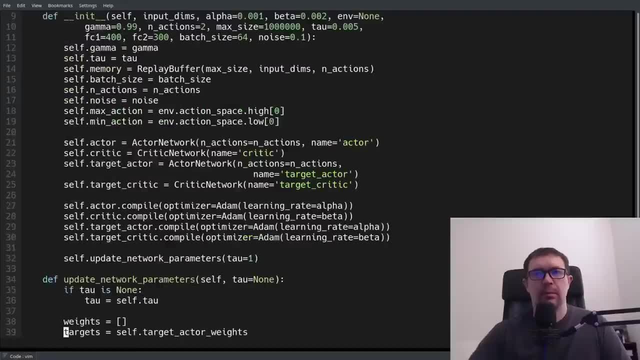 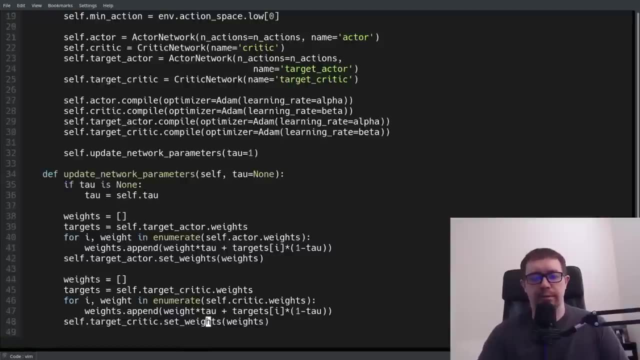 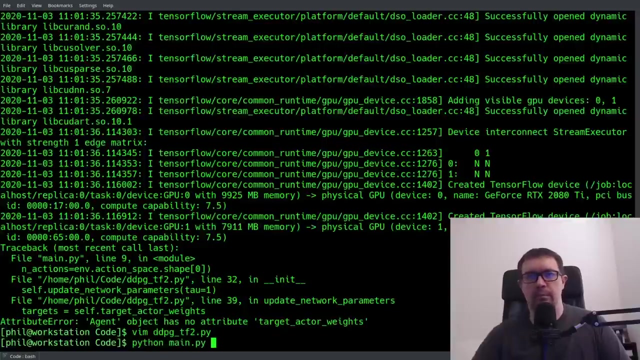 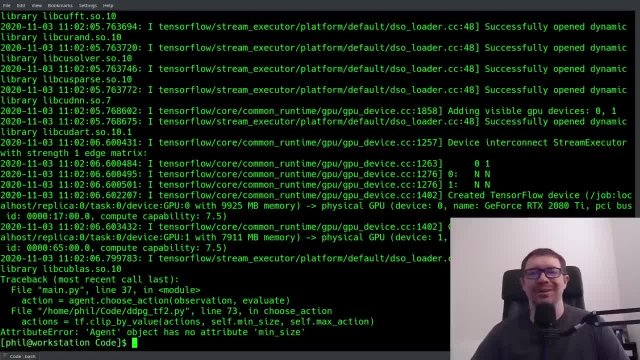 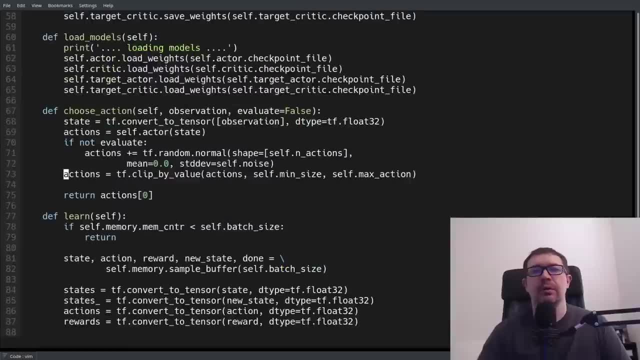 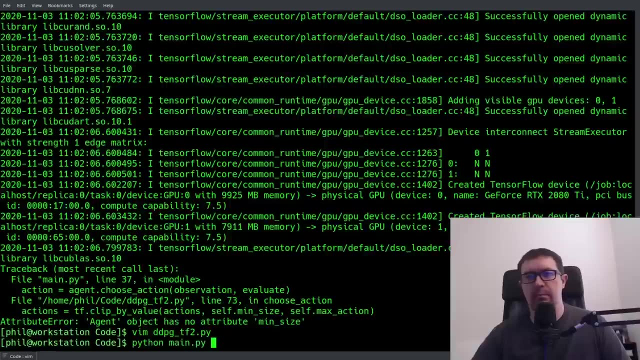 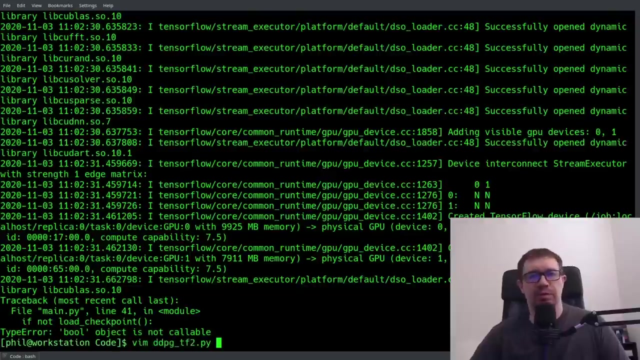 size. okay, oh, it's in action. that's in line 73. yeah, it's min action and max action, of course. all right, that's in main line 41. see, this is why I have a cheat sheet, because even even with the cheat sheet, I make a number of typos. so you can. 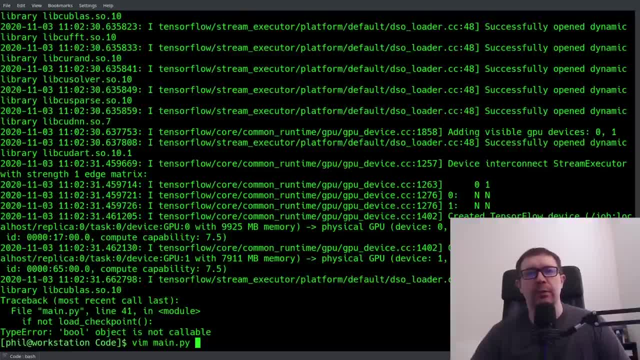 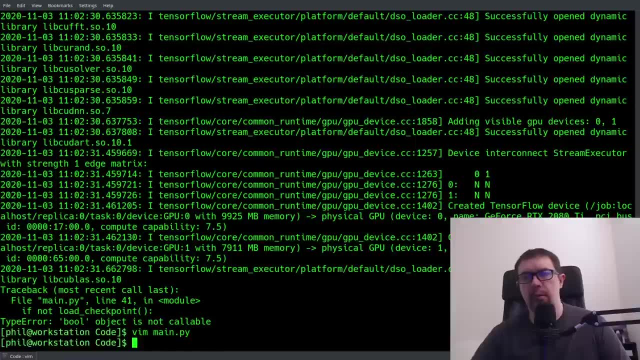 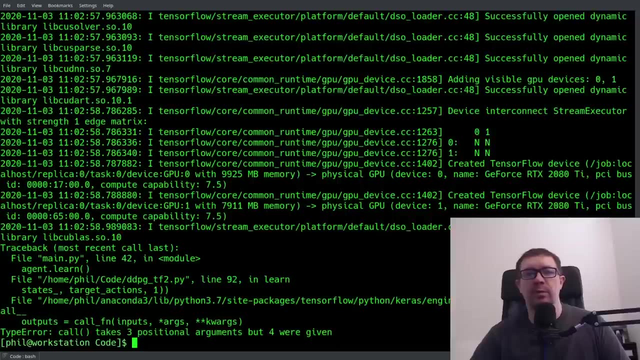 imagine what it's like if I were to try to do it on camera. that is in line 41. if not, load cheat sheet checkpoint. there we go. good grief call takes three position arguments, but four were given. all that's because I have my parenthesis in the wrong place. 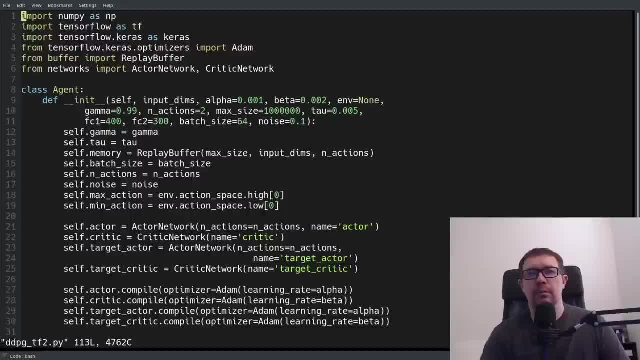 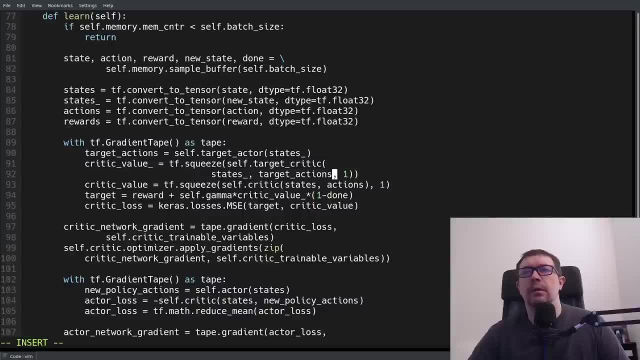 ok, that is in line 92. so the state's target action. so the, because I have my parenthesis in the wrong place. okay, that is in line ninety-two. so the state's target action. so the state's target action. so the parentheses goes here. yeah, that's right. 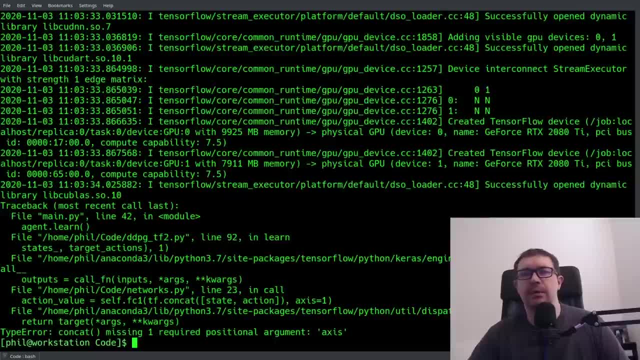 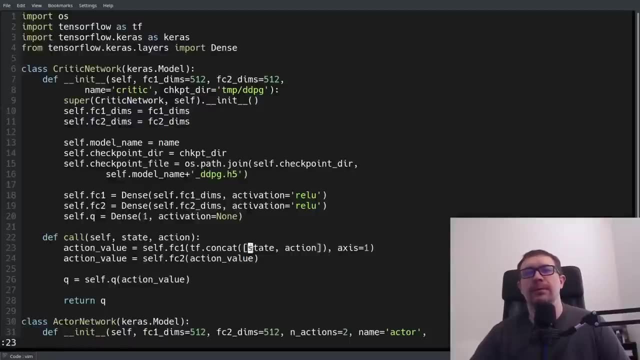 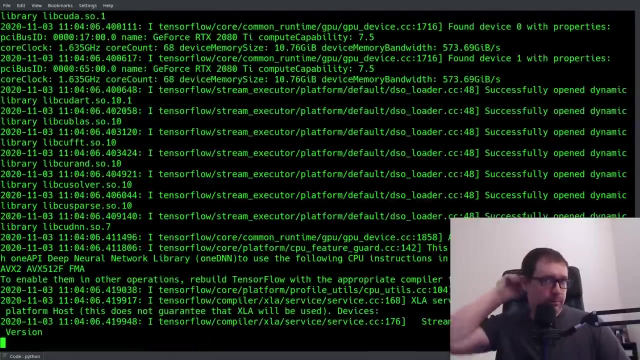 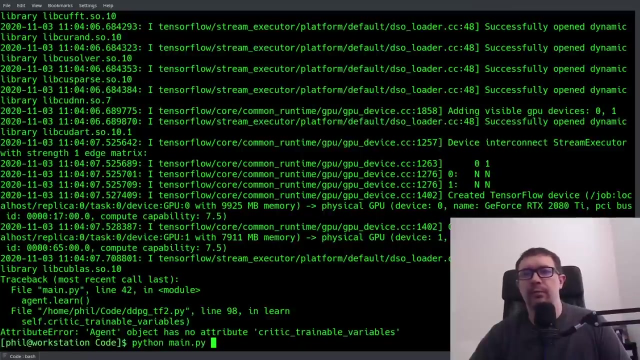 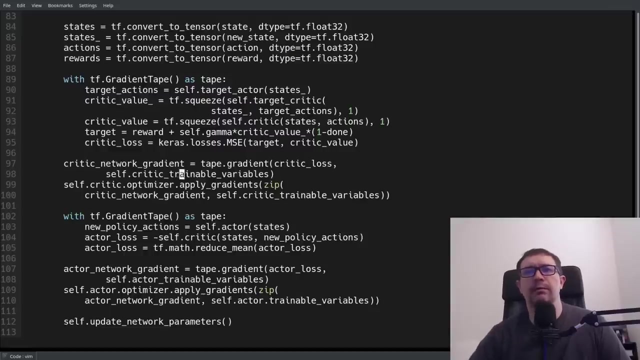 my goodness can cat missing one required positional argument? oh, because I have the, because I have an extra parentheses. okay, so this is bad even for me. line 23: so then we need a second friend to see their critic. trainable underscore variables. once again, that is a trainable dot variables. that is in line 98. I thought I looked for that. 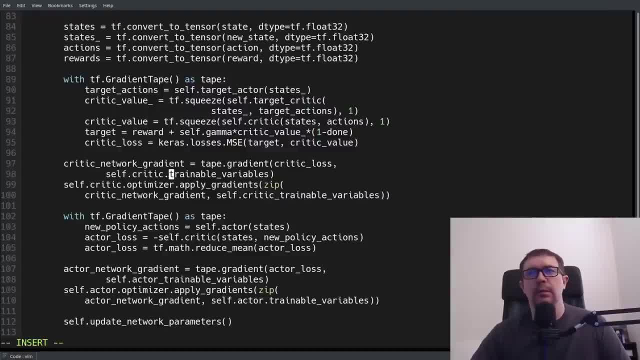 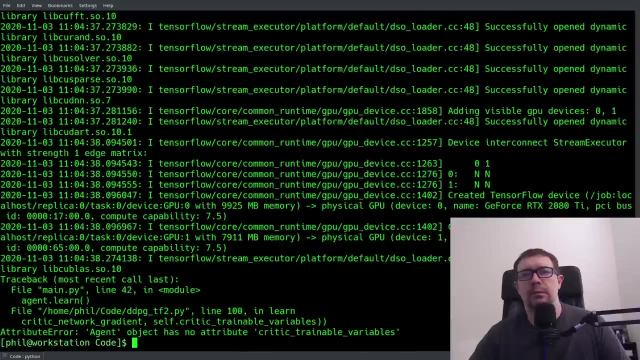 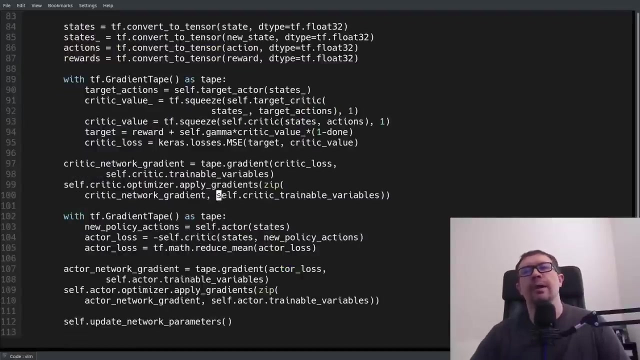 oh no, I didn't critic dot trainable variables and I did the same thing here. all right, what I just fixed that, did I not line 100? didn't I just fix that? no, I did not just fix that. brilliant okay, actor dot- okay. this is what happens when you don't do this for a month. making YouTube videos is a. 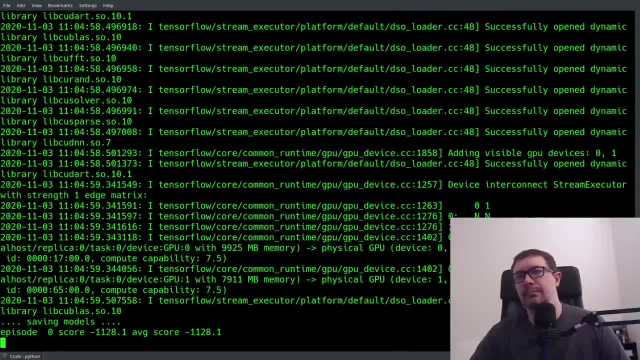 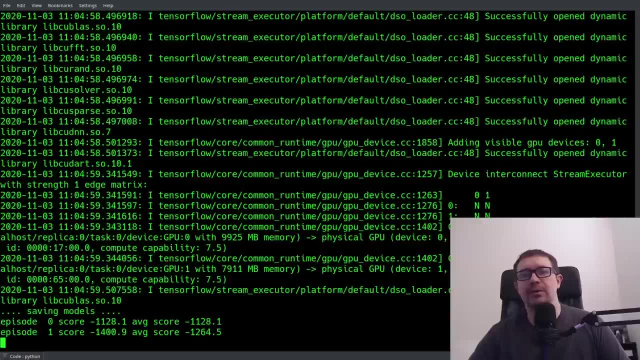 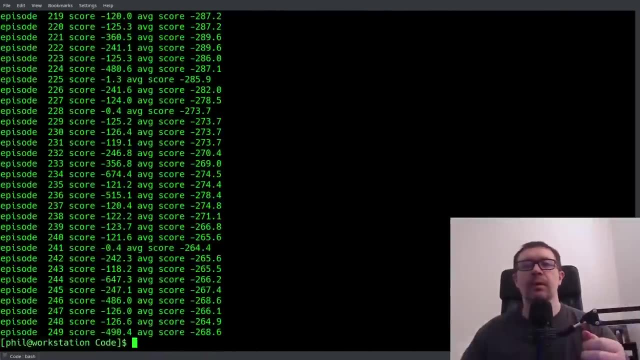 perishable skill. okay, perfect, now it is actually working. I've got gotten through all of those typos and it has started to run, so I'm gonna let this go ahead and finish up and we're gonna see how it does. all right, so it has finished running and you can see that at the end it kind of takes. 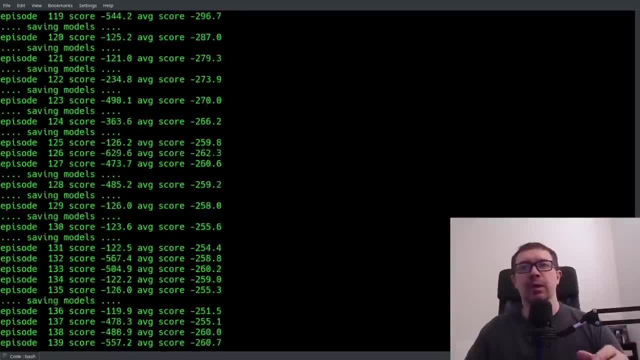 a little bit and says: well, I'm trying to run it and I get an idea. look at the atypical with actor critic type methods. so oftentimes what will happen is the agent will achieve some reasonable performance and then kind of start to taper off because the, as I said, the actor network is relatively sensitive to. 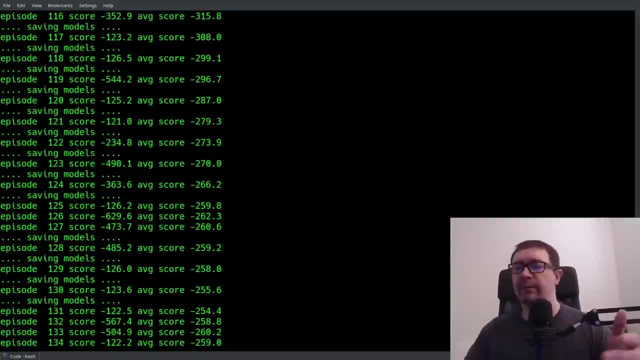 changes in its parameters. in this case it didn't fall off a cliff, like I've seen with things like actor critic or policy gradient methods, but it is still nonetheless sensitive to changes in its weights and is prone to deteriorations of performance late in the number of simulations. if you take a look at the 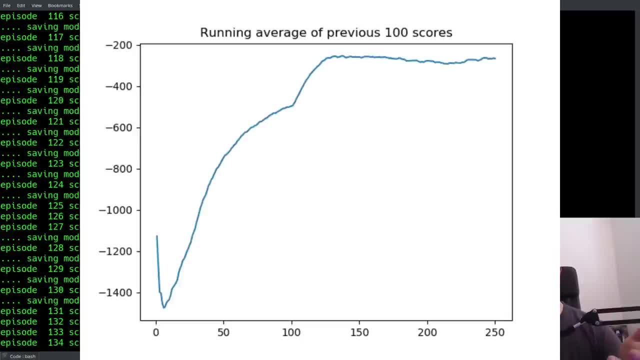 learning curve, you can see pretty clearly that it has an overall upward trend over time. so it is in fact learning. our technique is working. it's doing its job, but it's not. you know, it's nothing, at least for this environment. it's not the greatest thing since sliced bread. we could do a little bit more. 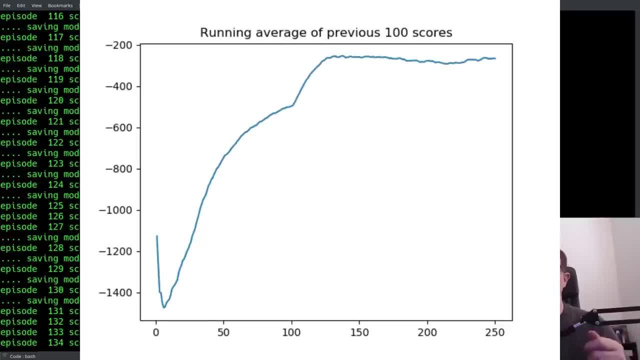 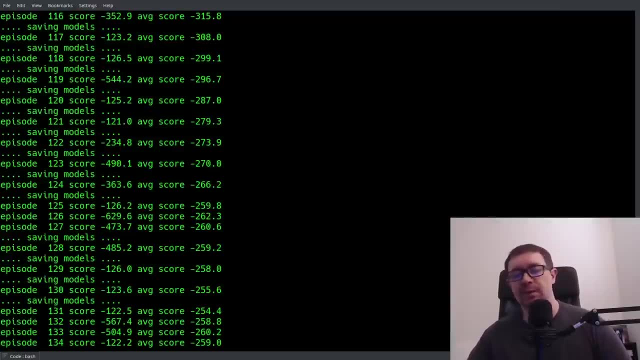 tuning to get it even better, but for now I think this is sufficient to a demonstrate that it works and to be have a solid tutorial on how to implement deep deterministic policy gradients. once again, shameless plug if you want to know how to go from paper to. 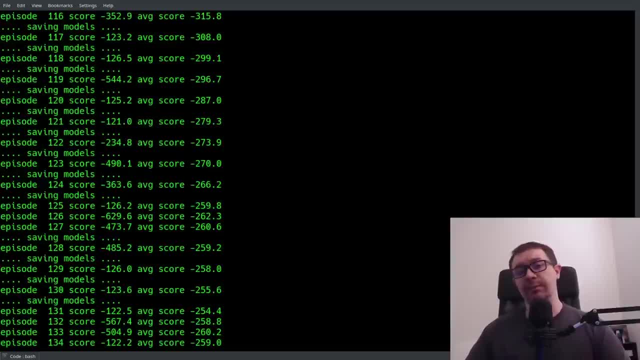 code. I show you how, in my two udemy courses on deep reinforcement learning, where we go through several papers per course- one on deep Q learning, one on actor critic methods- and implement all these algorithms from scratch, I show you how to implement pretty much everything from the papers, minus some super. 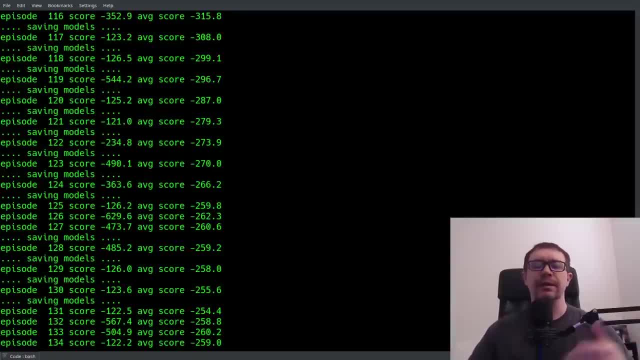 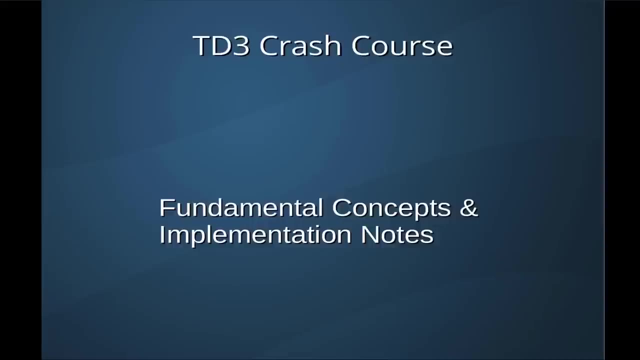 superfluous features. either way, if you made it this far, please leave a like, a subscribe, drop a comment down below you. I'll see you in the next video. welcome to a crash course in twin delayed deep deterministic policy gradients, or TD three for short. this is a very brief. 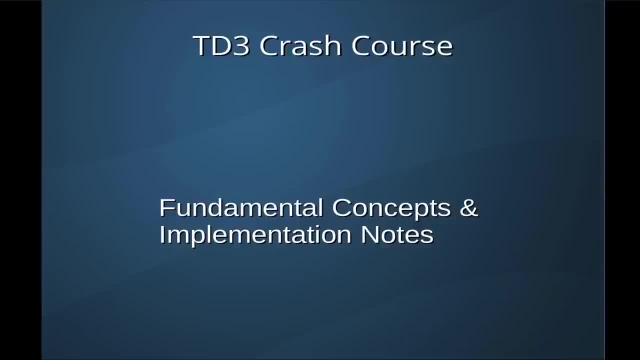 lecture that's going to cover the fundamental concepts and implementation notes for our coding tutorial, which will follow this lecture. if you want the full details of how this algorithm works, I highly recommend you read the paper titled addressing function approximation error in actor critic methods. it's very 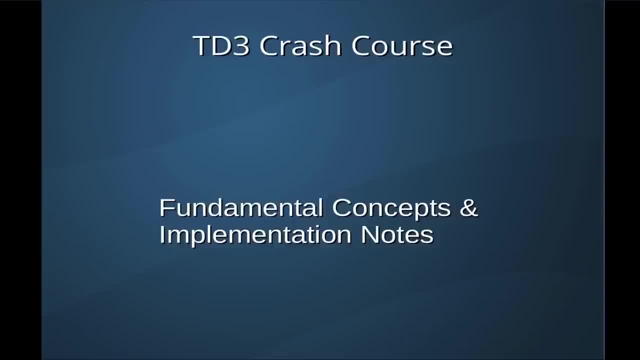 well written, very technical, very detailed and it's going to help you in your practical. very detailed and it covers significantly more detail in depth than I will do here. I'm just going to give you broad strokes and some idea of what we're going to be doing in our coding tutorial and we're gonna be using 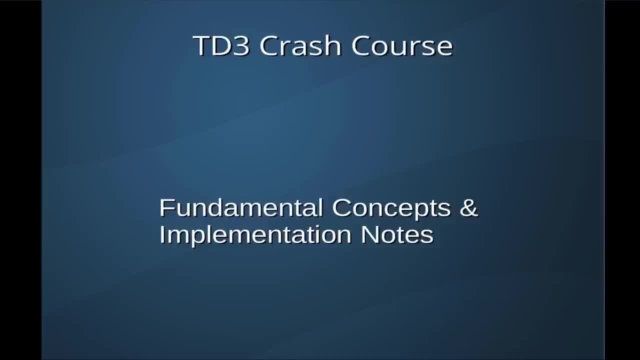 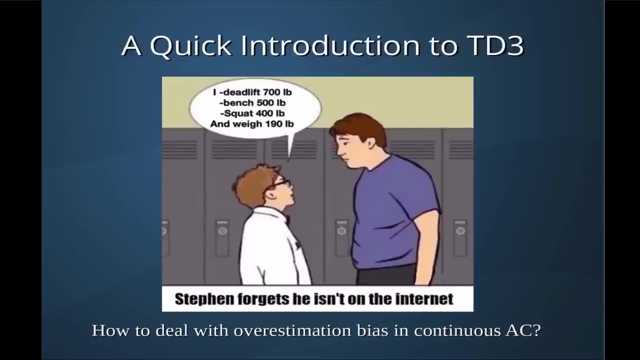 tensorflow 2, by the way, for our coding tutorial, so make sure you have that installed. so TD 3 exists to deal with a fairly straightforward issue: how do we deal with overestimation, bias and continuous action space actor critic methods? if you're not familiar with this video, just like most other video, and if you haven't done it yet, please consider subscribing to give a thumbs up. this way, it will give you a shout out and also make sure you hit the notification bell. so I'll see you in the next video. bye, bye, and then I'll see you in the next video. this is a very 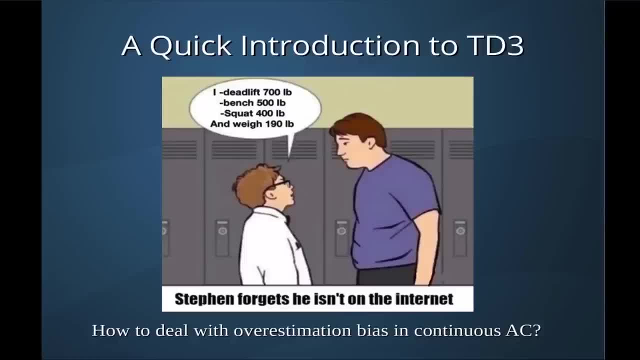 with overestimation bias. it is a tendency of agents to incorrectly estimate the value of a state on the high end, So it says this state is worth more than it actually is And this is a problem because the agent will attempt to access that state in the future, which leads to a sub. 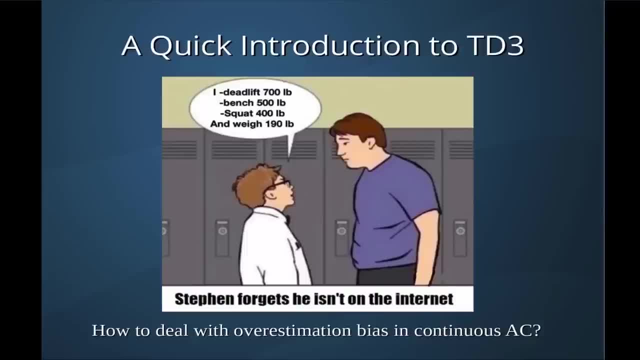 optimal policy because there are other, more profitable states out there. So this is a pretty big problem, particularly when you're trying to approximate the agent's policy, as we are in actor critic methods, But it's not clear where this would even come from. In Q learning we get 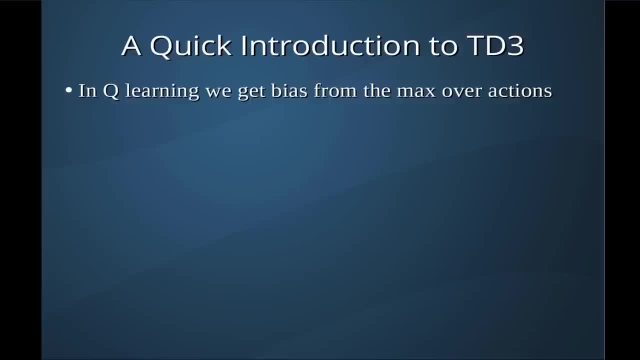 biased because we take a max over our actions in our update rule for either the table or our deep neural network. So there's some maximization or overestimation built in right from the beginning and that's pretty easy to see. But there is no max in our update rule for actor critic methods. So 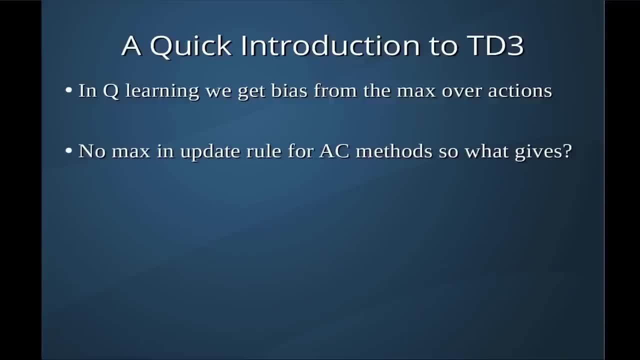 what gives. Where could this overestimation bias come from? Well, on a somewhat theoretical level, I kind of argue. they don't do this in the paper, but the way I think of it is that we have stochastic gradient ascent where we're attempting to maximize the product of our probabilities. 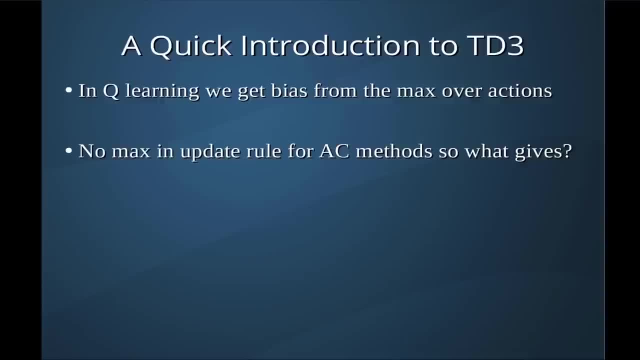 our policy and the rewards or returns the agent receives over time. So there is some implicit drive to maximize score over time And so when you get natural variation in your rewards or in the trajectory through the state space, you can end up with some increased. 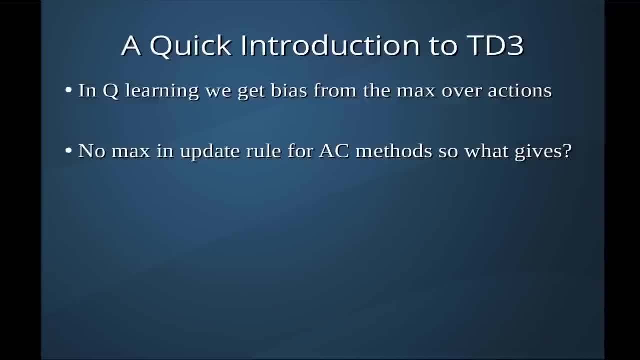 correct estimations of the values of states because of natural high variance, which is typical for deep reinforcement learning problems. However, more fundamentally, overestimation comes from approximation errors. Now, this isn't something they prove in the paper, because this is a result that dates all the way back to the early 1990s, when people were just starting to 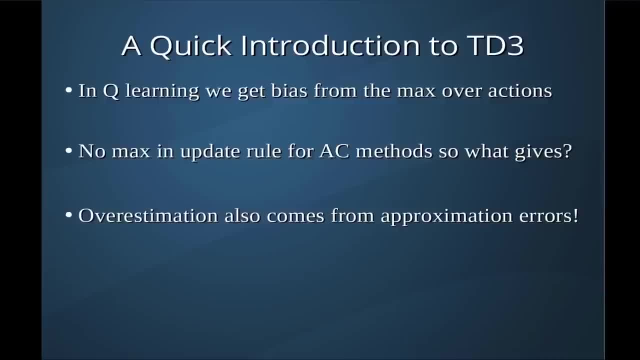 talk about Q learning, And so it's been known for a while. but the basic idea is that when you attempt to use some mathematical method, you're going to end up with an overestimation of the data. So if you use a mathematical apparatus to estimate a function in a high dimensional space, 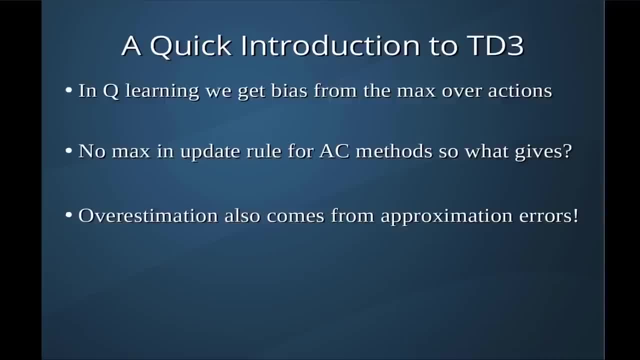 you get approximation errors and that results in overestimation. Now what is our source of overestimation or approximation error? In this case, it's going to be a deep neural network. Neural networks are, of course, universal function approximators. Mostly, there are obvious. 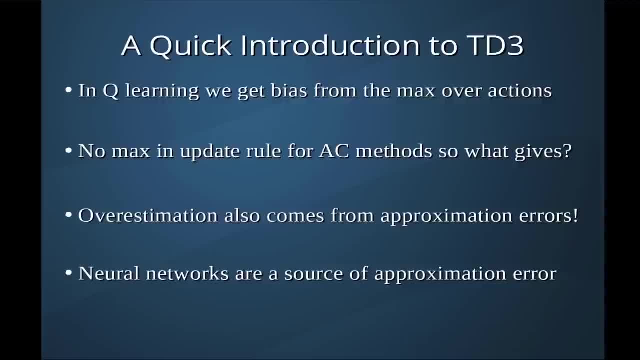 exceptions, you know, discontinuous functions, they can choke on, the function has to be differentiable, and all that good stuff. But for all the stuff we deal with, neural networks are, you know, going to be a universal function approximator, And so that leads to a source of 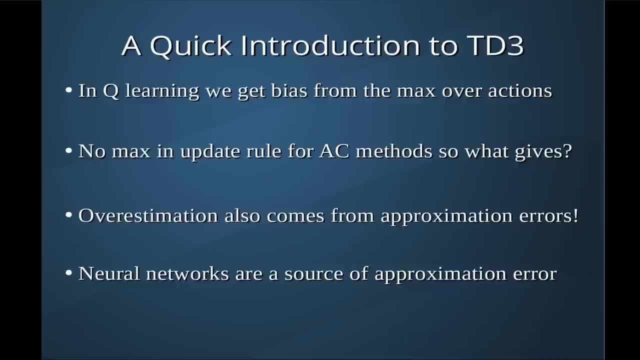 error. Now, this is inherent to any approximation method either: tiling, like binning, anything like that. So it's not that neural networks are bad, It's just whenever you have a function approximation, you're going to have some error. Okay, because you don't have an infinite amount of time to 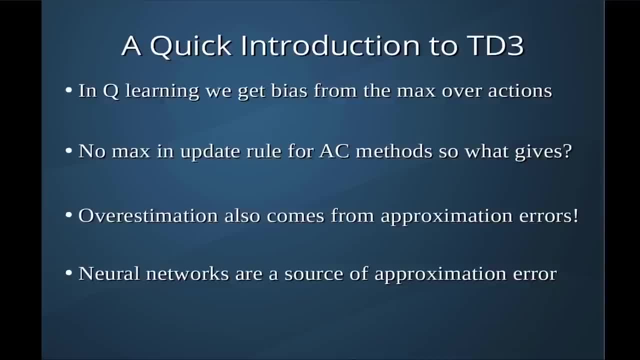 collect an infinite number of samples to get infinite precision. you're always going to have to lop off your estimate at some point where there are more decimal points. you're going to have to lop off your estimate at some point where there are more decimal points. 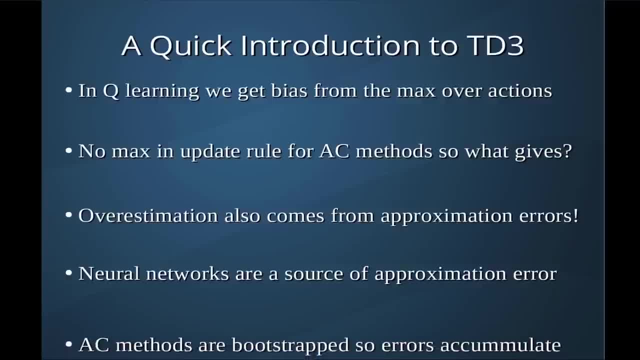 should you be able to collect more data. Worse yet, actor critic methods are bootstrapped. Well, this means is that we're going to be using our initial estimates to perform updates to later estimates, And so you have some errors in your early estimates that propagate to your later. 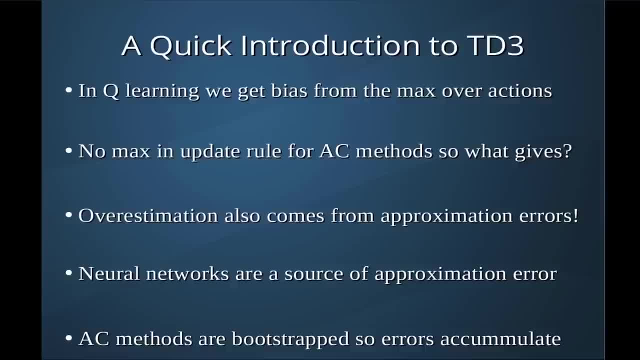 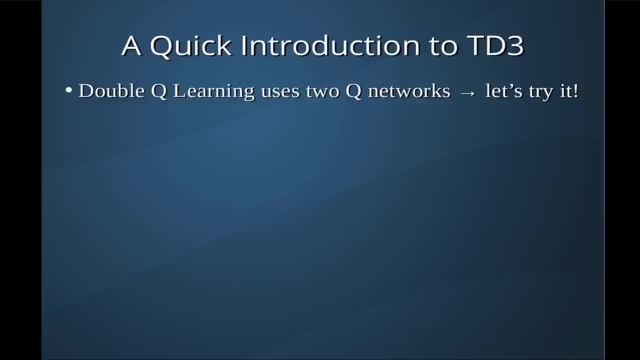 a rather ingenious solution. they use in that algorithm two different Q networks and you alternate their use in the update rule, And so you're never taking a max over actions of the same network that you use to choose an action when you're trying to update the value. 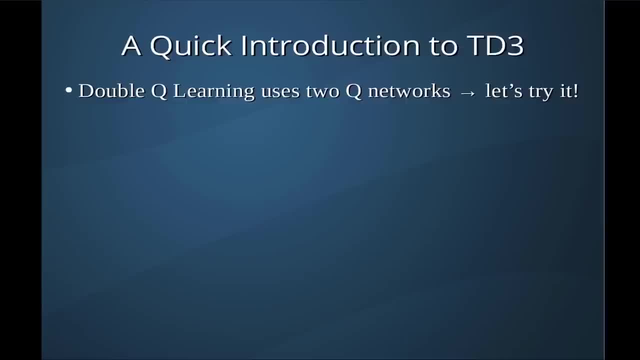 of that action, And so it seems like it's a reasonable thing to try. So, in particular, that's what they do. Now I want to point something out: that in double Q learning- deep, double D, deep, double Q learning- they use a not exactly analogous solution. 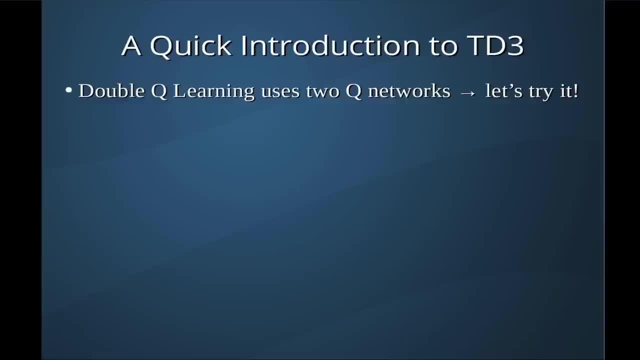 deep, double D, deep, double Q learning. they use a not exactly analogous solution to the tabular case of double Q learning. they use something slightly different which doesn't work in actor critic methods, as they detail in the paper they're going to use. 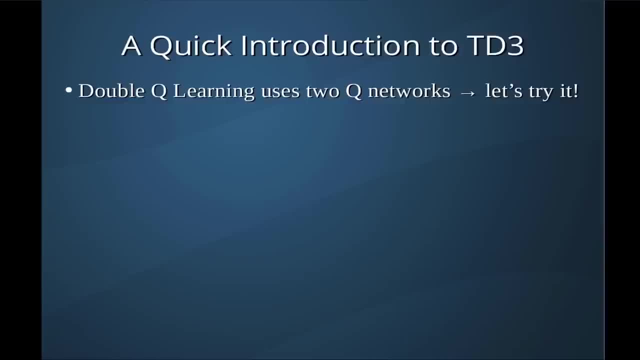 a more exact replica of the tabular version of double Q learning And they're going to perform a slight modification where they're going to clip the inputs of the actions to the Q networks, the double Q networks, which is going to tend to underestimate, and we're going to be taking a min. 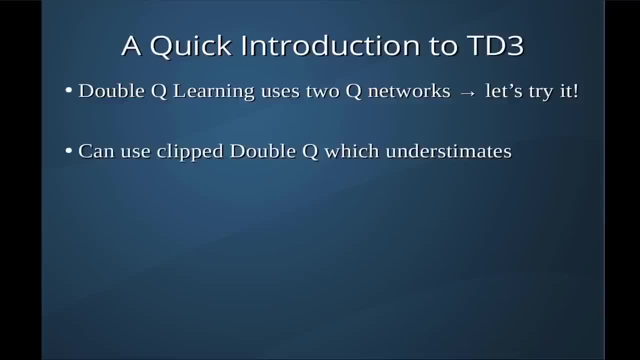 So later on you'll see in the algorithm that we're going to feed some clipped actions to our Q networks and then take the minimum. So whatever the minimum value is, we're going to take that which tends to underestimate. Now you may say, Dr Phil, isn't that a problem? Not really, And 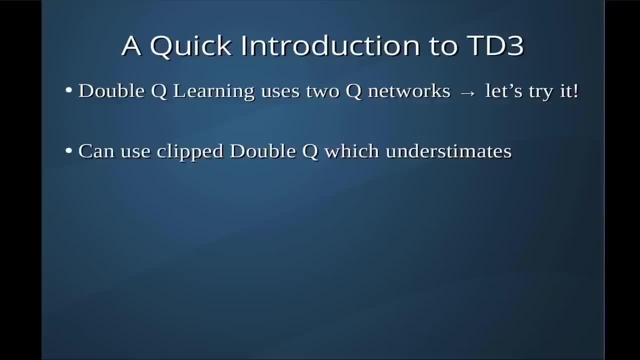 the reason it's not a problem is because if we underestimate actions, those actions become less attractive to the agent And so it's not likely to take those actions again, And so that kind of dampens that out over time, And so that's what they're going to do, And so they're going to. 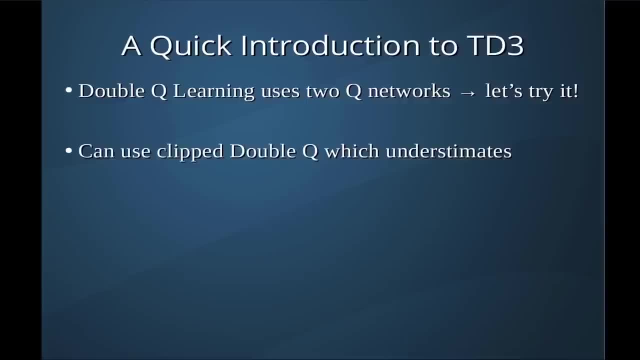 take that out over time. It's a natural feedback mechanism to deal with that issue. So that is rather nice And it's baked right into the algorithm. The other innovation is that they're going to delay policy updates to give the critic network time to converge. So the policy network. 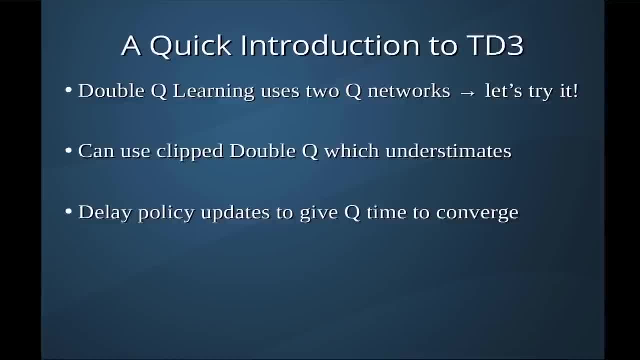 is very slowly changing function, whereas the Q network can change much more quickly. So you have two different time scales there, And that's where the delayed part comes from. Another innovation is we're going to use target networks for the actor and both critics. 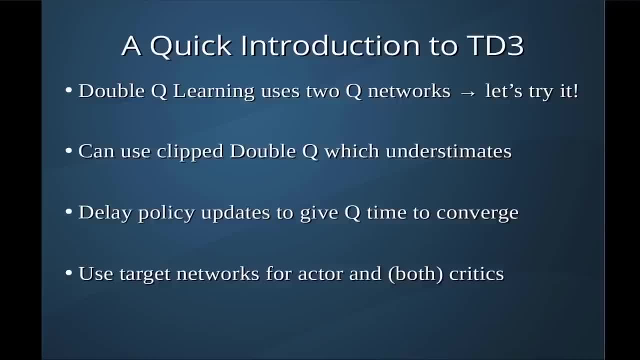 Since we're doing an analog of double Q learning which uses two Q networks, it stands to reason we're going to have two critics And we're going to have target networks for all the things. So we're going to have an actor, a target actor, two critics and 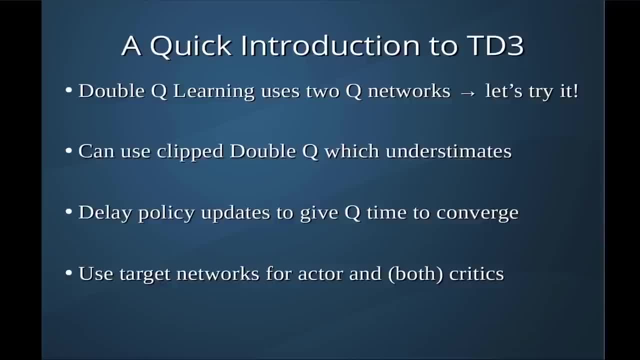 two target critics, So a total of six deep neural networks. We're going to have all the neural networks in the world. The other thing we're going to need is a soft update to the target networks. So you have a couple of options for updating the weights of your target networks. One is you could 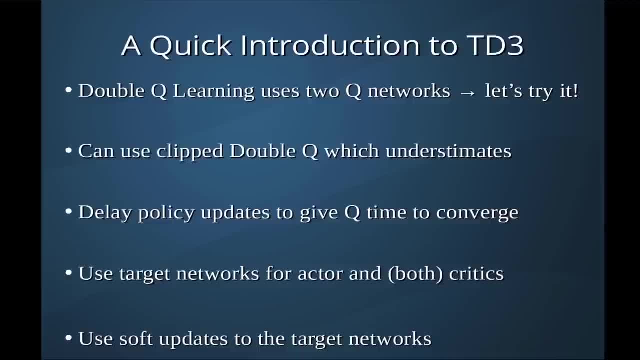 do a stochastic gradient descent on those directly. Another option is to take the parameters from your online networks that you're actively performing gradient descent on and copy those to the target networks directly. Or a third option is to do some slowly varying interpose between the two, So you're going to update the online networks every time. step or 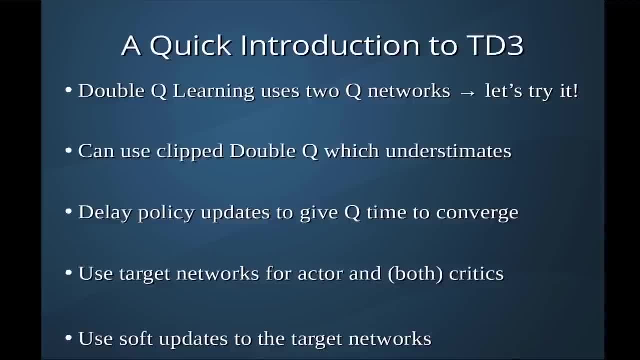 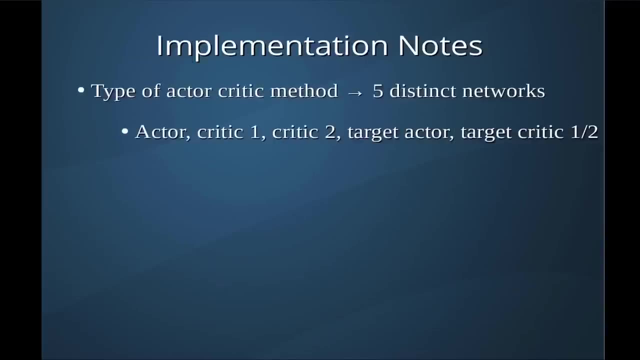 time steps in the case of the policy, And then you're going to do some slowly changing update to those target networks And that will introduce an additional hyperparameter called TAU to our agent, which you will see later. So this is an actor-critic method And we're going to have actually six distinct— I have 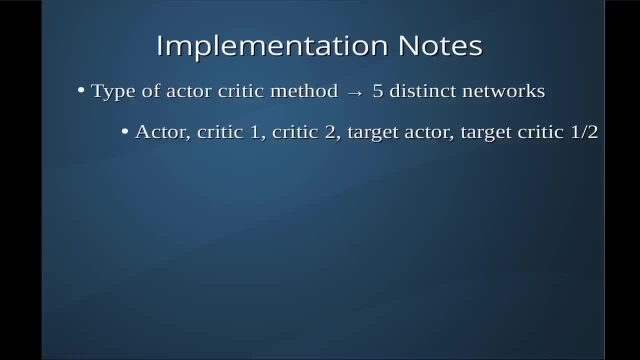 a typo there? Sorry, I can't count, despite having a PhD in physics. So we're going to have an actor, two critics: a target actor and then two target critics. As I said, the purpose of the critic. 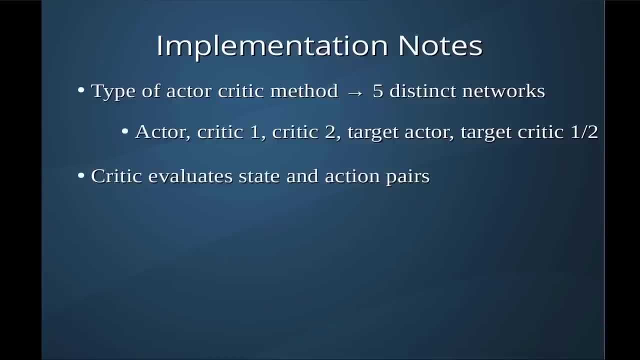 critic is to be critical. it is to evaluate the values of state and action pairs. so it says, hey, in this particular state we took some action. i think this was valuable or not, and that will help to update the agent's estimate of the values of those pairs and to choose better actions for. 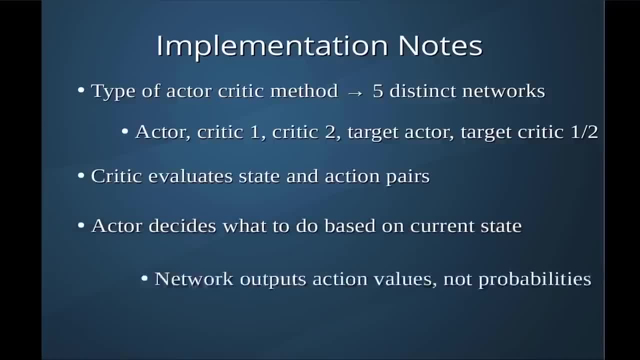 given states. over time, the actor will decide what to do based on the current state, and it's important to note here that our deep neural network is going to output action values which are continuous numbers, not discrete numbers, not probabilities. now, that makes this a deterministic algorithm. that's where the name of the algorithm comes in: twin delayed deep deterministic policy gradients. 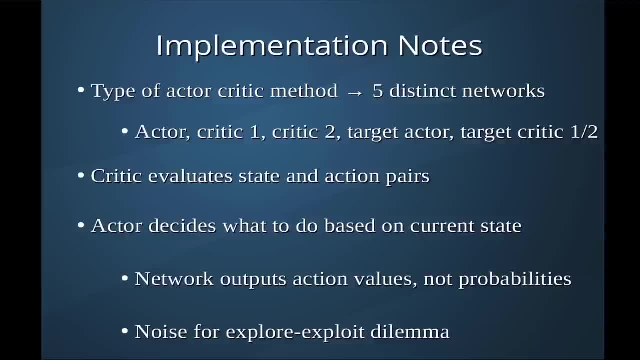 it's an extension of deep deterministic policy gradients, and so we have a bit of a problem there, because we're dealing with approximation, right, we're approximating a q function, we're approximating a policy, we're approximating all the things and we never know exactly. 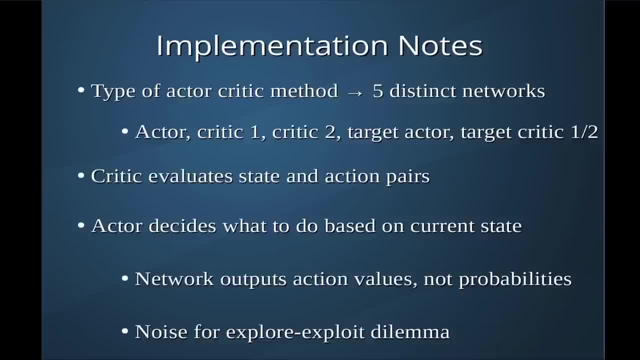 how accurate our approximations are, and so we never know if we are correctly evaluating states and action pairs. so we never know if, given some state, if this action is really the most beneficial action we could possibly take, or if there's some other more beneficial action out there waiting to. 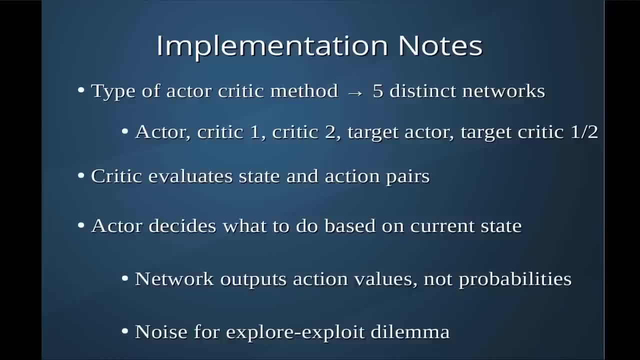 be discovered. that is called the explore- exploit dilemma. do we explore suboptimal actions or exploit what we think are the most beneficial actions? and the extent to which you engage in those two activities is the dilemma, and there are a number of solutions to that: deep q, learning uses, epsilon, greedy action selection. 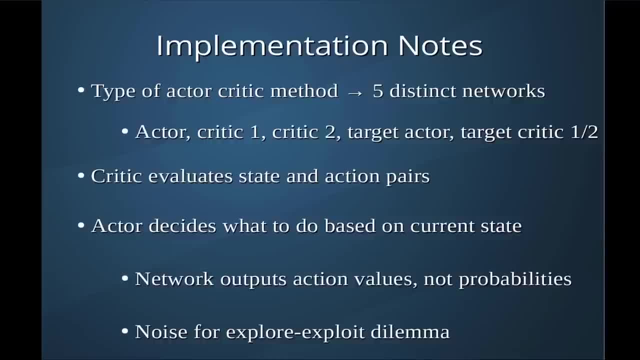 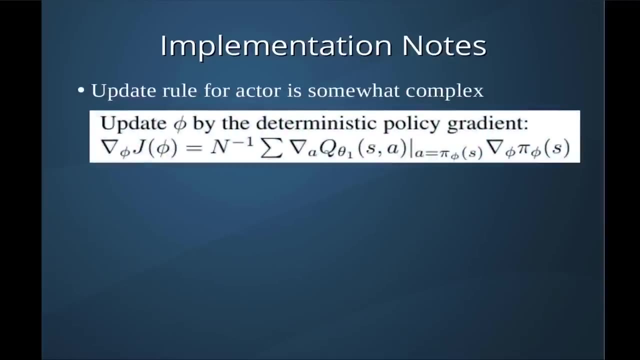 where you just take random actions some fixed proportion of the time. but in this case we're going to be adding noise to the output of our actor network when we decide what actions to take. the update rule for actor looks a little bit scary, but it's actually not so. this is the update. 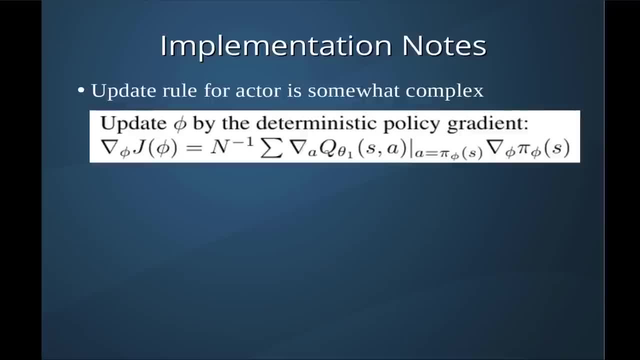 rule from the paper. j is going to be our loss function for our action and we're going to be taking the cost function with respect to the factor. it's a function of phi, the parameters of the policy network, and you want to take the gradient of the cost function with respect to the parameters. 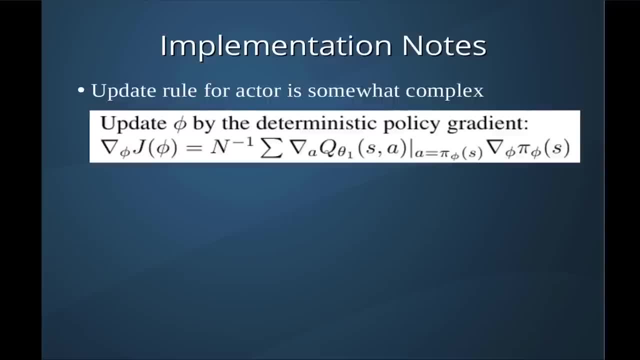 of the policy network and it's given by one over m times the sun, the sum or a mean, an average. so our loss function is going to be a mean and it's going to be the product, in this particular equation, of the gradient of the first critic network with respect to the actions chosen by the policy network. 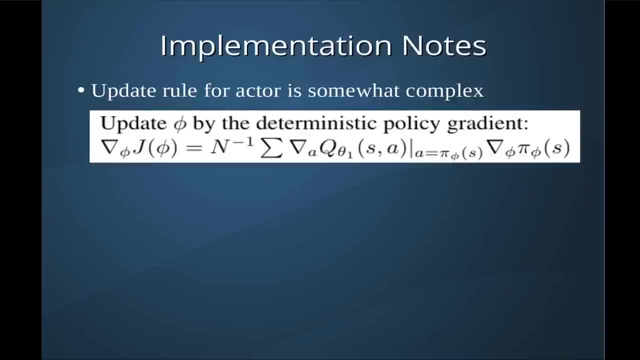 multiplied by the gradient of the policy network with respect to its parameters. now this looks intimidating, but it's actually not. this is the application of the chain rule to the loss function. so they have taken the gradient of the loss function with respect to phi, but the loss 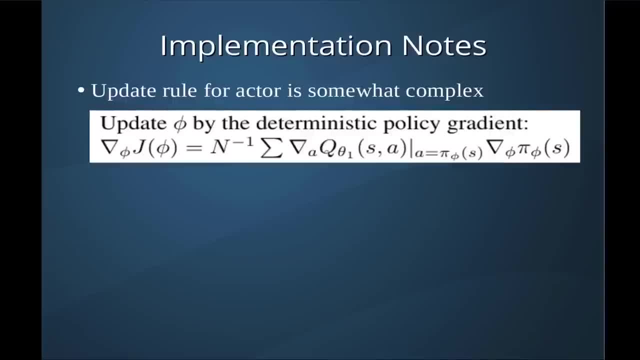 function is proportional to the output of the first critic network. of course the first critic deep neural network has its own set of neural network parameters. it doesn't have an explicit on the neural network parameters of the policy network, so it's very difficult to take a gradient. 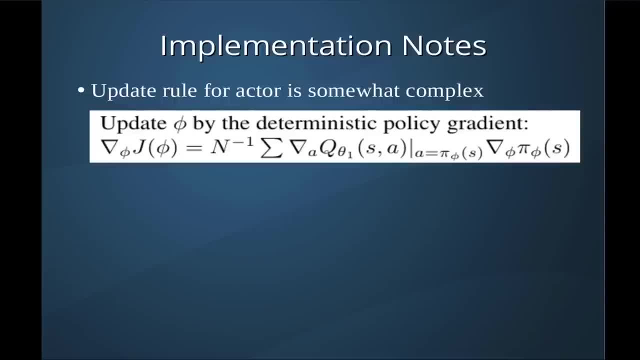 right, something that doesn't depend on something else. so the dependence is implicit. it comes from the fact that those actions are chosen according to the output of our policy network, and so you have to apply the chain rule. in reality, all we're going to do is the following: we're going to 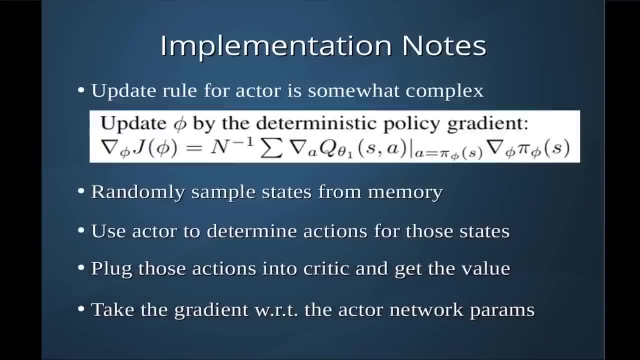 randomly sample states from our memory. we're going to use our actor network to determine actions from those states. so we're not going to be using the actions from our memory. we're going to figure out what actions the agent thinks we should take. now we're going to plug those actions into our critic. 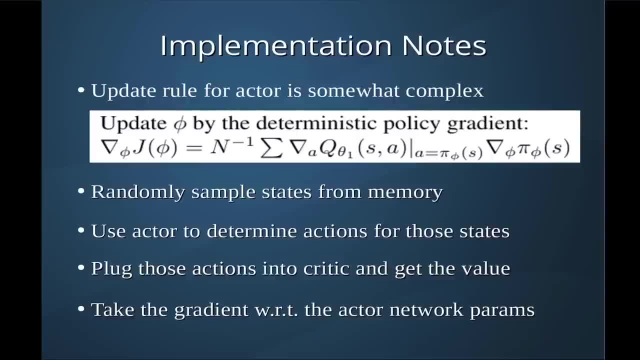 and get some value. specifically the first critic, never the second, only the first. that's just by design. and then we're going to take the gradient with respect to the actor network parameters. now we don't have to calculate that gradient. tensorflow is going to do it for us, we just have to do the 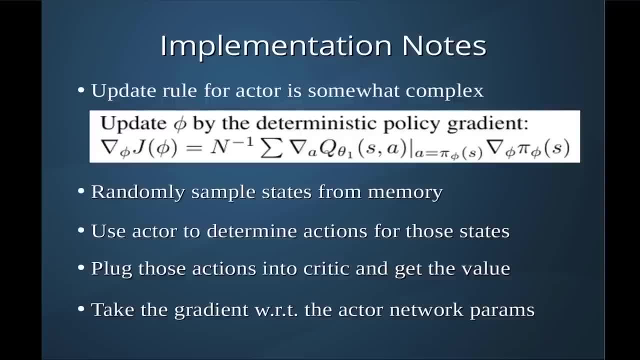 first three things: where we have sample states using actor, determine actions for those states and plug those into our critic a with the states to get some value and then take the gradient with respect to the actor network parameters. now, keep in mind that this update isn't performed every time step. it's performed every. 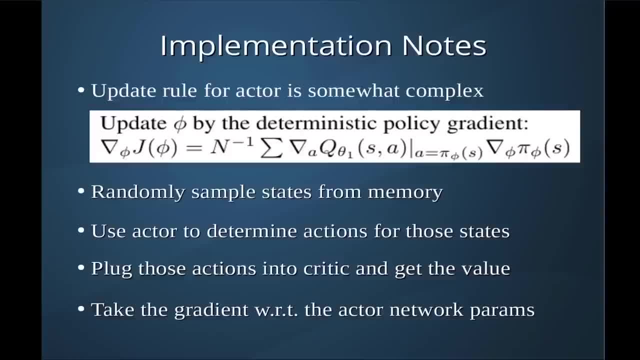 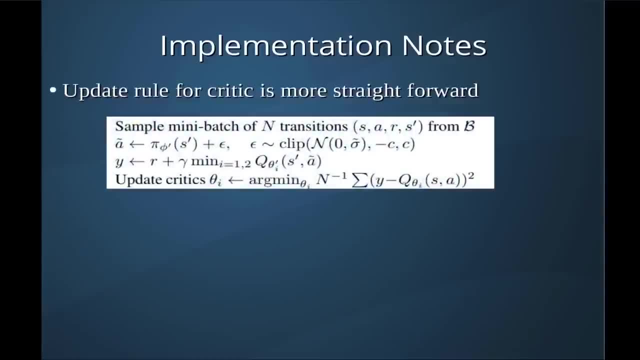 other time. step how often you perform. it is a hyper parameter of the algorithm, but it is not every single time. step now nominally. the update rule for the critic is a little more straightforward. so again, you're going to sample a batch of transitions from your memory. 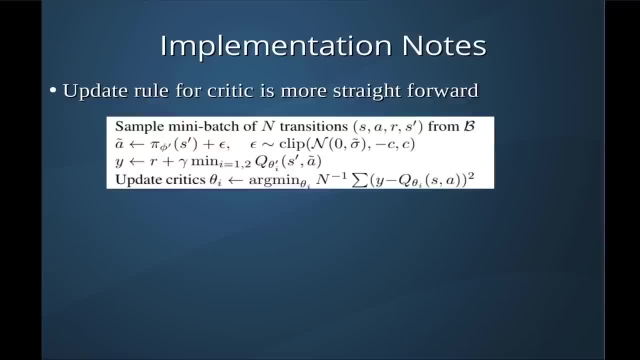 you're going to put the new states that the agent receive observed after taking some action through the target actor network. that's that a tilde parameter there. and then you're going to add in some clipped noise. it's just going to be a normally distributed noise with mean 0 and some. 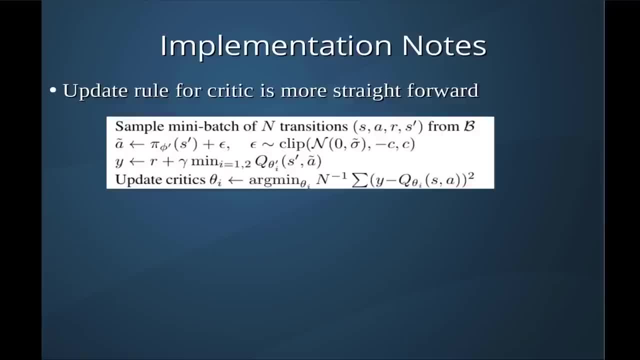 standard deviation, something like 0.2, and we're going to clip it in the range of minus 0.5 to positive 0.5. so that's where the clipping comes in for our double q learning and the actual double q part comes in. 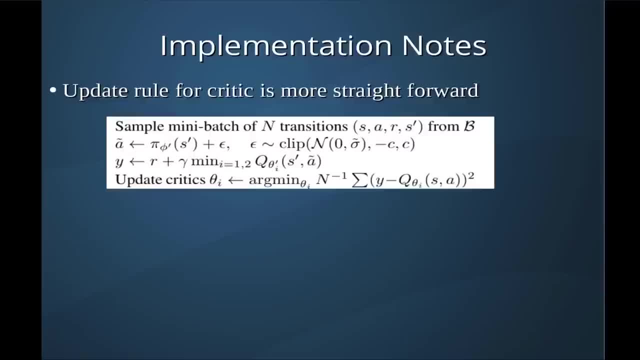 when we calculate our targets y. so we're going to take the reward that we sample from our buffer and add it to the product of the gamma, which is the discount factor- 0.99 or so, and we're going to take the minimum of the output of the two target critic networks. so we'll say we're going. 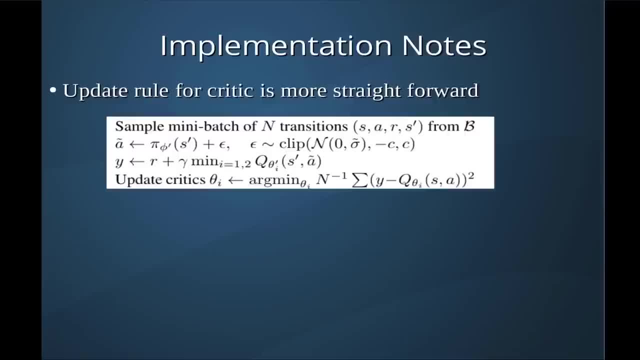 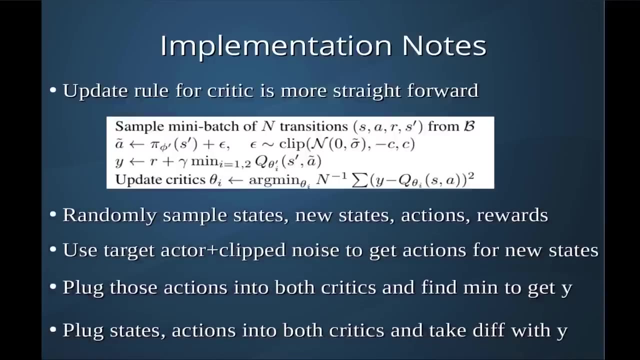 to feed the new states through the new states and those clipped actions through both target critic networks, and then we're going to see which one is the minimum and take that for our target value and we're going to input that target value into our loss function. again, you have a 1 over n multiplied. 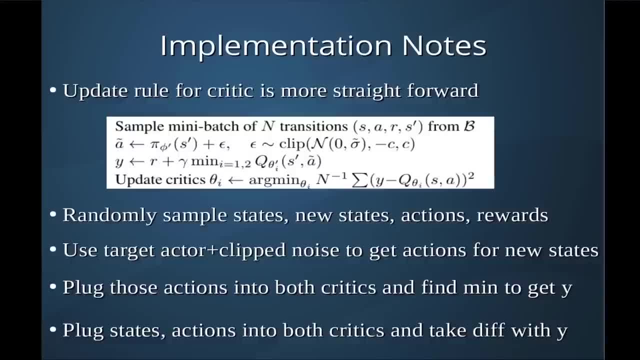 by some, multiplied by something squared, that is a mean squared error and it's the mean squared error between that target y and the output of both of our critic networks. so our loss is going to have two different components. it's going to have a loss for critic 1, where you have q, sub theta, sub 1. 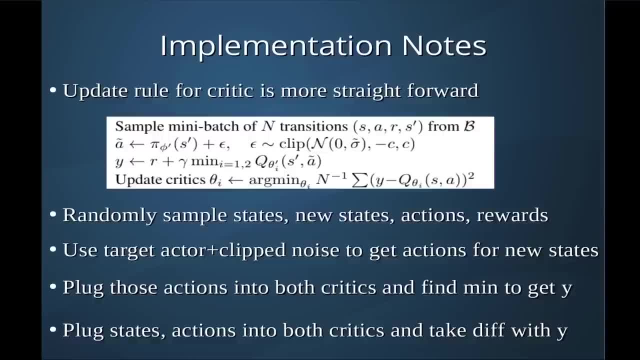 and then i'll have a loss for q sub theta sub 2.. so we'll have two losses. and then when we do our gradient tape, we're going to have to pass in the persistent equals true flag to our function call so that it keeps track of network parameters between gradient. 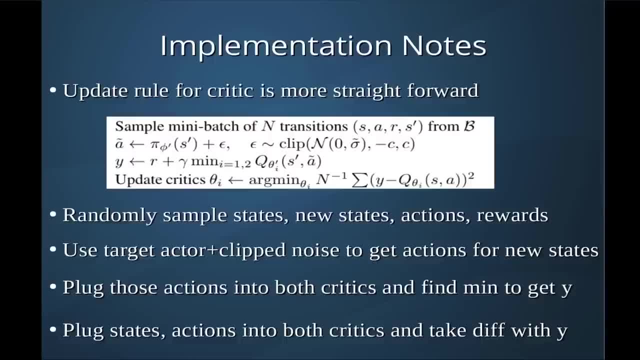 ascent steps and so these. the rest of this verbiage is just kind of the verbal description of what we want to do. it's going to be much easier once you see it written in code. i assure you it's not that difficult. next we have to handle the question of target network. 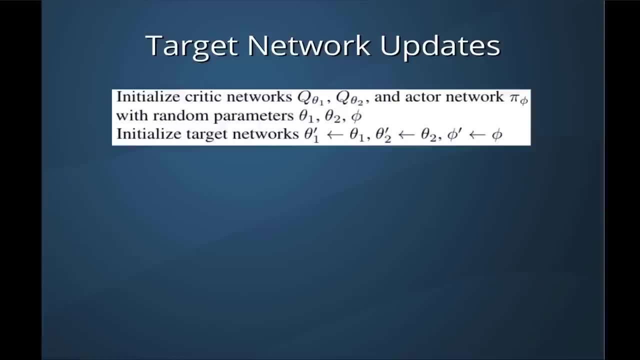 So at the very beginning in our constructor for our agent class, we're going to go ahead and initialize actor, two critic networks and then a target actor and two target critic networks And when we first start out we want to initialize those target networks. 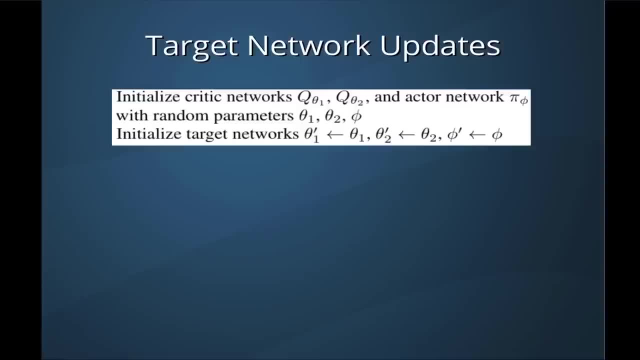 with the exact values of the online networks, And so we're going to have a special case in our target network update function that handles the very beginning of the program And every other time step we're going to use the following expression to update the weights: 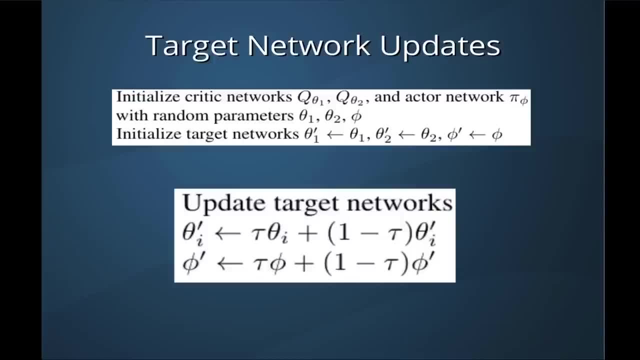 So on the left side you have theta and phi prime, where the i on the theta denotes either critic one or two. Phi is the parameter for our critic network- excuse me, policy network- and the thetas are the parameters for our critic networks. 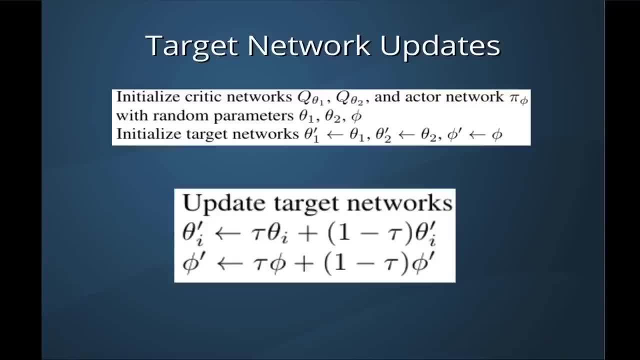 And so you're going to multiply tau, some small number- 0.005 in this case- by the values of the current online network and add in one minus tau times the old values of the critic network. So it'll be a small number multiplied by the current values of your online networks. 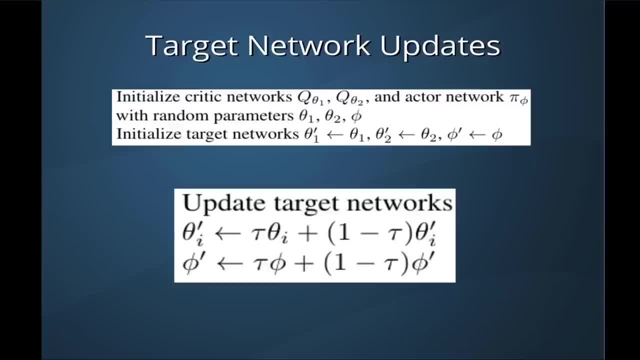 plus something that's almost one multiplied by the old values of your target networks. It's going to be a slowly changing update to our target networks. Other thing to note is that we're only going to be performing this update when we update the actor network. 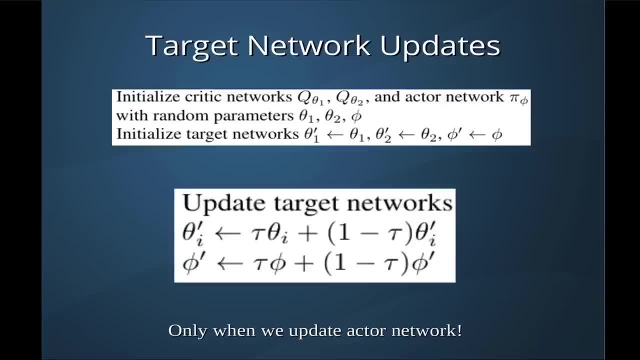 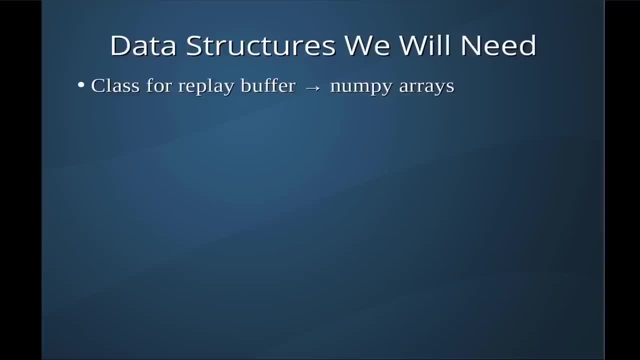 So it's not every time step In this case, it'll be every other time step- Very, very important. So for this program we're going to need a number of data structures. We're going to need a class for our replay buffer, the agent's memory. 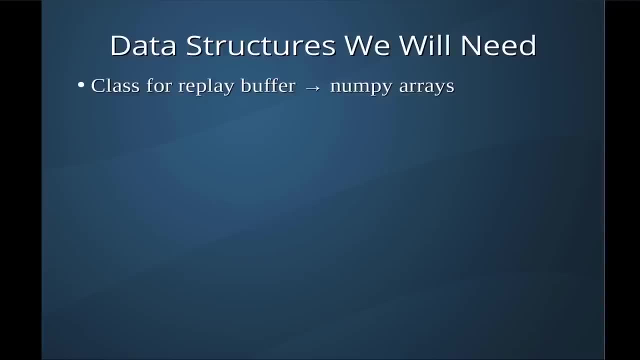 Now I like to use numpy arrays. It is not the best way or the only way to do it, It's just my preferred way. So follow along with me in the tutorial, Do it that way And then, when you play around with the code later, to understand it better. 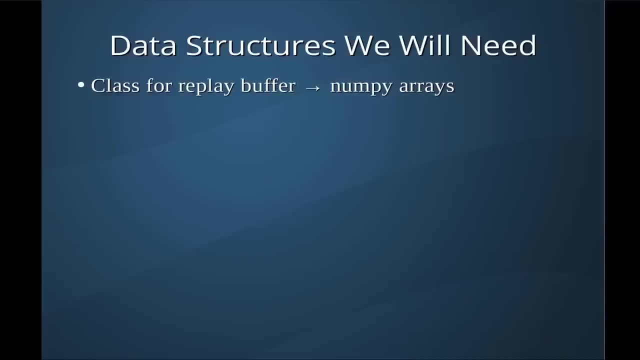 go ahead and rewrite the replay buffer to something that makes more sense to you. That's a great way to get started with. modifying the program is with the replay buffer. Next we're going to have Classes for our actor network and our critic network. 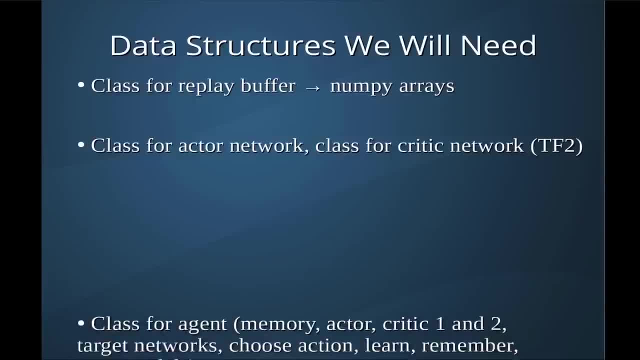 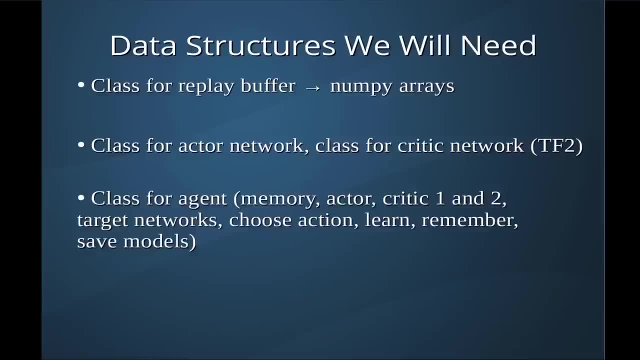 And those are, of course, written in TensorFlow 2.. We'll have another class for our agent, And that is really going to tie everything together. It's going to have a memory that keeps track of transitions. It's going to have an actor, two critics, target networks for each of those. 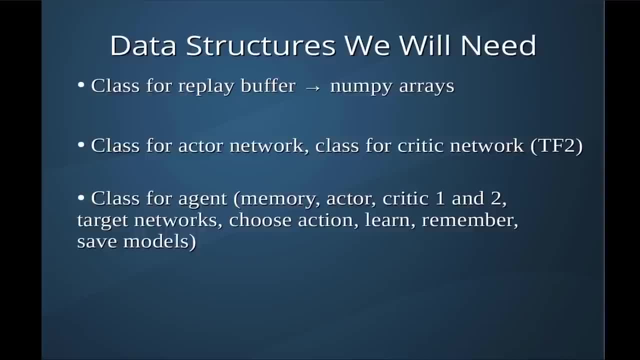 A function to choose an action based on the current state, A function to learn that performs the update rules we just went over, An interface function with its memory that I call remember, just to store transitions In the agent's memory, as well as functionality to save models and perform target network updates. 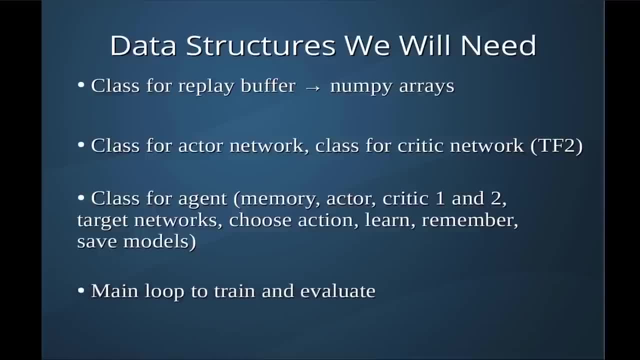 which I forgot to write here. Finally, we're going to need a main loop to train and evaluate our algorithm. So we're going to be using the open AI gym and the bipedal walker in particular, because this is a kind of difficult environment for other algorithms. 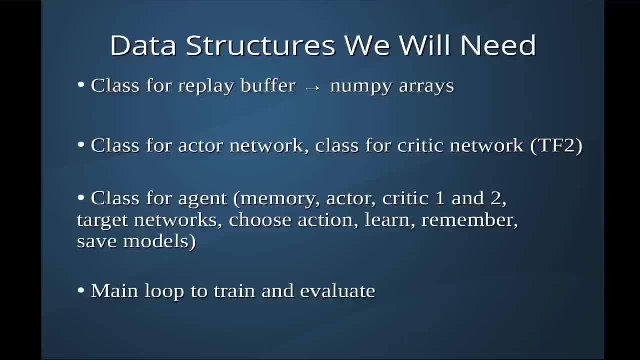 It's a continuous action space with a pretty large state space. I think it has 24 different components in the state, So we're going to be using the open AI gym and the bipedal walker in particular space. if I'm not mistaken, some relatively large number. So it's a bit difficult for agents to 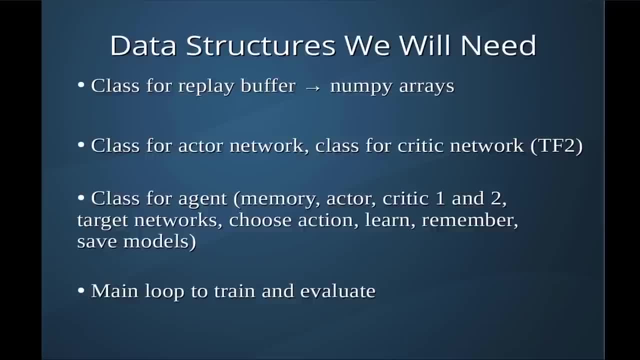 learn And in fact it's going to take my computer around six or seven hours to complete the evaluation. I'm filming this after I do the code, So it'll take a while to run. So if it takes forever on your computer, don't panic. That's normal, quite normal. So all that out of the way. 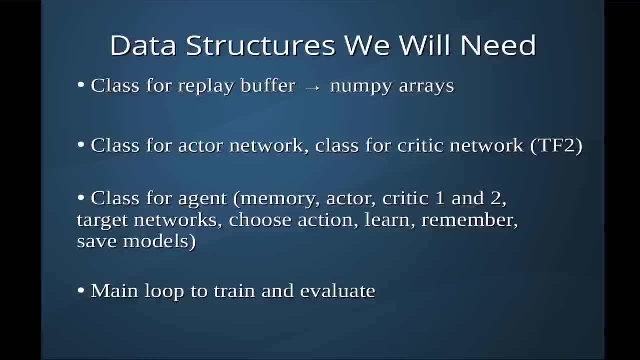 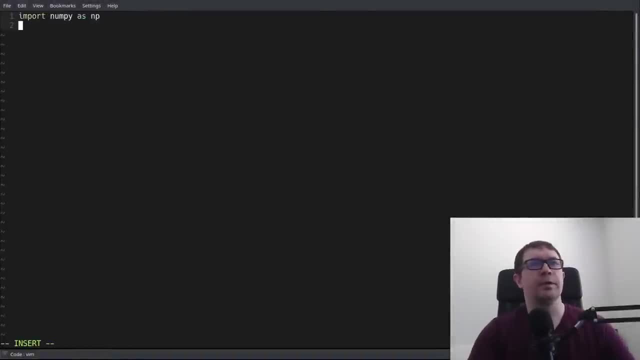 let's go ahead and get started in the coding portion of this tutorial. All right, so we begin, as usual, with our imports. We will need NumPy, the base TensorFlow package. We will need TensorFlowkeros. We will need layers. 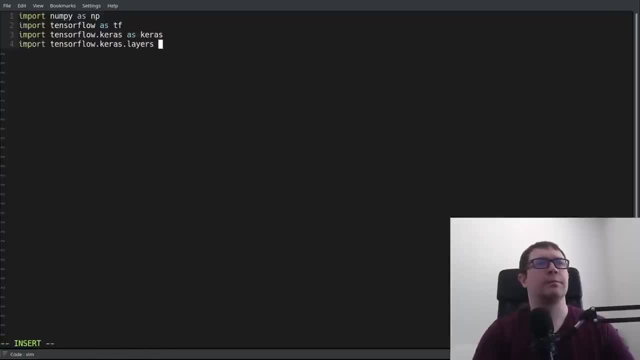 from: yeah, import dense, That is for constructing our deep neural networks, And we will need our atom Optimizer or the gradient descent, And we will need OS for file joining operations, for model checkpointing. Let's start with our replay buffer class Now. this should be very familiar to you. 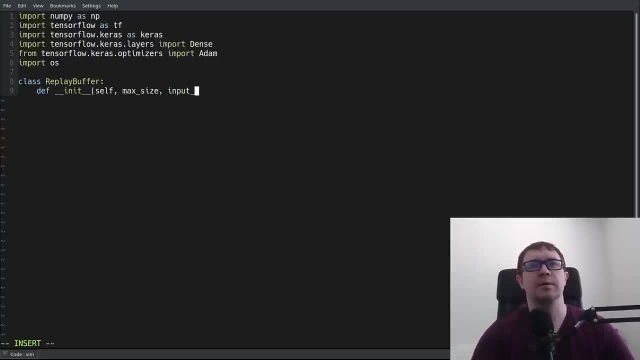 if you're used to deep Q learning, We'll need a max size, input, shape and number of actions as input to our constructor. Now, remember, we're dealing with continuous action spaces, So this number of actions is really a number of components to our model. So we're going to need a number of 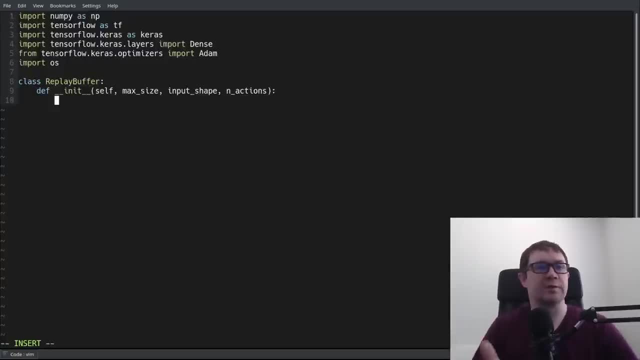 components to our continuous action. I just name it that for consistency with my deep Q learning code. So we will save the appropriate member variables. We use a memory counter instantiated at zero. because our memory is finite, We'll need our state memory, which we'll initialize as zeros. 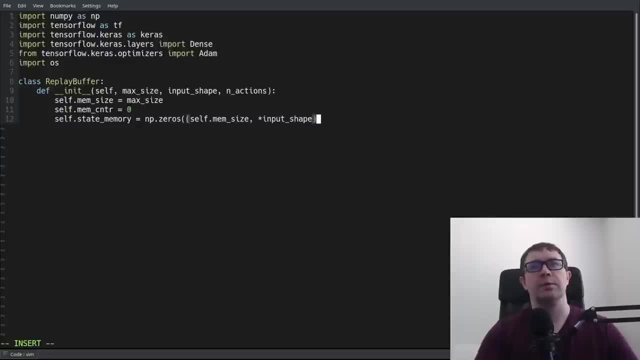 and the shape, mem size and star input shape. The star idiom just unpacks a an array. in this case, whatever the shape of our input dimensionality is from our environment, We will of course need a new state memory And that's the same shape that keeps track of the new. 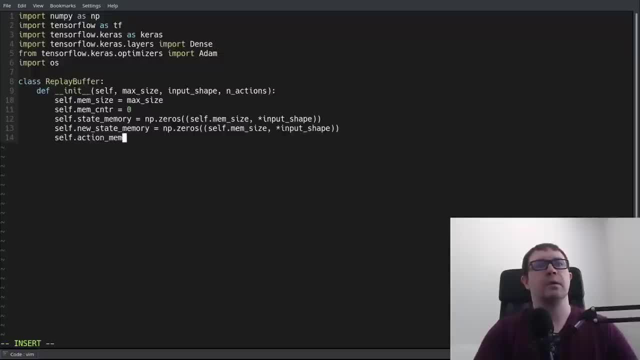 states that we are going to see an action memory And remember. of course again, number of actions is number of components to our action. Reward memory in the shape of memory size and a terminal memory. We're going to use NumPy, NumPy. 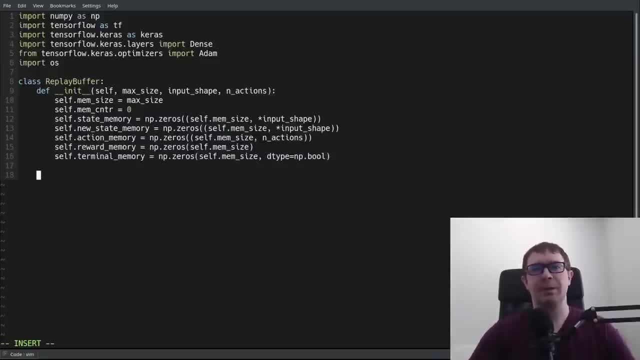 NumPy bool as our data type. That'll keep track of our terminal flags, The reason being that the value of the terminal state is always zero, And so we keep track of the done flags from our environment to accommodate that. So let's store a transition That takes the state observed, action taken, reward received: new state. 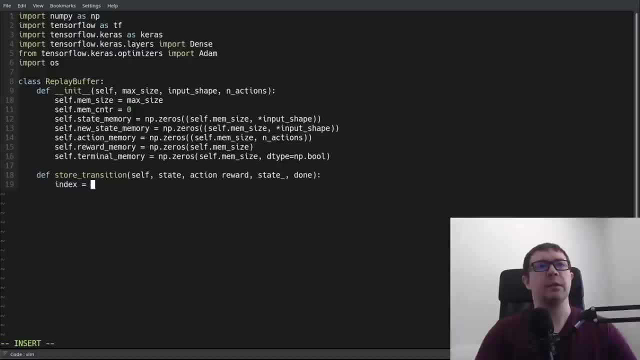 observed and terminal flag received as input. We want to know what the first available memory position is, And that's memory counter modules, mem size that has a property that it will overwrite earlier memories with newer memories as soon as the memory fills up And then go ahead and 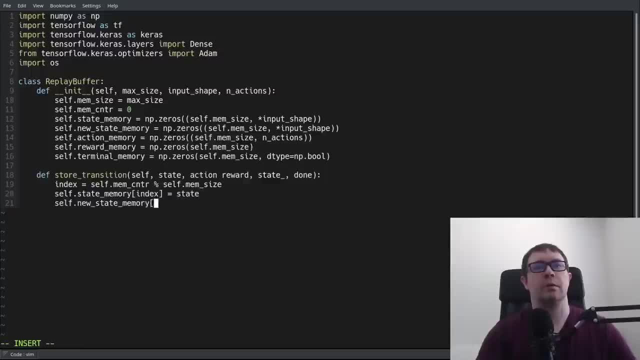 save our variables, We'll state underscore, terminal memory, And that's all of them. I believe, and very important, we want to increment our memory counter By one. Next, we have to handle the function to sample our buffer, And that'll just take a batch. 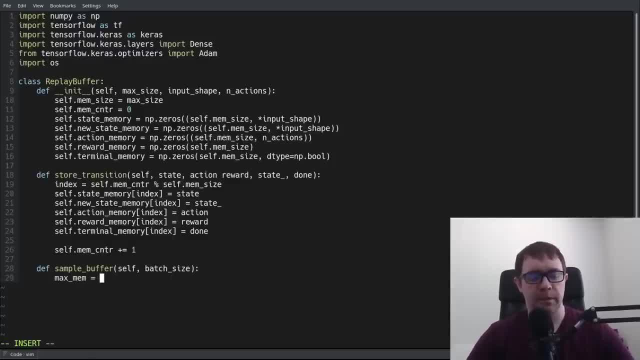 size as input. We want to know what the position of our maximum field of memory is, And that's given by this minimum of mem counter and mem size. because we don't want to sample zeros, we initialize our memory with zero, So we just sample the entire buffer. then we're probably going to end up sampling. 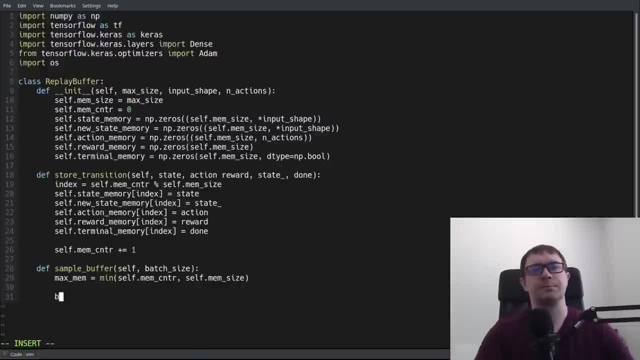 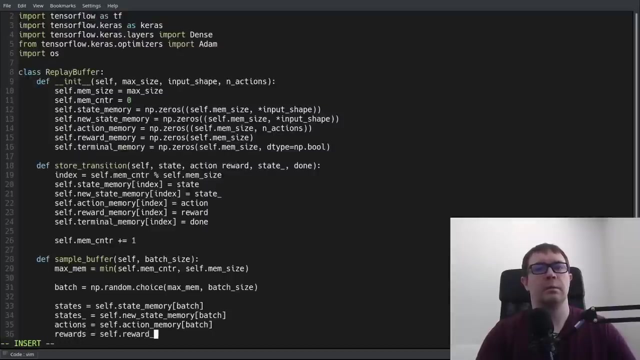 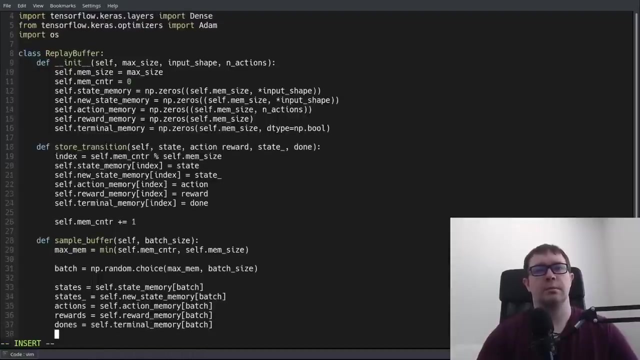 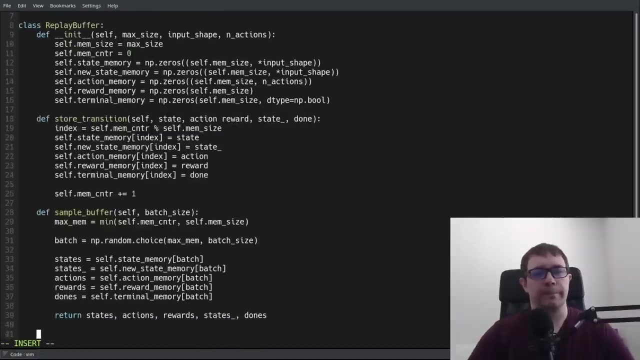 zeros Until we fill up that buffer, which is totally useless. So then the batch is going to be a random choice from zero to maximum in shape, batch size. Then go ahead and do you reference our variables Correct And dones. Alright, that wraps up our replay memory. That's very, very simple, Probably the most straightforward. 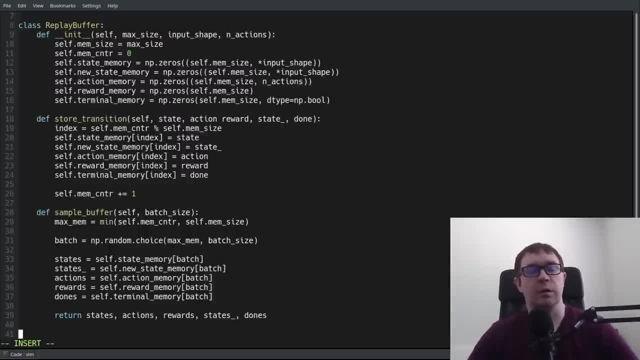 class and the entire project. Next, we're going to move on to our critic network. Alright, so now we're going to leave that aside for a few seconds And we're going to quickly jump over to our Next. we're going to move on to our critic network. 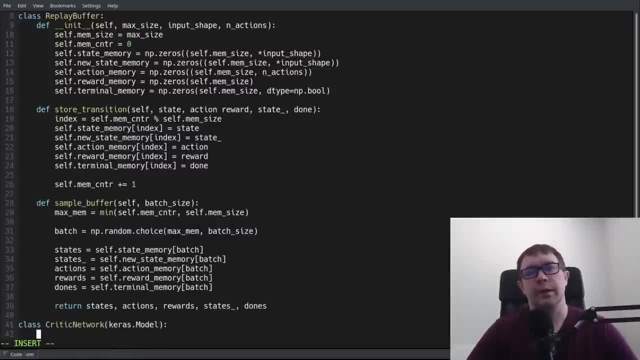 And then we're going to save our dp from in here, So we're going to just do a little typo. this will dump back into here. Now, let's say I'm down loop features That will derive from charismodel, so we get access to all of the properties of that particular base class. 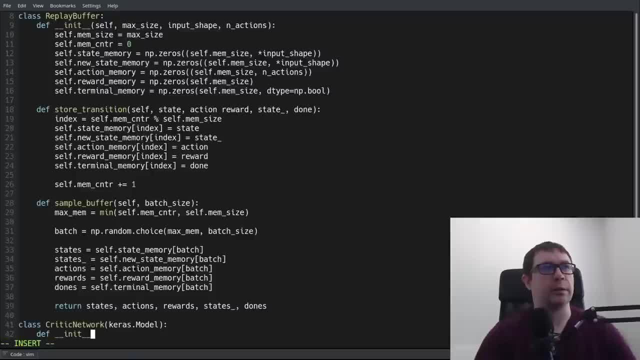 That'll help with using the gradient tape for learning. later on We're going to take some inputs for the number of dimensions for the first and second fully connected layers, number of actions- again number of components, a name for the purpose of model checkpointing and a checkpoint directory. 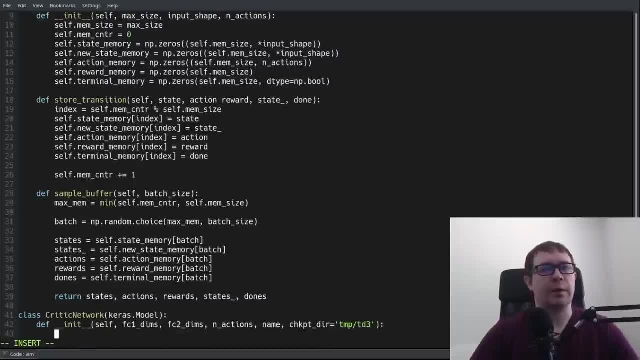 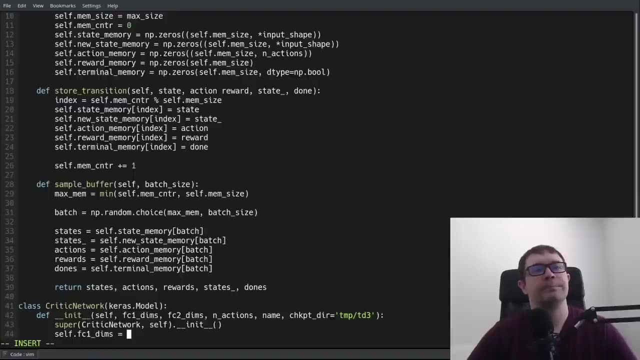 We will have to do a make directory on that before you begin, otherwise you will get an error and it will not work. Let's call our super constructor and start saving stuff. Do I need to do that? Yeah, why not? So? 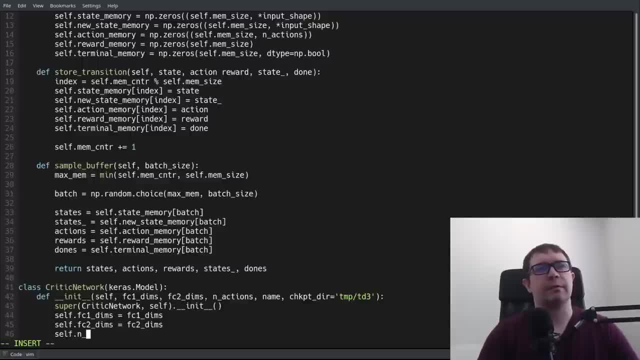 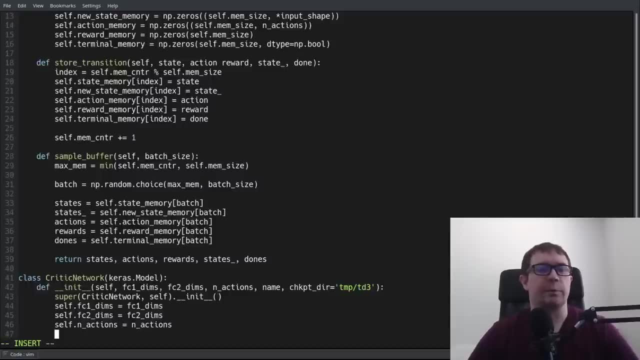 The purpose of the name. The purpose of the name is the fact that we're going to be saving target networks as well as regular networks, and there are going to be two critics, so we want to be able to keep all of those straight when we handle model checkpointing. 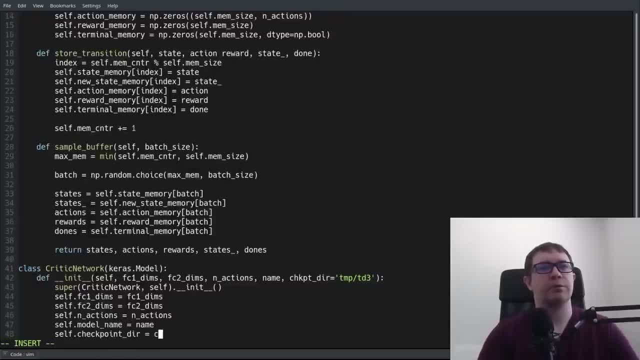 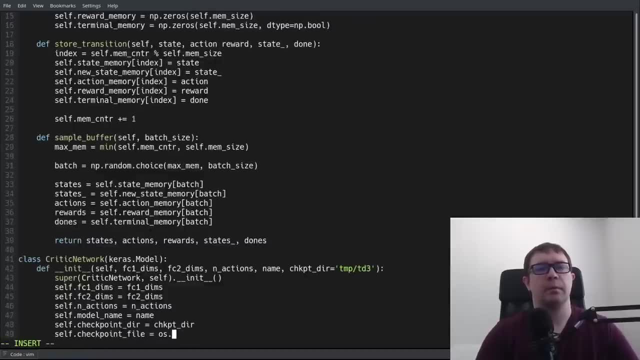 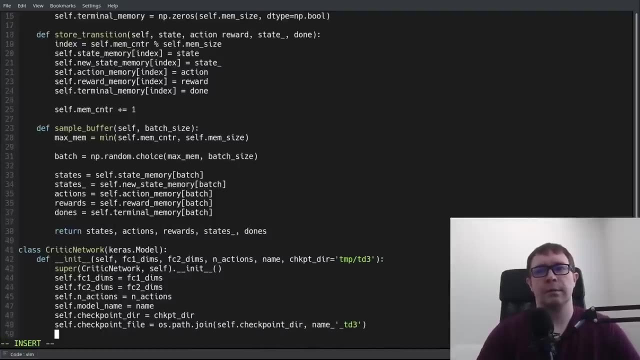 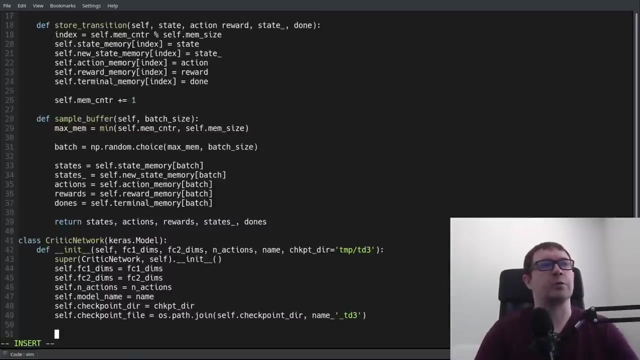 So we'll save our model name checkpoint directory and the checkpoint file And I like to append the algorithm name to the checkpoint file so that if I do everything in one working directory when I'm experimenting, all the names tell me exactly which file correspond to which algorithm. 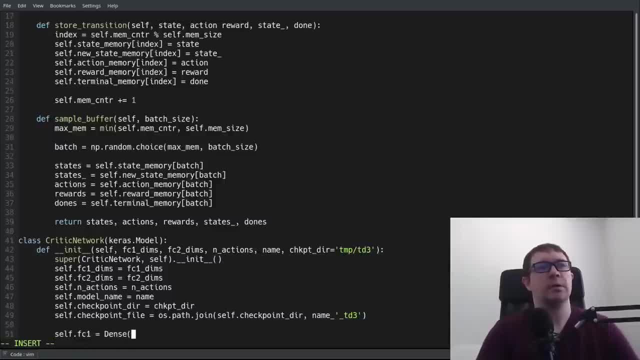 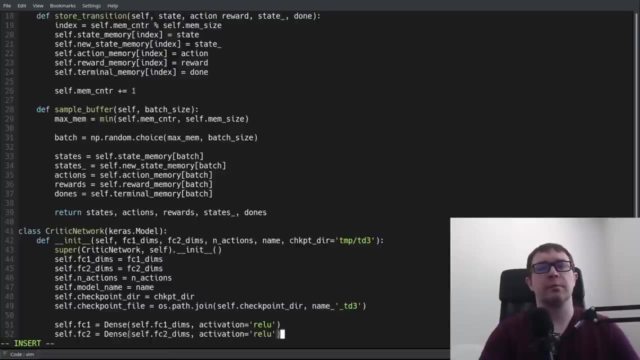 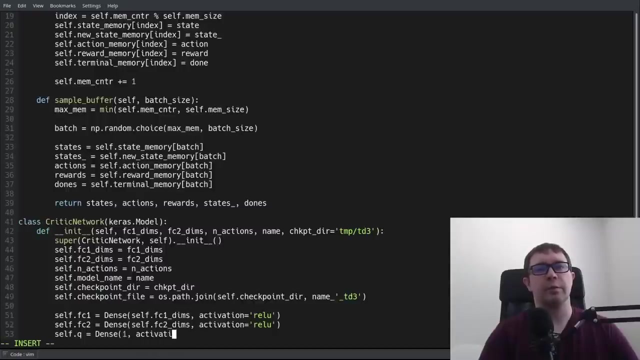 You don't have to do that, it's just my own personal convention. So for our deep neural network, we'll start with a dense layer with a relu- ReluActivation, Second dense layer with reluActivation And an output that will be single-valued with no activation. 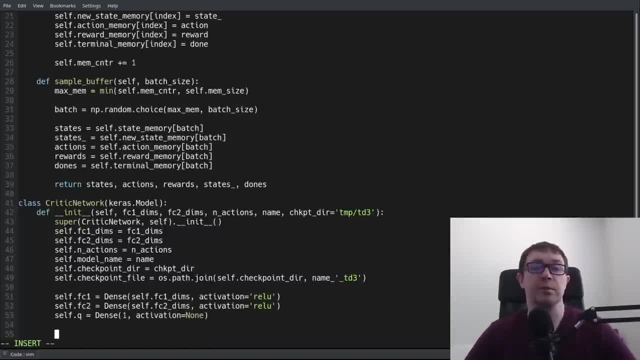 Now keep in mind. one interesting thing about TensorFlow 2 is that we don't have to specify the number of input dimensions. it infers it from the inputs. That's a pretty nice Feature. So now we define our feed forward. In this case, we call it call. 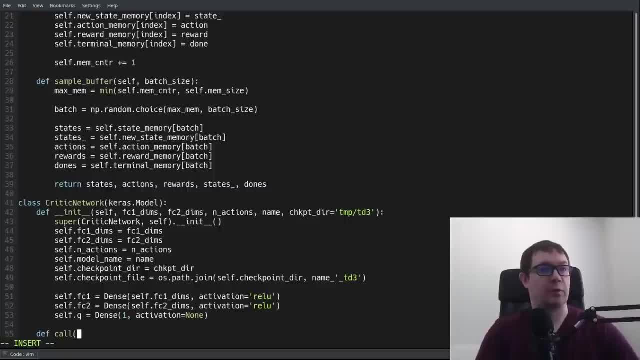 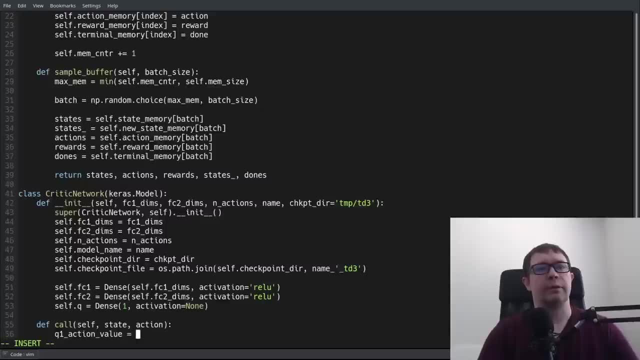 That'll allow us to use the name of an object as a function call. basically, We need a state and action as input. We'll have a Q1 action value And we will want to concatenate our state and action along the first axis. 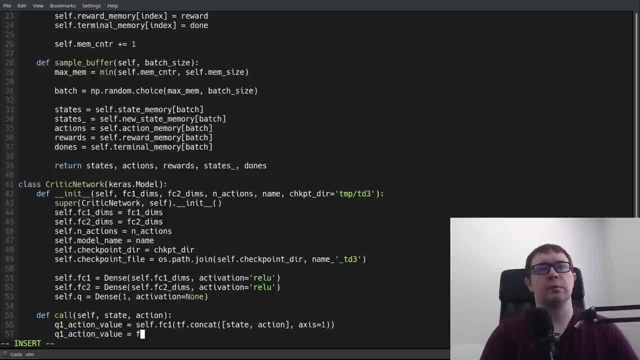 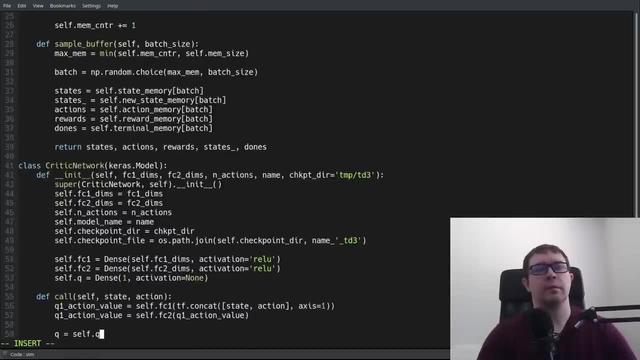 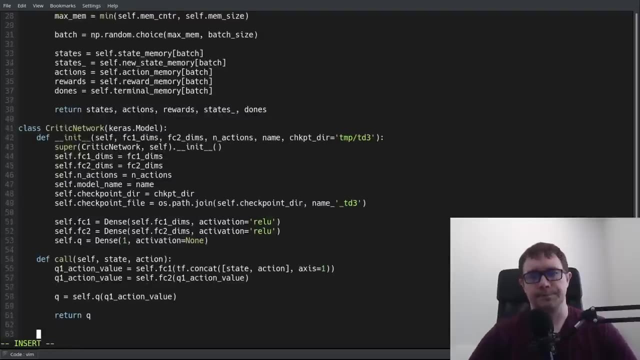 And We will feed that. We'll feed that through FC2, Q1 action value And then pass it through the final layer: Action value and return. Now keep in mind that the critic evaluates the value of both the action and state. 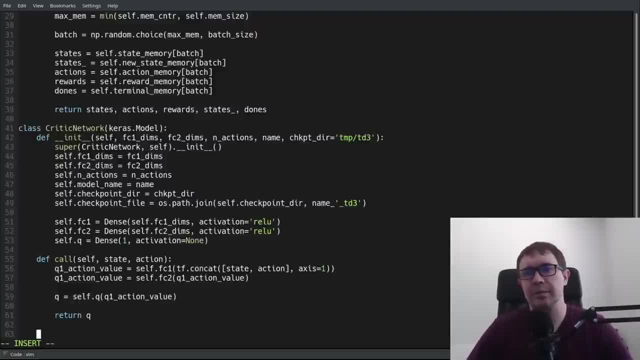 so that's why we have to concatenate the two values. That is it for our critic network, Very, very straightforward. Next, we're going to handle our output Actor network, And that again derives from charismodel, Just the same as the critic network. 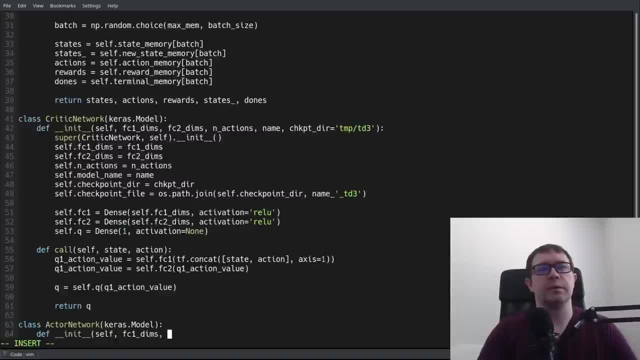 Our initializer takes dimensionality as input again as well. Number of actions. And you know what Did I? I'm sorry, I'm checking something here. No, I did not For a second there. I thought I passed in input shape to the critic network. 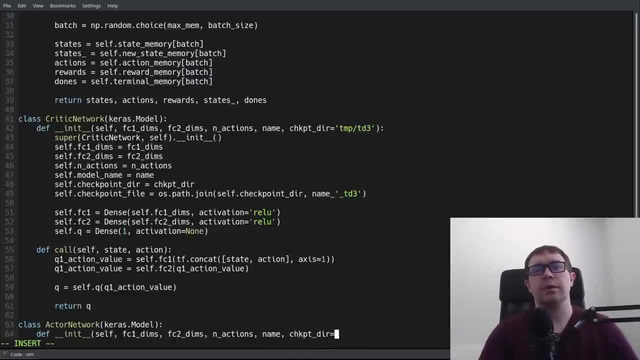 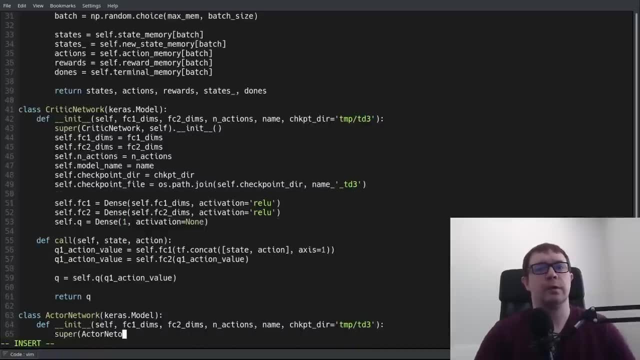 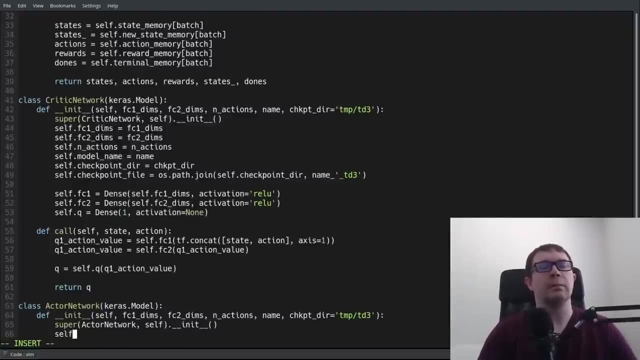 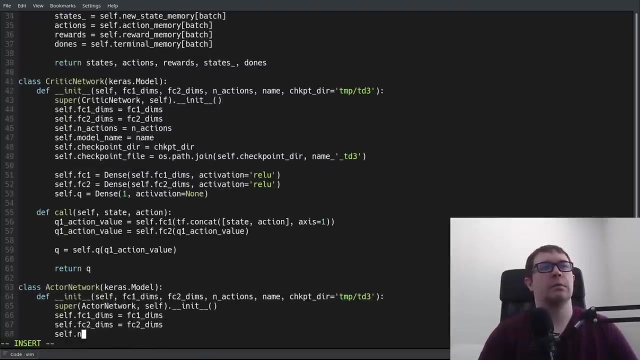 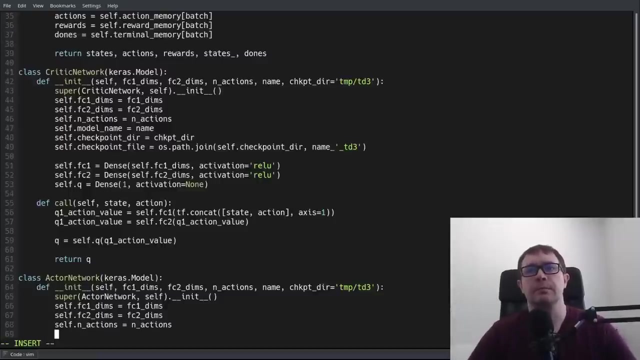 That would have been totally unnecessary. Checkpoint directory equals temp td3.. We want all of the models to live in the same directory. Very, very helpful, And then we can go ahead and start saving stuff. And I'm looking at this and as I look at what I'm doing here, 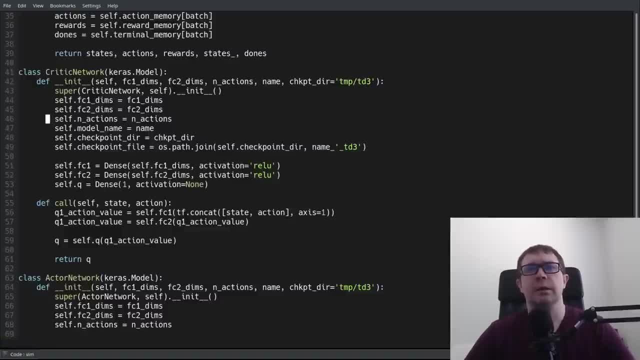 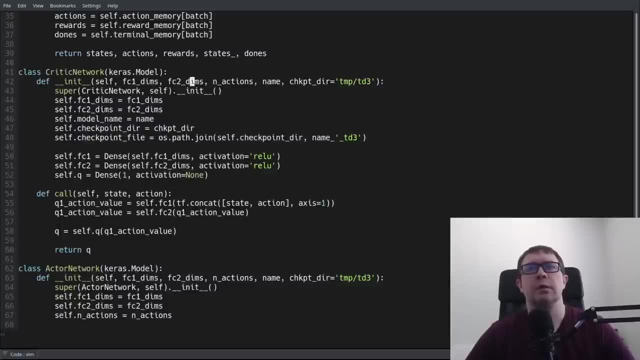 so I like to modify stuff on the fly. I don't think I actually need this and actions here, so let's go ahead and delete that, Just for the sake of cleanliness. We will need it in the actor, of course. Yeah, let's keep it nice and clean. 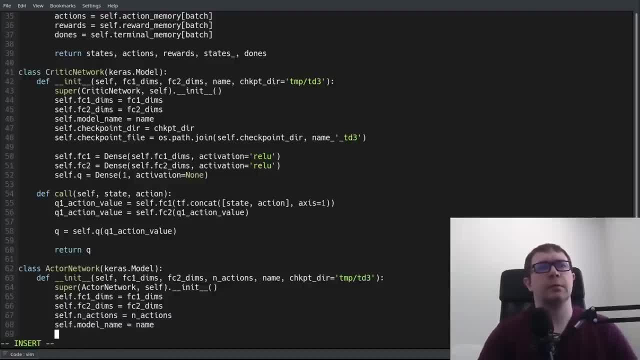 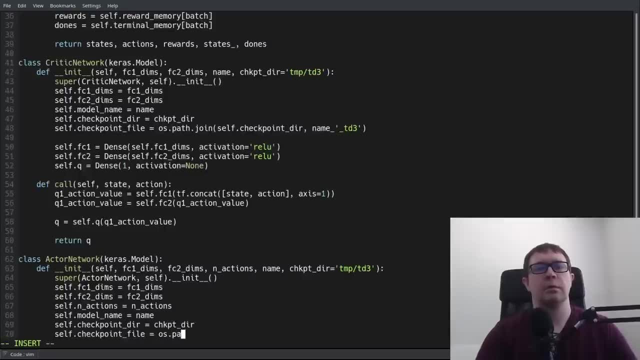 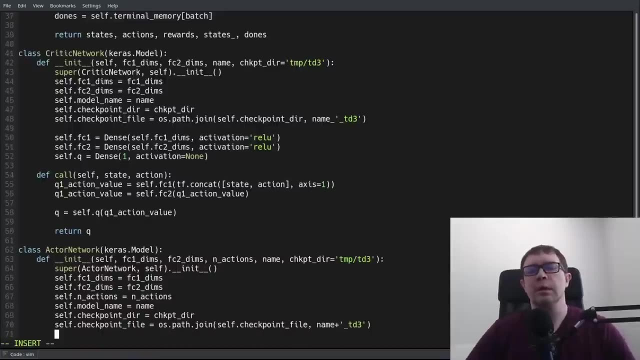 Model name: Checkpoint directory Plus td3.. And just for clarity, that name will have stuff like target actor, target critic actor or critic, So we can keep all of those particular networks straight. And of course the two critics will be critic one or critic two. 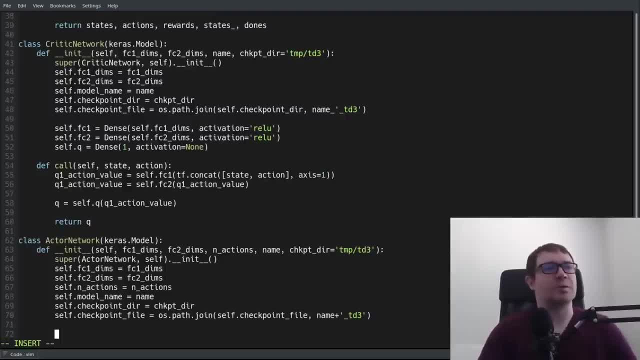 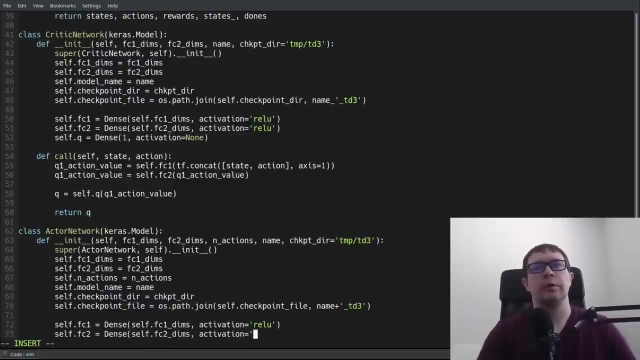 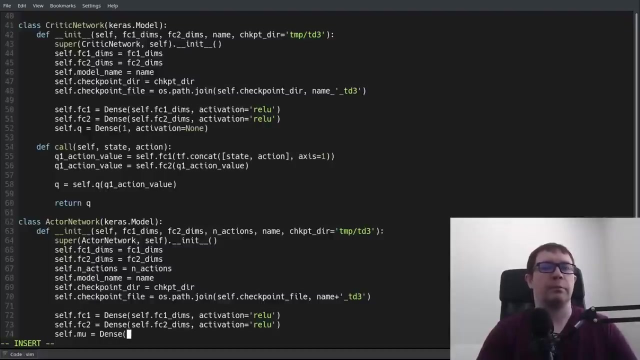 because we have very interesting naming conventions. So now we'll have our deep neural network, Again a simple dense layer With ReLU activations for the first two layers And then mu for our output, And that will take an actions as our output dimensionality. 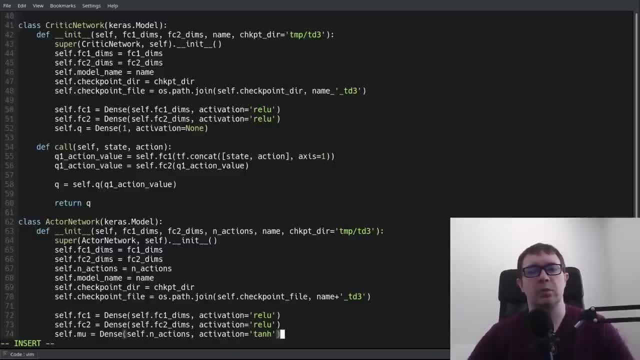 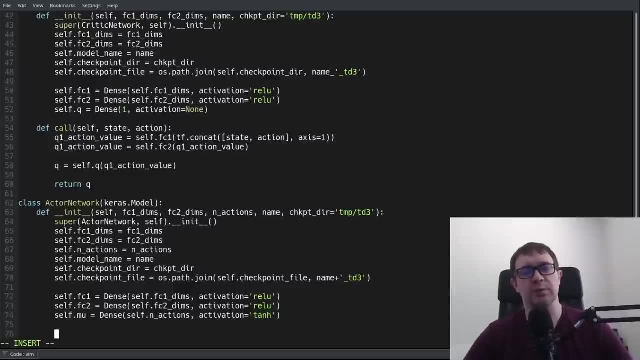 with a tan hyperbolic activation. The tan hyperbolic is bound between minus one and plus one. If you want to take into account boundaries of actions that are beyond plus or minus one, you can multiply this output by the maximum bounds for your environment. 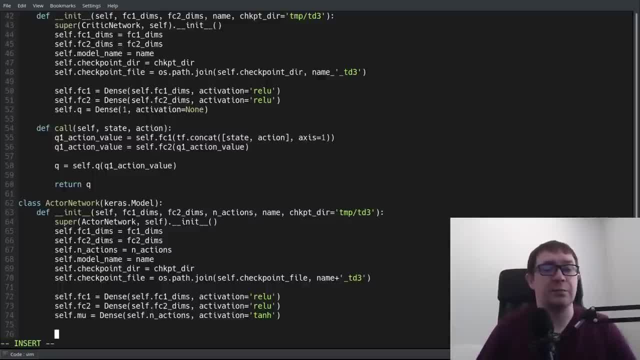 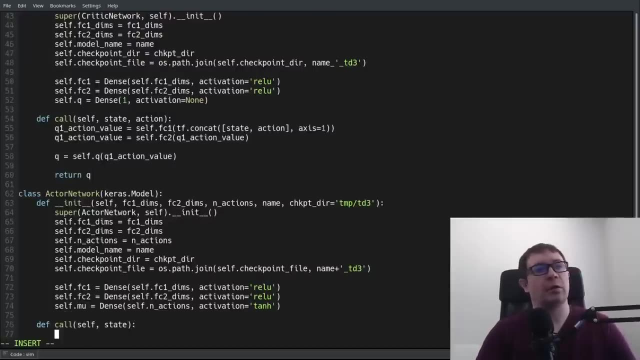 So some environments will have a max action of plus or minus two, which, of course, plus or minus one is oftentimes less than you know two. So you have to take that into account, depending on the environment. So again, we need a call function to handle the feed forward. 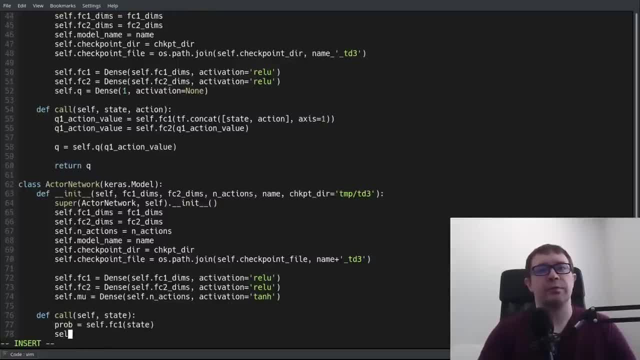 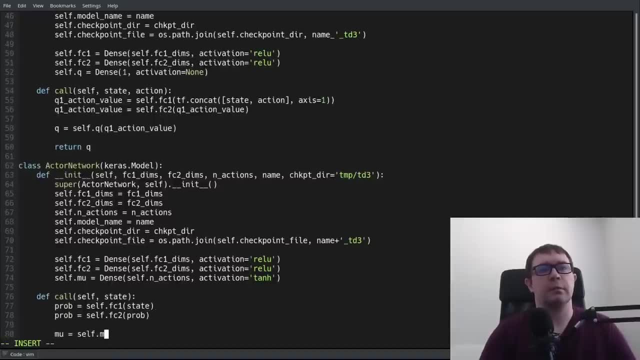 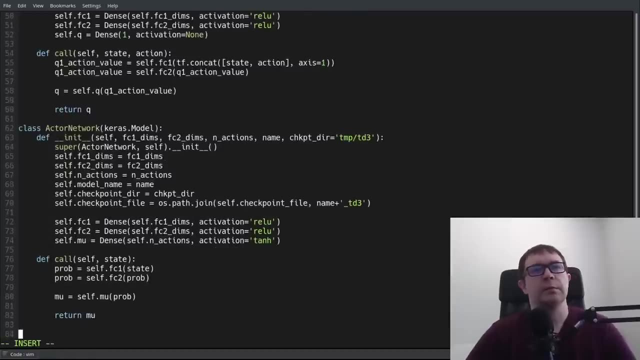 So pass our state through the first fully connected layer, second fully connected layer and pass that through the final layer and return it. So that is it for our actor network. Next we need an agent class to tie everything together and to handle all of the really interesting functionality. 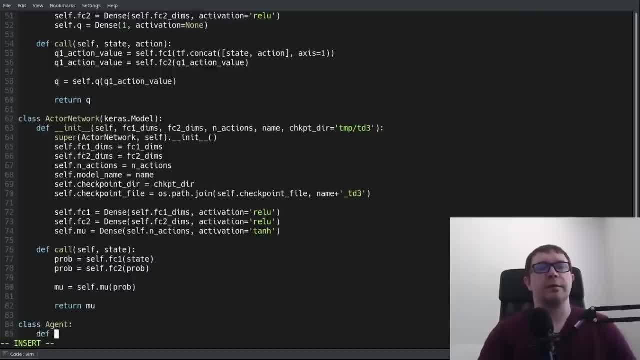 So our agent doesn't derive from anything, But our super constructor- excuse me, our constructor is going to take a whole slew of inputs, So we need a couple different learning rates. Reason being: you want to accommodate the capacity for different learning rates for your actor and critic networks. 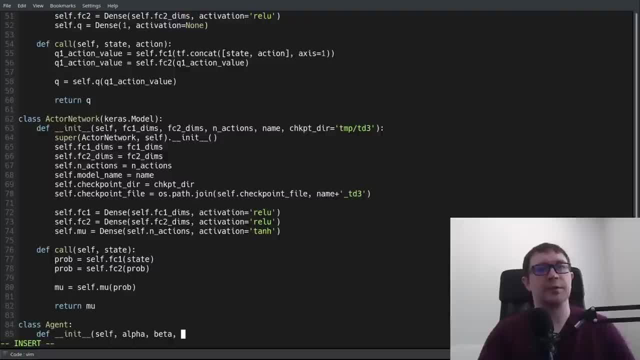 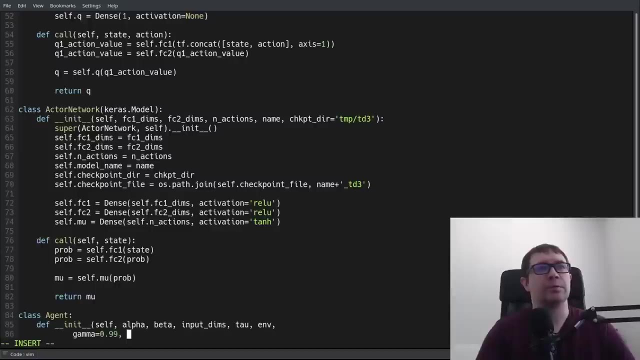 Sometimes they learn best with different learning rates. Input dims. you'll need that for your memory. Tau for your soft update rule. Your environment: for a number of important variables from the environment, Default gamma is 0.99.. The update actor interval will default it to every other iteration. 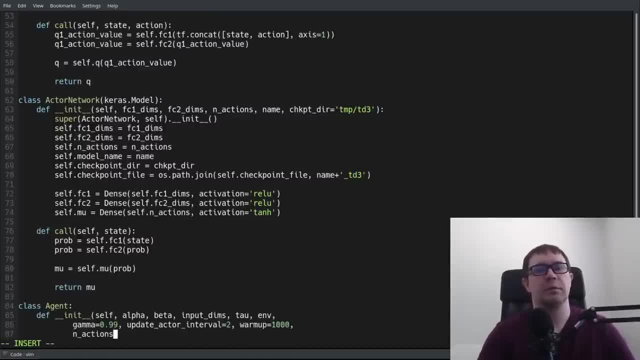 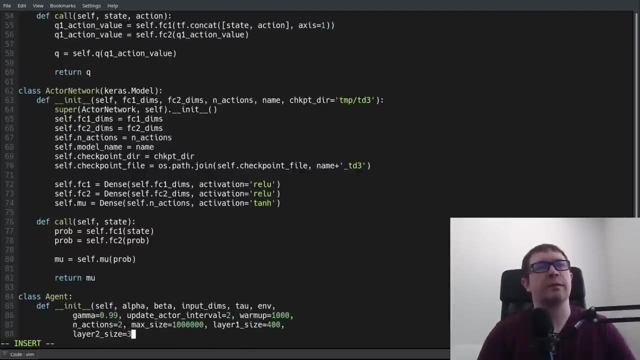 A warm up of a thousand steps. Just a default value for inactions: Max size of a million transitions. Layer one size: 400.. Layer two size, that's our FC1 and 2 dims respectively. A batch size default of 300. 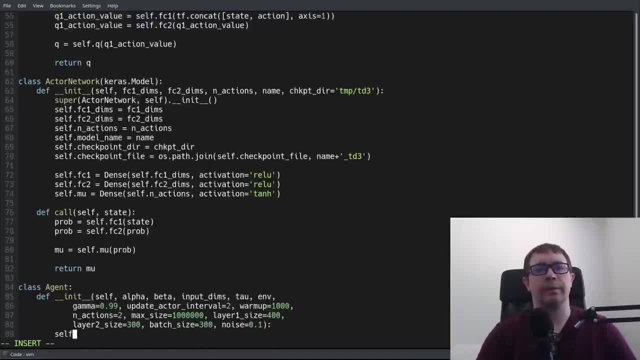 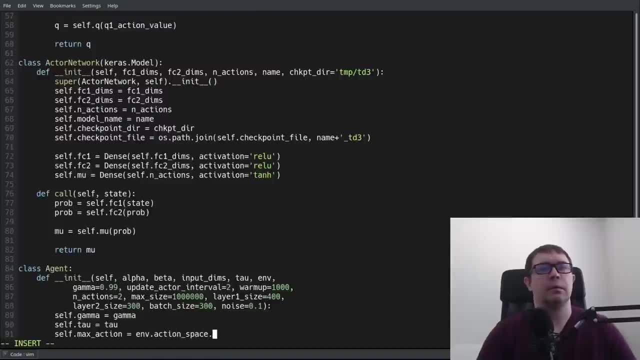 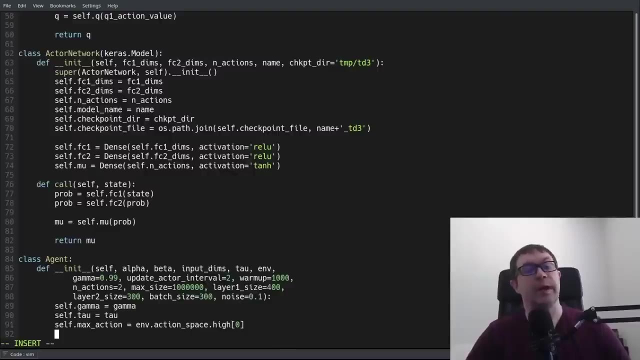 And a noise of 0.1.. Let's go ahead and start saving stuff. Since we will be adding in noise, we're going to have to perform a clamping on our actions to make sure that the actions, the action plus the noise, don't fall outside the allowable bounds. 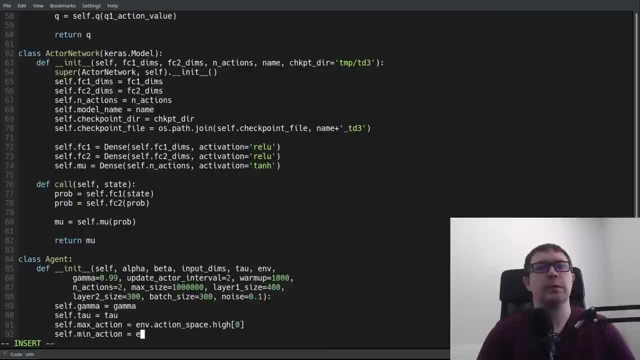 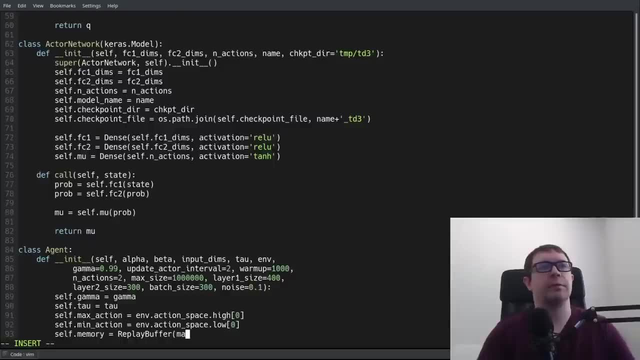 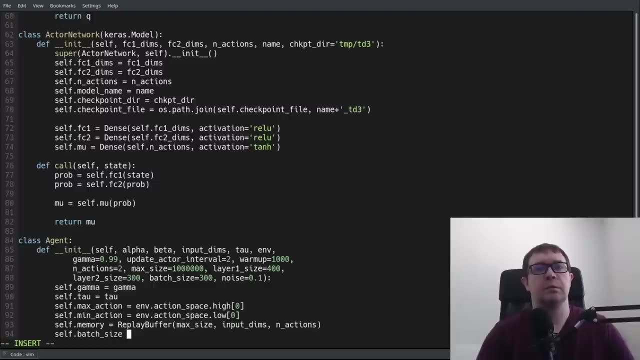 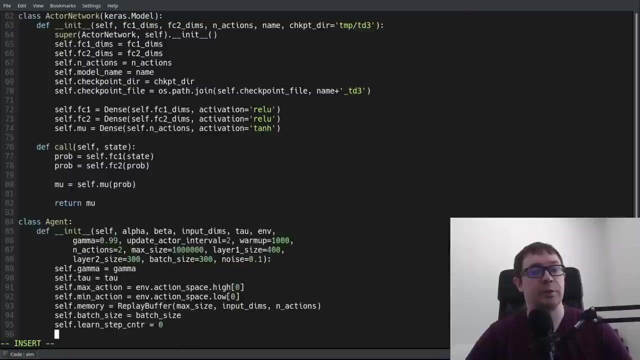 of the environment or below. We'll need our memory. That's a replay buffer. Then we need batch size. We'll need a learn step counter. We'll need that because we're doing the delayed part of TD3.. We're going to delay the updates of the actor network. 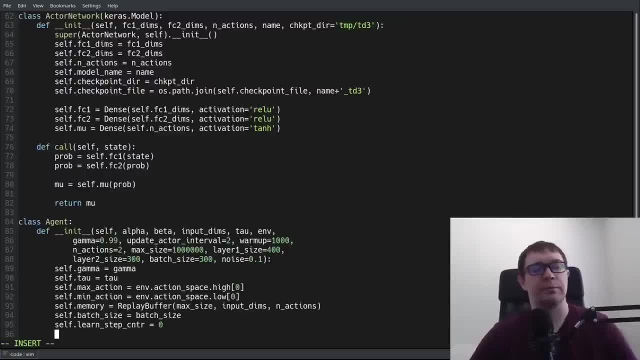 to every two different iterations of the update of the critic network to give the critic network time to converge. Then we have- you know, I'm looking at my cheat sheet here- Oh, a time step. Why do I have a time step? 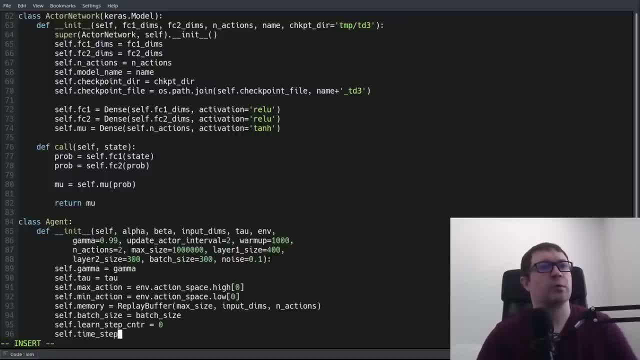 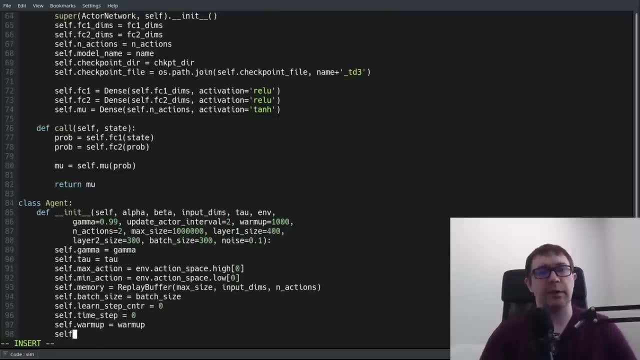 Excuse me one moment. No, I believe the time step is for the warm up procedure. We shall double check that later. If not, I'll come back and delete it in the GitHub, And we don't want to forget. number of actions. 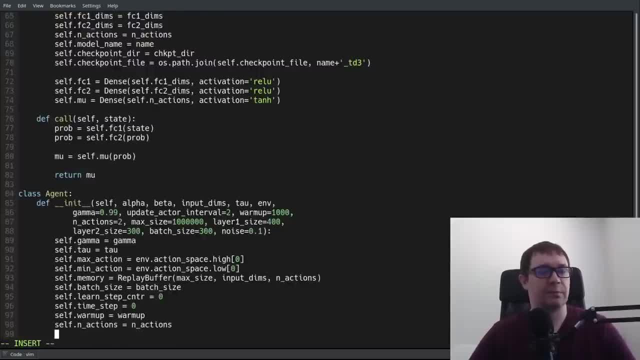 Sorry, I write this code, you know, sometimes well in advance of doing the video, because I get distracted by other stuff And so when I come back to it I don't always know what I was thinking. That is the benefit of comments. 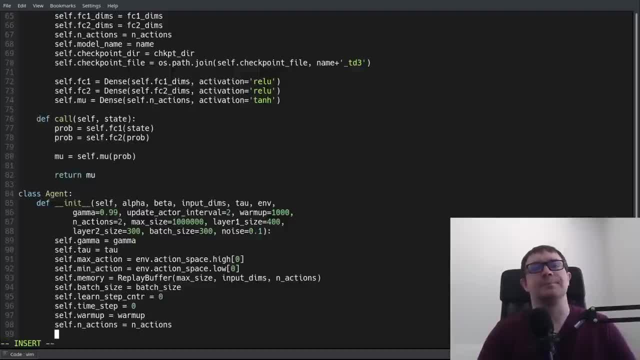 which I don't really do for this stuff. Sue me, I probably should. We do need our update actor iteration, And that is update actor interval. Excuse me, let me close my door. My toddler is rampaging And next we can go ahead and start defining our actors and critics. 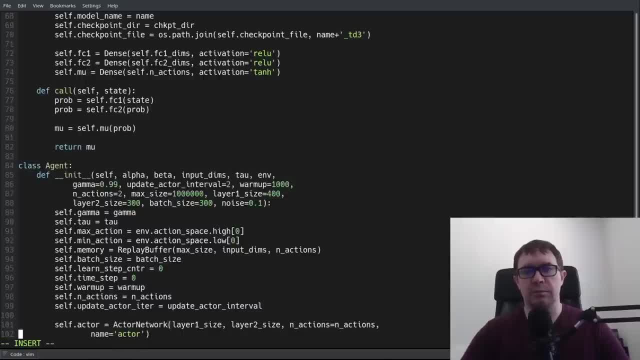 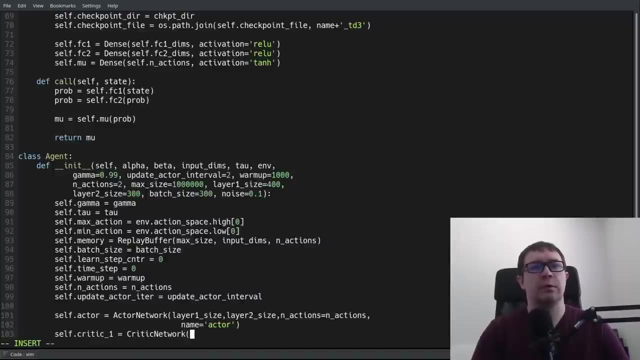 And so the name will just be actor, because we are quite creative. To maintain compliance with the pet bait style guide, Let's go ahead and delete a couple spaces. Critic one is a critic network, Your one size layer to size, And we don't need 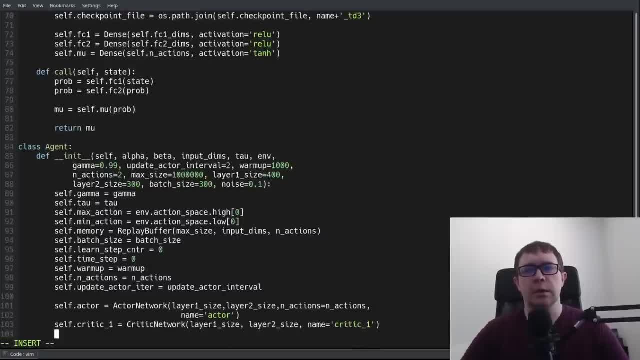 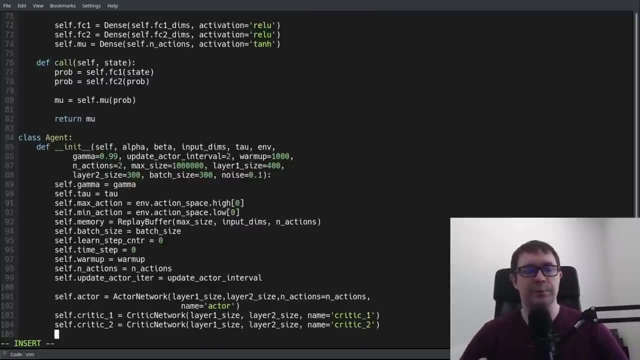 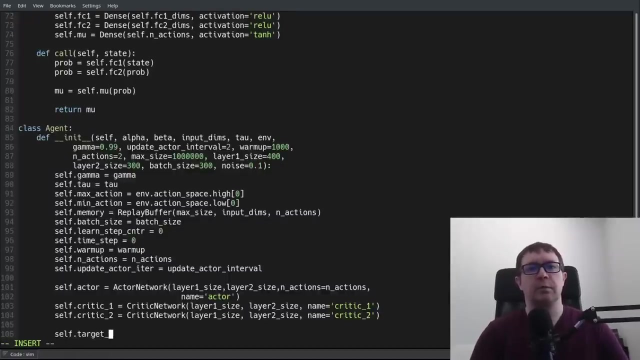 number of actions there because I deleted it, So its name will be critic one, Likewise for critic two. And again, the purpose of this is to handle the double Q learning update rule. Next we will need a target actor, Layer two size. 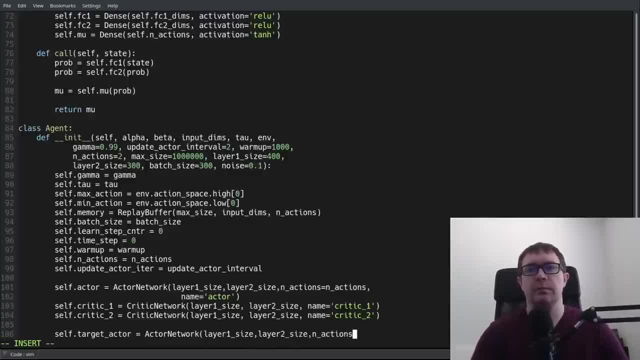 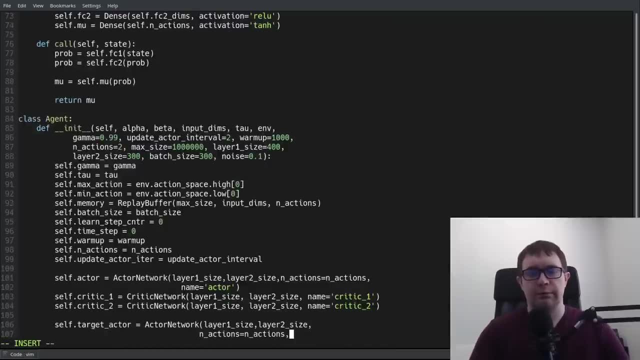 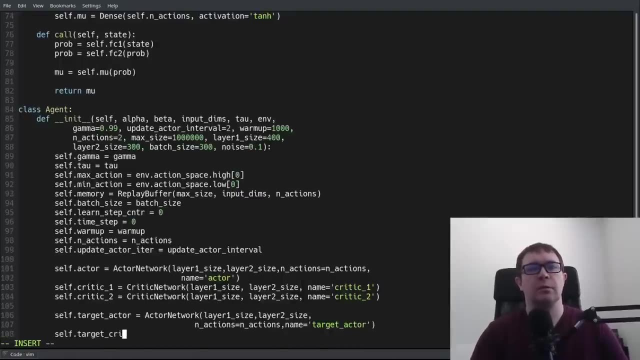 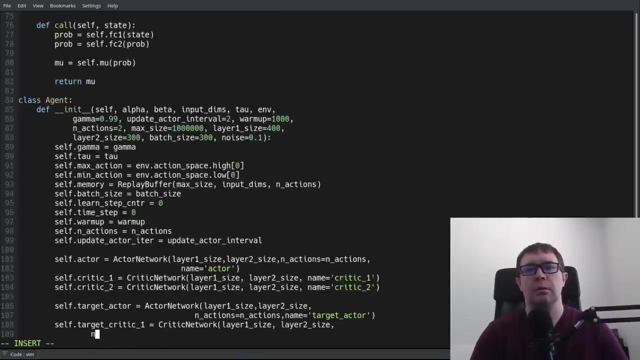 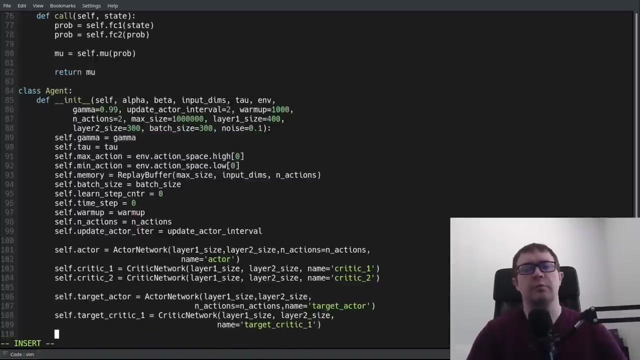 Let me go ahead and delete spaces. Oh, you know what Silly style guides. And finally a name of target actor. Then we will need target critic, one With a very original name of target critic, one Similarly critic net target critic two. 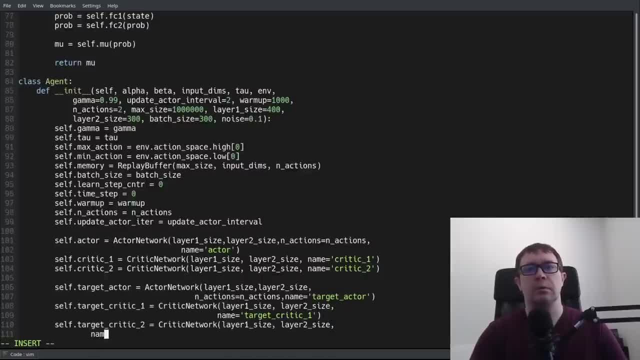 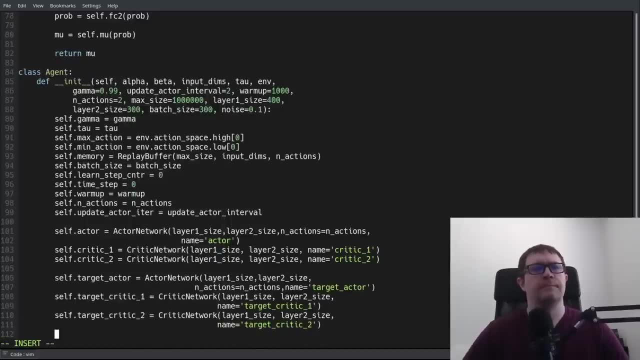 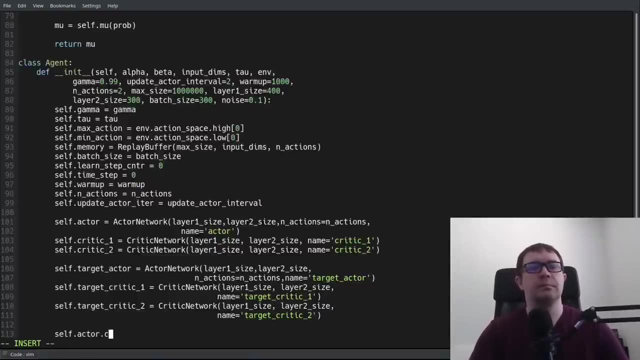 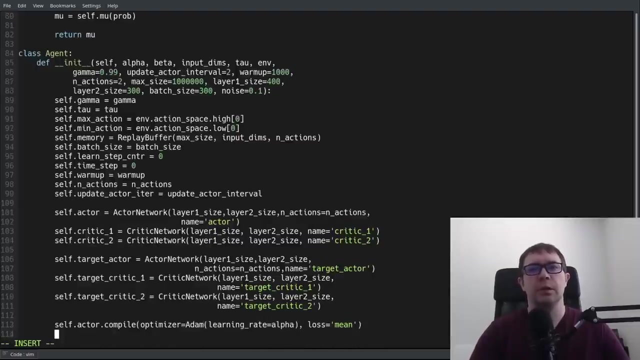 And that is it for our networks. Next we have to compile them, because this is a tensorflow two, And that is where our learning rates come into play. So we will use our atom optimizer with a learning rate defined by alpha for our critic. Our loss would just be a mean. 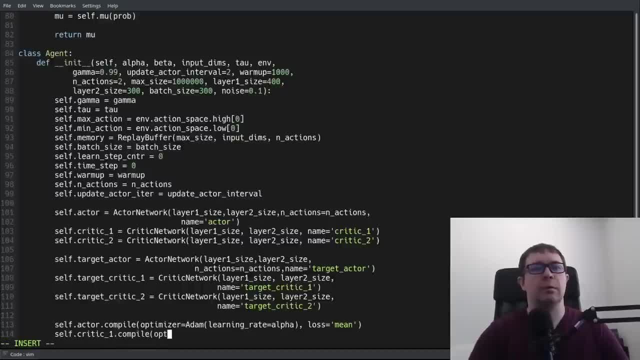 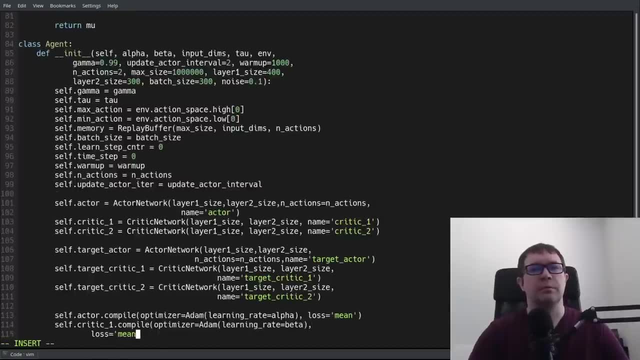 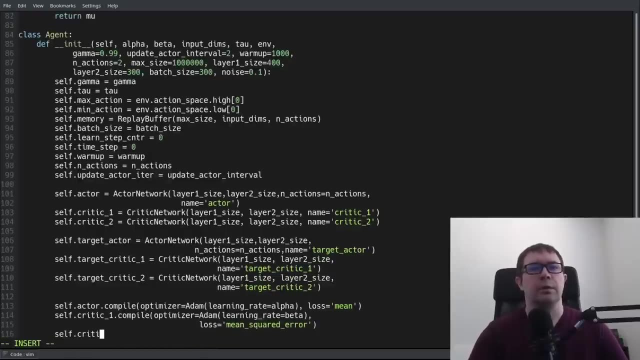 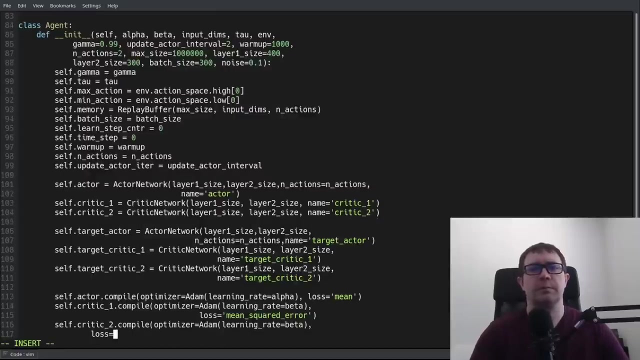 And our critic one: Learning rate of beta, A loss of mean squared error. And critic two Have to do the same thing. Do I need- Yes, I do, I do need parentheses there- Mean squared error, And then we will handle our target networks nest. 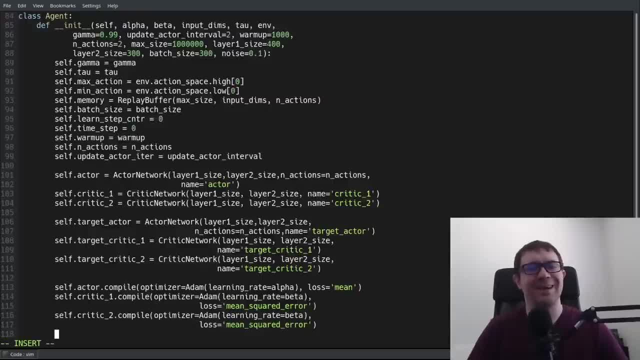 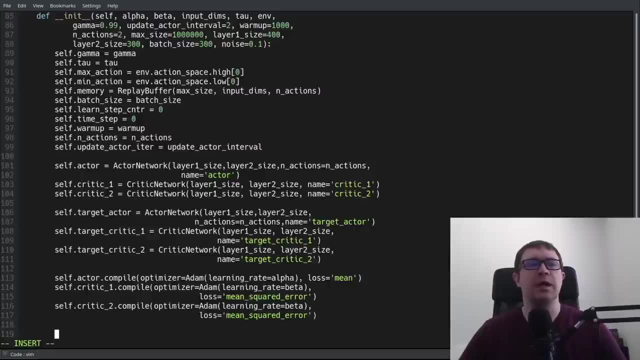 Target networks, nest Next. That is a tongue twister, So we have to compile the target networks just by convention with tensorflow two. We're not going to be performing any stochastic gradient descent or atom in this case- On those particular networks. we're going to be doing the soft network updates. 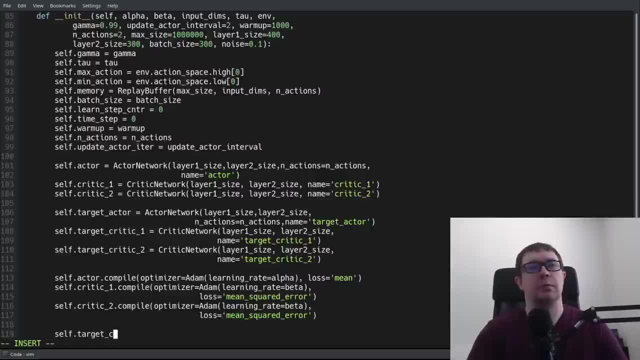 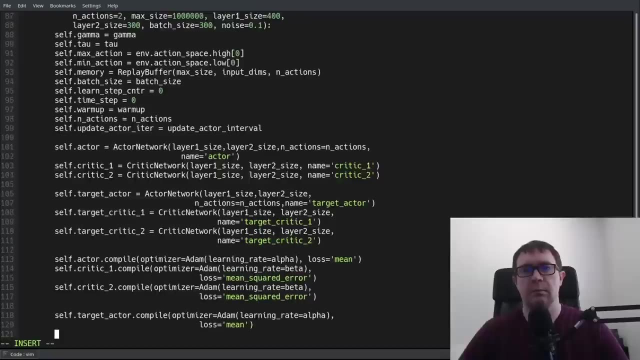 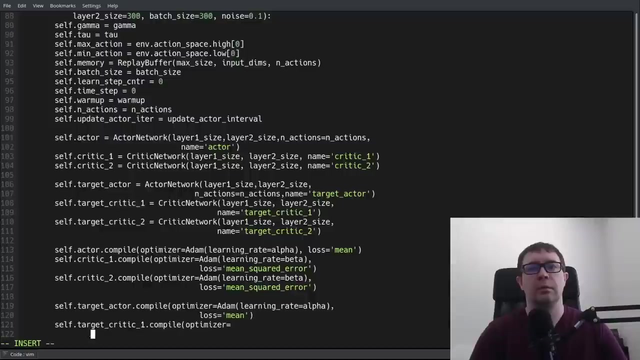 But we still have to compile them nevertheless. That is just by convention. Learning. rate of alpha Loss equals mean Target critic one, Because we need to. That is just a neither information one. We're going to need two culprits. for the first to stop the reading unt begin. 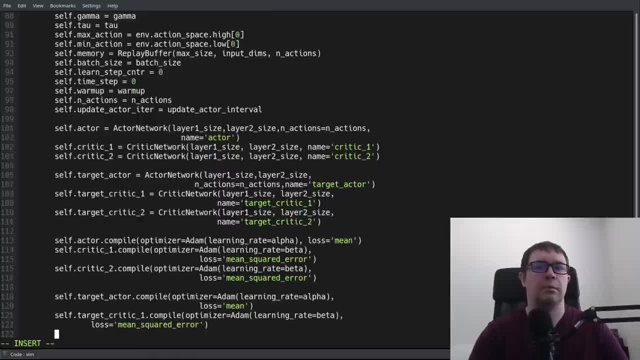 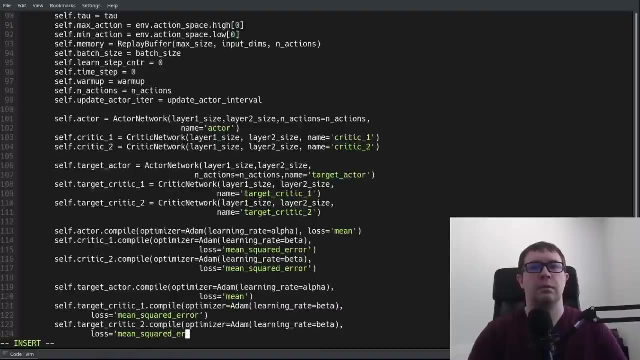 ожу. It saysken Will copy after when: Dios pathetic and fewer until Here it comes. Now out here We have A smallizi of f. Ok, I should be able to. All right, OK, Now would be great. 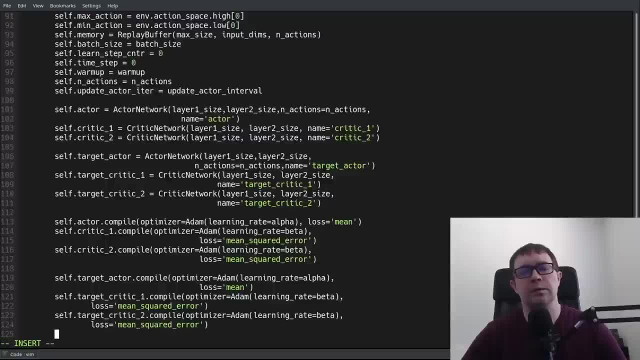 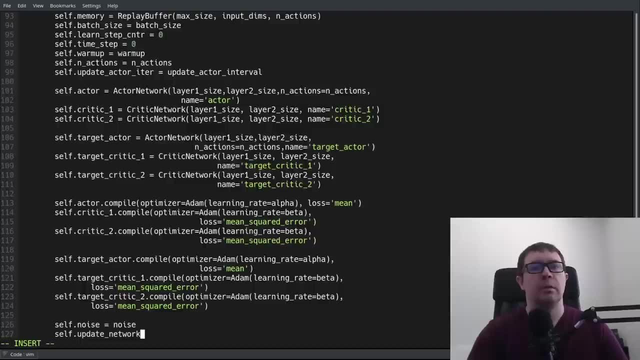 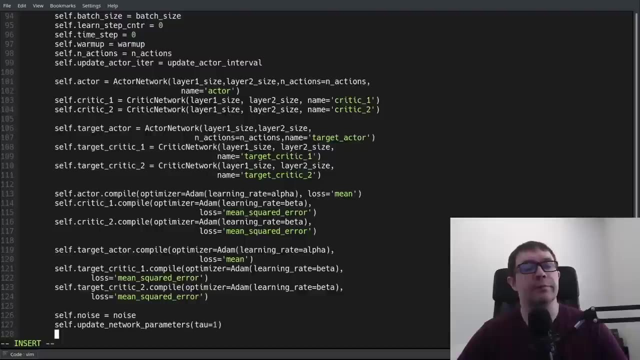 All, whether naked, color Or of f. Okay, so that is all of our networks. Selfnoise we'll keep track of as well. Update network parameters with the default value of tau equals one. I do that because on the first step of the update, 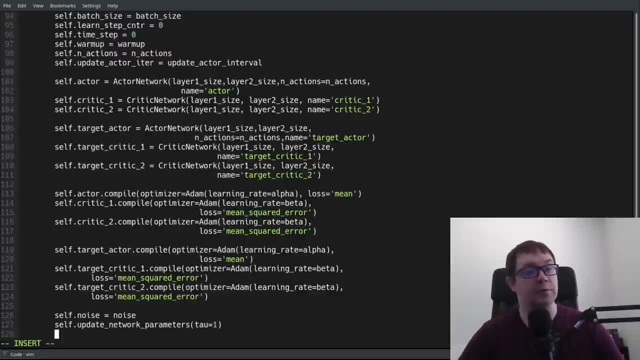 we have to set the values of our target networks equal to the starting values of the online networks, And so we pass in a value of tau equals one to perform an exact update or a hard update instead of a soft update. We'll handle that function toward the end. 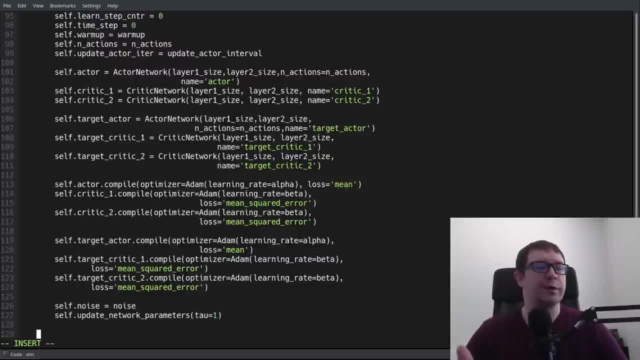 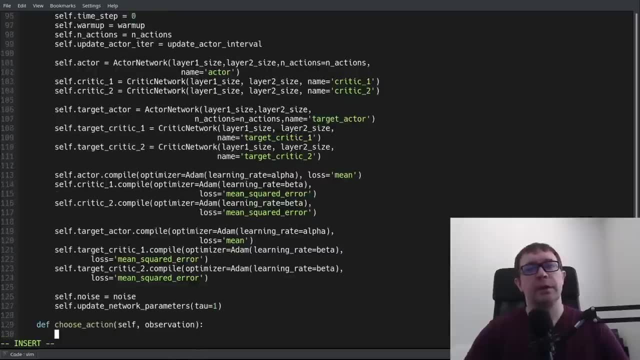 For now, I want to get to the choose action: remember and learn functionality, because that's where all the really interesting stuff is. So let's go ahead and choose an action based upon an observation of the current state of the environment as input. 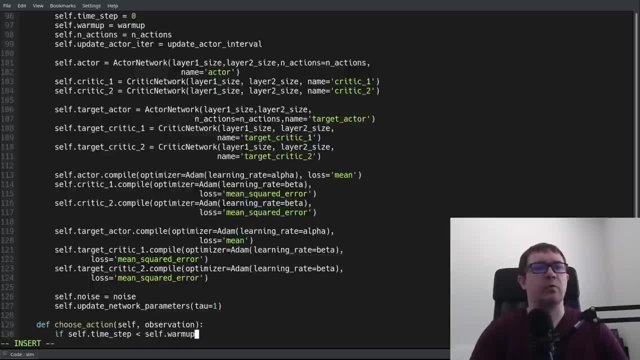 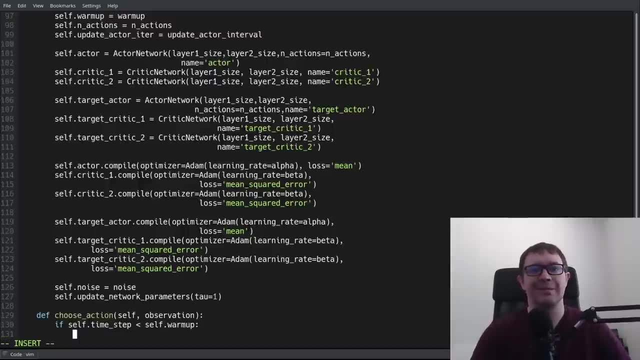 So if our time step is less than our warm-up period, yeah, that's why we need the time step to handle the current state of the environment, The warm-up, as I suspected. glad I didn't delete that We're going to select an action at random. 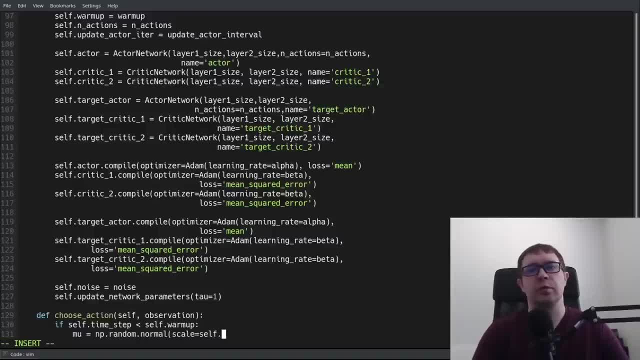 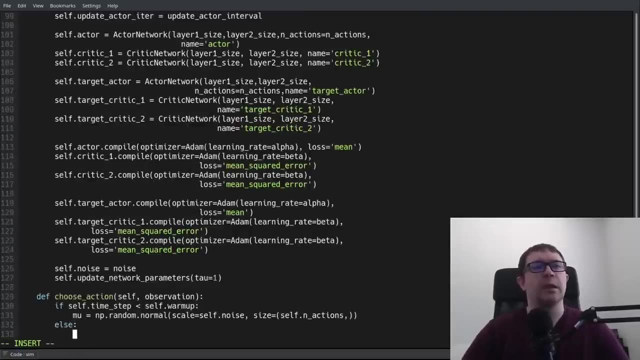 with just a normal distribution with a scale defined by our noise parameter in the shape of number of actions comma. so we get a batch there, Sorry, an array of scalars. Otherwise we want to go ahead and convert our state to a tensor. 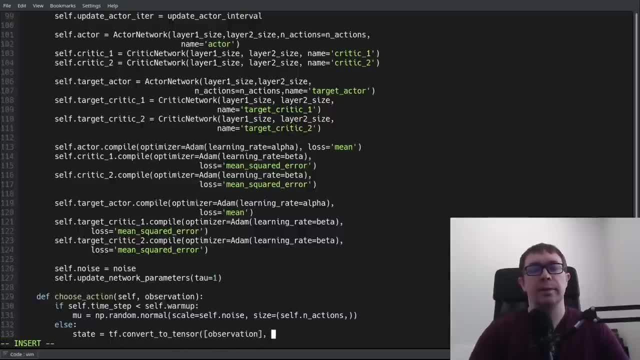 And add on a batch dimension. That's just the way that the inputs are expected to be fed into the deep neural network. We have to add that batch dimensionality And I have tf float 32 here. It must be due to some sort of precision thing. 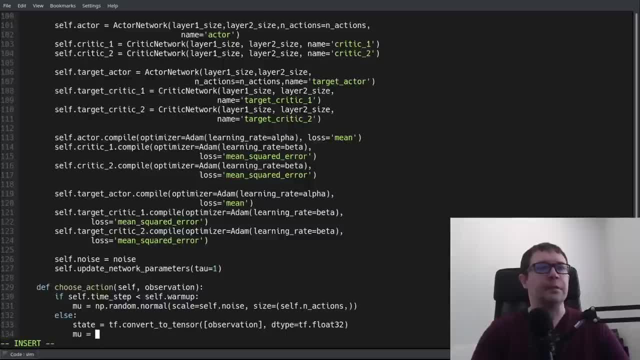 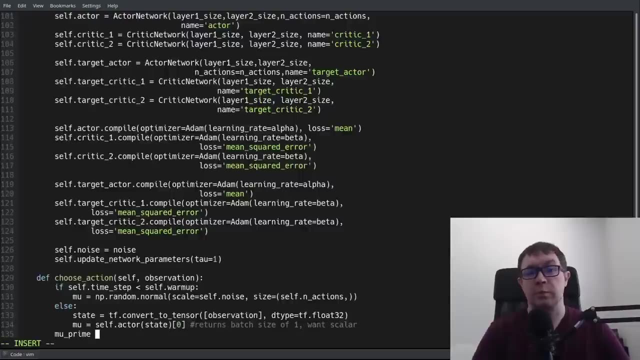 that makes TensorFlow happy. So then we want to pass our state through our actor network and receive our mu, And we're doing that because it returns batch size of one want scaler. Then we'll say mu prime, which is where we handle the noise. 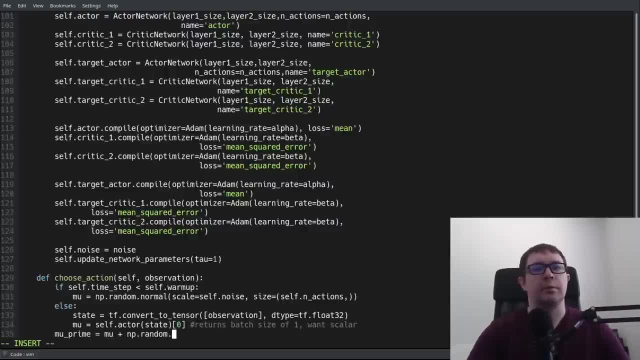 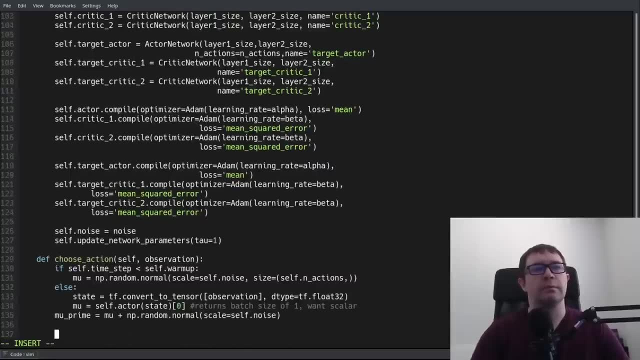 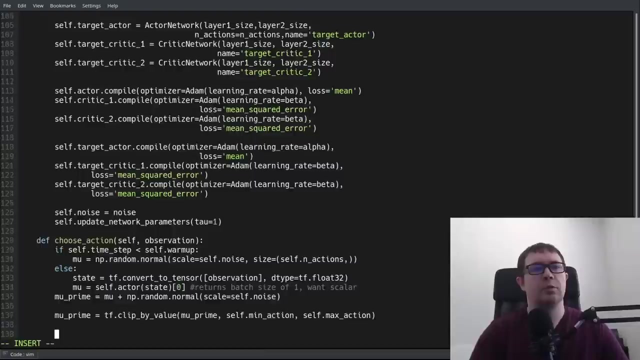 equals mu plus mp. random normal scale equals selfnoise And mu prime is tf clip by value because again that noise could take us outside the bounds of our environment. So we'll clamp mu prime between min action and max And we'll say: remember state action, increase our time step by one. 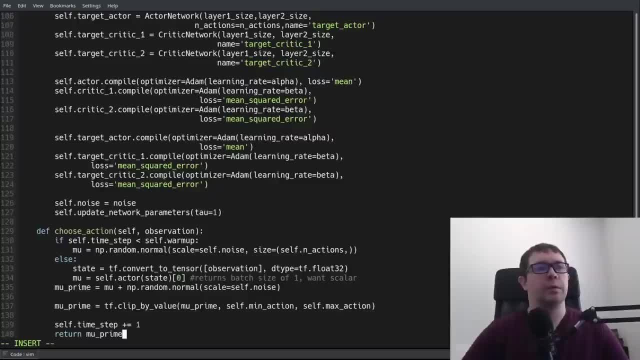 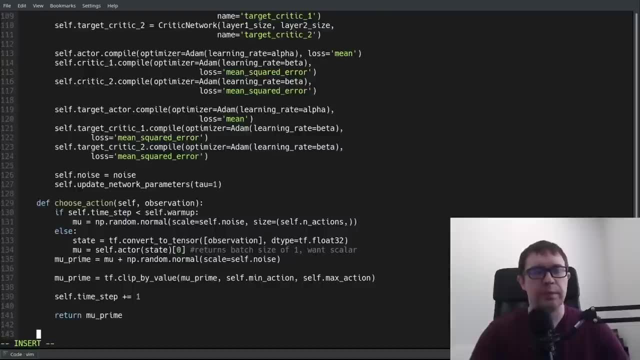 very important And we want to return mu prime. OK, That's it for our choose action. Now let's handle the simple interface function to remember a transition. So remember state action, reward new, state done and we'll say memorystore. 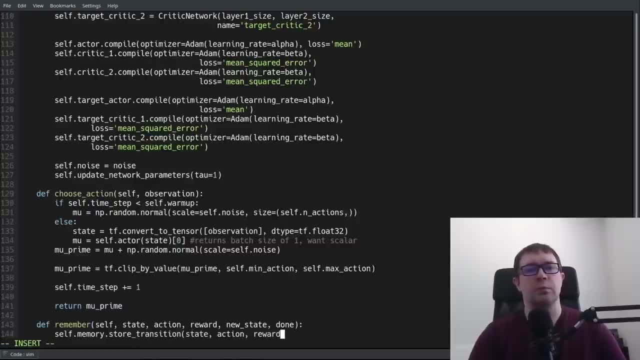 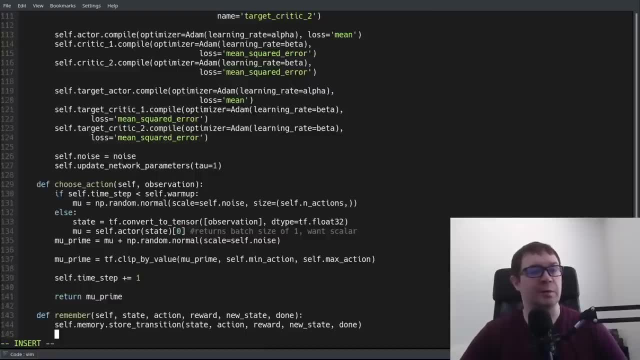 Transition Memorystoretransition state action reward, new state done. and that's just because we have to interface with the memory in some way. you don't want to have the agent class calling. you don't want to have the agent class interacting with private variables from your memory. that would be poor software design. so 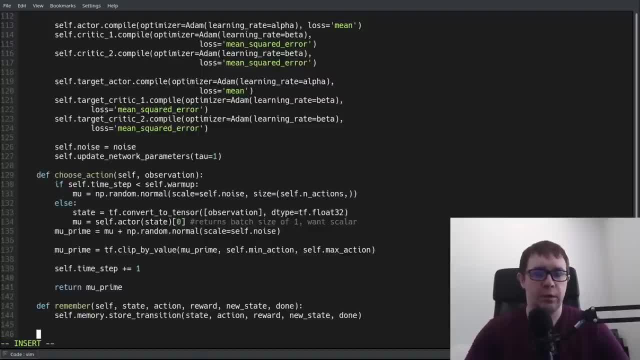 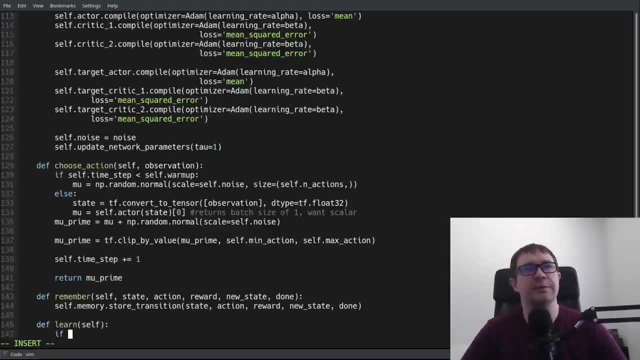 next we handle the most interesting function in the whole program, which is the learn function, and the very first thing we want to do is say, hey, if we haven't filled up at least batch size of memory, we probably don't want to be learning, so we'll say selfmemorymemcounter. 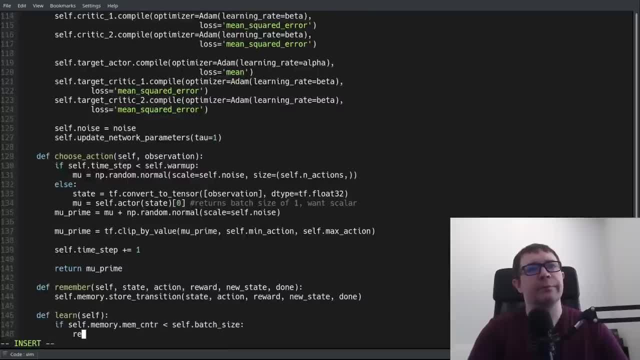 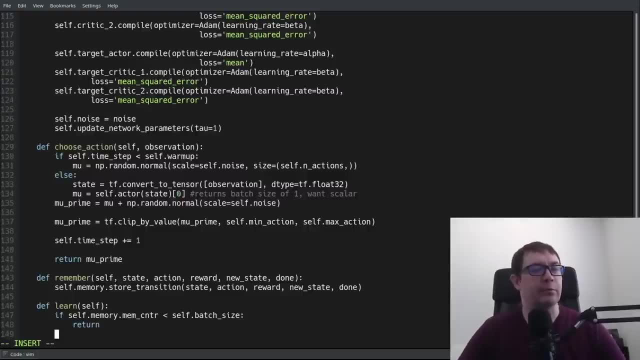 plus and batch size. now, if it's not, if it's not greater than the batch size or equal, to go ahead and return. now, since we're doing a warm-up, that won't be the case, because the batch size is just a few hundred, the warm-up is a thousand. so by the time we get through the warm-up, 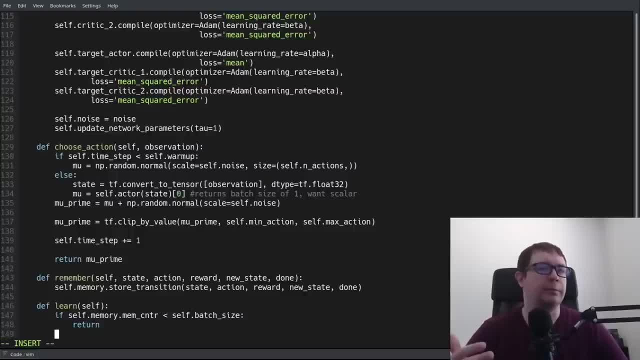 we're going to be able to say, hey, if we haven't filled up at least batch size of memory, we probably. then we're already well into filling up the batch size of memories. But if you decided not to do a warm-up, then that would be important. 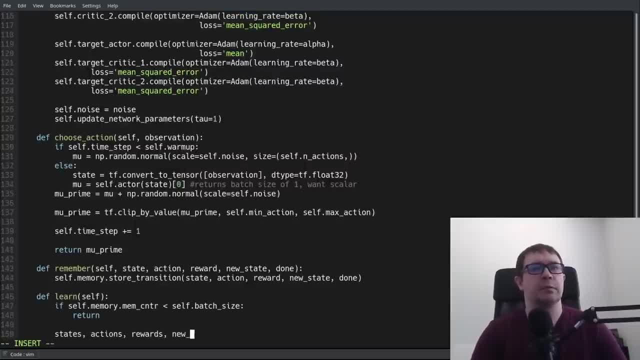 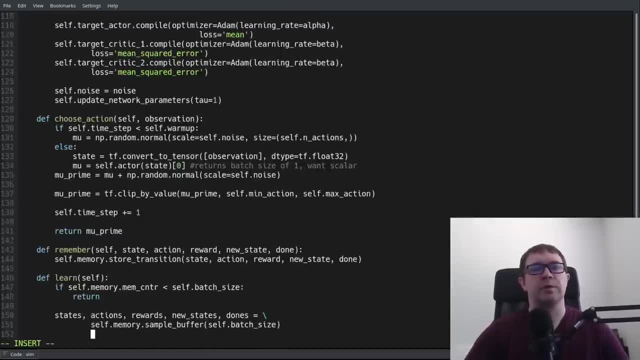 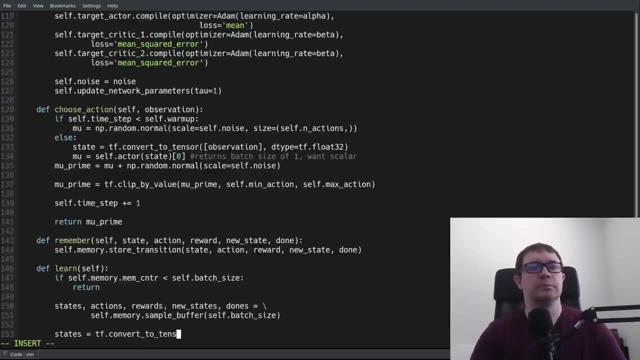 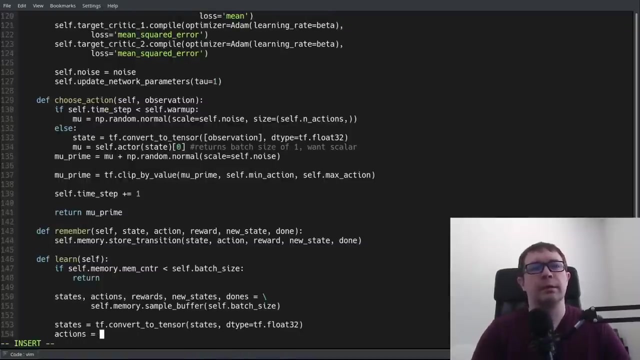 So we'll start by sampling our memory Self-memory sample buffer, Pass in our batch size And then we want to convert all of those to TensorFlow tensors- And I have to be very pedantic with data types here. I think there could be issues if you do not. 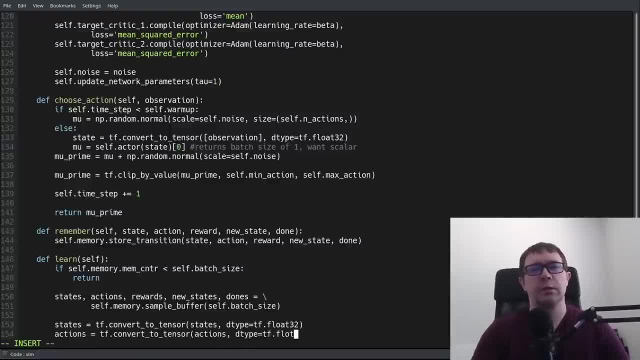 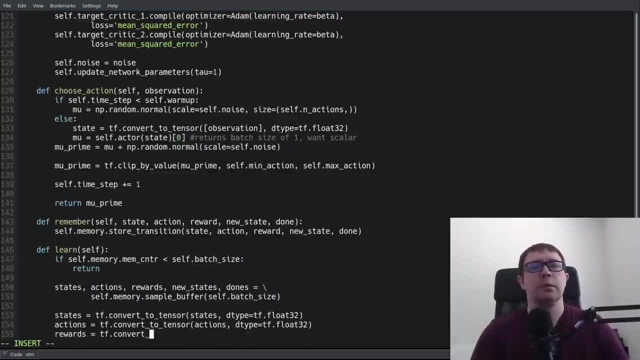 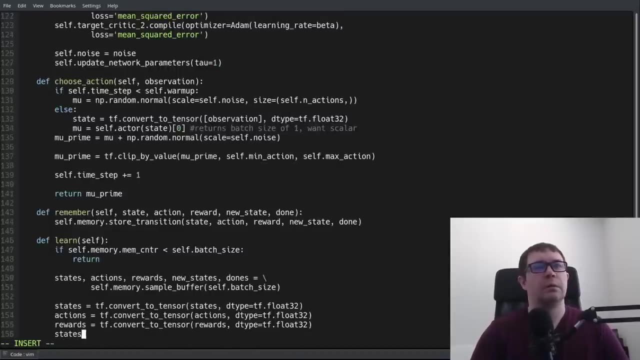 As I recall- I think it barks at you about data types because it expects certain types of floating point variables in some places and other types elsewhere, And we don't have to convert the duns to a tensor because we're not sticking that in a deep neural network. 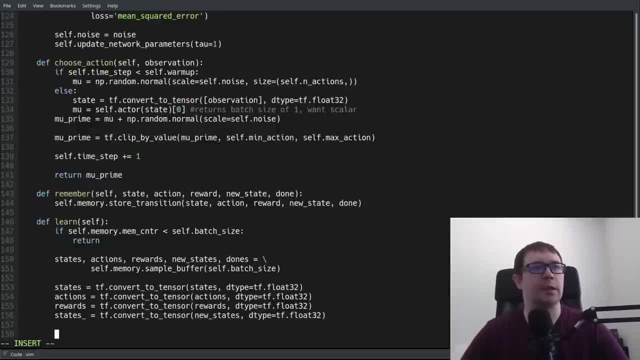 We're just using that as a multiplicative factor, so we can leave it as a NumPy array. Now we're going to handle our update to the critic network, because we do that every time step, And then we'll handle the update to the critic network. 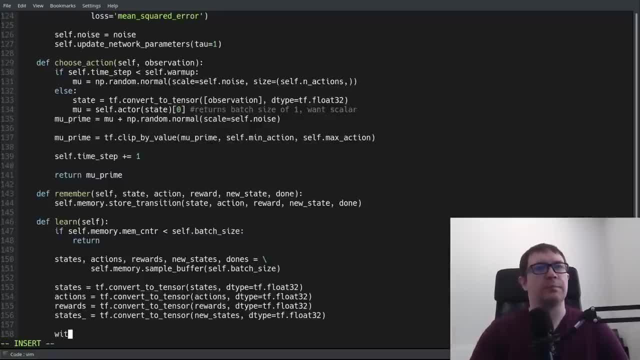 And then we'll handle the update to the critic network, And then we'll handle the update to our actor network. So we'll say the TF gradient tape. You know I have persistent equals, true? Oh, because I have two different networks. 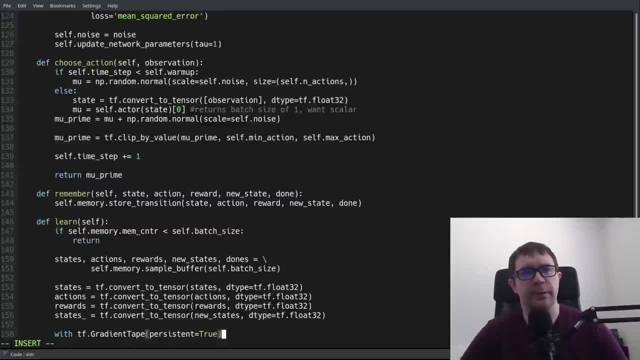 Yeah, so you need two different. If you're using two different updates for one group, excuse me. if you're using two different applied gradients for a single tape, then you need to pass in the persistent equals true variable parameter, excuse me, or argument. 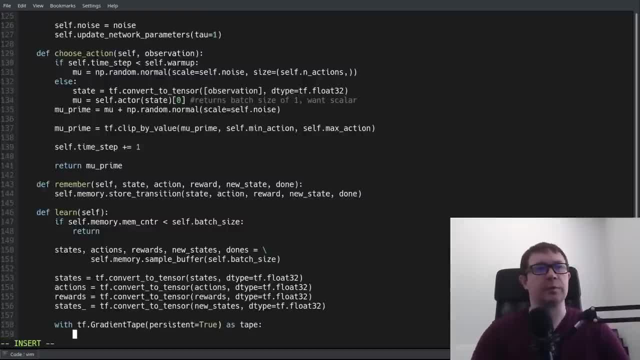 Otherwise you don't need that persistent equals true if you just have, say, a single network that you're performing an update on. So we want the actions according to our target actor for the new states, And then we're going to go ahead. 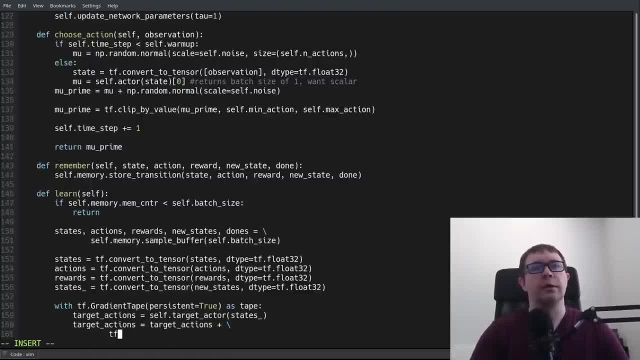 and add on a noise parameter to that that we're going to clip between the range of minus 0.5 and positive 0.5.. So clip by value: MP, random, normal 0.2 minus 0.5, 0.5.. 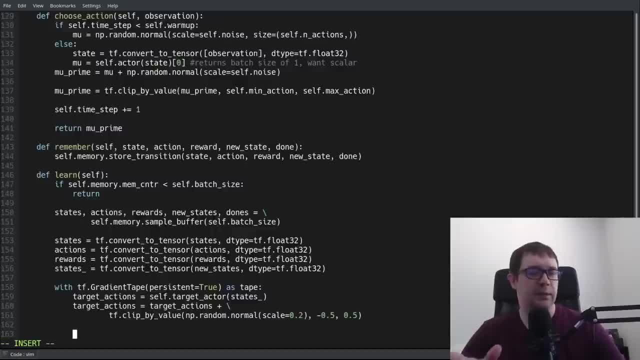 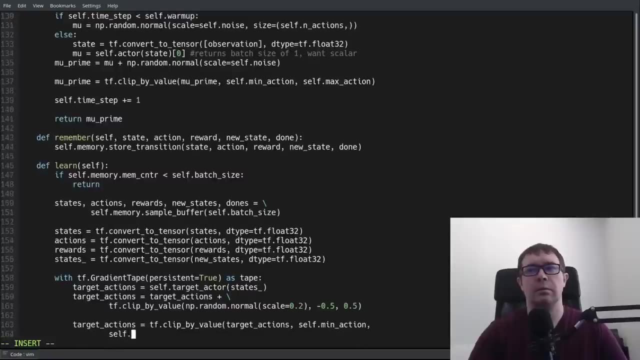 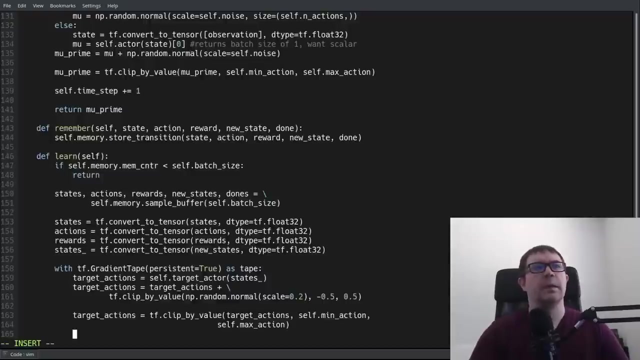 And then we're going to go ahead and clip that again, because again the addition of that noise could take the action outside of the bounds of our environment. And then we're free to go ahead and start calculating our critic values. So Q1 underscore the critic value. 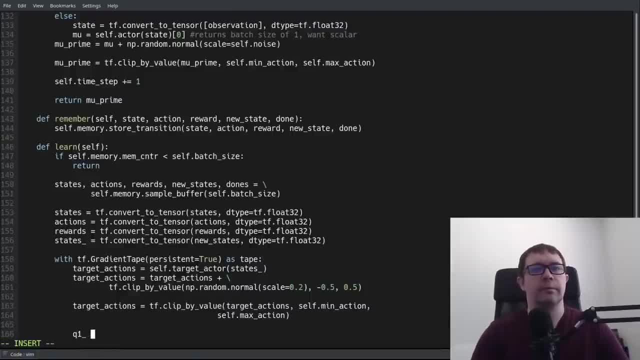 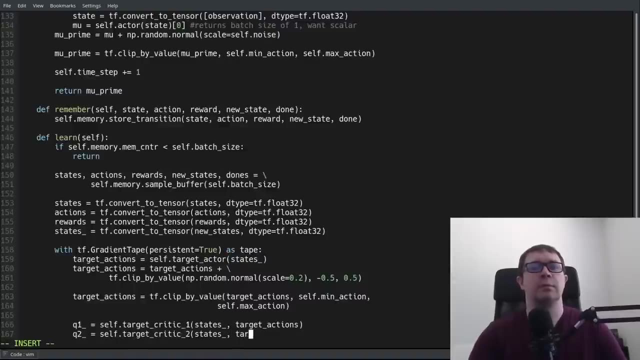 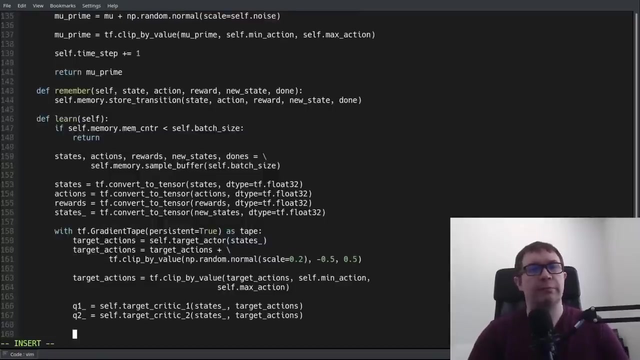 according to the first target critic, is the feedforward of the new states and target actions through the first target critic, Q2 underscore is very similar. It's just the evaluation of the new states and target actions. according to the second critic, Now again, we're going to have to go ahead. 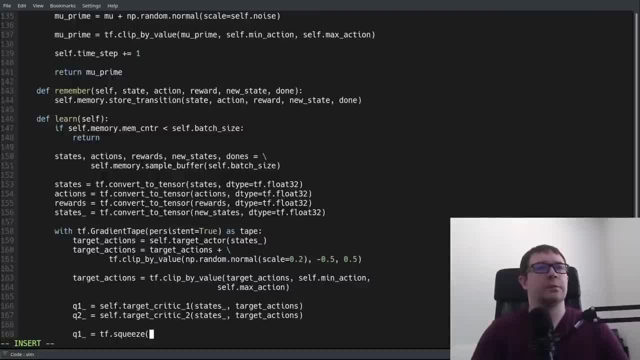 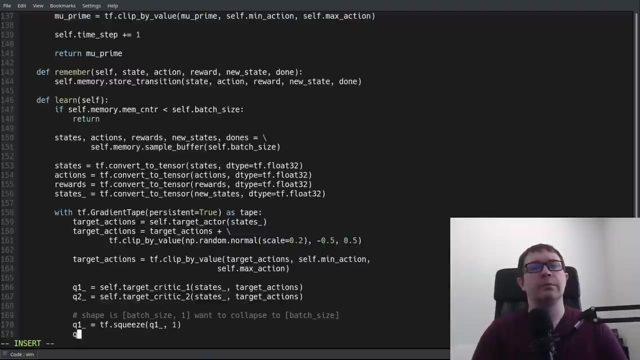 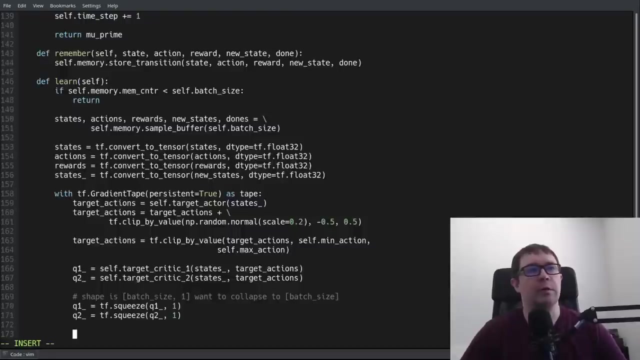 and squeeze that output, And the reason is that our shape is batch size by one Want to collapse to batch size, And we have to do that for Q2 as well. Excuse me, Excuse me, Excuse me, And then we're going to need the value of the states. 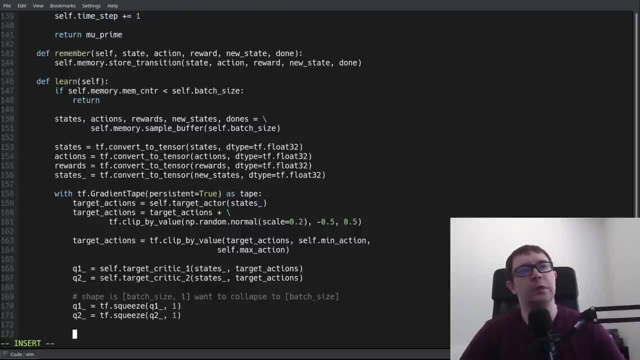 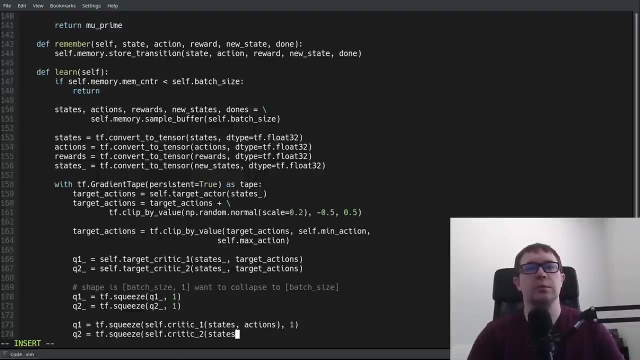 and actions the agent actually took, according to the regular critic one and two networks. So we'll call those Q1. And we'll just go ahead and squeeze those right away. Critic one: states actions squeezed along the first dimension. Critic two: states actions one. 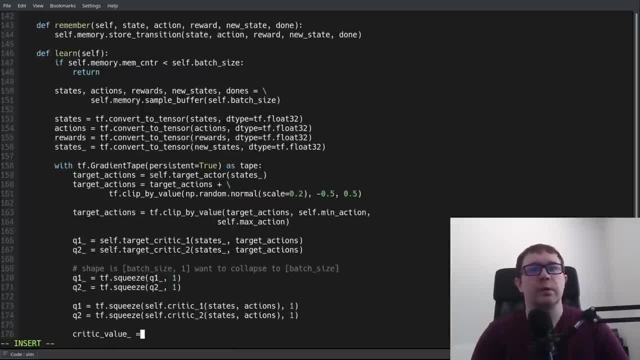 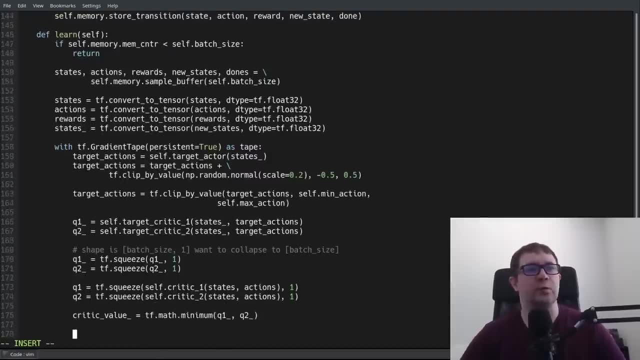 And then we're going to say that our critic value for the new states is the minimum of Q1 underscore, Q2 underscore, And then we're going to need our target value, the Y, from our paper rewards plus gamma times, critic value times one minus duns. 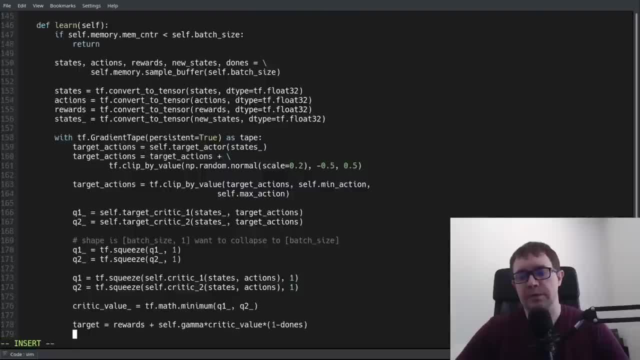 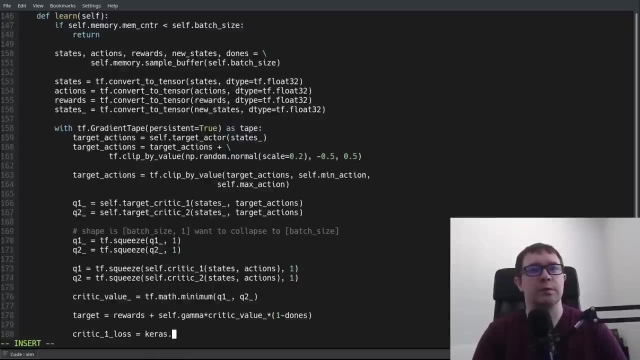 That will set the value Of the second term here. gamma times, critic value. There should be an underscore there. Sorry, to zero. everywhere The done flag is true. And then we have our losses. So critic one loss, Karis. losses dot mean squared error between the target and Q1.. 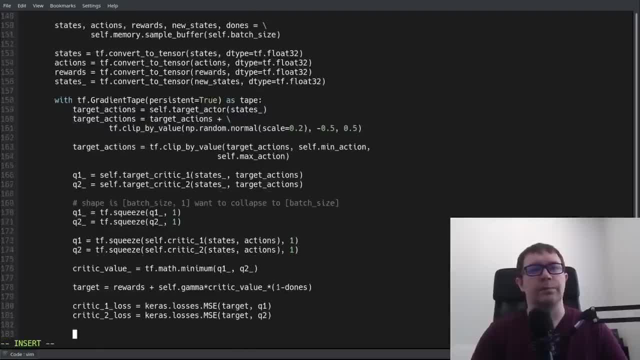 Mean, squared error, target and Q2.. So that is it for the calculation of the, the critic losses. Now we have to handle the calculation of the gradients. Now we don't have to do anything special for that, The tensorflow package handles that for us. 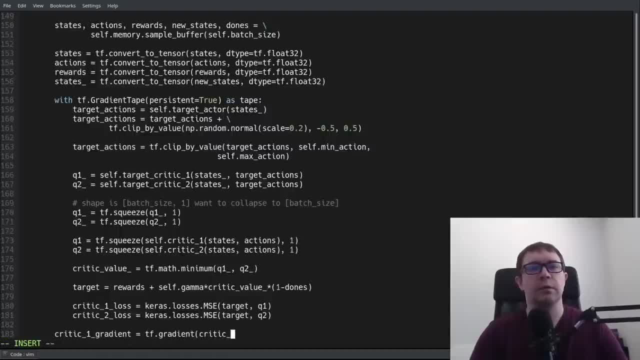 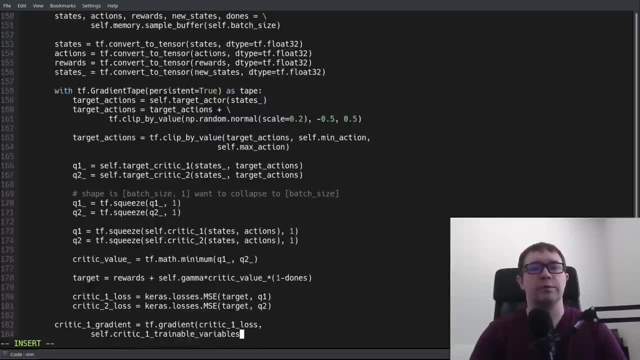 So tape dot gradient the gradient. critic one loss with respect to the critic one trainable variables. So that should be dot, not an underscore. I make that mistake frequently. Critic one critic, underscore one dot. trainable variables. Yeah, that is right. 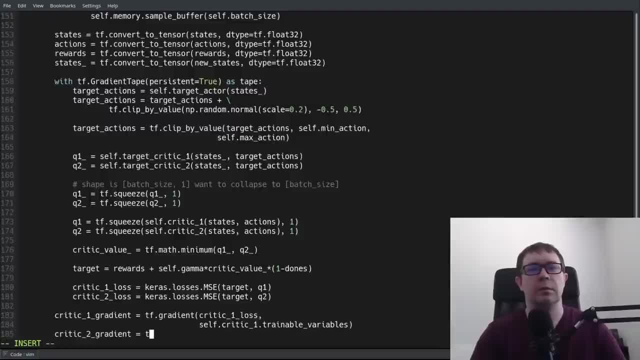 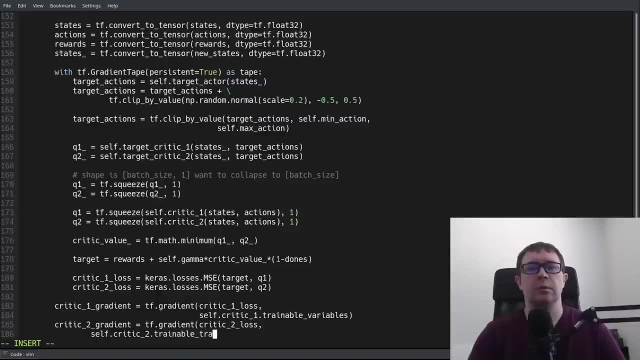 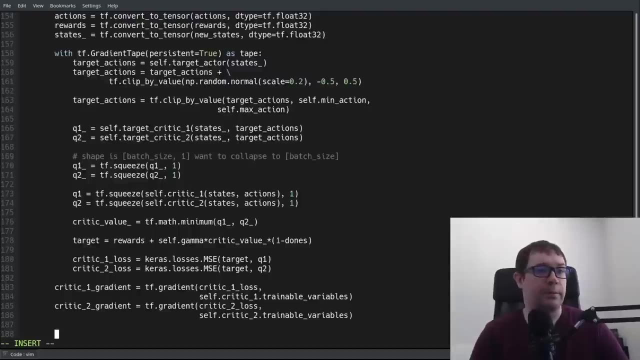 And then we need the critic: two gradient Critic, two loss cell dot critic, two trainable variables- Same deal. Then we need to go ahead and apply those gradients, So calling our optimizer dot apply gradients function And that expects a, a. 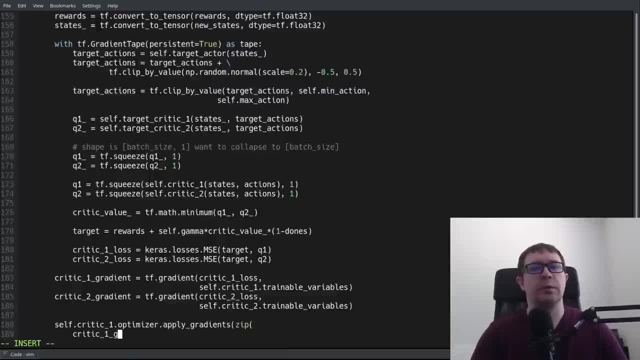 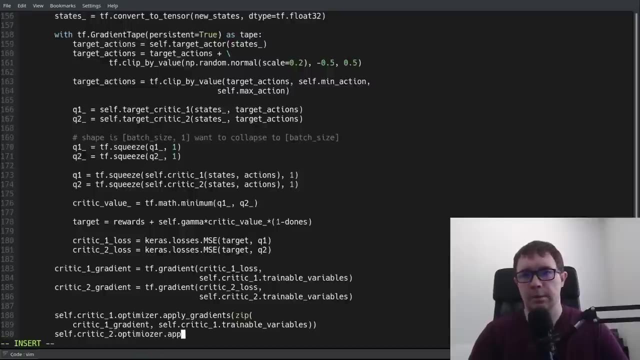 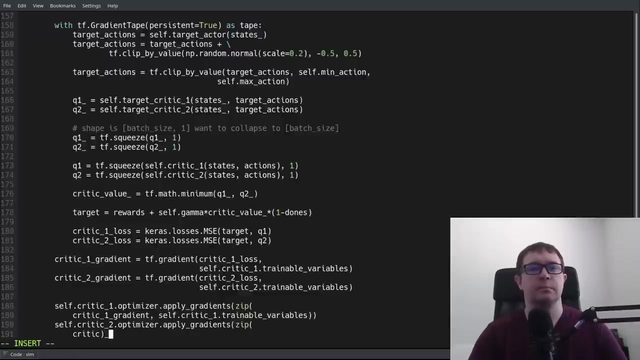 zip as input. We're going to zip the critic one gradient and the self-critic one- trainable variables: Same thing for critic two. Optimizer. Err To gradient, We're going to zip it. Okay. And then we want to increment our learn step counter because that gets. 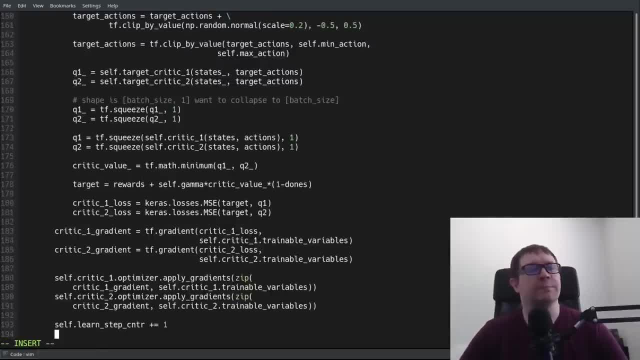 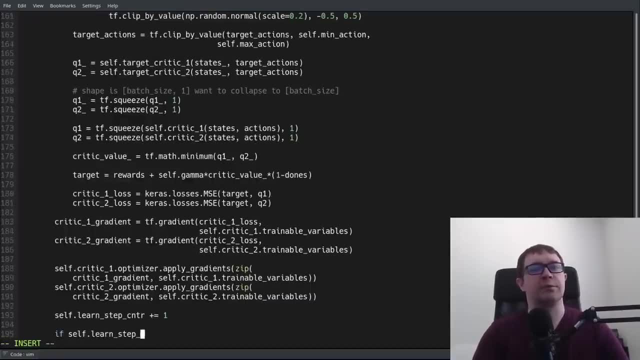 incremented every time we update our critic networks. And then we have to address the question of: is it time to update our actor network? So we'll say: if that learn step counter, modulus, self dot, update actor interval iter- sorry, is not equal to zero, then return. 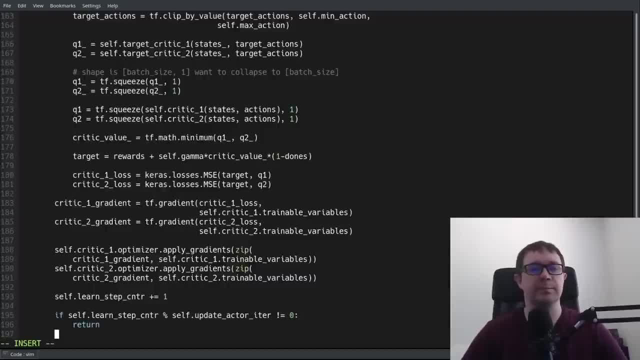 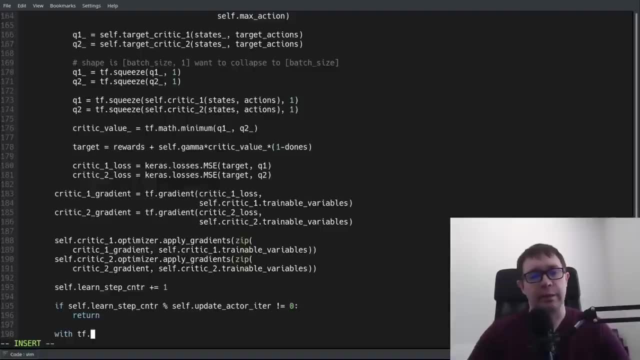 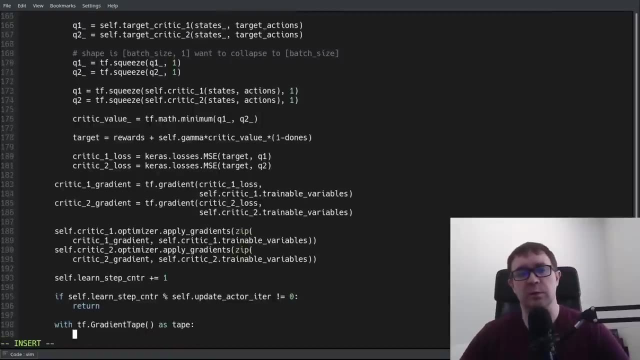 So if it's not every n steps, then go ahead and return. And if we haven't returned, then we're going to go ahead and calculate the loss for our actor network. So, with TF gradient tape as tape, and here since we're just dealing with one loss, 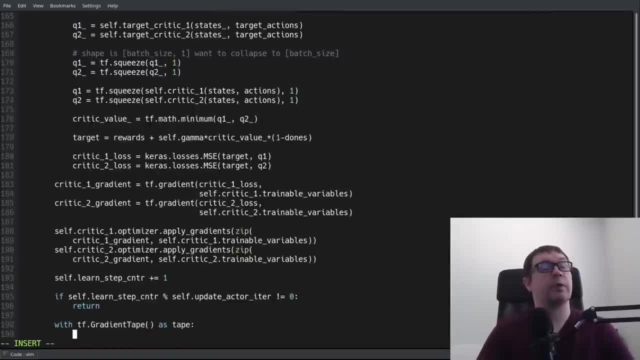 we don't have to call the persistent equals true, We don't have to pass in the persistent equals true argument. So we'll say: our new actions, our the actions chosen by the current parameters or actor network for the current set of states. 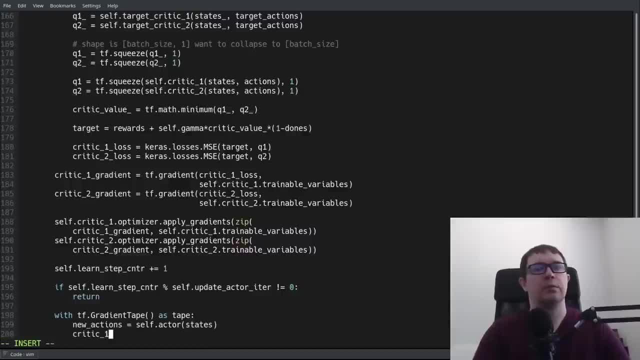 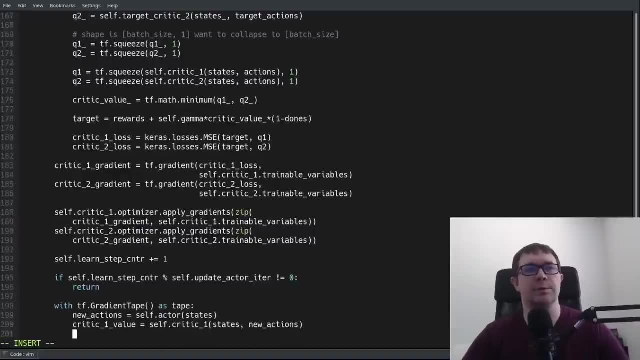 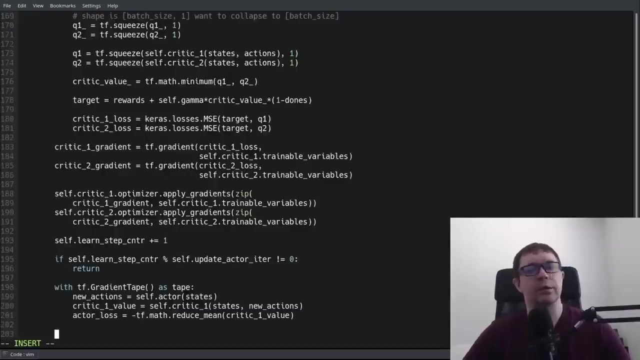 The states. the agent saw along the way. the critic one value is self dot. critic one of those states and new actions. And then our actor loss was negative. TF math reduce mean critic one value. And this may look a little strange to you, but this is how we're going to handle the gradient of the output of one network with respect to the parameters of a network. 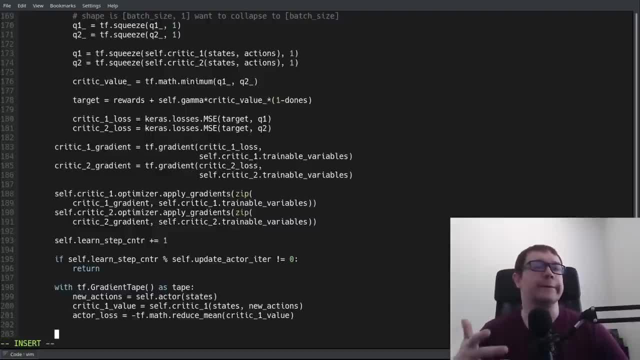 It's kind of like how you apply the chain rule to the, to the loss of the output of the critic network with respect to the parameters of your target actor, your actor network. Sorry, I hope that makes sense. So then we do the same thing where we calculate our green gradient. 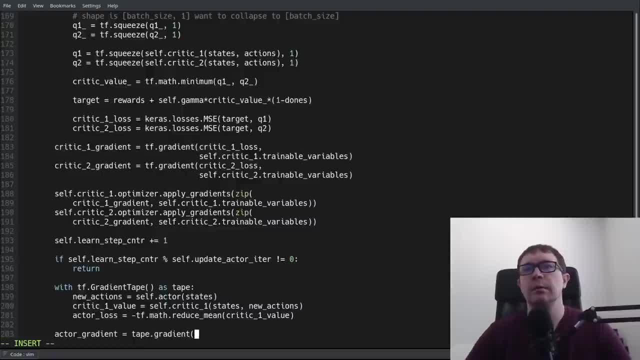 Tape dot gradient. Sorry, Tape dot gradient Did I call? let me make sure I didn't make a mistake. I did make a mistake up here, Sorry. So this should be taped out gradient, not TF. That is one less error to worry about when we get to running the program. 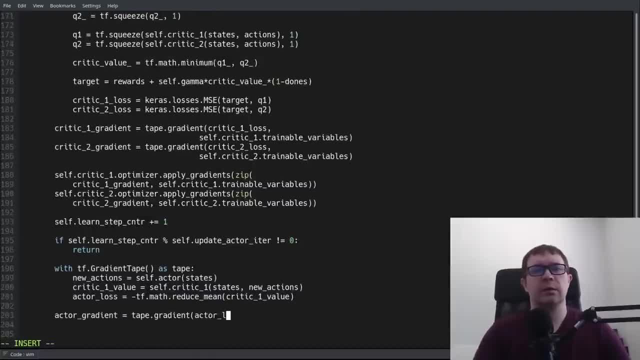 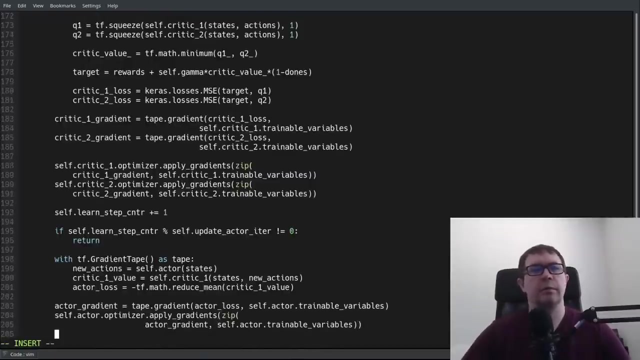 Sorry about that. So, tape dot gradient: actor loss actor trainable variables. I'm going to step our optimizer by applying our gradients Again. that takes a zip as input: actor gradient, self dot- actor trainable variables. Okay, So then finally, 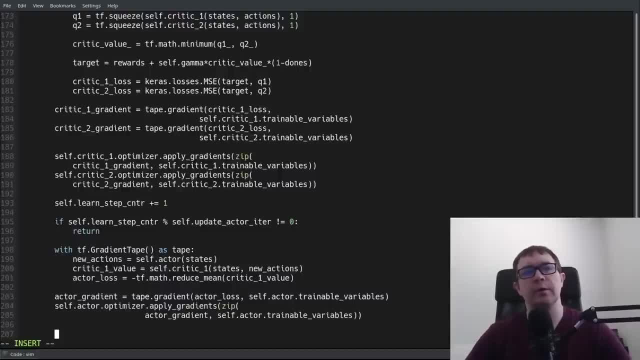 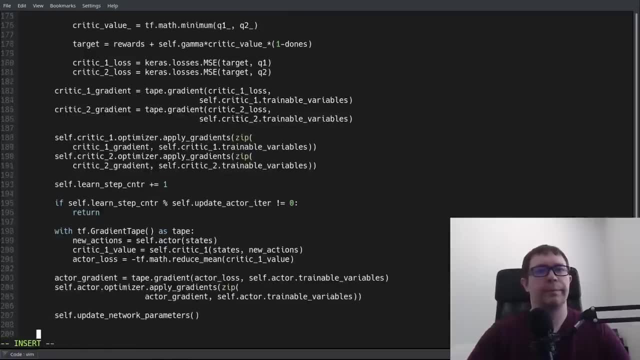 at the end of the learning function. we want to update Our network parameters. Okay, So that really handles all of the learning algorithm for our agent. All that's left now is to update our network parameters and then handle the model savings. So just a few functions left. 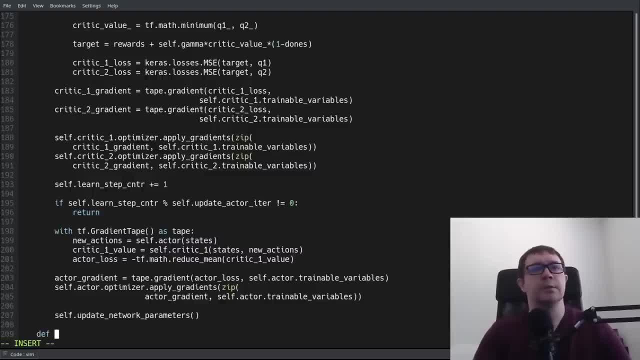 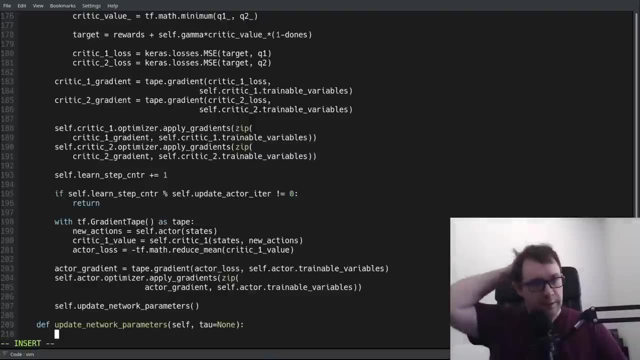 and then we can go right our main loop and see how it does. So. network parameters: Um, so we're going to pass in a default value of towel for none. Remember that at the top of our, rather the end of our initializer we pass in. a towel equals one to handle a hard update. 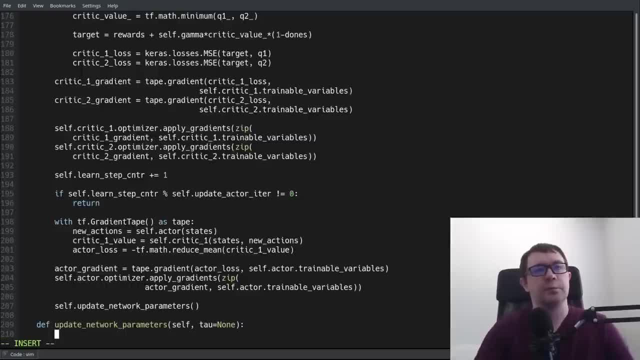 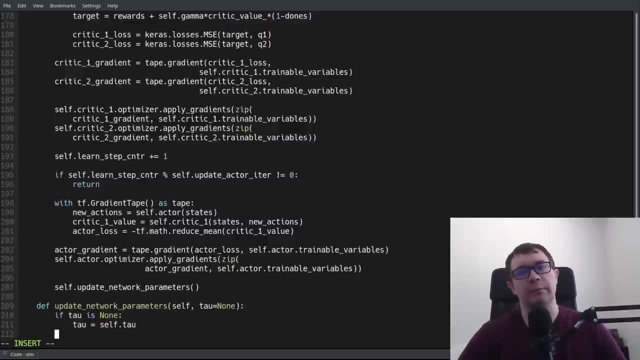 Uh, every other time we're going to pass in a none. So we'll say if towel is none, then towel equals self dot towel. So every time other than the first time we call this, we're going to use the stored value for towel. 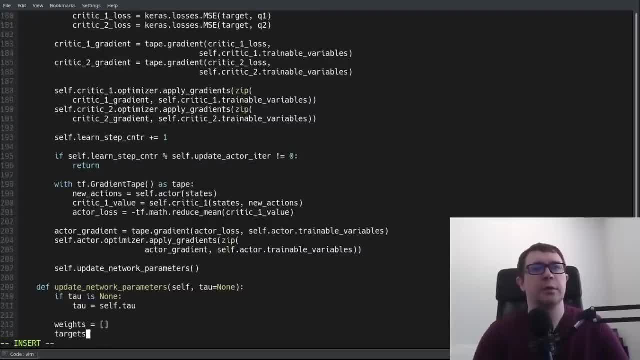 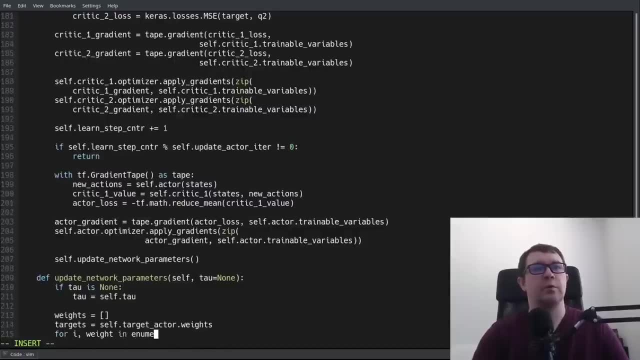 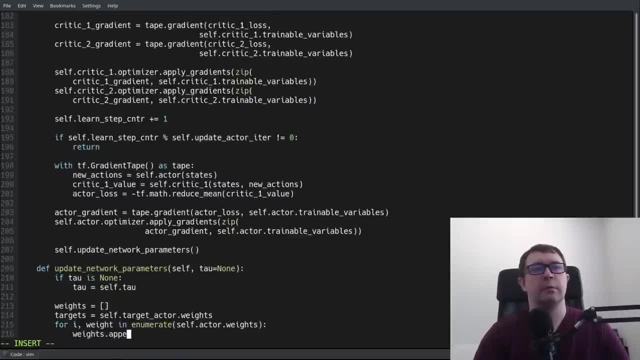 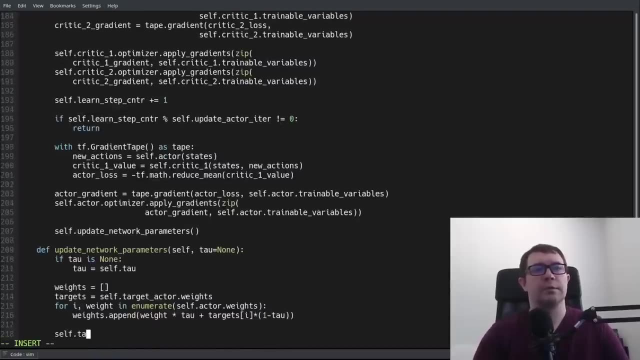 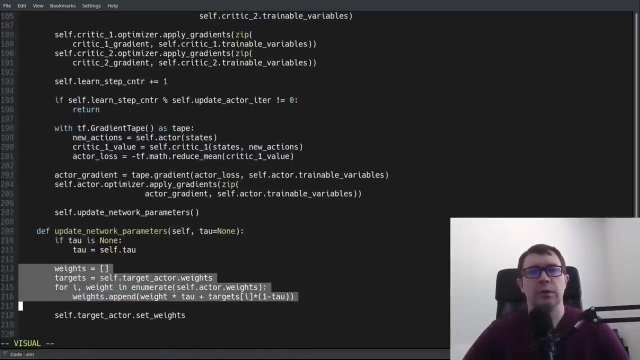 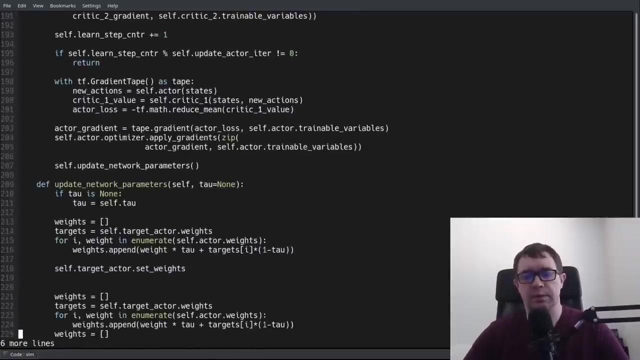 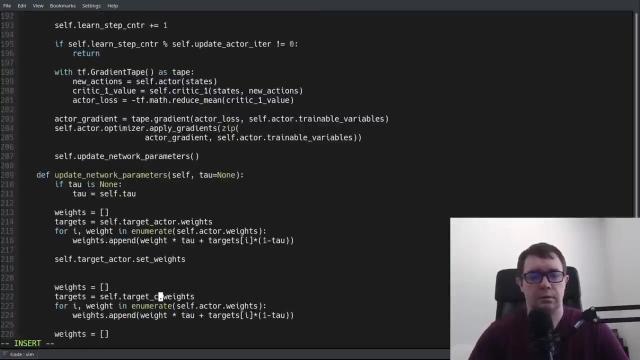 Bain's dot append: uh weight times towel plus targets, Sub I times one minus towel. There we go. and then self dot target actor dot set weights, and I am going to yank this and paste and paste again and then say: target critic one, self dot critic one. 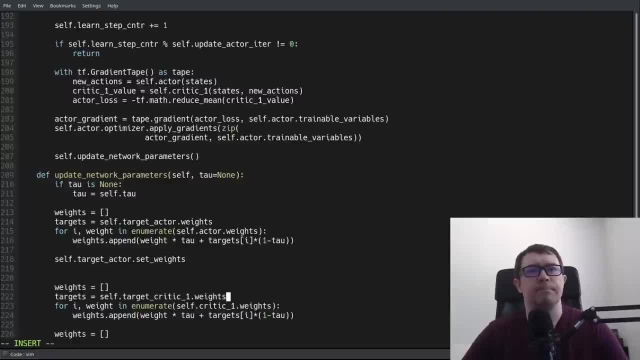 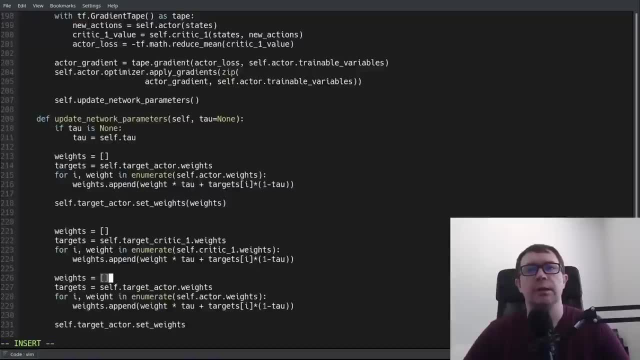 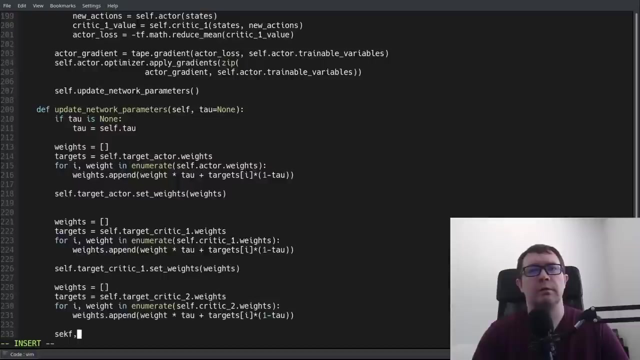 weights, set weight. sorry, I forgot to set the actual value of the weights. how sloppy of me. and then say self dot target critic. one set weights weights, and then we have target critic to enumerate two weights, weights dot append. and then self dot target critic to set weights. 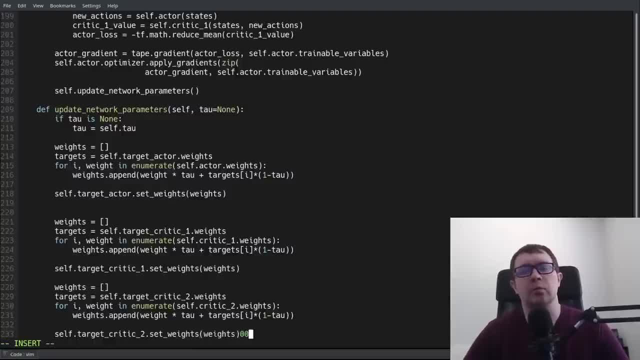 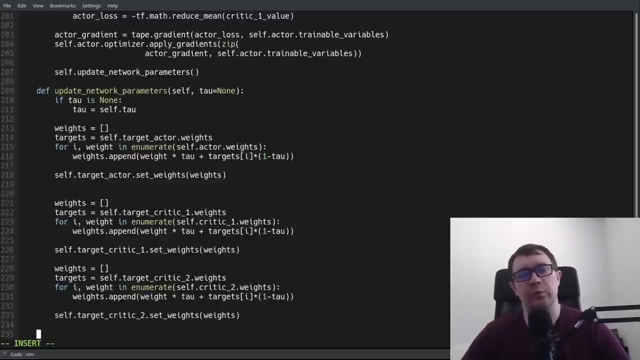 and that handles our update rule for our two networks. sorry, my num lock key is off there, okay, so if it isn't clear what's going on here, we are iterating over the weights of our actor and critic- one critic, two networks. then we're doing the calculation for the soft update rule, saving that in a temporary list and 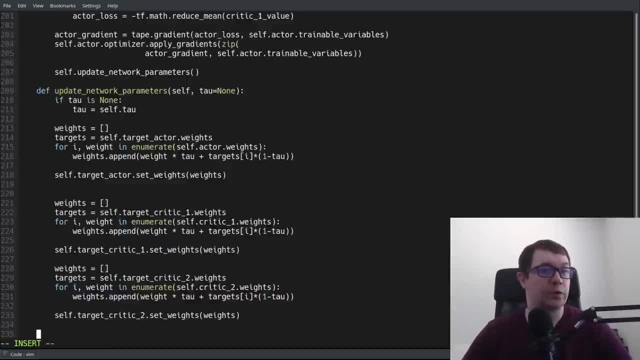 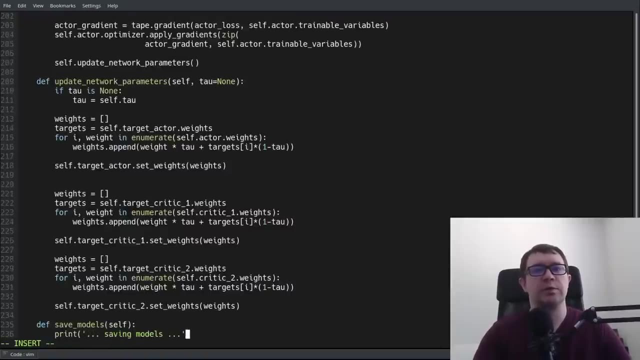 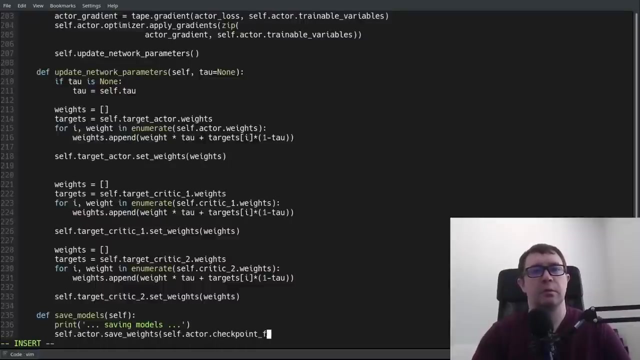 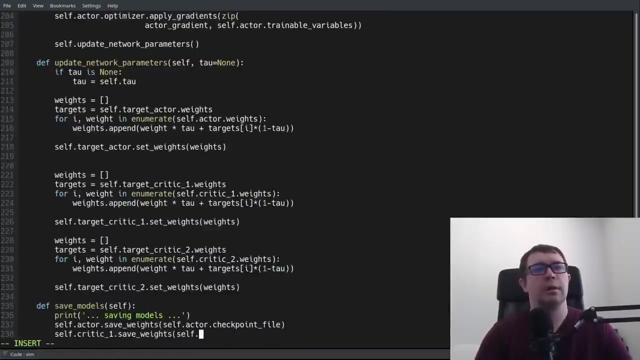 uploading that list to the target actor or target critic one or critic two networks. now we can handle the save model functionality. this is the easiest part of the whole project. so print saving model is just a little debug statement to let us know something is going on. save weights: self dot. actor dot checkpoint file dot critic one. 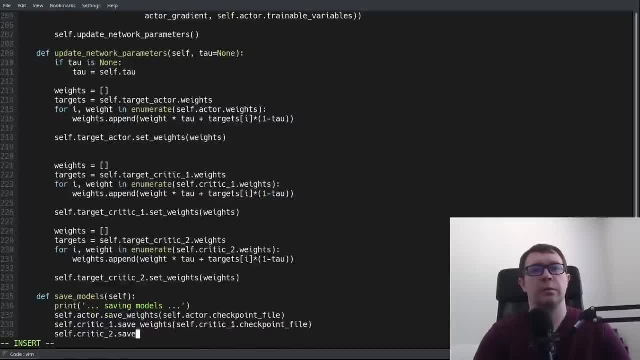 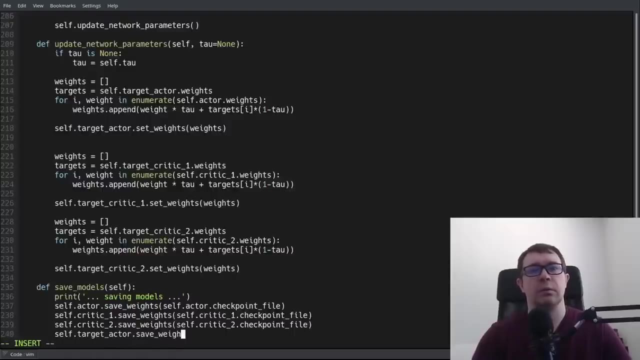 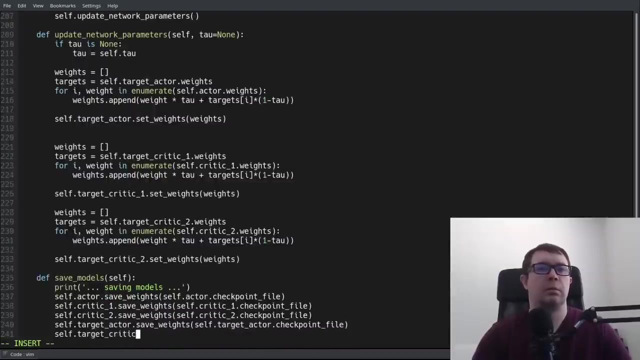 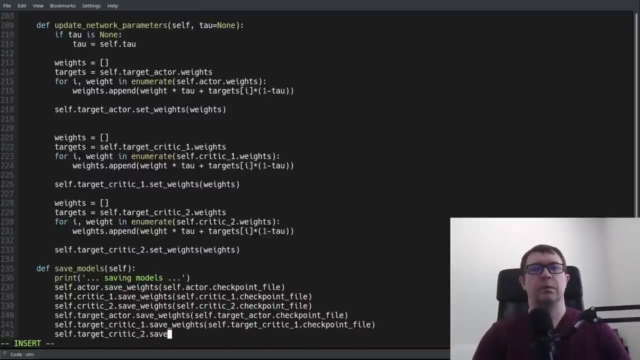 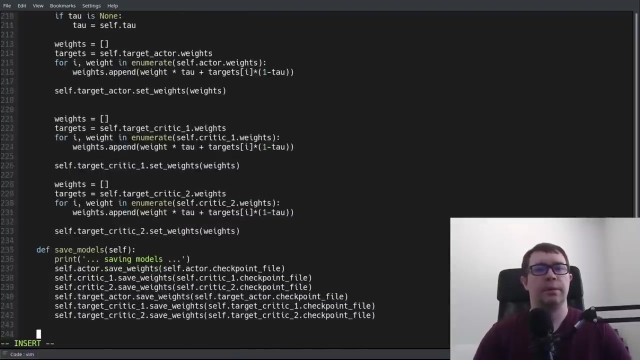 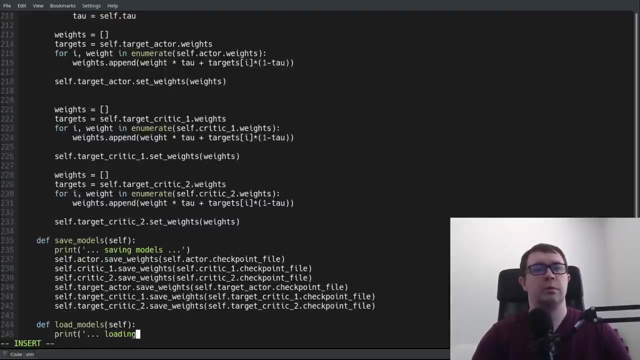 checkpoint file, checkpoint file. and then we have our target networks as well, and then we have our target networks as well, and then we have our target networks as well. good grief. then we do the inverse, then we do the inverse, then we do the inverse operation of loading our models. 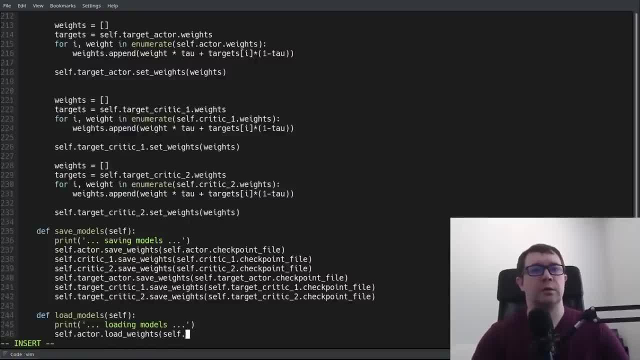 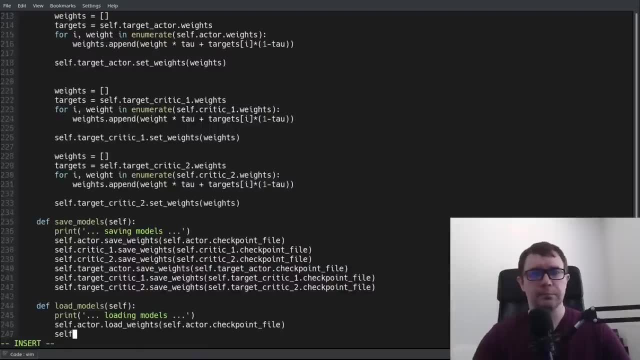 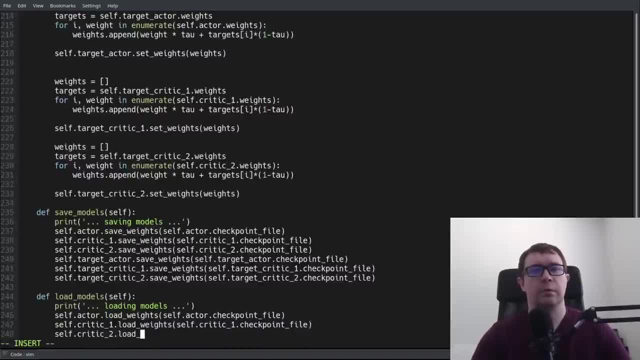 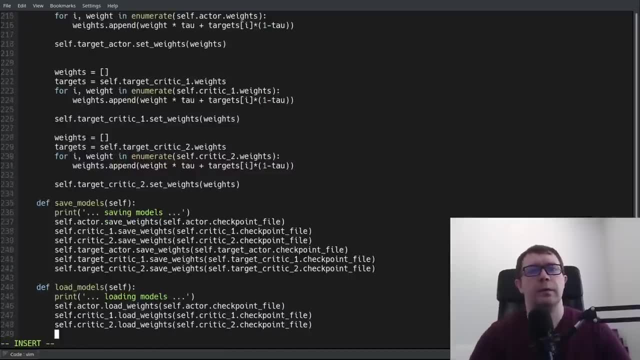 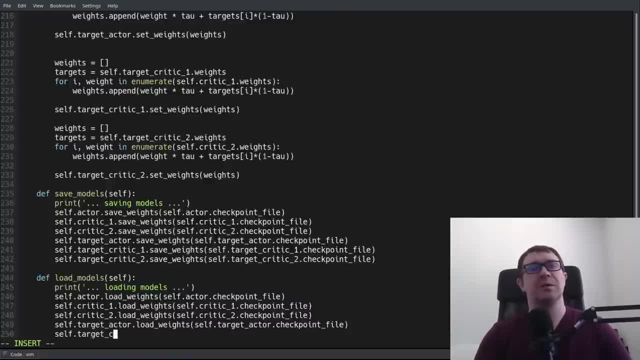 names to save my wrists. a little bit of names to save my wrists. a little bit of work here, but work here, but work here. but hindsight is always 20, 20 i guess. hindsight is always 20, 20, i guess hindsight is always 20, 20, i guess. target critic one. 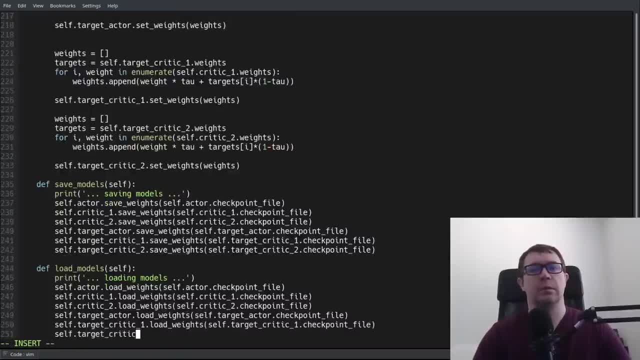 target critic: one target critic, one checkpoint file. okay, so that is it for the main code for. okay, so that is it for the main code for. okay, so that is it for the main code for our td3 algorithm. now we get to handle our td3 algorithm. now we get to handle. 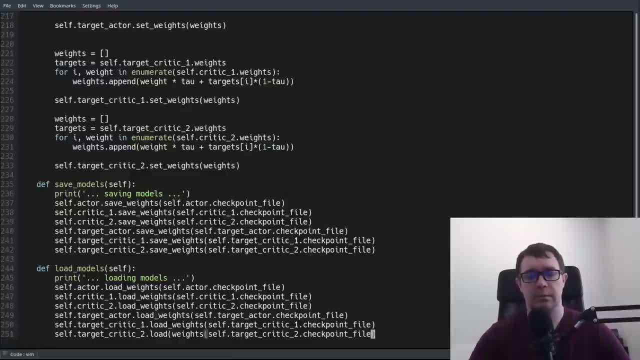 our td3 algorithm. now we get to handle the main loop. so let's go ahead and code the main loop. so let's go ahead and code the main loop. so let's go ahead and code that. up that, up that up now, of course, before we can. 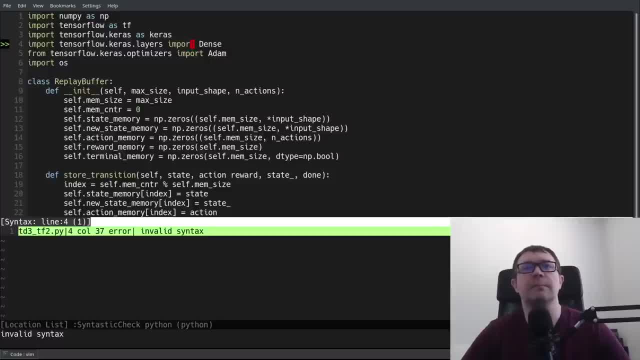 now, of course, before we can, now, of course, before we can, i have an invalid syntax, i have an invalid syntax. i have an invalid syntax right here, at the very beginning, right here at the very beginning, right here at the very beginning: um tensorflowkeroslayers, um tensorflowkeroslayers. 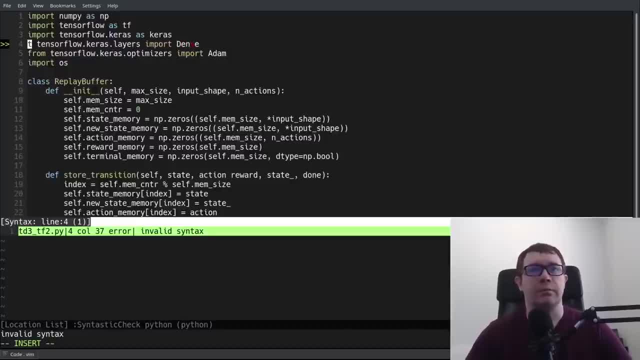 um tensorflowkeroslayers. oh oh, oh, sorry that's because it's a from. sorry that's because it's a from. sorry that's because it's a from import dense. i'll have to notate that in import dense. i'll have to notate that in. 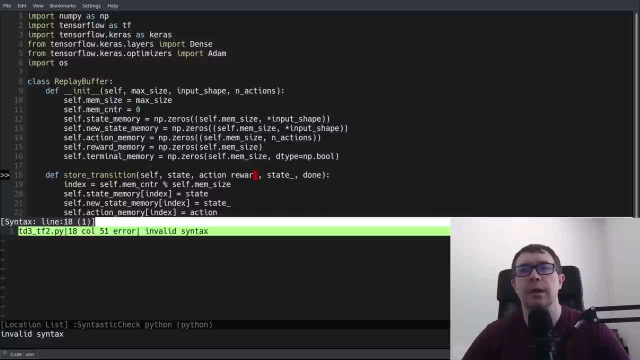 import dense. i'll have to notate that in the video, the video, the video. and i have another issue here and i have another issue here and i have another issue here. uh def store transition, uh def store transition, uh def store transition. where is it unhappy? where is it unhappy? 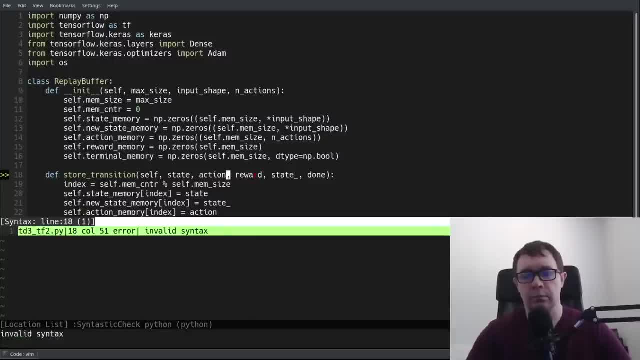 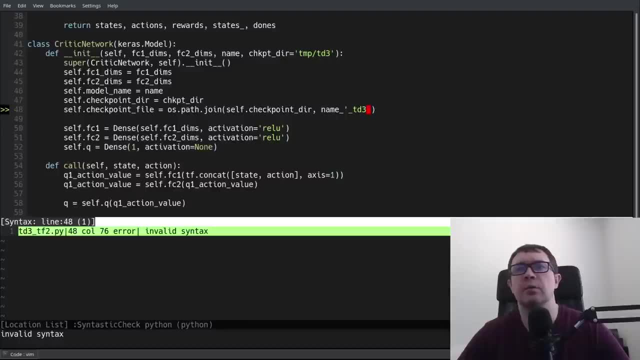 where is it unhappy? i am missing a comma. i am missing a comma. i am missing a comma. of course, of course, of course, and, and and i have another issue: os path join. i have another issue. os path join. i have another issue: os path join, name, name. 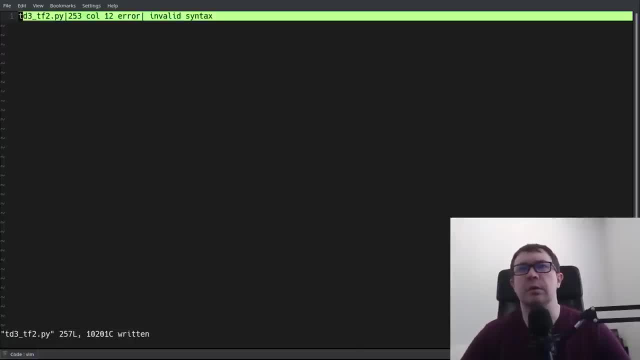 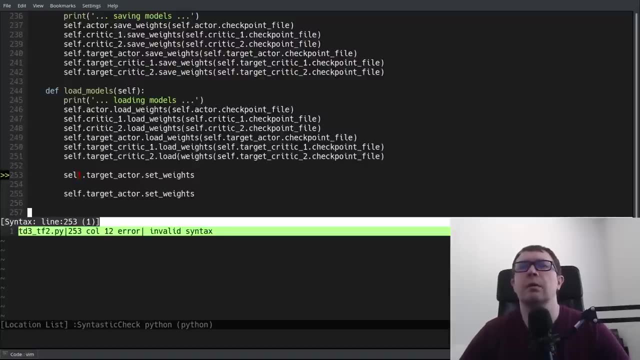 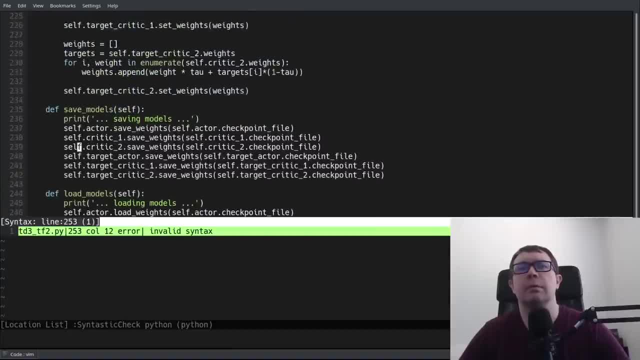 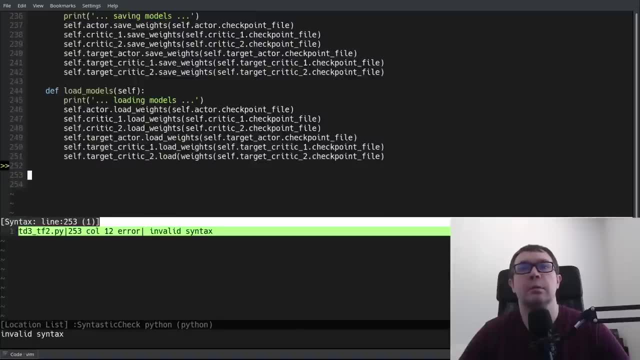 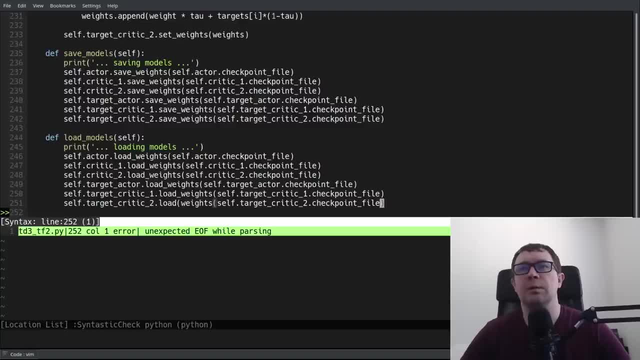 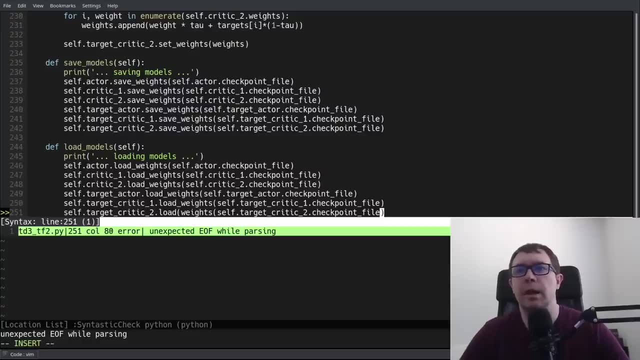 stroke or something, don't remember it. very strange, very strange, very strange, okay, unexpected, okay, unexpected, okay, unexpected. end of file. let's delete there. end of file. let's delete there. end of file. let's delete there. same same same. uh, am i forgetting a? uh, am i forgetting a? 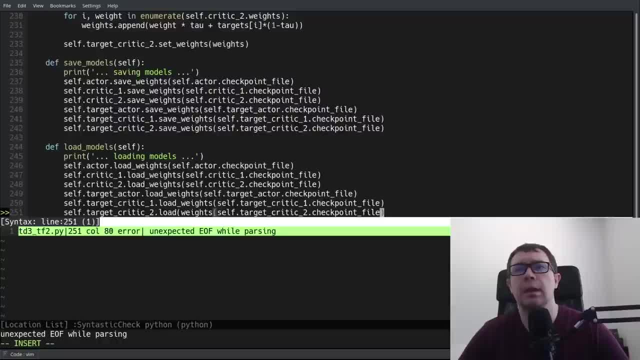 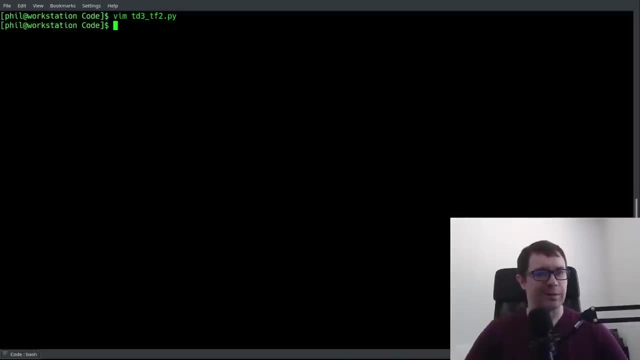 uh, am i forgetting a parenthesis somewhere? parenthesis somewhere, parenthesis somewhere. uh, uh, uh, i am, i am. i am because i have right there. all right, finally, good grief, that's a all right. finally good grief, that's a all right. finally, good grief, that's a whole lot of typos. 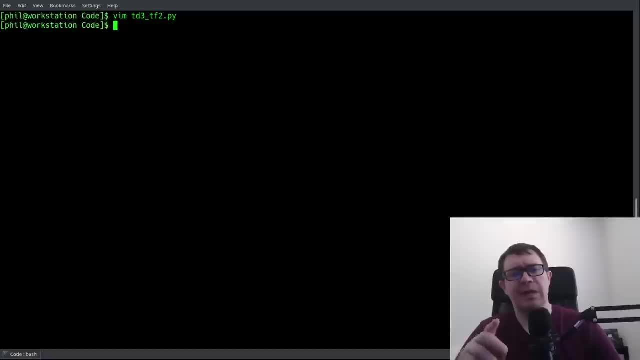 whole lot of typos, whole lot of typos. now some people suggest that i upgrade my now some people suggest that i upgrade my. now some people suggest that i upgrade my vim, vim, vim and to actually catch that stuff on the. and to actually catch that stuff on the. 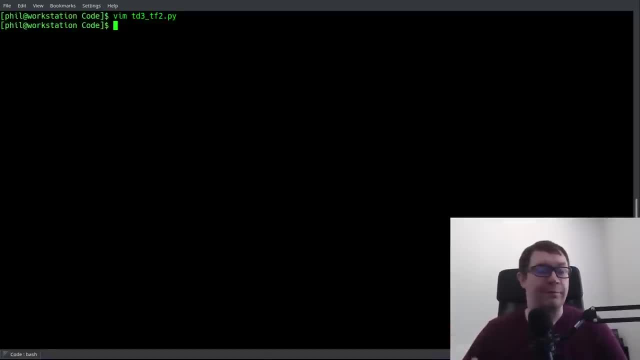 and to actually catch that stuff on the fly. and you're absolutely right, i'm fly. and you're absolutely right, i'm fly. and you're absolutely right, i'm going to do that, going to do that, going to do that when i finally force myself to do it. 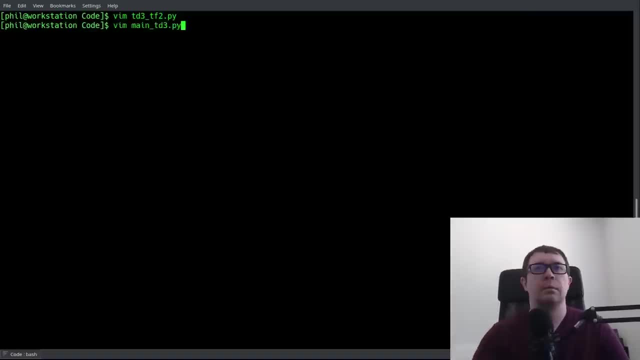 when i finally force myself to do it, when i finally force myself to do it. let's go ahead, let's go ahead, let's go ahead in the meantime and write our main loop in the meantime and write our main loop in the meantime and write our main loop. so we want to import. 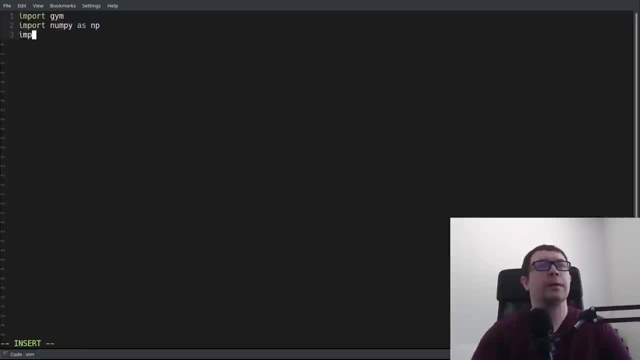 so we want to import. so we want to import: jim, jim, jim, numpy, numpy, numpy. we'll need our agent, we'll need our agent, we'll need our agent and we'll need our utility file and we'll need our utility file and we'll need our utility file. uh, plot learning curve, you can do a git. 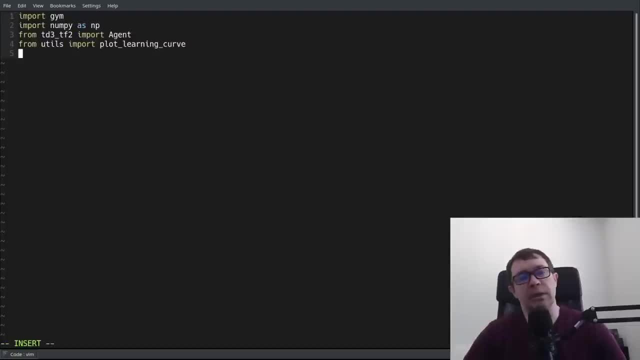 uh plot learning curve. you can do a git uh plot learning curve. you can do a git clone on my github to get that clone on my github. to get that clone on my github to get that. it's just a matplotlib pi plot with. it's just a matplotlib pi plot with. 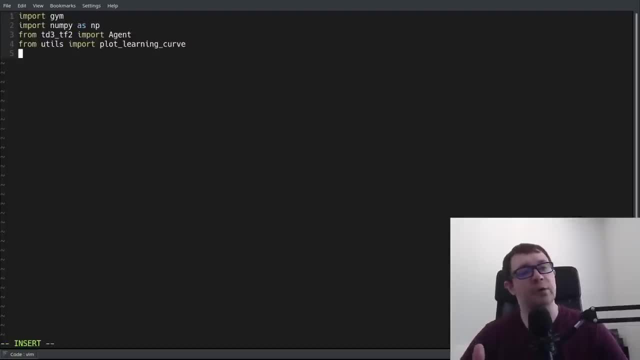 it's just a matplotlib pi plot with some labeled axes, some labeled axes, some labeled axes. uh, where we're taking an average of the uh, where we're taking an average of the uh. where we're taking an average of the previous 100 games running. previous 100 games running. 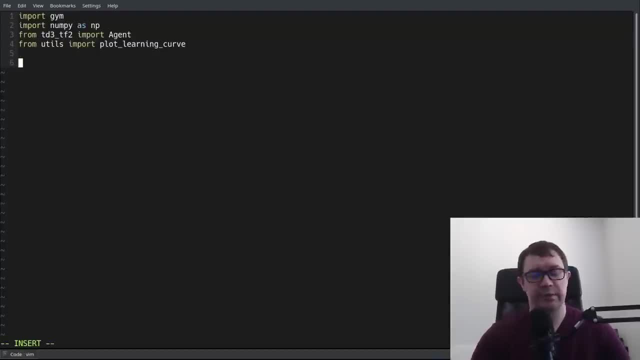 previous 100 games running. um, i don't include that in all my videos. um, i don't include that in all my videos. um, i don't include that in all my videos. i just kind of, i just kind of, i just kind of reference my github. reference my github. 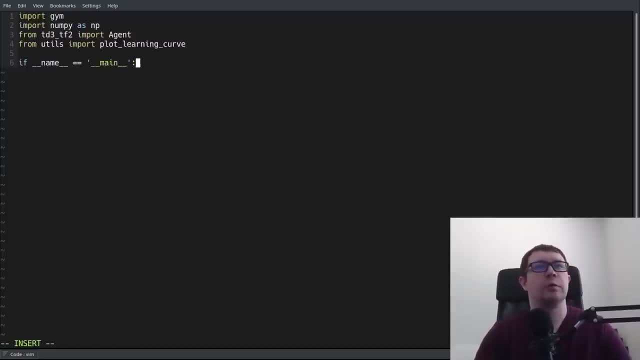 reference my github. you can just do a plot. you can just do a plot. you can just do a plot if you wish. if you wish, if you wish. name equals main name equals main name equals main jimmake, jimmake, jimmake. we're going to be doing the bipedal. 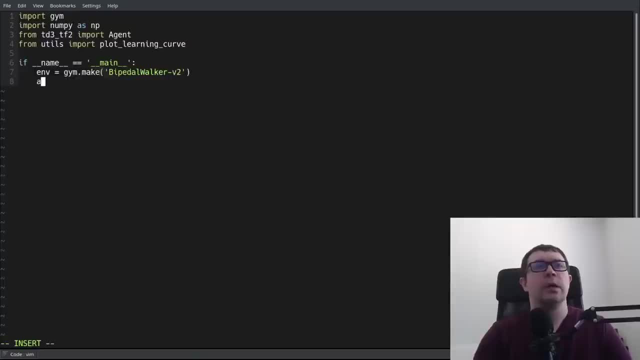 we're going to be doing the bipedal, we're going to be doing the bipedal walker v2, walker v2, walker v2, and we're going to call our and we're going to call our and we're going to call our agent constructor. 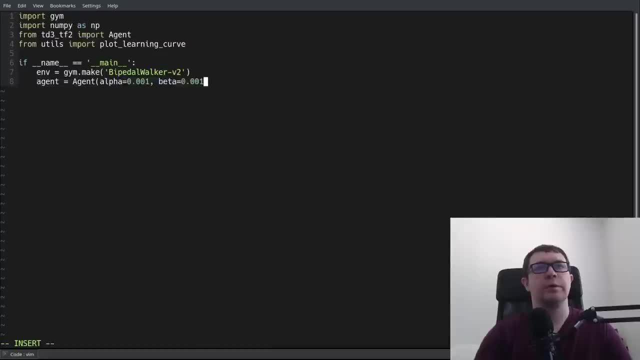 agent constructor. agent constructor alpha 0.01. a beta of 0.001. our input dimensions will be determined. our input dimensions will be determined. our input dimensions will be determined by our environment, so we don't have to. by our environment, so we don't have to. 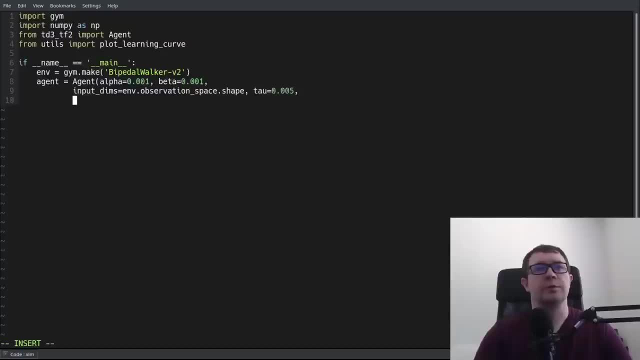 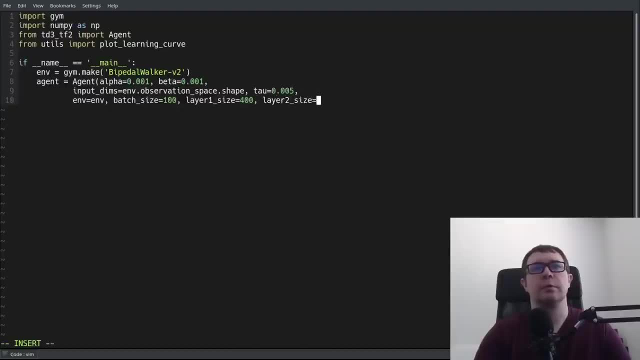 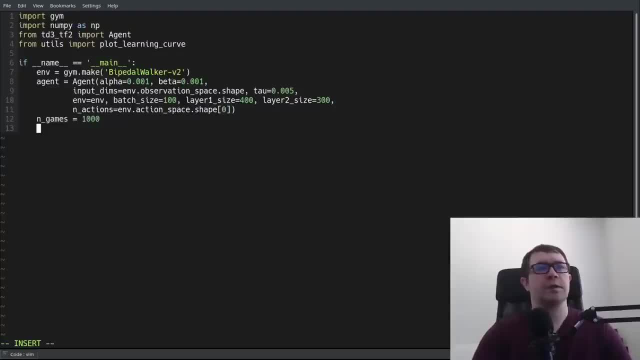 by our, by our environment, environment, environment. we'll let this bad boy play a thousand. we'll let this bad boy play a thousand. we'll let this bad boy play a thousand. games, games, games, and we'll call our file name. and we'll call our file name. 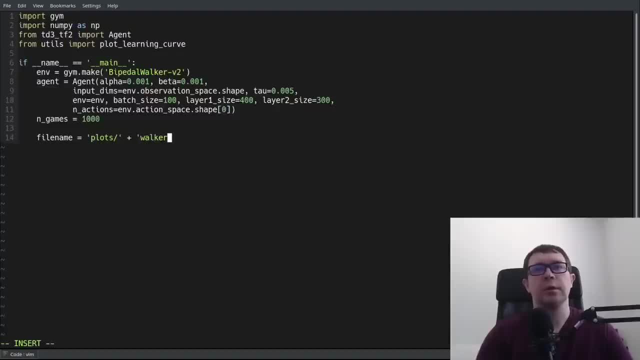 and we'll call our file name: plots plus walker underscore. plots plus walker underscore. plots plus walker underscore. now, keep in mind, you have to do make now. keep in mind, you have to do make now. keep in mind you have to do make dirt plots and make dirt temp. slash gd3. 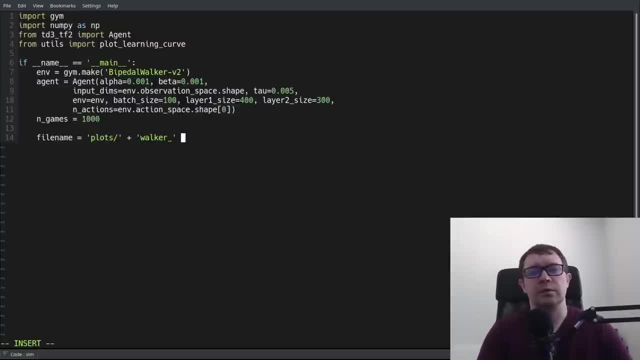 dirt plots and make dirt temp slash gd3. dirt plots and make dirt temp slash gd3. to correctly execute. to correctly execute, to correctly execute the code, the code. the code because it'll expect that, those because it'll expect that those because it'll expect that those directories exist. 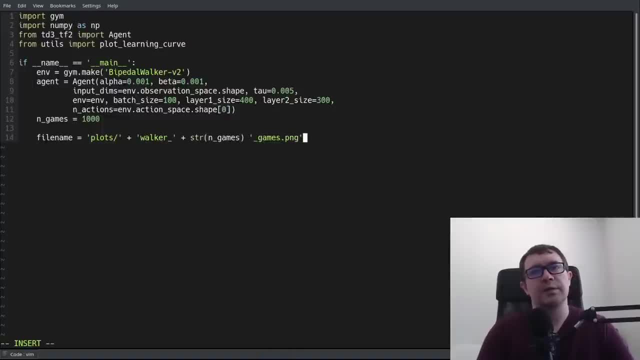 directories exist. directories exist. pass in number of games. pass in number of games. pass in number of games: uh as a variable for your file name. uh as a variable for your file name. uh as a variable for your file name. that way, if you run it over and over, 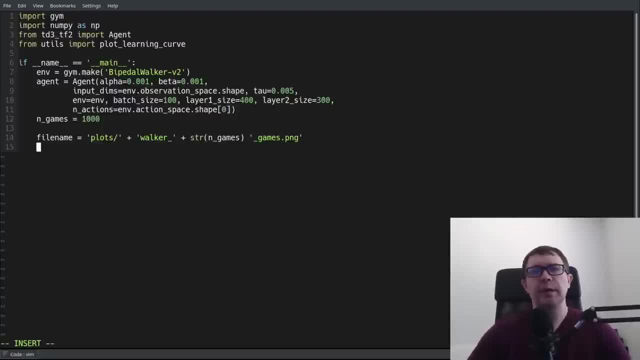 that way, if you run it over and over that way, if you run it over and over again with different numbers of games, it again with different numbers of games, it again with different numbers of games, it won't overwrite the same plot you can. won't overwrite the same plot you can. 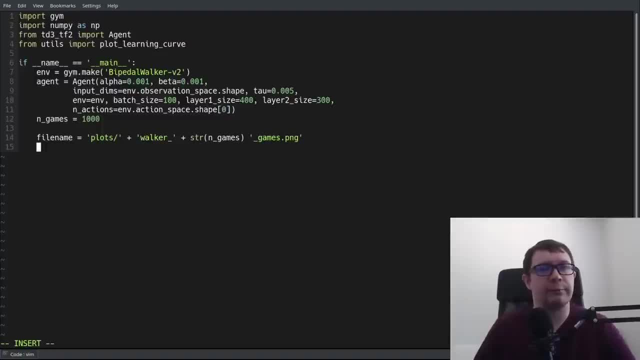 won't overwrite the same plot. you can also include things like learning rates. also include things like learning rates. also include things like learning rates as part of your variable name for your, as part of your variable name for your, as part of your variable name for your file names. i recommend doing that. i'm. 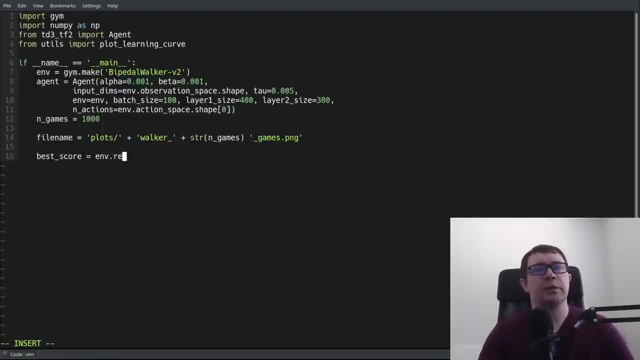 file names. i recommend doing that. i'm file names. i recommend doing that. i'm just not doing it here, just not doing it here, just not doing it here. so we need to keep track of our. so we need to keep track of our. so we need to keep track of our best score. it's the minimum score of 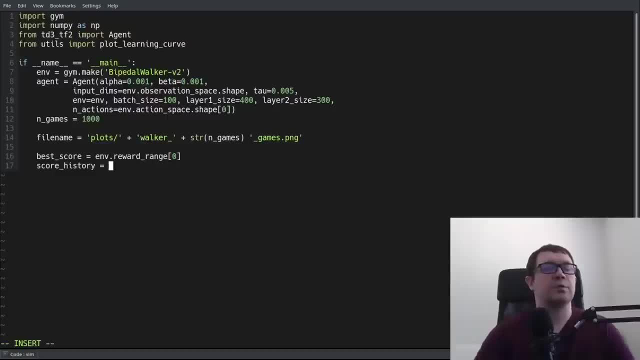 best score. it's the minimum score of best score. it's the minimum score of our environment, our environment, our environment, and the reason is we want to save our, and the reason is we want to save our, and the reason is we want to save our best models. 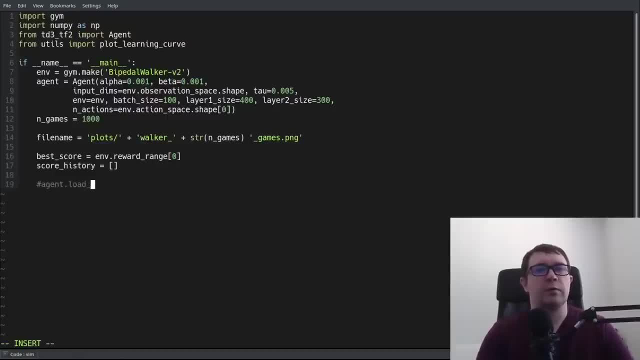 best models, best models. keep track of your score history. if you keep track of your score history, if you keep track of your score history, if you want to load models, want to load models, want to load models, now is the appropriate time to do that. now is the appropriate time to do that. 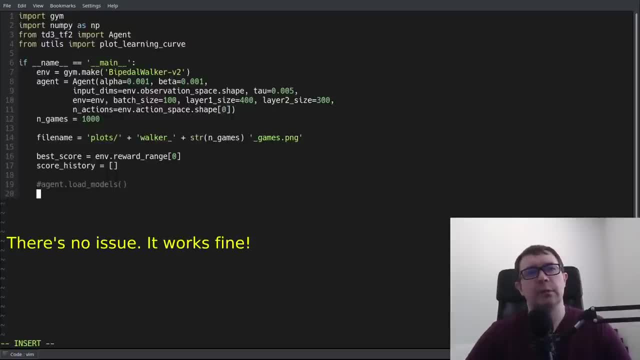 now is the appropriate time to do that. actually, you know what we may need. actually, you know what we may need. actually, you know what we may need. there may be an issue where there may be an issue where there may be an issue where we have to actually instantiate. 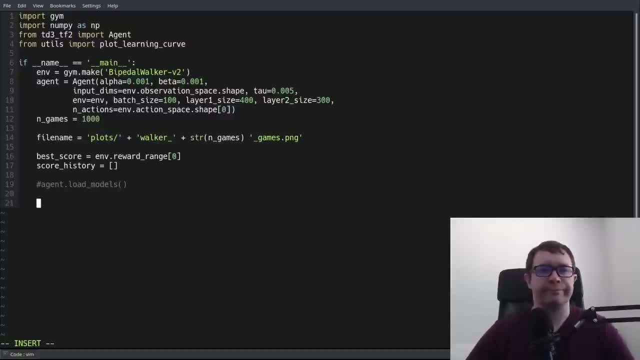 we have to actually instantiate. we have to actually instantiate our network with some variables to load our network with some variables, to load our network with some variables to load the models, the models, the models. open up an issue on my github if that's open up an issue on my github if that's. 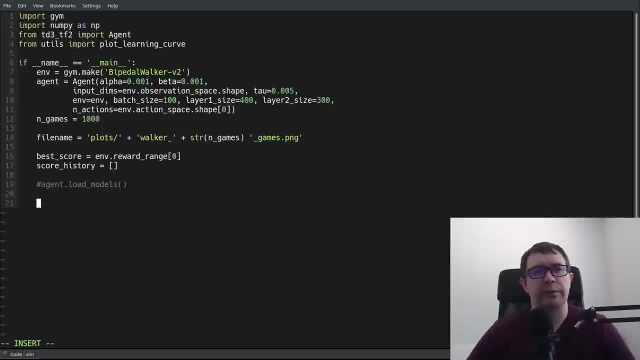 open up an issue on my github, if that's the case, and i will write the correct the case, and i will write the correct the case and i will write the correct code. i won't bother code. i won't bother code. i won't bother with the video. i'll leave that as an. 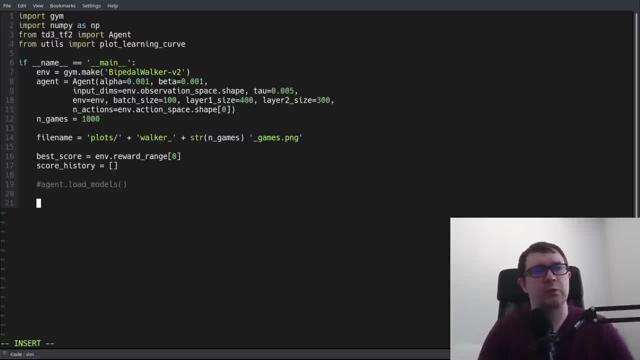 with the video. i'll leave that as an with the video. i'll leave that as an exercise for the viewer. but if it turns exercise for the viewer, but if it turns exercise for the viewer, but if it turns out to be a problem, raise an issue and 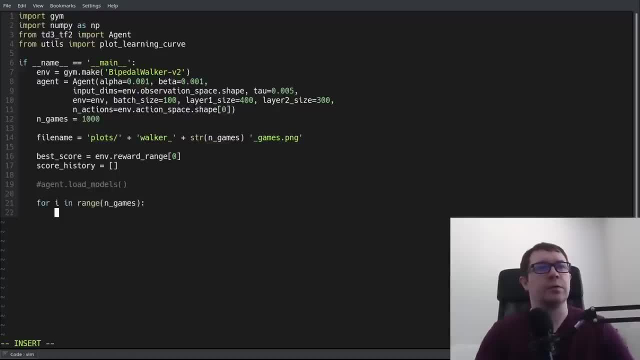 out to be a problem. raise an issue and out to be a problem. raise an issue and i can fix that. i can fix that. i can fix that. not a huge deal, not a huge deal, not a huge deal. let's go ahead and play our games start. 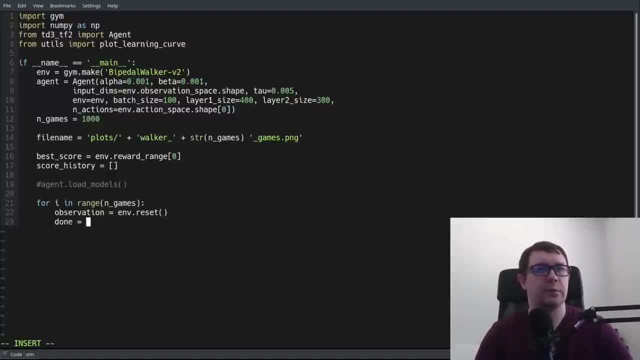 let's go ahead and play our games start. let's go ahead and play our games. start by resetting the environment at the top. by resetting the environment at the top, by resetting the environment at the top of every episode, of every episode, of every episode, reset the done flag and zero. 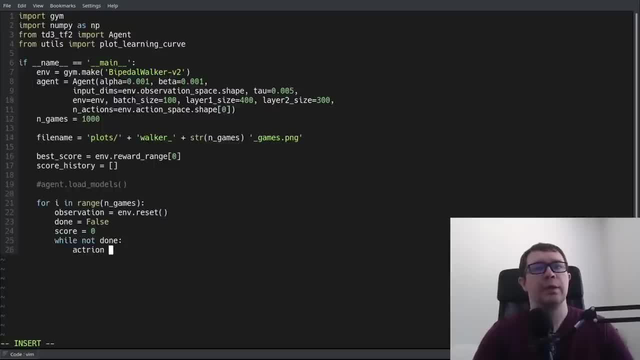 reset the done flag and zero. reset the done flag and zero. and let's play our episode while not done. and let's play our episode while not done. and let's play our episode while not done. action, action, action. eagles agent dot. choose action based on. eagles agent dot. choose action based on. 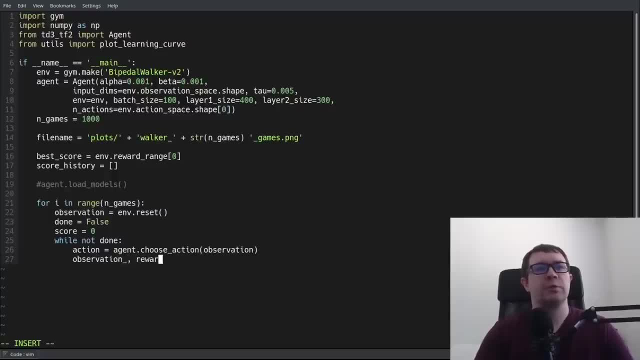 eagles agent dot. choose action based on the observation, the observation, the observation. let's take that action. get the new state. let's take that action. get the new state. let's take that action. get the new state reward done and debug info from our. reward done and debug info from our. 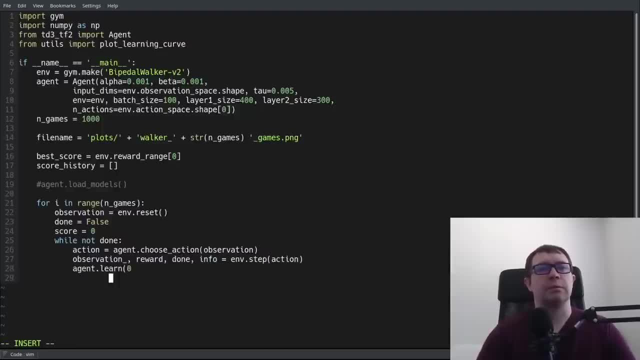 reward done and debug info from our environment, environment, environment. uh call our learn function. uh call our learn function. uh call our learn function. uh keep track of our score. uh keep track of our score. uh keep track of our score and set the current state. and set the current state. 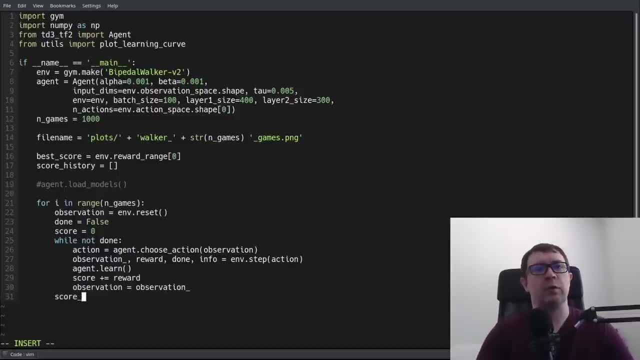 and set the current state to to to the new state very important. if you, the new state, very important. if you, the new state, very important. if you don't do that, nothing is going to go well. don't do that, nothing is going to go well. don't do that, nothing is going to go well for you. 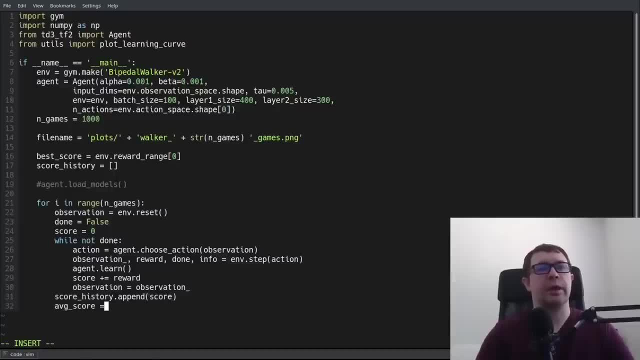 for you, for you. let's depend on our score at the bottom. let's depend on our score at the bottom. let's depend on our score at the bottom of every episode and calculate our of every episode. and calculate our of every episode and calculate our average minus 100 onward. if our average score is. 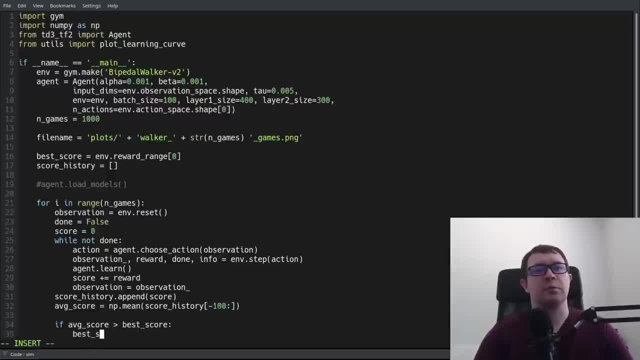 minus 100 onward. if our average score is minus 100 onward. if our average score is greater than our best score, greater than our best score, greater than our best score, then set the best score to that average, then set the best score to that average, then set the best score to that average. and. 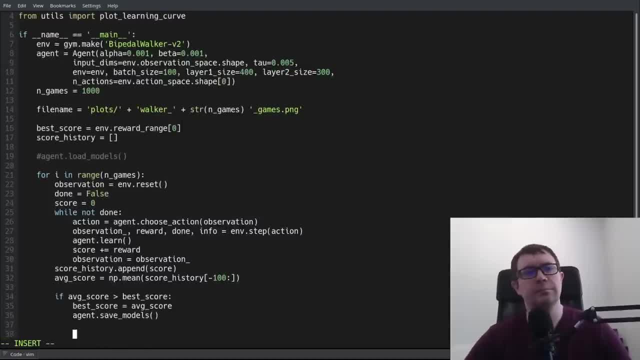 and and save our models, save our models, save our models. and then we want to print some debug. and then we want to print some debug and then we want to print some debug. information episode: I score 1f average. information episode: I score 1f average. 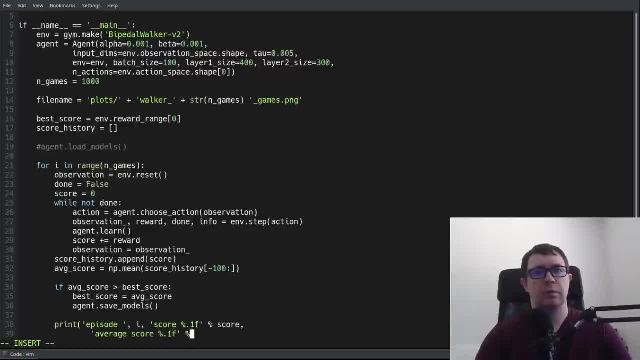 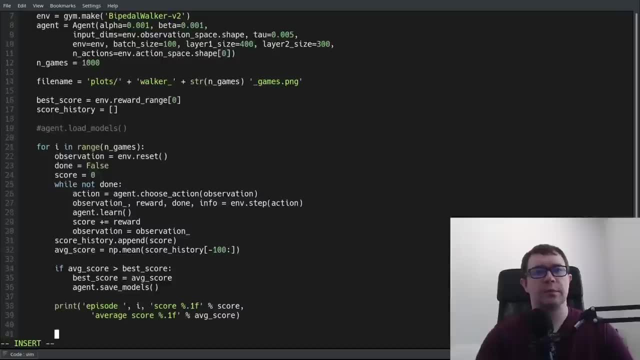 information episode: I score 1f- average score- average score. and at the end of score: average score. and at the end of score: average score. and at the end of all the games. let's go ahead and handle all the games. let's go ahead and handle all the games. let's go ahead and handle our plotting. our x-axis is just the. 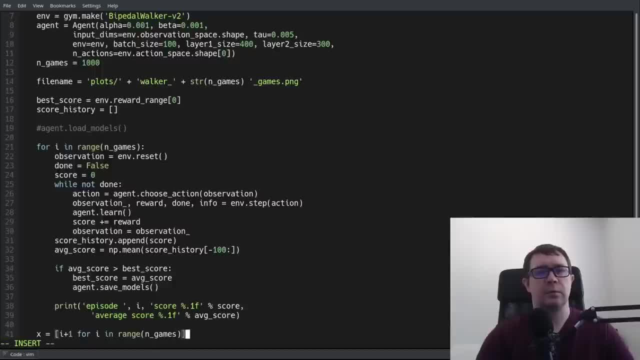 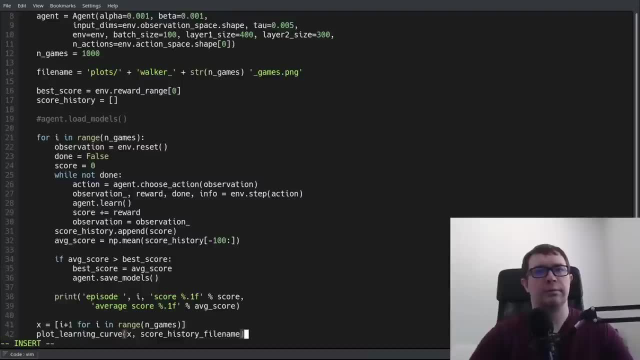 our plotting our x-axis is just the. our plotting our x-axis is just the number of games, number of games, number of games. and call plot learning curve: alright, so moment of. and call plot learning curve: alright, so moment of. and call plot learning curve: alright, so moment of truth. let's go ahead and see. 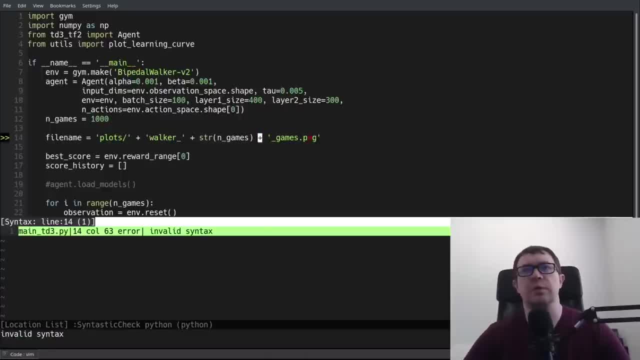 truth. let's go ahead and see truth. let's go ahead and see where I have my invalid syntax. I forgot an where I have my invalid syntax. I forgot an where I have my invalid syntax. I forgot an addition sign. they're very simple addition sign. they're very simple. 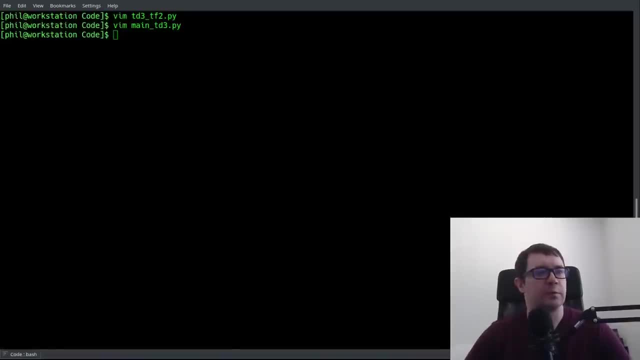 addition sign. they're very simple. alright, let's try it. oh, you know what? alright, let's try it. oh you know what? alright, let's try it. oh you know what, I'm running it over in this other. I'm running it over in this other. I'm running it over in this other terminal, and okay, so it saves models. it. 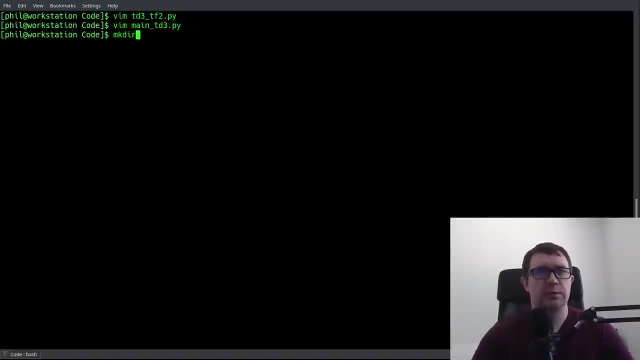 terminal and okay, so it saves models. it terminal and okay, so it saves models. it is learning, is learning, is learning. that is good to know. let's do a make der, that is good to know. let's do a make der, that is good to know. let's do a make der temp slash td3. I should already have. 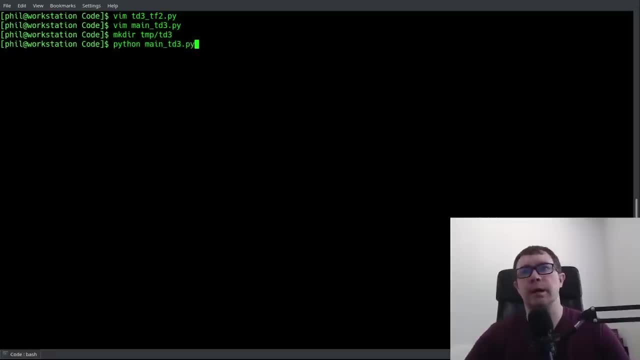 temp slash td3. I should already have temp slash td3. I should already have plots: Python main td3 dot pi moment of plots. Python main td3 dot pi moment of plots. Python main td3 dot pi moment of truth. okay, so it says actor network truth. okay, so it says actor network. 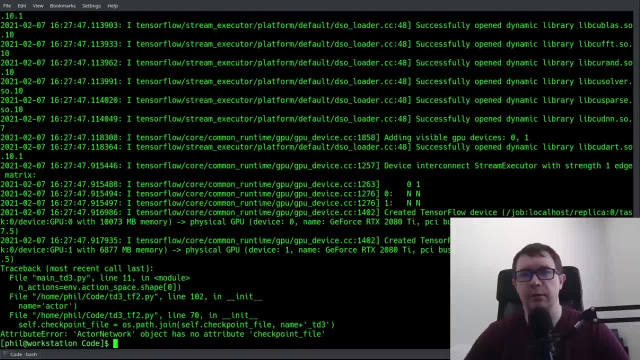 truth. okay. so it says: actor network object has no attribute checkpoint file. object has no attribute checkpoint file. object has no attribute checkpoint file. I didn't oh, it's checkpoint directory. I didn't oh, it's checkpoint directory. I didn't oh, it's checkpoint directory. so that is in td3 tf2. 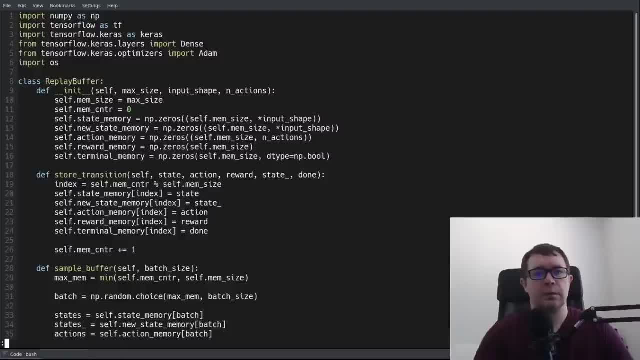 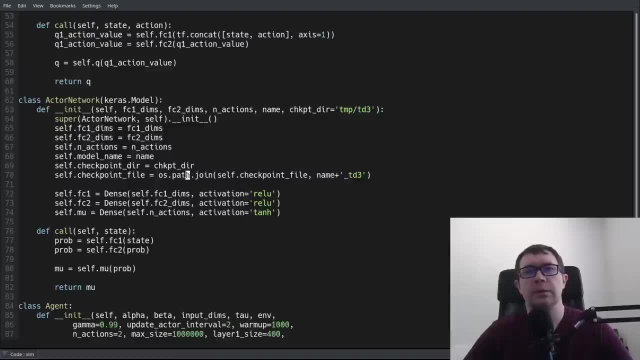 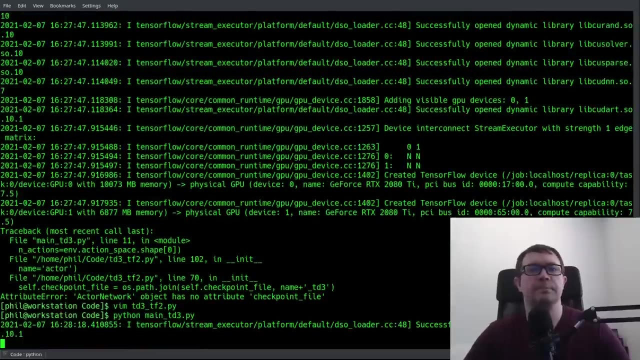 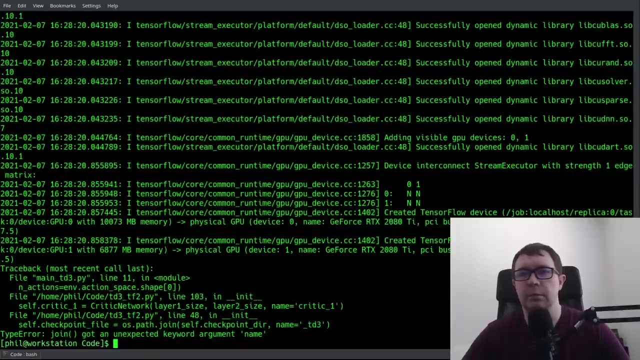 so that is in td3 tf2. so that is in td3 tf2. that is in line 70, so that is here. okay, try it again. got that is in line 70, so that is here. okay, try it again. got that is in line 70, so that is here. okay, try it again. got an unexpected argument. name that is. 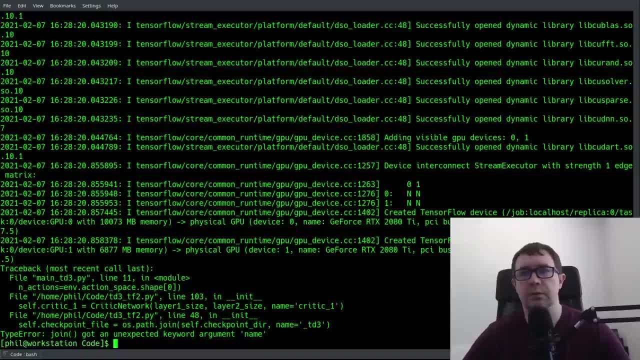 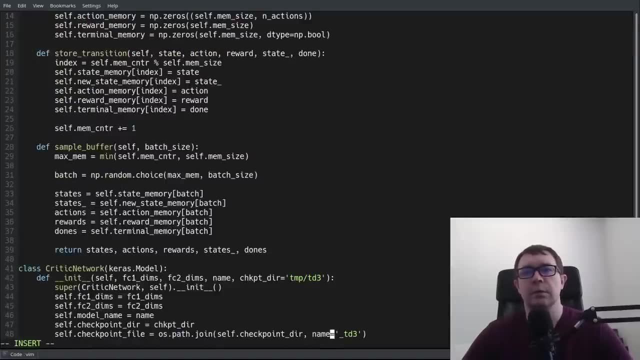 an unexpected argument name. that is an unexpected argument name that is in, in, in, in, in, in. oh, that's because, okay, that is in line 48, that is super trivial, it's. oh, that's because, okay, that is in line 48, that is super trivial, it's. 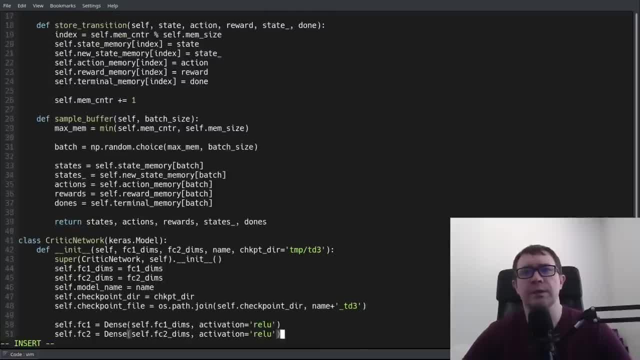 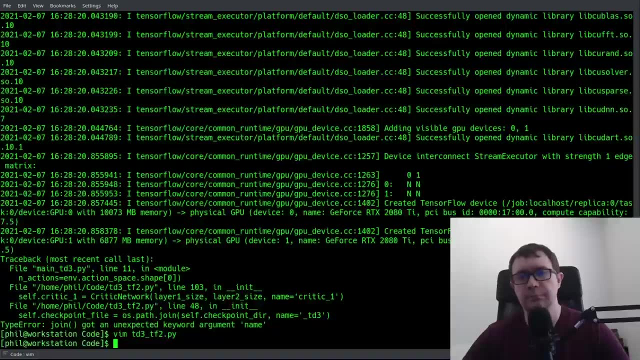 oh, that's because, okay, that is in line 48. that is super trivial, it's not. name equals its name. plus, did I not? name equals its name. plus did I not? name equals its name. plus, did I do that down here as well? no, I did not. I'm. do that down here as well. no, I did not. I'm do that down here as well. no, I did not. I'm not looking forward to editing this, not looking forward to editing this, not looking forward to editing this. this is gonna be a lot of work, okay, so. 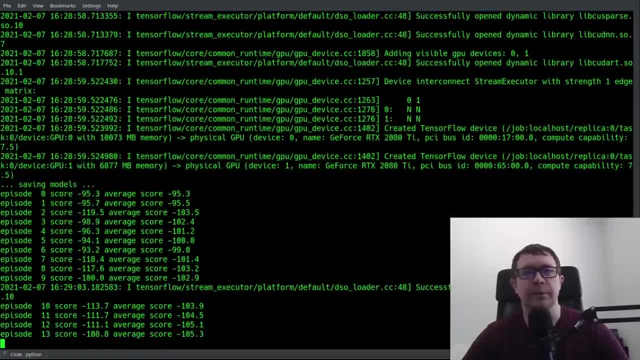 this is gonna be a lot of work, okay, so this is gonna be a lot of work, okay. so it saves models right off the bat and it saves models right off the bat and it saves models right off the bat and starts running. okay, so I'm gonna let. 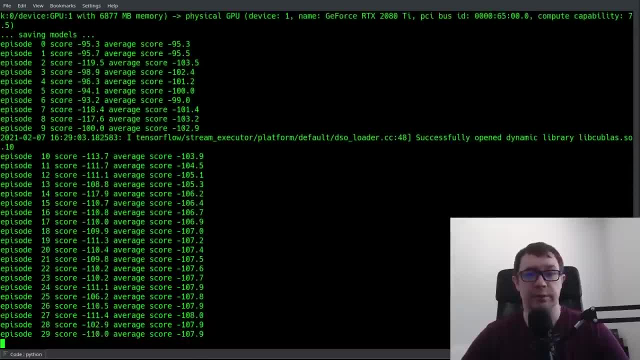 starts running. okay, so I'm gonna let starts running. okay, so I'm gonna let this run for a while, and then we're this run for a while, and then we're this run for a while, and then we're gonna see how it does. okay, so I did. 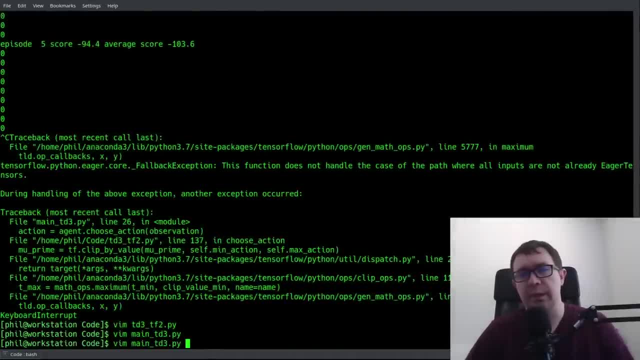 gonna see how it does okay. so I did gonna see how it does okay. so I did something very stupid and I let it run something very stupid and I let it run something very stupid and I let it run and noticed it wasn't actually learning. and noticed it wasn't actually learning. 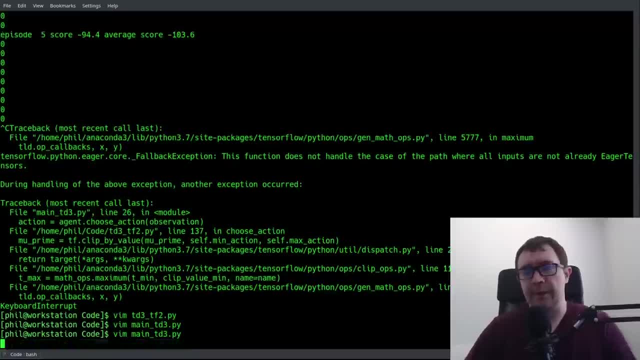 and noticed it wasn't actually learning, and so that's a problem and the reason, and so that's a problem. and the reason and so that's a problem and the reason it's not learning is because I forgot to. it's not learning is because I forgot to. 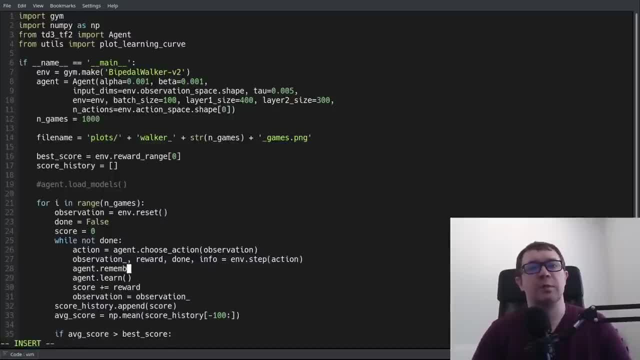 it's not learning is because I forgot to store the transition. so we have to say store the transition. so we have to say store the transition. so we have to say: agent: remember observation action, reward. agent- remember observation action, reward. agent- remember observation action, reward, observation, underscore and done okay. 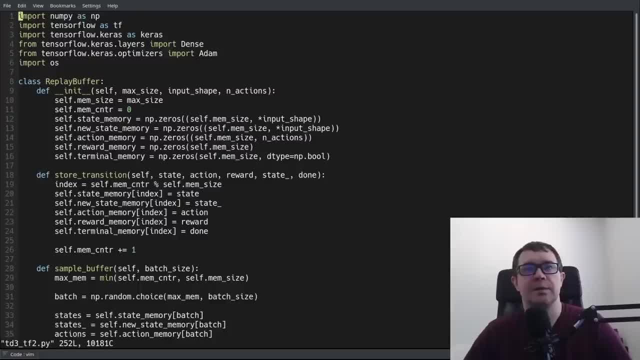 observation underscore and done okay. observation underscore and done okay. and then I got to get rid of the print and then I got to get rid of the print and then I got to get rid of the print statements. I stuck in here for debug statements. I stuck in here for debug. 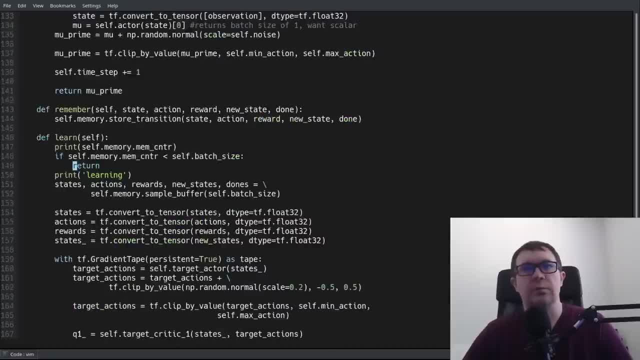 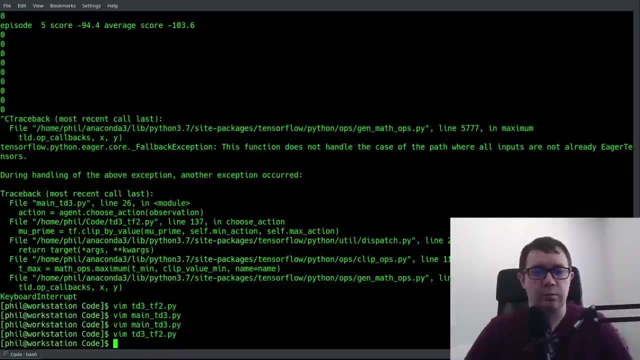 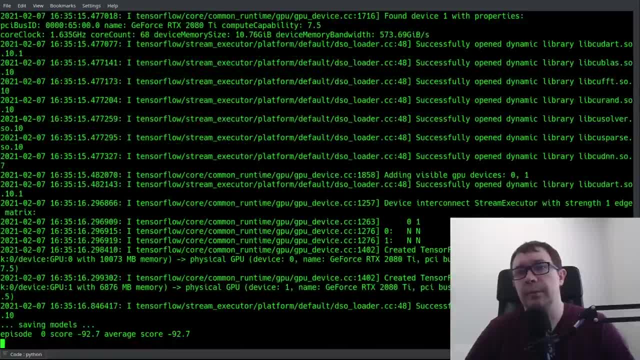 now let's do Python main td3 dot PI. now let's do Python main td3 dot PI. and now it should work without any funky. and now it should work without any funky. and now it should work without any funky. print statements. okay, now I'm gonna take 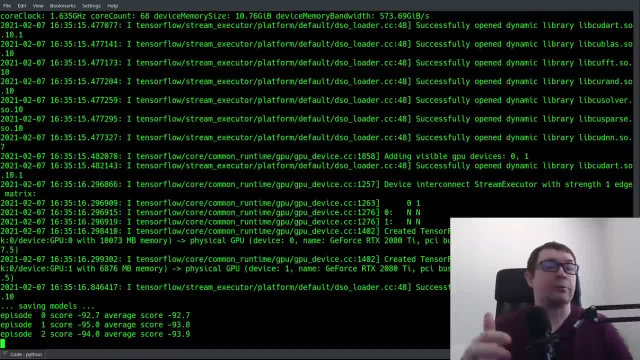 print statements. okay, now I'm gonna take print statements. okay, now I'm gonna take off for a little bit and see what's off for a little bit, and see what's off for a little bit and see what's going on and the reason I noticed this. 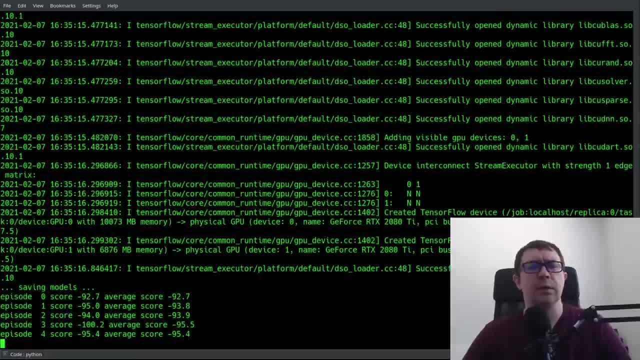 going on, and the reason I noticed this going on and the reason I noticed this wasn't learning is because it was wasn't learning- is because it was wasn't learning is because it was executing much too quickly. I blasted executing much too quickly. I blasted executing much too quickly. I blasted through 350 games in just about a minute. 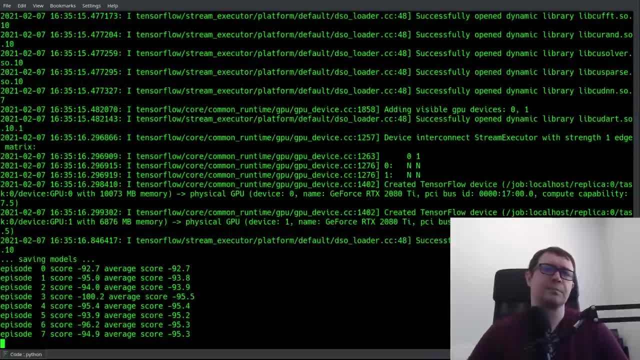 through 350 games in just about a minute. through 350 games in just about a minute. which tells me it's not doing anything. which tells me it's not doing anything. which tells me it's not doing anything useful in the GPU. so I'm not this run. 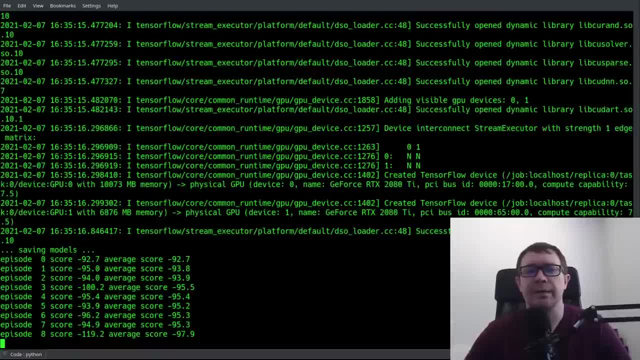 useful in the GPU, so I'm not this run useful in the GPU, so I'm not this run. that'll probably take an hour or two and that'll probably take an hour or two, and that'll probably take an hour or two, and I'm gonna come back and see how it did. 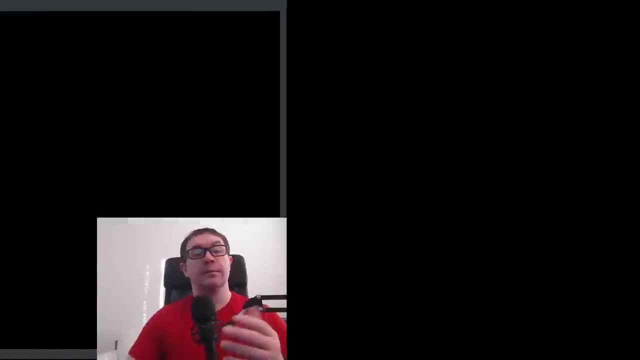 I'm gonna come back and see how it did. I'm gonna come back and see how it did and we'll take a look at its performance, and we'll take a look at its performance and we'll take a look at its performance. now, here we are. it's the next morning. 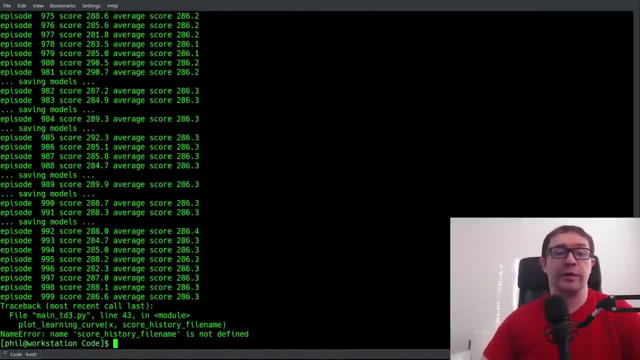 now, here we are. it's the next morning. now, here we are. it's the next morning. this took around six or seven hours to. this took around six or seven hours to. this took around six or seven hours to run, so I just waited until morning to run. so I just waited until morning to. 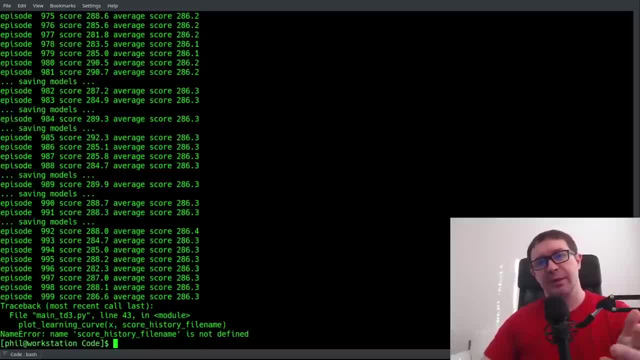 run, so I just waited until morning to film this. but in typical Phil style, the film this. but in typical Phil style, the film this. but in typical Phil style, the file name for the. the function call for file name for the. the function call for file name for the. the function call for the plot. learning curve function has a. 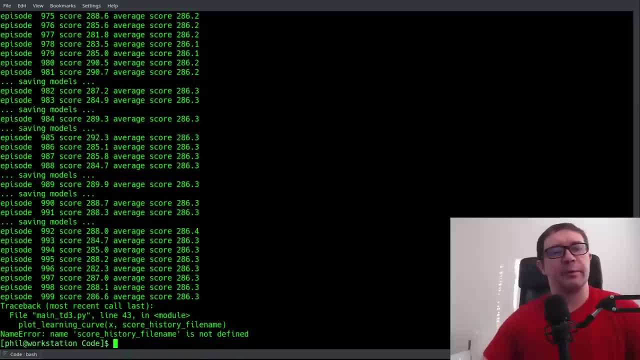 the plot learning curve function has a. the plot learning curve function has a typo in it, and so we don't have an typo in it. and so we don't have an typo in it, and so we don't have an actual plot from the performance of this. 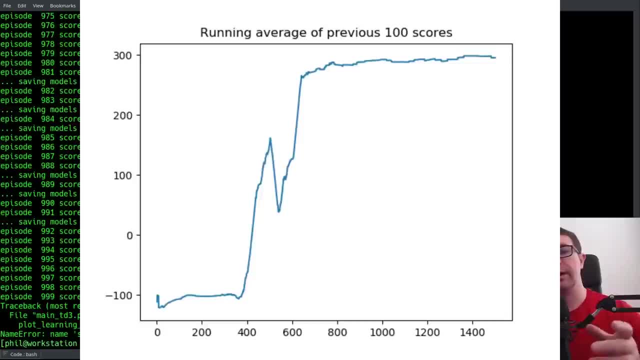 actual plot, from the performance of this actual plot, from the performance of this particular run. however, I will show you a particular run. however, I will show you a particular run. however, I will show you a plot of a similar run where it. plot of a similar run where it. 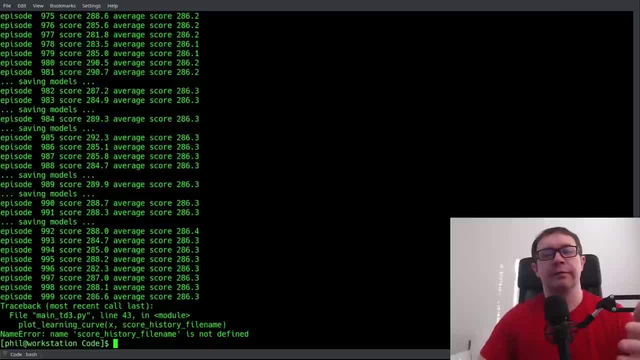 plot of a similar run, where it achieved an approximately similar score, achieved an approximately similar score. achieved an approximately similar score. you can see that it does indeed learn it. you can see that it does indeed learn it. you can see that it does indeed learn. it achieves a high score of around 285 288. 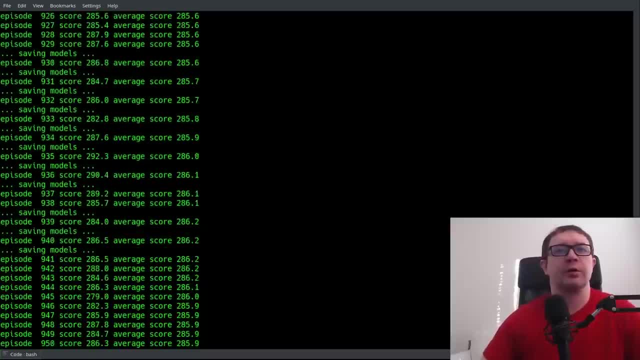 achieves a high score of around 285- 288. achieves a high score of around 285- 288- about 290 or so, depending on the run. you about 290 or so, depending on the run. you about 290 or so, depending on the run. you get some run to run, variation and 300. 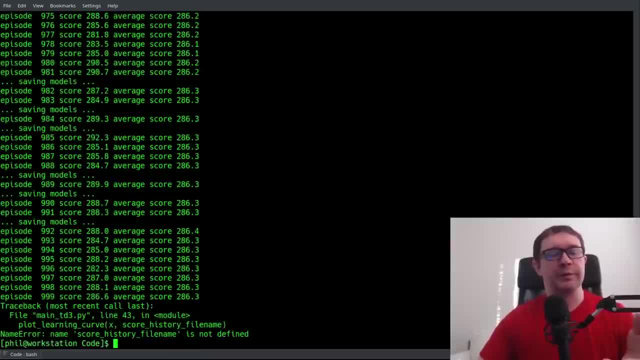 get some run to run variation and 300. get some run to run variation and 300 is the highest possible score you can get. is the highest possible score you can get. is the highest possible score you can get for this environment, so I would for this environment, so I would. 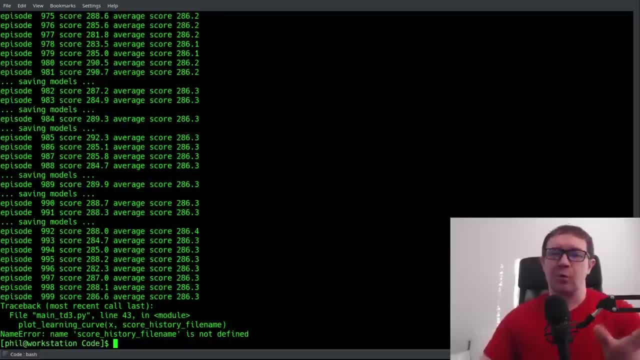 for this environment. so I would consider this pretty much strong evidence. consider this pretty much strong evidence. consider this pretty much strong evidence of learning. it's not a world-class of learning. it's not a world-class of learning. it's not a world-class result. but that's not what we were. result, but that's not what we were result, but that's not what we were aiming for anyway. we just wanted to aiming for anyway. we just wanted to aiming for anyway. we just wanted to understand the gist of the algorithm and understand the gist of the algorithm, and 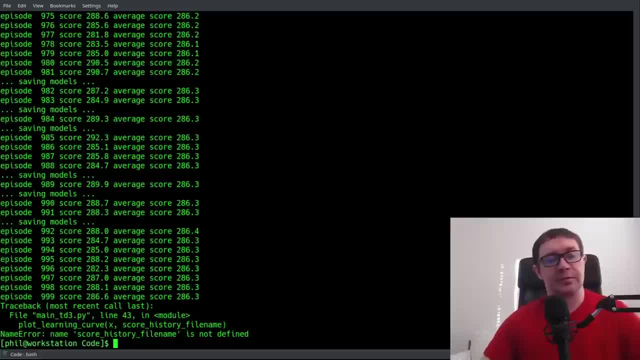 understand the gist of the algorithm and implement it correctly, and demonstrate implement it correctly. and demonstrate implement it correctly and demonstrate that we do in fact understand how it, that we do in fact understand how it, that we do in fact understand how it works. mission accomplished. you can pat. 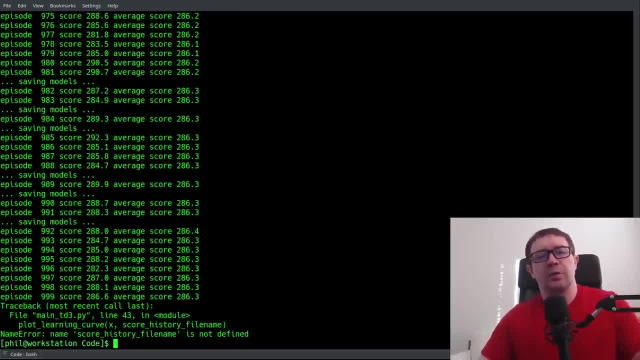 works, mission accomplished. you can pat works- mission accomplished. you can pat yourself on the back. for that, I'll also yourself on the back. for that, I'll also yourself on the back. for that. I'll also show you some footage of the Walker kind. show you some footage of the Walker kind. 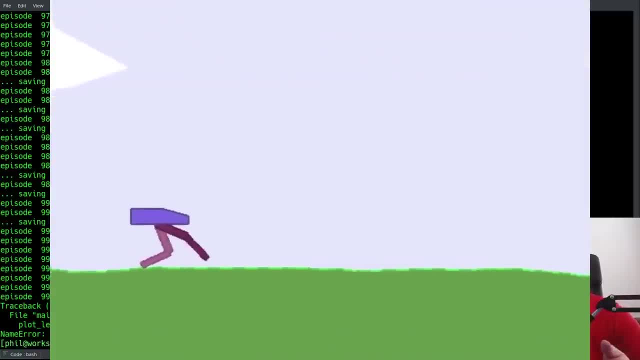 show you some footage of the Walker kind of stumbling along so you can see how it of stumbling along. so you can see how it of stumbling along, so you can see how it looks once it's fully trained you can. looks, once it's fully trained, you can. 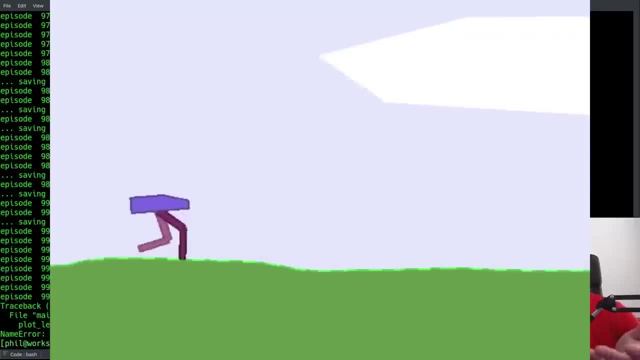 looks. once it's fully trained you can see it has kind of a funny gate, but it see it has kind of a funny gate. but it see it has kind of a funny gate, but it does in fact manage to learn to walk, does in fact manage to learn to walk. 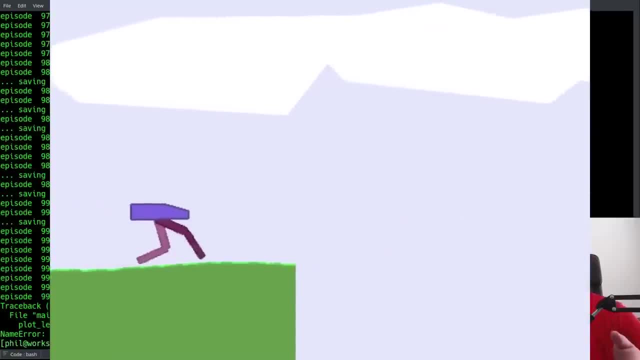 does in fact manage to learn to walk. that is pretty impressive. starting from that is pretty impressive. starting from that is pretty impressive. starting from just totally random actions. learning how, just totally random actions. learning how to walk within just six or seven hours, to walk within just six or seven hours. 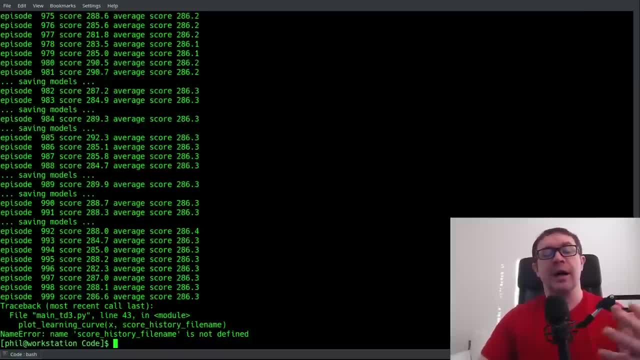 to walk within just six or seven hours. of only humans were so competent. I hope of only humans were so competent. I hope of only humans were so competent. I hope that was helpful. leave a comment down that was helpful. leave a comment down that was helpful. leave a comment down below with any questions, suggestions. 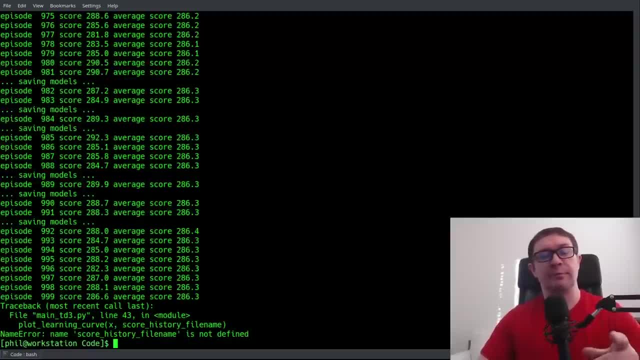 below with any questions. suggestions. below with any questions, suggestions. anything you'd like to see next? give a anything you'd like to see next. give a anything you'd like to see next. give a thumbs up a subscribe if you haven't. thumbs up a subscribe if you haven't. 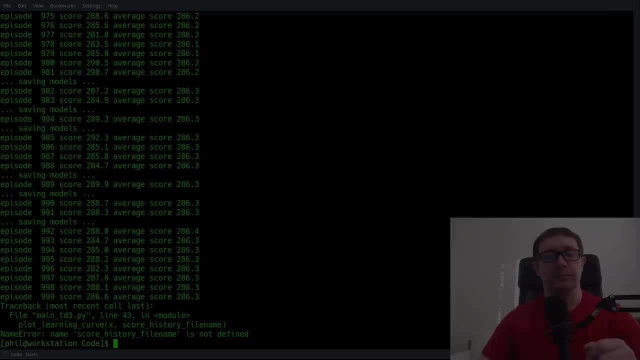 thumbs up a subscribe if you haven't already, and I'll see you in the next. already, and I'll see you in the next. already, and I'll see you in the next video. welcome to a crash course and video. welcome to a crash course and video. welcome to a crash course and proxmo policy optimization. before we. 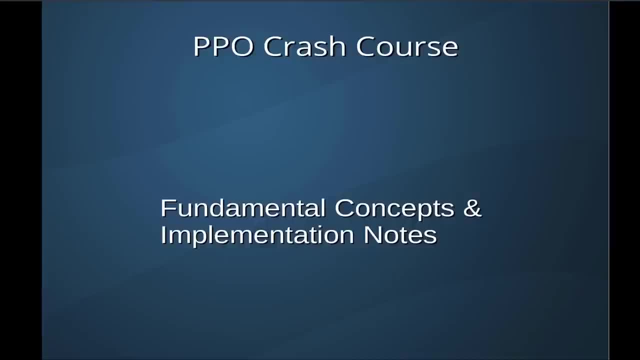 proxmo policy optimization. before we proxmo policy optimization, before we begin a quick shameless plug, my udemy. begin a quick shameless plug, my udemy. begin a quick shameless plug my udemy. courses on deep reinforcement learning, courses on deep reinforcement learning. courses on deep reinforcement learning, specifically actor critic methods and 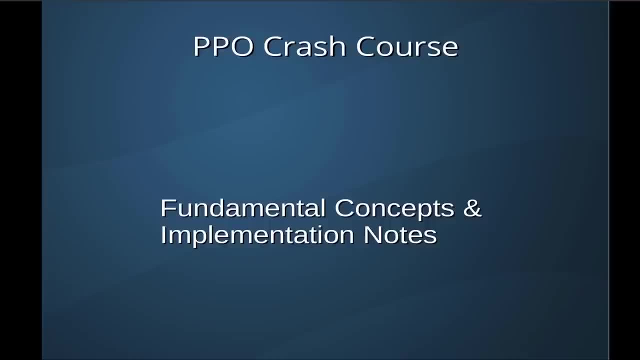 specifically actor critic methods and specifically actor critic methods and deep Q learning are on sale right now. deep Q learning are on sale right now. deep Q learning are on sale right now. learn how to turn papers into code link. learn how to turn papers into code link. learn how to turn papers into code link in the description below, so proximal. 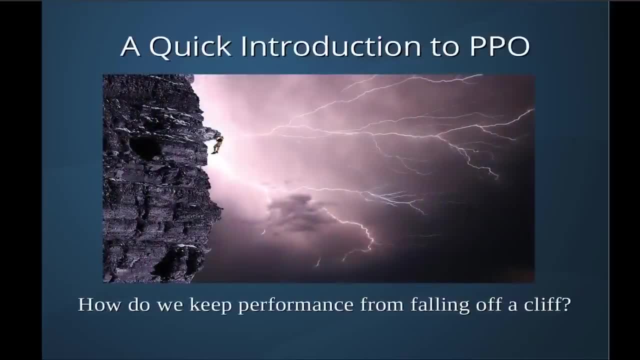 in the description below, so proximal in the description below, so proximal. policy optimization, or PPO for short, was policy optimization or PPO for short, was policy optimization or PPO for short. was created for a pretty simple reason, and created for a pretty simple reason, and 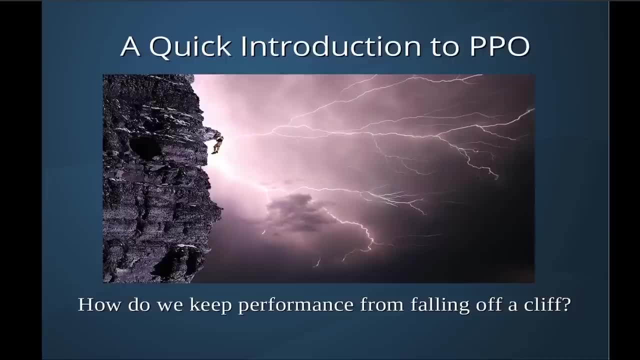 created for a pretty simple reason and that is that in actor critic methods, that is that in actor critic methods, that is that in actor critic methods, oftentimes we see that the performance, oftentimes we see that the performance, oftentimes we see that the performance can fall off a cliff, the agent will be. can fall off a cliff. the agent will be can fall off a cliff. the agent will be doing really well for a little while and doing really well for a little while and doing really well for a little while and suddenly an update to the neural network. suddenly an update to the neural network. 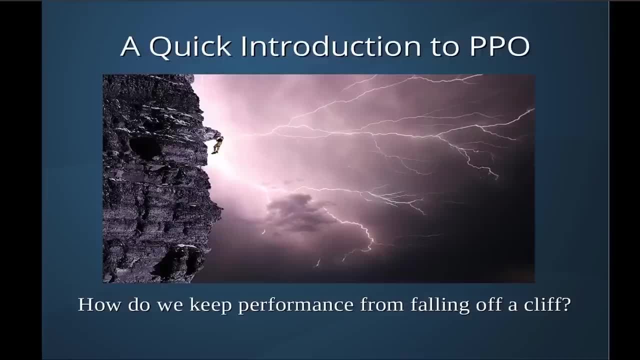 suddenly, an update to the neural network will cause the agent to simply lose its, will cause the agent to simply lose its, will cause the agent to simply lose its its understanding of how to play the game, its understanding of how to play the game, its understanding of how to play the game, and so performance tanks, and never 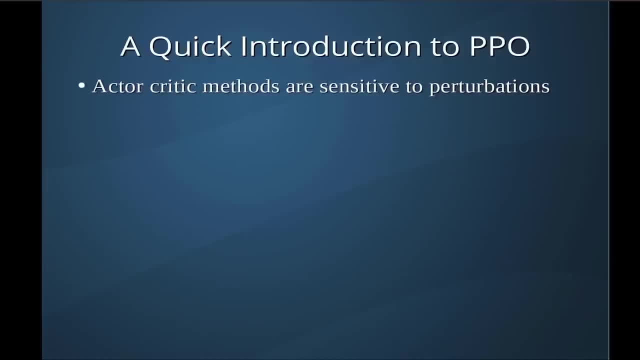 and so performance tanks and never and so performance tanks and never really recovers. now this happens because really recovers. now this happens because really recovers. now this happens because actor critic methods are incredibly. actor critic methods are incredibly. actor critic methods are incredibly sensitive to perturbations. the reason: 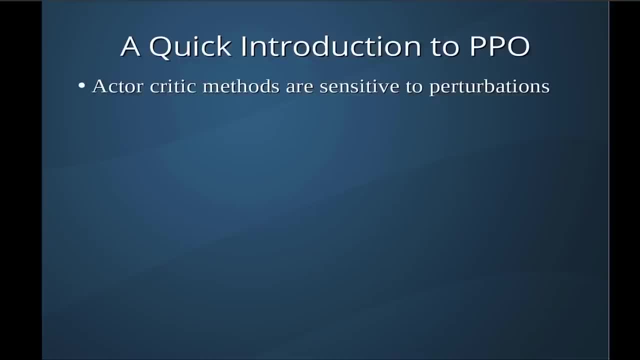 sensitive to perturbations, the reason sensitive to perturbations? the reason being that small changes in the being, that small changes in the being, that small changes in the underlying parameters to our deep neural underlying parameters to our deep neural underlying parameters to our deep neural network- the weights, for instance- can 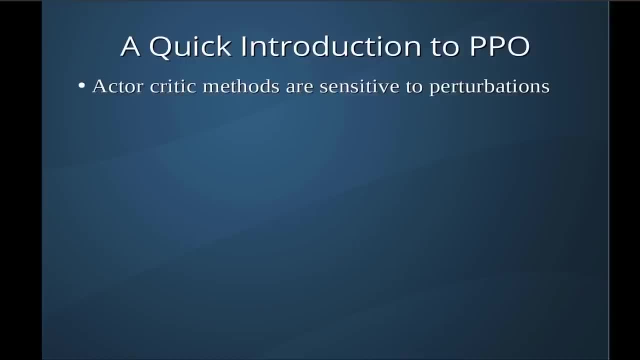 network the weights, for instance, can network the weights, for instance, can cause large jumps in policy space and so cause large jumps in policy space and so cause large jumps in policy space, and so you can go from a region of policy space. you can go from a region of policy space. 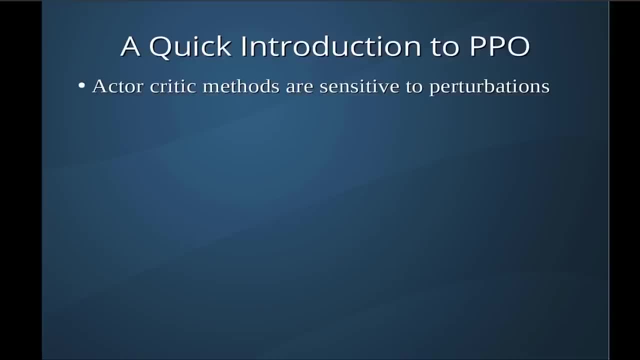 you can go from a region of policy space where performance is good to a region of where performance is good, to a region of where performance is good, to a region of policy space. or performance is bad, just policy space. or performance is bad, just policy space. or performance is bad just by a small tweak to the underlying. 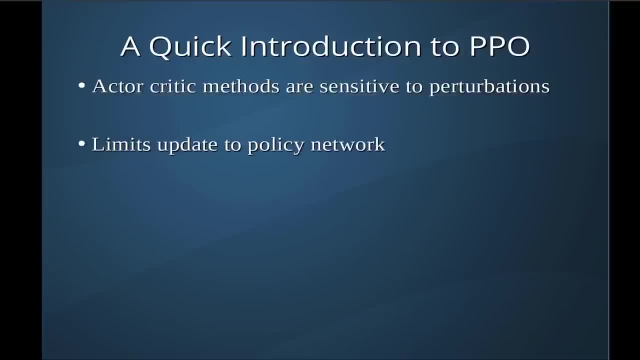 by a small tweak to the underlying, by a small tweak to the underlying parameters of your deep neural network, parameters of your deep neural network, parameters of your deep neural network. PPO addresses this by limiting the PPO addresses this by limiting the PPO addresses this by limiting the updates to the policy network it has a. 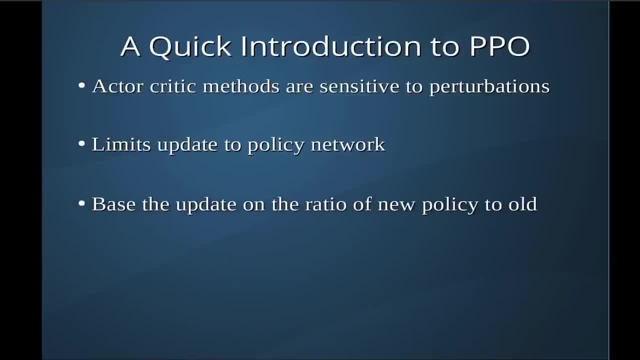 updates to the policy network. it has a updates to the policy network. it has a number of mechanisms for doing this, but number of mechanisms for doing this, but number of mechanisms for doing this. but the basic idea is that we're gonna base. the basic idea is that we're gonna base. 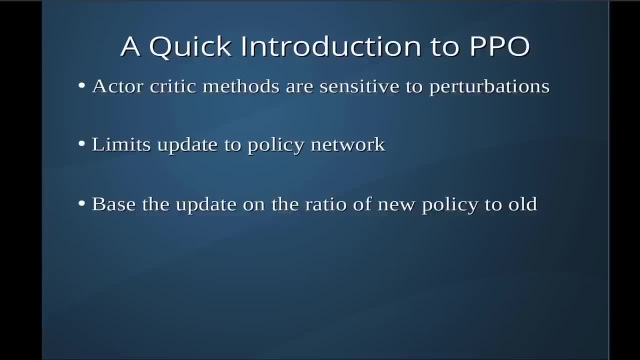 the basic idea is that we're gonna base the updated each step on the ratio of the updated each step, on the ratio of the updated each step, on the ratio of the new policy to the old and we're the new policy to the old and we're. 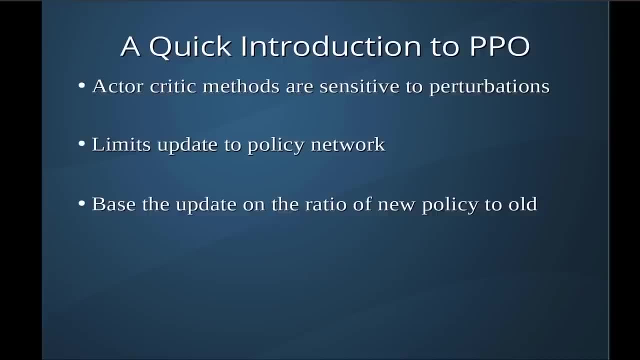 the new policy to the old and we're gonna constrain that ratio to be within a, gonna constrain that ratio to be within, a, gonna constrain that ratio to be within a specific range to make sure we're not specific range, to make sure we're not specific range, to make sure we're not taking really huge steps in parameter. 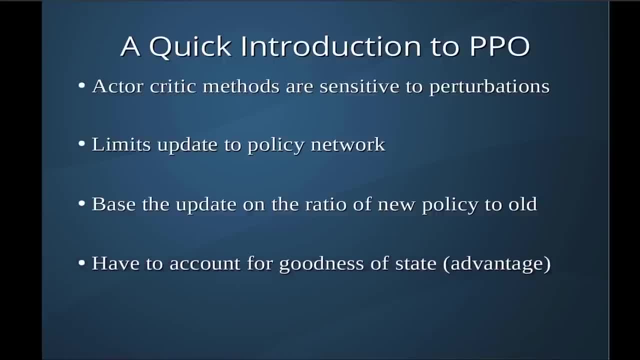 taking really huge steps in parameter, taking really huge steps in parameter space for our deep neural network of space, for our deep neural network of space, for our deep neural network. of course, we also have to account for the course. we also have to account for the course. we also have to account for the goodness of state, in other words, the. 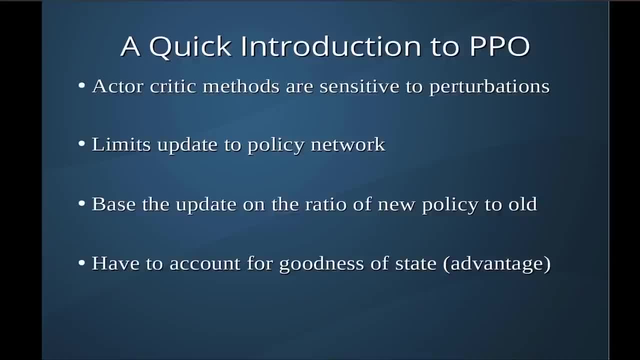 goodness of state, in other words, the goodness of state, in other words the advantage- how valuable each state is, and advantage, how valuable each state is, and advantage, how valuable each state is, and the reason being naturally that we, the reason being naturally that we, the reason being naturally that we want the agent to select states that are: 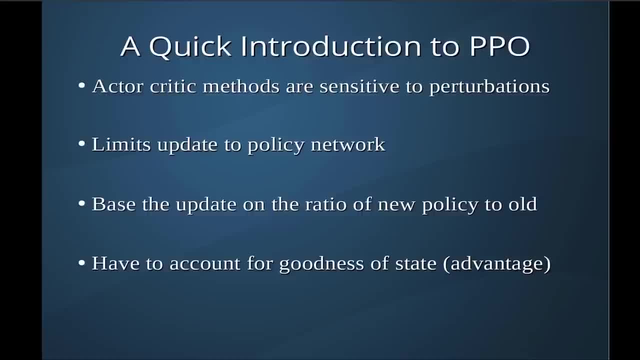 want the agent to select states that are. want the agent to select states that are highly profitable to it over time. so it highly profitable to it over time. so it highly profitable to it over time. so it wants to find the best possible states. wants to find the best possible states. 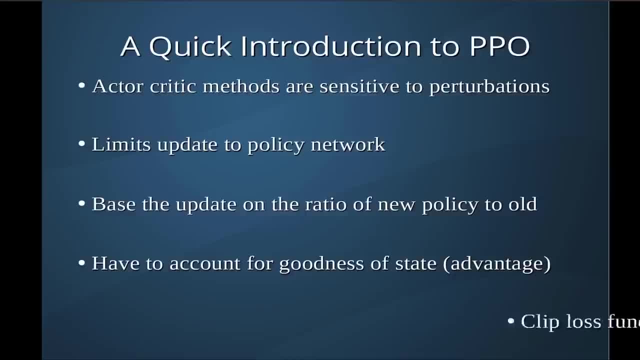 wants to find the best possible states, now taking into account the advantage, now taking into account the advantage, now taking into account the advantage can cause the the loss function to grow. a can cause the the loss function to grow. a can cause the the loss function to grow a little bit too large, and so we're going. 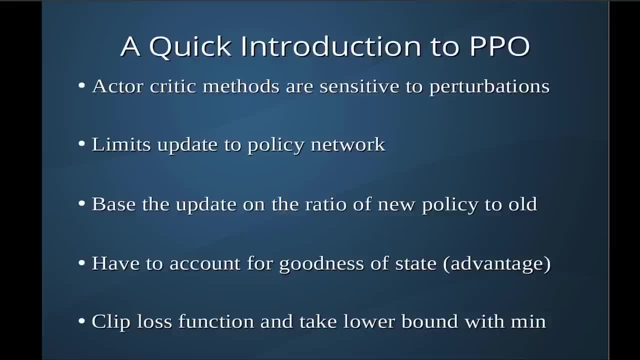 little bit too large and so we're going little bit too large and so we're going to be introducing a way of dealing with, to be introducing a way of dealing with, to be introducing a way of dealing with that by clipping the loss function and that by clipping the loss function, and 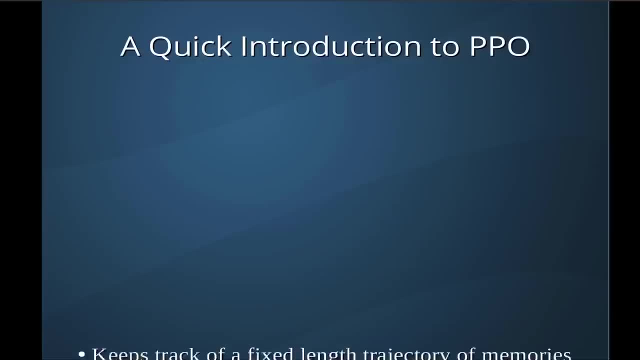 that by clipping the loss function and taking the lower bound with the minimum, taking the lower bound with the minimum, taking the lower bound with the minimum function. something else we're going to function. something else we're going to function. something else we're going to be doing that's different than what you. 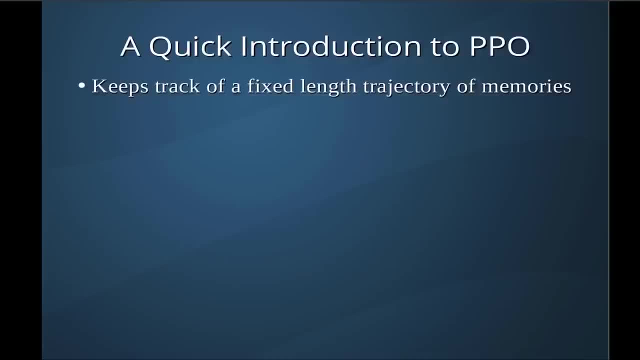 be doing. that's different than what you be doing. that's different than what you may be used to. is that, instead of may be used to? is that instead of may be used to? is that, instead of keeping track of something like, say, a, keeping track of something like, say, a. 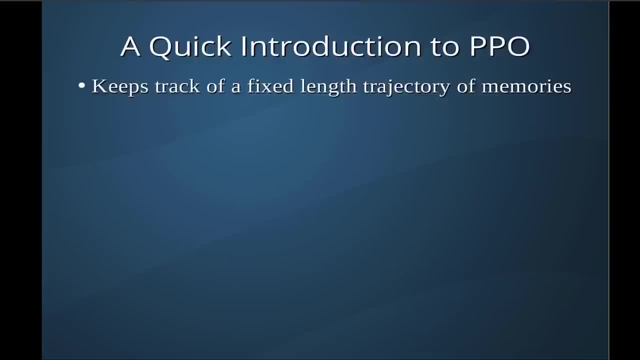 keeping track of something like, say, a million transitions and then sampling a million transitions, and then sampling a million transitions and then sampling a subset of those at random. we're going subset of those at random. we're going subset of those at random. we're going to be keeping a very small fixed length. 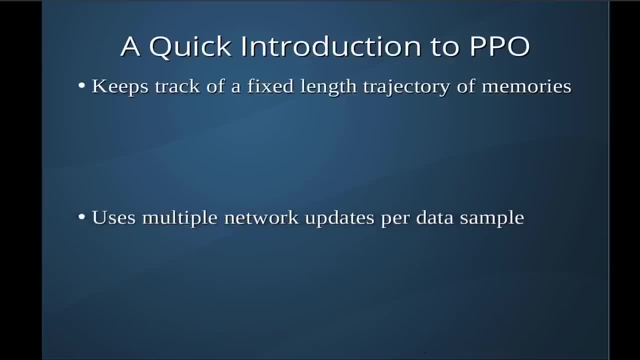 to be keeping a very small fixed length, to be keeping a very small fixed length, trajectory of memories. and we're going trajectory of memories and we're going trajectory of memories and we're going to be doing multiple network updates per to be doing multiple network updates per. 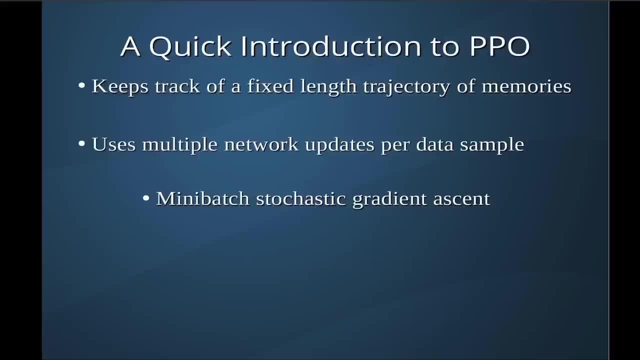 to be doing multiple network updates per data sample. using mini batch stochastic data sample. using mini batch stochastic data sample. using mini batch stochastic gradient descent: it's worth noting that gradient descent. it's worth noting that gradient descent. it's worth noting that you can also use multiple parallel. 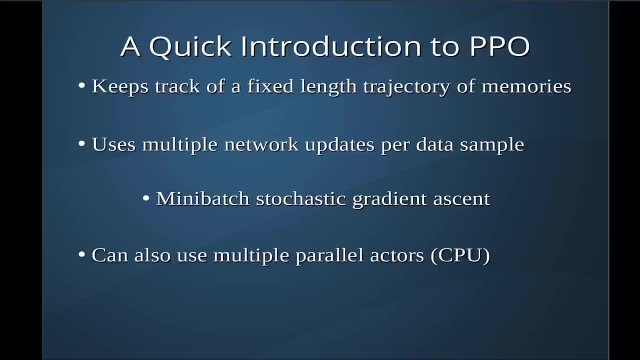 you can also use multiple parallel. you can also use multiple parallel actors on the CPU, something like what actors on the CPU? something like what actors on the CPU? something like what you would do in a3c, but we're not going. you would do in a3c, but we're not going. you would do in a3c, but we're not going to deal with that in this particular. to deal with that in this particular, to deal with that in this particular tutorial. I'm just going to show you how tutorial. I'm just going to show you how. 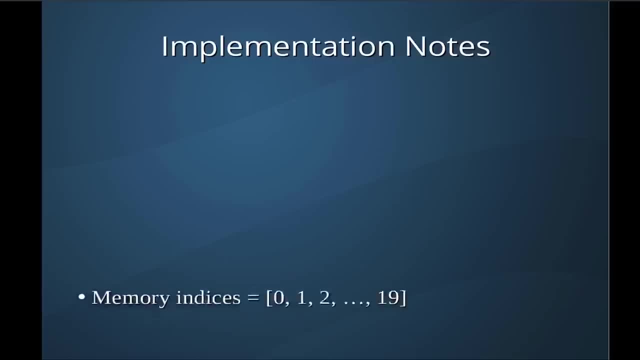 tutorial. I'm just going to show you how to do the GPU implementation. so let's to do the GPU implementation. so let's to do the GPU implementation. so let's talk about the mini batch gradient. talk about the mini batch gradient. talk about the mini batch gradient. descent for a second. so we're gonna keep. 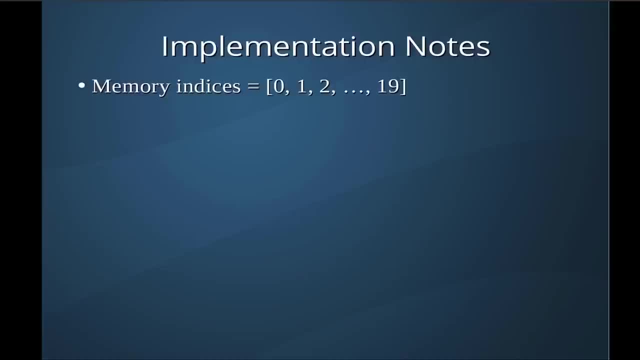 descent for a second. so we're gonna keep descent for a second. so we're gonna keep track of a list of memory indices from track, of a list of memory indices, from track of a list of memory indices from, say, 0 to 19, and that's for the case of. 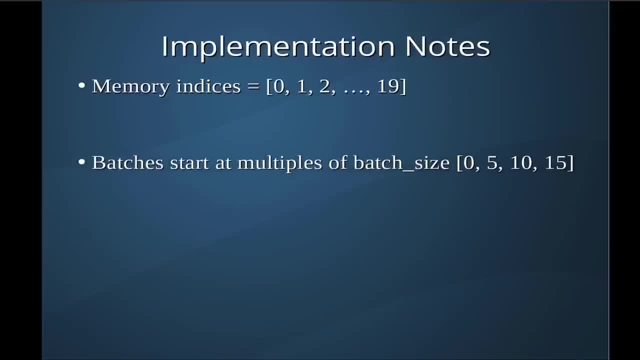 say, 0 to 19, and that's for the case of track, of a list of memory indices from, say, 0 to 19, and that's for the case of taking a look at 20 transitions, and let's taking a look at 20 transitions, and let's 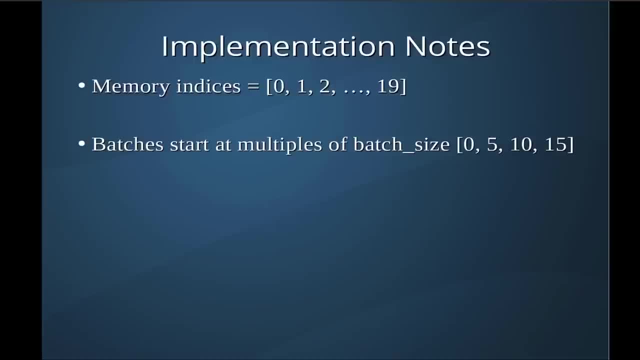 taking a look at 20 transitions and let's say we want to take a batch of size 5, say we want to take a batch of size 5, say we want to take a batch of size 5, and so those batches could start at, and so those batches could start at. 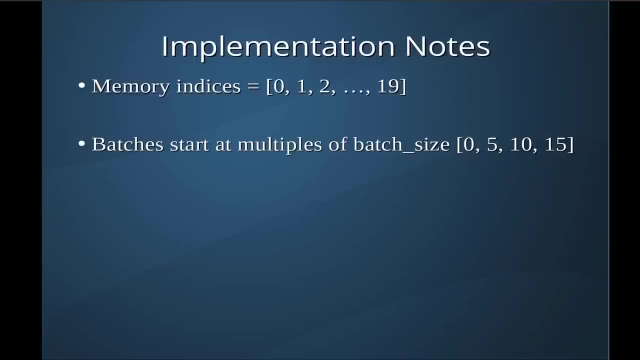 and so those batches could start at position 0, 5, 10 or 15. those are the only position: 0, 5, 10 or 15. those are the only position: 0, 5, 10 or 15. those are the only possible positions for it to start such. 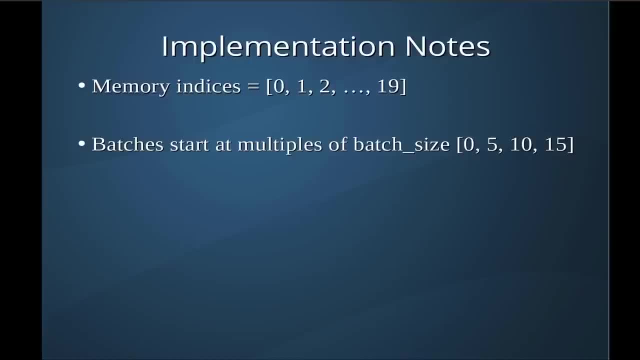 possible positions for it to start, such possible positions for it to start, such that you get all the memories you don't that you get all the memories. you don't that you get all the memories, you don't get any overlap, and that it all works. get any overlap and that it all works. 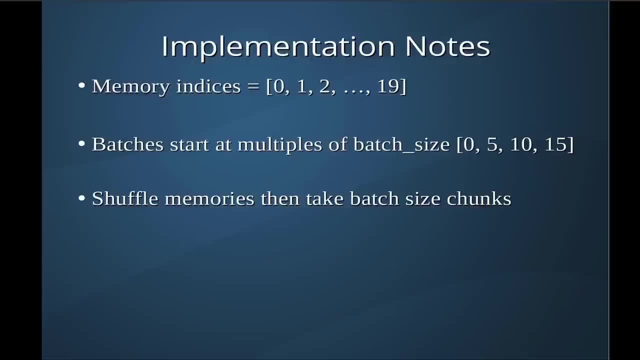 get any overlap and that it all works for five up to nine is the next batch, for five up to nine is the next batch, for five up to nine is the next batch, and so on and so forth. it's relatively, and so on and so forth. it's relatively. 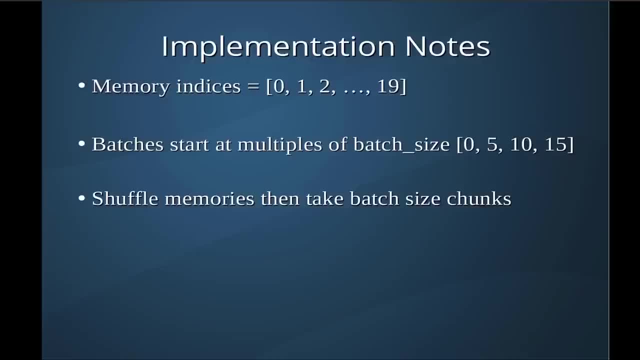 and so on and so forth. it's relatively straightforward when you see it in code, straightforward when you see it in code, straightforward when you see it in code, but it's kind of difficult to explain as but it's kind of difficult to explain as but it's kind of difficult to explain as you're coding it. so just know that we're. 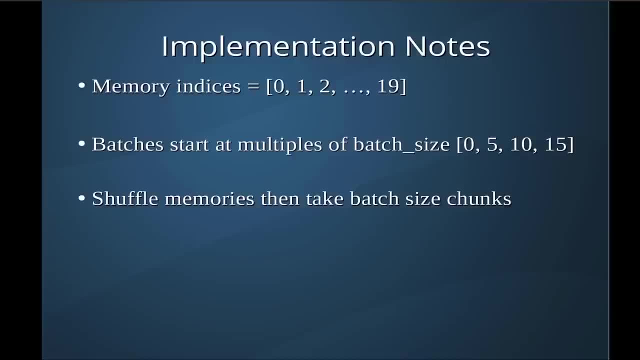 you're coding it, so just know that we're. you're coding it, so just know that we're taking back size chunks of shuffled. taking back size chunks of shuffled. taking back size chunks of shuffled. memories for a mini batch. stochastic memories for a mini batch. stochastic memories for a mini batch: stochastic gradient: ascent. 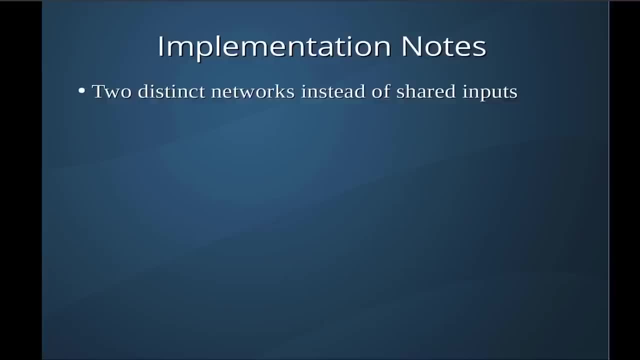 gradient ascent. gradient ascent- other things we need to know. is that other things we need to know is that other things we need to know is that we're going to be using two distinct. we're going to be using two distinct. we're going to be using two distinct networks for our actor and our critic. 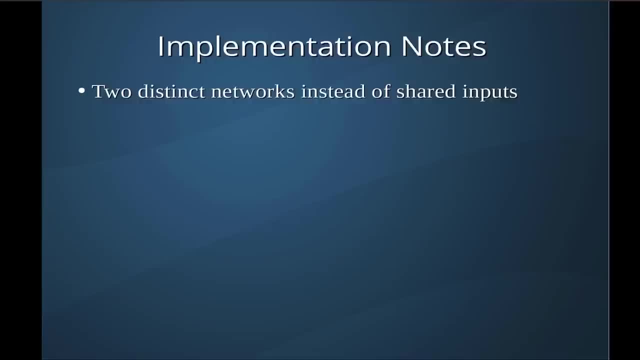 networks for our actor and our critic. networks for our actor and our critic. instead of having a single network with. instead of having a single network with. instead of having a single network with shared inputs and multiple outputs, shared inputs and multiple outputs, shared inputs and multiple outputs. now, you certainly can use a shared 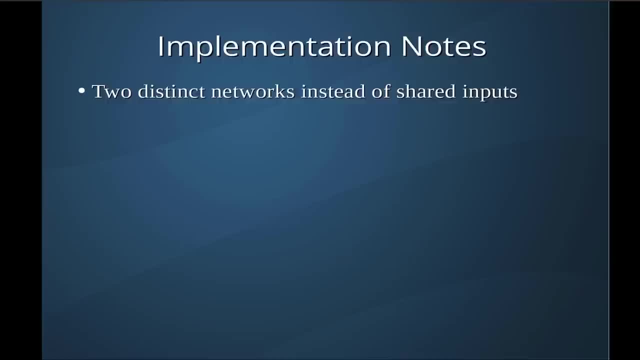 now you certainly can use a shared. now you certainly can use a shared input with multiple outputs, but it input with multiple outputs, but it input with multiple outputs but it complicates the loss function a little, complicates the loss function a little, complicates the loss function a little bit and i found that performance is. 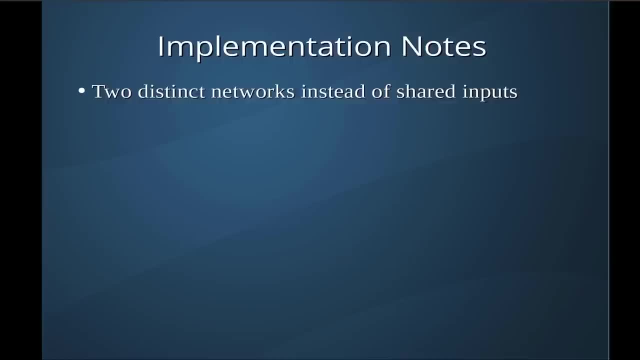 bit and i found that performance is bit and i found that performance is generally adequate with two distinct. generally adequate with two distinct. generally adequate with two distinct: networks for simple environments: networks for simple environments, networks for simple environments. so the critic will evaluate the states. so the critic will evaluate the states. 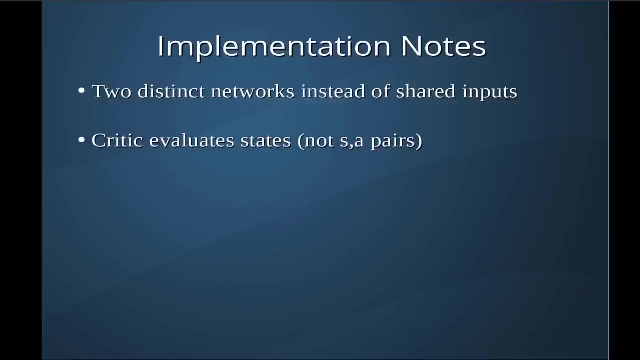 so the critic will evaluate the states of the agent encounters, of the agent encounters, of the agent encounters. and it gets the name critic because it and it gets the name critic because it and it gets the name critic because it literally criticizes the decisions that literally criticizes the decisions that. 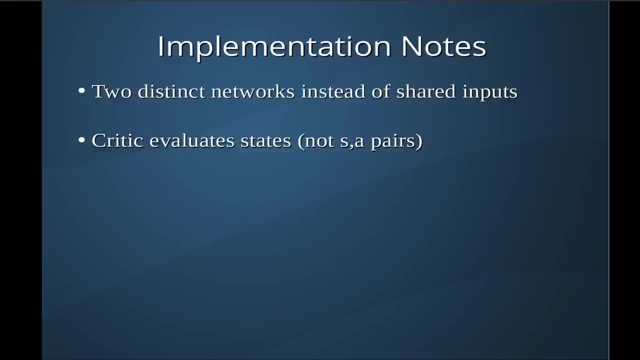 literally criticizes the decisions that the actor makes based on which states it the actor makes. based on which states it the actor makes, based on which states it ends up in. so it says hey, ends up in. so it says hey, ends up in. so it says hey, this particular state was valuable. we 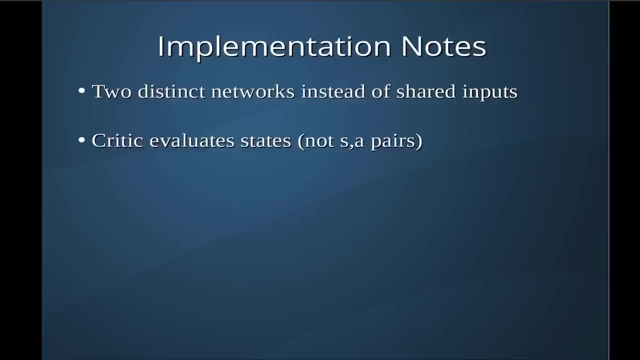 this particular state was valuable. we, this particular state was valuable. we did good or this state is stupid. we did, did good or this state is stupid. we did, did good or this state is stupid. we did bad. do better, next time bad. do better, next time bad. do better next time now. this is in contrast to state and 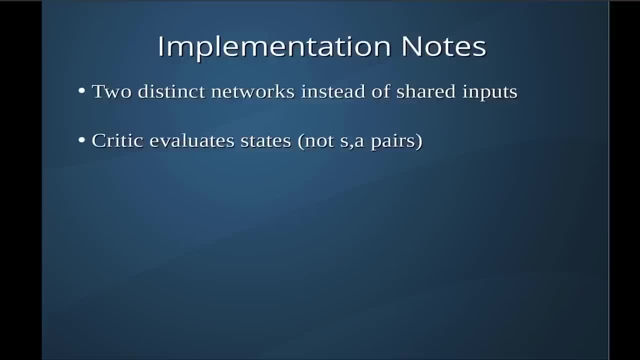 now this is in contrast to state, and now this is in contrast to state and action pairs for something like say deep action pairs for something like say deep action pairs for something like say deep q learning, but it's in line with what q learning? but it's in line with what. 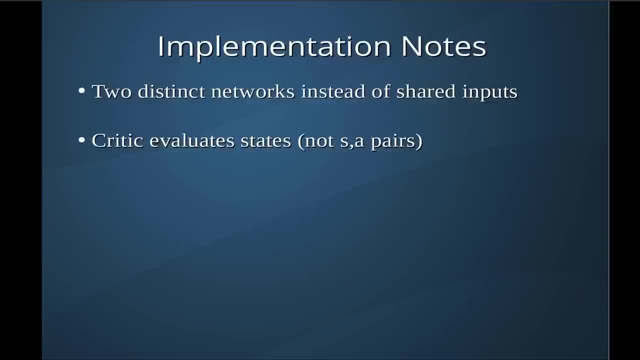 q learning, but it's in line with what other actor critic methods use and of course, the actor decides what to. and of course the actor decides what to. and of course the actor decides what to do based on its current state. do based on its current state. do based on its current state. so our network is going to output. 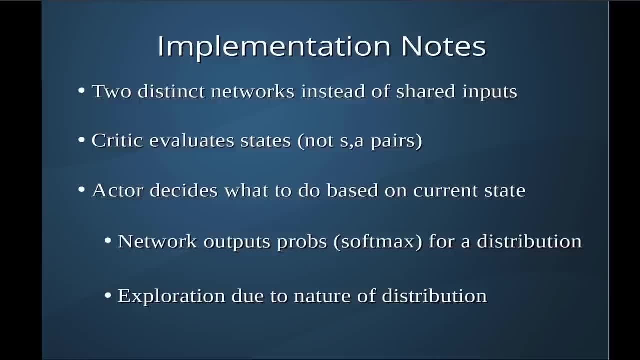 so our network is going to output. so our network is going to output probabilities using a soft max, probabilities using a soft max, probabilities using a soft max activation, and we'll use that for a activation, and we'll use that for a activation, and we'll use that for a categorical distribution and pi torch. 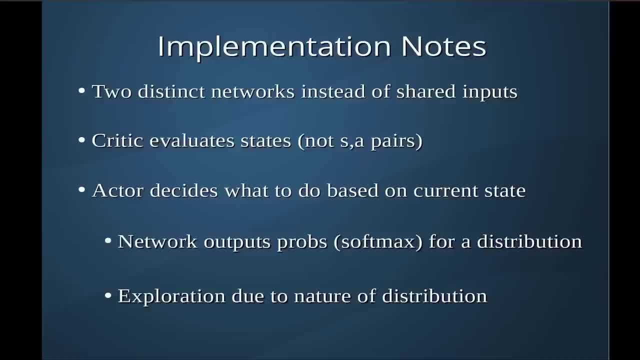 categorical distribution and pi torch. categorical distribution and pi torch. so we'll have, in the case of the cart, so we'll have in the case of the cart, so we'll have, in the case of the cart, pull we'll have a couple actions. pull we'll have a couple actions. 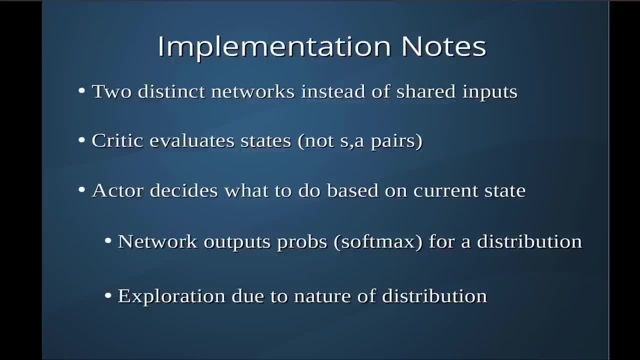 pull. we'll have a couple actions and some probabilities selecting each and some probabilities selecting each and some probabilities selecting each action, and then we will use the action and then we will use the action and then we will use the probabilities determined by our deep, probabilities determined by our deep. 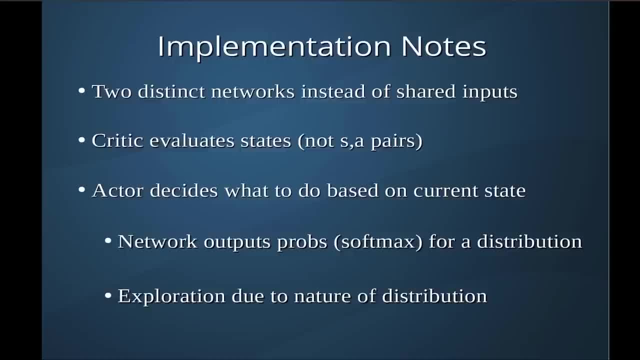 probabilities determined by our deep neural network to feed into a neural network. to feed into a neural network, to feed into a distribution that we can sample and use, distribution that we can sample and use, distribution that we can sample and use for the calculation of the log. for the calculation of the log. 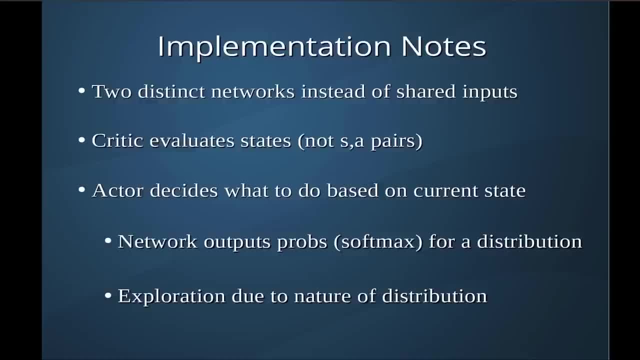 for the calculation of the log probabilities. more on that momentarily probabilities- more on that momentarily probabilities- more on that momentarily. it's also worth noting that exploration- it's also worth noting that exploration- it's also worth noting that exploration is going to be taken care of for us due. 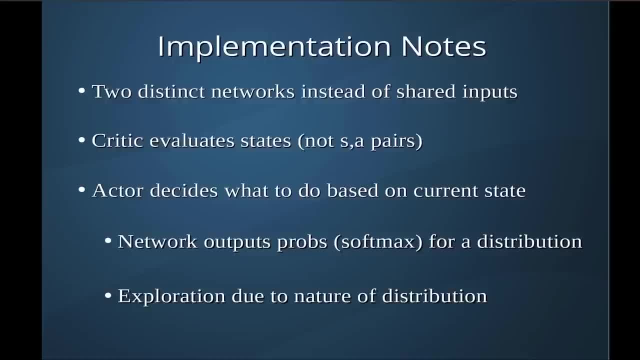 is going to be taken care of for us. due is going to be taken care of for us due to the fact that we're using a, to the fact that we're using a to the fact that we're using a distribution, so it's probabilistic and. 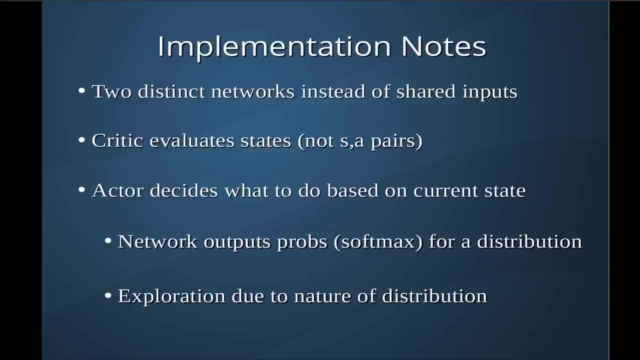 distribution, so it's probabilistic, and distribution, so it's probabilistic, and it's set up so that each element has it's set up, so that each element has it's set up so that each element has some finite probability. so some finite probability, so some finite probability. so, even if the probability of one action 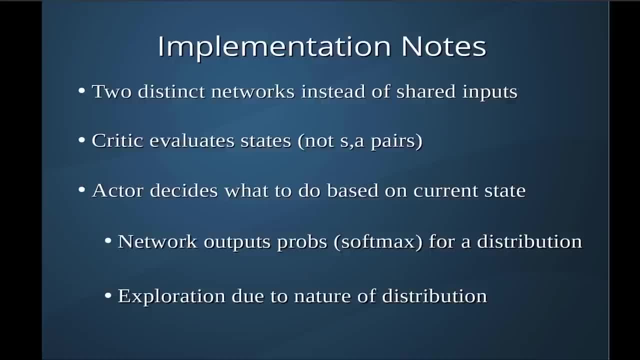 even if the probability of one action, even if the probability of one action goes arbitrarily close to one, goes arbitrarily close to one, goes arbitrarily close to one, the probability selecting the other action, the probability selecting the other action, the probability selecting the other action stays finite, so that at least some of stays finite, so that at least some of stays finite, so that at least some of the time it's going to get some, the time it's going to get some, the time it's going to get some exploration- this is in contrast to exploration. this is in contrast to. 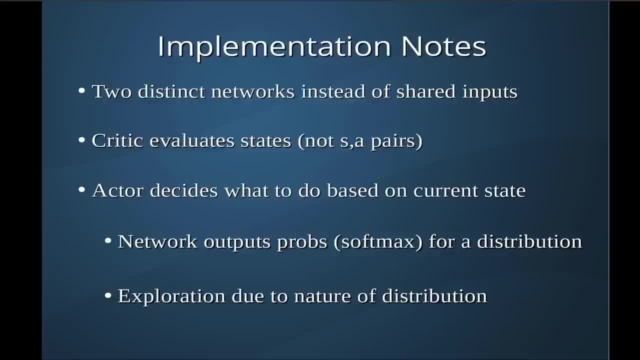 exploration. this is in contrast to something like, say, epsilon greedy action, something like say: epsilon greedy action, something like say: epsilon greedy action. selection and deep q learning: where you selection and deep q learning, where you selection and deep q learning, where you select off, uh off optimal actions about. 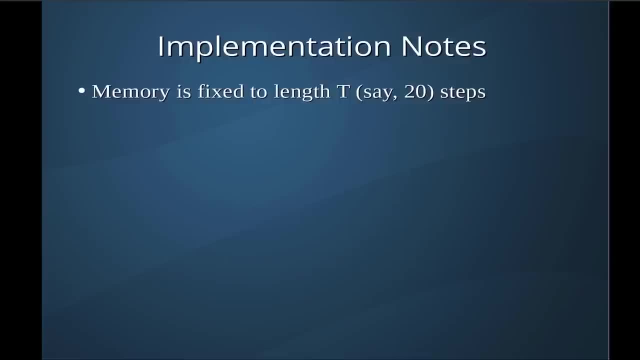 select off, uh off optimal actions. about select off, uh off optimal actions. about ten percent of the time, ten percent of the time, ten percent of the time. as i said earlier, our memory is going to, as i said earlier, our memory is going to. as i said earlier, our memory is going to be fixed to a length of capital t. 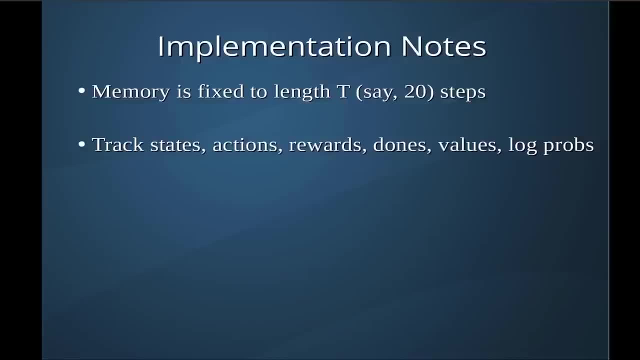 be fixed to a length of capital t be fixed to a length of capital t. in this case, we'll use 20 different steps. in this case, we'll use 20 different steps. in this case, we'll use 20 different steps. we're going to keep track of the states. 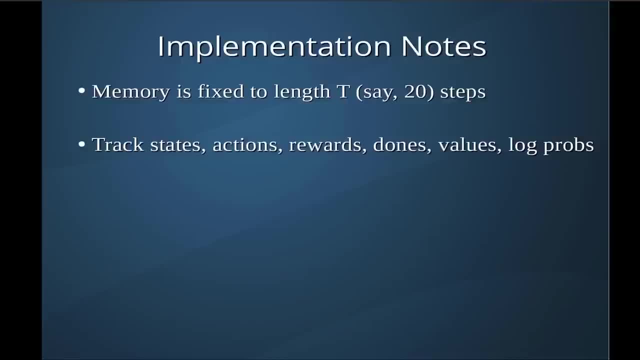 we're going to keep track of the states. we're going to keep track of the states, the agencies, the actions it takes, rewards the agencies. the actions it takes rewards the agencies. the actions it takes, rewards it receives, it receives. it receives the terminal flags, the values of those. 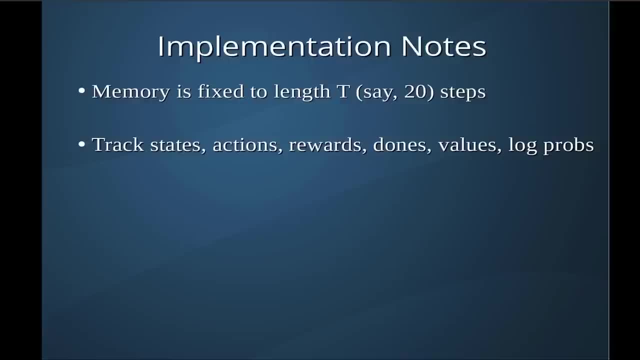 the terminal flags, the values of those the terminal flags, the values of those states according to the critic network states, according to the critic network states, according to the critic network, and the log of the probability of, and the log of the probability of and the log of the probability of selecting those actions that'll become. 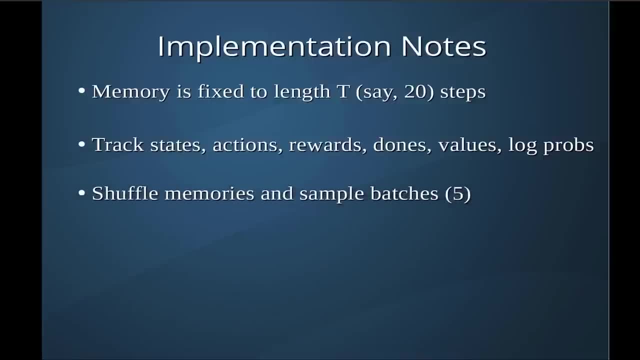 selecting those actions that'll become, selecting those actions that'll become important later in our update rule, important later in our update rule, important later in our update rule. as i said, we're going to shuffle those. as i said, we're going to shuffle those. as i said, we're going to shuffle those memories and sample a batch size of five. 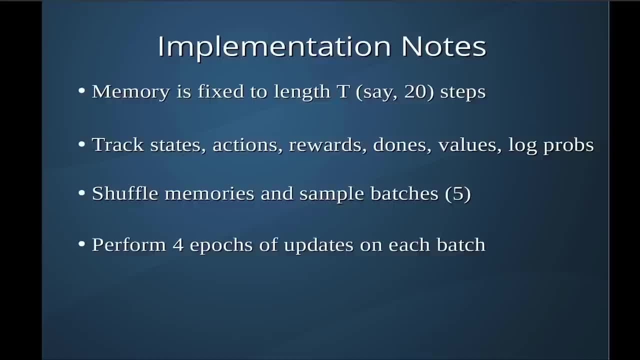 memories and sample a batch size of five memories and sample a batch size of five and we're going to perform four epochs of and we're going to perform four epochs of and we're going to perform four epochs of updates on each batch. updates on each batch. 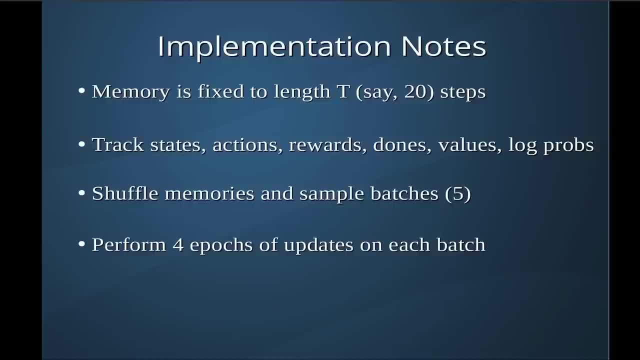 updates on each batch. now these parameters are chosen. now these parameters are chosen. now these parameters are chosen specifically for this particular, specifically for this particular, specifically for this particular environment. and that's one of my environment, and that's one of my environment and that's one of my criticisms of ppo is that there are a 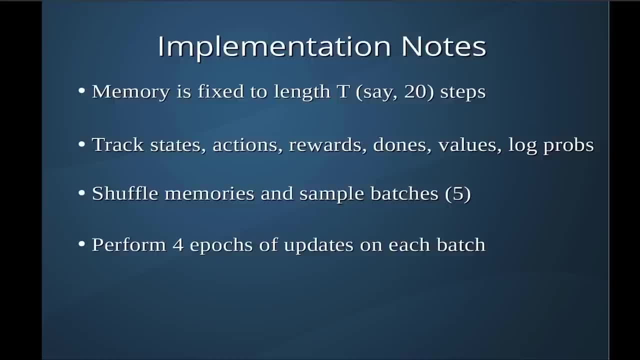 criticisms of ppo is that there are a. criticisms of ppo is that there are a number of parameters to play with number of parameters. to play with number of parameters. to play with hyperparameters. the memory length is hyperparameters. the memory length is hyperparameters. the memory length is one hyperparameter. 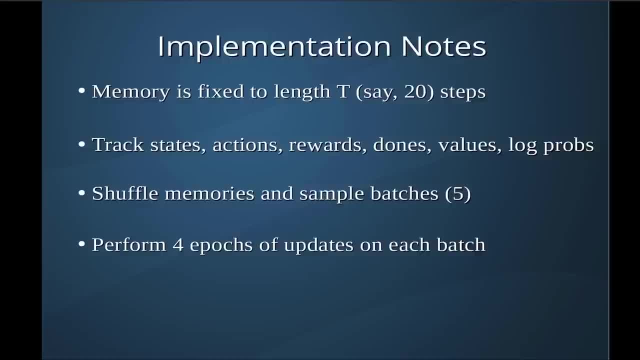 one hyperparameter. one hyperparameter the batch size and number of epochs, as the batch size and number of epochs, as the batch size and number of epochs, as well as learning rate. and another well as learning rate. and another well as learning rate, and another parameter we're going to see later all. 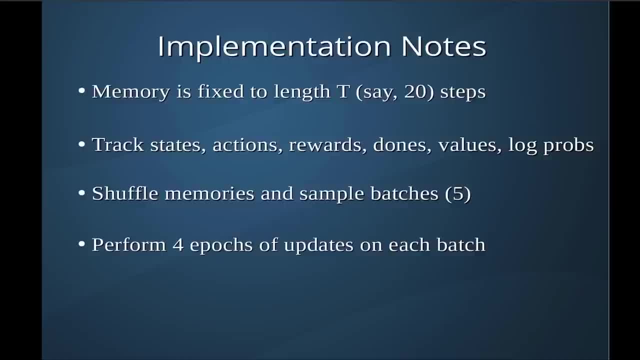 parameter we're going to see later, all parameter we're going to see later, all play roles of hyper parameters in our play. roles of hyper parameters in our play, roles of hyper parameters in our model. and so there is a lot to tune here. model, and so there is a lot to tune here. 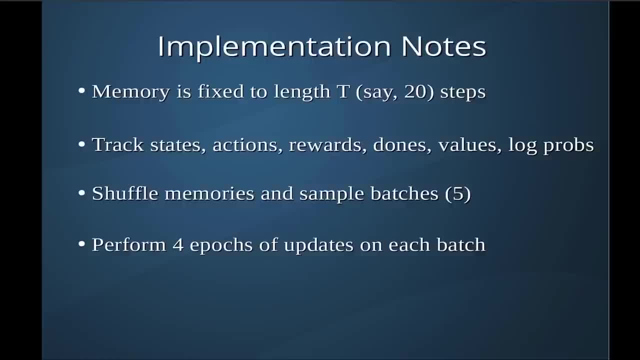 model and so there is a lot to tune here. but these parameters work really well. but these parameters work really well. but these parameters work really well for the um cart pull environment. so you for the um cart pull environment, so you for the um cart pull environment. so you won't have to do any tweaking. 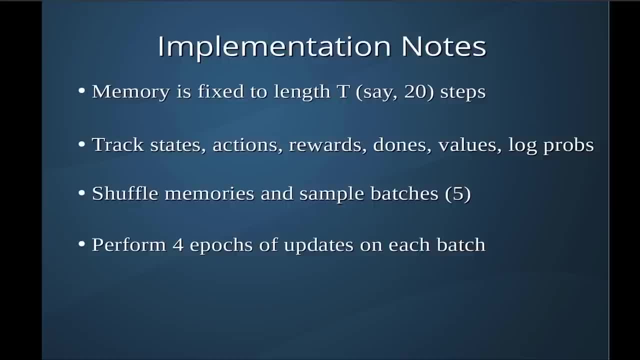 won't have to do any tweaking, won't have to do any tweaking for that other thing to note, for that other thing to note, for that other thing to note is that this memory length capital t is that this memory length capital t is that this memory length capital t should be much less than the length of 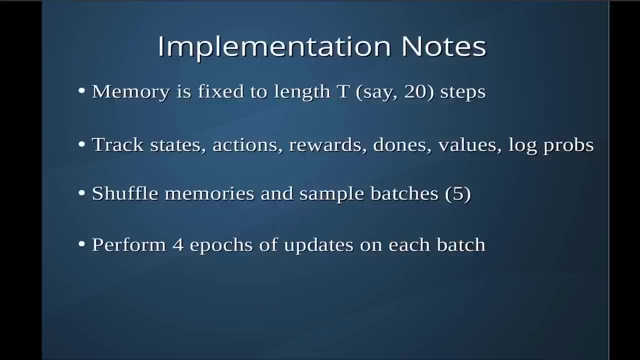 should be much less than the length of, should be much less than the length of the episode, the episode, the episode. so, in the case of the cart pull the. so in the case of the cart pull the. so in the case of the cart pull, the maximum episode length is 200 steps. 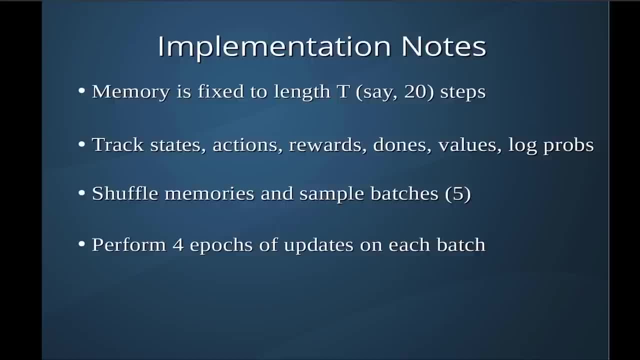 maximum episode length is 200 steps. maximum episode length is 200 steps, and so 20 steps is significantly less, and so 20 steps is significantly less, and so 20 steps is significantly less than that. so i think it qualifies than that. so i think it qualifies. 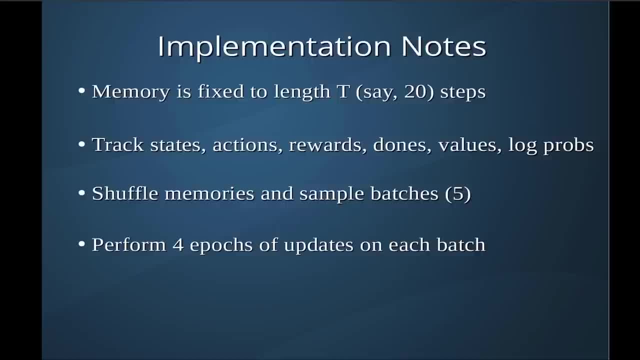 than that. so i think it qualifies. you would want to use something that you would want to use, something that you would want to use something that encompassed more than one episode, encompassed more than one episode. encompassed more than one episode. for instance, that would probably break. 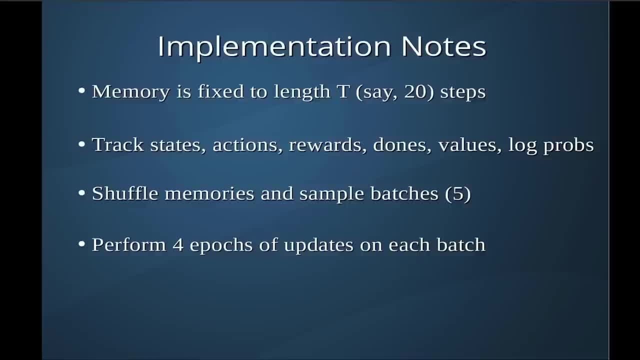 for instance, that would probably break. for instance, that would probably break the algorithm and result in poorer the algorithm and result in poorer the algorithm and result in poorer performance relative to using a capital performance relative to using a capital performance relative to using a capital t much less than the episode length. so 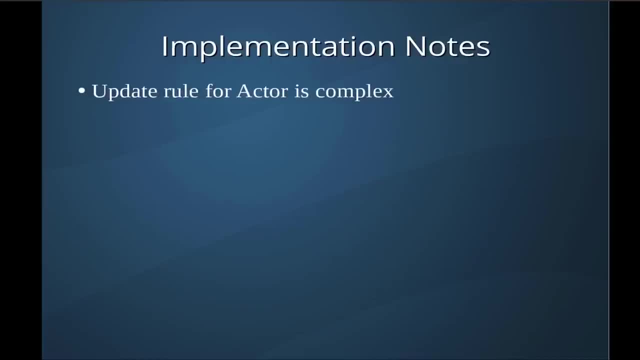 t much less than the episode length. so t much less than the episode length. so all this is relatively simple. all this is relatively simple. all this is relatively simple, but what isn't so simple is the update. but what isn't so simple is the update, but what isn't so simple is the update rule for our actor. so here's where all 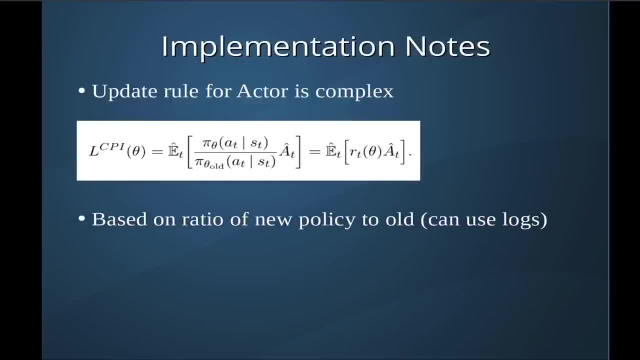 rule for our actor. so here's where all rule for our actor. so here's where all the math comes in. the math comes in, the math comes in. so we have this quantity loss, cpi, this. so we have this quantity loss, cpi, this. so we have this. quantity loss, cpi. this stands for conservative policy iteration. 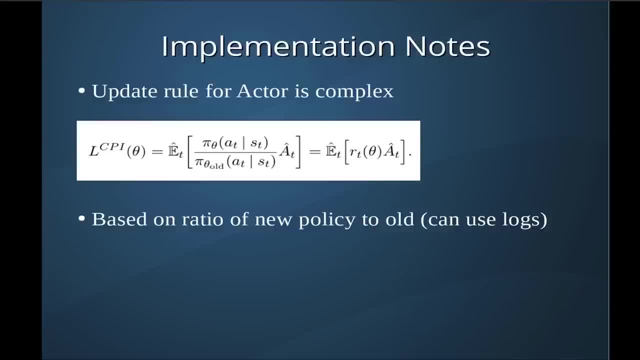 stands for conservative policy iteration, stands for conservative policy iteration, and it's given by the expectation value, and it's given by the expectation value, and it's given by the expectation value, which is just an average of the product, which is just an average of the product, which is just an average of the product of the ratio. 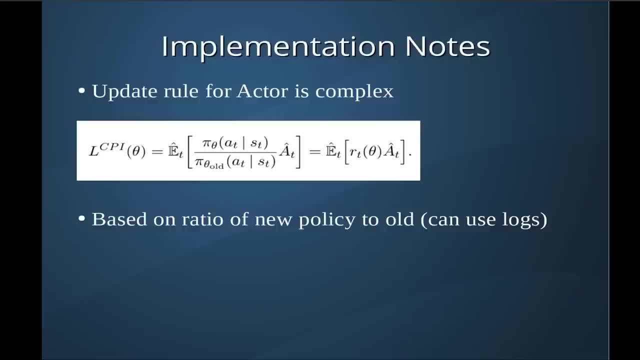 of the ratio, of the ratio of the policy under the current of the policy under the current of the policy under the current parameters, to the policy under the old parameters, to the policy under the old parameters, to the policy under the old parameters, multiplied by this a hat. 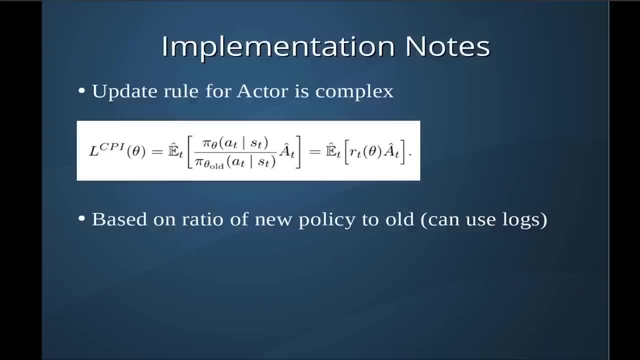 parameters multiplied by this: a hat parameters multiplied by this: a hat sub t. more on that in a second sub t. more on that in a second sub t, more on that in a second. and they, just, they and they just and they, just, they and they just and they, just they and they just abbreviate that ratio is r sub t. 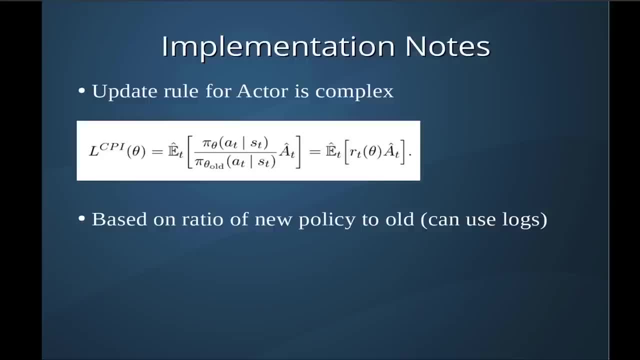 abbreviate that ratio is r sub t. abbreviate that ratio is r sub t. now, if you're not familiar with deep now, if you're not familiar with deep now, if you're not familiar with deep reinforcement learning or reinforcement reinforcement learning or reinforcement reinforcement learning or reinforcement learning in general, the policy is a. 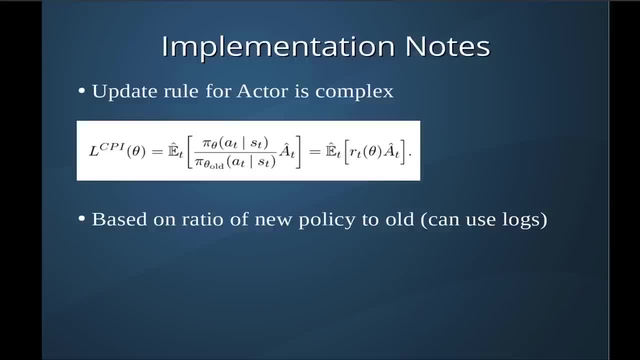 learning in general. the policy is a learning in general. the policy is a probability distribution. that is what our probability distribution, that is what our probability distribution, that is what our actor is attempting to model. is a actor is attempting to model. is a actor is attempting to model. is a probability distribution. the policy. 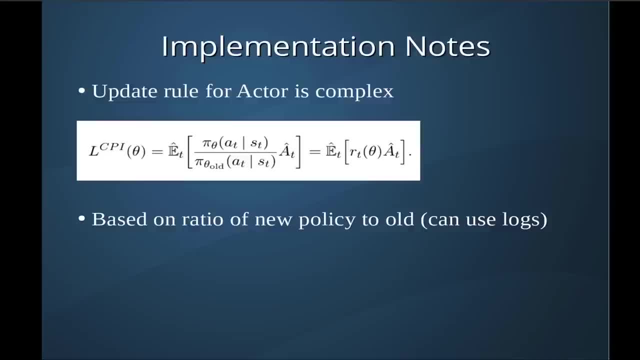 probability distribution: the policy. probability distribution: the policy. and this policy is a mapping between: and. this policy is a mapping between: and this policy is a mapping between states and states, and states and actions and probabilities. so, given you're actions and probabilities, so given you're actions and probabilities, so given you're in state s sub t and you took action a. in state s sub t and you took action a in state s sub t and you took action a sub t. what was the probability of sub t? what was the probability of sub t? what was the probability of selecting that action according to the? selecting that action according to the. 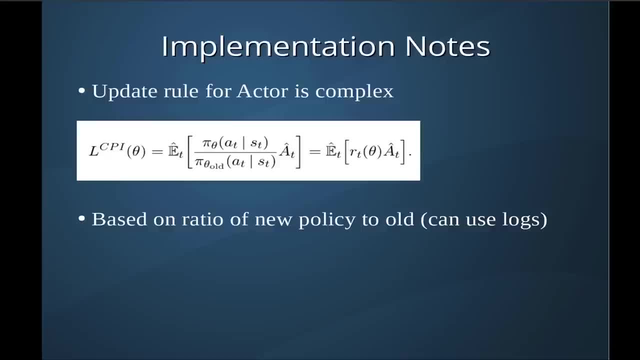 selecting that action according to the distribution, distribution, distribution. and so in the denominator we have theta, and so in the denominator we have theta, and so in the denominator we have theta: old, that is the old, that is the old. that is the probability of selecting action a sub t. 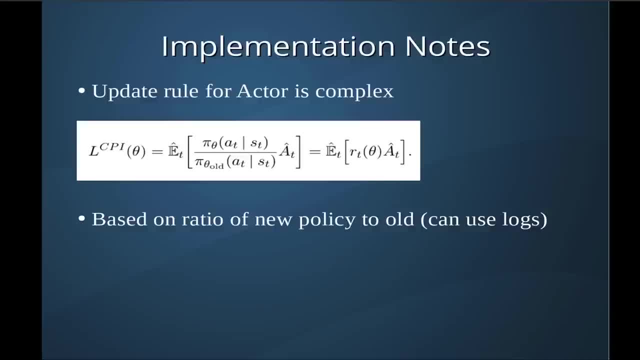 probability of selecting action a sub t. probability of selecting action a sub t. given state s sub t, given state s sub t, given state s sub t under the old parameters of your deep, under the old parameters of your deep, under the old parameters of your deep neural network. so we're going to play 20. 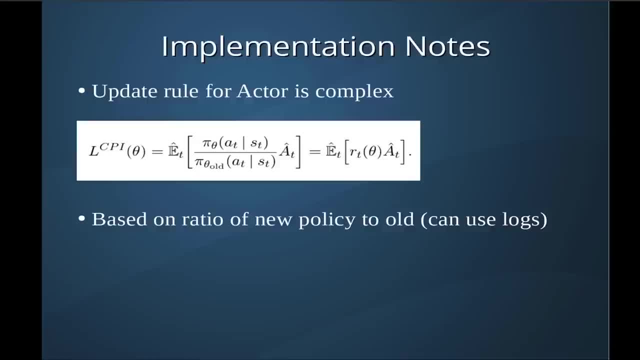 neural network. so we're going to play 20 neural network. so we're going to play 20 steps, and then the agent is going to steps, and then the agent is going to steps, and then the agent is going to perform a learning update. perform a learning update. 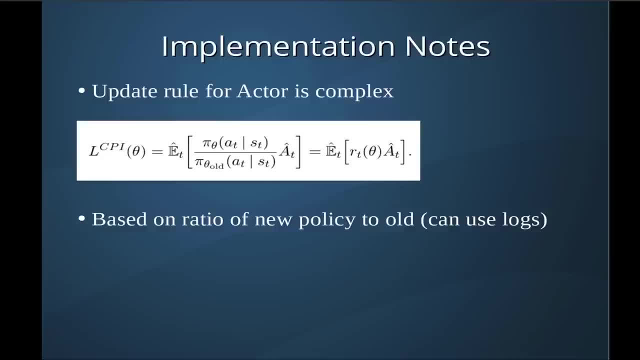 perform a learning update and it's going to do a mini batch. and it's going to do a mini batch, and it's going to do a mini batch- stochastic gradient descent, and so after stochastic gradient descent, and so, after stochastic gradient descent, and so after computing, that first batch, the 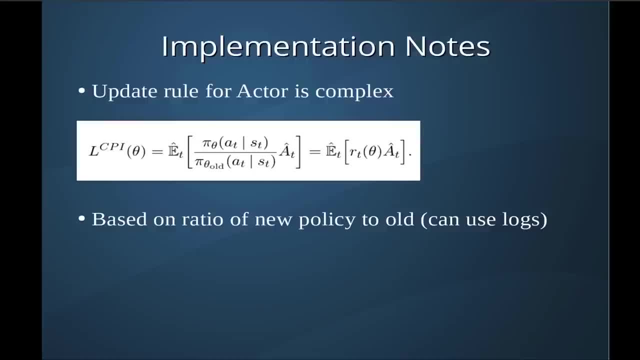 computing that first batch the computing that first batch the parameters of the deep neural network, parameters of the deep neural network, parameters of the deep neural network. change right. that's how change right. that's how change right. that's how the batches work. you compute the loss. the batches work, you compute the loss. 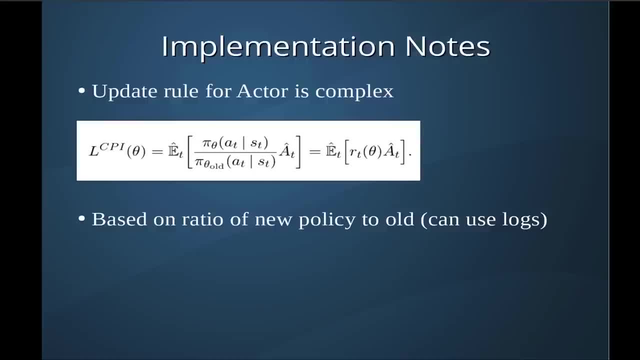 the batches work, you compute the loss with each batch and update your with each batch, and update your with each batch and update your parameters. and so, right after you've parameters, and so right after you've parameters, and so right after you've calculated that first batch of memories, 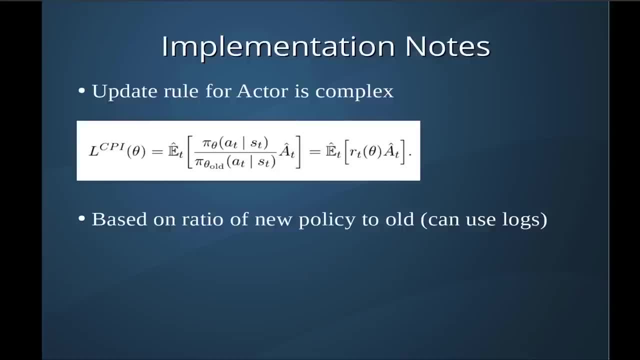 calculated that first batch of memories. calculated that first batch of memories, the loss for that, and updated your deep the loss for that and updated your deep, the loss for that, and updated your deep. neural network, neural network, neural network: the theta changes, and so the policy pi. the theta changes, and so the policy pi. 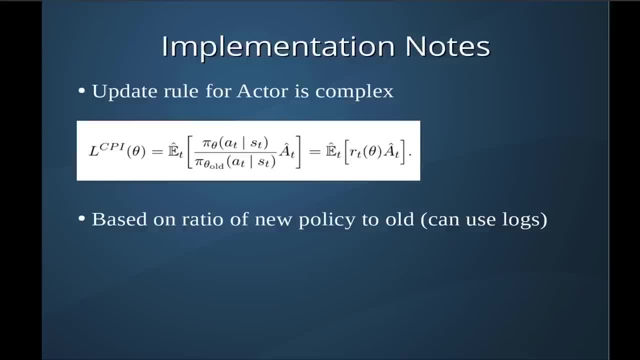 the theta changes, and so the policy pi is going to change as well, is going to change as well, is going to change as well, and so we have to keep track of the, and so we have to keep track of the and so we have to keep track of the parameters. 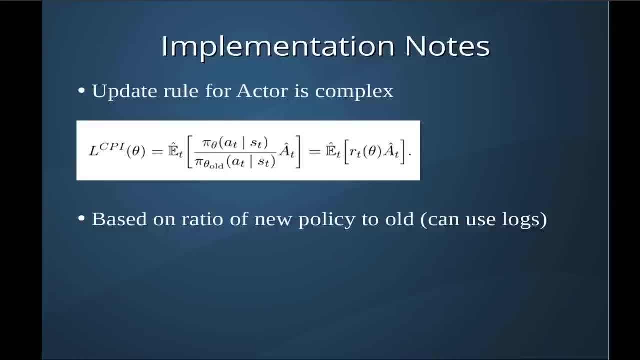 parameters, parameters, excuse me of the. the probabilities, excuse me of the. the probabilities, excuse me of the. the probabilities of selecting each action at each time, of selecting each action at each time, of selecting each action at each time, step in our memory and then on a step in our memory, and then on a. 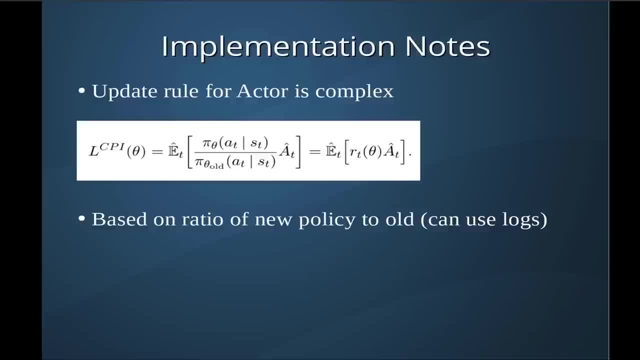 step in our memory and then, on a learning function, we're going to pass learning function. we're going to pass learning function. we're going to pass those states through our actor network. those states through our actor network, those states through our actor network, get the probabilities, the probability. 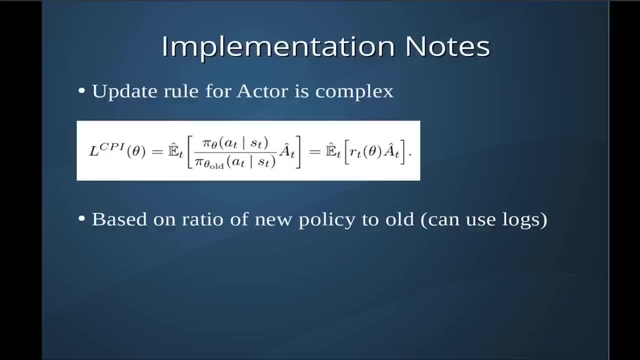 get the probabilities, the probability, get the probabilities, the probability distribution, and find out what the distribution and find out what the distribution and find out what the probability. selecting action a sub t is probability. selecting action a sub t is probability. selecting action a sub t is sampled from our memory, according to the 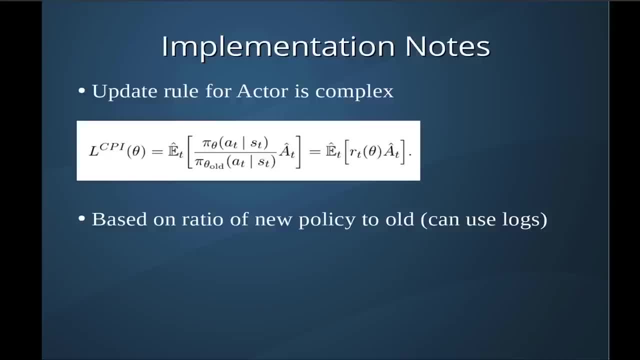 sampled from our memory. according to the sampled from our memory. according to the current values: current values, current values of the deep neural network. it'll be a of the deep neural network. it'll be a of the deep neural network. it'll be a little bit more clear in code. 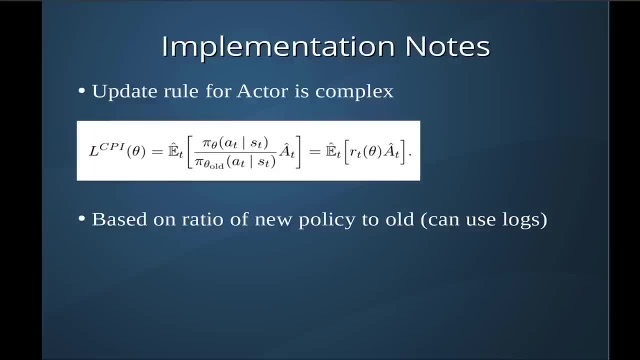 little bit more clear in code. little bit more clear in code. just know that we have to keep track of. just know that we have to keep track of. just know that we have to keep track of log probes as we go along and we're log probes as we go along and we're. 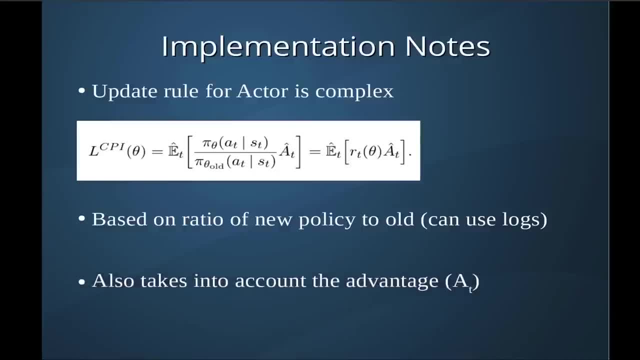 log probes as we go along, and we're going to be recalculating them in the, going to be recalculating them in the going to be recalculating them in the learning loop, learning loop, learning loop. one thing we also see is that it takes. 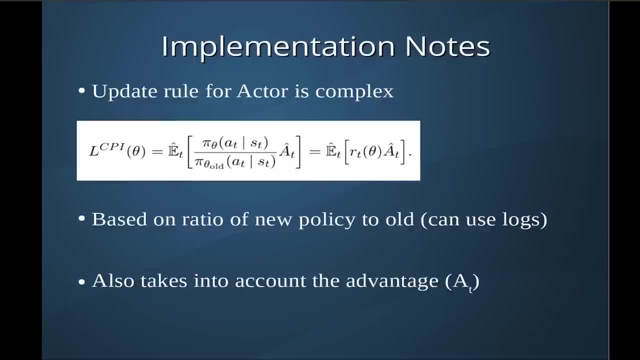 one thing we also see is that it takes. one thing we also see is that it takes into account the advantage which is at into account, the advantage which is at into account, the advantage which is at a hat sub t, so the advantage is just a: a hat sub t, so the advantage is just a. 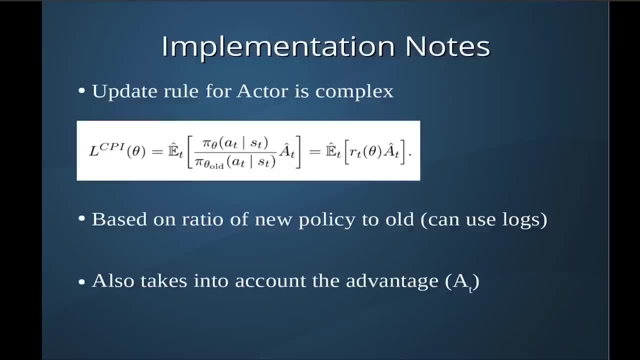 a hat sub t. so the advantage is just a measure of the goodness of each state. measure of the goodness of each state. measure of the goodness of each state. we'll get to the calculation of that in a. we'll get to the calculation of that in a. 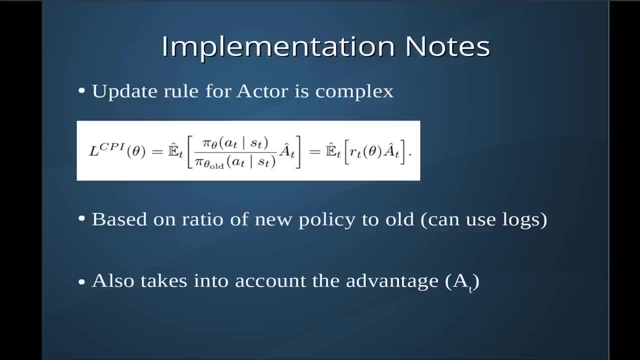 we'll get to the calculation of that in a few minutes, few minutes, few minutes, but one thing to note is that this, but one thing to note is that this, but one thing to note is that this ratio, ratio, ratio pi sub theta over pi sub theta old. 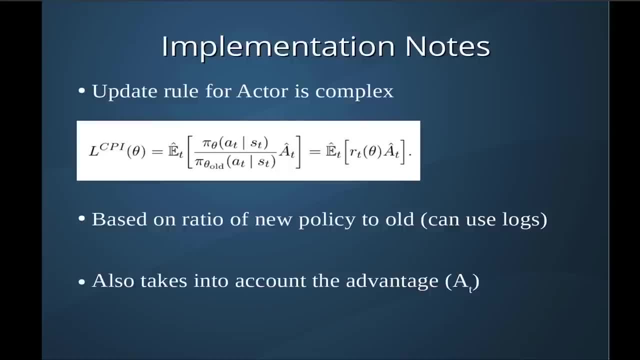 pi sub theta over pi sub theta old, pi sub theta over pi sub theta old can have an arbitrary value. right because can have an arbitrary value. right because can have an arbitrary value. right because you could have. let's say you could have, let's say you could have, let's say pi theta being 0.99 pi theta old. 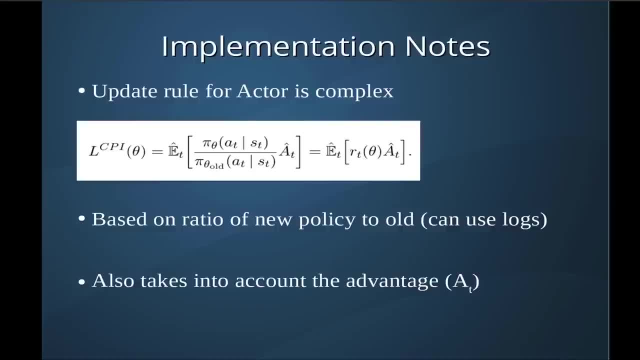 pi theta being 0.99 pi theta old, pi theta old: 0.01, and so that's a pretty large number, 0.01. and so that's a pretty large number, 0.01. and so that's a pretty large number and in particular, if you multiply it by: 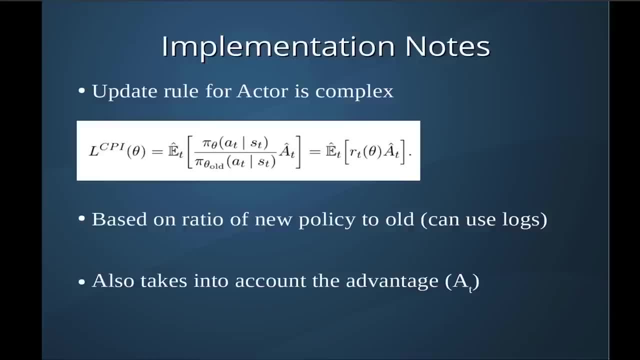 and in particular, if you multiply it by, and in particular, if you multiply it by an advantage that is like say 10, 20, an advantage that is like say 10, 20, an advantage that is like say 10, 20, whatever, then that can also still be a 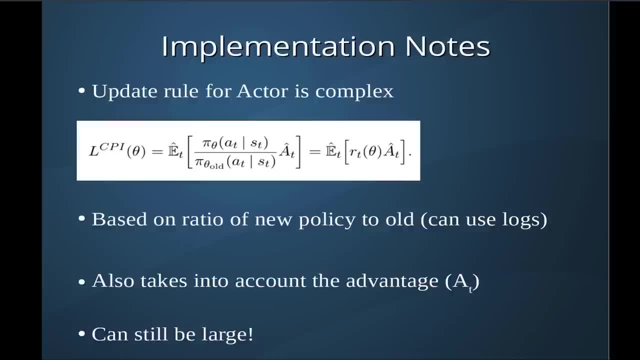 whatever, then that can also still be a whatever, then that can also still be a large number, large number, large number, and so we have to deal with that right, and so we have to deal with that right, and so we have to deal with that right, because the whole point of this is that 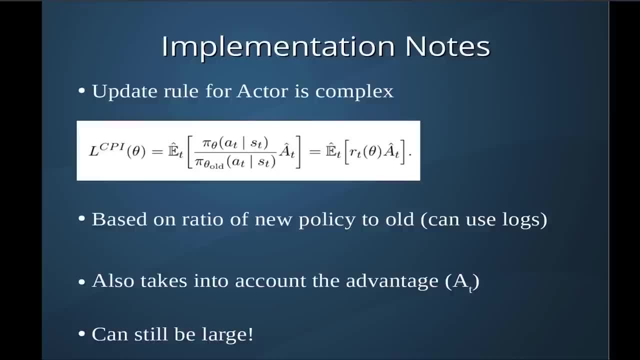 because the whole point of this is that, because the whole point of this is that we want to constrain, we want to constrain, we want to constrain the updates to our deep neural network, the updates to our deep neural network, the updates to our deep neural network, to be some relatively small amount. 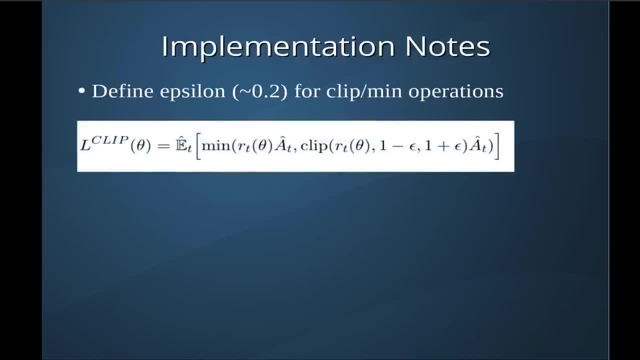 to be some relatively small amount, to be some relatively small amount, and so the way you deal with that is by and so. the way you deal with that is by and so. the way you deal with that is by adding an additional hyper parameter. adding an additional hyper parameter. 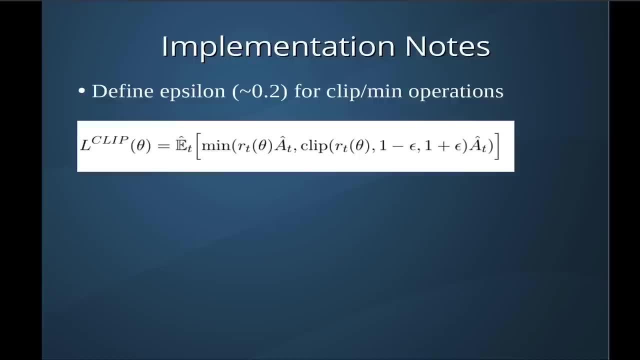 adding an additional hyper parameter: epsilon- epsilon. epsilon that you use to clip that ratio, so what that you use to clip that ratio, so what that you use to clip that ratio. so what we're going to do is we're going to clip. we're going to do is we're going to clip. 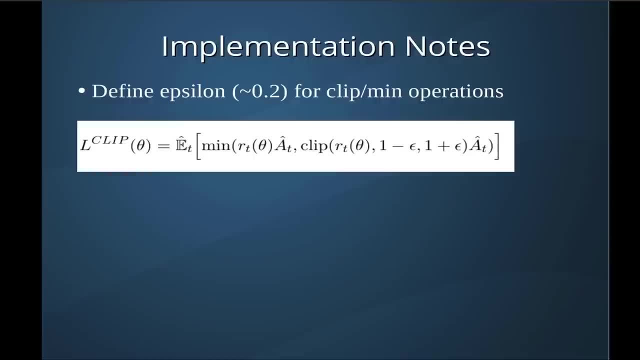 we're going to do is we're going to clip that ratio within the range one minus that ratio within the range one minus that ratio within the range one minus epsilon to plus epsilon to plus epsilon to plus one plus epsilon. so let's say from 0.8. 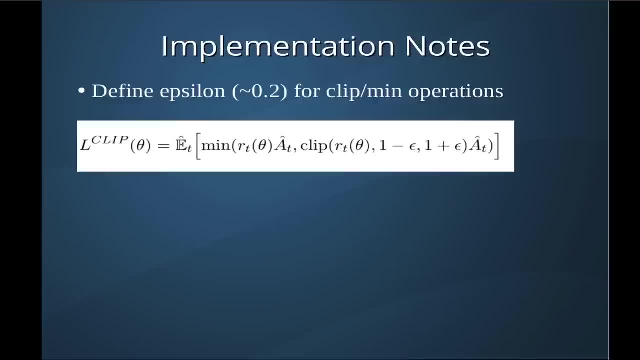 epsilon to plus 1.8. epsilon to plus 1.8 to 1.2. so that ratio is going to be to 1.2. so that ratio is going to be to 1.2. so that ratio is going to be constrained to be close to one. constrained to be close to one. constrained to be close to one, and you're going to multiply that by the, and you're going to multiply that by the, and you're going to multiply that by the advantage, and so that'll give you some advantage, and so that'll give you some. 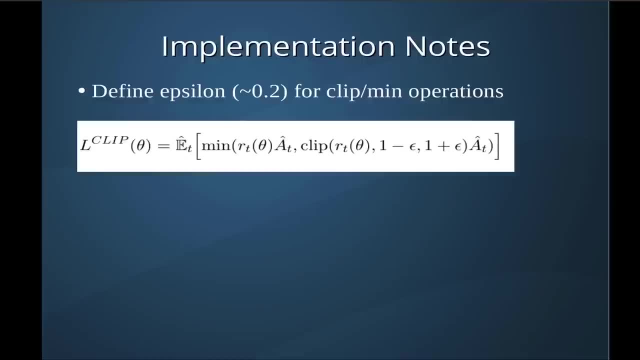 advantage, and so that'll give you some number, number, number, and then you want to take the minimum of, and then you want to take the minimum of, and then you want to take the minimum of that clipped number, that clipped number, that clipped number, the clipped ratio multiplied by the. 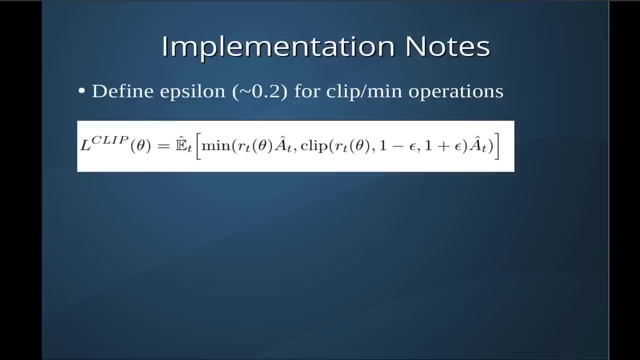 the clipped ratio multiplied by the. the clipped ratio multiplied by the advantage and the unclipped ratio, the clipped ratio multiplied by the advantage. take the minimum advantage, take the minimum advantage, take the minimum, and that is what we will use for the loss and that is what we will use for the loss. 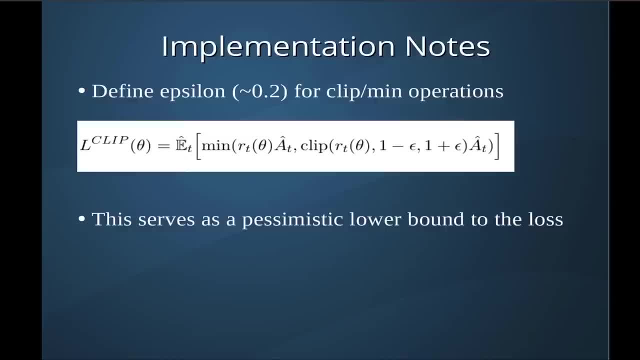 and that is what we will use for the loss for our actor network, for our actor network, for our actor network. so this serves as a pessimistic lower. so this serves as a pessimistic lower. so this serves as a pessimistic lower bound to the loss, bound to the loss. 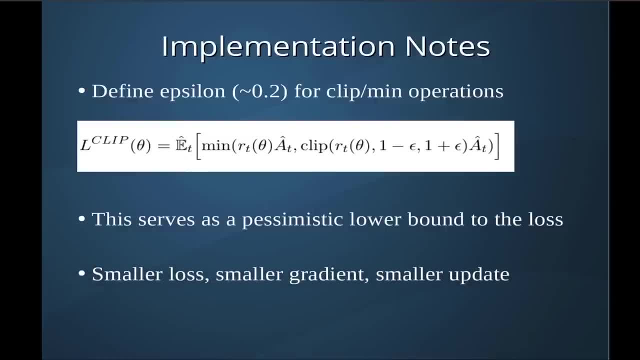 bound to the loss and they don't go into any real depth in. and they don't go into any real depth in and they don't go into any real depth in the paper on the reasoning for this, the paper on the reasoning for this, the paper on the reasoning for this. uh, but to my mind- and this could be wrong- uh, but to my mind, and this could be wrong. uh, but to my mind, and this could be wrong. you know, i am an idiot sometimes, but my. you know i am an idiot sometimes, but my, you know, i am an idiot sometimes, but my understanding is. understanding is. 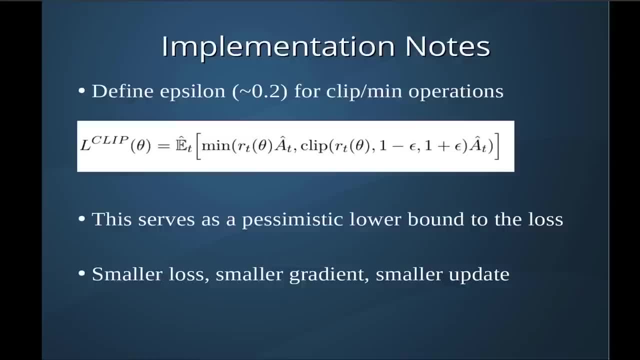 understanding is: smaller loss, smaller gradient, smaller. smaller loss. smaller gradient, smaller. smaller loss, smaller gradient, smaller. update. that's the whole point of it. update. that's the whole point of it, update. that's the whole point of it. so let's talk about this advantage now. so let's talk about this advantage now. 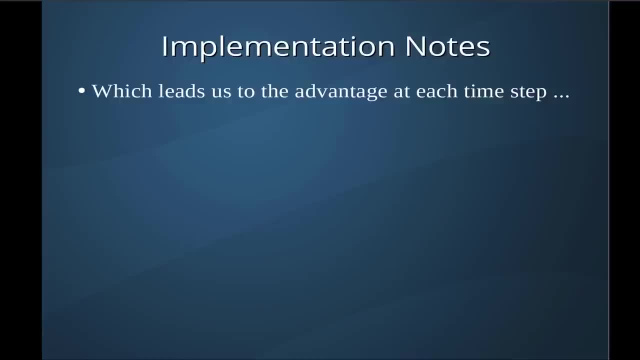 so let's talk about this advantage now. so, so, so, this advantage has to be calculated at. this advantage has to be calculated at. this advantage has to be calculated at each time step, and it's given by each time step, and it's given by each time step, and it's given by this equation. now, don't freak out, this is 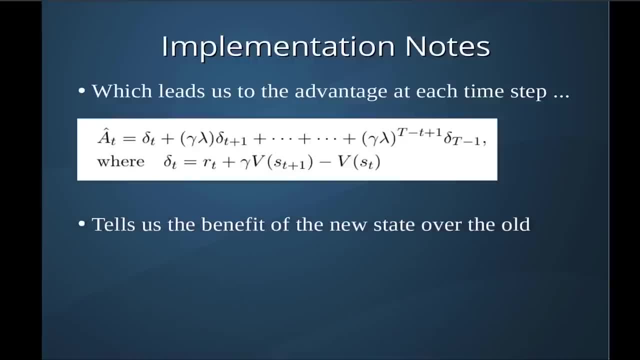 this equation now, don't freak out. this is this equation. now don't freak out. this is relatively straightforward. once again, it relatively straightforward. once again, it relatively straightforward. once again, it tells us the benefit of the new state, tells us the benefit of the new state, tells us the benefit of the new state over the old. well, how do we know that we? 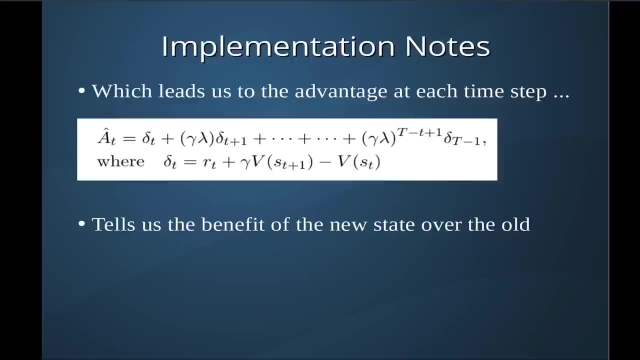 over the old? well, how do we know that? we over the old? well, how do we know that? we know that because it's proportional to know that, because it's proportional to know that, because it's proportional to or equal to the sum of the delta sub t. or equal to the sum of the delta sub t, or equal to the sum of the delta sub t, where the delta sub t is just the reward, where the delta sub t is just the reward, where the delta sub t is just the reward at a time step. 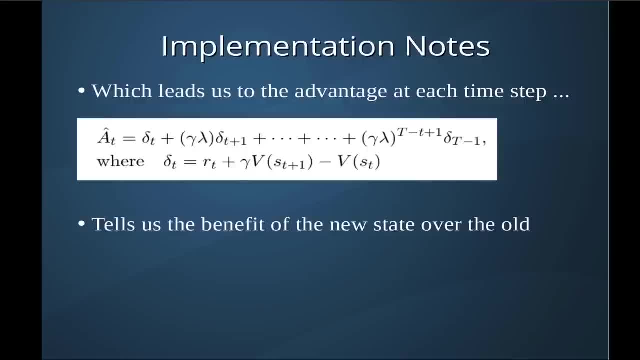 at a time step, at a time step, plus the difference in the estimated, plus the difference in the estimated, plus the difference in the estimated value of the new state and the current value of the new state, and the current value of the new state and the current state. so it tells you what is the. 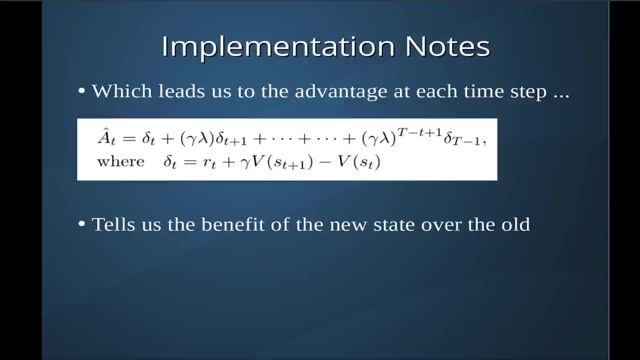 state. so it tells you what is the state. so it tells you what is the difference in the value between the next difference in the value between the next difference in the value between the next bet- the next state we encounter- and the bet- the next state we encounter- and the. 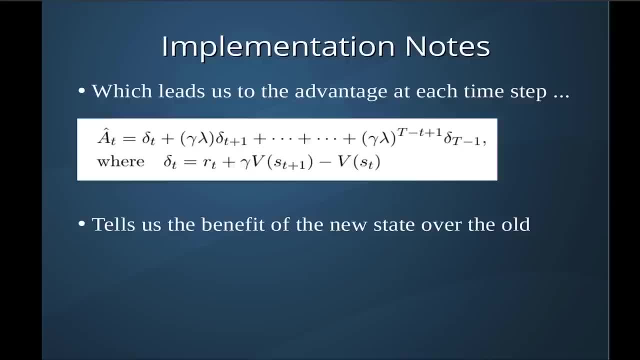 bet the next state we encounter and the current state, and of course you have the current state and of course you have the current state, and of course you have the gamma in front of the v, which is the gamma in front of the v, which is the gamma in front of the v, which is the output of the critic network, because we 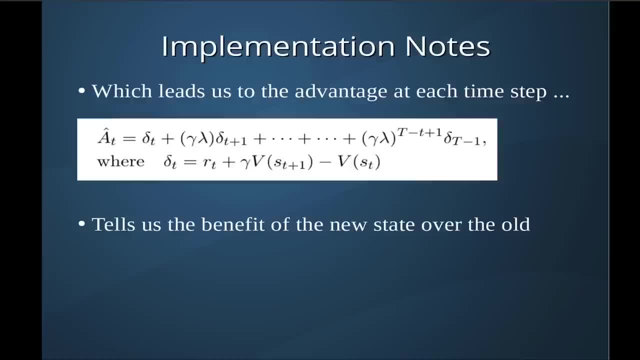 output of the critic network. because we output of the critic network, because we always discount the values of the next, always discount the values of the next, always discount the values of the next states, because we don't know the full states, because we don't know the full. 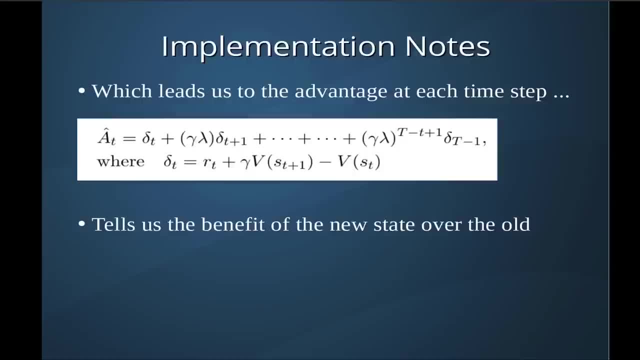 states because we don't know the full dynamics of the environment, and so the dynamics of the environment, and so the dynamics of the environment, and so the that reward is uncertain. there's always that reward is uncertain. there's always that reward is uncertain. there's always some uncertainty around state. 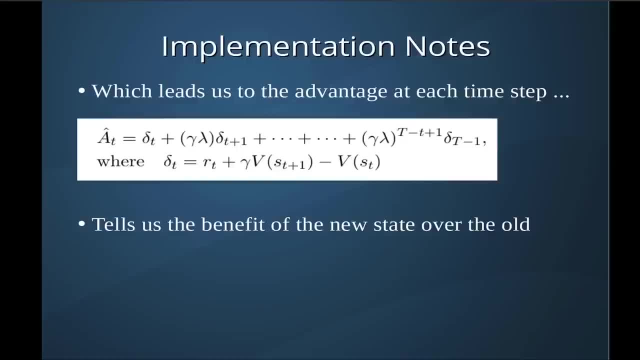 some uncertainty around state, some uncertainty around state transitions, and then in the top transitions, and then in the top transitions and then in the top equation. you just sum that where you're equation. you just sum that where you're equation. you just sum that where you're gonna be summing over gamma multiplied. 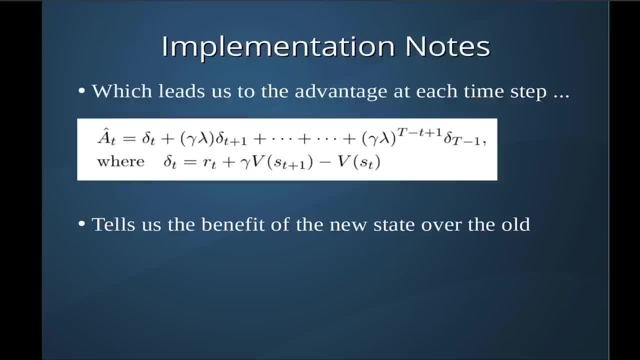 gonna be summing over gamma multiplied. gonna be summing over gamma multiplied by lambda. so this quantity gamma is by lambda, so this quantity gamma is by lambda. so this quantity gamma is again the normal gamma is 0.99. that we. again the normal gamma is 0.99 that we. 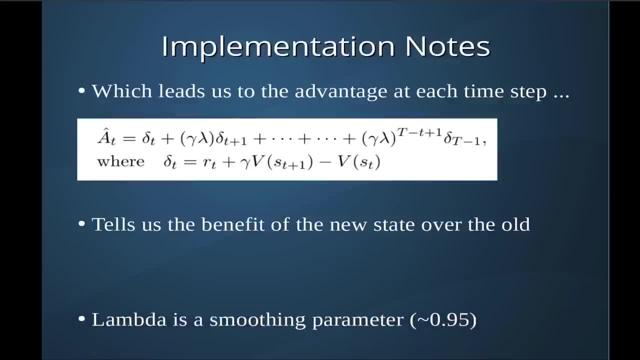 again, the normal gamma is 0.99. that we typically use, but this parameter lambda typically use, but this parameter lambda typically use, but this parameter lambda is a type of smoothing parameter. it is a type of smoothing parameter. it is a type of smoothing parameter. it helps to reduce variance and we're going. 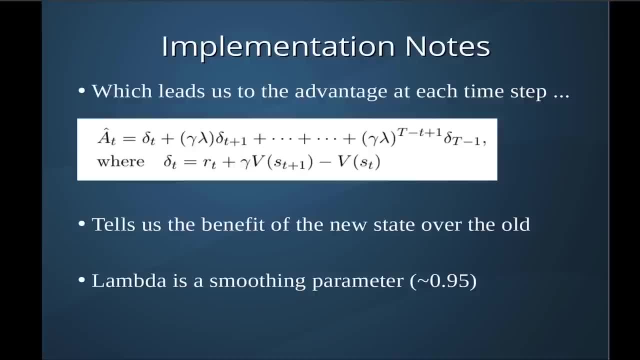 helps to reduce variance and we're going helps to reduce variance and we're going to use a value of 0.95 and for to use a value of 0.95 and for to use a value of 0.95 and for implementation, we're just going to use a. 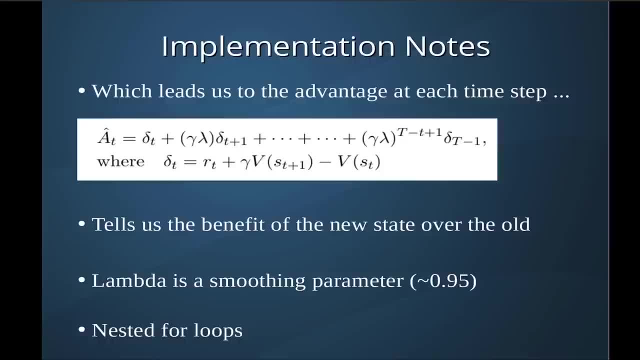 implementation. we're just going to use a implementation. we're just going to use a couple of nested for loops. so you're couple of nested for loops, so you're couple of nested for loops. so you're gonna start out at time t equals 0 and gonna start out at time t equals 0 and. 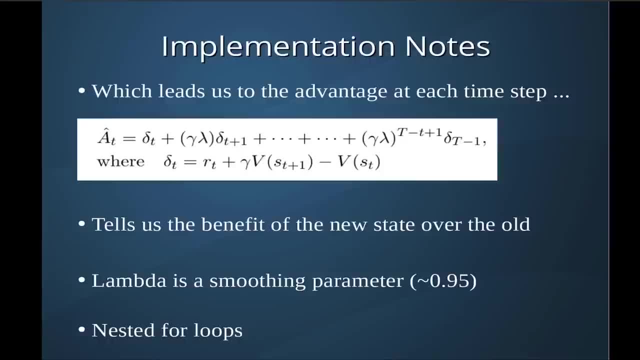 gonna start out. at time t equals 0, and then some from that step all the way up, then some from that step all the way up, then some from that step all the way up to capital T minus 1. so if we have 20, to capital T minus 1. so if we have 20, 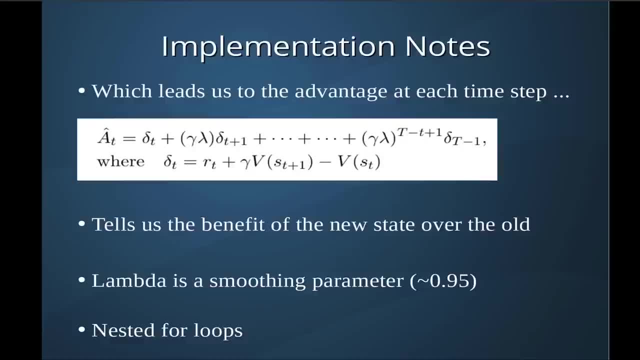 to capital T minus 1. so if we have 20 states, you're gonna go from 0 to capital states. you're gonna go from 0 to capital states. you're gonna go from 0 to capital T minus 1, 0 to 18, and you have to do. 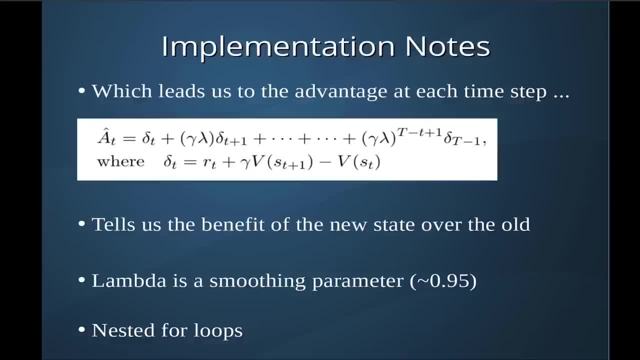 T minus 1: 0 to 18. and you have to do T minus 1: 0 to 18. and you have to do that because you have the V of s sub T, that, because you have the V of s sub T, that, because you have the V of s sub T plus 1, you don't want to try to evaluate. 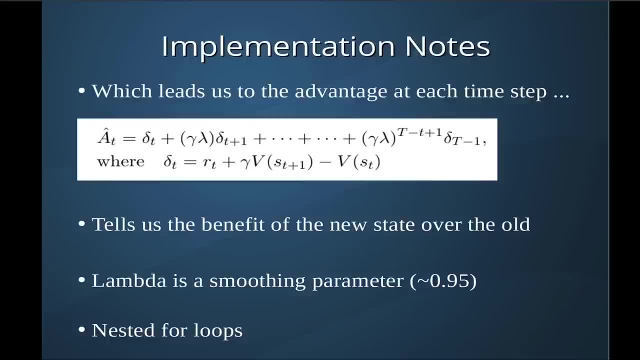 plus 1. you don't want to try to evaluate plus 1. you don't want to try to evaluate something beyond the number of actual something, beyond the number of actual something, beyond the number of actual states that you have. that won't work out. states that you have. that won't work out. 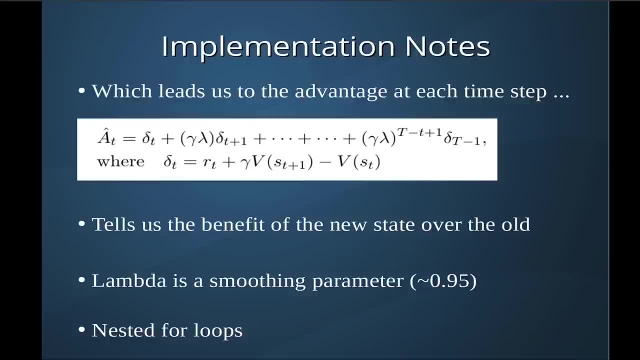 states that you have that won't work out right, and so it's going to be right, and so it's going to be right, and so it's going to be relatively straightforward. once you see relatively straightforward, once you see relatively straightforward, once you see it in action, and we're going to be. 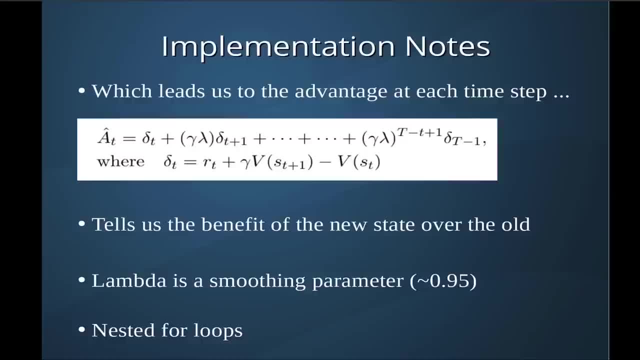 it in action and we're going to be it in action and we're going to be keeping track of that gamma times lambda. keeping track of that gamma times lambda, keeping track of that gamma times lambda, which is a multiplicative constant, that which is a multiplicative constant, that. 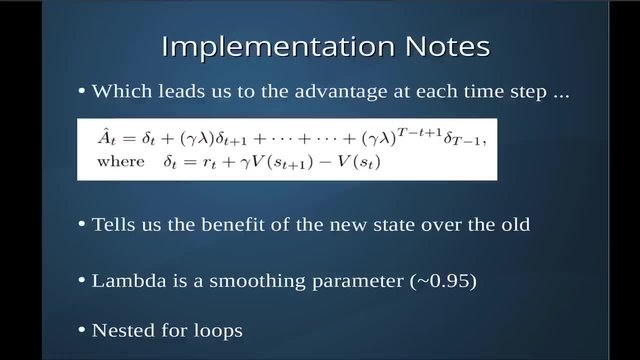 which is a multiplicative constant that increases its power by 1 with each increases its power by 1 with each increases its power by 1 with each iteration of the inner loop. all that'll iteration of the inner loop. all that'll iteration of the inner loop. all that'll be made clear in the code. but 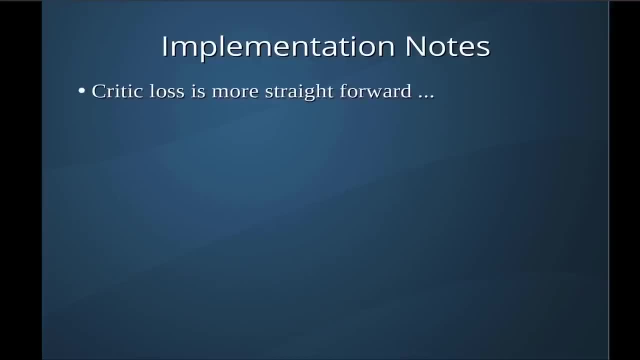 be made clear in the code. but be made clear in the code. but fortunately the critic loss is a little, fortunately the critic loss is a little. fortunately the critic loss is a little bit more straightforward. so we need bit more straightforward. so we need bit more straightforward, so we need something called the return. so the 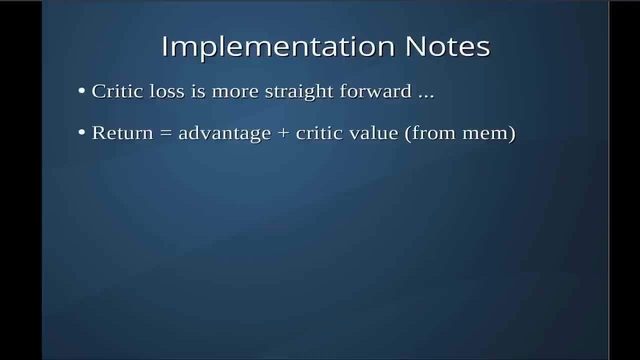 something called the return, so the something called the return, so the return is just equal to this sum of the return is just equal to this sum of the return is just equal to this sum of the advantage and the critic value based on advantage and the critic value based on. 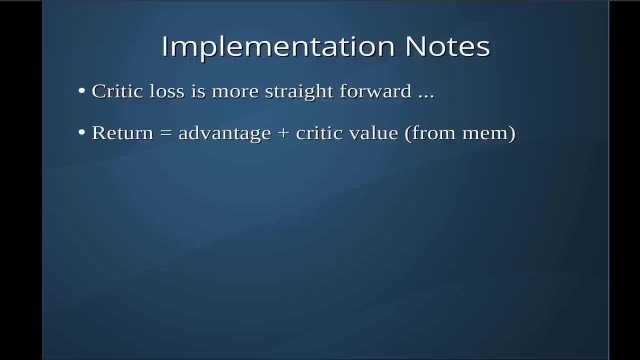 advantage and the critic value based on the memory. so, whatever the agent, the memory. so, whatever the agent, the memory. so, whatever the agent, estimated the value of a particular state. estimated the value of a particular state. estimated the value of a particular state to be at the time that it took it is. 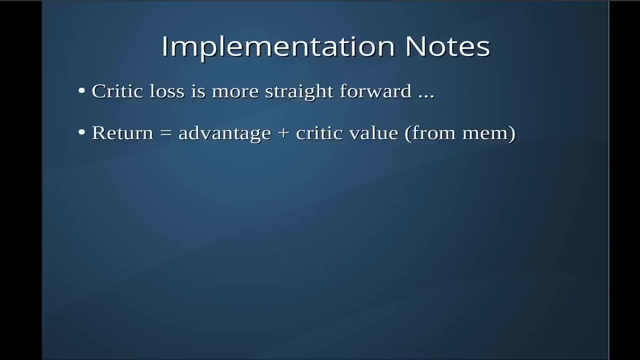 to be at the time that it took. it is to be at the time that it took. it is what we're going to be using for the, what we're going to be using for the, what we're going to be using for the critic value in our return, and then the. 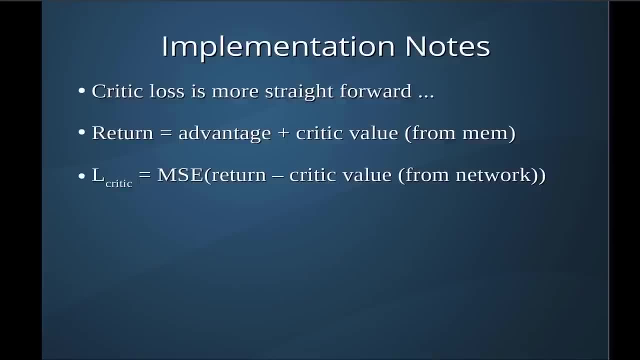 critic value in our return, and then the critic value in our return, and then the loss of the critic is just going to be. loss of the critic is just going to be. loss of the critic is just going to be the mean squared error between the, the mean squared error between the. 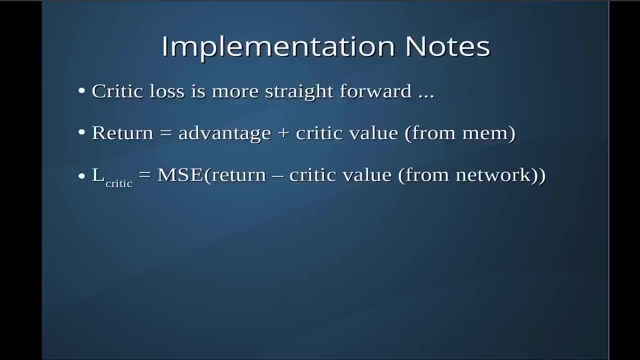 the mean squared error between the return and the critic value based on the return and the critic value based on the return and the critic value based on the current values of the deep neural, current values of the deep neural, current values of the deep neural network. so once again, we're going to be. 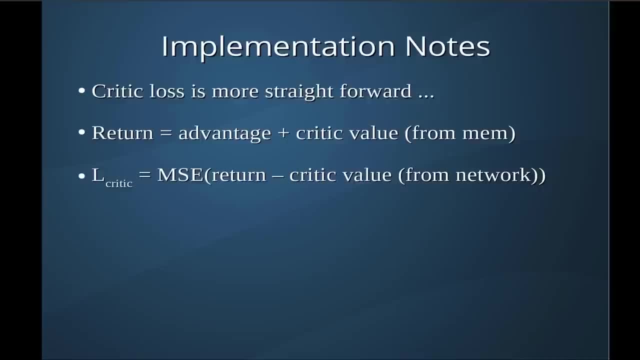 network. so once again we're going to be network. so once again we're going to be passing the states through the critic, passing the states through the critic, passing the states through the critic network to get its estimate of values network to get its estimate of values network to get its estimate of values. and we're going to be also using the 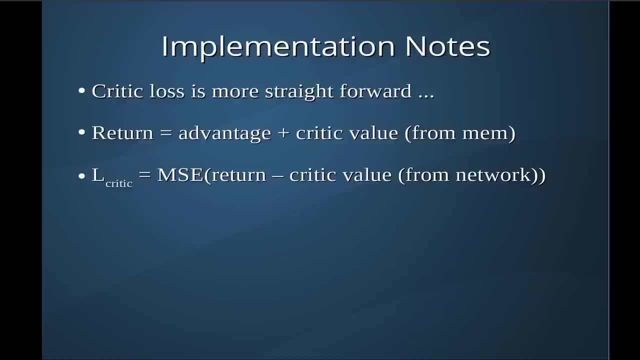 and we're going to be also using the and we're going to be also using the values from the memory as well. so values from the memory as well, so values from the memory as well. so relatively straightforward- even easier. relatively straightforward- even easier. relatively straightforward- even easier when you see it in code. so we have two. 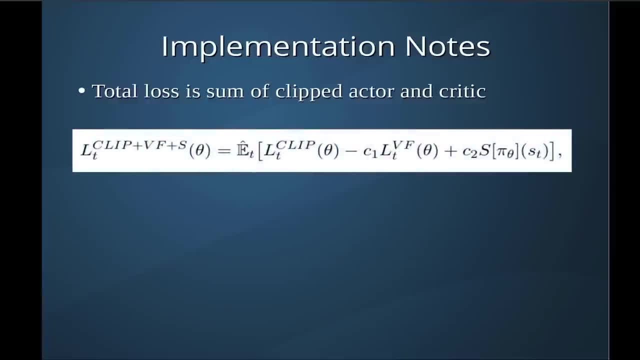 when you see it in code, so we have two. when you see it in code, so we have two different losses and we have to sum them. different losses, and we have to sum them. different losses, and we have to sum them, and so that'll be the sum of the clipped. 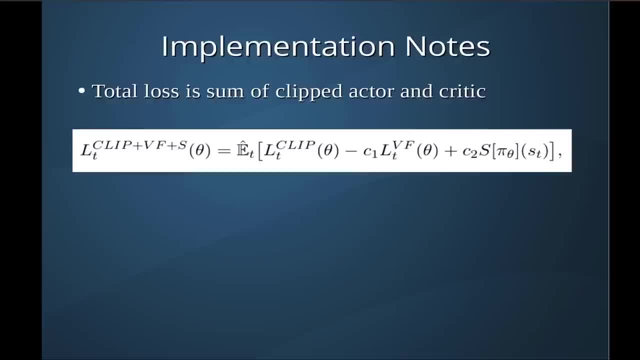 and so that'll be the sum of the clipped, and so that'll be the sum of the clipped actor and critic. so a couple things to actor and critic. so a couple things to actor and critic. so a couple things to take is going to be positive and the loss. 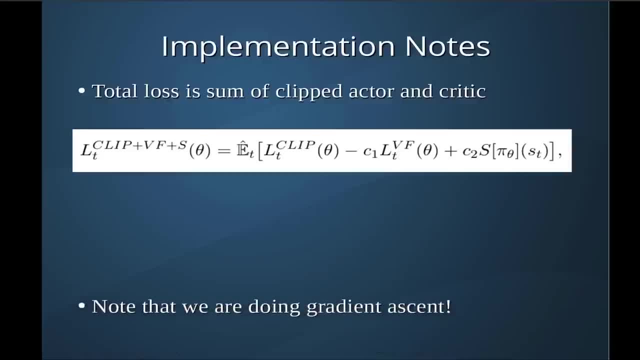 take is going to be positive and the loss take is going to be positive and the loss of our actor is going to be negative, of our actor is going to be negative, of our actor is going to be negative because we are doing gradient ascent and because we are doing gradient ascent and 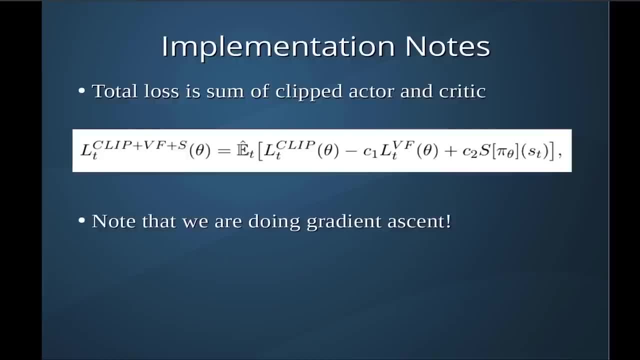 because we are doing gradient ascent and not gradient descent. we have to not gradient descent. we have to not gradient descent. we have to multiply by negative. one other thing to multiply by negative. one other thing to multiply by negative. one other thing to note is that we have this other 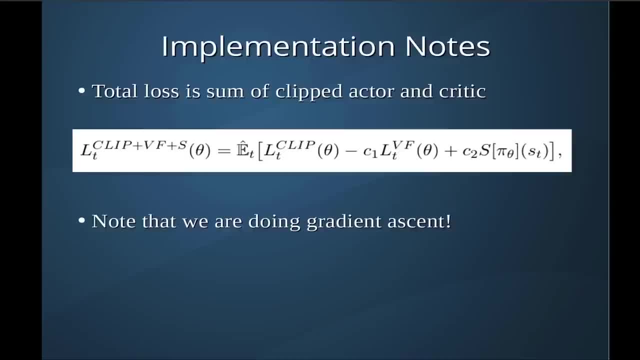 note is that we have this other note is that we have this other parameter here C to this coefficient parameter, here C to this coefficient parameter, here C to this coefficient: multiplied by s, s is an entropy term and multiplied by s, s is an entropy term and multiplied by s- s is an entropy term. and that only comes into play when you. 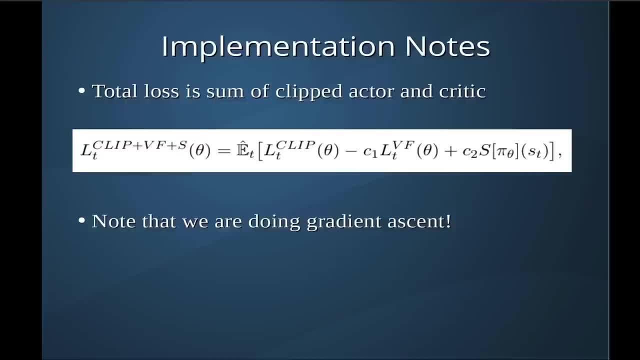 that only comes into play when you. that only comes into play when you have a deep neural network with shared lower. have a deep neural network with shared lower. have a deep neural network with shared lower layers and actor and critic outputs layers and actor and critic outputs layers and actor and critic outputs at the top. so we don't have to worry about. 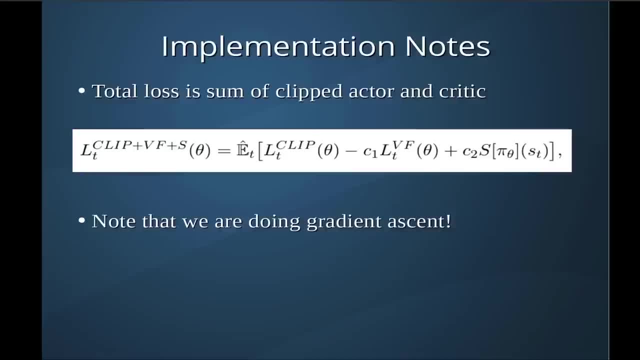 at the top, so we don't have to worry about at the top. so we don't have to worry about that in our particular implementation. that in our particular implementation, that in our particular implementation in this tutorial, because we're doing two in this tutorial, because we're doing two. 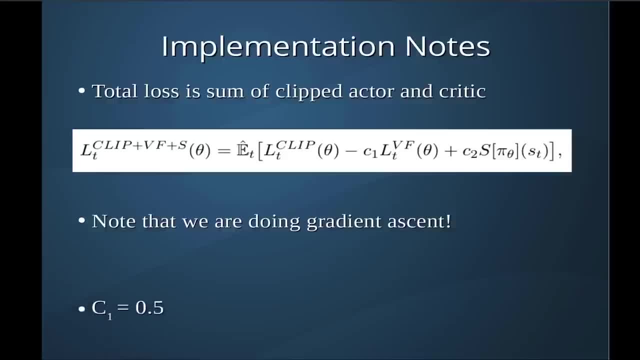 in this tutorial, because we're doing two separate networks for the actor and the separate networks for the actor and the separate networks for the actor and the critic, and I'm going to use a critic and I'm going to use a critic and I'm going to use a coefficient of 0.5 for the loss for the. 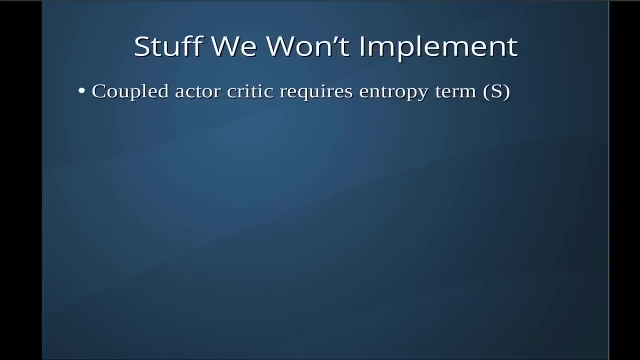 coefficient of 0.5 for the loss, for the coefficient of 0.5 for the loss for the critic. as I said, we're not going to be critic. as I said, we're not going to be critic. as I said, we're not going to be implementing the entropy term because, 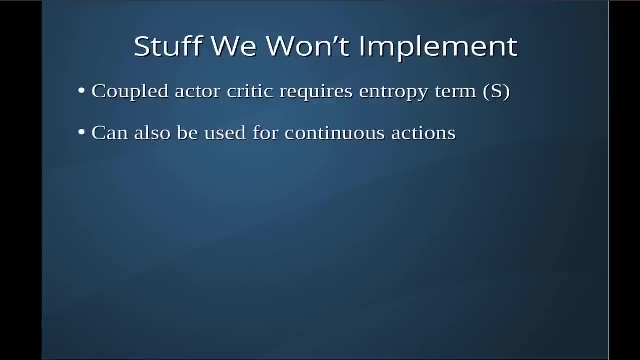 implementing the entropy term, because implementing the entropy term, because we're doing two distinct networks, we can. we're doing two distinct networks, we can. we're doing two distinct networks. we can also use this for continuous actions. also use this for continuous actions. also use this for continuous actions. there, you would use a different output. 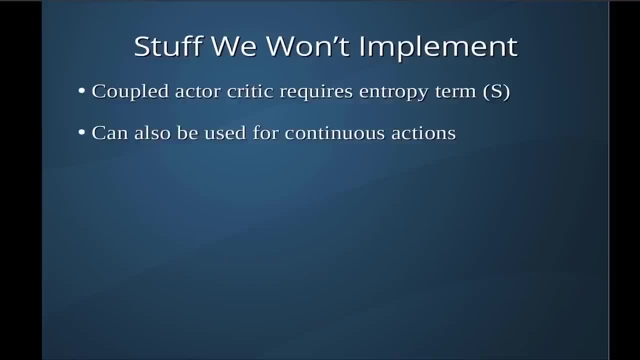 there, you would use a different output. there, you would use a different output for your actor network, and indeed that's for your actor network and indeed that's for your actor network, and indeed that's what the paper really is geared for. as what the paper really is geared for as 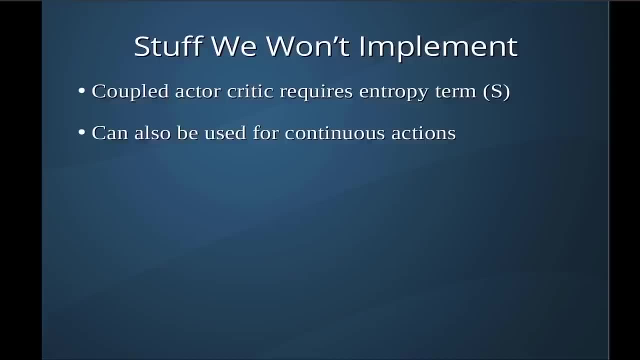 what the paper really is geared for. as for continuous action spaces, but we're for continuous action spaces, but we're for continuous action spaces, but we're going to be doing the very simple, going to be doing the very simple, going to be doing the very simple, discrete case. other thing: we won't. 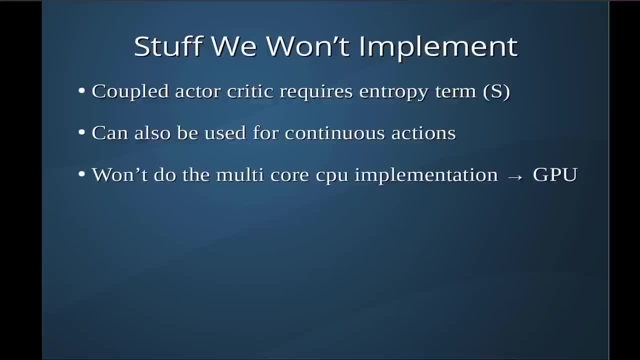 discrete case. other thing we won't- discrete case, other thing we won't implement- is the multi-core CPU implement. is the multi-core CPU implement. is the multi-core CPU implementation. because that introduces implementation, because that introduces implementation, because that introduces even more complexity. we're just going. 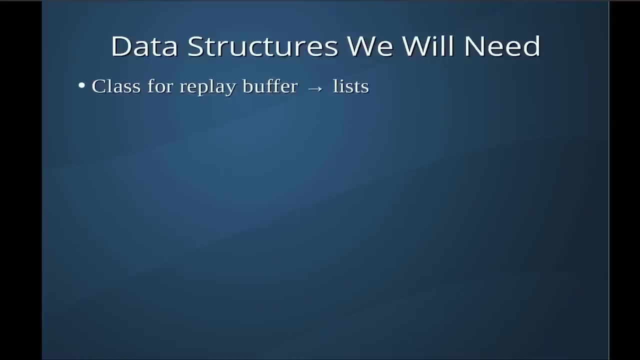 even more complexity. we're just going even more complexity. we're just going to be using the GPU. so what do we need for to be using the GPU? so what do we need for to be using the GPU? so what do we need for this project? we're gonna need a class. 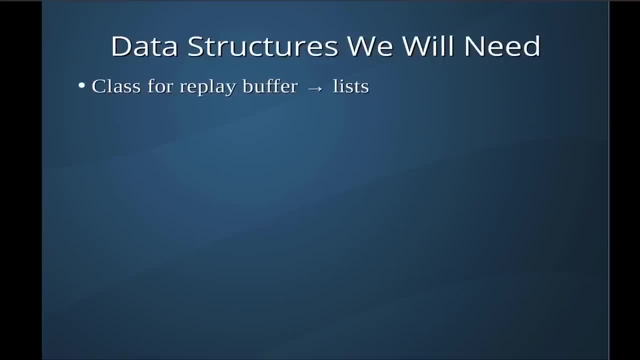 this project, we're gonna need a class. this project, we're gonna need a class for the replay buffer, and we're just for the replay buffer and we're just for the replay buffer and we're just going to use lists for this, normally. I going to use lists for this, normally I. 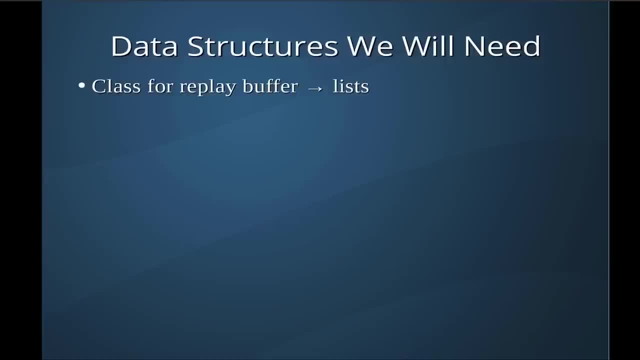 going to use lists for this. normally I like to use numpy arrays, but in this, like to use numpy arrays, but in this, like to use numpy arrays, but in this case, lists turn out to be a simpler case. lists turn out to be a simpler case. lists turn out to be a simpler implementation. so that's what we're. 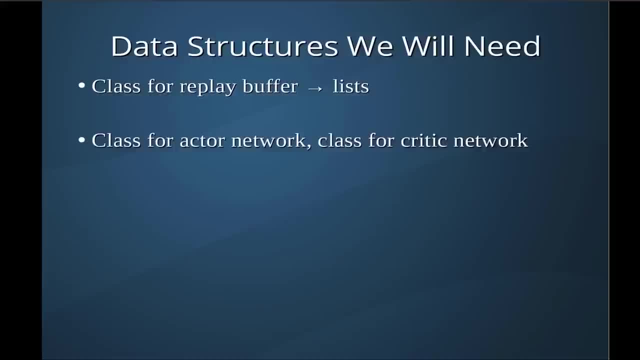 implementation. so that's what we're implementation. so that's what we're gonna go with. we're also going to need a gonna go with. we're also going to need a gonna go with. we're also going to need a class for our actor network and a class. 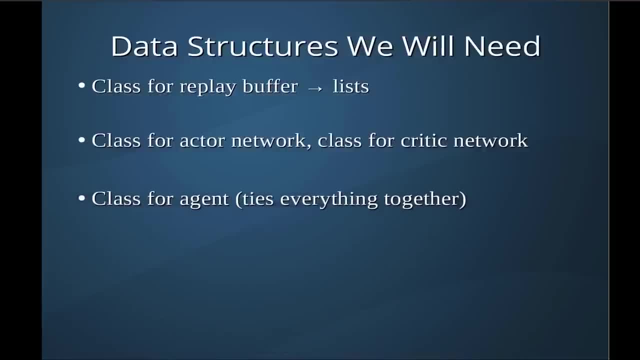 class for our actor network and a class class for our actor network and a class for the critic network. we'll need a class for the critic network. we'll need a class for the critic network. we'll need a class for agent that's going to tie, class for agent that's going to tie. 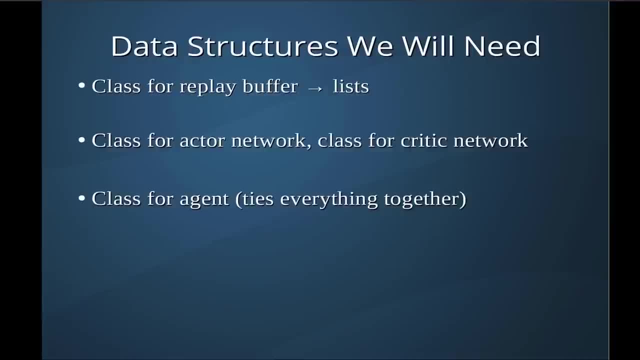 class for agent that's going to tie everything together. that'll have actor- everything together. that'll have actor- everything together. that'll have actor and critics that invoke actor and critic and critics that invoke actor and critic and critics that invoke actor and critic. constructors, as well as a memory for 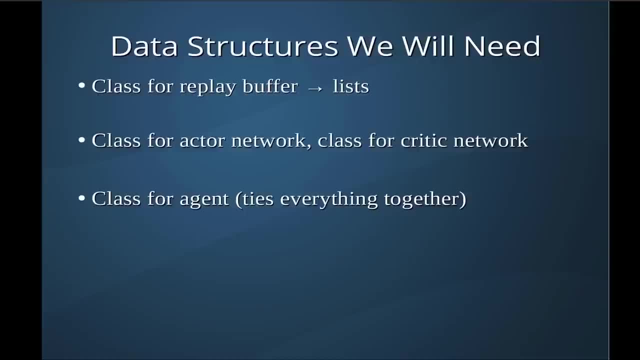 constructors, as well as a memory for constructors, as well as a memory for storing the appropriate data. it also storing the appropriate data. it also storing the appropriate data. it also functions for choosing actions: storing functions for choosing actions. storing functions for choosing actions, storing memories, saving models and learning from. 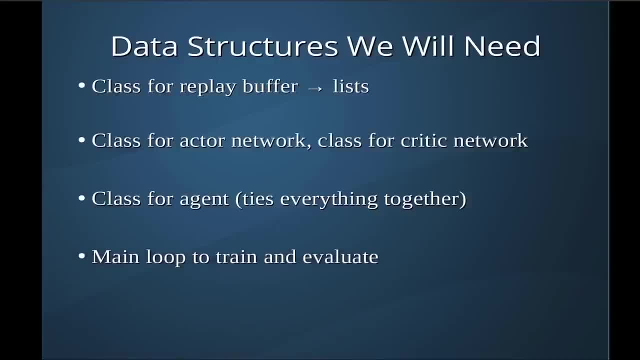 memories saving models and learning from memories, saving models and learning from its experiences, and in a separate file, its experiences and in a separate file, its experiences and in a separate file. we're gonna have a main loop to train. we're gonna have a main loop to train. 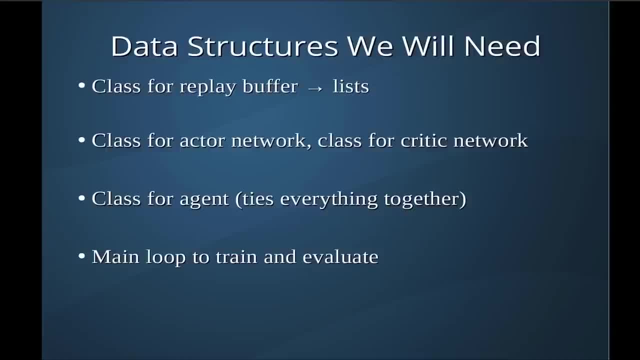 we're gonna have a main loop to train, which is also linked in the description, which is also linked in the description, which is also linked in the description below. if you want to come hang out below, if you want to come hang out below, if you want to come hang out with some really, really smart people who 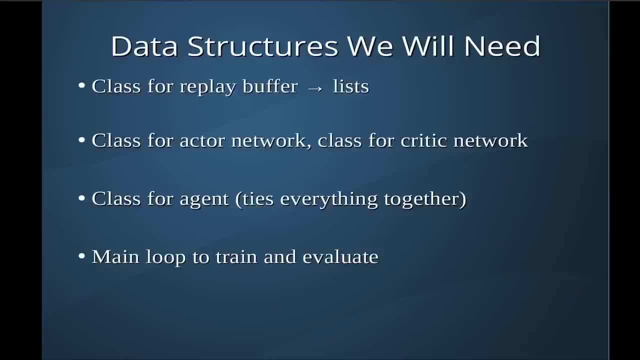 with some really really smart people who, with some really really smart people who talk about, talk about, talk about artificial intelligence: ranging from all artificial intelligence, ranging from all artificial intelligence, ranging from all sorts of different things, every single sorts of different things, every single sorts of different things every single day. check that link in the description. 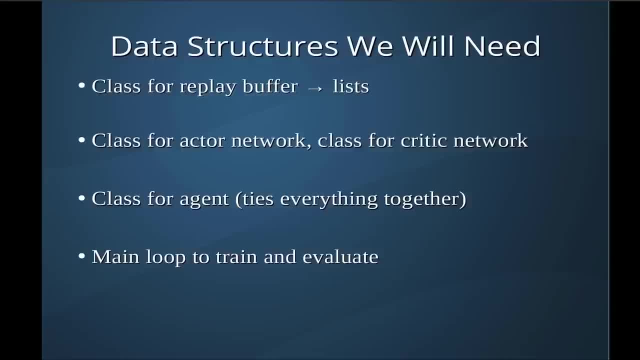 day. check that link in the description day. check that link in the description for the discord. so william came to me for the discord. so william came to me for the discord. so william came to me and said: hey, phil, i found an implementation of ppo that i find to be in line with your general philosophy of software minimalism. 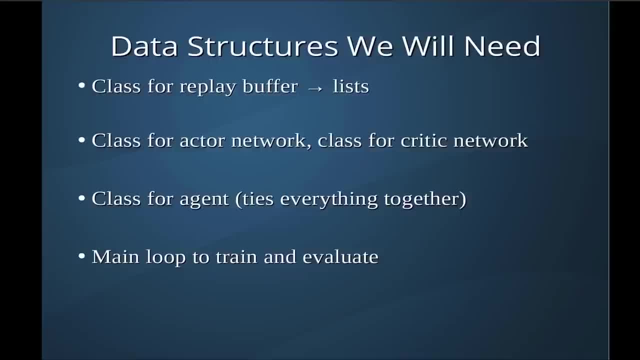 and he showed it to me and i looked at it and it helped clarify quite a few questions i had after reading the paper. now the software you see here is pretty much my own code, but it was inspired by william woodall's code, so shout out to him for helping me out on this, because the paper 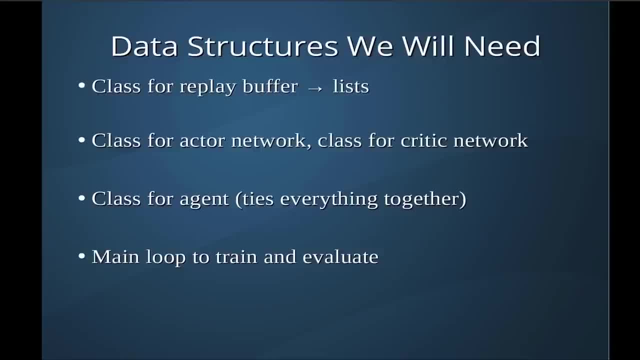 really isn't all that clear to me, even after reading it a few times. other thing i want to say- and i'll talk a little bit more about this in the coding section- is that when i normally define deep neural networks, actors and critics in particular, i will use the convention of saying: 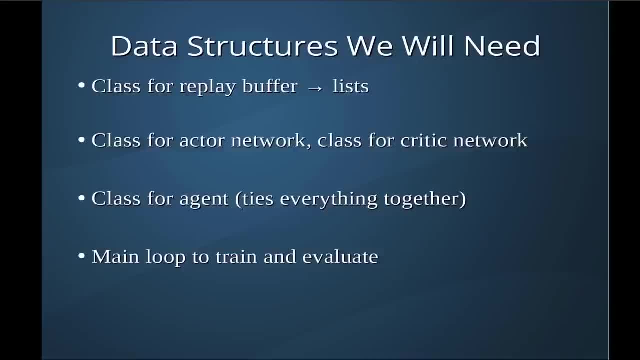 selflayer name equals nnlinear. selflayer name next, you know, equals nnlinear. and then i'll write the feed forward function where you use the member variables, that selflayer one, as something you can call as an object to call and then calling activation functions within that. now what i found is that doesn't really work very well. in fact i have to. 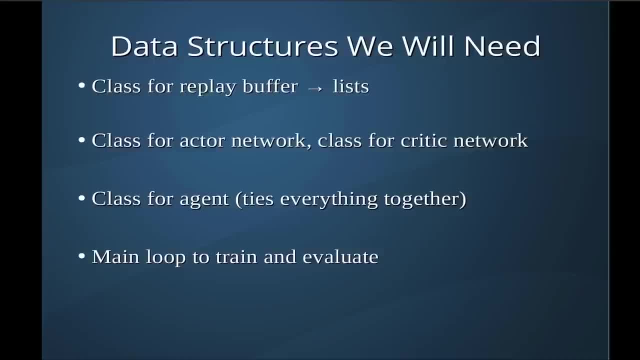 use nnsequential to create the models for this, and that's one of the biggest takeaways i had from william woodall's code is that, uh, by using the nnsequential you really get this thing to work and, for whatever reason, i cannot get as good a performance using my conventional 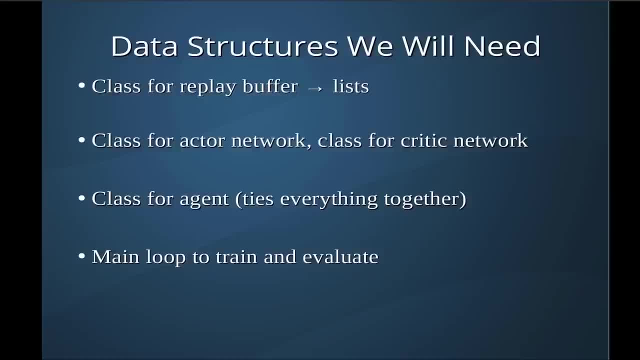 typical way of writing these networks. now that i can't think of any reason why that should be the case, but it is something i've observed. i tested it. uh, just altering that one chunk of code- how i define the models, and running it several times to take into account run to run. 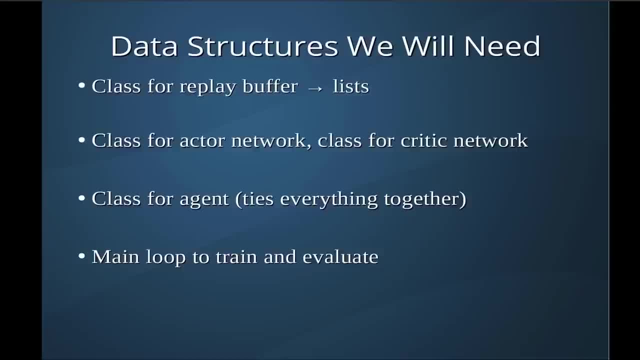 variation, and it seems to be repeatable for me. so maybe i don't know, maybe it's a configuration issue on my system, maybe it's something i'm doing wrong elsewhere. i don't know, i don't think. so all of that out of the way, let's go ahead and get into the coding portion. 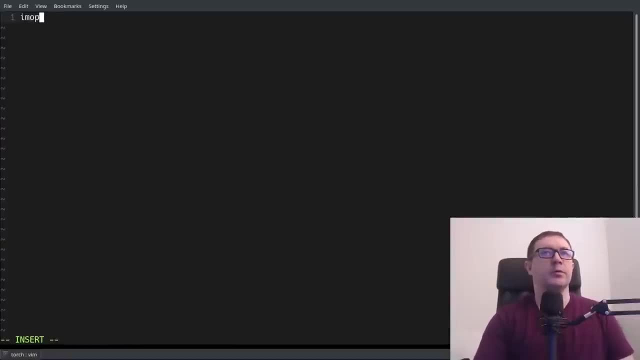 all right, so let's go ahead and jump right into it with our imports. they're going to be pretty light. we'll need os to handle file joining operations for numpy type stuff and all of the torch packages. we'll need an end for our sequential model. we will need optim and we will also need our categorical distribution. 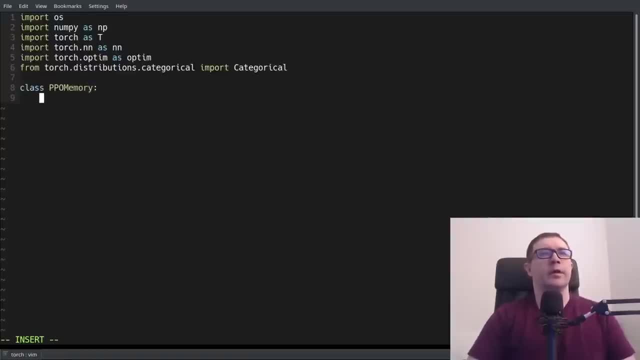 so we'll start with our ppo memory class, and this will be pretty simple for the most part. the only input for our constructor is a batch size and we will just implement the memory with lists. so we'll keep track of the states encountered, the log probes- i'll just call it problems for brevity- the values that our critic calculates. 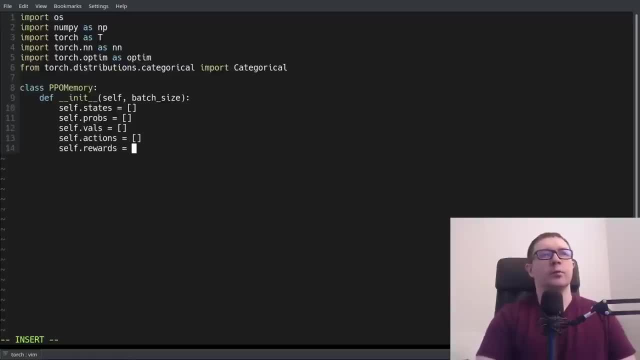 the actions we actually took, rewards received and the terminal flags. so next we need our function to generate our batches. so our strategy is going to be the following: we're going to have a list of integers that correspond to the indices of our memories and then we're going to have batch size chunks of those memories. so 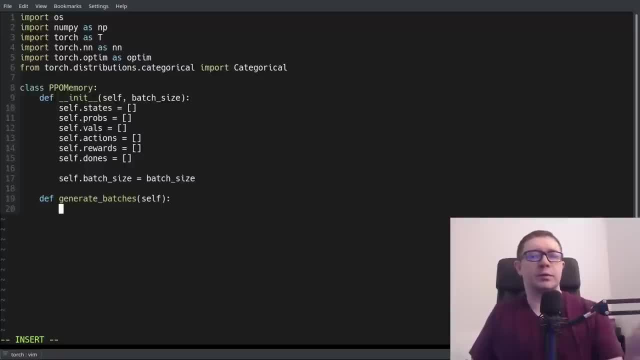 indices from 0 to, say, 4, and then 5 to 10, so on and so forth, or whatever our batch size is. we're going to shuffle up those values, so we're just going to have a list of those numbers and then we're not. 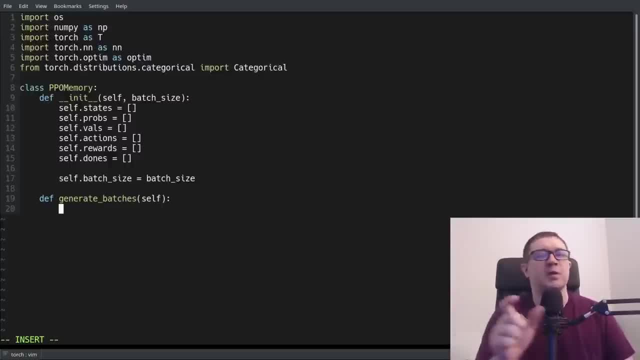 going to do anything else. we're just going to have the memory index and we're just going to put in the to shuffle those indices and take those batch size chunks of those shuffled indices. So the first thing we need to know are the number of states we are going to want to get our batch. 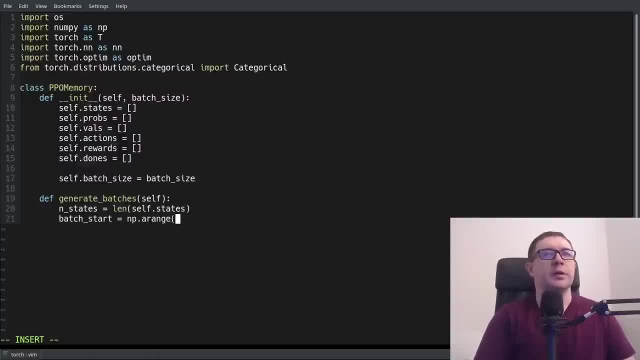 start list or array. I suppose that'll go from zero to and states and batch size, steps, batch size. it would help if I could type our indices And that is just the number of states in our trajectory. We're going to want to shuffle that so that we handle the stochastic part of the mini. 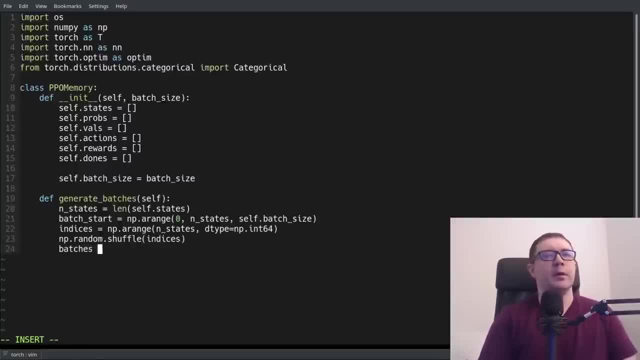 batch and stochastic gradient ascent, And then we can go ahead and take our batches using a list comprehension. So it's going to be those indices- I to I, plus self dot batch size for i in rain, for i in batch start. So it's going to take all of the 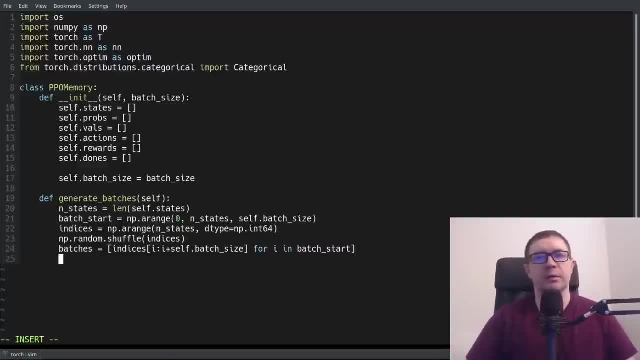 possible starting points of the batches, either 05, 10, etc. And go for in the indices from that all the way up to i plus batch size. So we're going to get the whole batch from our indices And then we're going to want to return an array for each of those And this gets a little bit. 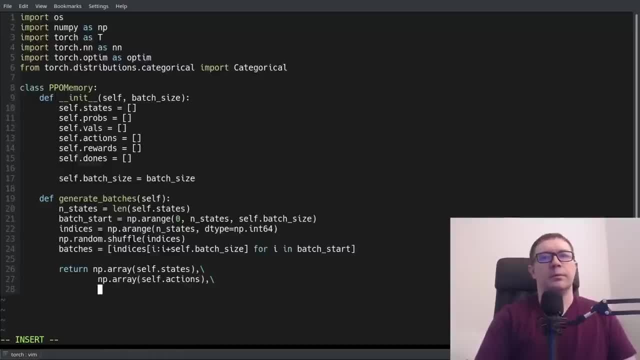 messy. So we're going to want to return an array for each of those, And this gets a little bit messy. I have to be very careful not to mess up the order, because of course, the order in which you return the memories definitely matters. later on We'll need rewards, And then we're also going. 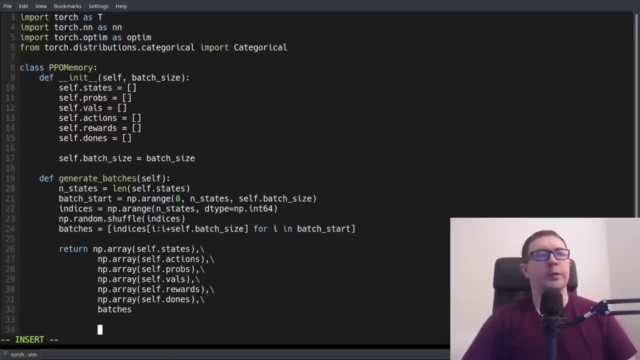 to want to return the batches, And the reason why will become apparent later. it's because we're returning the entire array here and we're going to want to iterate over the batches. So now we need a function to store a memory And that'll take a state, action, probability, value, reward and done. 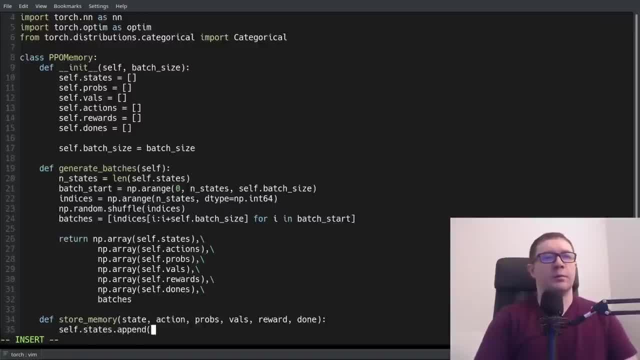 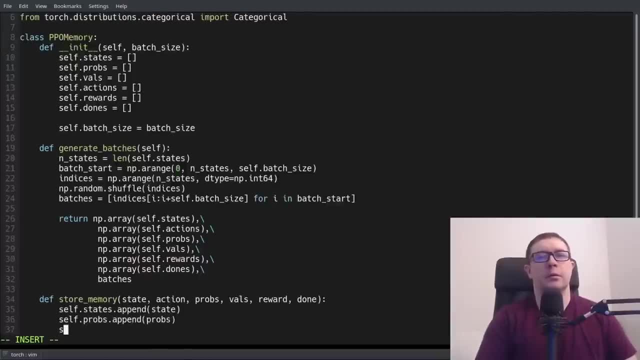 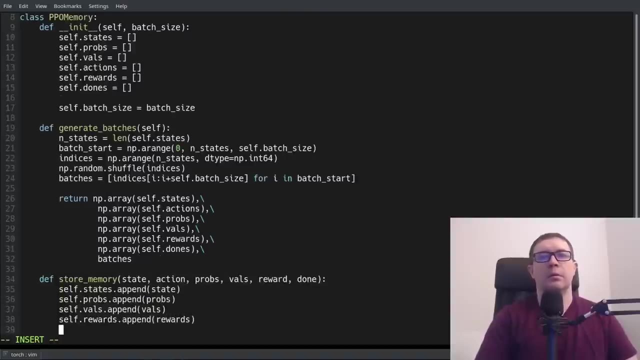 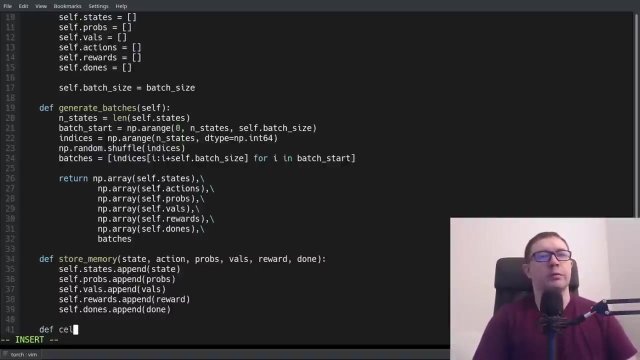 as input, And all we're going to do is append each of those elements to the respective list. That is reward singular. And then, finally, we need a function to clear the memory at the end of every trajectory, And I forgot the self argument here. 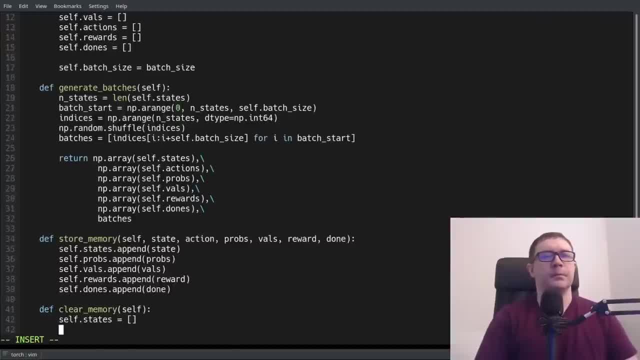 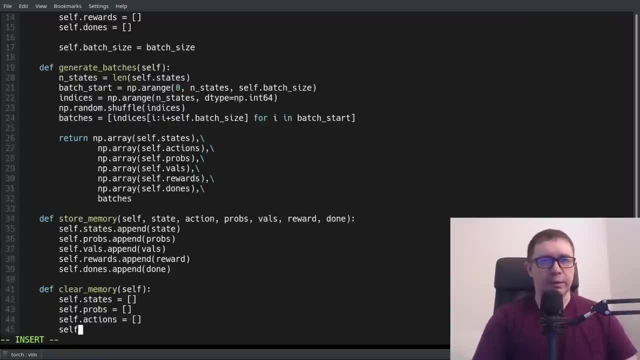 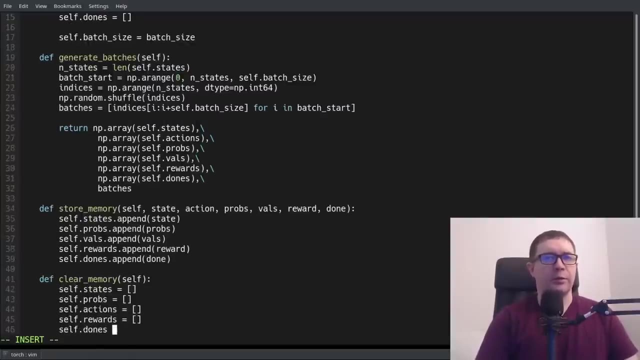 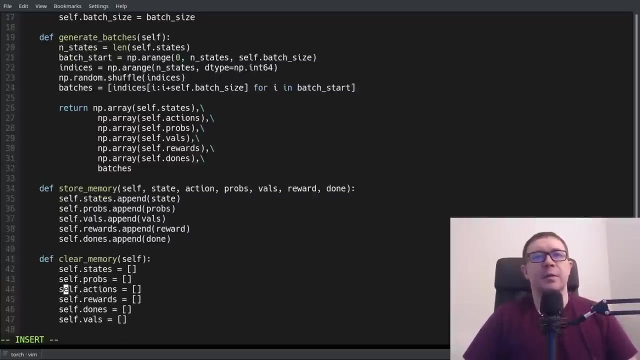 And mini rant here: I really don't like some aspects of Python. It took me much longer than I would care to admit to get this to run, Not because the algorithm I implemented was incorrect, but because I had a mismatch. So here I had, I believe, action, And up here it was actions, or perhaps. 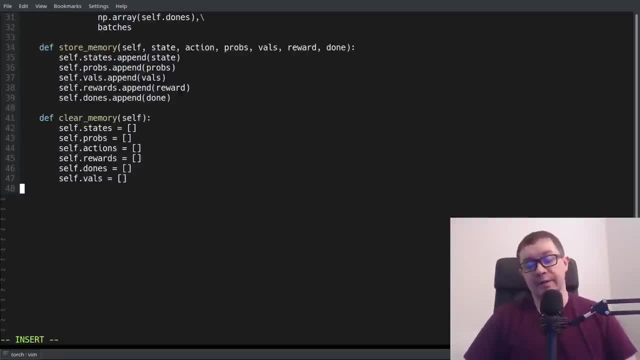 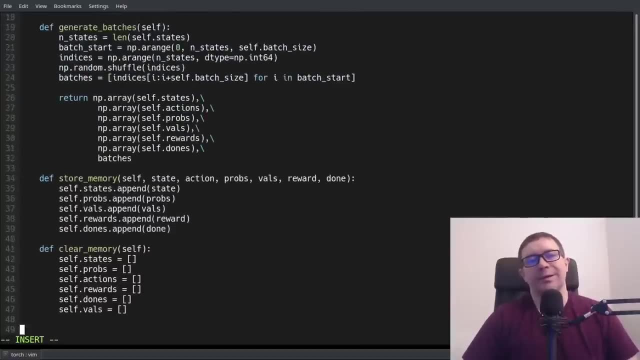 vice versa in my original implementation. So I'm going to go ahead and do that And I'm going to run the actual implementation. So it didn't flag as an error, because it's not really an error, particularly where Python is concerned, And so it was quite a nuisance, Pretty, pretty painful. 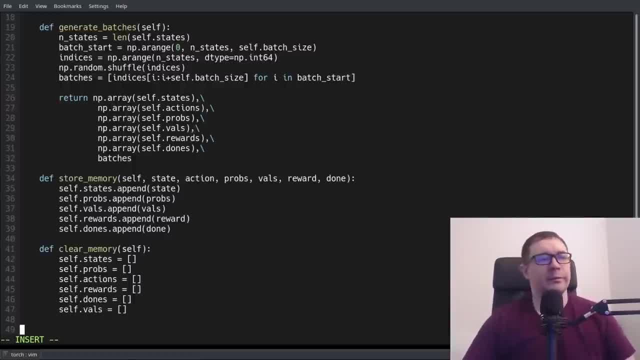 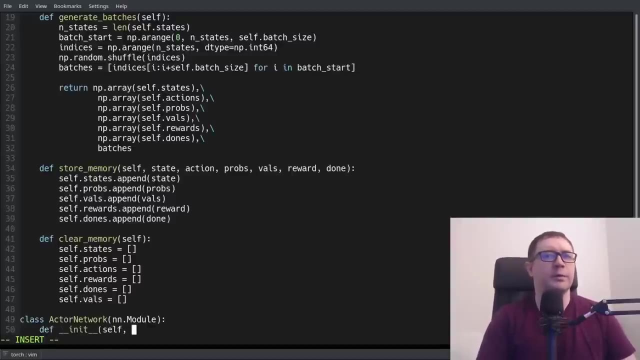 to track that down. Of course, if we're more strongly typed language, then that wouldn't be an issue, But I digress. So now let's handle our actor network And that will derive from the base nnmodule class. Our initializer is going to be pretty strong and we're going to have to 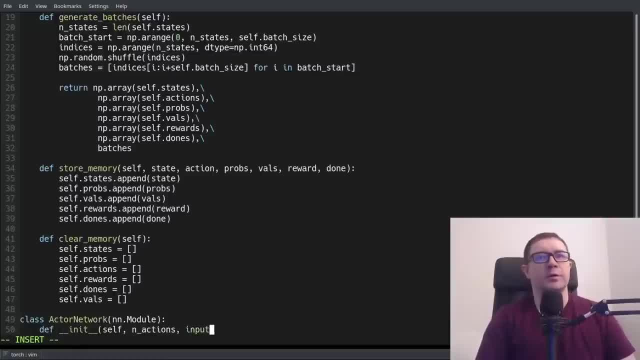 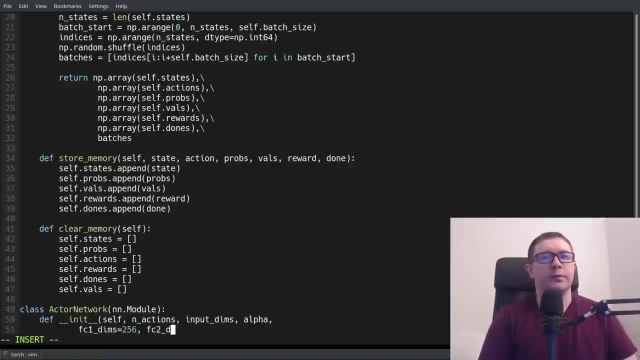 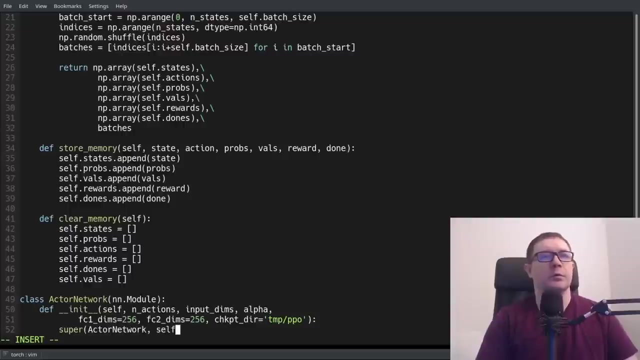 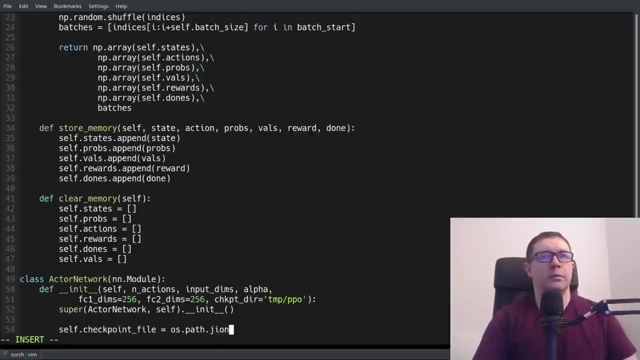 straightforward for actor. we will need the number of actions, the input dims, a learning rate, alpha number of fully connected dims for the first and second fully connected layers and a checkpoint directory. and we're also going to need to call our super constructor and then create our checkpoint file, checkpoint. 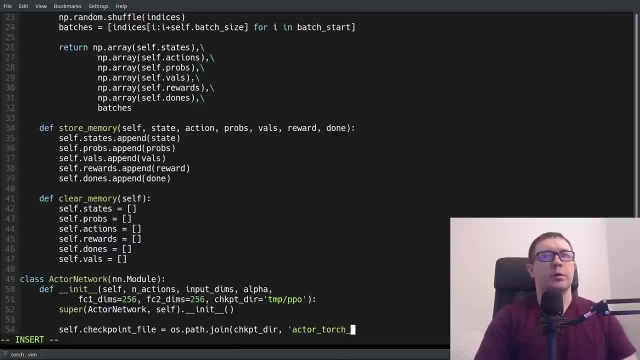 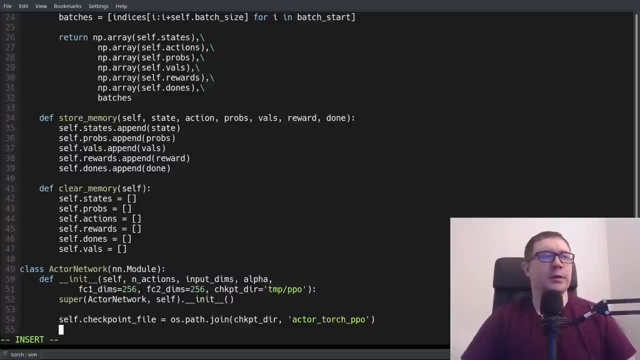 directory and actor torch PBO. now I do it this way because I'll often do development in a single root directory and I don't want to get models mixed up. if you have a different way, a more organized way of writing software, then you can do it in a single directory and you can do it in a single directory and 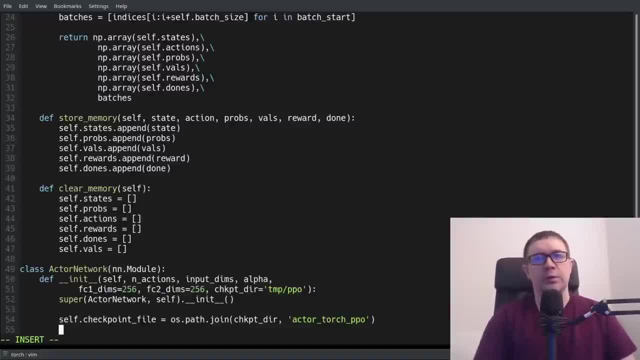 you can do it in a single directory and you can perhaps skip this path join. you can perhaps skip this path join. you can perhaps skip this path join. operation and just use a file by itself. operation and just use a file by itself. operation and just use a file by itself. but let's move on to the actual deep. 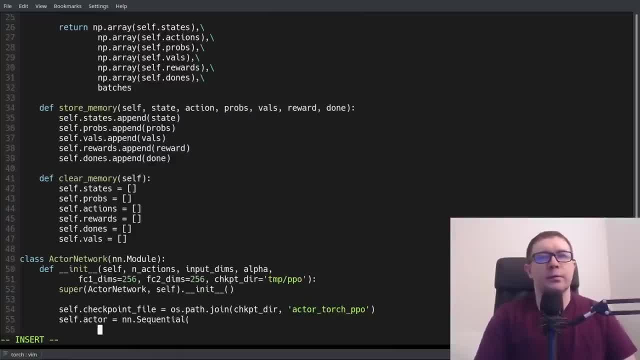 but let's move on to the actual deep. but let's move on to the actual deep neural network. we're gonna want a linear neural network. we're gonna want a linear neural network. we're gonna want a linear layer that takes star input- dims so layer that takes star input- dims so. 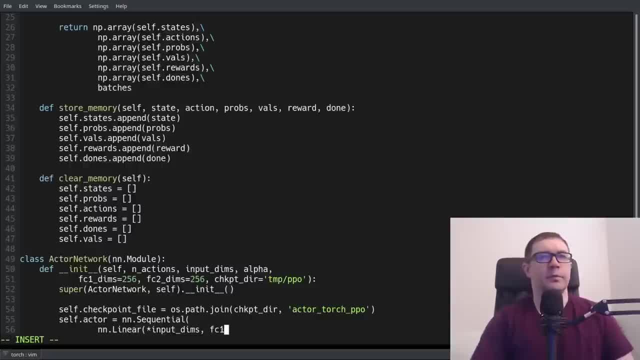 layer that takes star input dims. so we're gonna unpack the input dims. so we we're gonna unpack the input dims. so we we're gonna unpack the input dims. so we have to pass in a list and it's going to have to pass in a list and it's going to. 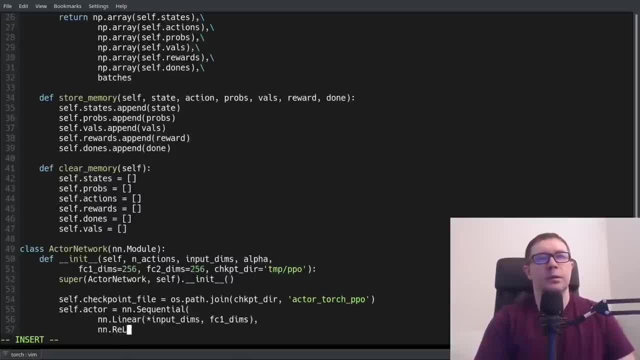 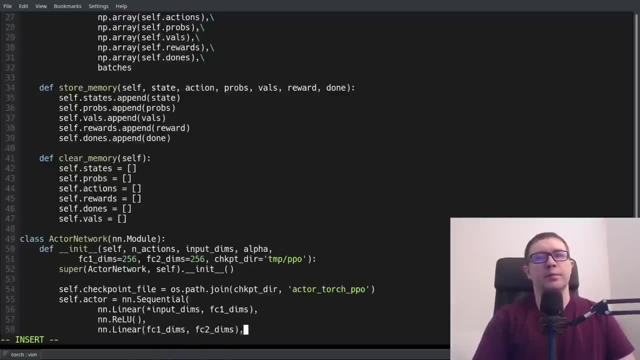 have to pass in a list and it's going to output: FC 1 dims, a relu activation output. FC 1 dims, a relu activation output. FC 1 dims, a relu activation function. another linear layer that takes function. another linear layer that takes function. another linear layer that takes FC 1 dims as input, now puts FC 2 dims. 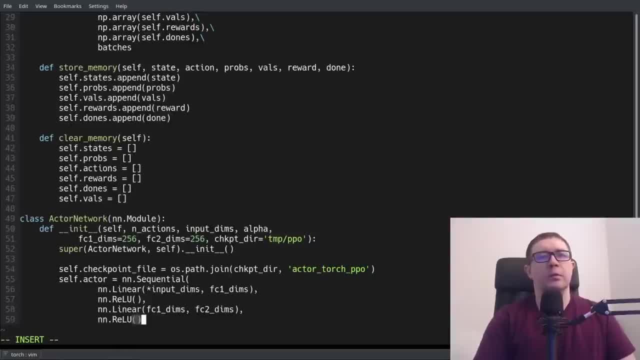 FC 1 dims as input, now puts FC 2 dims. FC 1 dims as input, now puts FC 2 dims. that gets a relu activation as well. that gets a relu activation as well. that gets a relu activation as well. another linear layer that takes FC 2. 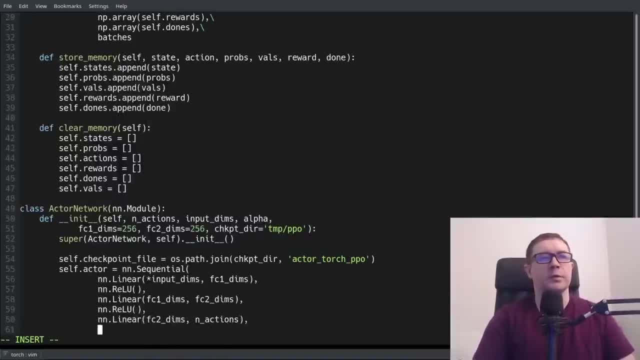 another linear layer that takes FC 2. another linear layer that takes FC 2: dims as inputs and outputs. a number of dims as inputs and outputs. a number of dims as inputs and outputs. a number of actions, and then we're gonna use a soft actions and then we're gonna use a soft. 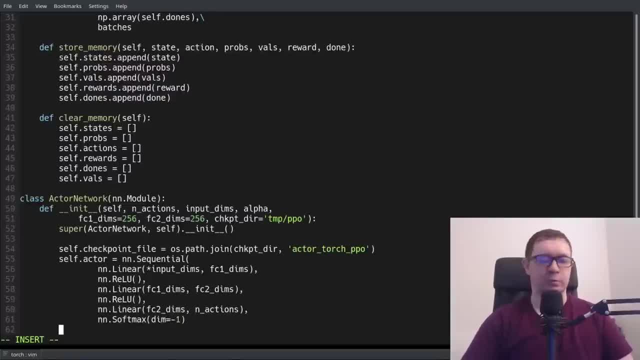 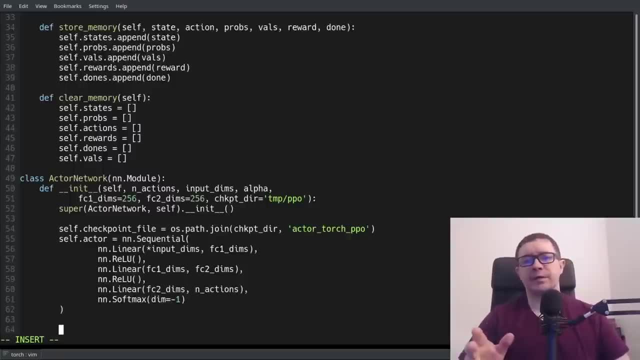 actions. and then we're gonna use a soft max activation along the minus 1 max activation along the minus 1 max activation along the minus 1 dimension. so that's the whole of our dimension, so that's the whole of our dimension, so that's the whole of our actor network. the soft max takes care of. 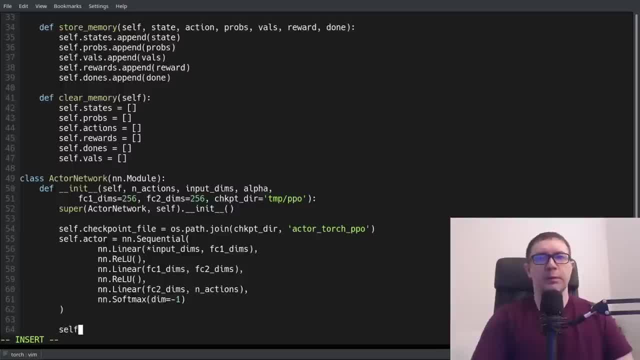 actor network. the soft max takes care of actor network. the soft max takes care of the fact that we're dealing with the fact that we're dealing with the fact that we're dealing with probabilities and they have to sum to 1: probabilities and they have to sum to 1. 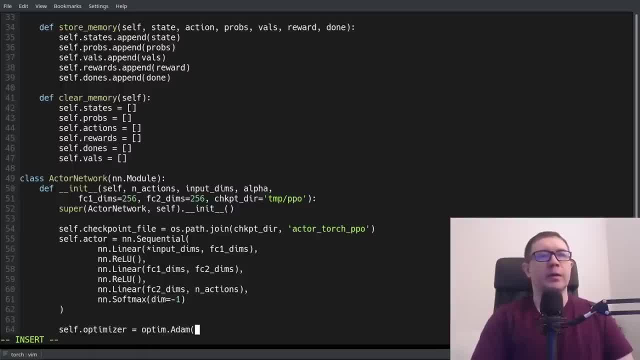 probabilities and they have to sum to 1. so our optimizer is going to be an atom. so our optimizer is going to be an atom. so our optimizer is going to be an atom optimizer. what are we going to optimize optimizer? what are we going to optimize optimizer? what are we going to optimize the parameters with learning rate of? 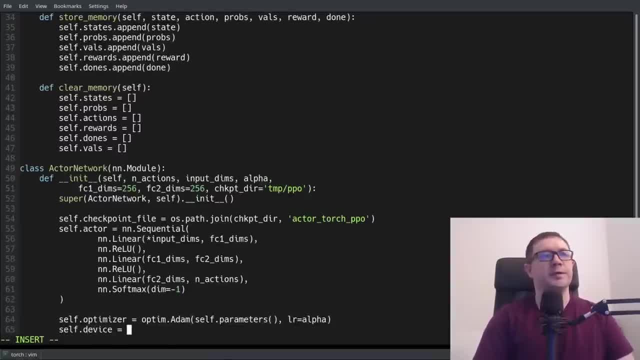 the parameters with learning rate of the parameters, with learning rate of alpha. of course we need to handle the alpha. of course we need to handle the alpha. of course we need to handle the device which would be our GPU if possible, device which would be our GPU if possible. 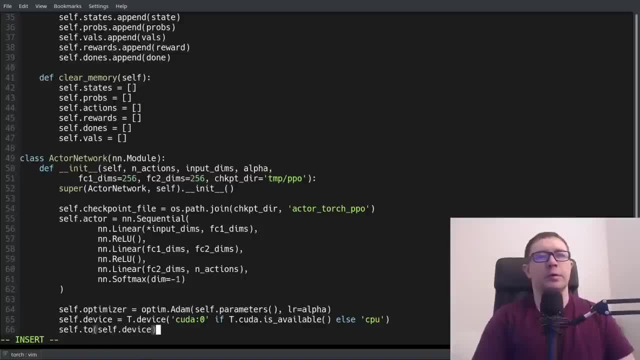 device, which would be our GPU, if possible. then we want to send the entire network. then we want to send the entire network. then we want to send the entire network to the device. next we have our feed to the device. next we have our feed to the device. next we have our feed forward function and that'll take a. 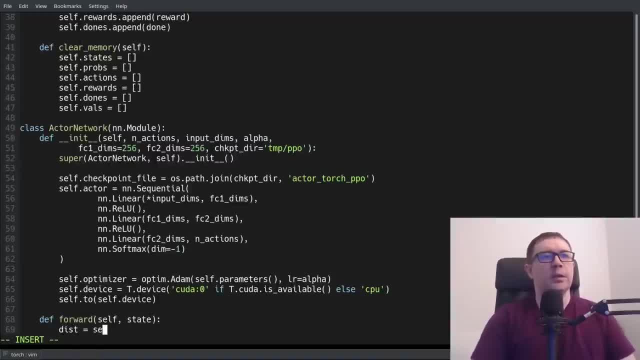 forward function and that'll take a forward function and that'll take a single state or batch of states as input. single state or batch of states as input, single state or batch of states as input. so we want to pass, so we want to pass, so we want to pass that state through our new deep neural. 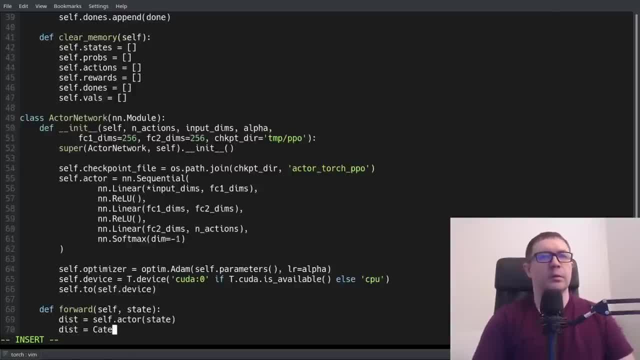 that state through our new deep neural, that state through our new deep neural network and get the distribution out and network and get the distribution out and network and get the distribution out and then use that to define a categorical, then use that to define a categorical, then use that to define a categorical distribution which we are going to 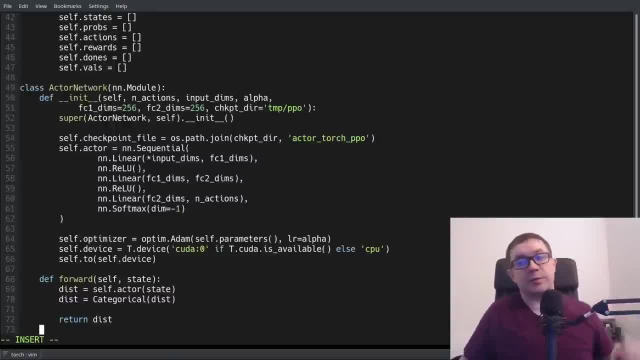 distribution which we are going to, distribution which we are going to return. so what this is doing is it is return. so what this is doing is it is return. so what this is doing is it is calculating a series of probabilities, calculating a series of probabilities, calculating a series of probabilities that we're going to use to draw from a 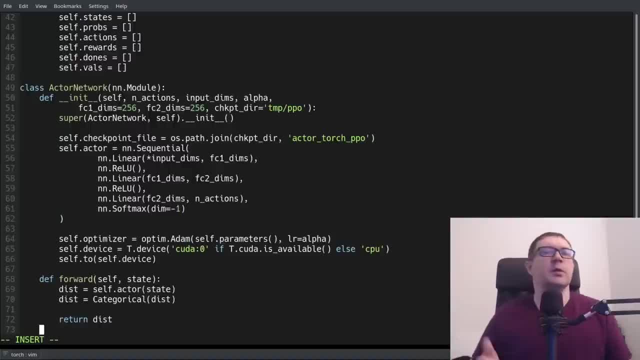 that we're going to use to draw from a, that we're going to use to draw from a distribution to get our actual action distribution, to get our actual action distribution, to get our actual action, and then we can use that to get the log, and then we can use that to get the log. 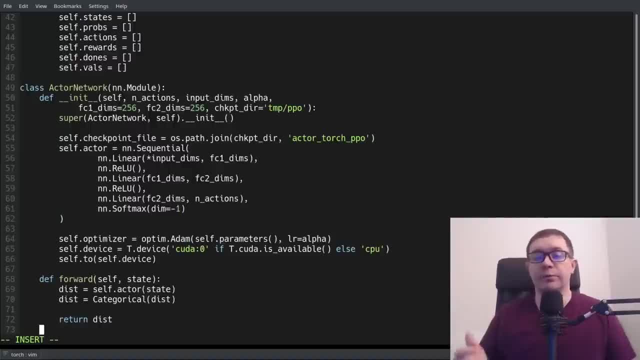 and then we can use that to get the log probabilities for the calculation of the probabilities, for the calculation of the probabilities, for the calculation of the ratio of the two probabilities in our ratio, of the two probabilities in our ratio of the two probabilities in our update for our learning function. then we 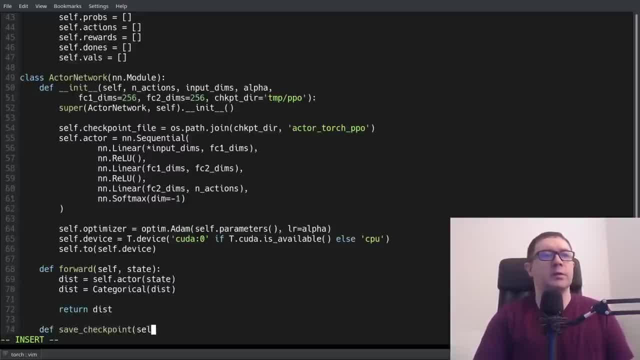 update for our learning function. then we update for our learning function. then we have a couple of bookkeeping functions. have a couple of bookkeeping functions. have a couple of bookkeeping functions. save checkpoint now we're going to want. save checkpoint now we're going to want. 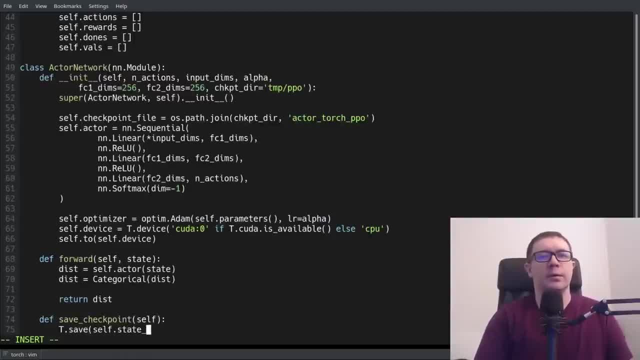 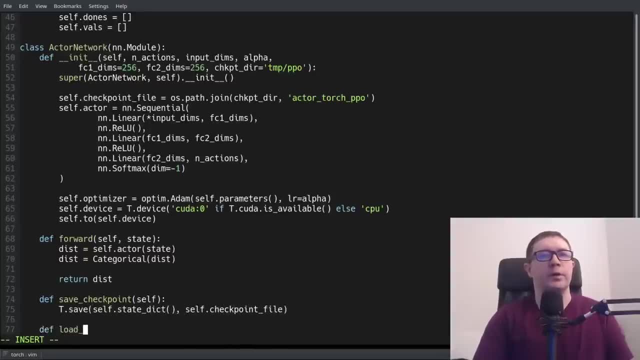 save checkpoint. now we're going to want to say torch dot, save state dictionary. to say torch dot, save state dictionary. to say torch dot, save state dictionary for our network, and we're going to say for our network and we're going to say for our network, and we're going to say that into a checkpoint file. then we need 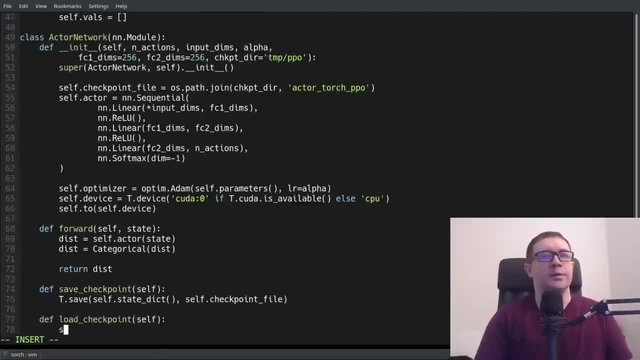 that into a checkpoint file, then we need that into a checkpoint file. then we need a load checkpoint and that is self dot a load checkpoint, and that is self dot a load checkpoint. and that is self dot load state dictionary. what are we going? load state dictionary. what are we going? 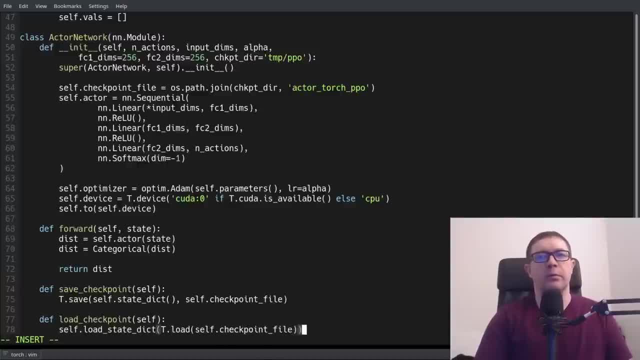 load state dictionary. what are we going to load? a checkpoint file. and that's to load a checkpoint file. and that's to load a checkpoint file. and that's really it for the actor network. it's really it for the actor network. it's really it for the actor network. it's pretty straightforward. the critic network. 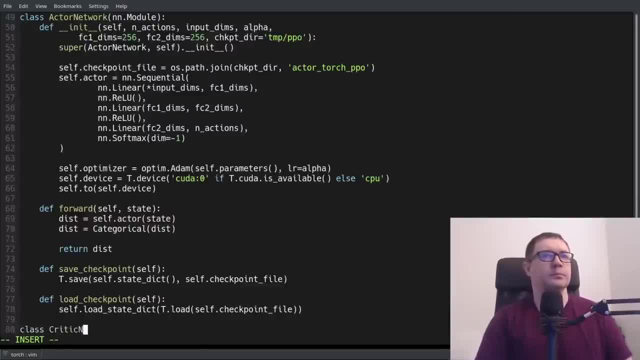 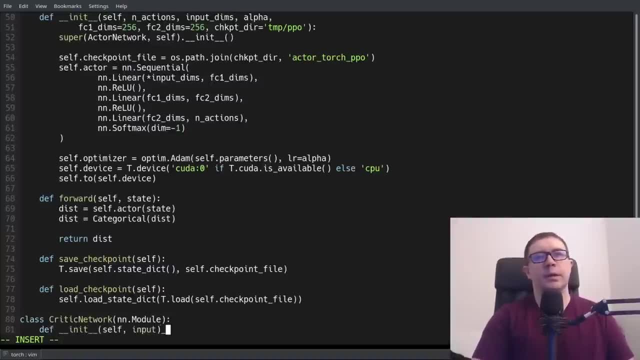 pretty straightforward. the critic network pretty straightforward. the critic network is also straightforward, and that also is also straightforward, and that also is also straightforward and that also derives from an end up module, derives from an end up module, derives from an end up module. here we don't need the number of actions. 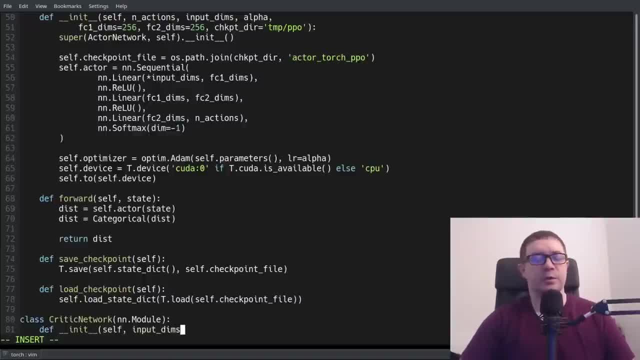 here we don't need the number of actions. here we don't need the number of actions because the output of the critic is, because the output of the critic is, because the output of the critic is single-valued, it just outputs the value. single-valued, it just outputs the value. 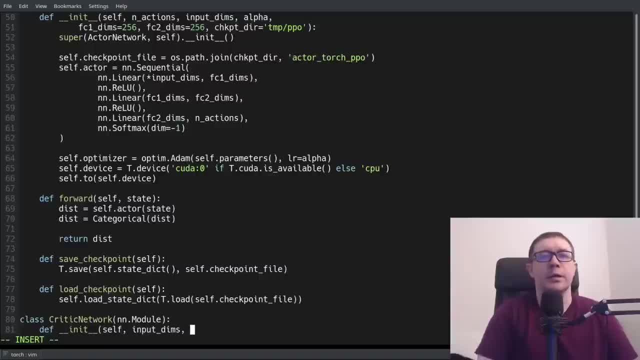 single-valued. it just outputs the value of a particular state, so it doesn't of a particular state. so it doesn't of a particular state. so it doesn't care how many actions there are in the care, how many actions there are in the care, how many actions there are in the action space. but it does need a. 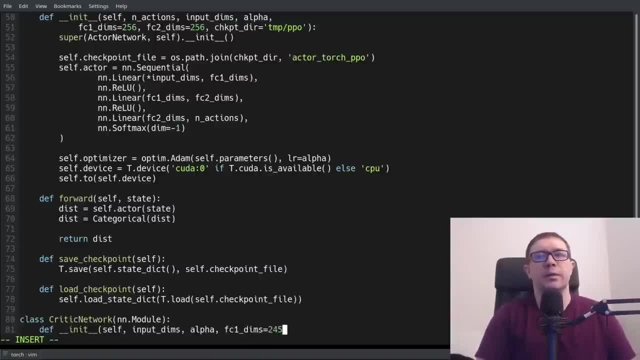 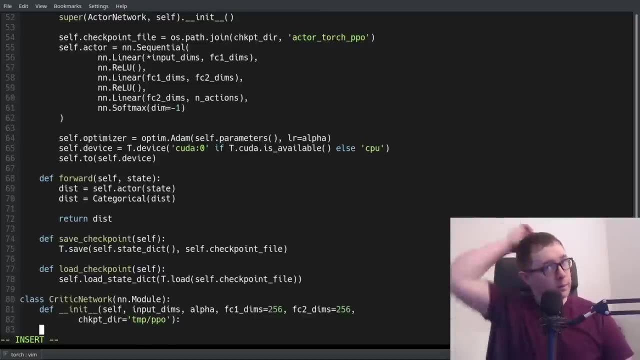 action space. but it does need a action space. but it does need a learning rate alpha. it does need some learning rate alpha. it does need some learning rate alpha. it does need some dimensions to 56 and a checkpoint dimensions to 56 and a checkpoint dimensions to 56 and a checkpoint directory. and then we need to call the. 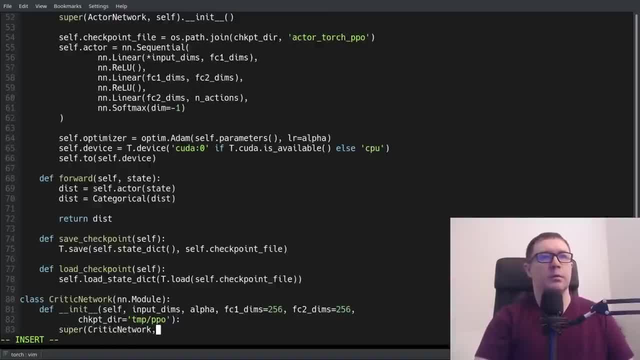 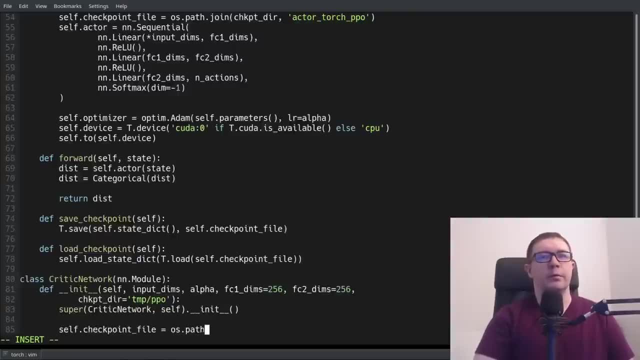 directory, and then we need to call the directory, and then we need to call the super constructor and same deal, the super constructor and same deal, the super constructor and same deal, the checkpoint file, the check point checkpoint file, the check point checkpoint file, the check point directory and critic torch. so that way: 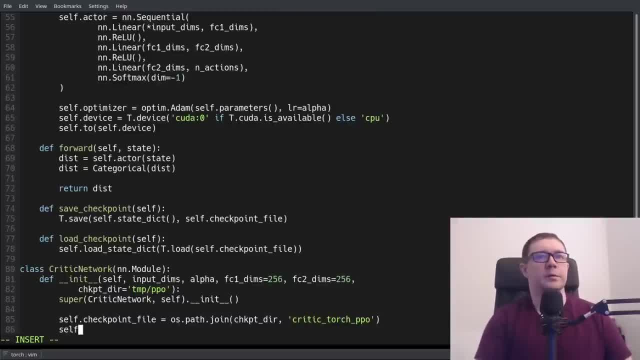 directory and critic torch. so that way, directory and critic torch. so that way we can differentiate between the actor, we can differentiate between the actor, we can differentiate between the actor and critic model files and critic model files and critic model files. and we will again use the sequential model. 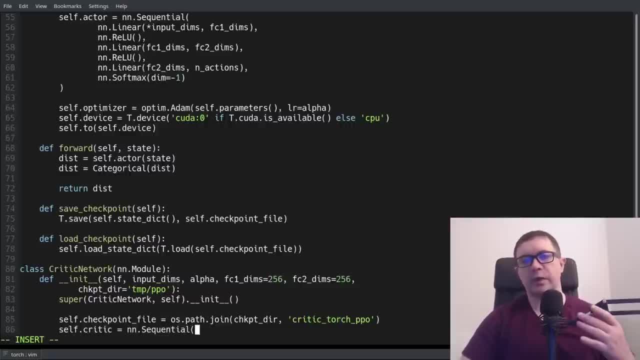 and we will again use the sequential model, and we will again use the sequential model, and so in the shout-out I was, and so in the shout-out I was, and so in the shout-out I was talking about William Woodall's implementation, talking about William Woodall's implementation. 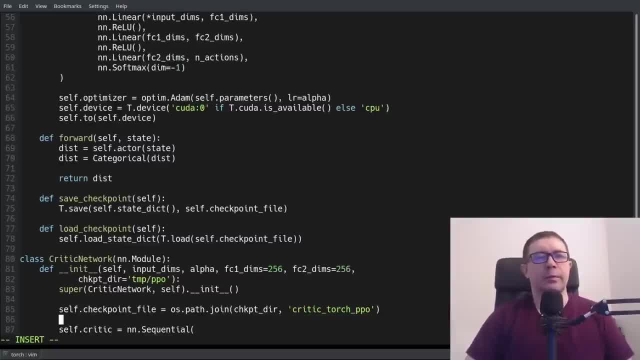 talking about William Woodall's implementation as well as something else. I as well as something else, I as well as something else. I observed so what I meant by the alternate method observed. so what I meant by the alternate method observed, so what I meant by the alternate method of doing a model, was, if you say: 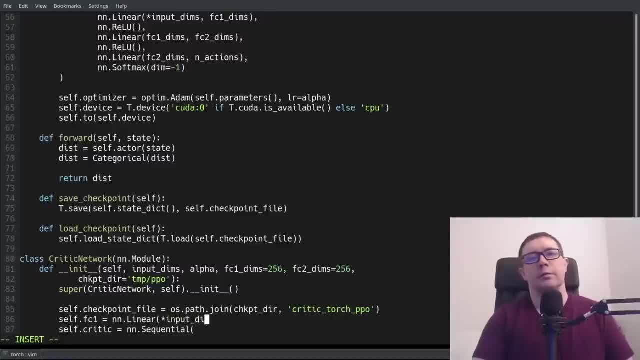 of doing a model was. if you say of doing a model was, if you say selffc1 and in linear, you know if you selffc1 and in linear you know if you selffc1 and in linear you know if you do it that way. have FC 1, FC 2, the. 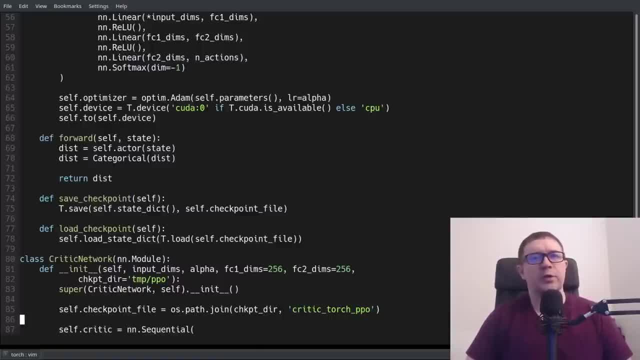 do it that way. have FC 1, FC 2, the. do it that way: have FC 1- FC 2, the separate layers defined. without the separate layers defined, without the separate layers defined, without the sequential model. it actually does sequential model. it actually does sequential model. it actually does significantly worse than if you do it. 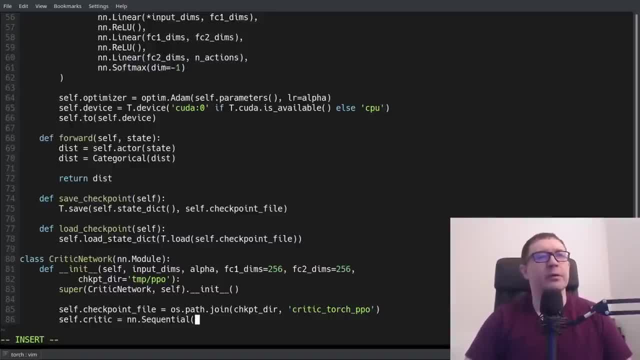 significantly worse than if you do it, significantly worse than if you do it with the sequential model. and I don't with the sequential model and I don't with the sequential model, and I don't know why I don't have a certainly, know why I don't have a certainly. 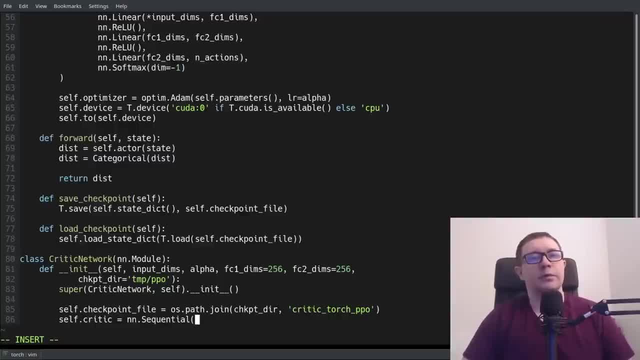 know why I don't have a. certainly there's no theoretical reason it should. there's no theoretical reason it should. there's no theoretical reason it should do it. it must be something under the do it. it must be something under the do it, it must be something under the hood, with the way in which pie torch is. 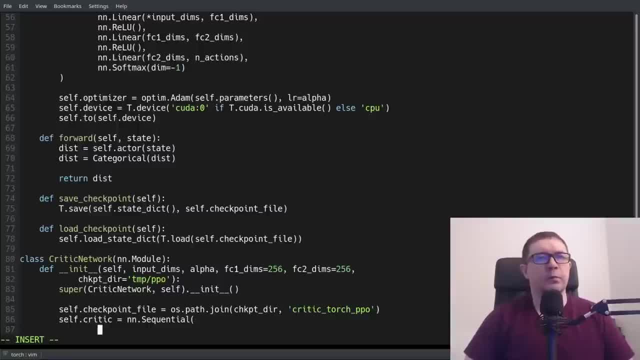 hood with the way in which pie torch is hood with the way in which pie torch is implementing things and it's no implementing things and it's no implementing things and it's no disrespect to the creators of pie torch, disrespect to the creators of pie torch, disrespect to the creators of pie torch. but this is one of my, you know, one of my. 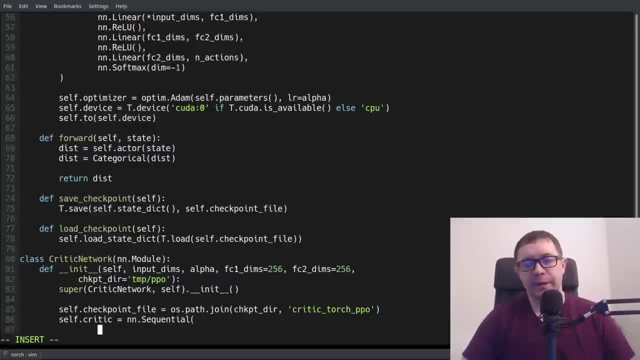 but this is one of my. you know one of my, but this is one of my. you know one of my biggest gripes with using these biggest gripes, with using these biggest gripes with using these third-party libraries- is you never know third-party libraries, is you never know? 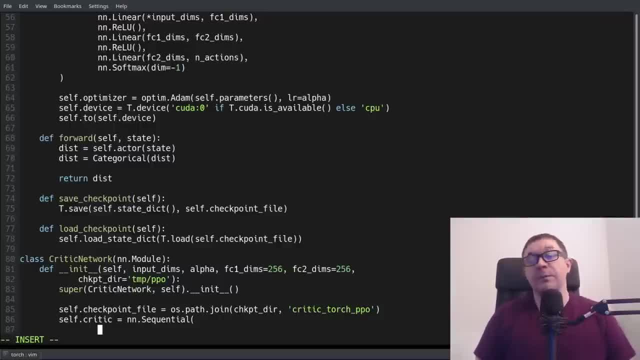 third-party libraries is you never know how they're implemented. so something how they're implemented, so something how they're implemented. so something doesn't operate the way you expect. you doesn't operate the way you expect. you doesn't operate the way you expect. you can certainly go look it up, it's. 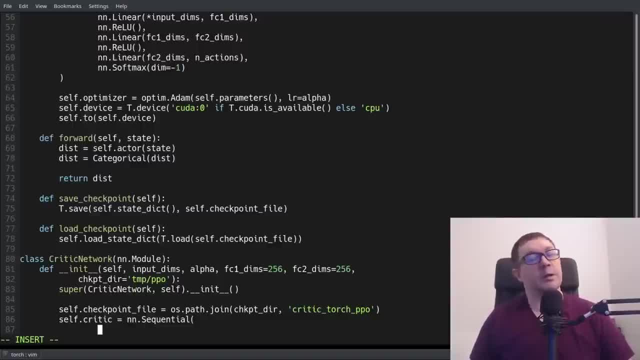 can certainly go look it up. it's can certainly go look it up. it's open source, but that is much easier said open source, but that is much easier said open source, but that is much easier said than done right. you have to be familiar than done right. you have to be familiar. 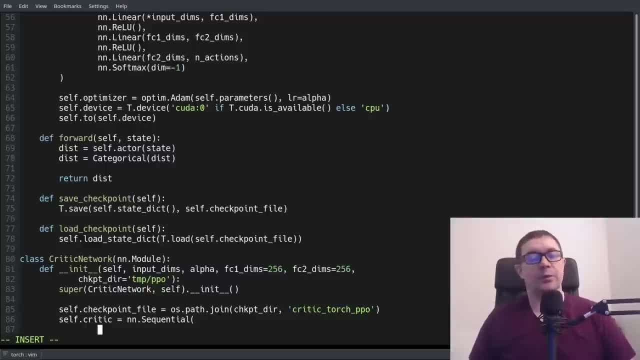 than done right. you have to be familiar with not the entire code base, but a with not the entire code base, but a with not the entire code base, but a really significant portion of it to be really significant portion of it, to be really significant portion of it to be able to make sense of a single file or a. 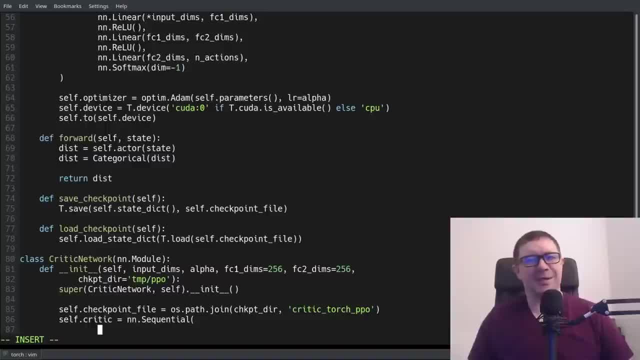 able to make sense of a single file or a able to make sense of a single file or a single way of doing things. so it really single way of doing things. so it really single way of doing things. so it really makes things opaque. it's an abstraction. 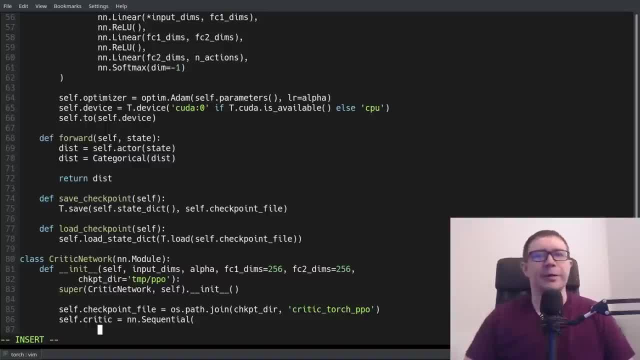 makes things opaque. it's an abstraction makes things opaque. it's an abstraction on top of an abstraction, and so I don't on top of an abstraction, and so I don't know. it's part of the good part of that. know it's part of the good part of that. 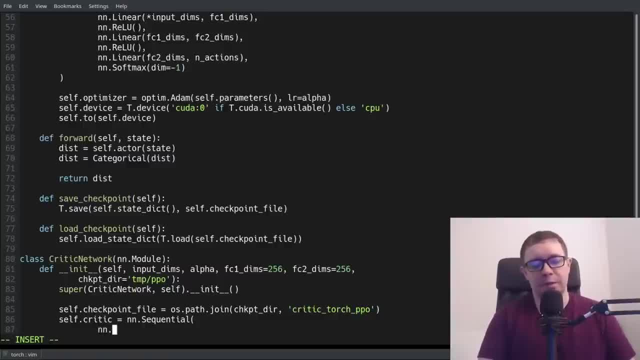 know. it's part of the good, part of that. it's the bad that comes with the good. it's the bad that comes with the good. it's the bad that comes with the good for having you know a robust library, for having you know a robust library. 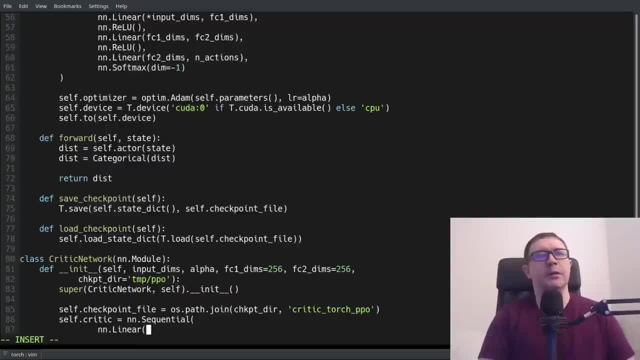 for having, you know, a robust library like pie torch. but I do it this way like pie torch, but I do it this way like pie torch, but I do it this way because it seems to work the best, and as. because it seems to work the best and as. 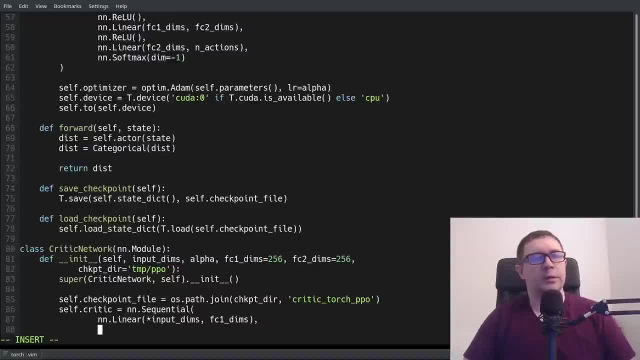 because it seems to work the best and as an aside, I also can't get it to work an aside, I also can't get it to work, an aside, I also can't get it to work very well in tensorflow 2 and I suspect very well in tensorflow 2 and I suspect 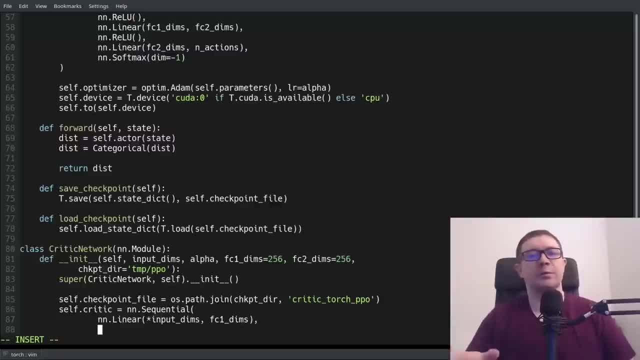 very well in tensorflow 2 and I suspect the. the reasons are related because the, the. the reasons are related because the, the. the reasons are related because the performance of the tensorflow 2 is on. performance of the tensorflow 2 is on. performance of the tensorflow 2 is on par with the type of performance I get. 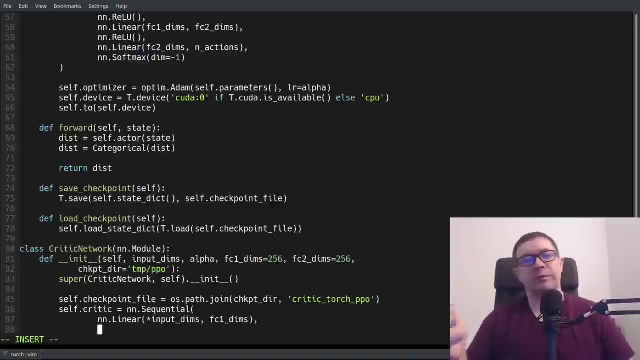 par with the type of performance I get. par with the type of performance I get from doing it the other way, where you from doing it the other way, where you from doing it the other way where you just define individual layers instead of just define individual layers instead of. 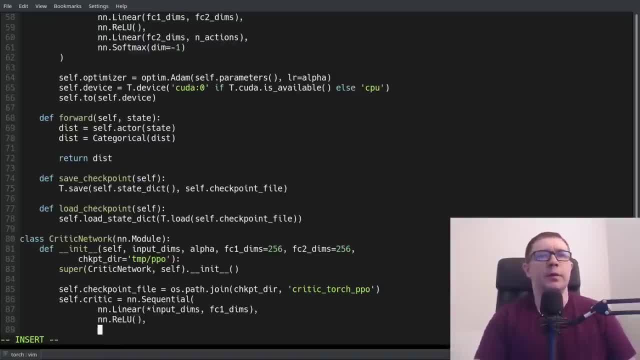 just define individual layers instead of a sequential model- so pretty interesting- a sequential model. so pretty interesting- a sequential model. so pretty interesting stuff. maybe one day I'll get super stuff. maybe one day I'll get super stuff. maybe one day I'll get super motivated and decide to go ahead and 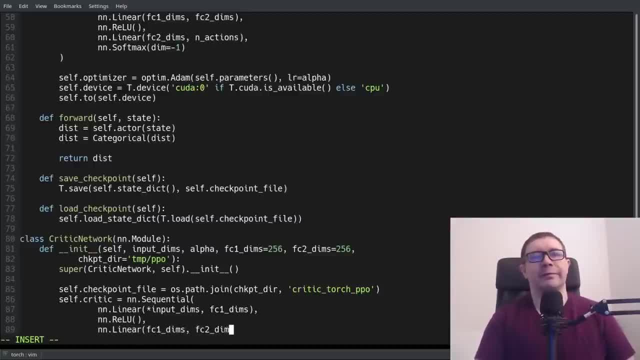 motivated and decide to go ahead. and motivated and decide to go ahead and figure it out, but I wouldn't hold my figure it out, but I wouldn't hold my figure it out, but I wouldn't hold my breath on that. so this is going to be a 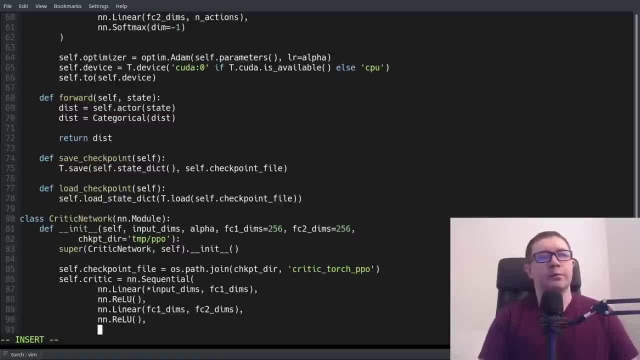 breath on that. so this is going to be a breath on that. so this is going to be a very similar model linear layers with very similar model linear layers with very similar model linear layers with value activations in between, the main value activations in between the main value activations in between. the main difference is that our output layer is 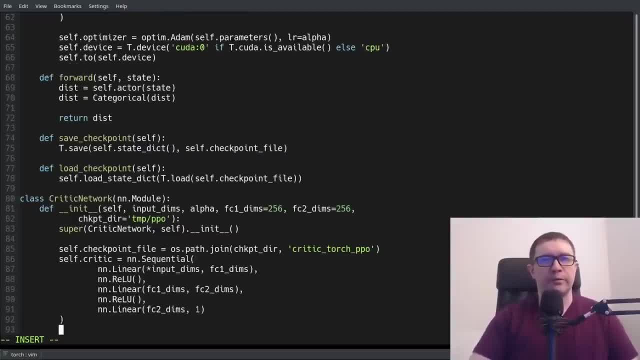 difference is that our output layer is. difference is that our output layer is going to be a linear layer, with no going to be a linear layer with no going to be a linear layer, with no activation and a single value output now. activation and a single value output now. 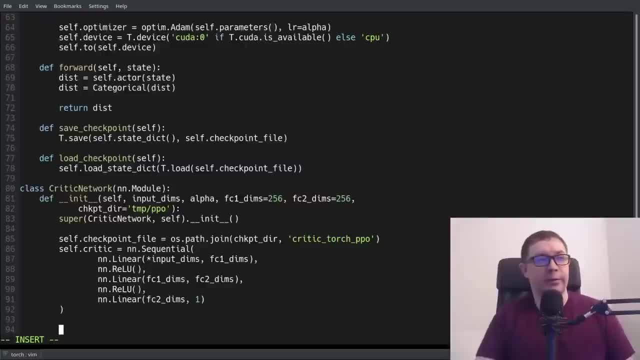 activation and a single value output. now, of course it handles the batch size. of course it handles the batch size. of course it handles the batch size automatically. so if you pass in a batch automatically, so if you pass in a batch automatically, so if you pass in a batch, you're gonna get a batch of outputs as. 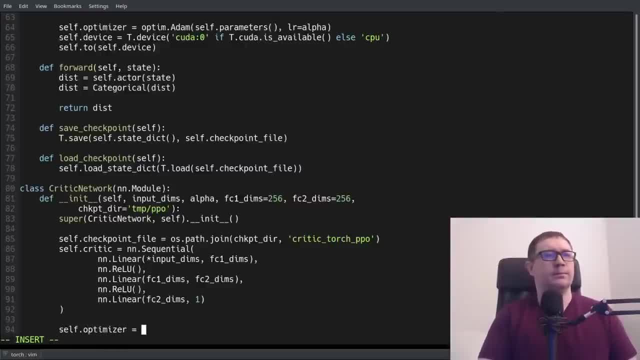 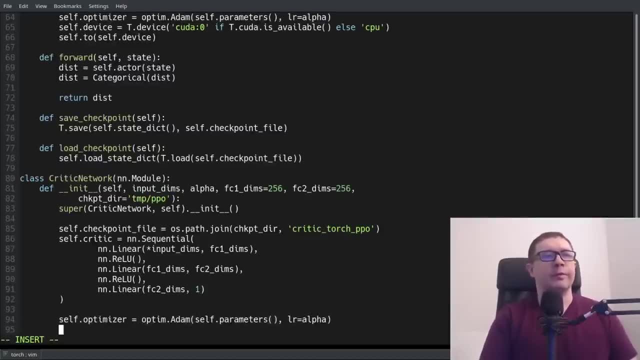 you're gonna get a batch of outputs, as you're gonna get a batch of outputs as well. again, we need our optimizer with well. again we need our optimizer with well. again, we need our optimizer with learning rate of Alpha as an aside about learning rate of Alpha. as an aside about. 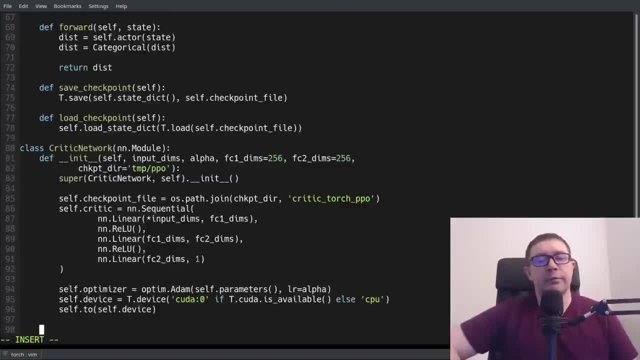 learning rate of Alpha. as an aside about the optimizer, I'm going to use this, the optimizer. I'm going to use this the optimizer. I'm going to use this same learning rate for both the actor, same learning rate for both the actor, same learning rate for both the actor and the critic, and it's entirely feasible. 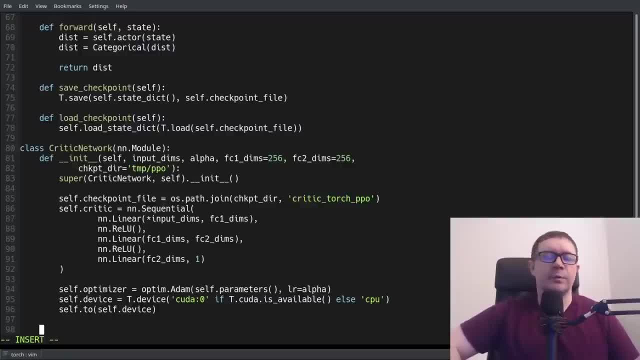 and the critic, and it's entirely feasible and the critic, and it's entirely feasible and possible and perhaps even advisable and possible, and perhaps even advisable and possible, and perhaps even advisable to use separate learning rates for both, to use separate learning rates for both, to use separate learning rates for both the actor and the critic, at least in 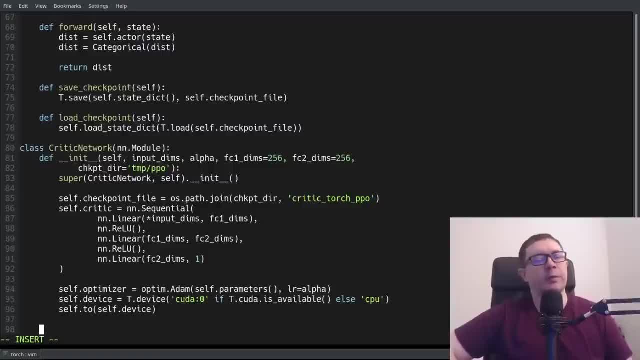 the actor and the critic, at least in the actor and the critic, at least in something like deep deterministic policy, something like deep deterministic policy, something like deep deterministic policy. gradients: you get away with a much gradients. you get away with a much gradients. you get away with a much larger, you know, by a factor of three or 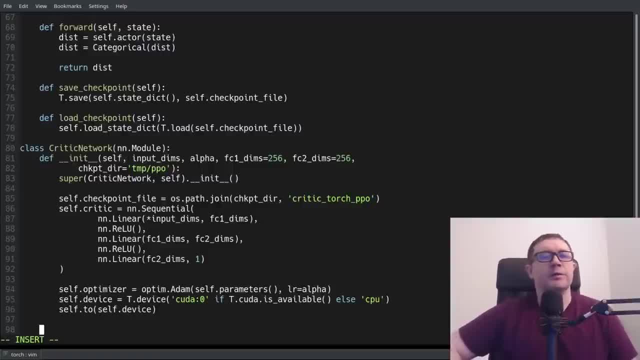 larger, you know by a factor of three or larger, you know by a factor of three or so, learning rate for your critic than so learning rate for your critic than so learning rate for your critic than you do. the actor, reason being as we. you do the actor, reason being as we. 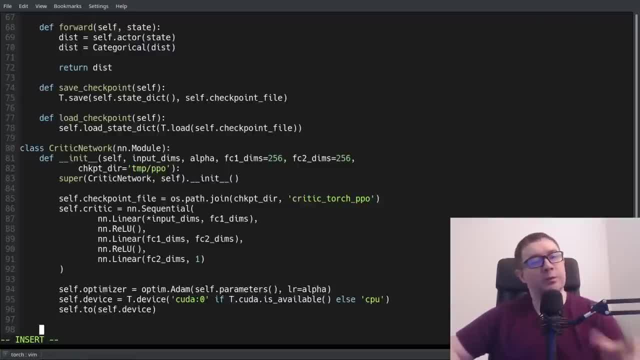 you do the actor. reason being: as we outlined the lecture, the actor is much outlined the lecture: the actor is much outlined. the lecture: the actor is much more sensitive to changes in the more sensitive to changes in the more sensitive to changes in the underlying parameters of its deep neural. 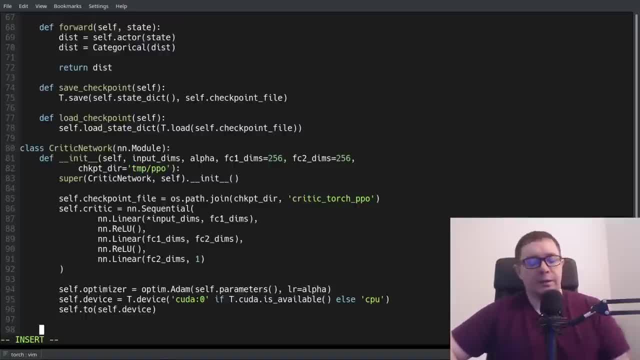 underlying parameters of its deep neural underlying parameters of its deep neural network now ostensibly, or network now ostensibly, or network now ostensibly, or theoretically, the the PPO method should, theoretically, the the PPO method should, theoretically, the the PPO method should account for that and allow you to use a. 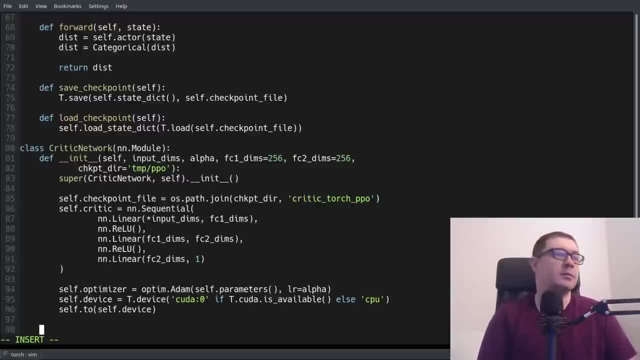 account for that and allow you to use a account for that and allow you to use a similar learning rate because the actor similar learning rate, because the actor similar learning rate, because the actor should be less sensitive than in the case, should be less sensitive than in the case. 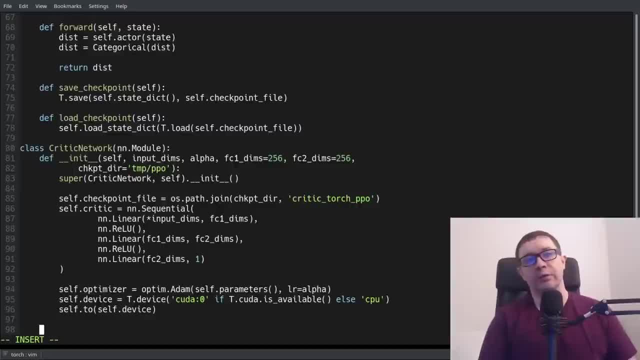 should be less sensitive than in the case of DDPG, but I haven't tested it. so one of DDPG, but I haven't tested it. so one of DDPG, but I haven't tested it. so one thing you can do in your spare time is 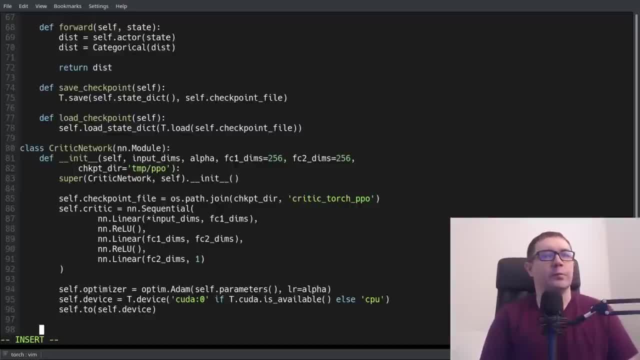 thing you can do in your spare time is. thing you can do in your spare time is play around with differing learning, play around with differing learning, play around with differing learning rates for both the actor and the critic. our forward feed forward function is: our forward feed forward function is: 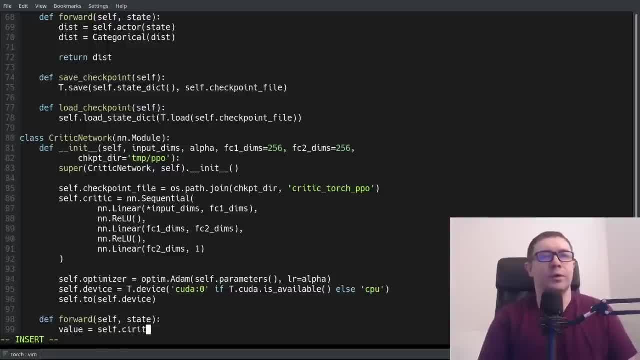 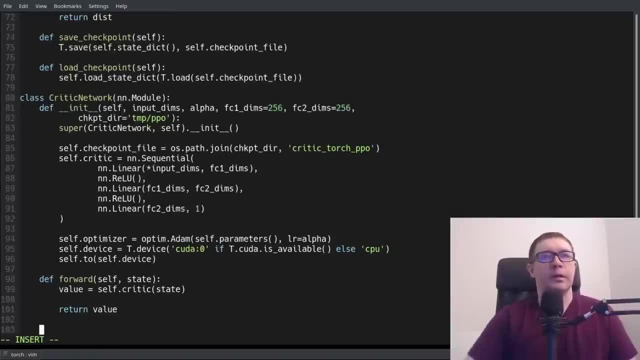 our forward feed forward function is pretty straightforward. you want to pass pretty straightforward. you want to pass pretty straightforward. you want to pass a state through your critic network and a state through your critic network and a state through your critic network and return that value. and we're gonna need 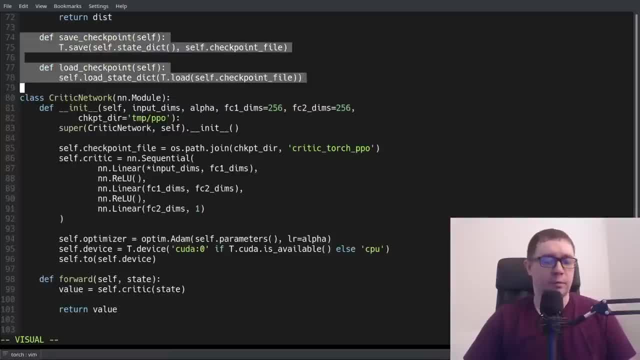 return that value and we're gonna need return that value and we're gonna need saving and loading checkpoints. I am just saving and loading checkpoints. I am just saving and loading checkpoints. I am just going to yank and paste those. because going to yank and paste those? because 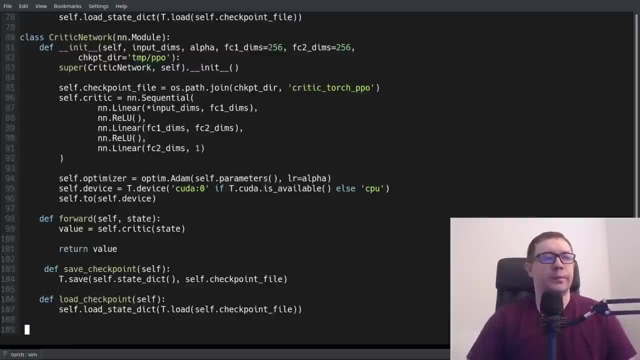 going to yank and paste those, because the functions are otherwise identical. the functions are otherwise identical, the functions are otherwise identical. and so that is it for our two networks. and so that is it for our two networks. and so that is it for our two networks. now we come to the heart of the problem. 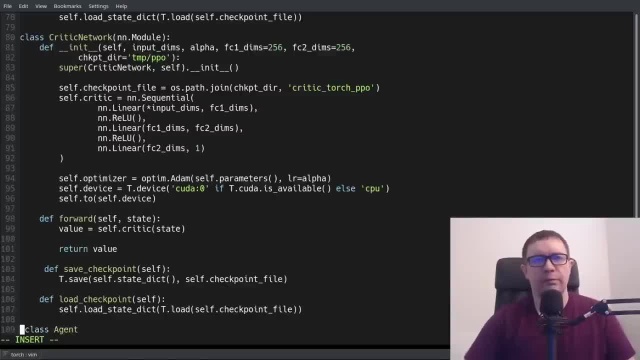 now we come to the heart of the problem. now we come to the heart of the problem, which is the agent class. do I have an which is the agent class? do I have an which is the agent class? do I have an extra? yes, I do, and this, of course, does. 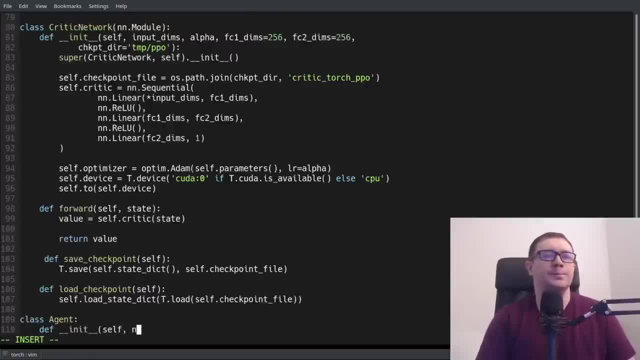 extra: yes, I do, and this, of course, does extra. yes, I do, and this, of course, does not derive from anything. this is our not derive from anything. this is our not derive from anything. this is our base agent class. we need number of base agent class. we need number of. 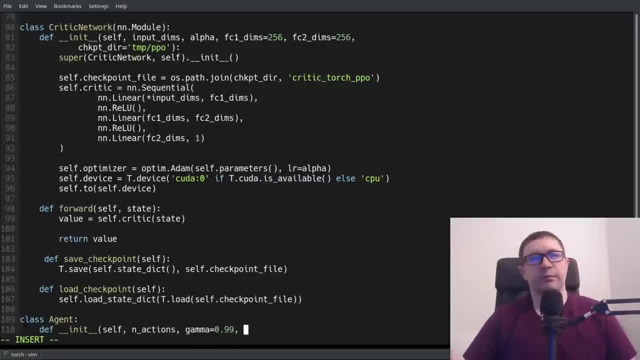 base agent class. we need number of actions. a default value for gamma. which actions. a default value for gamma which actions. a default value for gamma, which is a discount factor in the calculation, is a discount factor in the calculation, is a discount factor in the calculation of our advantages. typically we use 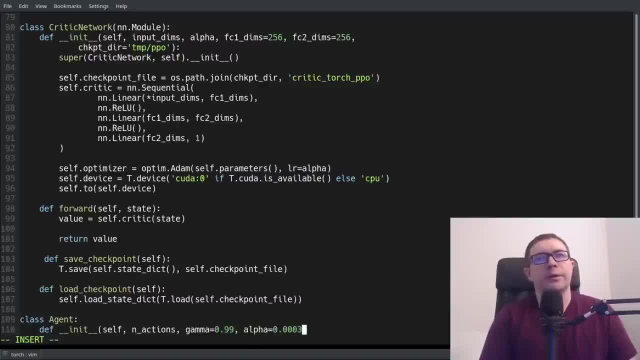 of our advantages. typically we use of our advantages. typically we use something like 0.99, a learning rate of something like 0.99, a learning rate of something like 0.99, a learning rate of 0.003 by 10 minus 4. I got this from the. 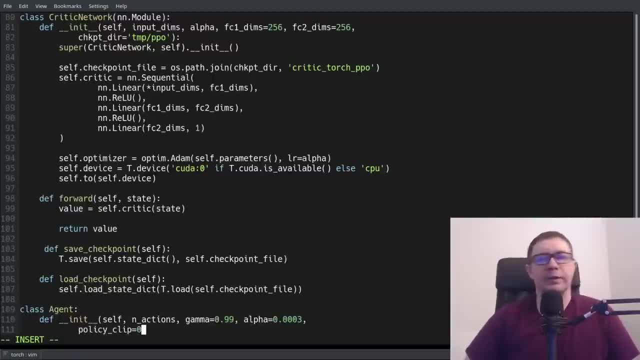 0.003 by 10 minus 4. I got this from the 0.003 by 10 minus 4. I got this from the paper. so if you read the paper, they do paper. so if you read the paper, they do paper. so if you read the paper, they do give you the hyper parameters and a. give you the hyper parameters and a give you the hyper parameters and a little bit of detail around the networks. little bit of detail around the networks. little bit of detail around the networks. they used, but it's not a very well. they used, but it's not a very well. 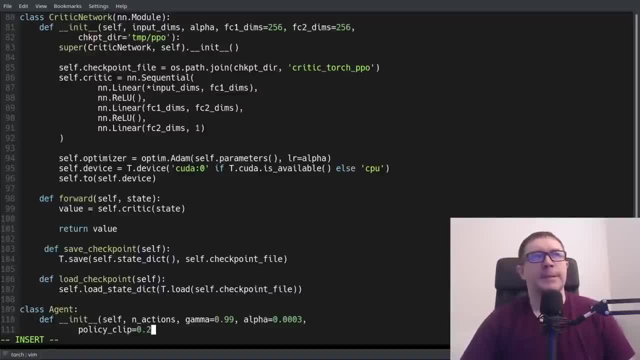 they used, but it's not a very well written paper. it's rather obtuse. so I'm written paper. it's rather obtuse, so I'm written paper. it's rather obtuse, so I'm not a huge fan of it, but we do have. not a huge fan of it, but we do have. 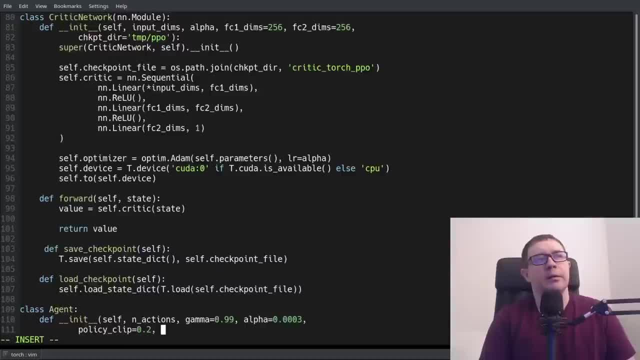 not a huge fan of it, but we do have some good default values from it. so some good default values from it. so some good default values from it. so policy clip. so in my cheat sheet here I policy clip. so in my cheat sheet here I policy clip. so in my cheat sheet here I have a value of 0.1 as a default. 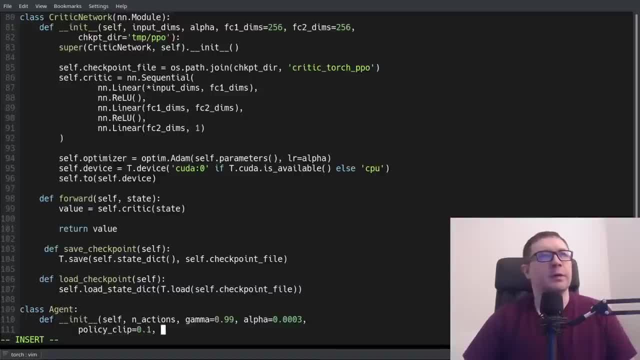 have a value of 0.1 as a default. have a value of 0.1 as a default, although in the paper they use 0.2. although in the paper they use 0.2, although in the paper they use 0.2. perhaps I was experimenting, I will have. 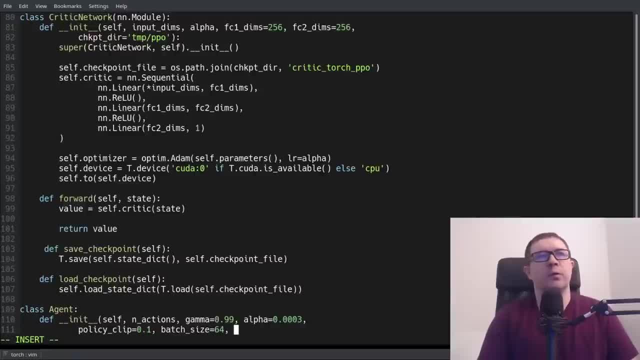 perhaps I was experimenting, I will have. perhaps I was experimenting, I will have to be careful with that. a batch size of to be careful with that. a batch size of to be careful with that. a batch size of 64, a default, and a 2048. so that is the. 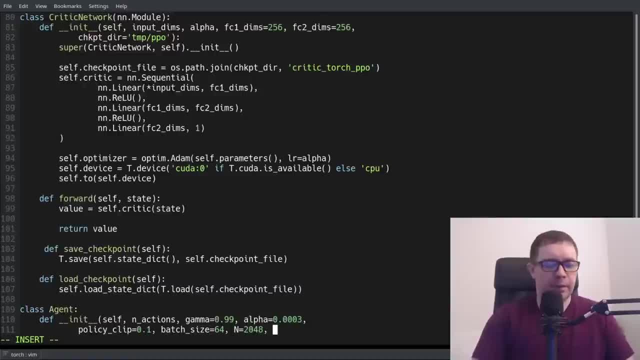 64 a default and a 2048. so that is the 64 a default and a 2048. so that is the horizon, the number of steps before we horizon, the number of steps before we horizon, the number of steps before we perform an update and a default for the. 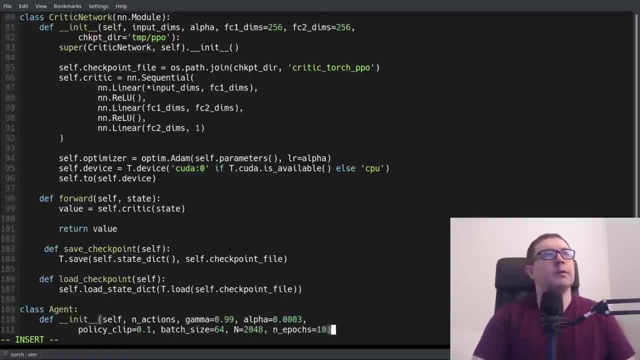 perform an update and a default for the. perform an update and a default for the number of epochs. now these parameters: number of epochs. now these parameters: number of epochs. now these parameters come from. these parameters come from the come from. these parameters come from the come from. these parameters come from the values for continuous environment. so the 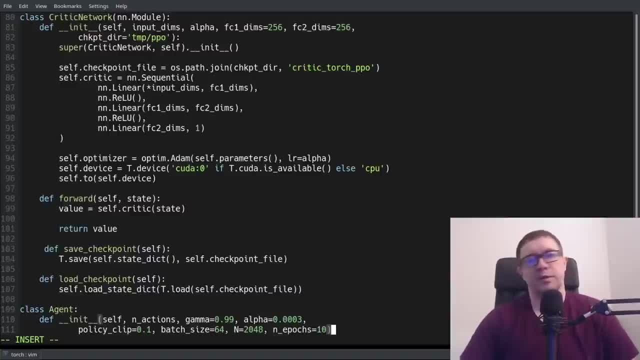 values for continuous environment. so the values for continuous environment, so the actual numbers we're going to be using, actual numbers we're going to be using, actual numbers we're going to be using- are going to be significantly smaller, as are going to be significantly smaller, as are going to be significantly smaller. as I said, we use an end of 23 epochs batch. 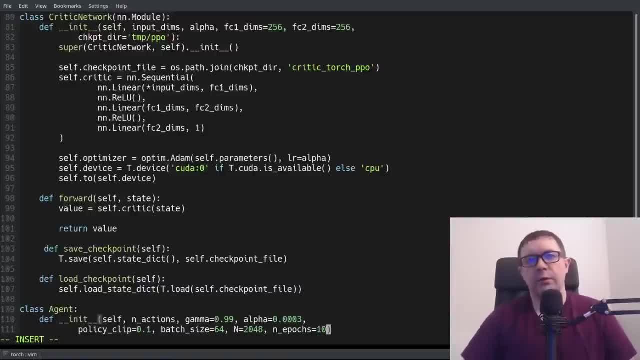 I said we use an end of 23 epochs batch. I said we use an end of 23 epochs batch, size of 5 instead of 64, and I'm going size of 5 instead of 64. and I'm going size of 5 instead of 64 and I'm going to go ahead and set that policy clip to. 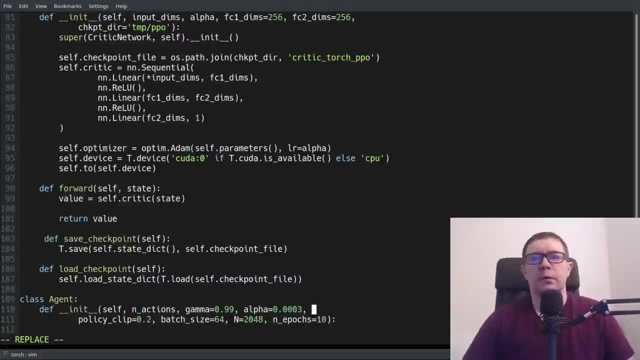 to go ahead and set that policy clip to. to go ahead and set that policy clip to 0.2. now that I'm looking at it, we need a 0.2. now that I'm looking at it, we need a 0.2. now that I'm looking at it, we need a GAE lambda. that is the lambda parameter. 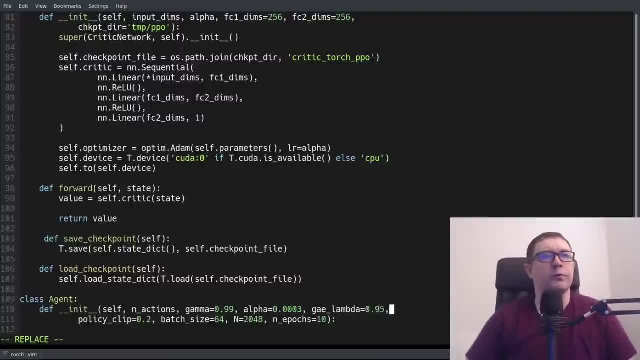 GAE lambda, that is the lambda parameter. GAE lambda, that is the lambda parameter. but of course you can't use lambda. but of course you can't use lambda. but of course you can't use lambda, because that is a reserved word for, because that is a reserved word for. 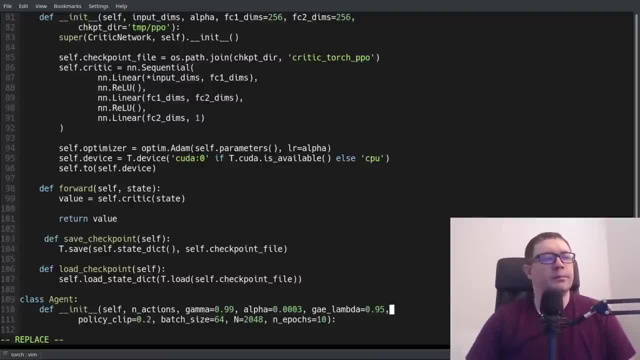 because that is a reserved word for Python. what else do we need? yeah, I think Python. what else do we need? yeah, I think Python. what else do we need? yeah, I think I'm missing something in my other file. I'm missing something in my other file. I'm missing something in my other file here. it's okay, I'll fix it on the fly, so 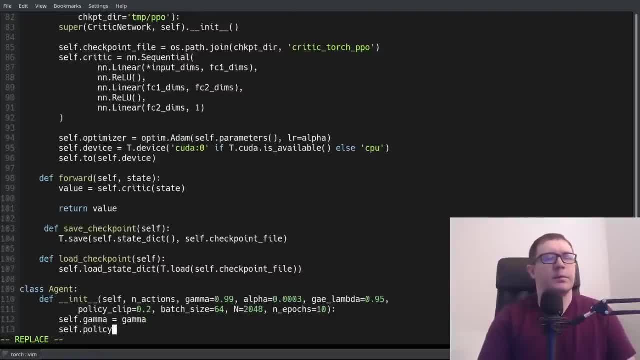 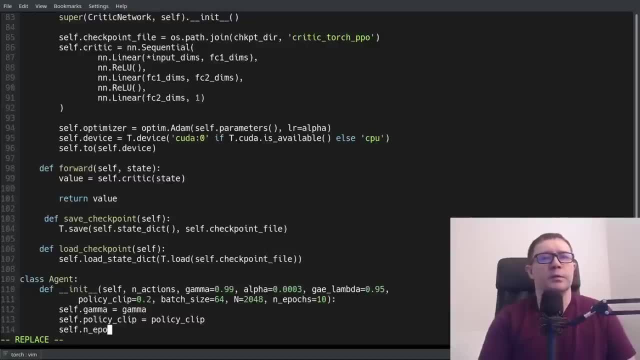 here, it's okay, I'll fix it on the fly. so here, it's okay, I'll fix it on the fly. so then we go ahead and save our, then we go ahead and save our, then we go ahead and save our parameters, a number of epochs and our GAE. 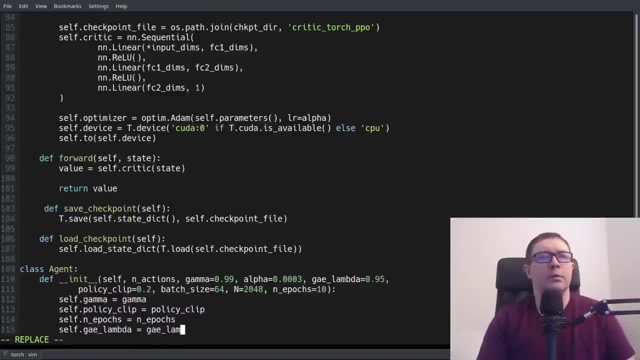 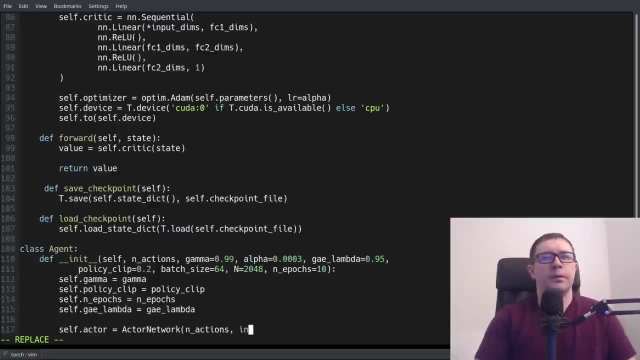 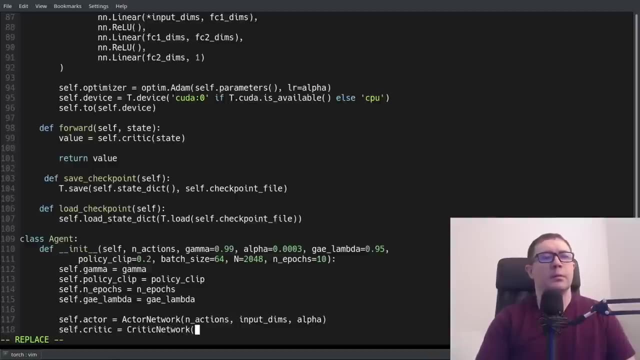 parameters a number of epochs and our GAE parameters. a number of epochs and our GAE lambda. need our actor network put in lambda. need our actor network put in lambda. need our actor network put in some, some, some. and learning rate takes input dims and. and learning rate takes input, dims and. 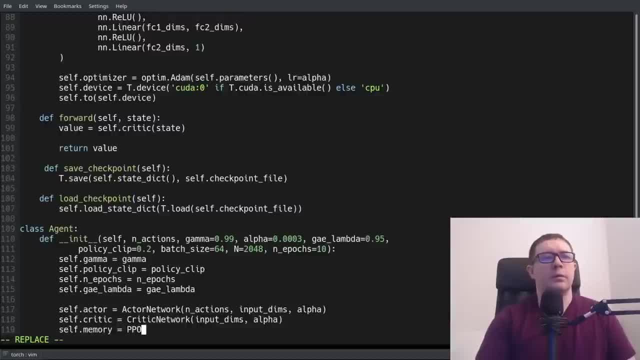 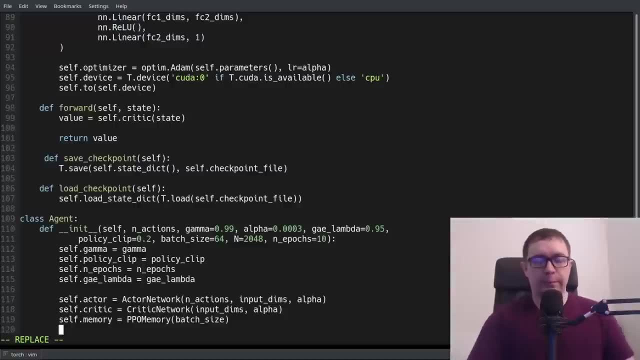 and learning rate takes input dims and alpha BBO memory batch size input. one alpha BBO memory batch size input. one alpha BBO memory batch size input: one second, all right. hopefully that is not second. all right. hopefully that is not second, all right. hopefully that is not as loud now the toddler is playing with. 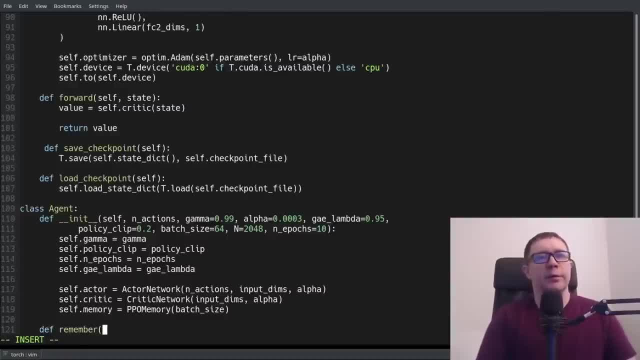 as loud now the toddler is playing with, as loud now the toddler is playing with his grandparents- always a hoot. so now we, his grandparents always a hoot, so now we, his grandparents, always a hoot. so now we need a function that handles the need a function that handles the. 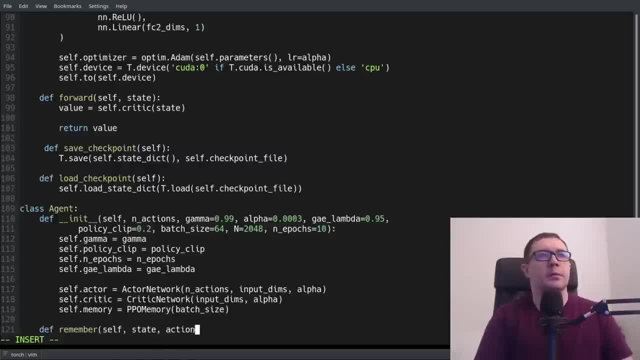 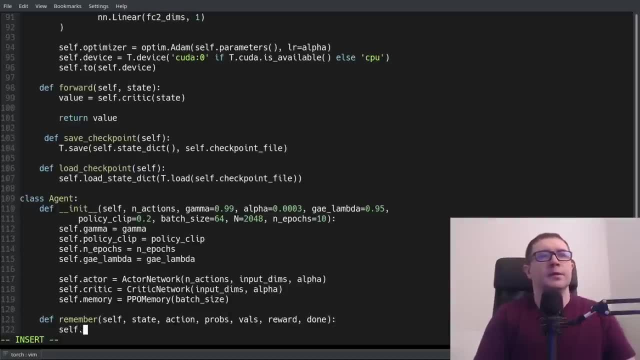 need a function that handles the interface between the agent and its interface between the agent and its interface between the agent and its memory. and it's just going to be very memory and it's just going to be very memory and it's just going to be very simple self memory, store memory. it's. 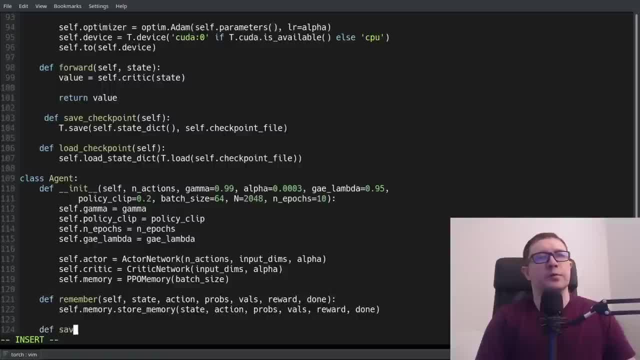 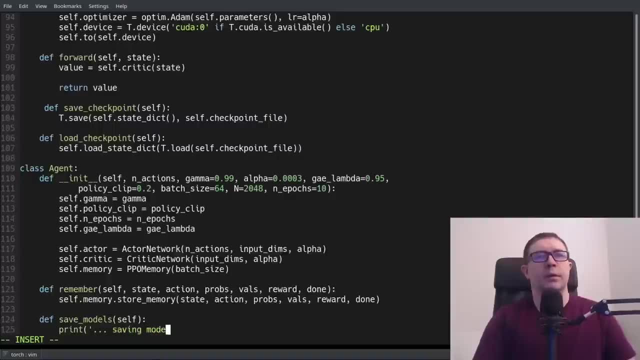 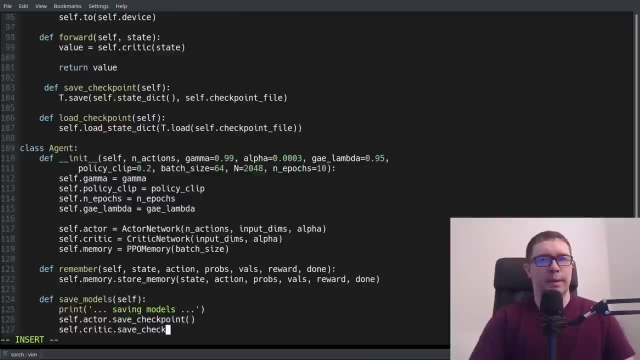 simple self memory store memory. it's simple self memory store memory. it's just an interface function. then we need just an interface function. then we need just an interface function. then we need a function to save our models. print a function to save our models. print a function to save our models, print saving models. that is just going to be an. 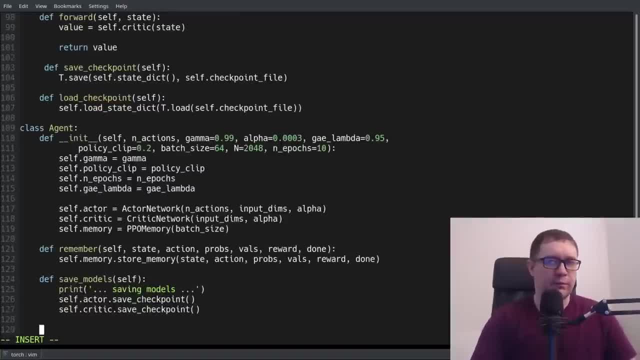 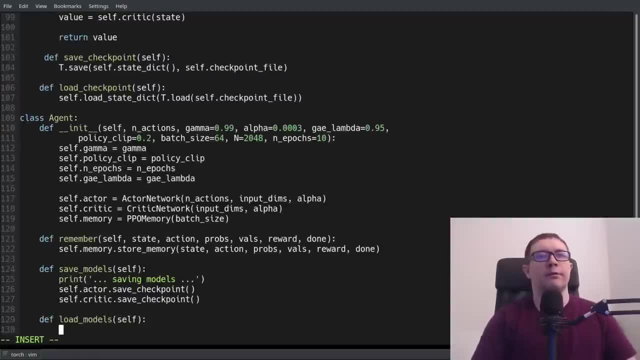 saving models. that is just going to be an saving models. that is just going to be an interface function between the agent and interface function between the agent and interface function between the agent and the save checkpoint functions for the, the save checkpoint functions for the, the save checkpoint functions for the underlying deep neural networks and very 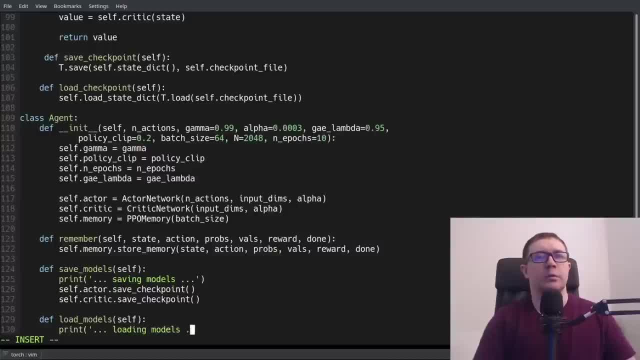 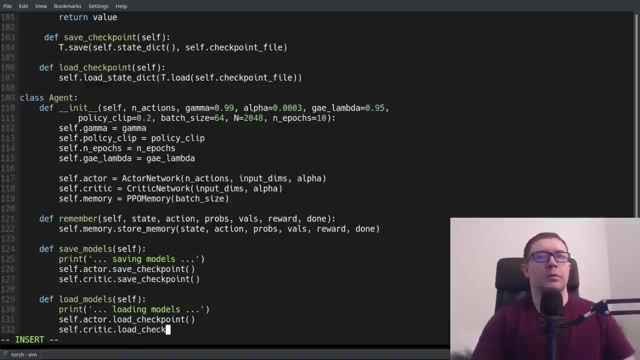 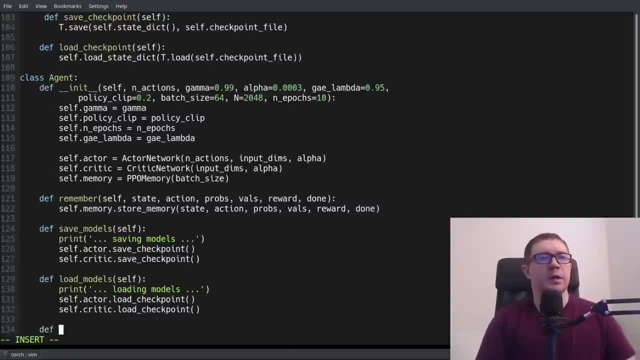 now we have a visitor. all right, that is it for our bookkeeping functions. next we it for our bookkeeping functions. next we it for our bookkeeping functions. next we need something to handle, choosing an need, something to handle. choosing an need, something to handle, choosing an action that'll take an observation of the 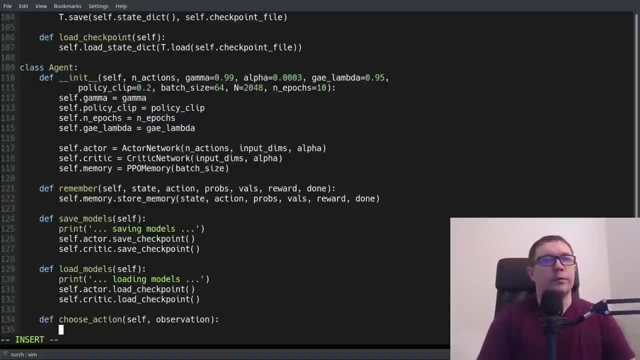 action that'll take an observation of the action that'll take an observation of the currency of the environment as input, currency of the environment as input, currency of the environment as input. and we want to convert that numpy array and we want to convert that numpy array and we want to convert that numpy array to a torch tensor and we're going to. 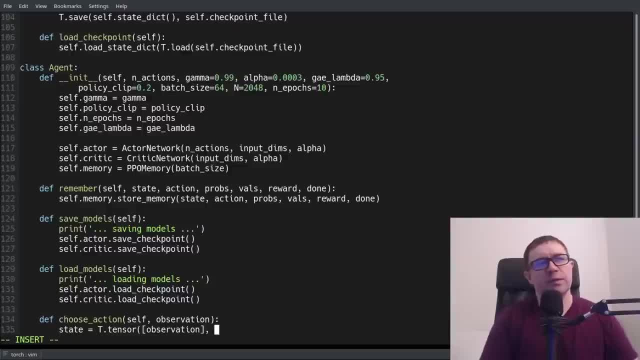 to a torch tensor and we're going to to a torch tensor and we're going to add a batch dimension because the deep add a batch dimension, because the deep add a batch dimension, because the deep neural network expects a batch dimension. neural network expects a batch dimension. 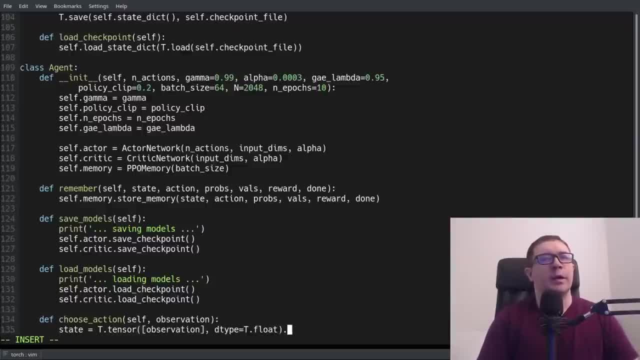 neural network expects a batch dimension, and we'll be sure to specify that it is. and we'll be sure to specify that it is, and we'll be sure to specify that it is float, and then we're going to go ahead. float, and then we're going to go ahead. 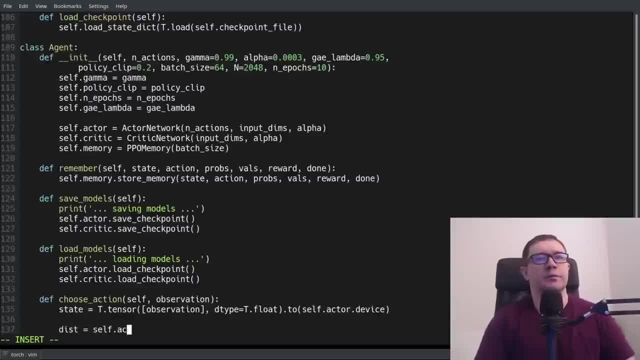 float and then we're going to go ahead and pass that through our neural and pass that through our neural and pass that through our neural networks. so dist equals self dot actor networks. so dist equals self dot actor networks. so dist equals self dot actor state. that'll give us our distribution. 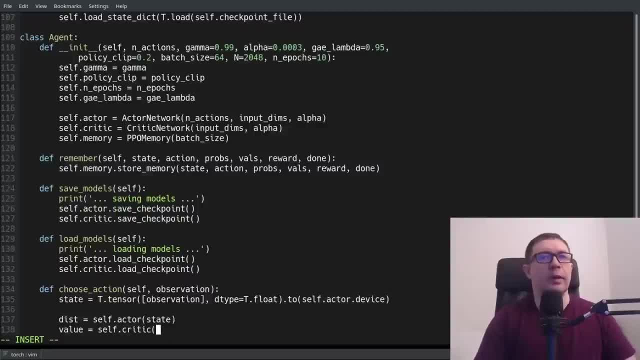 state that'll give us our distribution state that'll give us our distribution for choosing an action. we need the value for choosing an action. we need the value for choosing an action. we need the value of that particular state and then to get of that particular state and then to get. 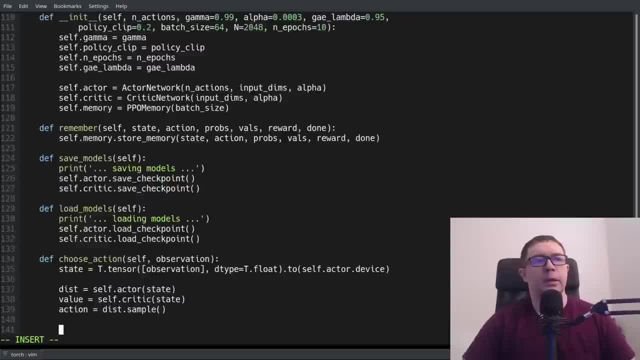 of that particular state and then, to get our action, we just sample our, our action, we just sample our, our action, we just sample our distribution, and then what we want to do- distribution, and then what we want to do, distribution, and then what we want to do is go ahead and squeeze to get rid of. 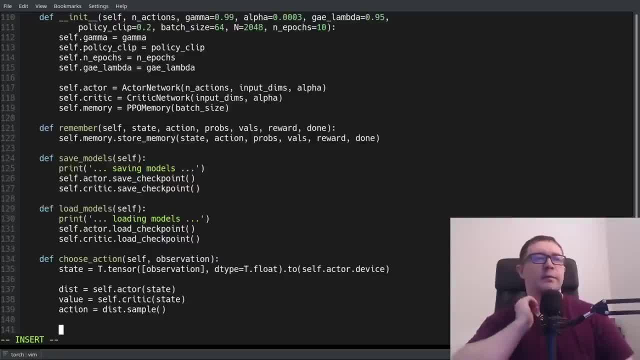 is go ahead and squeeze to get rid of is go ahead and squeeze to get rid of those batch dimensions and this might be those batch dimensions and this might be those batch dimensions and this might be something I added for tensorflow to I'm something I added for tensorflow to I'm. 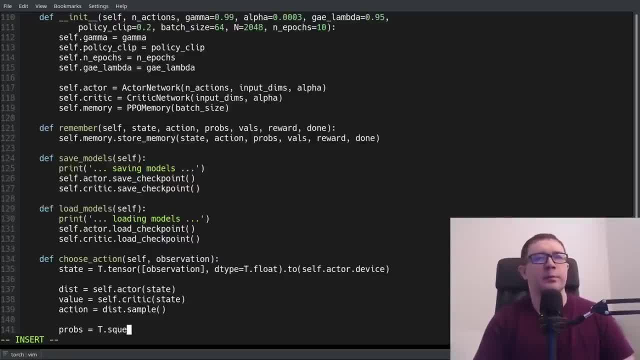 something I added for tensorflow to. I'm not. I don't remember if torch requires not. I don't remember if torch requires not. I don't remember if torch requires it, but it doesn't hurt anything. so for it. but it doesn't hurt anything, so for it. but it doesn't hurt anything. so for the problems, we want to go ahead and 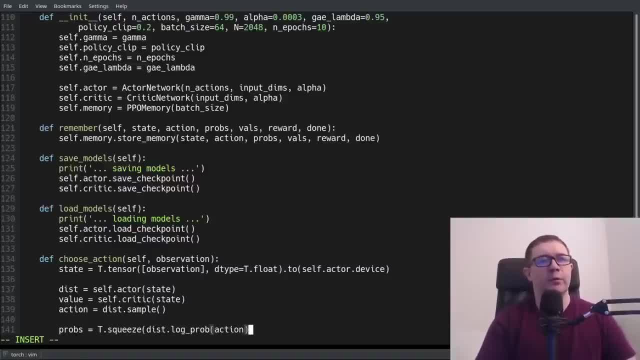 the problems we want to go ahead and the problems we want to go ahead and return the log probability of the action. return the log probability of the action. return the log probability of the action. we actually took that item, so that item. we actually took that item, so that item. 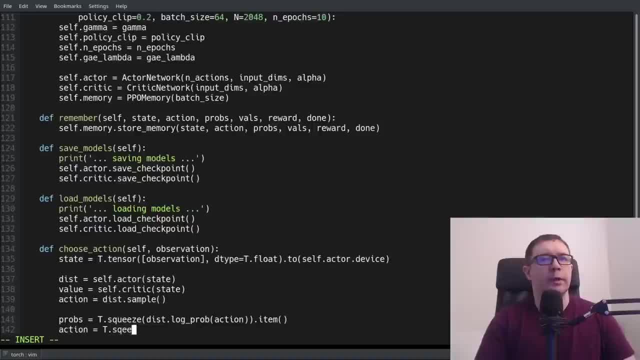 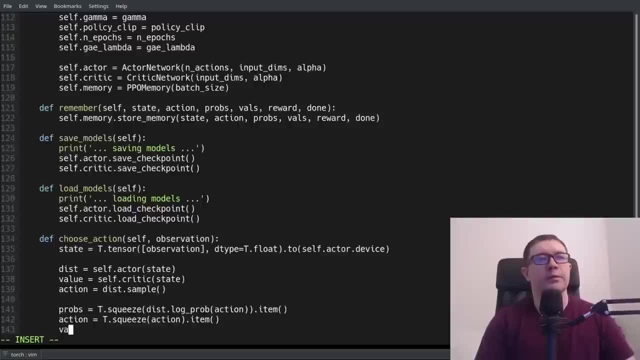 we actually took that item. so that item will give you an integer and likewise will give you an integer, and likewise will give you an integer, and likewise for the action: we want to squeeze it and for the action, we want to squeeze it. and for the action, we want to squeeze it and get the action, the item, out. and 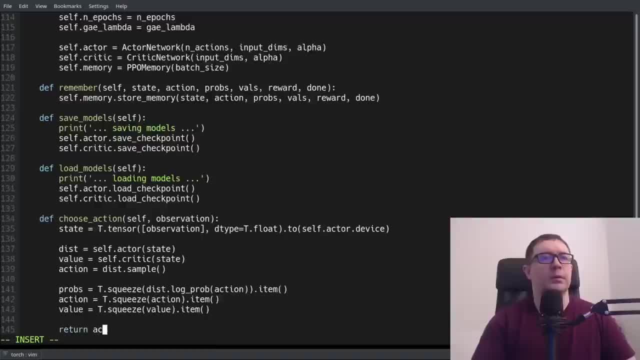 get the action the item out, and get the action- the item out, and similarly for the value, and then just similarly for the value, and then just similarly for the value, and then just return all three. so this will make our return all three. so this will make our. 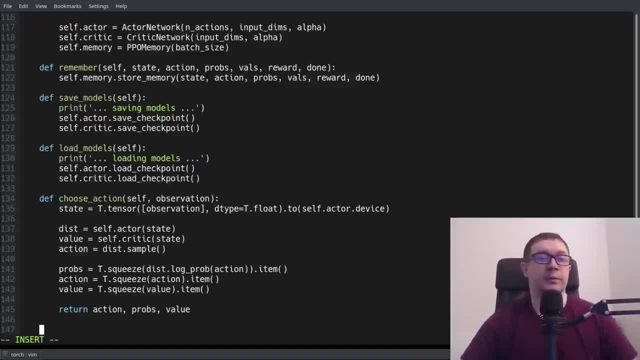 return all three. so this will make our main function look a little bit main function. look a little bit main function. look a little bit different than we're used to. because different than we're used to, because different than we're used to because we're going to be accepting three values. 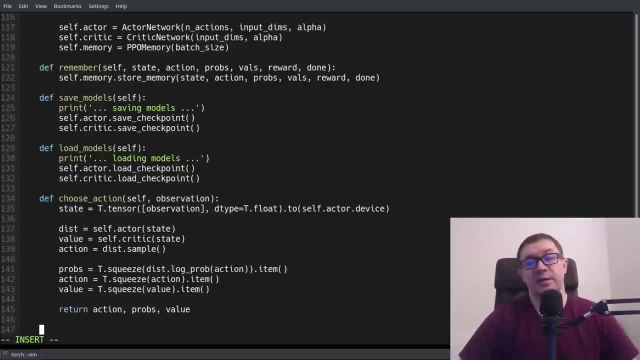 we're going to be accepting three values. we're going to be accepting three values from our cheese action function instead. from our cheese action function instead. from our cheese action function instead of one. but that's necessary for keeping of one. but that's necessary for keeping of one, but that's necessary for keeping track of the probabilities and values, as 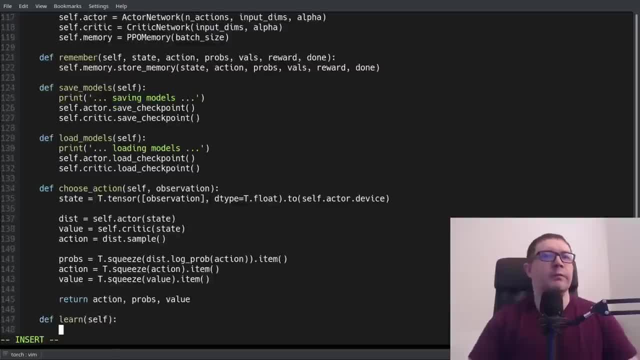 track of the probabilities and values, as track of the probabilities and values as well. next, we come to the meat of the well. next, we come to the meat of the well. next we come to the meat of the problem, so to speak, our learning problem, so to speak, our learning. 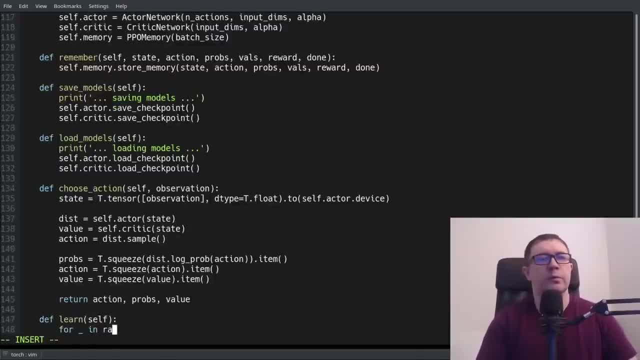 problem, so to speak, our learning function. so we want to iterate over the function. so we want to iterate over the function. so we want to iterate over the number of epochs. so we're gonna have in number of epochs, so we're gonna have in number of epochs, so we're gonna have, in this case, three epochs at the top of. 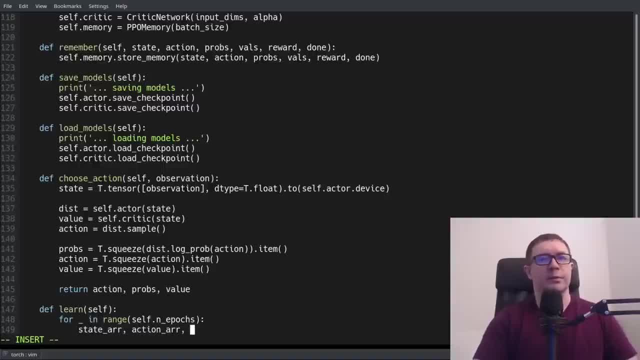 this case, three epochs at the top of this case, three epochs at the top of every epoch. we want to get our arrays every epoch. we want to get our arrays every epoch. we want to get our arrays, the old probabilities, the values, the. the old probabilities, the values, the. 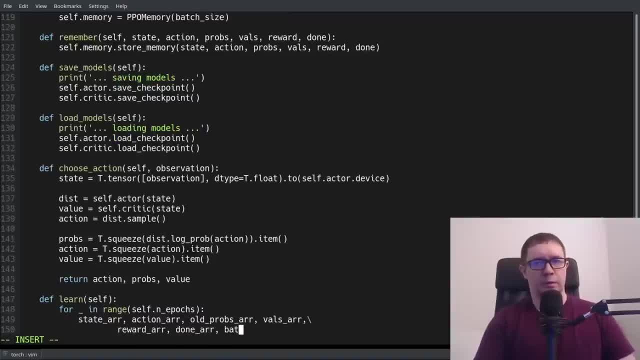 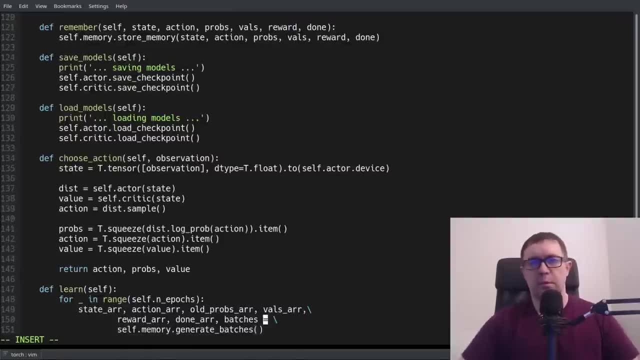 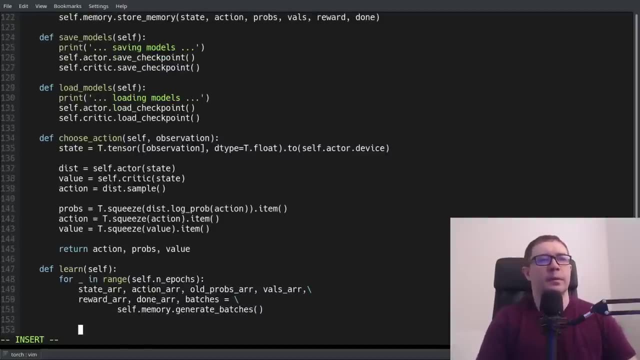 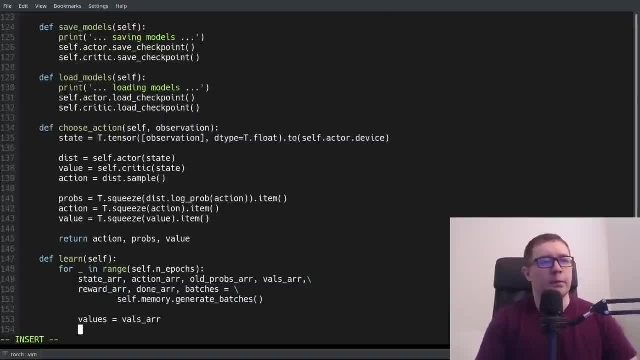 that, and then I'm just going to use a that, and then I'm just going to use a different notation here and go ahead and different notation here and go ahead and different notation here and go ahead and start calculating our advantages, so our start calculating our advantages, so our 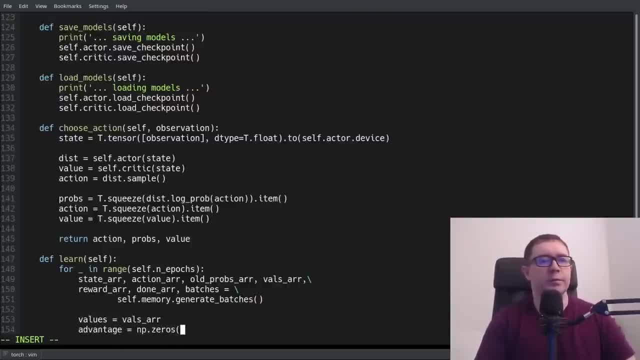 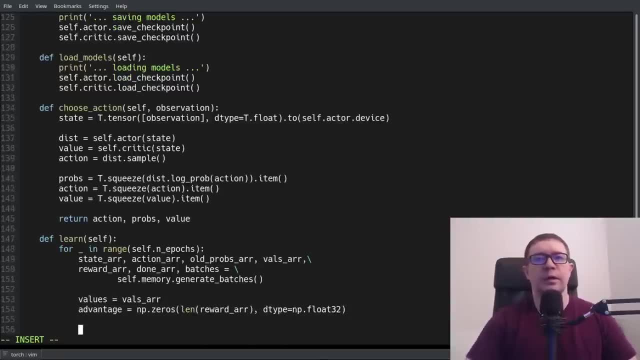 start calculating our advantages. so our advantage is just going to be a numpy advantage is just going to be a numpy advantage is just going to be a numpy array of zeros. Len reward type: MP- float- array of zeros. Len reward type- MP float- array of zeros. Len reward type: MP float 32. 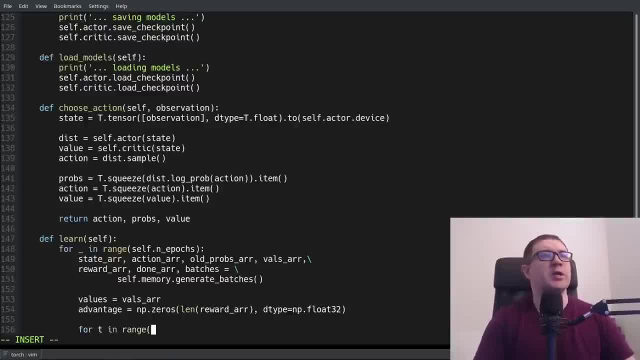 32, 32, and we're going to say for T in range so, and we're going to say for T in range so, and we're going to say for T in range. so for each time step, Len a reward array. for each time step, Len a reward array. 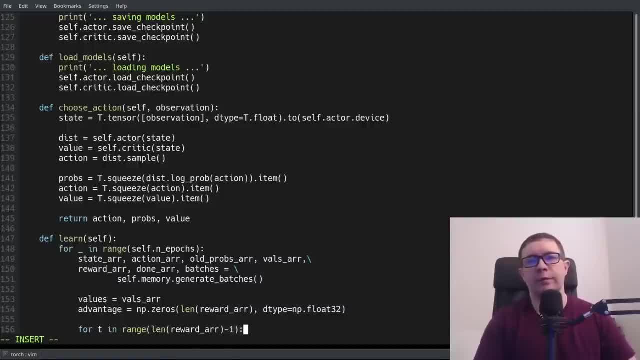 for each time, step Len a reward array: minus one because we don't want to. minus one because we don't want to. minus one because we don't want to overwrite the or go beyond the bounds of overwrite the or go beyond the bounds of overwrite the or go beyond the bounds of our array. our discount factor is going: 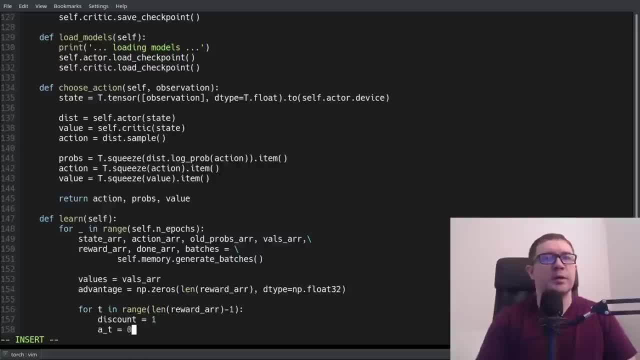 our array, our discount factor is going. our array, our discount factor is going to be one. the advantage at each time to be one. the advantage at each time to be one. the advantage at each time: step starts out as zero, so we're okay. in. step starts out as zero, so we're okay in. 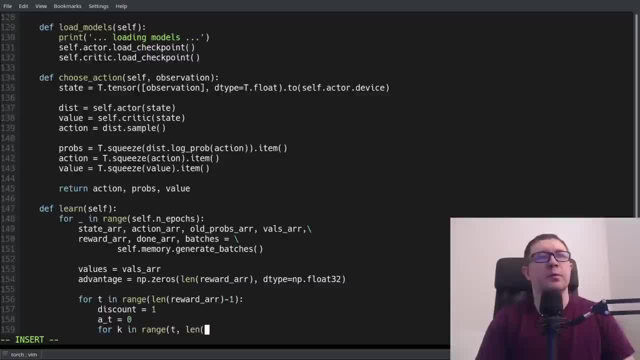 step starts out as zero. so we're okay in range. so we're going to start out at T range. so we're going to start out at T range. so we're going to start out at T and go from T to the same reward array and go from T to the same reward array. 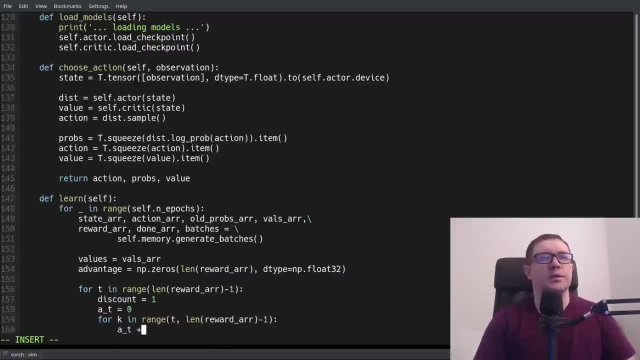 and go from T to the same reward array minus one, and say a sub T plus equals minus one, and say a sub T plus equals minus one, and say a sub T plus equals discount, so that GA e times lambda discount, so that GA e times lambda discount, so that GA e times lambda factor, which starts out as one times we. 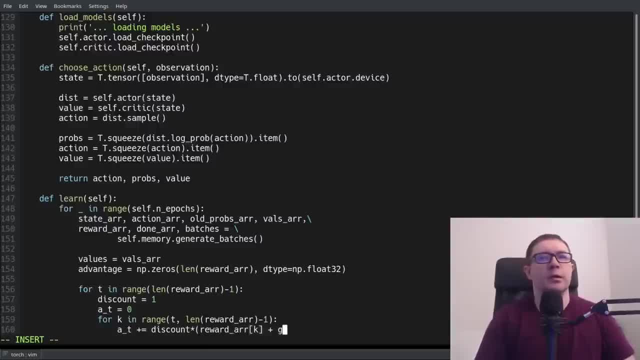 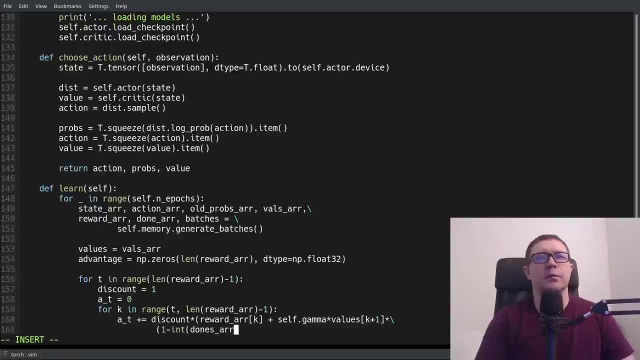 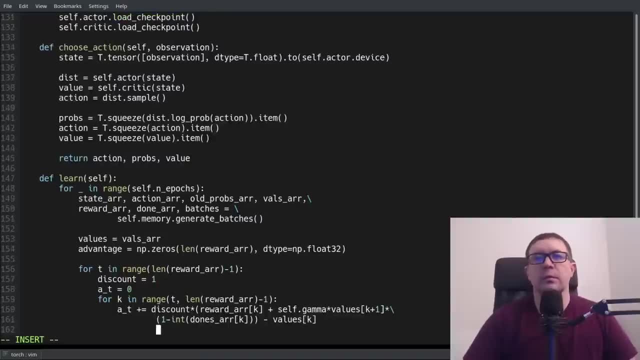 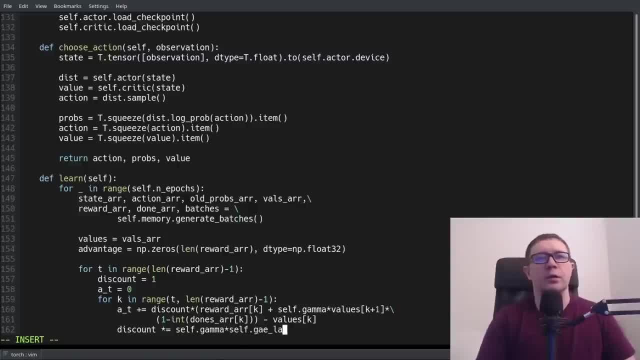 sub K. then we say: discount times equals self gamma times G lambda, and at the end self gamma times, G lambda, and at the end self gamma times, G lambda, and at the end of every calculation, at the end of every of every calculation, at the end of every. 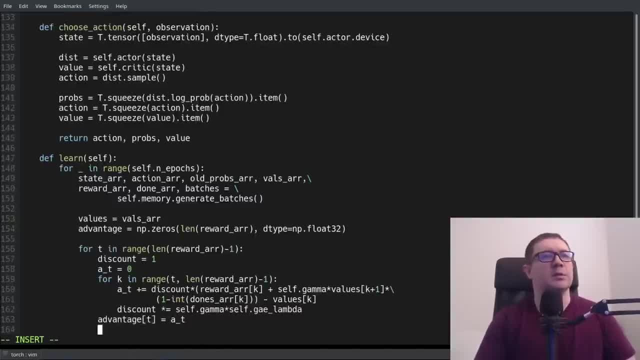 of every calculation, at the end of every K steps advantage sub T equals at a sub K steps advantage sub T equals at a sub K steps advantage sub T equals at a sub T, and at the end we're going to T and at the end we're going to. 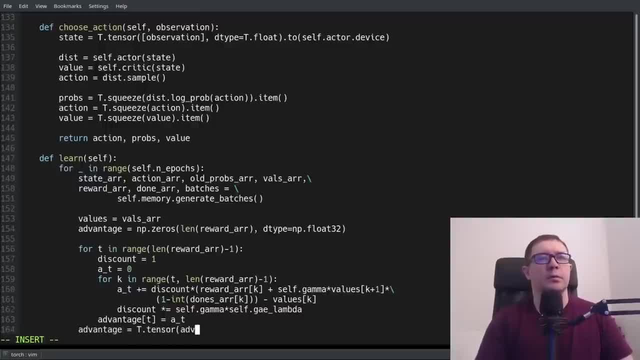 T, and at the end we're going to turn advantage to a tensor in particular, a turn advantage to a tensor in particular, a turn advantage to a tensor in particular, a CUDA tensor, and this is just a strict CUDA tensor. and this is just a strict CUDA tensor, and this is just a strict implementation of the equation from the. 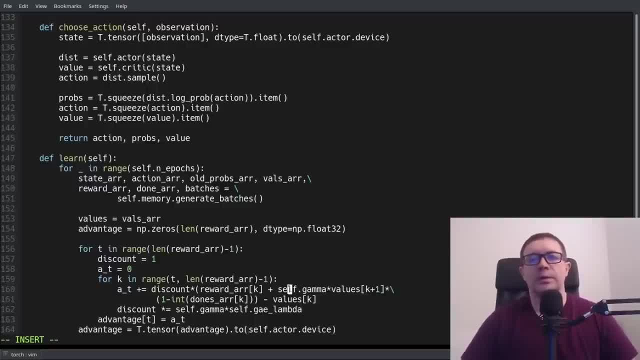 implementation of the equation from the implementation of the equation from the paper. so this right here in parentheses paper, so this right here in parentheses paper, so this right here in parentheses is the Delta sub T, so it's a reward. is the Delta sub T, so it's a reward. 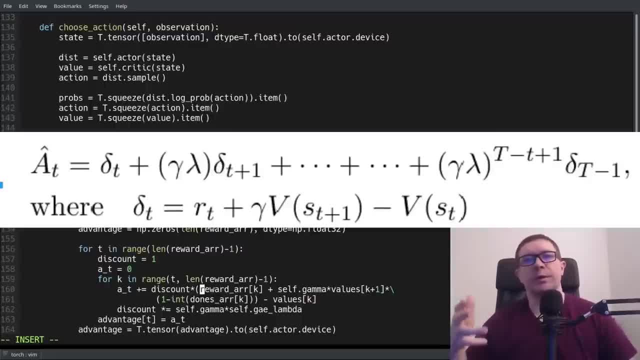 is the Delta sub T, so it's a reward. plus gamma times V sub T, plus 1 minus V, plus gamma times V sub T plus 1 minus V, plus gamma times V sub T plus 1 minus V sub T, or you know, we swap the K and T. 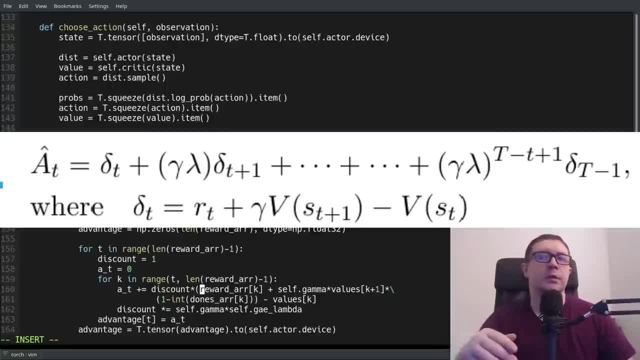 sub T. or you know we swap the K and T sub T, or you know we swap the K and T here and you need the 1 minus Duns on here. and you need the 1 minus Duns on here. and you need the 1 minus Duns on the values as a multiplicative factor of. 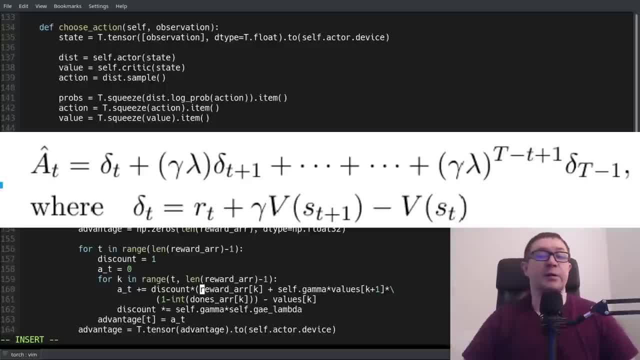 the values as a multiplicative factor of the values, as a multiplicative factor of the values of a T sub T plus 1, because the values of a T sub T plus 1, because the values of a T sub T plus 1, because the value of the terminal state is. 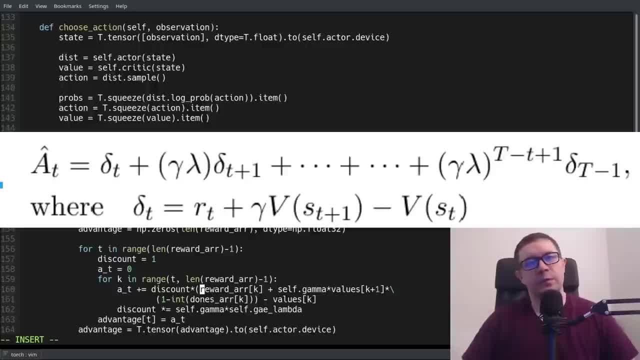 the value of the terminal state is. the value of the terminal state is identically zero. that's just a identically zero. that's just a identically zero. that's just a convention in reinforcement learning. it convention in reinforcement learning. it. convention in reinforcement learning. it predates the deep neural network. stub. predates the deep neural network stub. predates the deep neural network stub. it's just how we handle it. it's assumed. it's just how we handle it. it's assumed. it's just how we handle it. it's assumed. that's why they don't put it in the 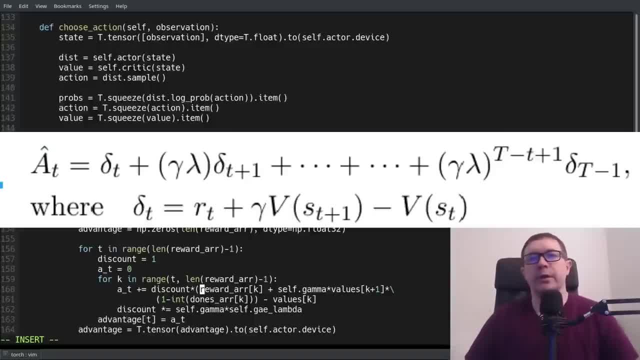 that's why they don't put it in the. that's why they don't put it in the calculation. it is assumed it's just a calculation. it is assumed it's just a calculation. it is assumed it's just a matter of convention. and then that matter of convention, and then that. 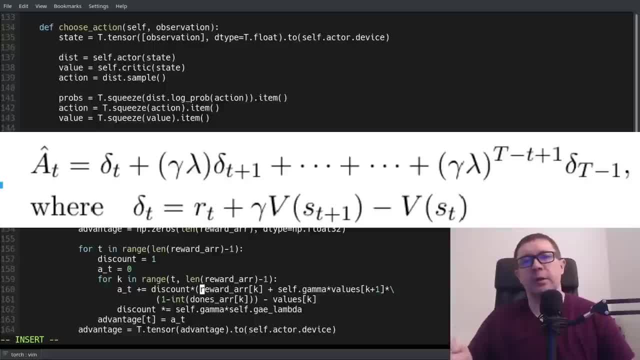 matter of convention. and then that discount is the GAE and the lambda discount is the GAE and the lambda discount is the GAE and the lambda multiplied by the gamma that takes care, multiplied by the gamma that takes care, multiplied by the gamma that takes care of the multiplicative factor. so it is. 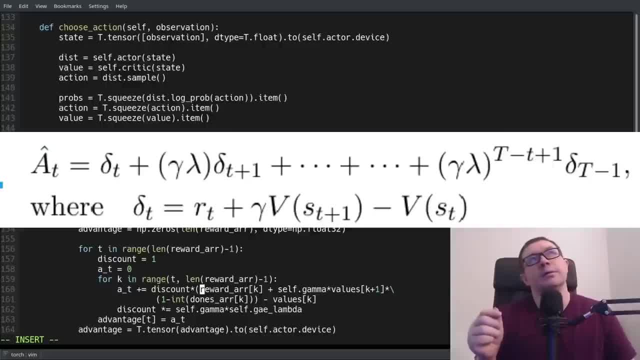 of the multiplicative factor. so it is of the multiplicative factor. so it is, though the gamma lambda to the T minus, though the gamma lambda to the T minus, though the gamma lambda to the T minus one power, or is it T minus K minus one one power, or is it T minus K minus one. 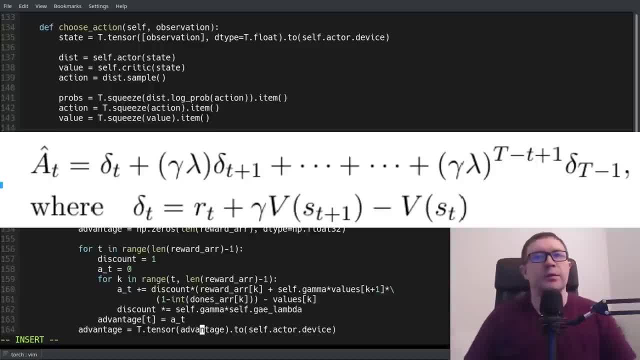 one power, or is it T minus K minus one, something like that power multiplied by something like that power, multiplied by something like that power multiplied by the Delta, and then you're summing it all the Delta, and then you're summing it all the Delta, and then you're summing it all up. so now we have our advantage. I'm 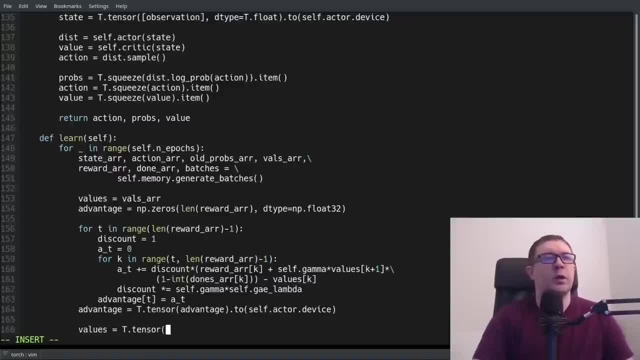 up, so now we have our advantage. I'm up, so now we have our advantage. I'm going to convert the values to a tensor. going to convert the values to a tensor, going to convert the values to a tensor as well, and I fully admit here that as well, and I fully admit here that. 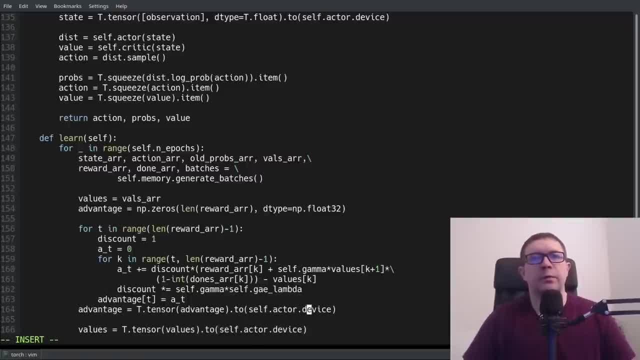 as well, and I fully admit here that, going from Val's array to you know what, going from Val's array to you know what, going from Val's array to you know what, in fact, let's do this now. let's leave it. in fact, let's do this now, let's leave it. 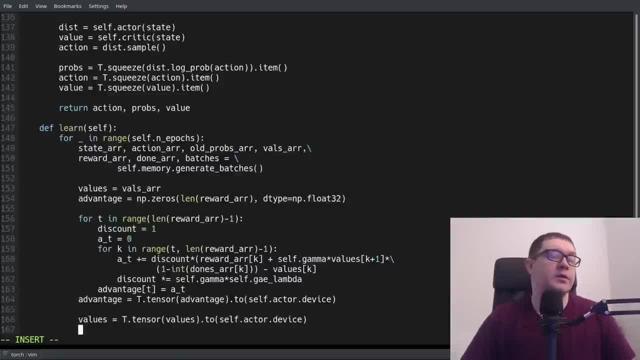 in fact, let's do this now, let's leave it the way it is may not be the most. the way it is may not be the most. the way it is may not be the most effective or, excuse me, the most effective or, excuse me, the most effective or, excuse me, the most efficient way of doing it, but sometimes 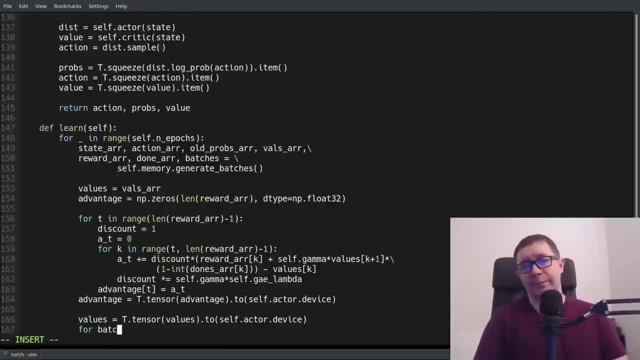 efficient way of doing it. but sometimes efficient way of doing it, but sometimes I just get stuff to work and then don't. I just get stuff to work and then don't I just get stuff to work and then don't go back and clean it up if you want to. 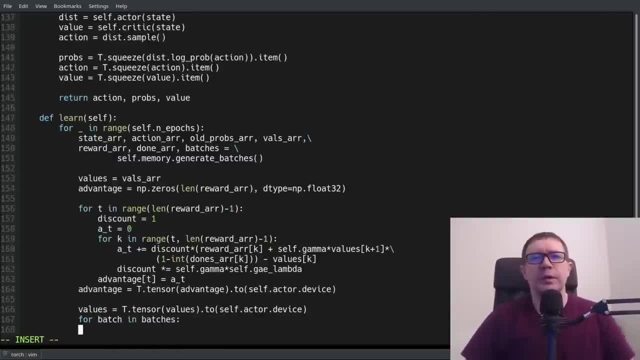 go back and clean it up. if you want to go back and clean it up. if you want to clean it up, please do so. I always clean it up. please do so. I always clean it up. please do so. I always invite that and it looks like I'm. 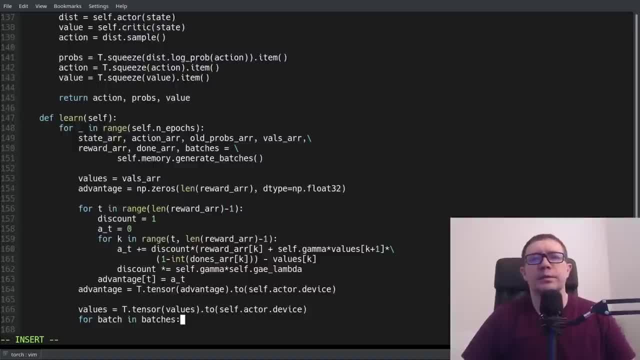 invite that, and it looks like I'm invite that, and it looks like I'm missing something here, because it is not missing something here, because it is not missing something here, because it is not automatically indenting, so I'm probably automatically indenting, so I'm probably. 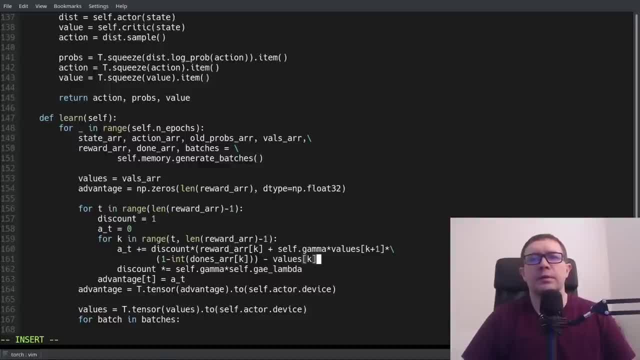 automatically indenting. so I'm probably missing a parenthesis somewhere, and it is missing a parenthesis somewhere and it is missing a parenthesis somewhere and it is right here, I believe. if I am NOT right here, I believe, if I am NOT right here, I believe, if I am NOT mistaken. yeah, there it goes, alright. so 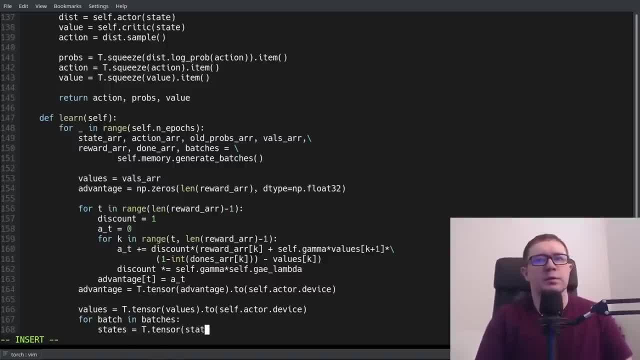 mistaken, yeah, there it goes alright. so, mistaken, yeah, there it goes alright. so then States is just going to be a, then States is just going to be a. then States is just going to be a. tensor state array sub batch D type. tensor state array sub batch D type. 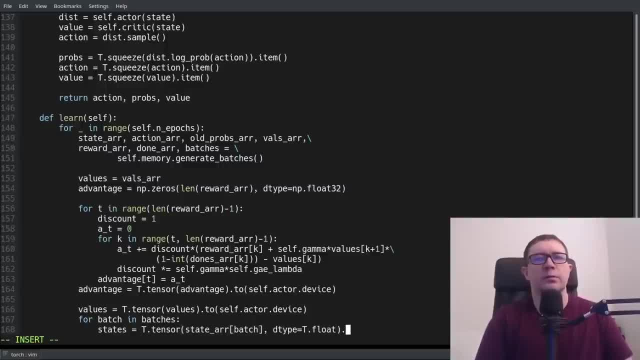 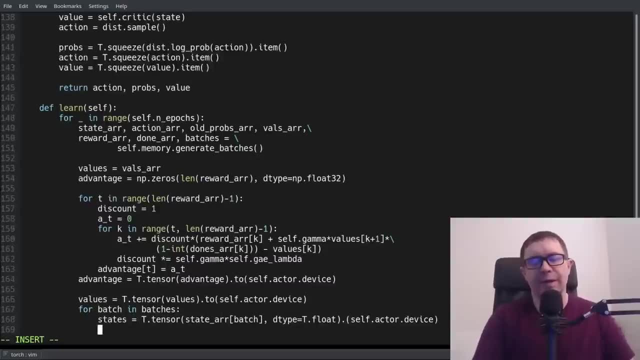 tensor state array, sub batch D: type T: dot float to salt on actor and dot. T dot float to salt on actor and dot. T dot float to salt on actor and dot device and we're kind of violating the device and we're kind of violating the device and we're kind of violating the pep-8 style guides, their style guide by 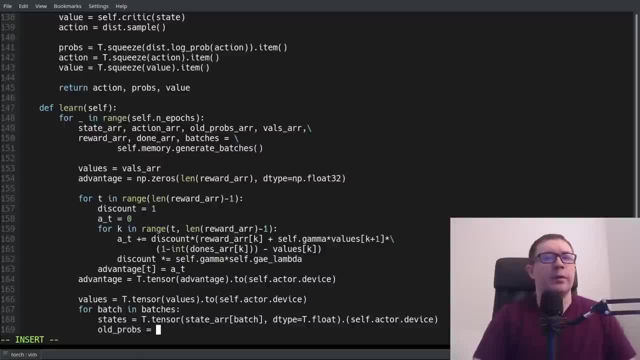 pep-8 style guides their style guide by pep-8 style guides their style guide by going beyond 80 characters. but I think going beyond 80 characters, but I think going beyond 80 characters, but I think we'll be alright, old probabilities gets, we'll be alright, old probabilities gets. 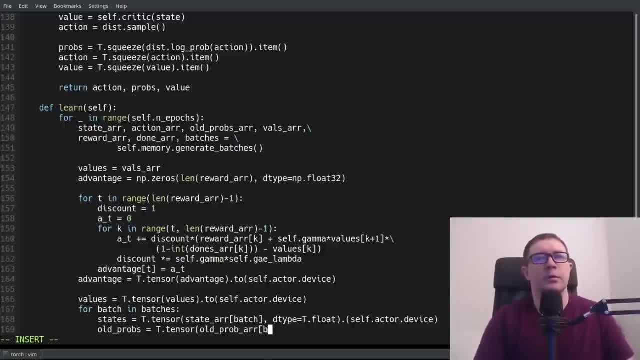 we'll be alright, old probabilities gets converted to a tensor and I don't need converted to a tensor and I don't need converted to a tensor and I don't need an explicit D type there. I don't think an explicit D type there, I don't think. 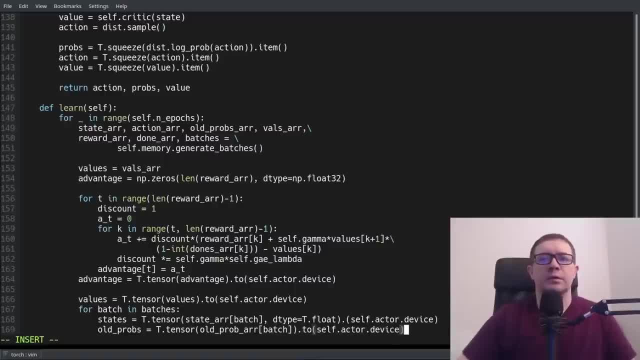 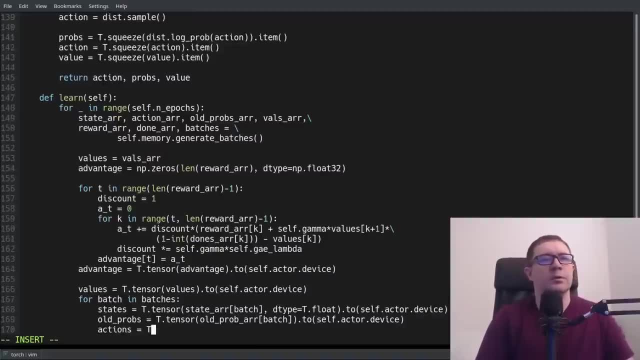 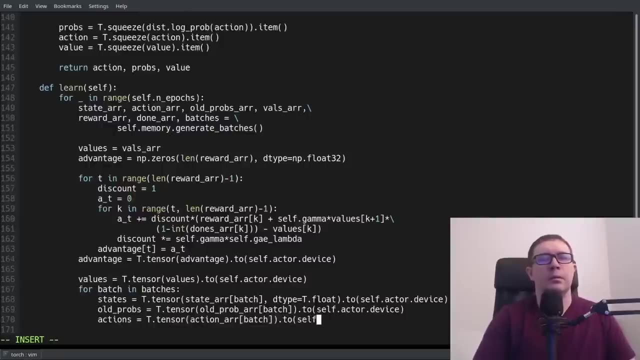 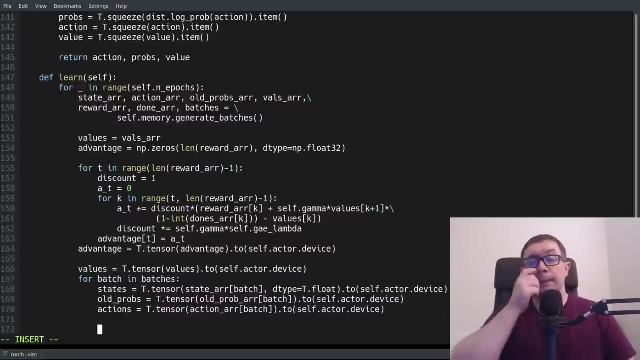 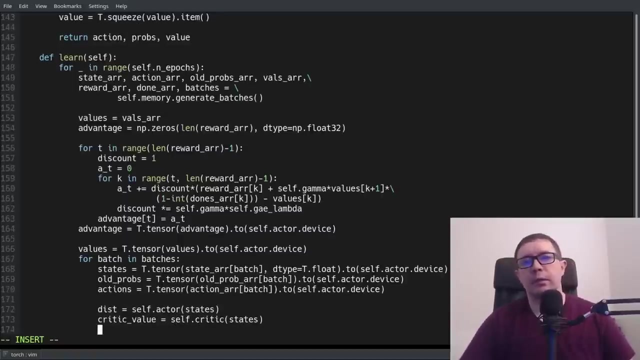 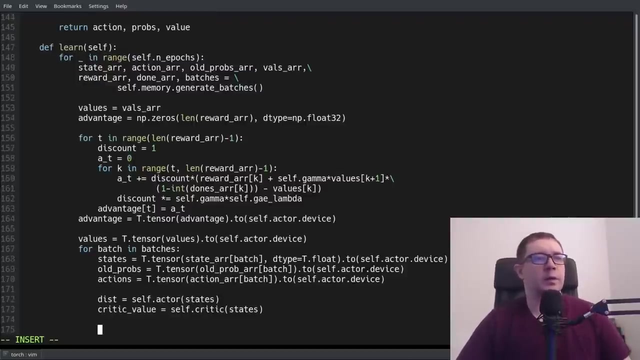 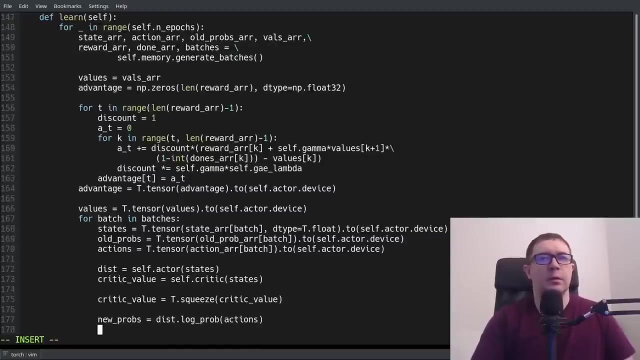 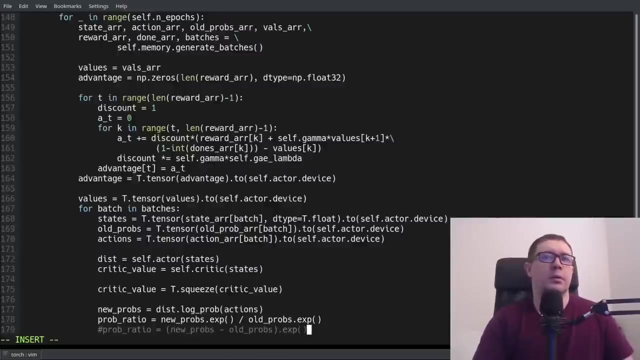 an explicit D type there. I don't think dot dot dot. to get the probabilities and take their. to get the probabilities and take their. to get the probabilities and take their ratio, you could also do this. those two ratio, you could also do this. those two ratio, you could also do this. those two are equivalent by the properties of. 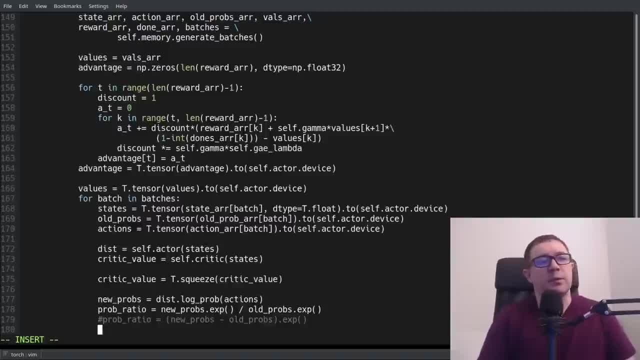 are equivalent by the properties of are equivalent by the properties of exponents, exponents exponentials, excuse, exponents, exponents, exponentials, excuse exponents, exponents, exponentials, excuse me. and then we're going to calculate our me, and then we're going to calculate our. 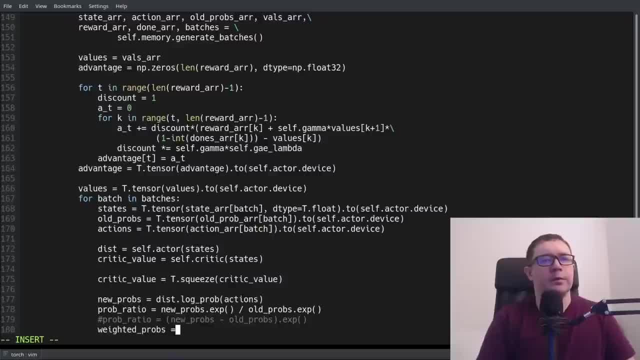 me, and then we're going to calculate our weighted probabilities. and sorry our weighted probabilities, and sorry our weighted probabilities and sorry our probability ratio. no, yeah, the weighted probability ratio. no, yeah, the weighted probability ratio. no, yeah, the weighted probabilities. I think I have two lines. probabilities: I think I have two lines. 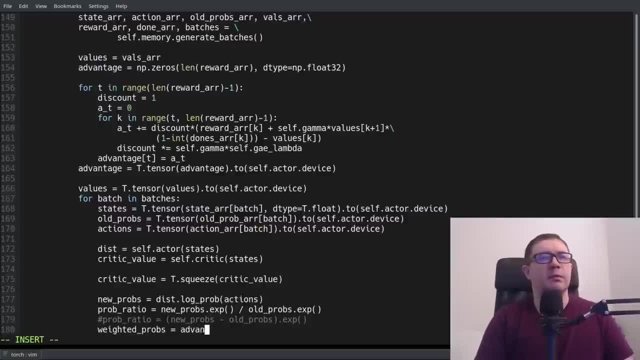 probabilities. I think I have two lines that do the same thing in there. that's that, do the same thing in there. that's that: do the same thing in there. that's funny, and that's going to be the funny, and that's going to be the funny and that's going to be the advantage. batch times: a probability. 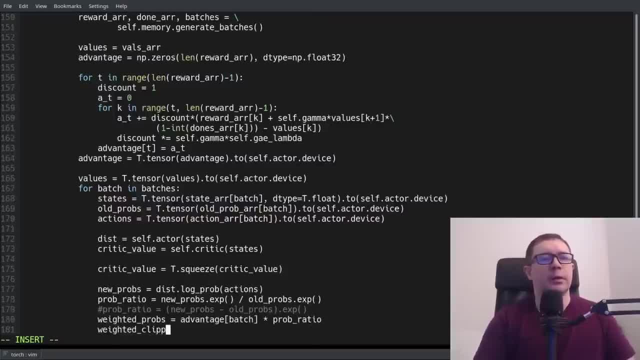 advantage, batch times a probability advantage, batch times a probability ratio, then we need the weighted clipped ratio, then we need the weighted clipped ratio, then we need the weighted clipped probabilities, and that is going to be probabilities, and that is going to be probabilities, and that is going to be the clamp of the prob ratio between one. 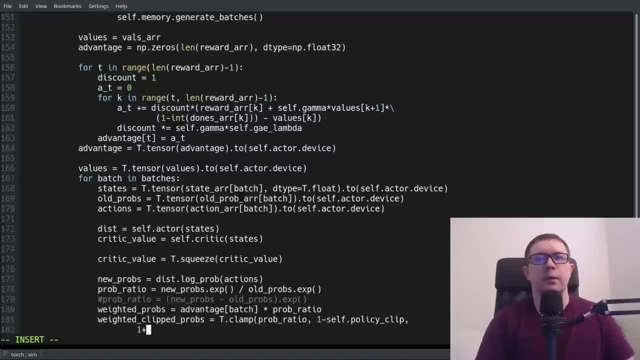 the clamp of the prob ratio between one. the clamp of the prob ratio between one minus self-taught policy clip and one minus self-taught policy clip and one minus self-taught policy clip and one plus self-taught policy clip multiplied. 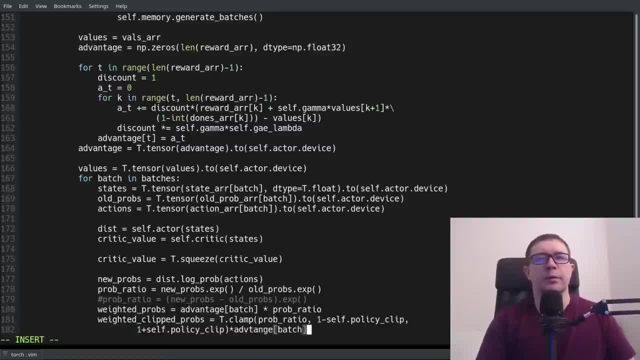 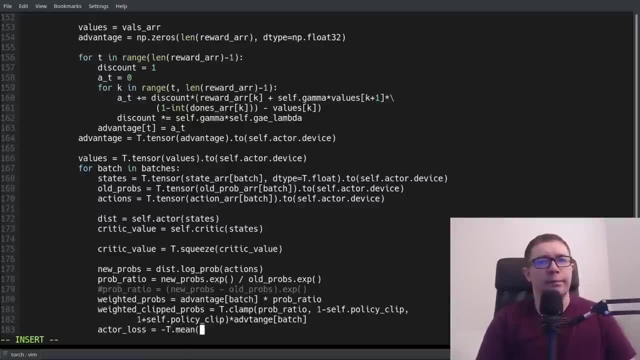 plus self-taught policy clip, multiplied plus self-taught policy clip, multiplied by advantage sub batch by advantage sub batch by advantage sub batch, now our actor loss is going to be the. now our actor loss is going to be the. now our actor loss is going to be the negative minimum of the weighted probs. 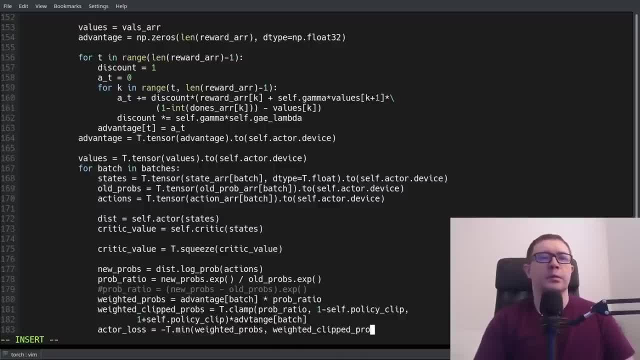 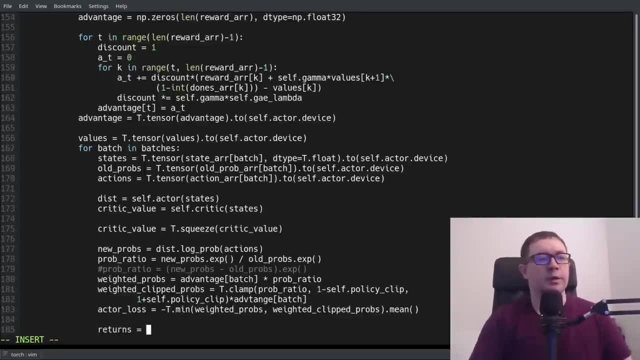 negative minimum of the weighted probs: negative minimum of the weighted probs or the awaited clipped probs dot mean. or the awaited clipped probs dot mean. or the awaited clipped probs dot mean. and our returns for our critic loss are. and our returns for our critic loss are and our returns for our critic loss are going to be the advantage plus the. 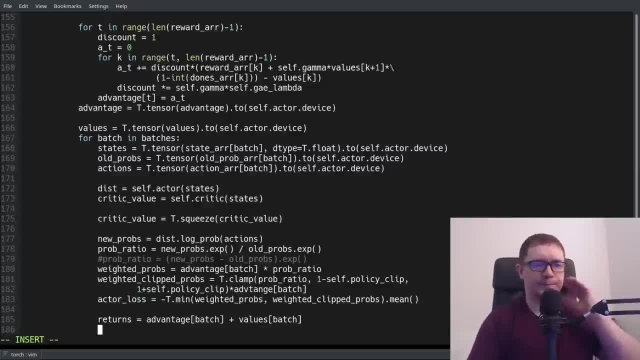 going to be the advantage plus the, going to be the advantage plus the values for that, values for that, values for that particular batch, and so our critic loss then is particular batch, and so our critic loss then is particular batch, and so our critic loss then is going to be the returns minus. 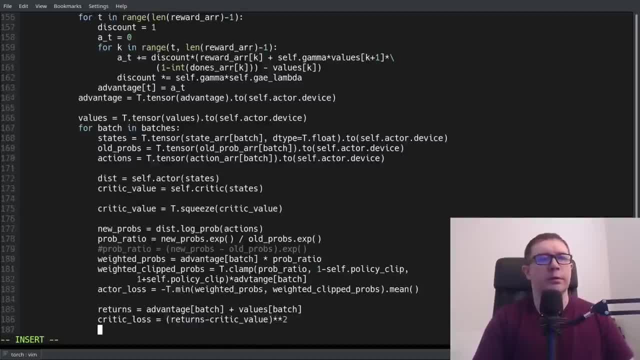 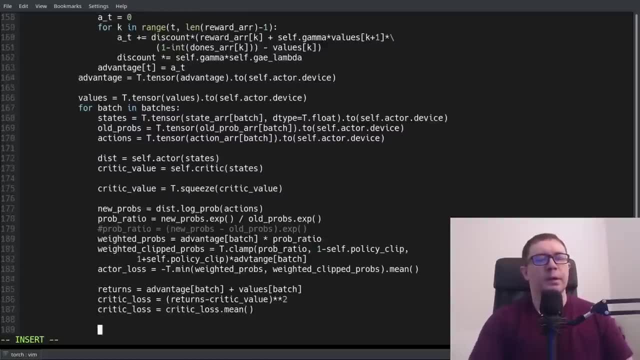 going to be the returns minus. going to be the returns minus critic value squared and the mean value. our critic value squared and the mean value. our critic value squared and the mean value. our total loss after loss plus 0.5 times. total loss after loss plus 0.5 times. 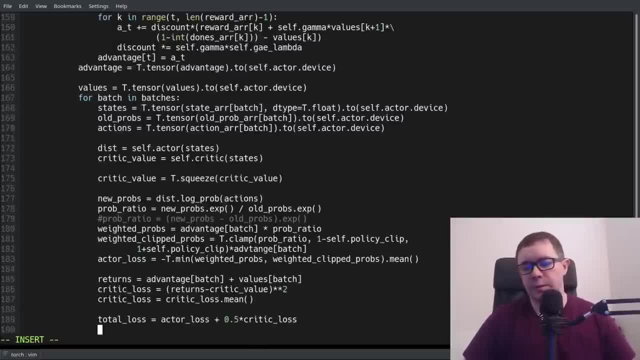 total loss after loss plus 0.5 times critic loss, critic loss, critic loss. remember we're doing gradient ascent and remember we're doing gradient ascent. and remember we're doing gradient ascent. and there's a negative sign in front of the. there's a negative sign in front of the. 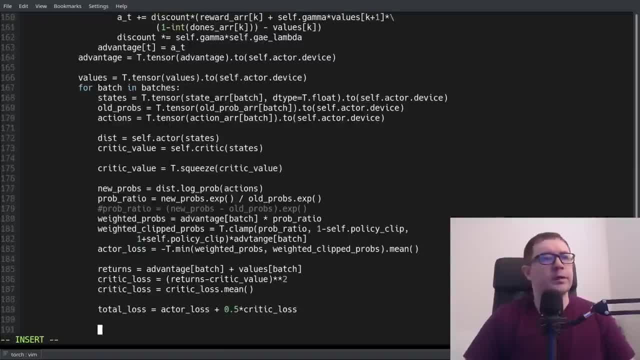 there's a negative sign in front of the actor. so we're not doing descent. that's actor. so we're not doing descent. that's actor. so we're not doing descent. that's another thing. that's kind of suboptimal. another thing, that's kind of suboptimal. 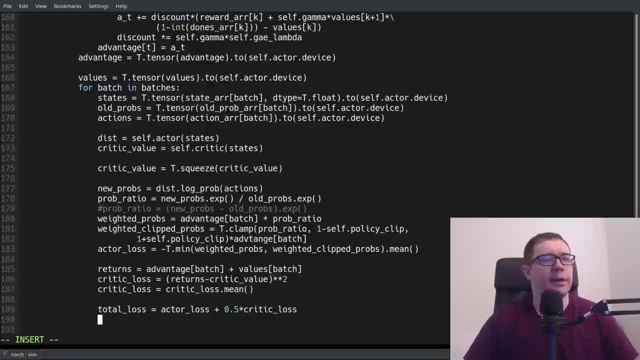 another thing that's kind of suboptimal, about the way the paper is written. you about the way the paper is written, you about the way the paper is written. you can get kind of confused about negative. can get kind of confused about negative. can get kind of confused about negative signs if you're not paying very careful. 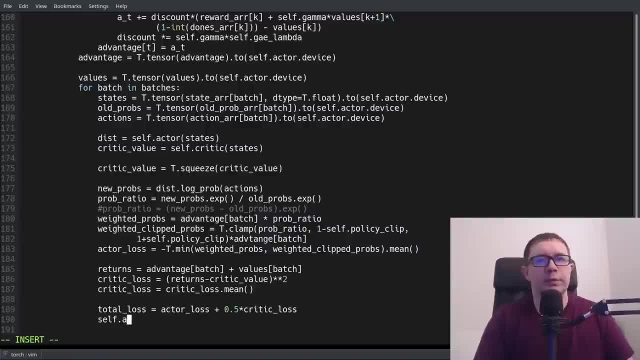 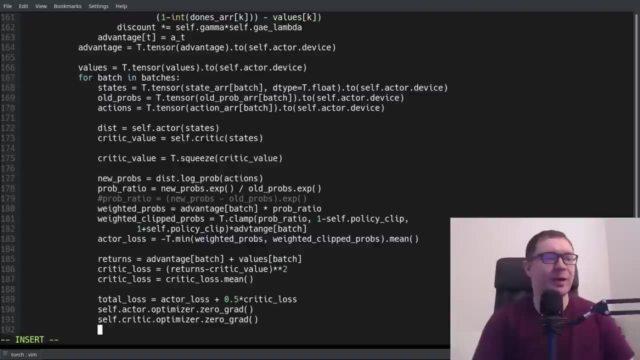 signs if you're not paying very careful signs, if you're not paying very careful attention, next we have to zero our attention. next we have to zero our Giving a concert downstairs. He's playing the drums by whacking on his toy box with some drumsticks. 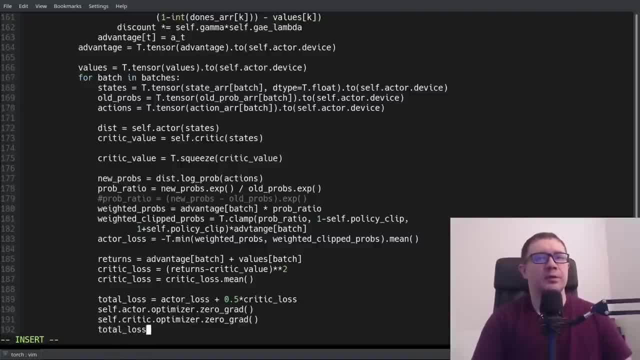 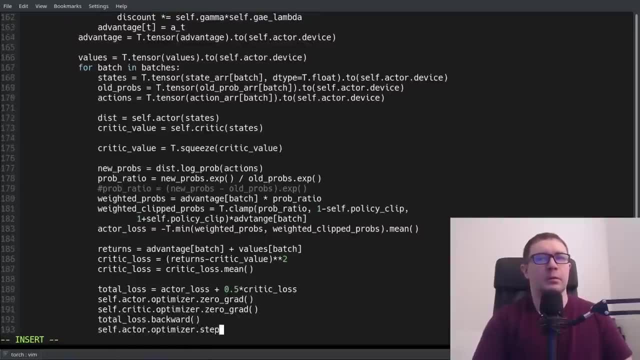 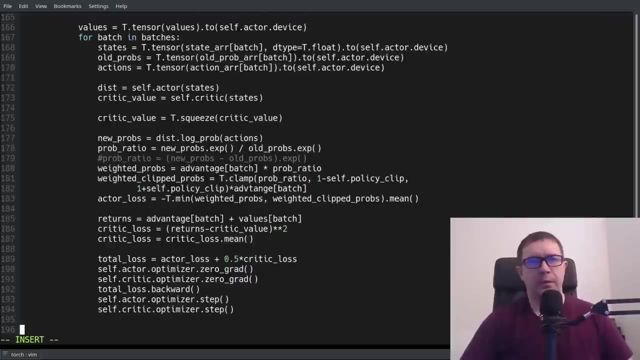 So we're gonna back, propagate our total loss and then step our optimizers And finally, At the end of every epoch- yeah, I think that's the right indentation- we want to clear our memory. So, at the end of all whoops, at the end of all the epochs, we want to clear our memory. 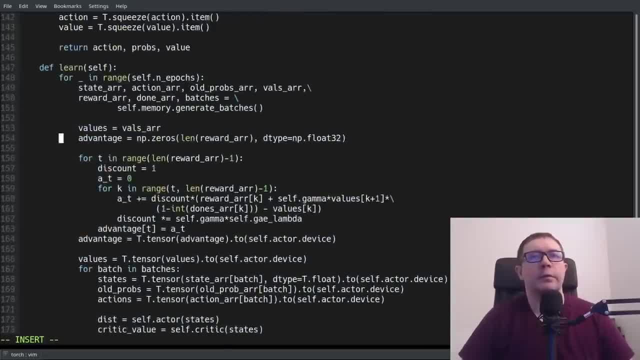 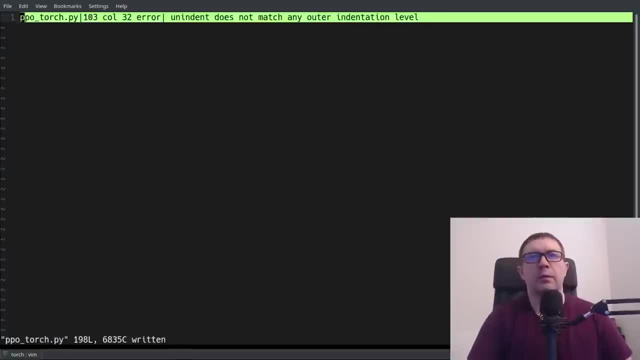 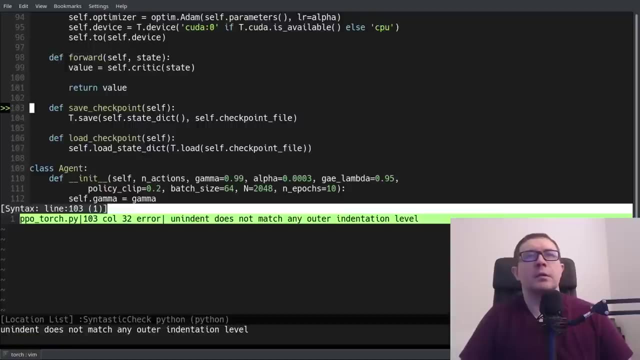 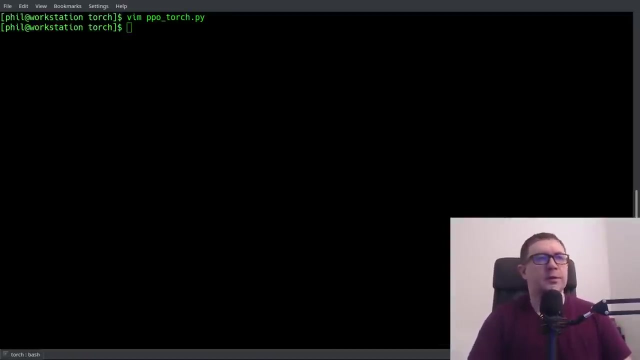 Let me just make sure I'm not Doing that Each epoch. No, I am NOT. Okay, that is good. So now let's do a right quit, and I have an indentation error here. I See That came in when I did the yank and paste. all right, so that is it for our 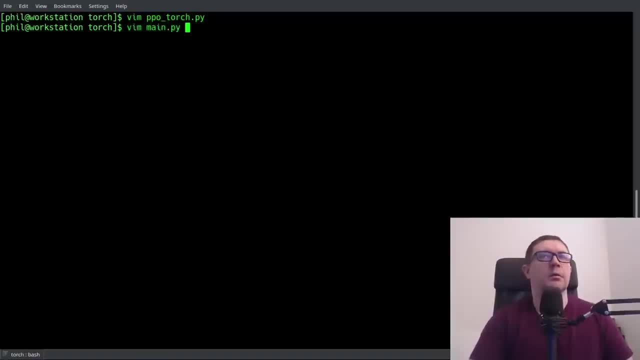 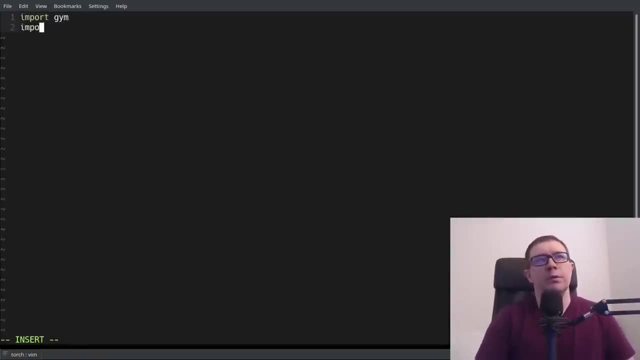 Agent file. let's go ahead and Take a look at main. so We start with our imports. We'll need a gym. We'll need numpy to keep track of the running average of our scores From PPO torch. We'll need our agent and 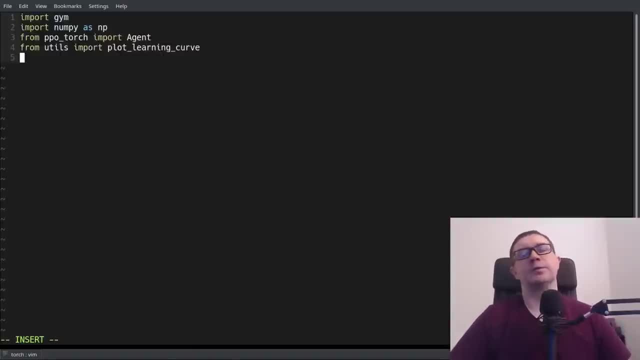 If you're new here, I have a utility file that I use, a map taught live Plot function to plot the running average of the previous hundred games For the learning curve. it's pretty trivial. You can just do a plot of the running average. Just do a git clone if you want to use my exact version. 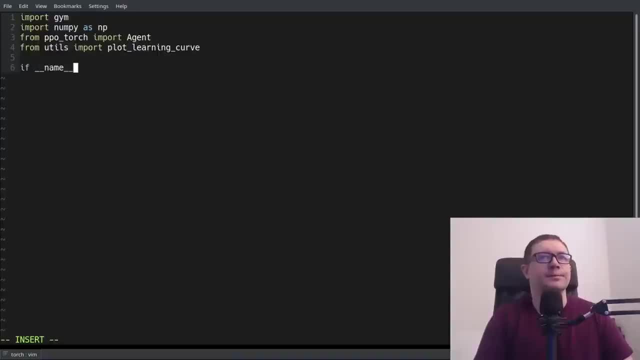 I don't go over it in every video because it's kind of redundant, but I Leave a link in the description to the github. so Go ahead and do a clone of that so you have that file or just write your own. So we're gonna use the very basic. 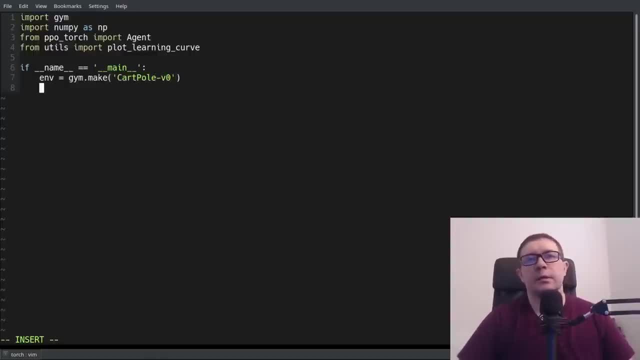 cardpull v0 Reason being. we don't need to spend a whole lot of time on a very computationally complex Environment to realize we made a mistake. so it's very easy to see if something got screwed up with the cardpull environment. this certainly will work on more advanced environments, but it does require a little bit of. 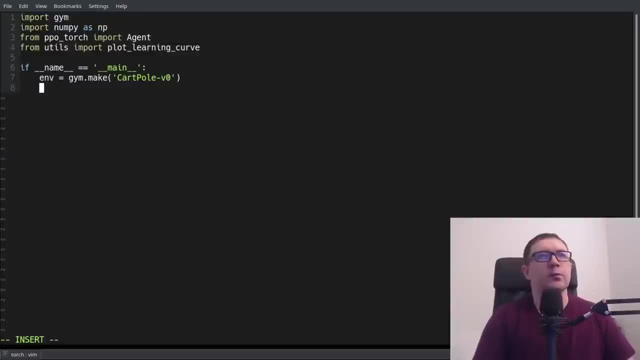 fine-tuning. so We'll just start with the cardpull and then you can play around with other environments at your leisure. so we use the parameters I dictated In the lecture. I think I changed in a review box to four Running rate of three. We can get the number of actions directly from our environment- very handy. 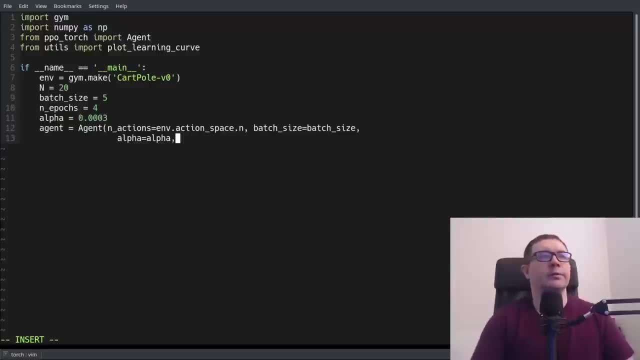 Pass in all the other relevant parameters. I Get the number of input dimensions from our environment And we're only gonna play 300 games. as I'm looking at this, I do realize that, And the parameters I did the last time I ran. I did do a policy clip of zero. 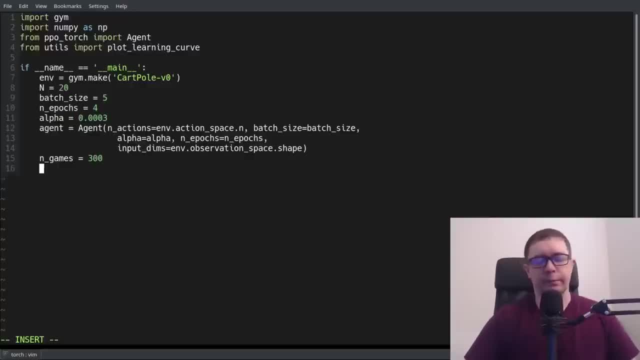 point one, but zero. point two comes from the paper and i'm pretty sure it works both ways. so we will find out. if we need to, we can go back and change the policy clip. uh, not a big deal. so plot slash cart pull dot png. we need to keep track of our best score. there's a minimum score for the. 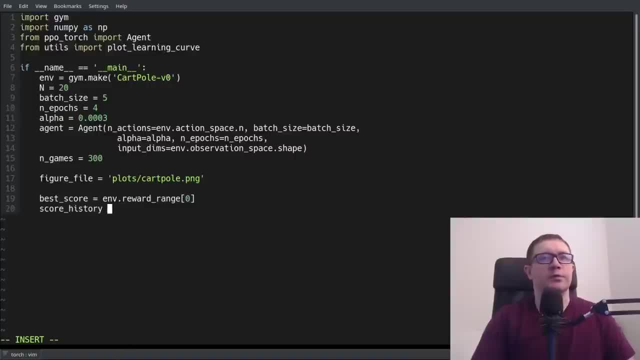 environment- empty list for our score history and um number of learned times. we call the learn function. you can make this a member variable of your agent, if you want, and an average score starting on a zero. we don't actually need that, but whatever. so we'll say at the top of: 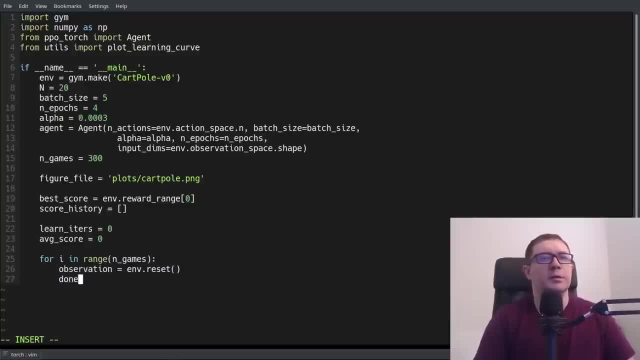 every episode. we want to reset our environment, set the terminal flag to false and accumulative score to zero. while we're not done, we need to choose an action based on the current state of the environment, um, get the new state reward done and debug info back from the environment. 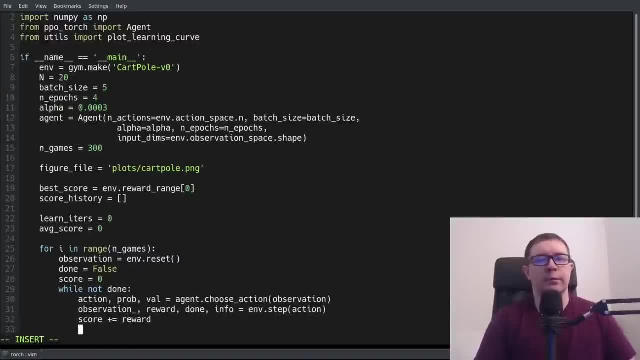 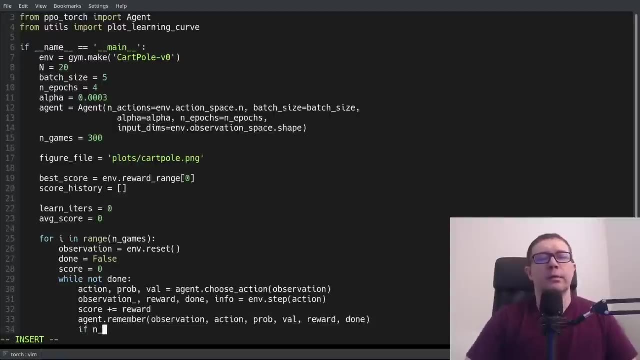 and increment our score by the reward and store that transition in the agent's memory: reward and done. and if n i do need an extra variable here, we'll say: and steps equals zero and that's the number of steps we've taken. we need that because we have to know how often or when it's time to. 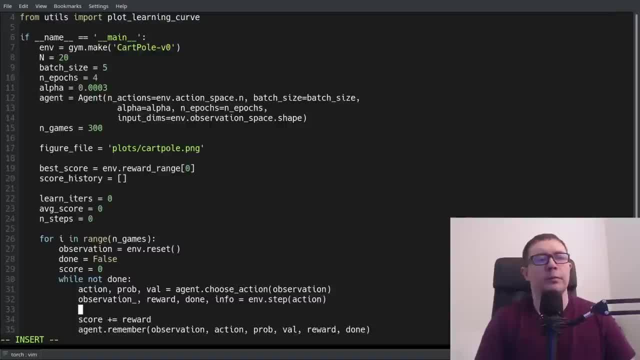 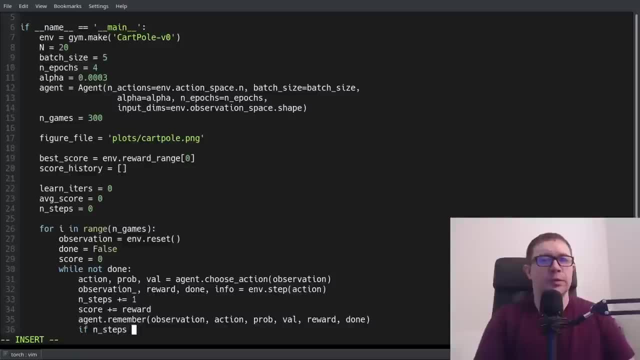 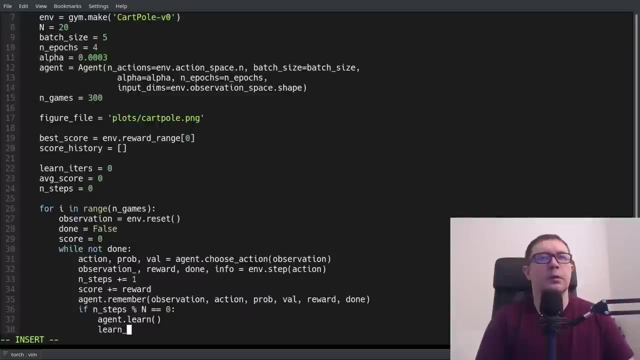 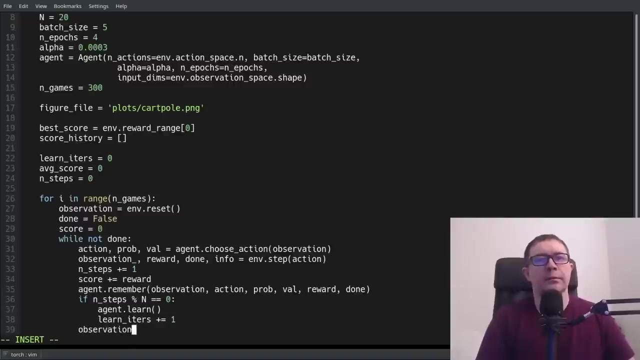 perform the learning uh function. so every time we take an action the number of steps goes up by one. so then steps: modulus n equals zero, then agent dot learn itters plus equals one, and then, no matter what happens, we want to set the current state to the new state of the environment. 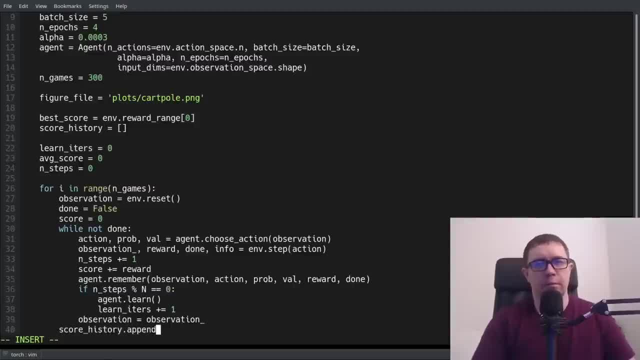 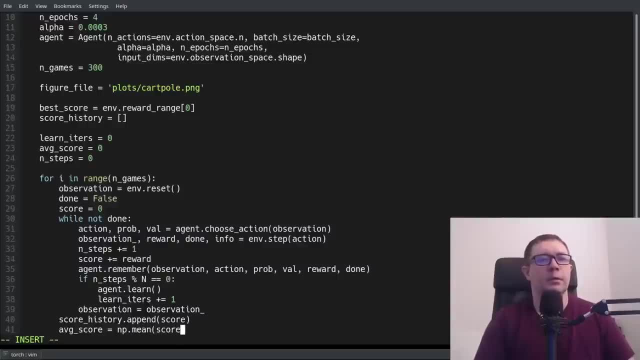 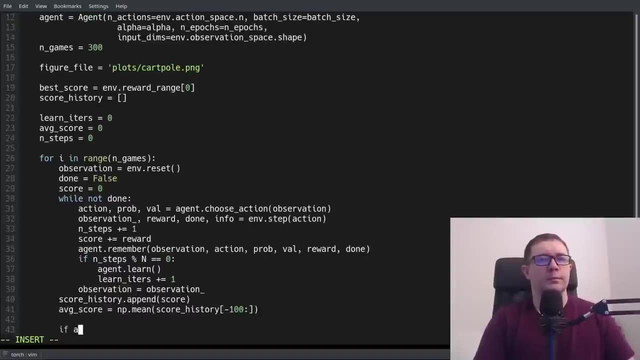 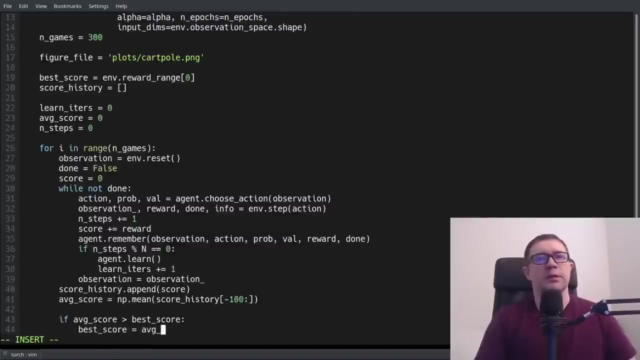 and the end of every episode append our score and calculate our mean and that's the previous 100 games. if that average score is better than the best known score, then set that best score to the current average and save your average score and then we're good to go. so we're going to. 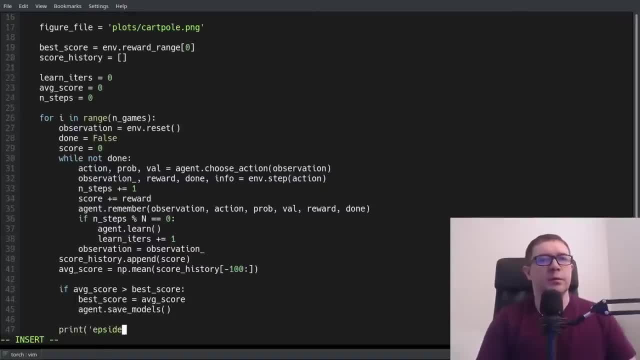 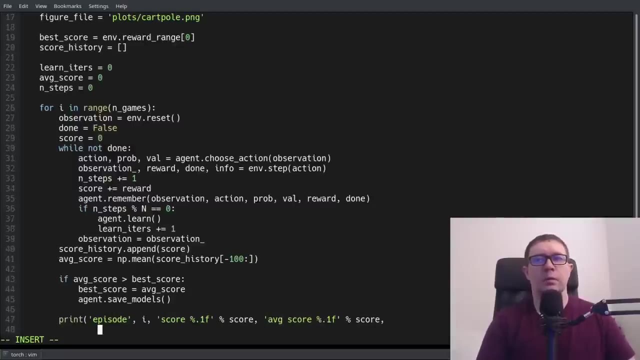 type our values in our code and run this scenario, and we also want some debug information, and we also want some debug information. we also want some debug information and we also want some debug information. is so de on score? of course, that should be an average score, the i like to print out. this isn't. 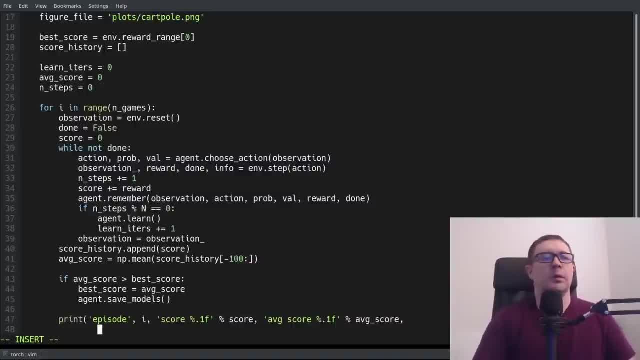 of course that should be an average score. the i like to print out. this isn't i like to print out. this isn't necessary, but the number of cases are away. but i'm going to give that a zero. an average is odd, so let's get rid of those two at all에도 and道derout. 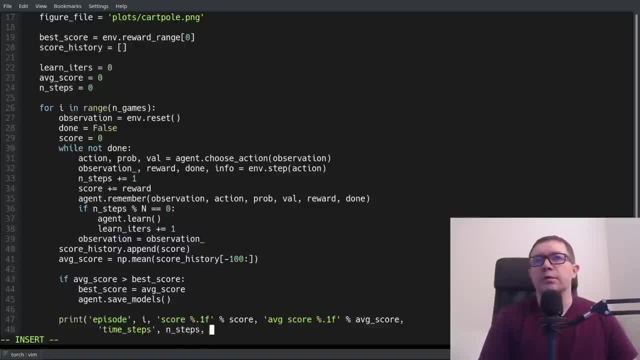 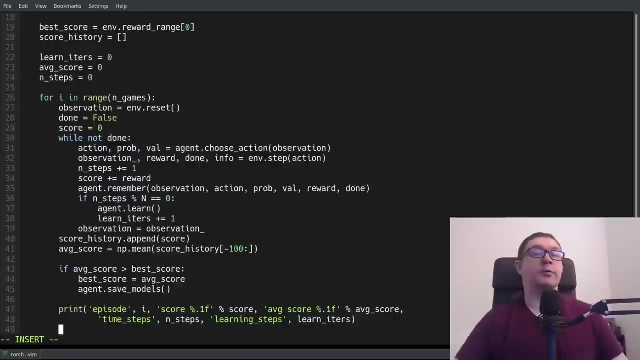 the number of steps that have transpired in total and the number of times the agent has called the learning function. this gives you an idea. this is I did this because, when I compare with the results of the paper, it wasn't clear to me if they were talking about the number of times they called the learning. 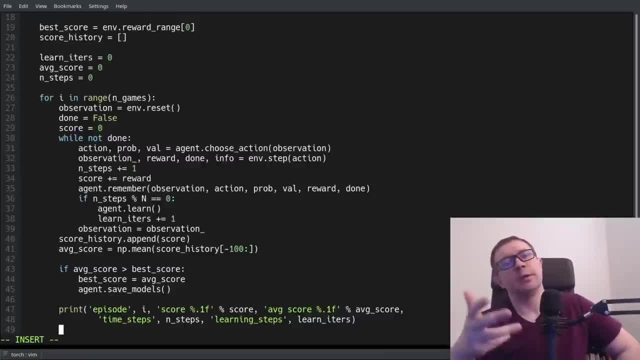 function or the actual absolute number of time steps in the environment. so I print out both his time steps and learning steps are totally optional. you don't have to print it out. it's not something that is required, so I just do it for my own clarification. we need an x-axis for our plot. lens score history. 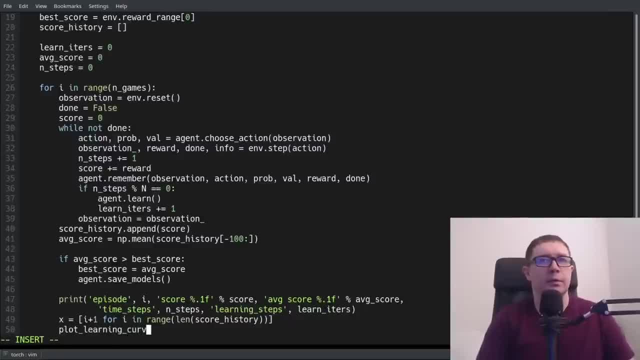 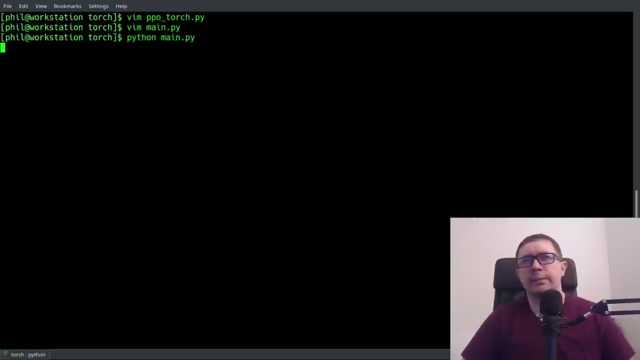 and plot learning. Oh, certainly, let's do this. We don't want to do it every single game, We want to do it at the end of all games. All right, Now, moment of truth. Let's see how many typos I made. 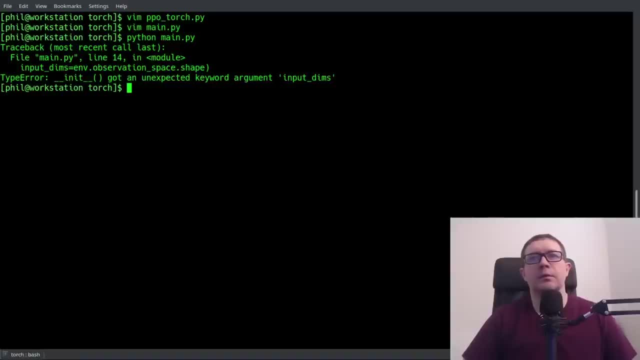 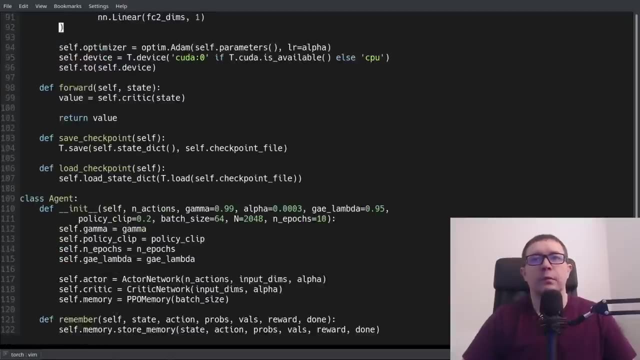 So it's telling me, and it got an unexpected argument: input dims. That's interesting. What do I call it? I don't have it there, And the reason is my computer had a hard lockup and I had to do a reboot. 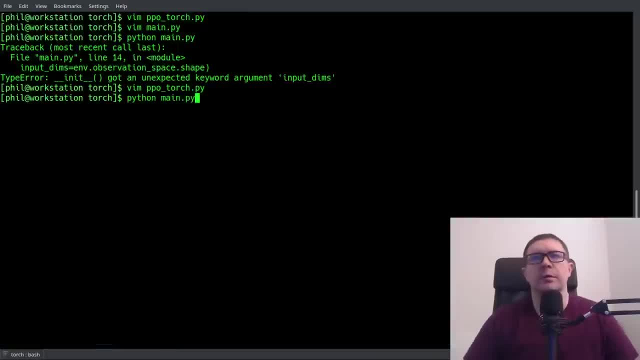 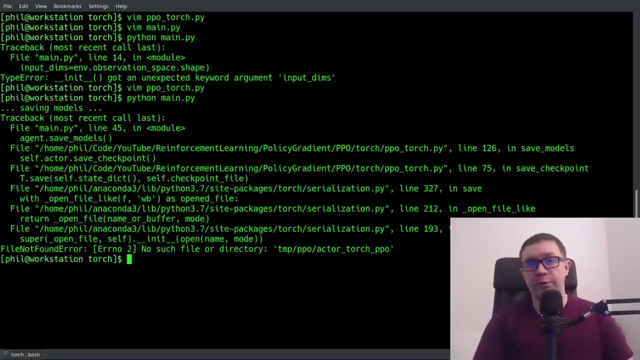 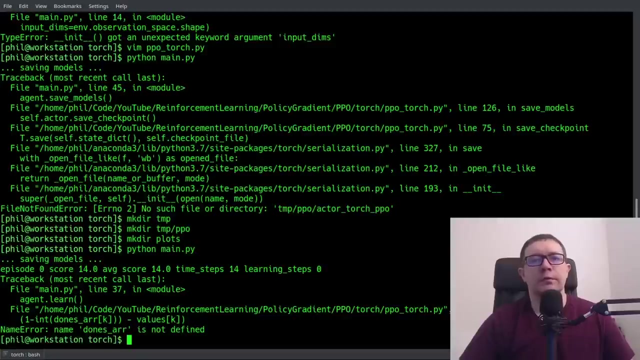 And it mutilated my cheat sheet for this, So there's bound to be some errors in here. Ah, I didn't do my make directories, So temp, PPO and plots. Let's try it again. Name done's array is not defined. 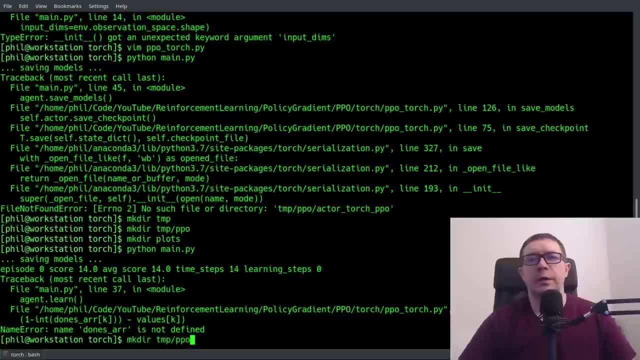 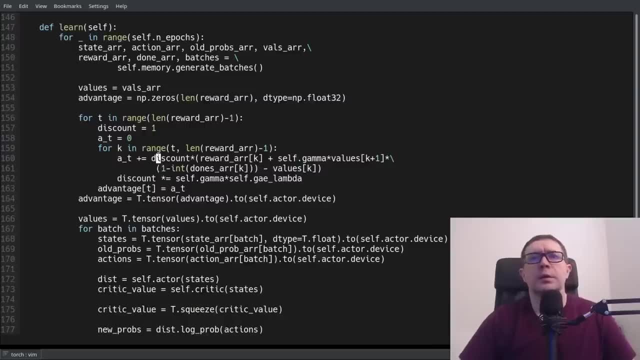 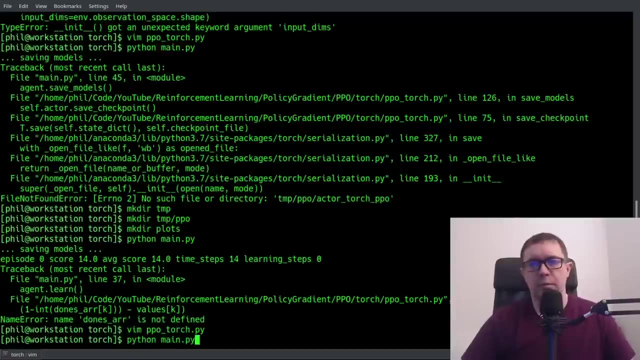 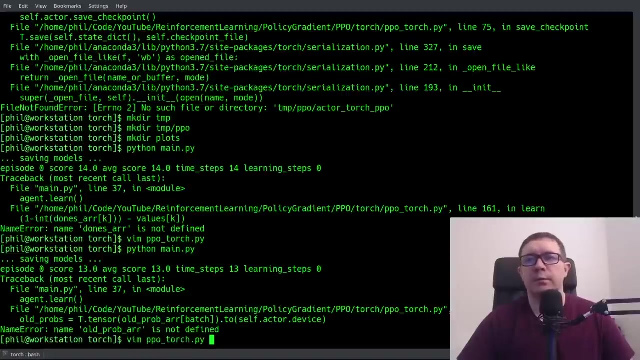 It's probably done array. That is in line 161.. So it is done's array. Yeah, We'll just change it there. I guess Old prob array is not defined. It's probably the same thing. Where am I? Yeah? 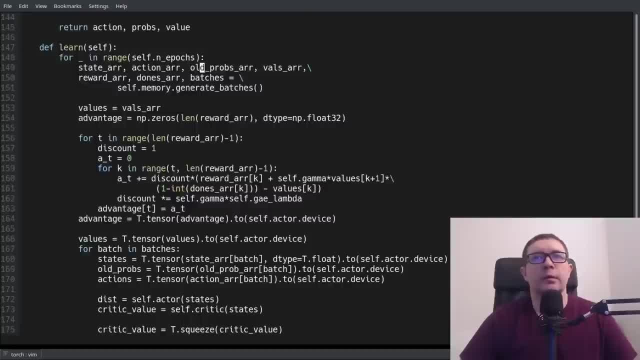 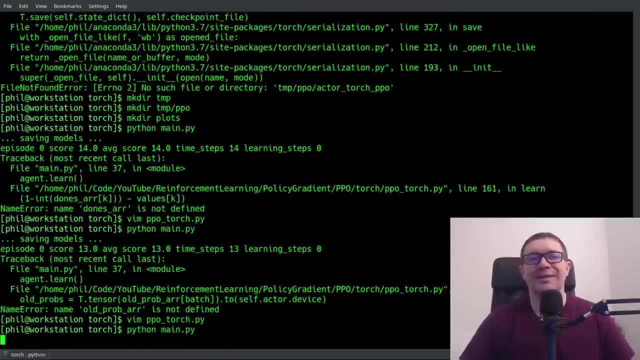 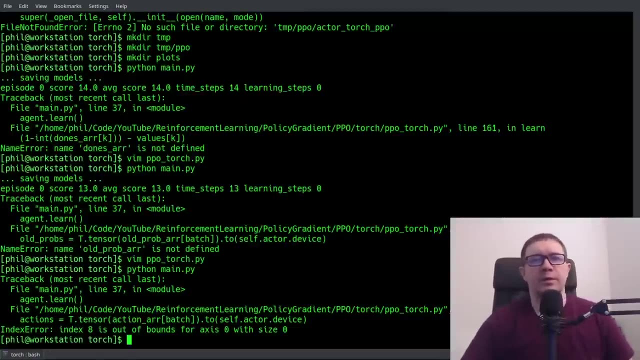 Old prob array. I'll do the opposite here. I'll make it singular just for the sake of not being consistent. Index eight is out of bounds. Okay, So then something has gone wrong. It's gone extremely wonky with the generation of the batches. 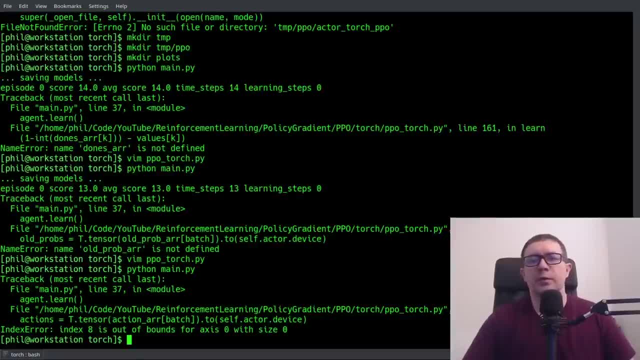 Okay, Let's take a look at that. Oh wait, let's read this a little bit more carefully. It says: index eight is out of bounds for axis zero with size zero. So our action array, oh, you know what? Let's take a look at our memory. 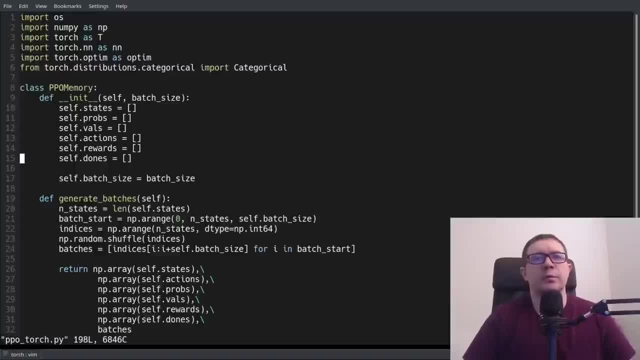 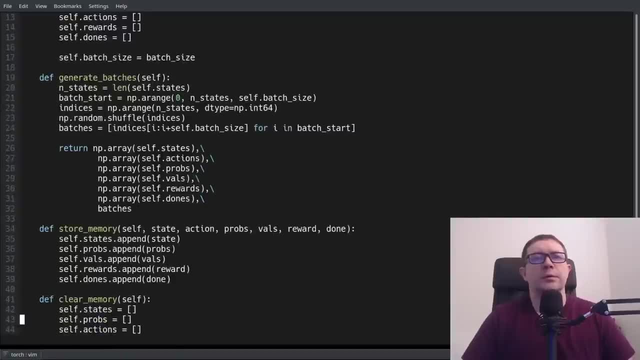 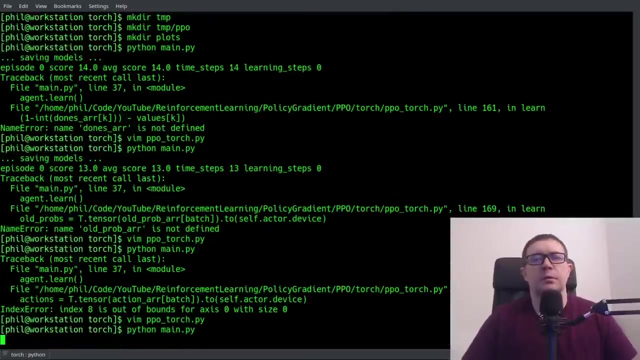 So it's action array. So here we have selfactions, We return the self actions, Selfactions. So dot, ah, there we go. That's why. So actionsappend action. All right, Now let's try it. Name advantage is not defined. 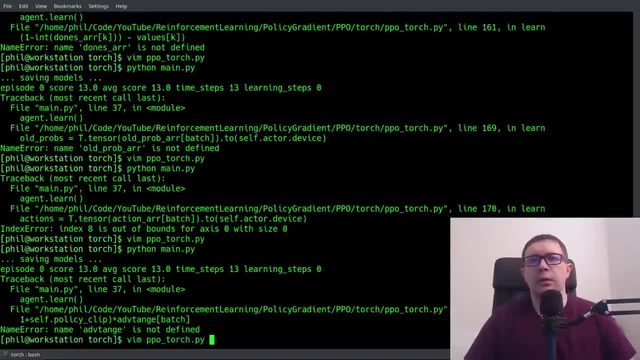 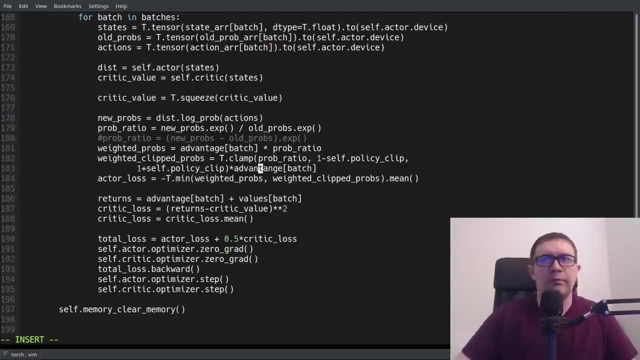 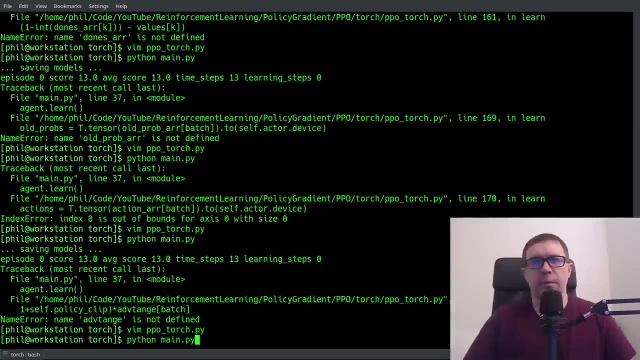 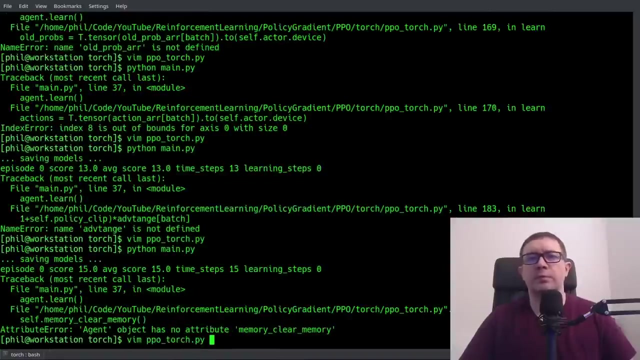 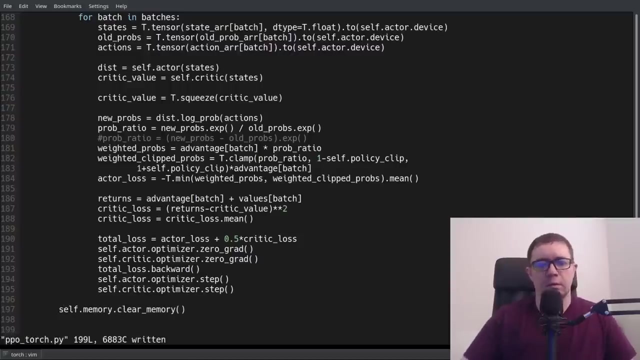 That is a typo. that is in line 183.. A advantage Did I? yeah, let's try that. Let's try it once more. Has no memory underscore. clear memory. that's memory dot, clear memory 197.. All right, 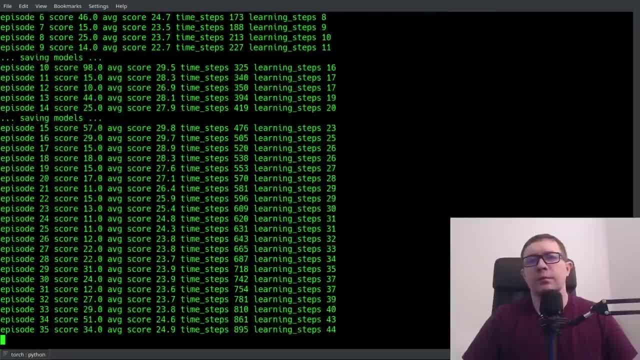 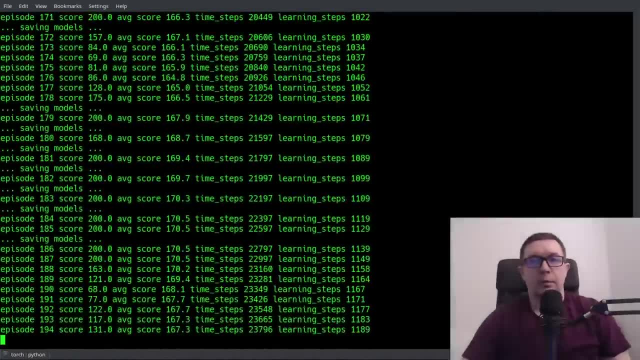 So now it is running, So I'll let that go for a few minutes. Okay, So we're going to let that go for a few minutes and we will see how it does. All right, So it has been running for a little bit, just a few minutes now. 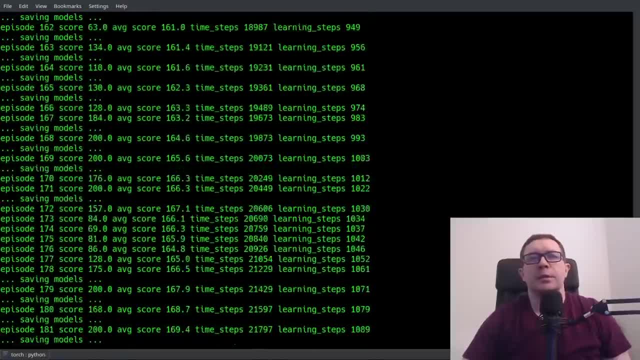 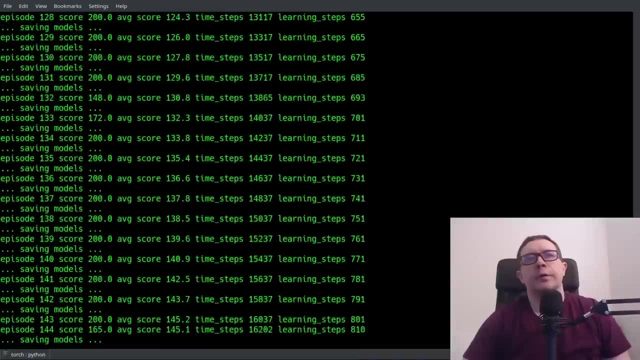 It runs relatively quickly And what I'm seeing is that we do get some oscillations in performance. You see, it will hit 200, for you know several games in a row, and then it will drop down into the mid 100s. even you know 66, something relatively low. And therefore, if you wait a little longer and you have, sir, a number 200, then you'll see that it works for a couple of times a day. So let's go ahead and repackage it. It's working. and I'll quickly get over to the first guy so that I can be able to do a teensy in three things. 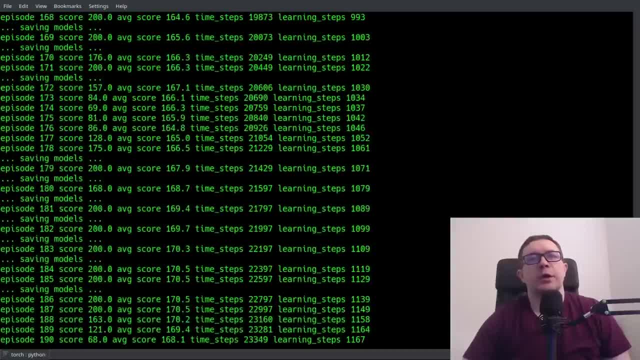 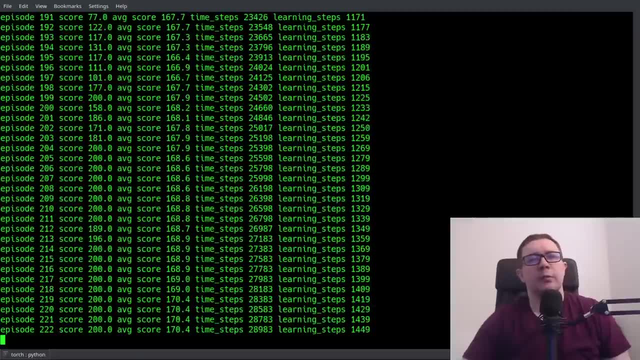 So it's good I don't have time and I'll scrap this stuff a。 low like that and there's a little chunk here where it dips below 100 points. so it's not a silver bullet, but it looks to be recovering, so we'll give it another 80 runs and see how it does. 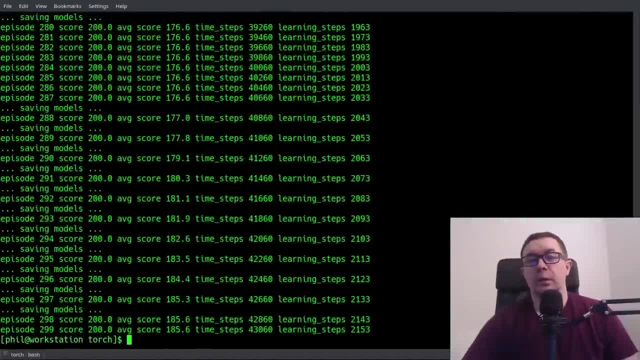 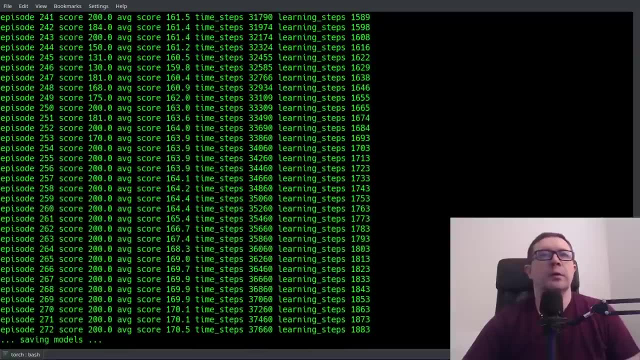 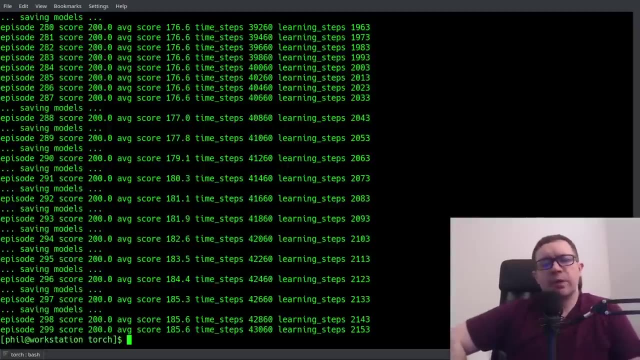 okay. so it has finished up and you can see that it finished strong with a long run of about 50 games, 45 games of a score of 200. so i commented when i was writing the agent that i was looking at my cheat sheet and had a policy clip value of 0.1. it could be that i had settled. 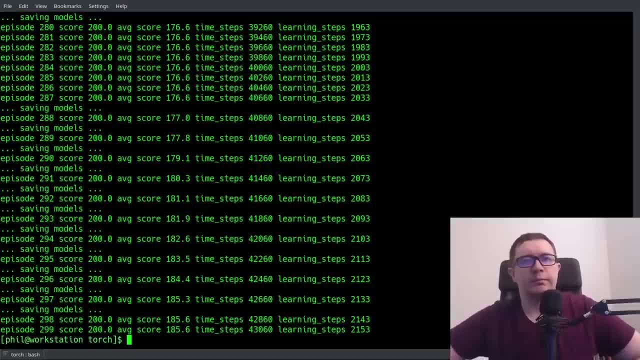 on that value based on some experimentation, and then changed it back just to be more consistent with the paper for this particular video. so that's something i would play with. other thing to consider is that there is significant run-to-run variation. that is a facet of pretty. 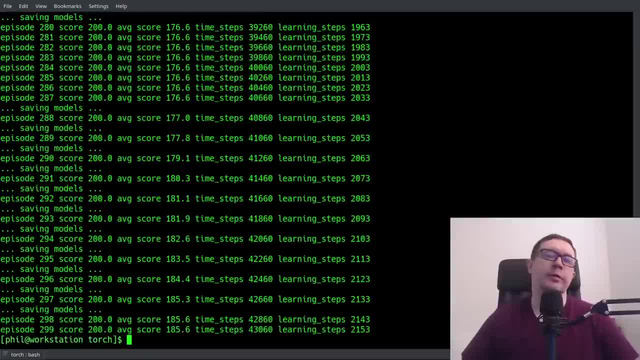 much every algorithm in deep reinforcement learning. it just has to do with the way the neural networks are initialized, as well as how the number of random number generators initialize the neural networks and how the neural networks are initialized and how the random number generators initialize the neural networks and how the random number generators. 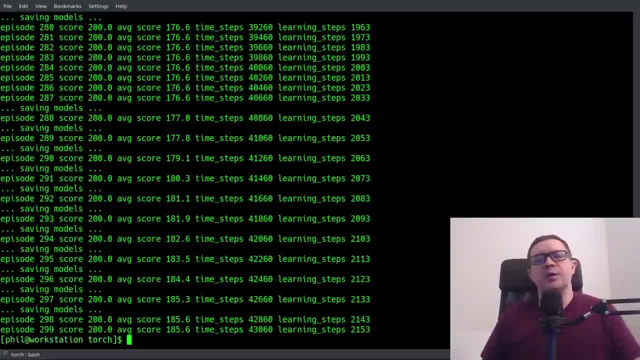 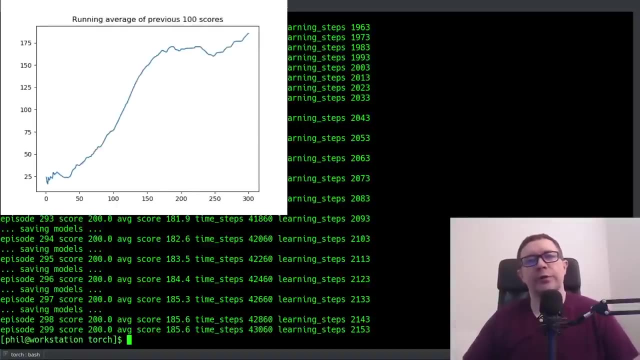 the environment. so when you see papers they'll typically report average values for, say, five or ten or whatever number of games and then a band to show the range of variance for run-to-run variation. but this is clear evidence of learning, you know, to achieve the score of 200 and under 300 games. 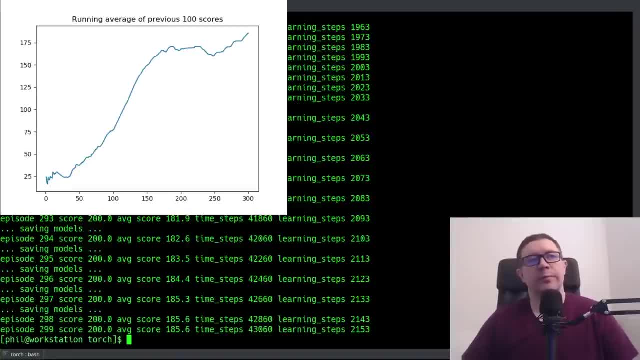 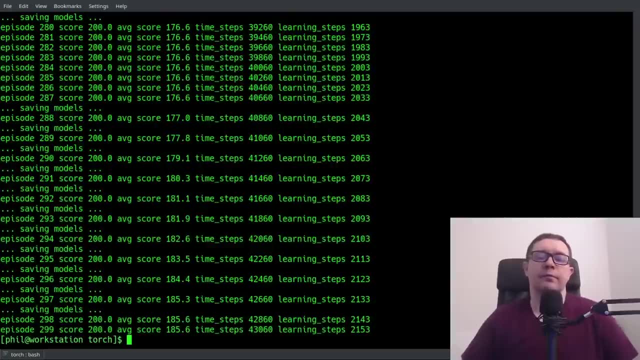 so i call this good. to me, this is fully functional. now there are a number of things you can do to improve on this. you can get it to work with continuous environments. you can bolt on some stuff for doing atari games, where you would need to add in convolutional neural networks as your input. 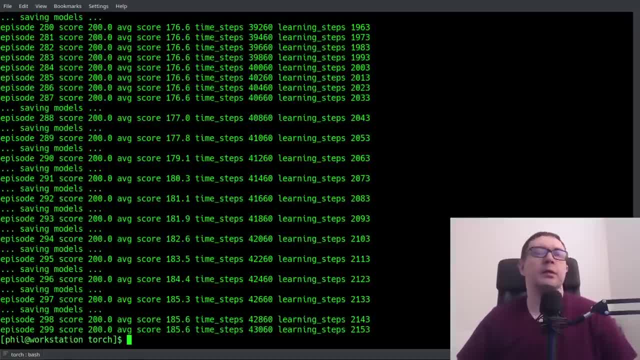 layers and then flatten them out to pass them to a linear layer for the actor and the critic. and you can see my earlier video on an ai learns to beat pong for q learning. there i go over all of the a lot of the stuff you need to do to modify the open aigm atari environment to do frame repeating. 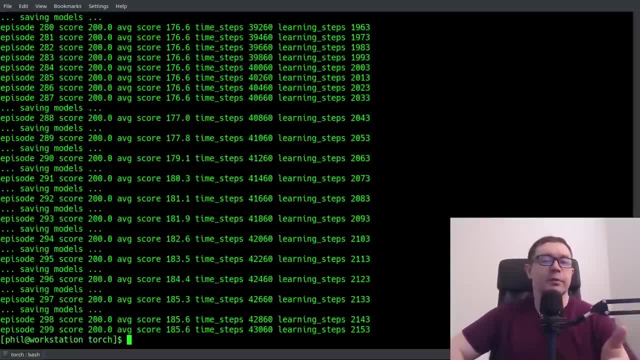 that's something they do in q learning. that's an exercise to the reader. um, actually i don't know. thinking back to the paper, i don't recall if they actually do any frame repeating or not in this particular algorithm, pvo- but it's just something to look at anyway. 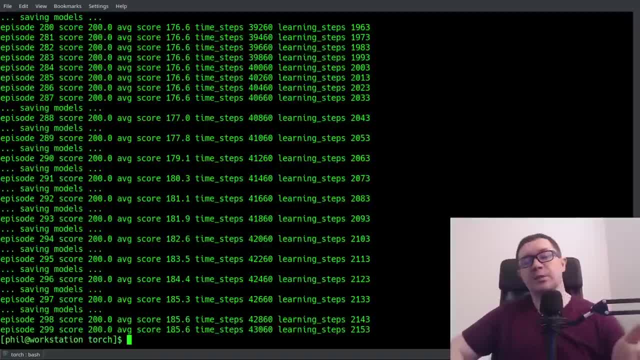 so there's a number of things you can do to improve upon it. i haven't added this module to my course yet. i'm still working on it. i really want to take some time to give more thought to the paper, because the paper isn't very well written and i'll probably have to do a lecture like one. 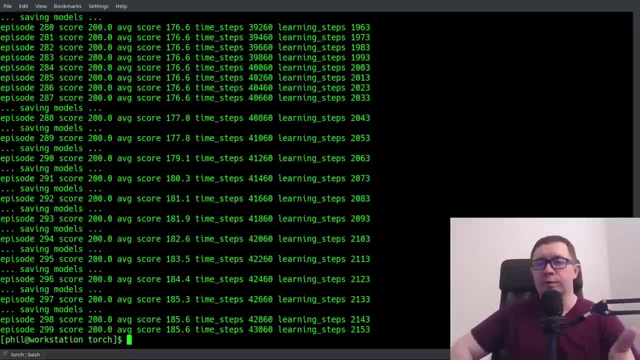 i did for uh this youtube video in the course, because the paper isn't very easy to implement just by reading it, so i hope that was helpful. that is ppo in just a few hundred lines. uh, full implementation in pytorch, solving the carpool environment. then you can easily modify this to do. 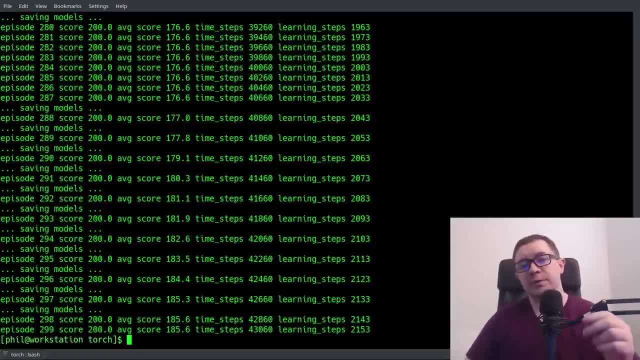 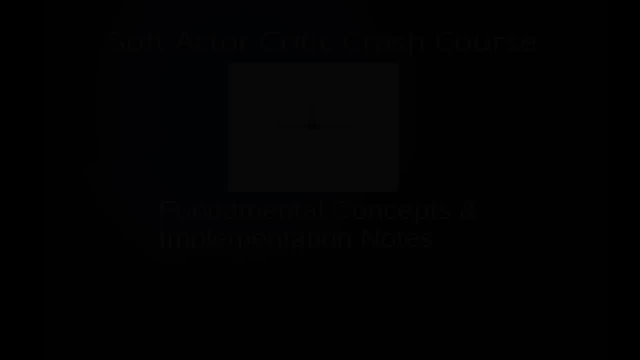 other environments as you wish. if you've made it this far, please consider subscribing. hit the bell icon, leave a like, a comment down below, and i'll see you in the next video. welcome to a crash in the world of soft actor critic methods. you're going to learn the least painful way to quickly. 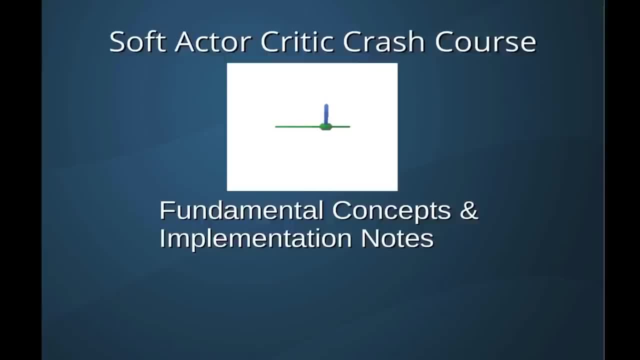 implement the soft actor critic algorithm using tensorflow 2.. we're going to implement this and test it on the pie bullet environment- the inverted pendulum- because it's relatively quick to compute. it runs pretty fast, so we'll know whether or not we got it right relatively quickly. 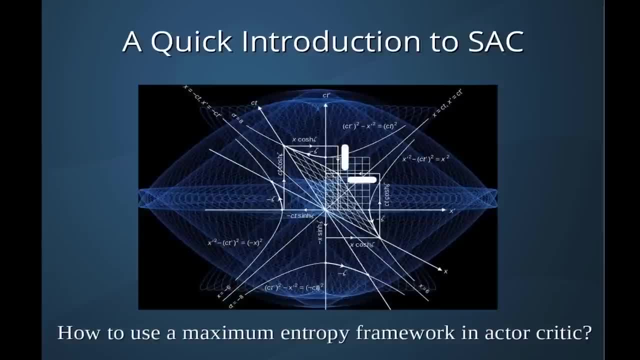 so what exactly is a solved actor critic algorithm? so this algorithm sets out to address a pretty fundamental issue in deep reading enforcement learning, which is: how do we use a maximum entropy framework in actor critic methods? we're going to go a little more detail into this in a moment, but that is the basic idea behind what we want to do. 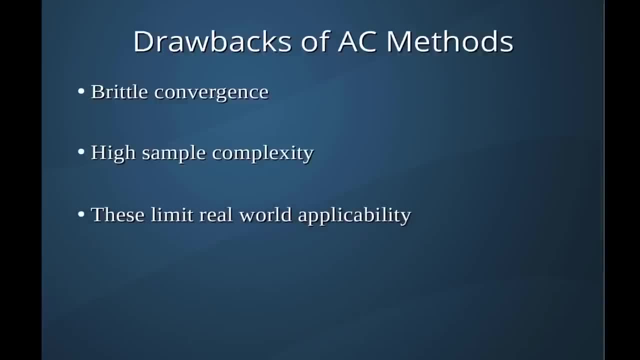 so why would this even be something worth considering? well, as you may be aware, actor critic methods have a number of fundamental limitations, not the least of which is the fact that they have what is called brutal convergence, meaning that they suffer from a high degree of hyperparameter, two and a half degrees of hyperparameter. two and a half degrees of hyperparameter. 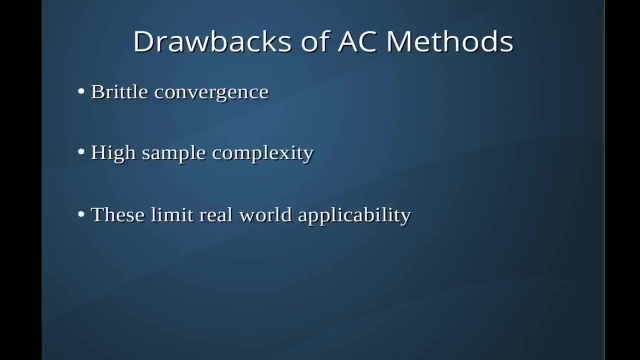 if you go monkeying around with hyper parameters, the agent breaks and doesn't know what to do in the environment, and so once you find a set of hyper parameters, you really have to stick with them. worse than that, you have a problem called high sample complexity, which is just a fancy way of 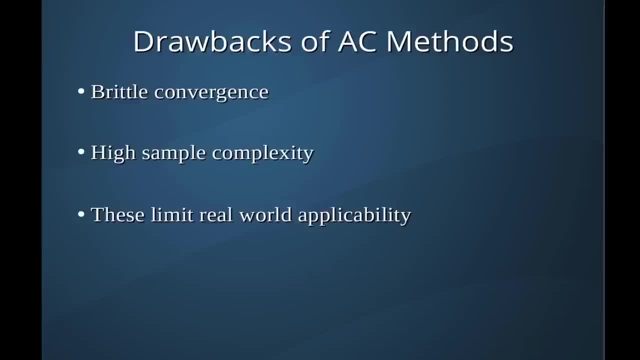 saying you need to play a whole bunch of games for the agent to figure out how it works. it's not very efficient for environments in which you have a large number of large state spaces and high number of actions in a continuous action space. worst of all these two fundamental drawbacks- 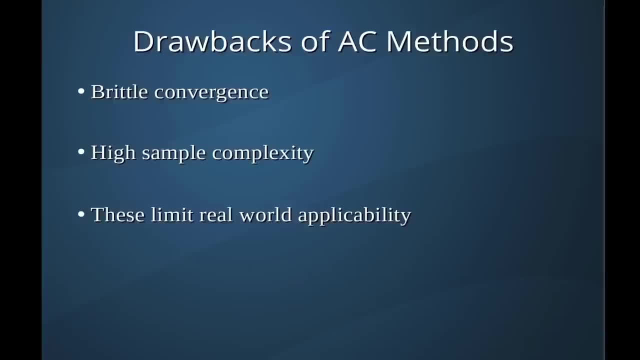 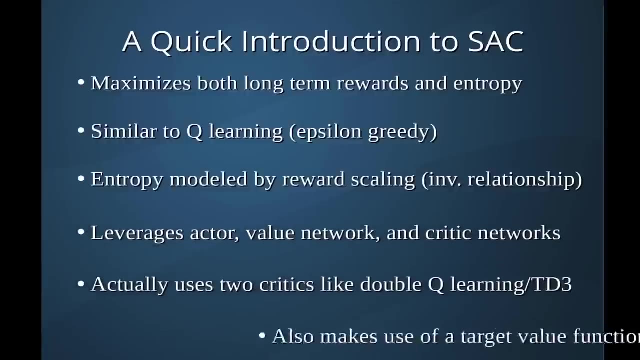 really limit real-world applicability, and it's probably one of the big reasons behind why we haven't seen any widespread adoption of deep reinforcement learning, something like, say, robotics so soft after critic. as i said, is a maximum entropy framework, and what this means specifically is that the agent is going to maximize both long-term rewards and entropy. well, what does enter even mean in this context? well, if you're working with a location, so say you might engage with community out skied orobsum and you'll even really record them during a Ohhh orbsum. on top of it, often offering the plan stronger terms, used for them 45% of the votes. you'll see more than vé to all these factors present in this margin, delivered with more pretended leverage rates. but more aren't seen. but дом pellší being important in the last part of the universe are really important days when you consider specific games. 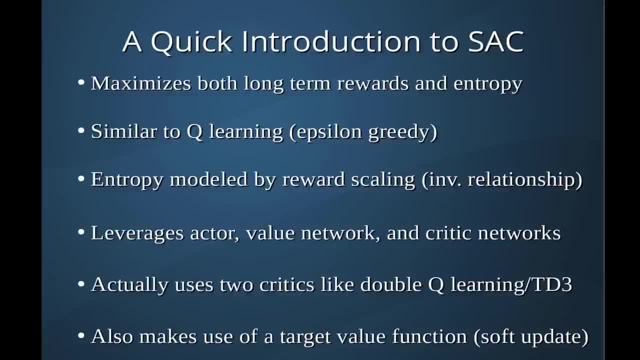 Well, if you're not familiar with the concept of entropy, it's, strictly speaking, a measure of disorder in your system. It stems from statistical physics and thermodynamics. It's basically the log of the multiplicity of your system, the number of ways of arranging the components of your system. 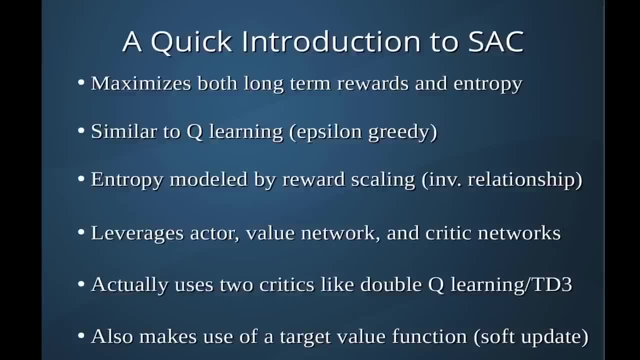 What does that mean in the context of deep reinforcement learning? It means the randomness of the actions of your agent. And you might wonder: why would you want to maximize both long-term rewards and randomness of your agent? The reason is that we need to have some degree of random actions to test our model of the world. 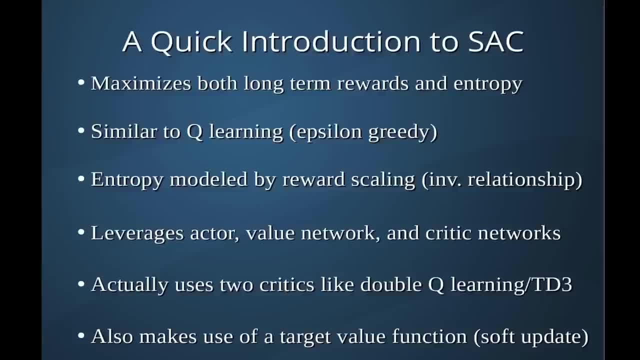 The agent starts out knowing absolutely nothing about the world and so should act as randomly as possible, And then, as it starts to figure out what actions lead to rewards, it should eventually start to converge on taking mostly those actions, but still spend some time exploring to make sure that there isn't some better action out there. 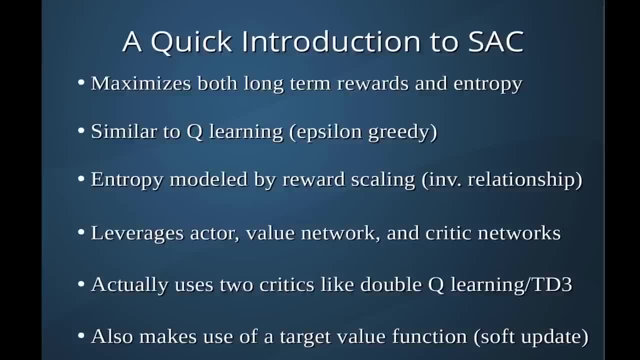 This isn't a totally alien concept to you if you're familiar with Q-learning. There we use what's called epsilon gradient action selection, where some proportion of the time- say 10% of the time- we take a random action, no matter what. even if we know what the best possible action is, we may still take a totally random action, simply because you can never be 100% certain that you're right. 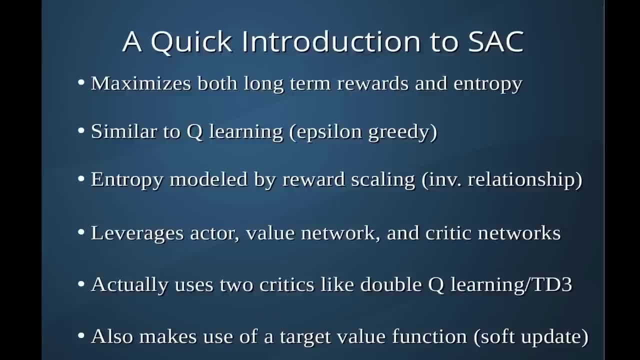 In this algorithm we're going to be modeling entropy by reward scaling, So we're going to have a multiplicative factor for our reward And there's going to be an inverse relationship between our reward scale And the degree of entropy in the system. 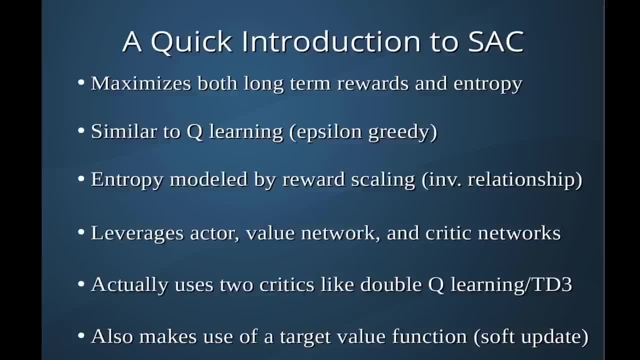 And you can kind of think of this intuitively, because if you increase the scaling on the reward, you're going to increase the contribution of that reward to the cost function, And so you're going to kind of tilt the neural network parameters towards maximizing that reward. 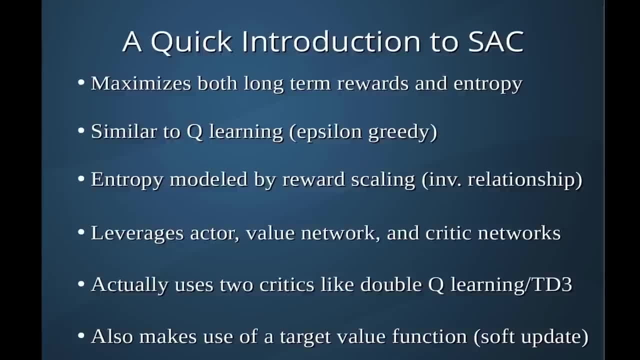 Whereas if you lower that parameter, then you're going to lessen the contribution of the signal of the reward to the updates of the neural network and so decrease its overall importance to the cost function. This algorithm is also going to leverage all the neural networks possible. 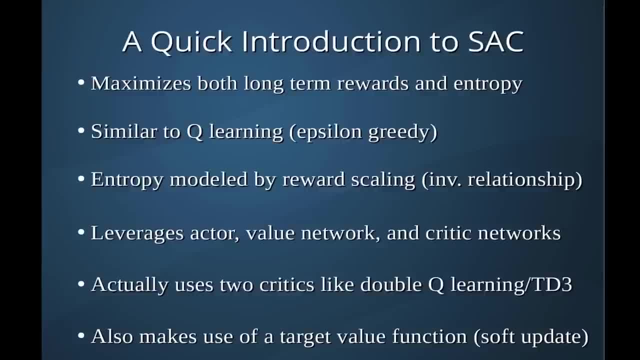 We're going to have networks for actors, value network and critic networks And, in particular, we're actually going to have two critic networks, which is going to be an exact analog of the double Q learning algorithm, as well as twin delayed deep deterministic policy gradients. 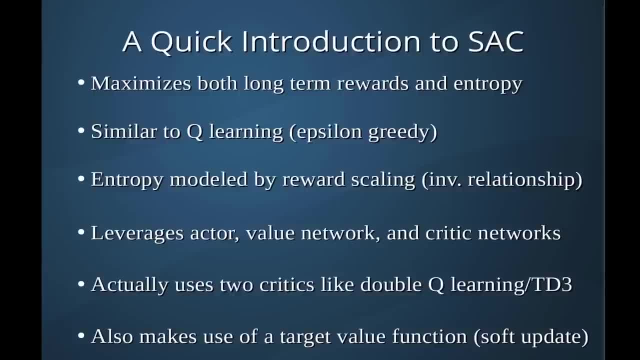 Another awesome algorithm for continuous action space environments. Please see other videos on this channel. if you don't know much about those, I have a multitude of videos covering both of those topics. They also make use of another innovation from Q learning, which is the use of a target value function. 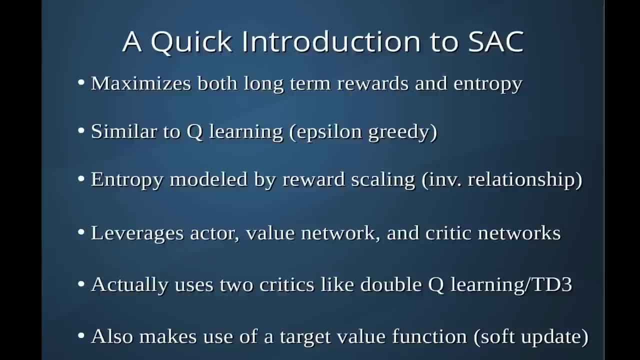 So the idea here is that we're going to be using our value function to track the values of states, to tell us which states are viable, so we can seek out those states again. That's the idea behind reinforcement learning, But the problem is that we're going to be updating that value function with each time step. 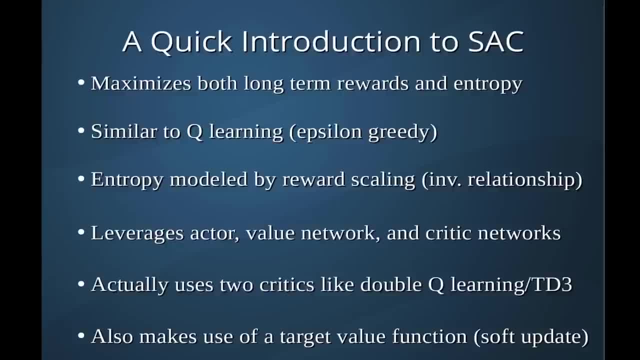 And so if you're updating it each time step and using it to evaluate the values of the states, then you're really going to be using that value function to track the values of states. And so if you're updating it each time step and using it to evaluate the values of states, 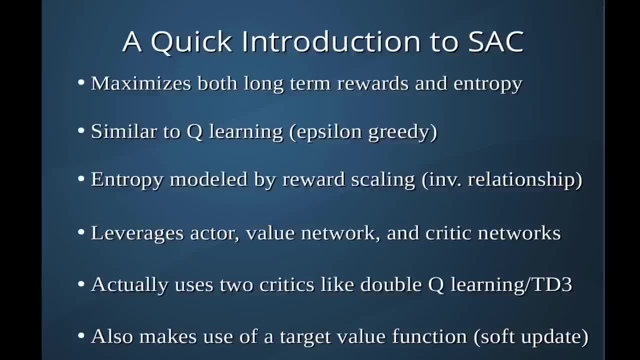 then you're really going to be using that value function to track the values of states again, And so if you're updating it each time step and using it to evaluate the values of states again, Then you're really chasing a moving target, And so the algorithm will suffer from instability. 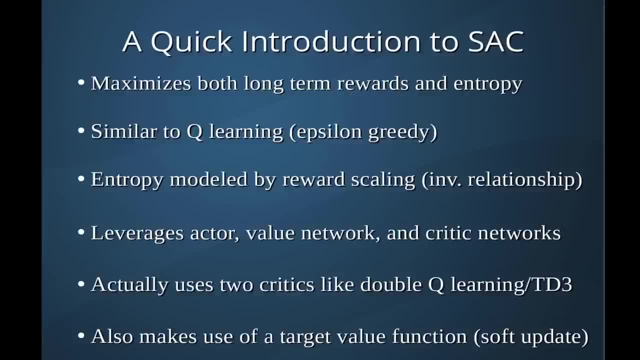 And that happens a lot in Q learning as well. The solution is to have a target value function which is updated only periodically or very slowly. So in Q learning we do a periodic update where we just exactly copy the network parameters from one network to another, from the online to the target network. 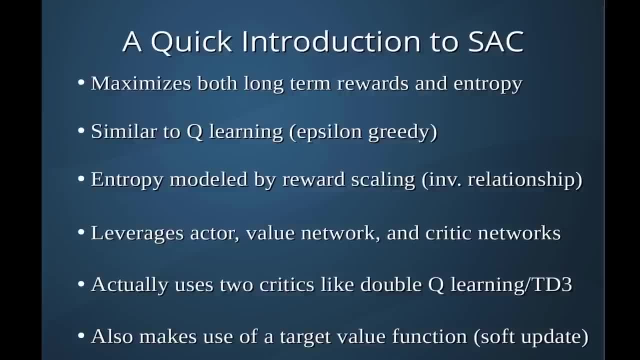 Here we're going to make use of a soft update where it's going to be some kind of moving average. So we're going to make use of a soft update where it's going to be some kind of moving average of the online and previous values of this target value network. 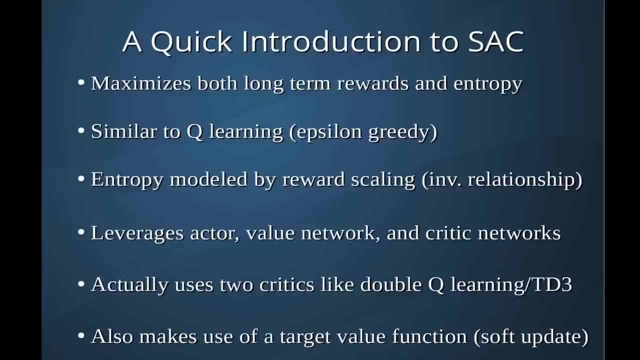 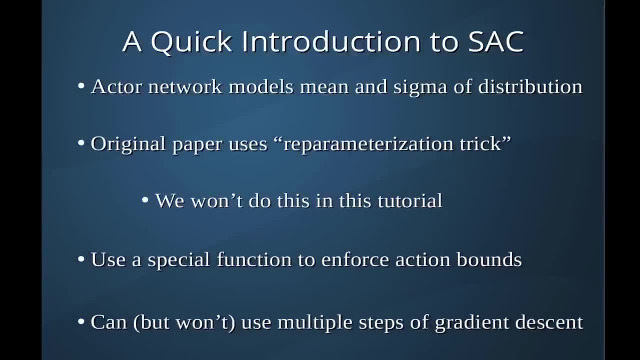 And I'll show you that equation later in this little lecture. So our actor network is going to model both the mean and sigma of a distribution. So this is a probabilistic policy. It is not a deterministic policy like in DDPG. So our actor network is going to output two parameters: a mean and sigma. 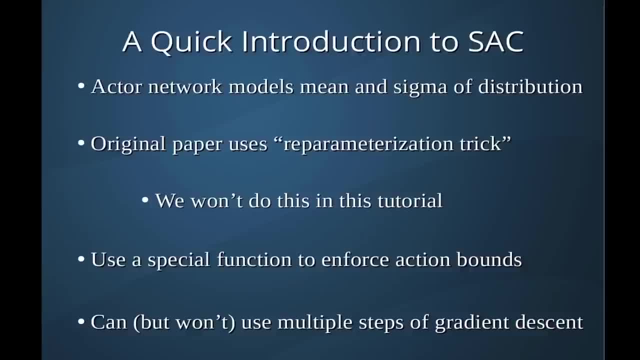 And then we're going to put that mean and sigma into a normal distribution And sample it to get an action. Now the original paper used what they call a reparameterization trick And I will fully admit I'm a little fuzzy on exactly what that means. 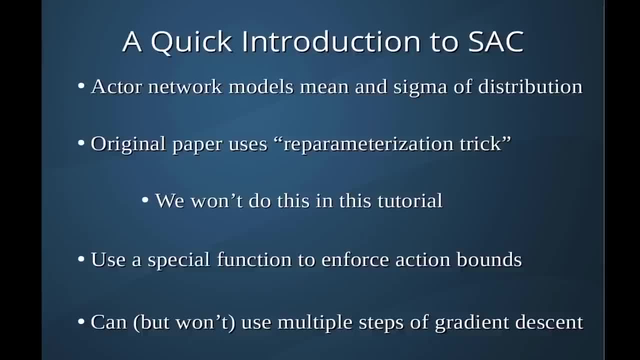 It kind of sounds like they are sampling some normal distribution and then adding on some additional noise to it. I implement this in what I believe to be a faithful implementation of this in PyTorch, But I'm not going to do it in this tutorial. 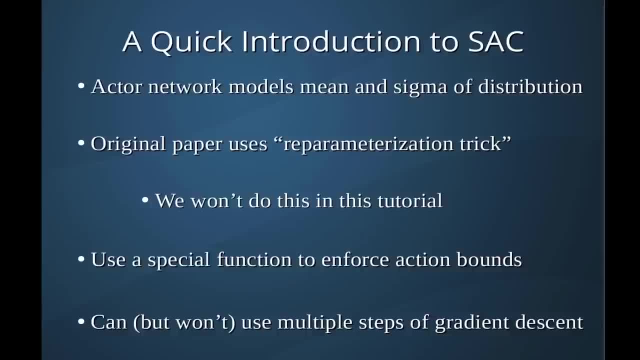 I think it's a little superfluous and I'm actually getting, you know, really good results Without it, So I'm kind of throwing it away. We do have a special function to enforce action bounds as well as to calculate the log of the probabilities of taking some actions. 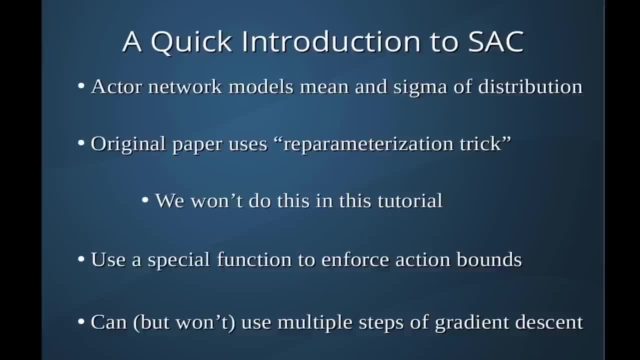 Because the log of the probability will play a big role in our update rules for our networks, which I'll get to momentarily, And I'll show you that function later on in lecture as well. Another thing to note is that we can use multiple steps of gradient descent, like we do in proximal policy optimization, or PPO. 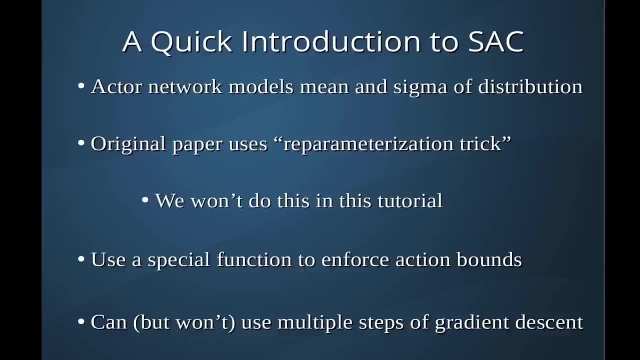 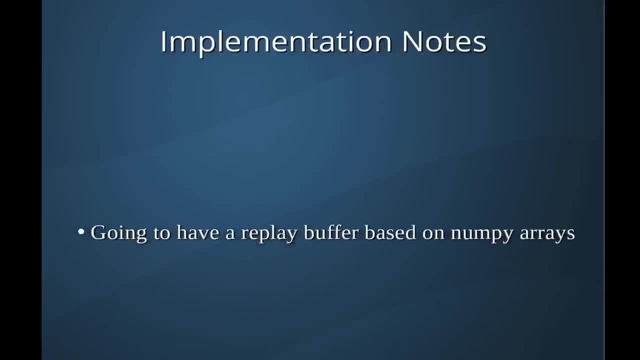 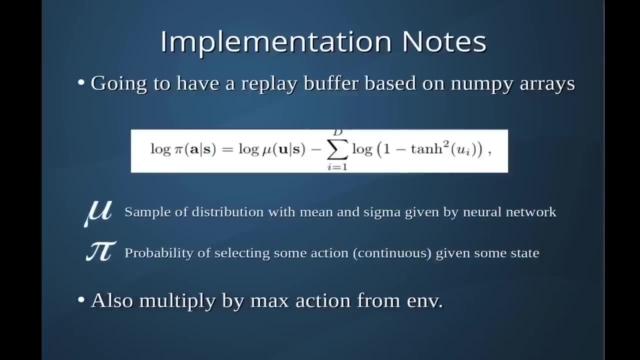 But we're not. We're not going to do that. We're going to just use one step of atom optimization per time step of the environment. Some other implementation notes: We're going to have a replay buffer based on numpy arrays. I prefer numpy arrays. 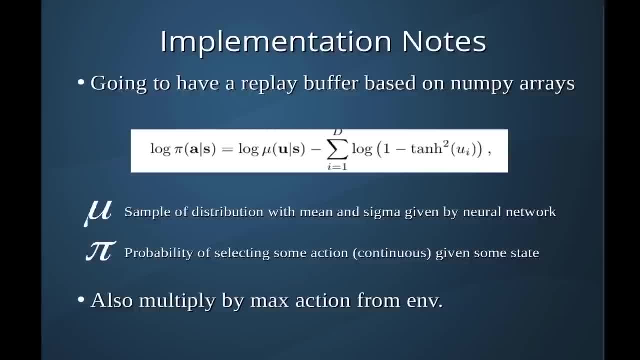 That is by no means the only way to do it, Not even necessarily the best way. It's just my preferred solution. Change that if you want. Now we're going to keep track of the states. the agent sees, the actions it took, the rewards it received. 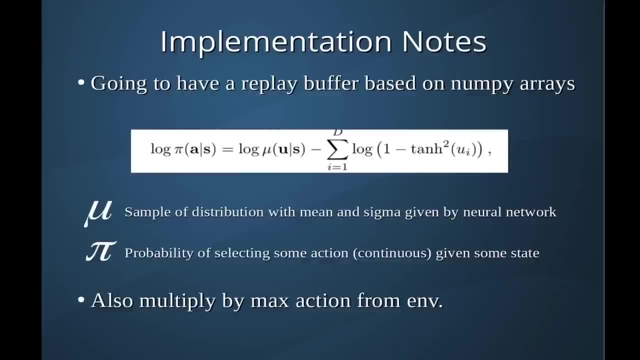 The new states that resulted from those actions, as well as the terminal flags from our environment. And the terminal flags are important because we have to use that in the update for our deep neural networks, Because when we're evaluating the values of states, we have to take into account whether or not that state was terminal. 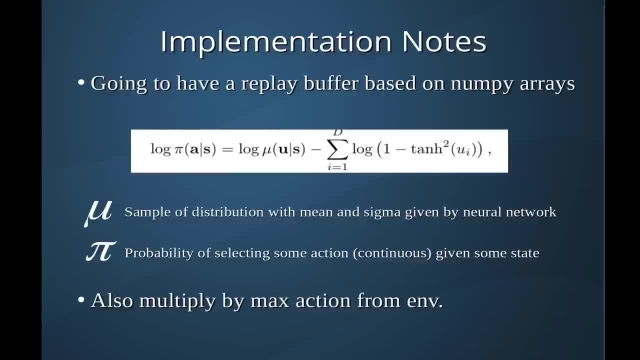 The reason is that terminal states have no value because the episode is over and no future rewards follow. The value is just the present value of the discounted future rewards, So if the episode is done, it's zero by default. Now this is the equation I alluded to earlier, where we were calculating the log of the probability of selecting some action given some state. 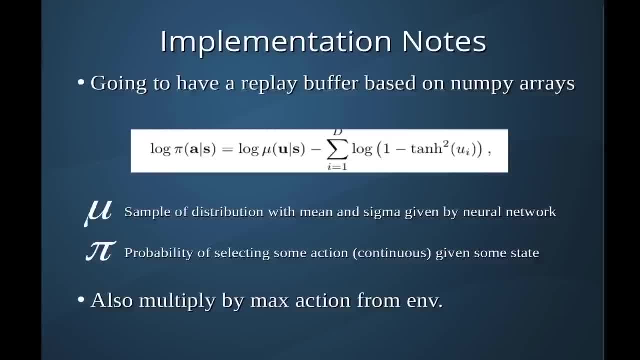 That's what that pi means. It's the probability of selecting an action, which is a continuous parameter given some state. This mu is our actual sample of a distribution with mean and sigma given by our deep neural network. So what is not the output of our deep neural network is the sampling of a distribution where the mean and sigma 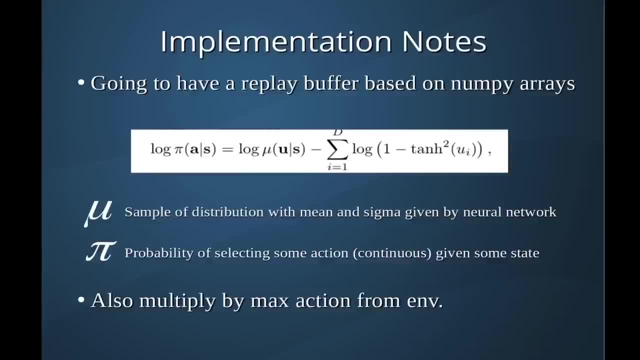 which are given by our deep neural network. And another thing to note here is that we are going to have to multiply our action by the max action from the environment. Reason being is that the action is going to be proportional to the tan hyperbolic function. 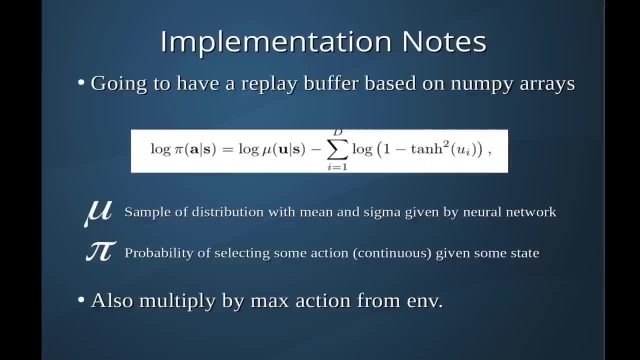 And that is bounded by plus or minus one, which not all environments are bound by plus or minus one. So you want to take into account that fact. We don't want to cut off half of our action space arbitrarily, So let's talk about updating our deep neural networks. 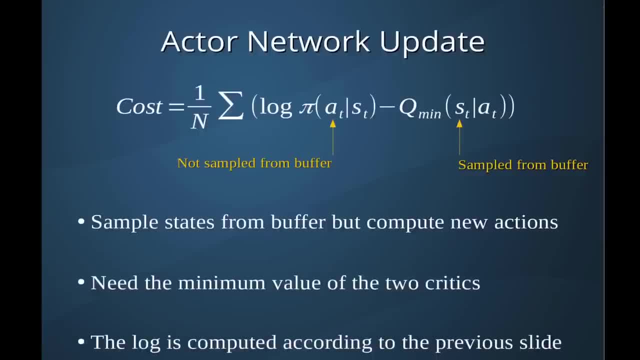 Our actor network update is pretty straightforward. What we're going to do is sample states from our buffer but compute new actions. So this is an off policy learning method where we're going to be using samples generated by one policy to update some newer policy. 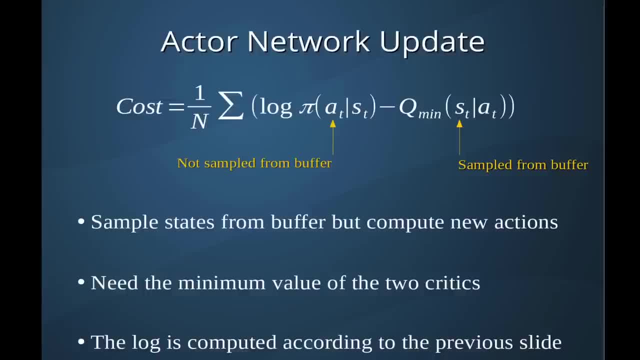 We're going to stick those states through our actor network and get new actions out on the other end, Compute that log. So we're going to do that. We're going to do a log prob based on what we saw on the previous slide. 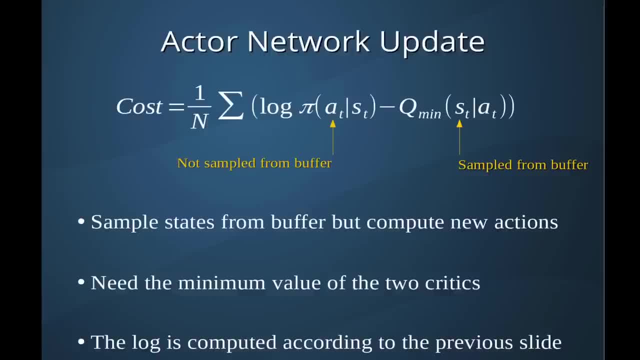 And then we're going to subtract off the minimum value of the two critics. So we're going to pass the states sampled from our buffer, the actions computed in our update according to the current values of our actor network, and then take the minimum of the critic evaluation of those state and action pairs. 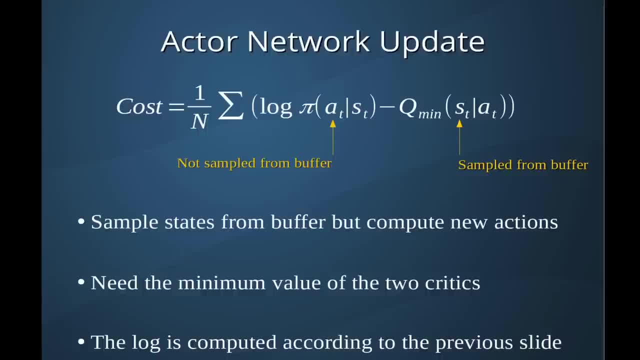 This is kind of the double Q learning rule in action. So that's why it has Q min And the one over n sum tells you that we're taking a mean of that quantity, That difference, Our value network update is a little bit more convoluted. 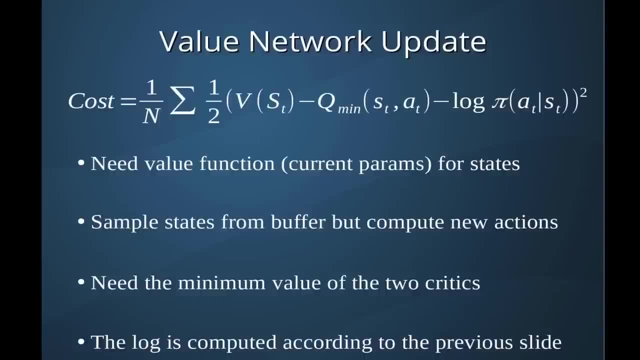 So we're going to have one half the mean squared error. That's what the one over n and one half of the difference squared tells you of the difference between the value function using the current parameters of our value function for the state sampled from our buffer. 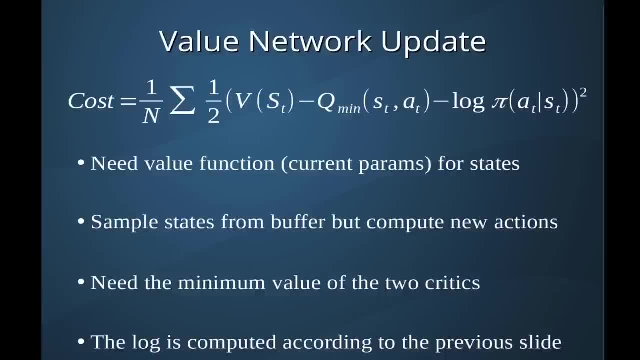 Again, we're going to subtract off the minimum of the Q values where the actions are chosen According to the new values of our actor network, and we're going to again subtract off that log of pi where again the action there is computed according to the current values of our actor network. 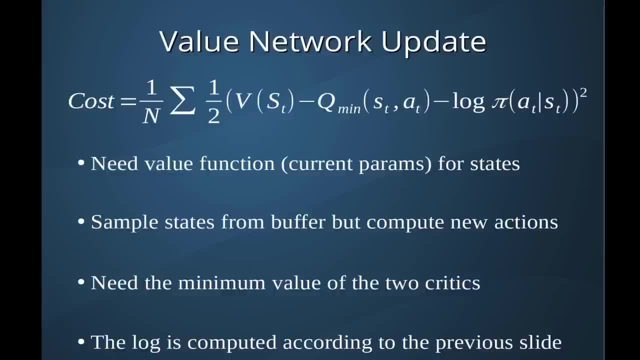 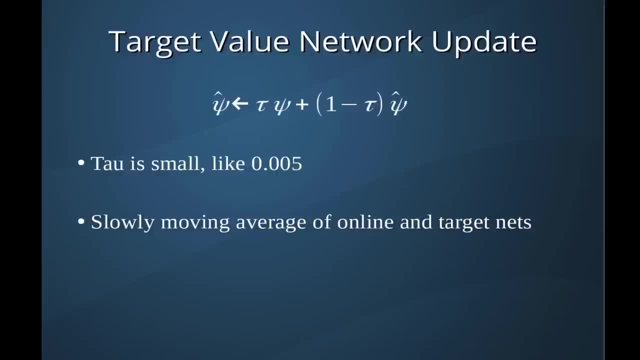 And again, the log is computed according to a couple of slides ago. The target value network, on the other hand, doesn't get any gradient descent to determine its new parameters. We're going to be updating its parameters with the following equation: So we're going to take this hyperparameter. 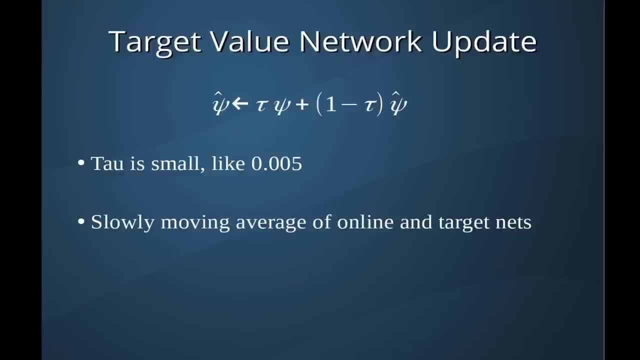 Tau and multiply it by the values of our online value network given by psi. That's just the symbol for the parameters for our value network And we're going to add on one minus tau. So point nine nine five multiplied by the current values of the target value network. 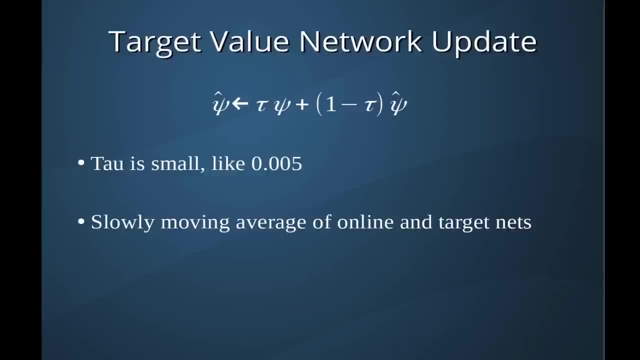 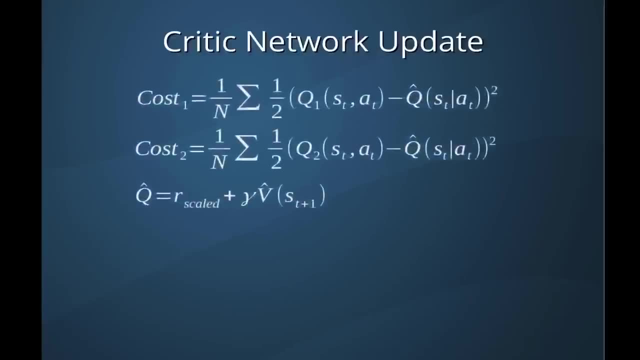 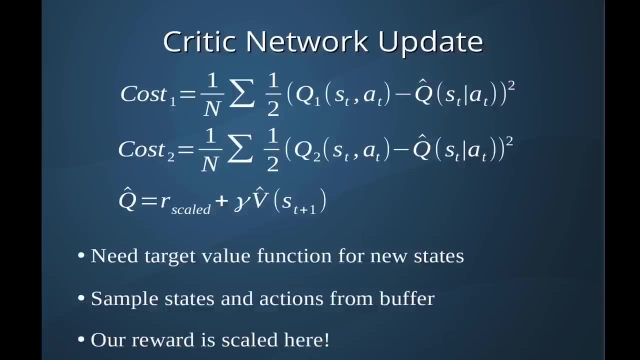 Take the sum of those two and upload those values to our target value network And it's a slowly moving average of online and target networks. Our critic network Gets a rather interesting update. So here both critics get updated, So there's no minimum operation here. 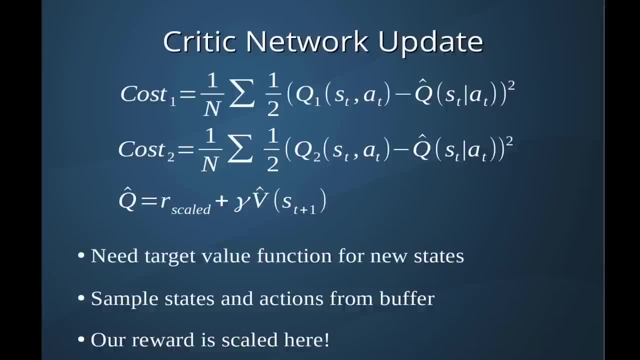 So there's two cost functions, one for each critic, and it's just given by the mean squared error of the difference between the output of the critic for the states and actions sampled from the buffer, And we're not calculating new actions here. That is one difference between the update of the critic and the actor and value networks. 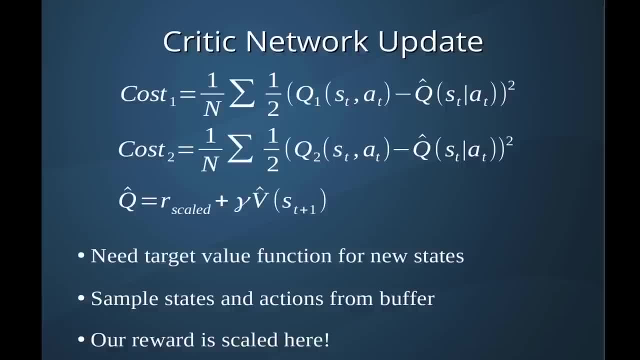 And we're subtracting off this quantity q hat, And that is where the Actual entropy comes into play. So it is a scaled reward plus the values of the new states according to our target value network. So this is where all the magic of the algorithm happens. 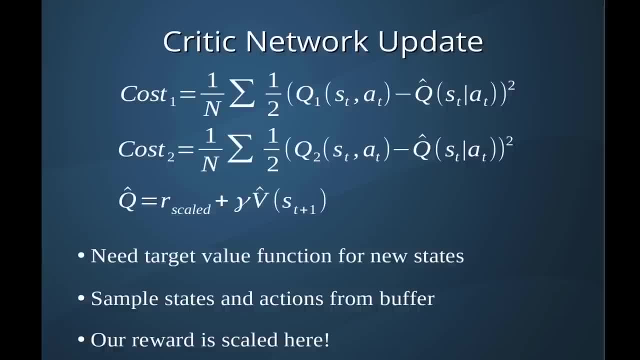 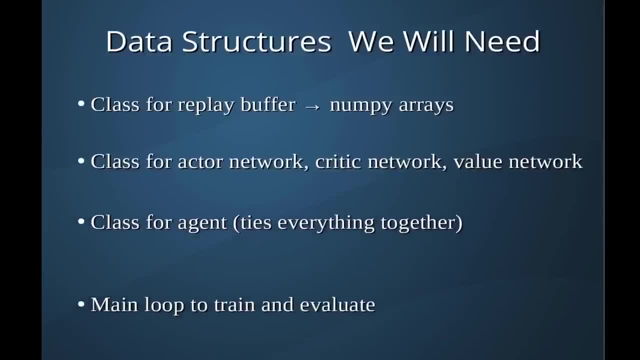 That's where the maximum entropy framework comes into play in this one little equation. Kind of neat, huh. So we're going to need a whole bunch of data structures, a class for our replay buffer- Again, that'll be numpy arrays. The actor network gets a class. 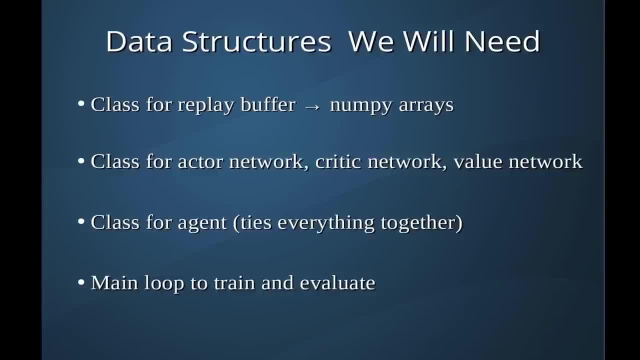 A critic network gets a class, So does the value network. Our agent gets its own class and that's going to tie everything together. That'll have functionality for choosing actions, saving models, learning as well as saving memories, And we will have a main loop to train and evaluate the performance of our agent. 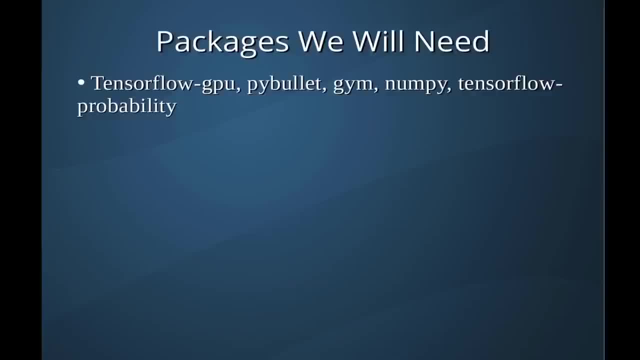 Now we're going to need a number of packages. We'll need TensorFlow. I prefer GPU. obviously, This is a highly computationally expensive algorithm, So if you have the GPU, please use it. We'll need PyBullet for environment. 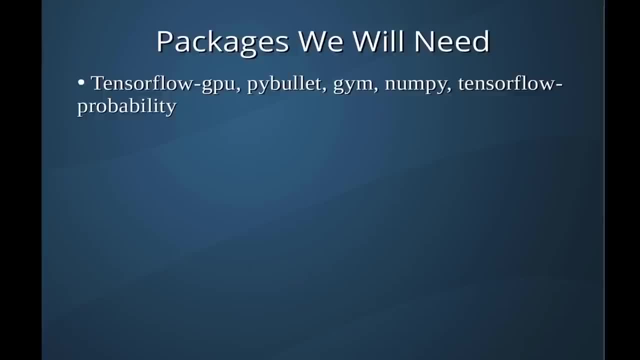 GIM, of course, NumPy and TensorFlow-Probability. That is the only way we can get access to this probability distribution. They're not built into the base TensorFlow package for some reason. Okay, that's it for a mini lecture, your crash course. 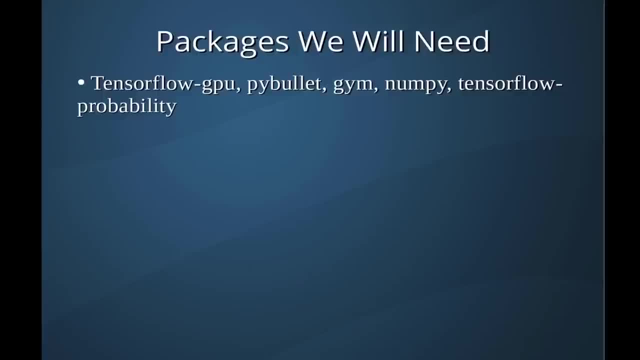 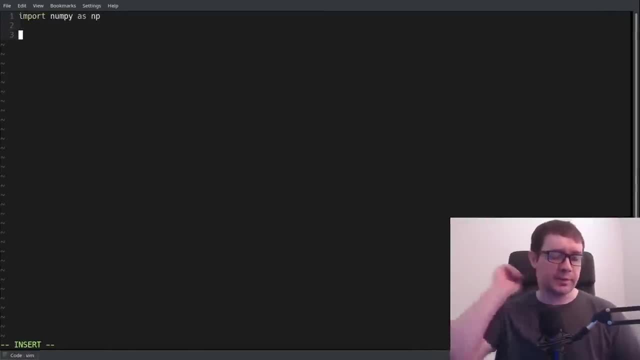 Now let's go ahead and throw you in the water and start coding. All right, so let's go ahead and get started with our buffer class and then we'll move on to do our networks and our agent class. So we're going to be using NumPy arrays for our memories. 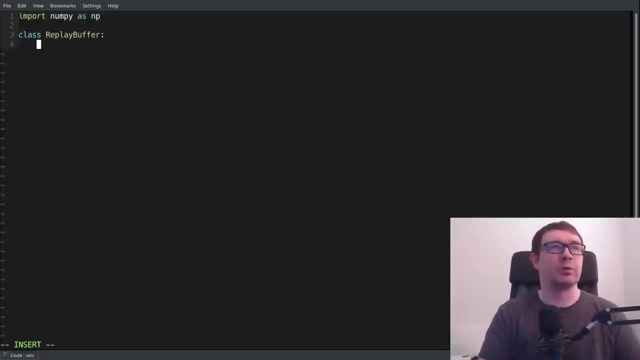 And so NumPy will be our only package dependence for this particular part of the agent. We'll need a max size, input shape and number of actions as input. We will need to save our max size, and we will also need a memcounter to keep track of the first available memory position. 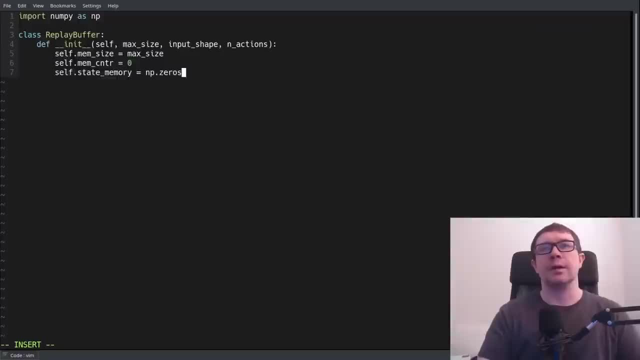 And our agent's memory is represented by NumPy arrays that we will initialize as zeros and the shape memsize by input shape, where input shape is some tuple or list. We need the new state memory as well, That are, the new states that the agent sees as a consequence of the actions it takes in the environment. 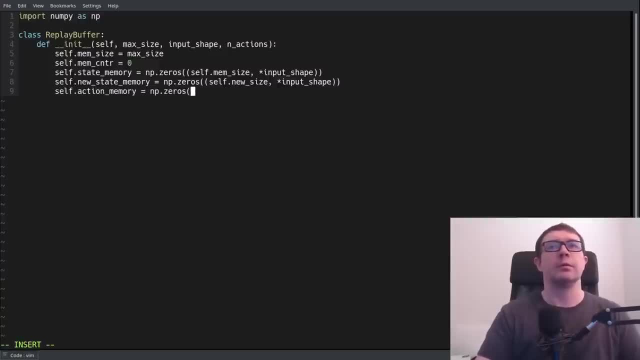 We need the action memory That is in shape, memsize by number of actions. Keep in mind: number of actions means number of components to the actions. Since these are continuous actions, they will have components along some dimension in action space. It's not an actual number of discrete actions. 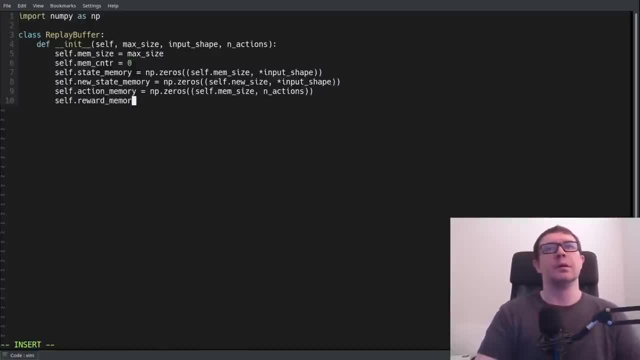 It's a little bit mishapely named, The reward memory, and that's just a vector and an array to keep track of the terminal flags we receive from the environment. and I'll go ahead and say that is num, uh type, numpy bool. next we need a function to store, trans, store a transition and, if it isn't clear, the 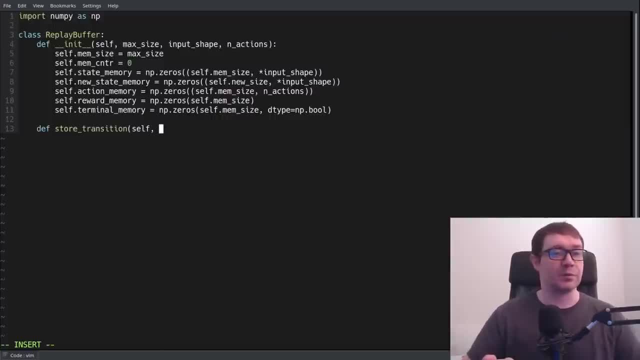 reason we need to store the terminal flags is because the value of the terminal state is always zero, because no future rewards follow the terminal state and so it has no value. so we will need to save all those parameters in our agent's memory, and we want to know what. 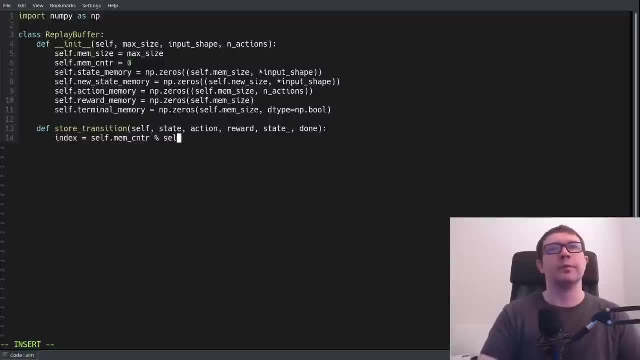 is the position of the first available memory and that's given by the modulus of mem counter and mem size. this has the property that when we overwrite the agent's memory we will go back to the very beginning, so we don't have to worry about going beyond the bounds of our array. 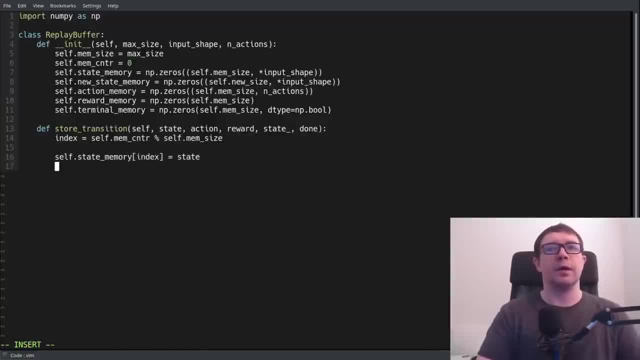 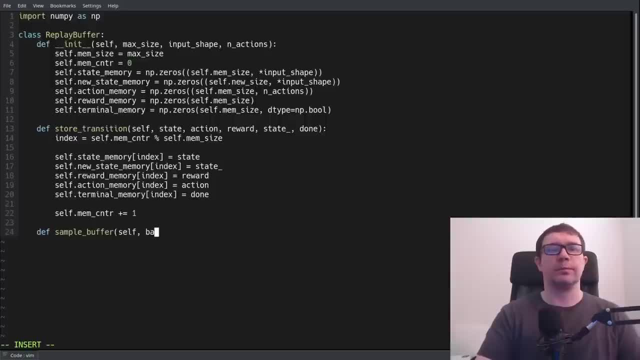 next, we need a function to sample our buffer, and I'm going to make a quick. I want to make a quick aside here. So in a question in the comment section someone asked: is there a way to sample memories according to how viable they were? 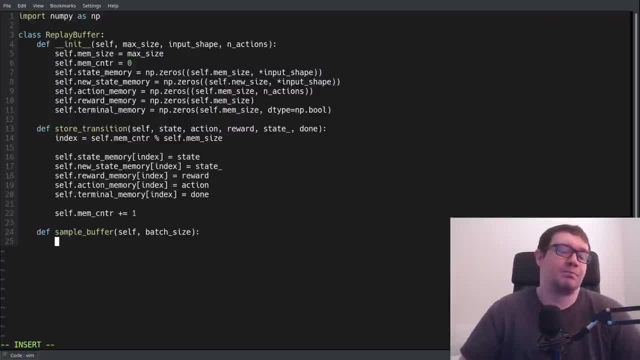 You know our early memories. the agent's acting randomly, doesn't know what it's doing, So what you know, what good is it to sample those memories? Isn't it more important to sample memories where we kind of knew what we were doing? 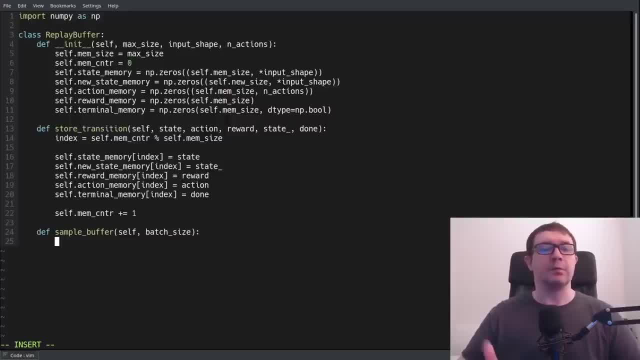 and had some reasonable model of the environment. And you can do that in something like prioritized experience replay, where you prioritize memories based on their utility. But in this case we're just doing uniformed sampling, So we just take the good with the bad. 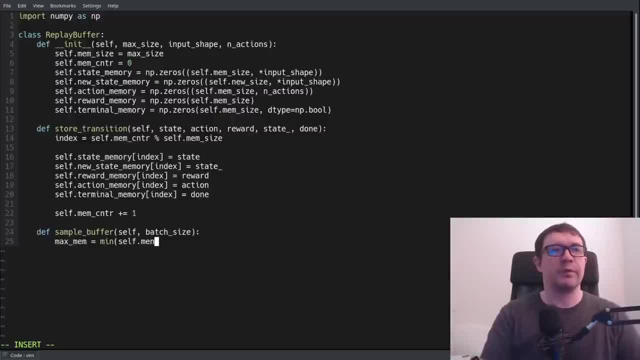 So we want to know, the first available memory, how far we have gone in our memory, And that's given by the minimum of the mem size and the mem counter. That's so that we're not, you know, if we've filled up half of our memory. 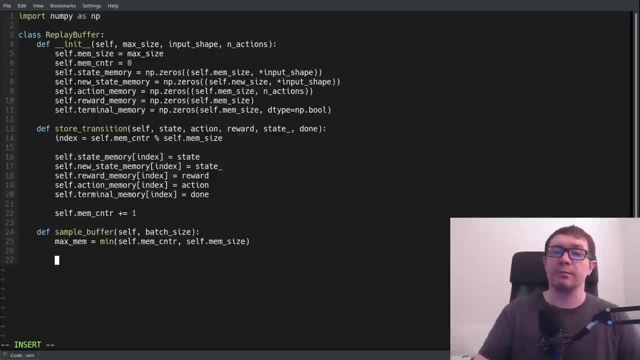 we don't want to sample the latter half, which is all zeros. We only want to sample the first half, which is filled up with, you know, useful transitions, And so then we're going to go ahead and take a batch size of memories. 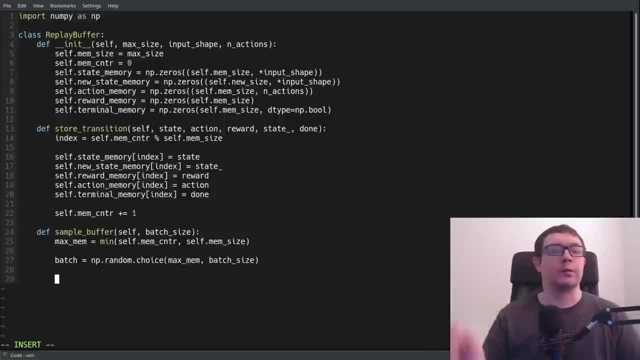 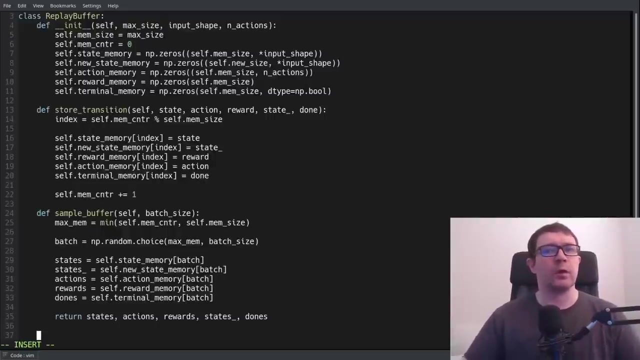 from our memory bank and go ahead and dereference them- Sorry, we need an extra space there- And then go ahead and return those states, actions, rewards, new states and terminal flags. And that is it for our memory buffer class. 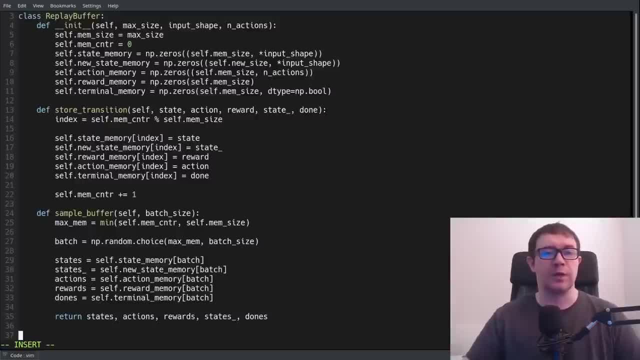 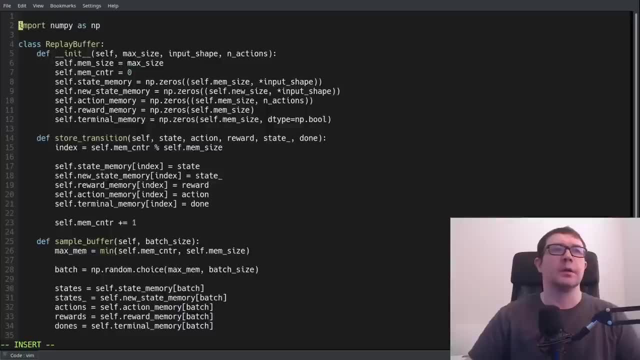 Next up, we're going to handle our networks for the agent. So the first thing obviously we want to do is come up and fix our imports because we're going to need- we're going to need more stuff than just NumPy. 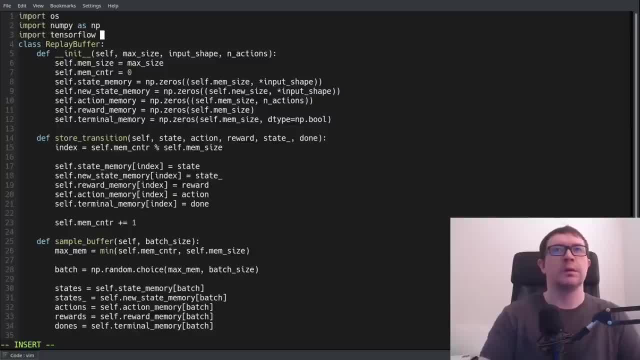 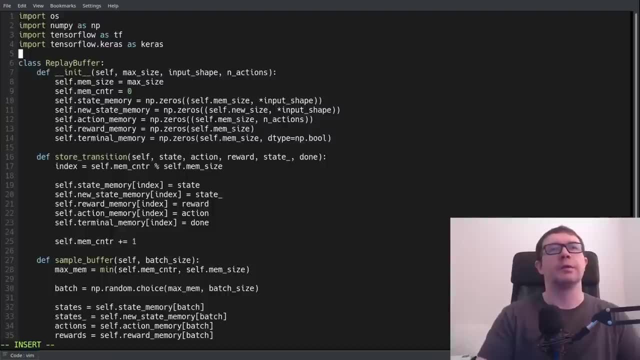 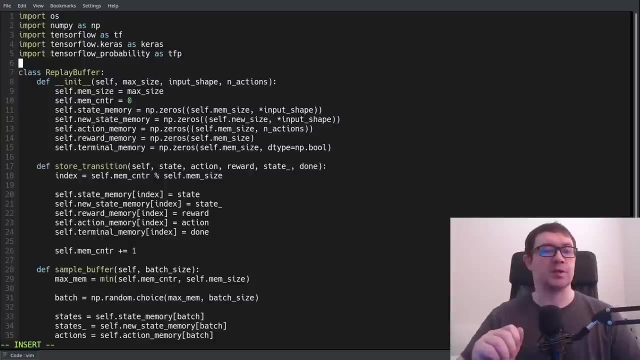 We're going to need OS, the base TensorFlow package, Keras, and we will need TensorFlow probability as TFP. Now you will have to install this package separately. It is not included in the base TensorFlow package, So see the TensorFlow documentation. 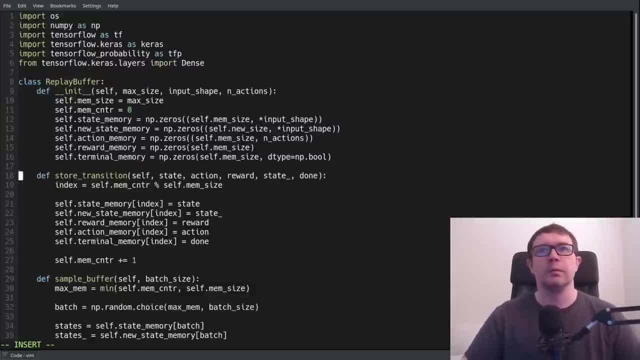 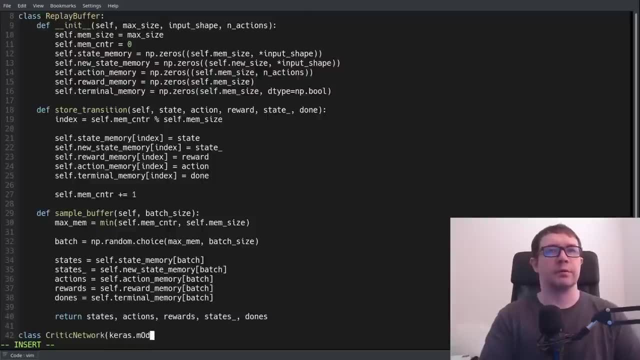 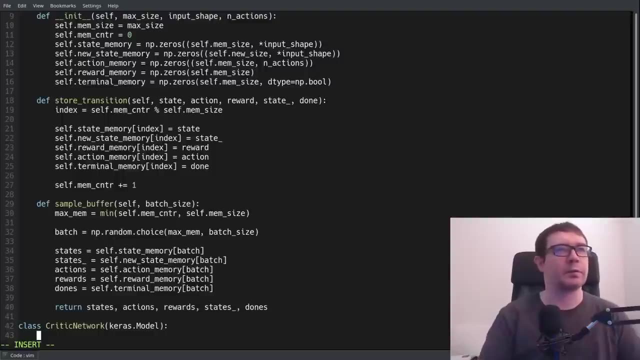 if that is something you don't know how to do, but you do need to do that installation separately. So our critic network will derive from Kerasmodel. I guess it's access to making use of the gradients and the gradient tape and all the other good stuff that we get from the base class. 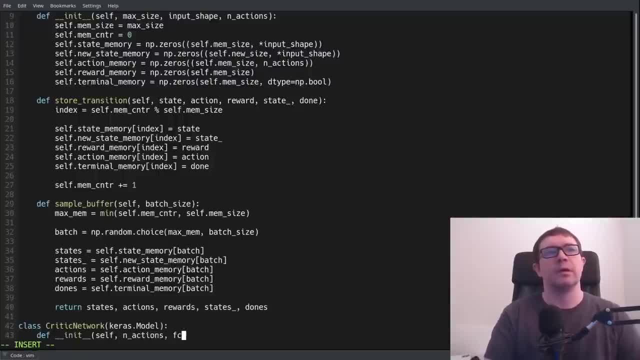 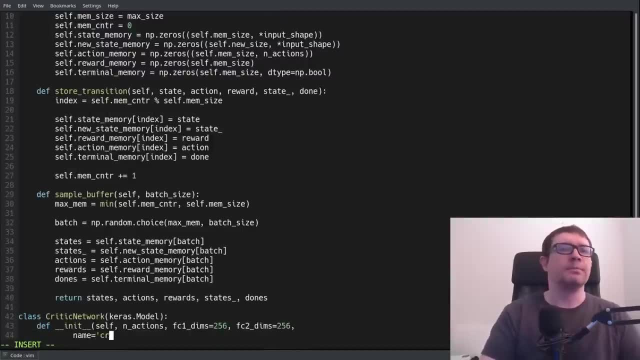 We will need a number of actions, a number of dims, FC1, FC2. dims A name, So the name is useful for model checkpointing, so we can keep track of which file corresponds to which network, And a directory for saving models. 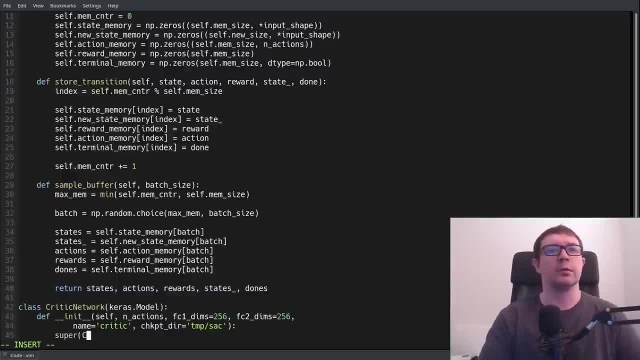 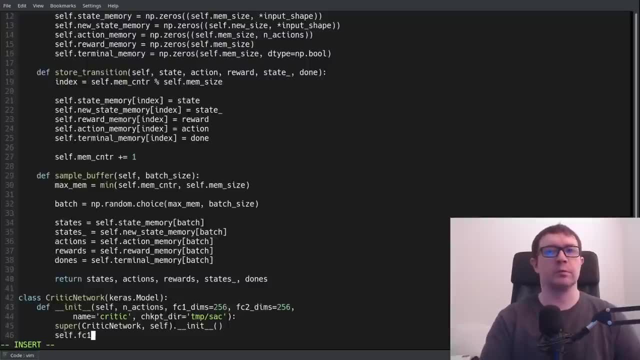 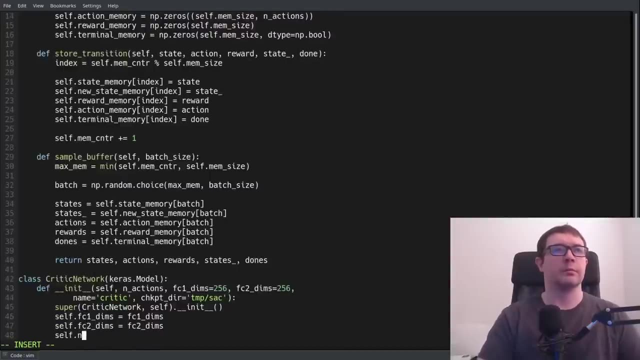 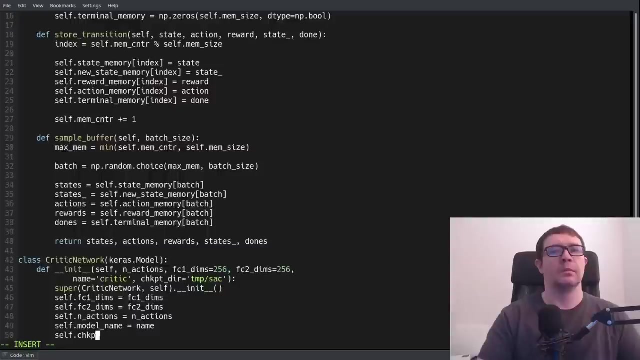 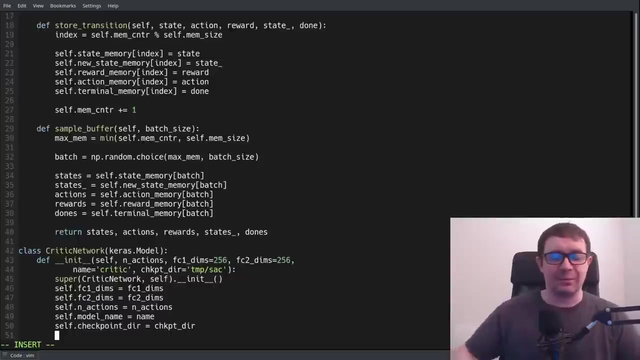 You have to do a make dir on that, otherwise you'll get an error. First thing you want to do is call your super constructor: Save the relevant Parameters. One of these days I'm going to shorten this checkpoint dir name, but not today. 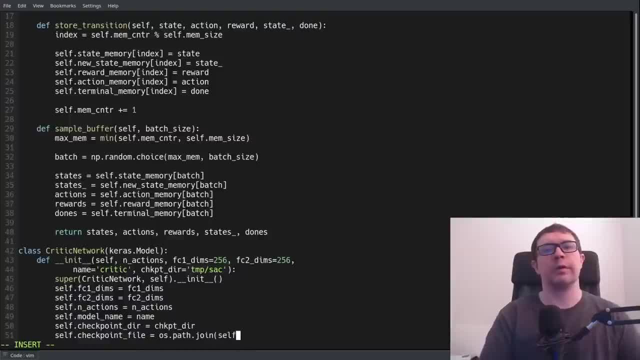 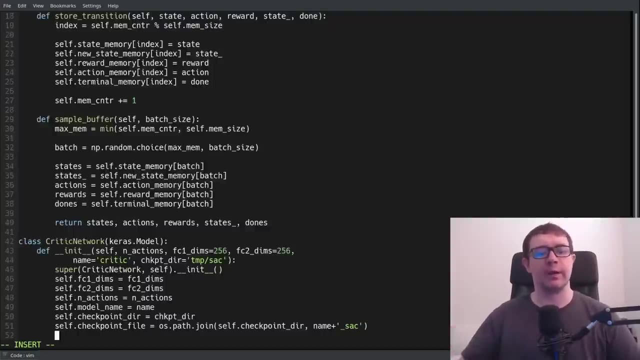 So then you want to join the checkpoint file name: Checkpoint directory- excuse me With the name and underscore soft actor critic. So that way when we save a bunch of stuff in a single directory, we know which file corresponds to which algorithm. 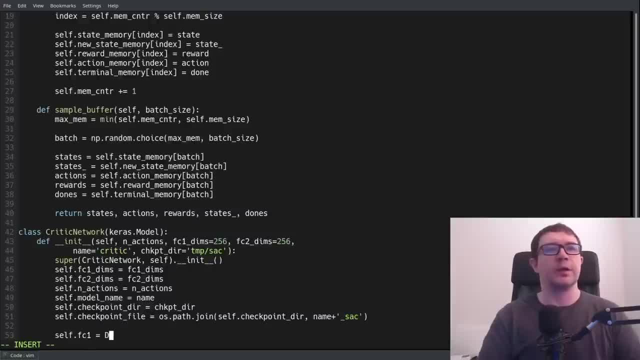 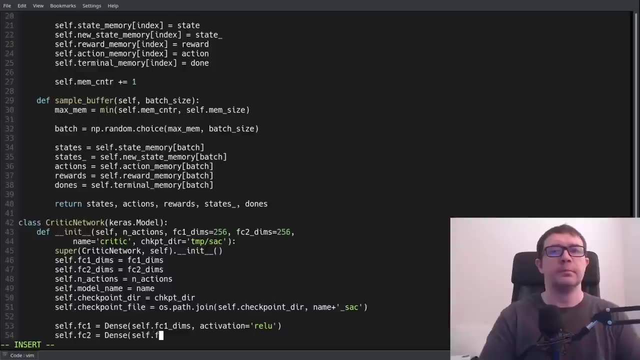 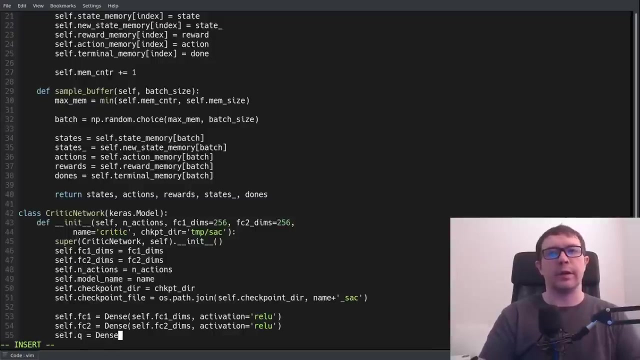 Next we can define our model. Our first fully connected layer is just a dense layer that has implied input dimensionality and takes FC1 dims as output with a radio activation. Likewise for our second layer And our final output is single valued with- excuse me, 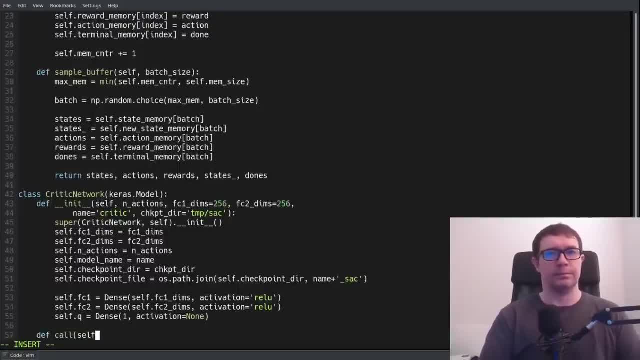 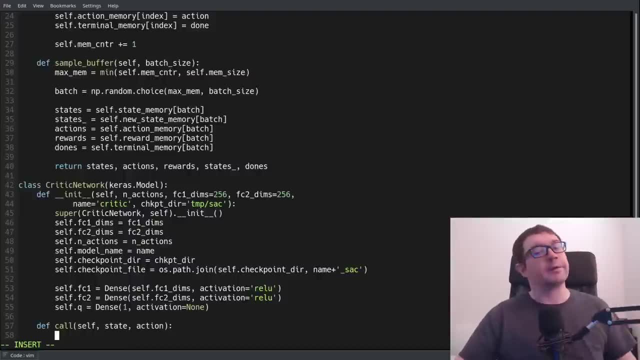 single node with no activation. So we have to input a state and action to our call function, because the critic network evaluates the values of state action pairs, And so the first thing we want to do is pass the concatenated state and action pair through the call function. 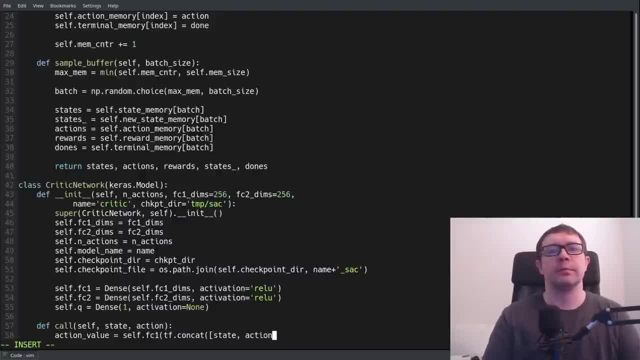 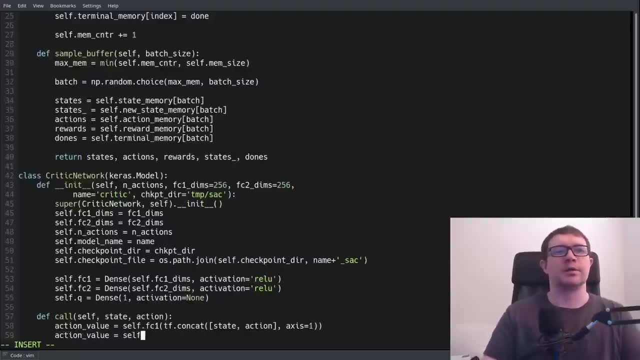 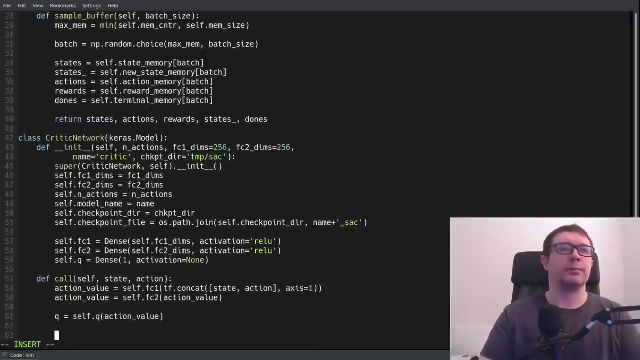 So we're going to pass the first fully connected layer And we want to concatenate along the first axis And pass that through the second fully connected layer And pass that through the output layer And return Pretty straightforward there. Next let's handle our value network. 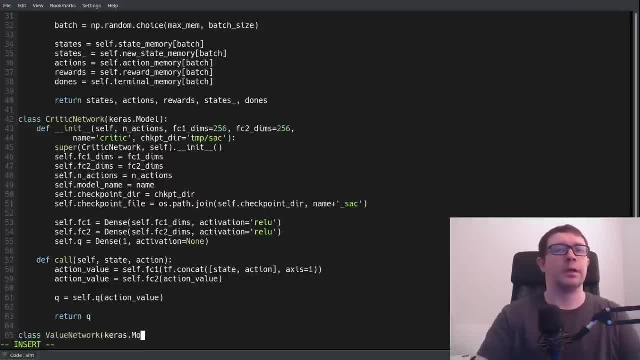 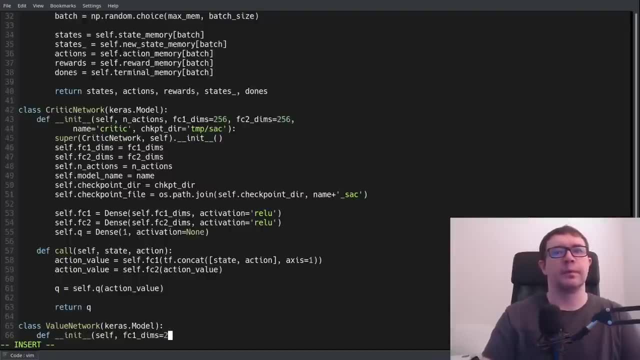 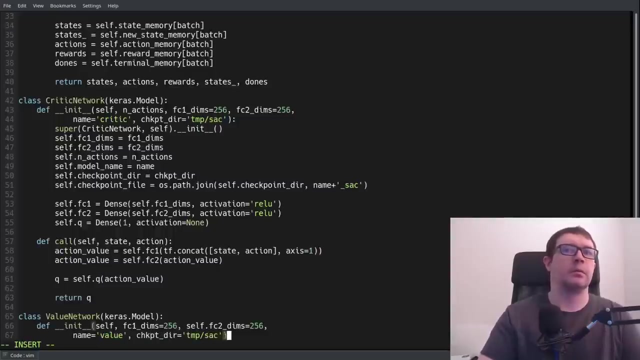 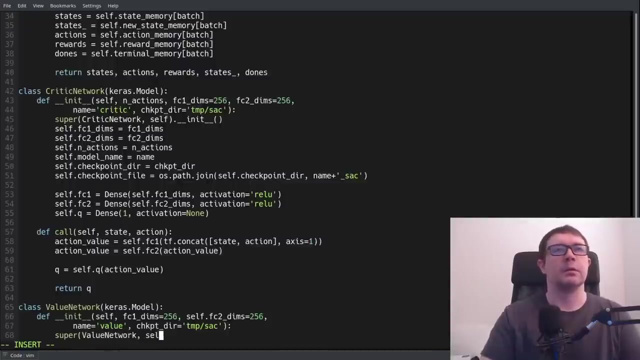 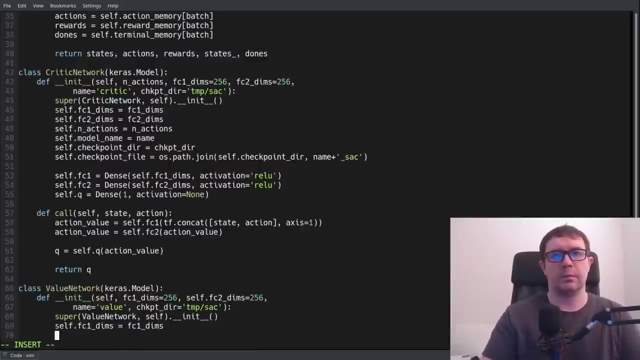 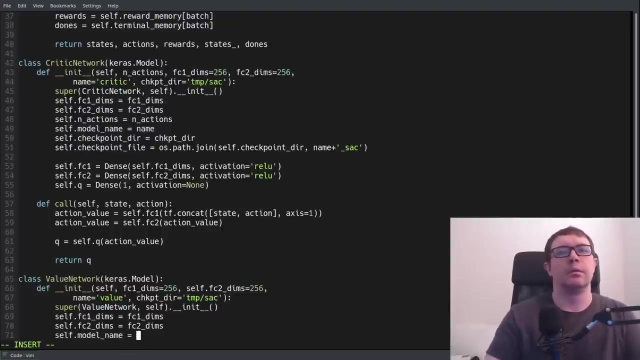 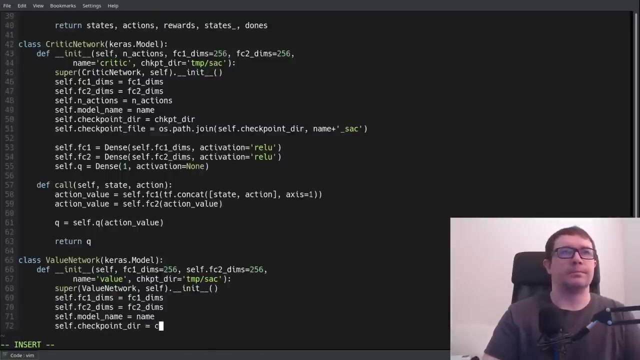 And again, that derives from kerasmodel, Let's Suppλmodel, And that derives from kerasmodel mutant declare sub express果. So we disappoint theع And we want to call our super constructor again. and if you wanted to get really fancy, you could write a base model, a base network class. 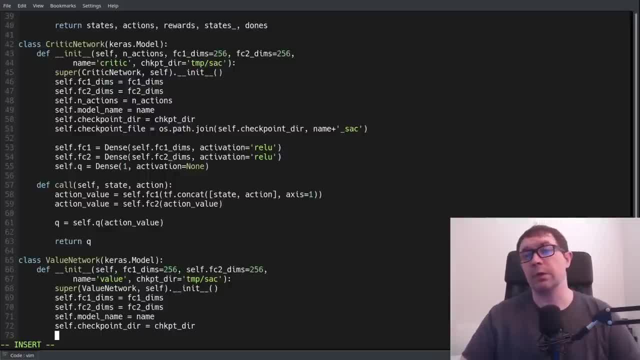 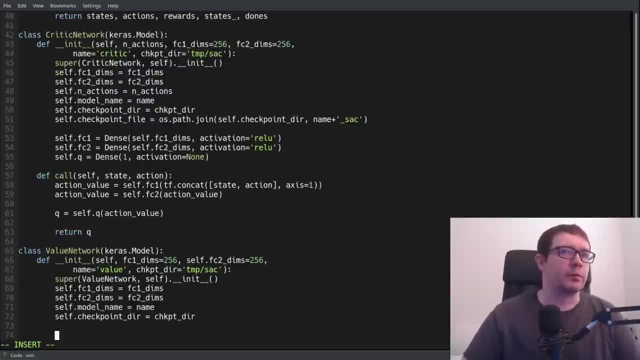 and then have everything derived from both the- I guess the base model class would derive from the Keras model and then everything that derives from that would derive from the base class, base model, sorry, base network class, but that can get kind of messy really quickly. 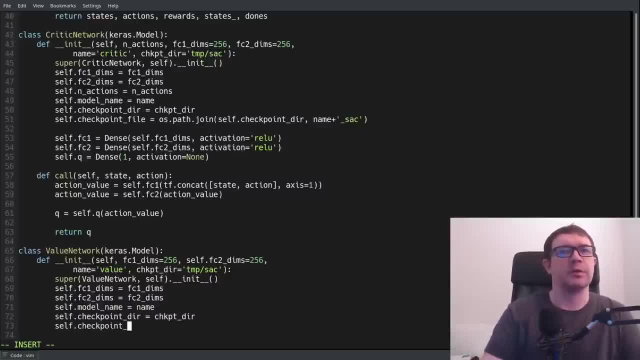 You have to deal with multiple inheritance. Maybe it's not as hard as I initially think it is, but it's an alternative path. It's an alternative way so that you don't have to keep writing like the same stuff over and over again. 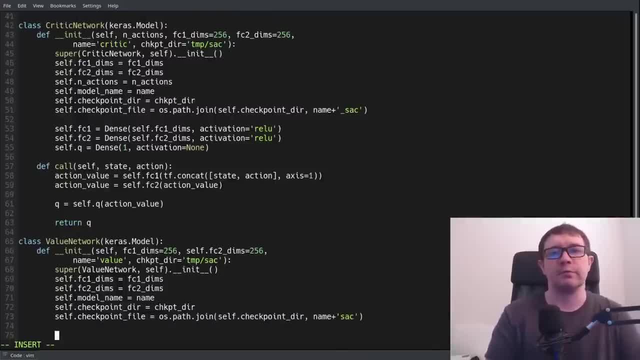 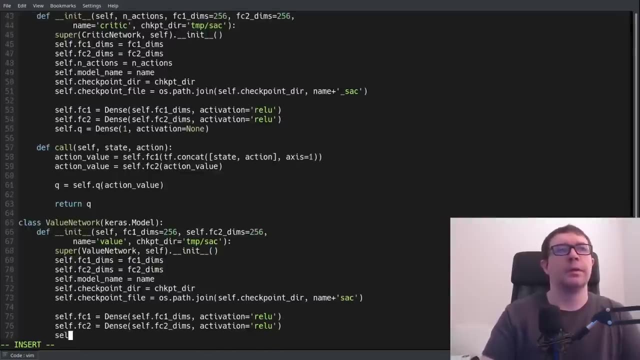 Okay, Because you notice there's a little bit of a gap here. There's a lot of overlap between the code of the network, so you can fix that with inheritance And our output is again going to be single valued with no activation. Now the call function here only takes the current state of the network. 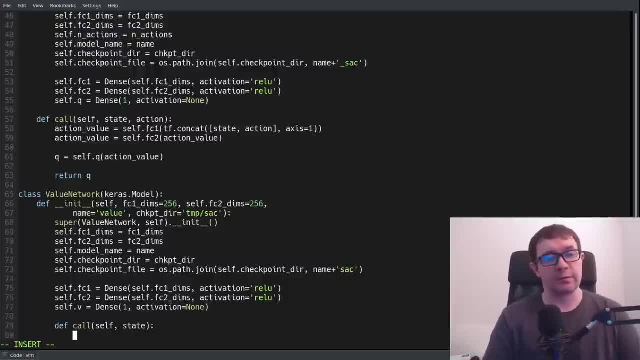 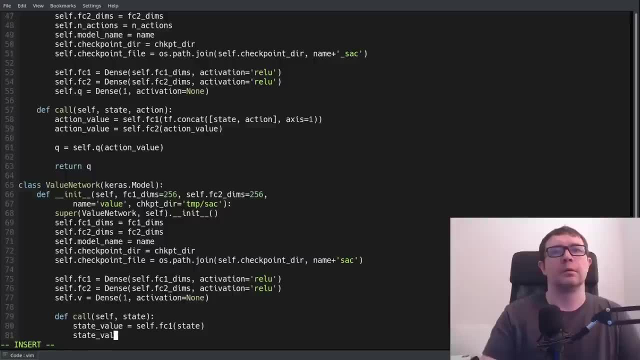 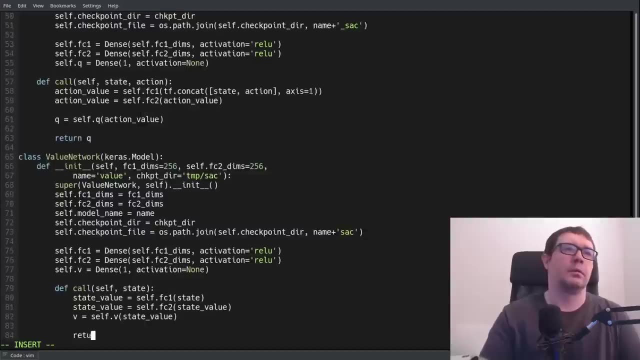 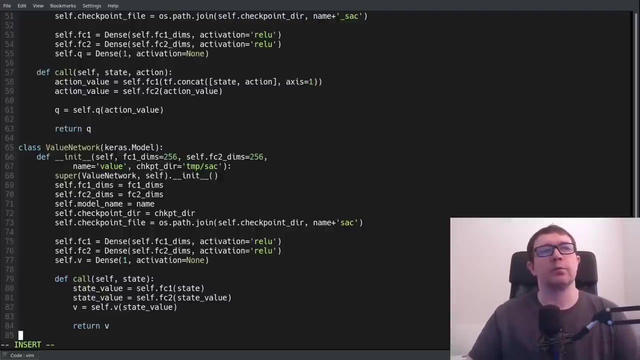 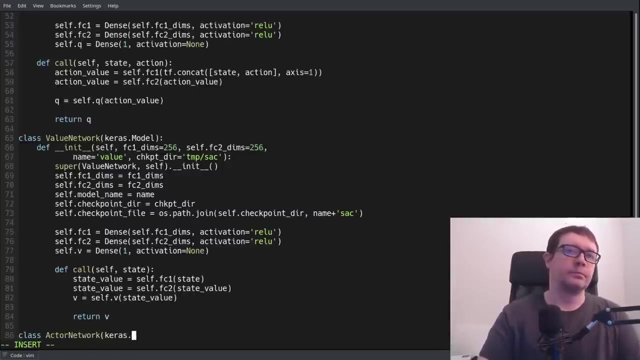 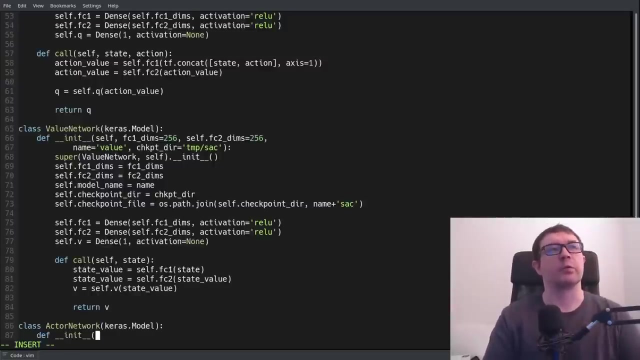 The value function is only concerned with the values of states, not state-action pairs. Then we just go ahead and pass all of those through and retrend them. Pretty straightforward. The real difficulty doesn't occur until the actor network and the difficulty will come in the call function as well as the sample normal. 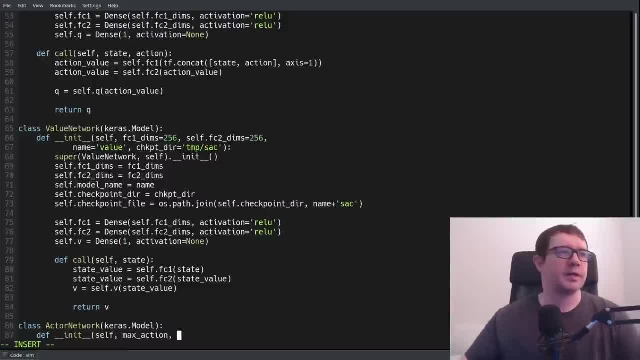 So we want to pass in a max action. Am I using that here, Sorry? I always kind of make stuff on the fly, kind of modify stuff on the fly. Yeah, So we do need that. SC1 dims, SC2 dims. 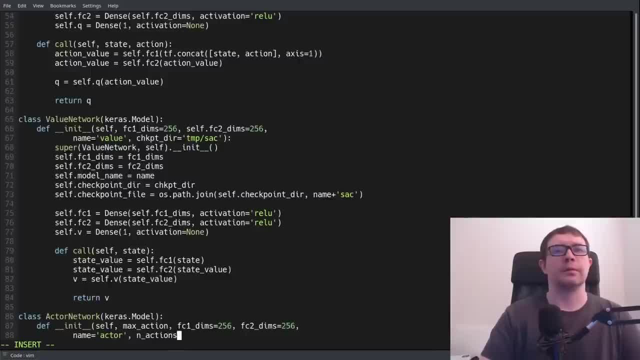 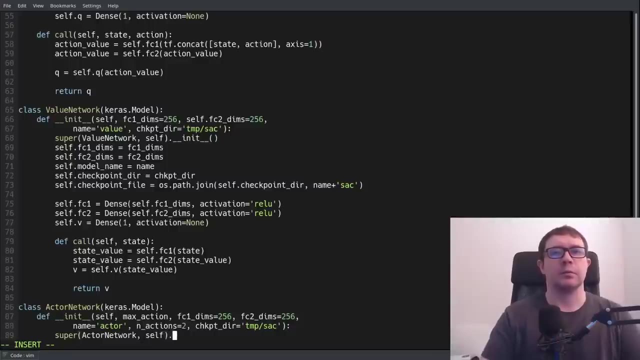 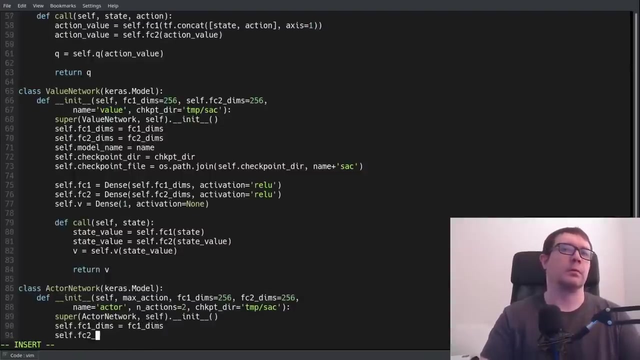 A name Number of actions. I'll use 2 by default. Again this number of components And a checkpoint directory. I'm going to call r superconstructor And save the relevant parameters: SC2.. And SAVE the relevant parameters. 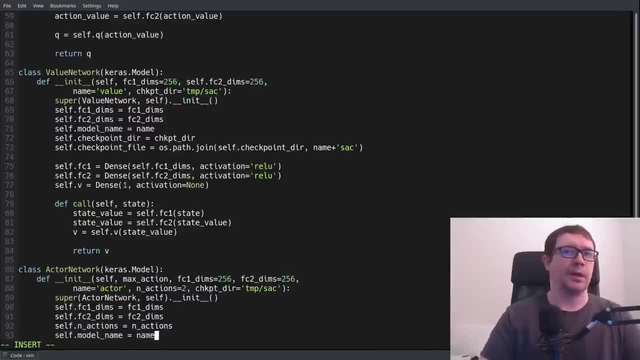 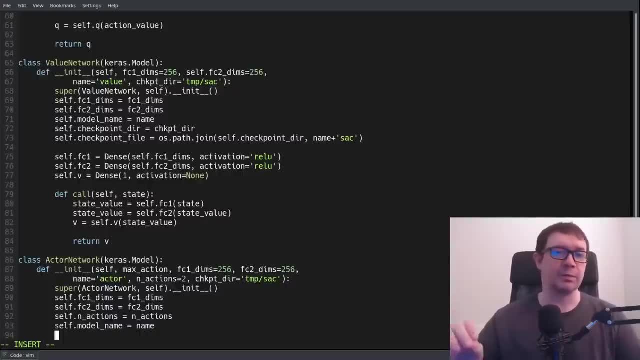 And SAVE the relevant parameters And SAVE the relevant parameters, OK, and then we have our model name. And, just as an aside, you can't use name. It's a reserved variable. You can't say selfname equals name, because name is reserved by the base class, charismodel. 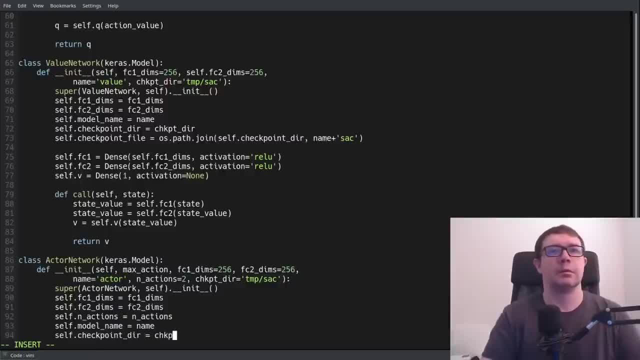 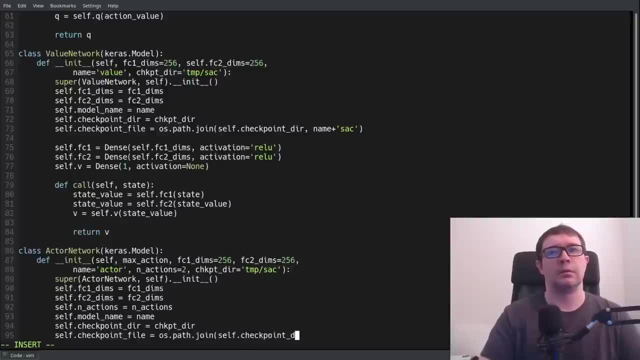 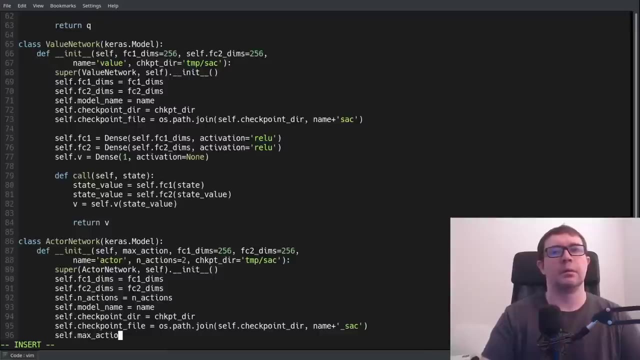 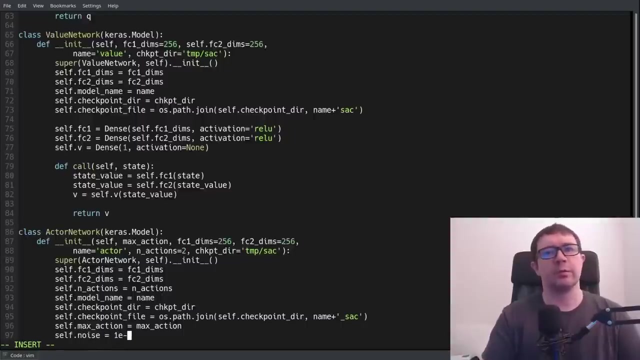 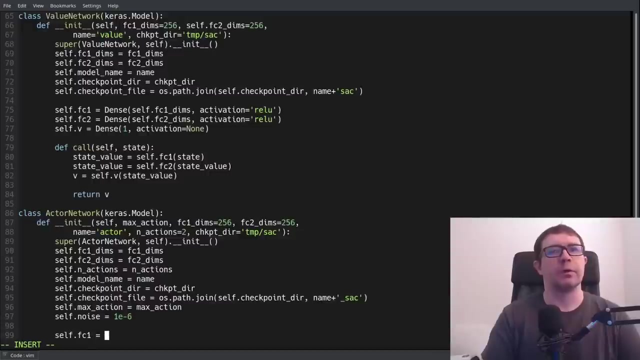 So you have to use model name. So we're not going to be using re-parameterization, but we will need some noise factor to make sure we don't get something that blows up when we take the log. You'll see what I mean very shortly. 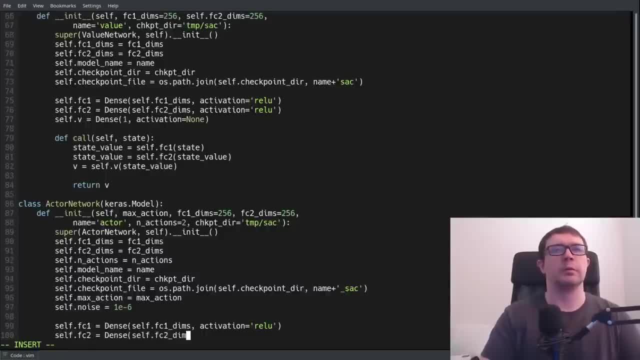 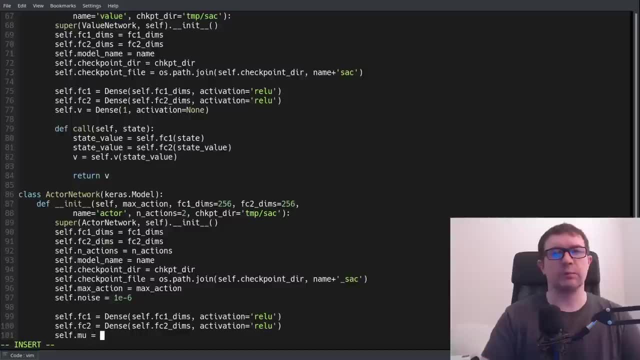 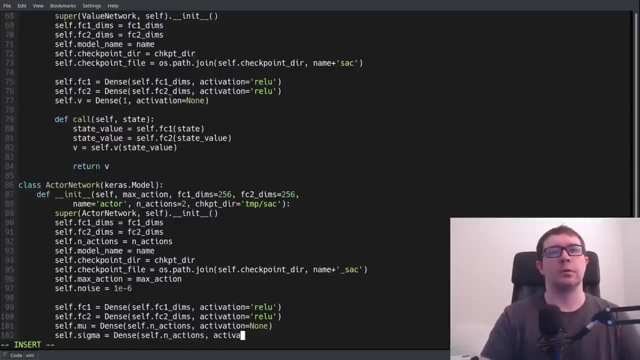 Our neural network by now should look pretty familiar. Value activations: Here's where things get interesting. Here's where things get interesting. We're going to have a mu for our distribution as well as a sigma with no activation, So let's go ahead and handle our call function. 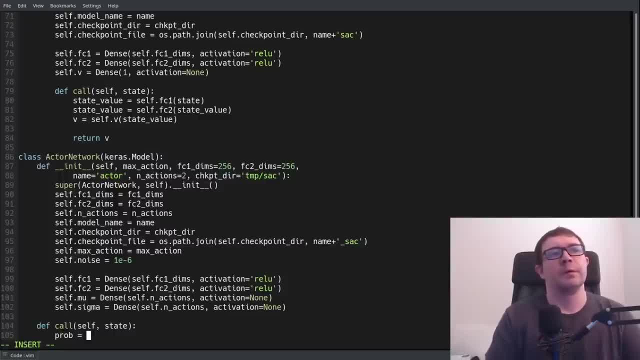 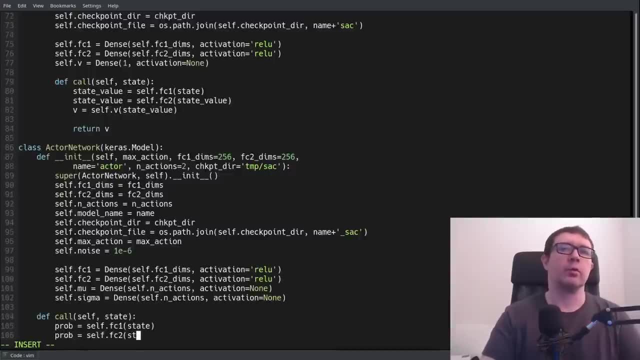 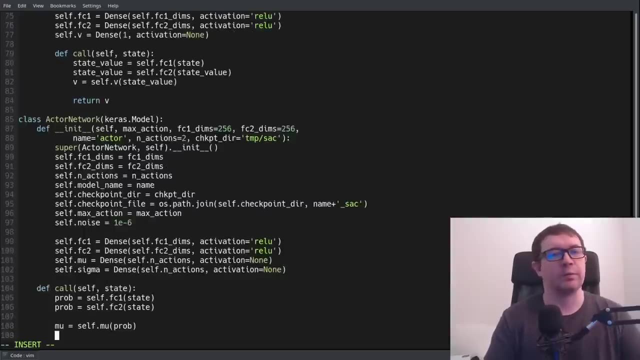 So we're going to get our- I called it prob here, but I don't know if I like that name now that I'm rewriting it, But I'm going to roll with it. So, mu, really, that prob is just the input of our first two layers. 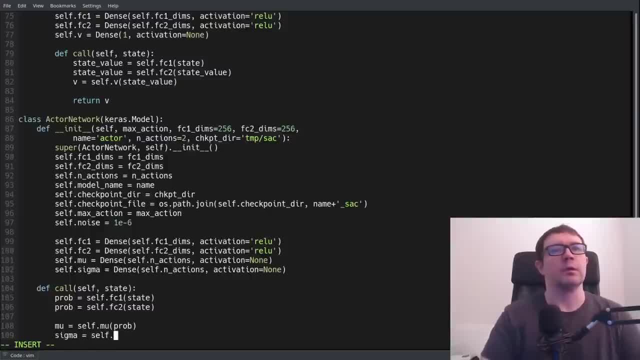 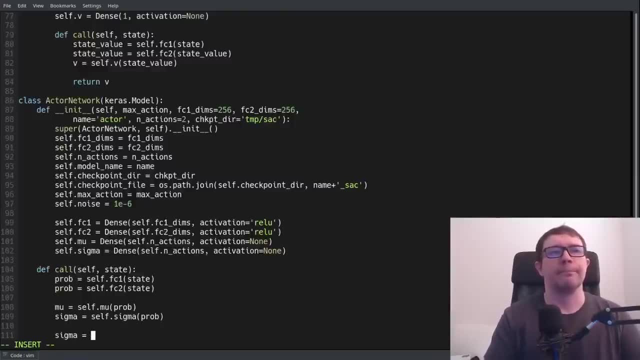 the pass-through of the state through the first couple layers, We'll have our sigma, which is a standard deviation of our distribution, And we're going to want to clip this. It may be the case that TensorFlow 2 doesn't need it. 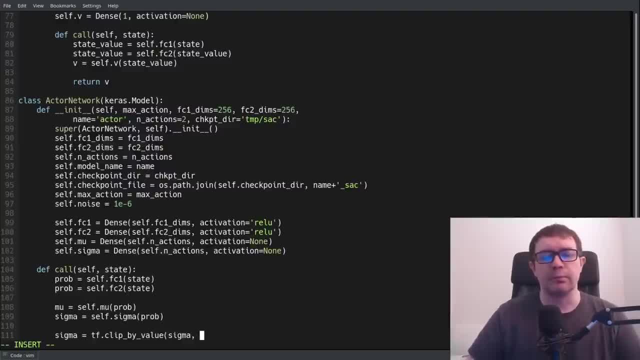 but when I was coding this up in PyTorch it The distribution would blow up if we had a noise of sorry, a sigma of zero. It didn't like a zero standard deviation distribution, which I can understand. I guess that's a direct delta function. 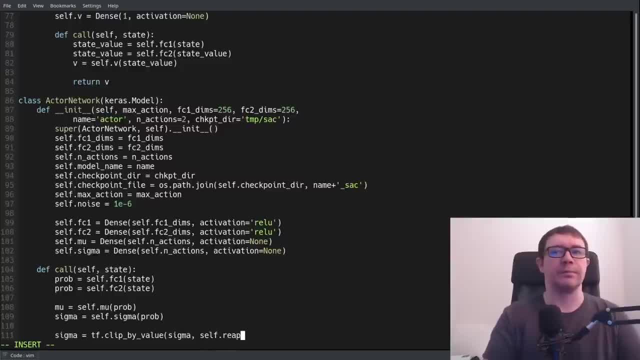 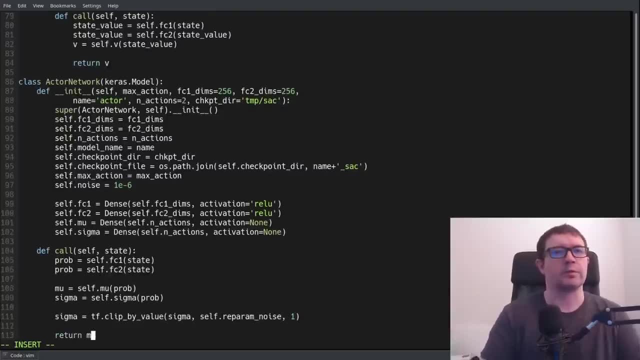 It's not exactly something that you would encounter every day, And I think the TensorFlow might actually fail a little bit more gracefully than the PyTorch in that respect, But I go ahead and clip it. So that goes between one by 10 to the minus six and one. 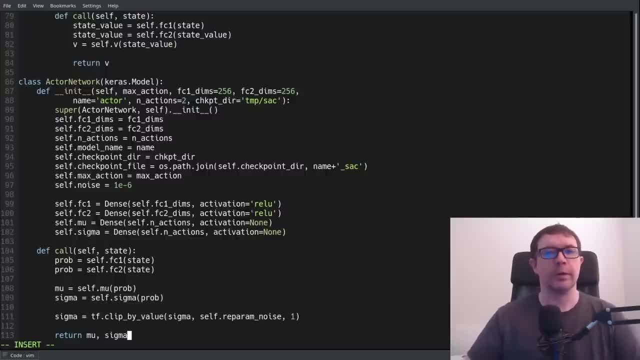 So we're going to constrain the standard deviation here to not be too large. That is something you can optimize on your own. I don't do extensive and detailed studies on all of this stuff. I just get it working, check that it conforms to the specifications laid out in the paper. 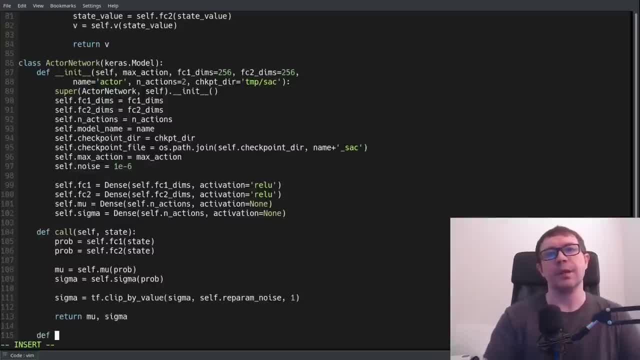 and then I get something reasonable on the output. But we're not done for the active network. We have the output of our deep neural network which is a mean and standard deviation for our distribution. Now we have to sample that distribution to get the actual action for our agent. 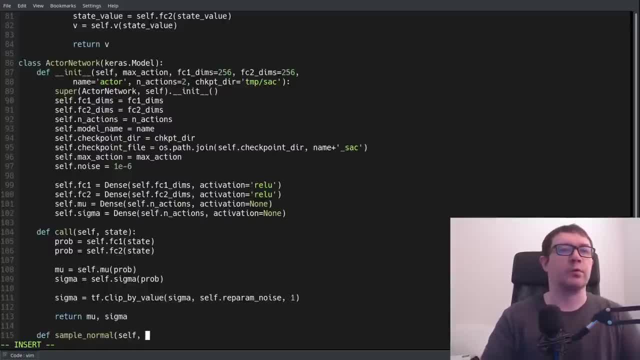 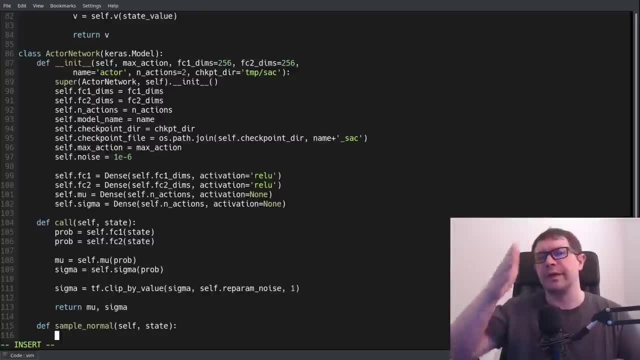 And I've stuck it on a function called sample normal And, as I stated, we're not going to be doing the reparameterization trick. I show students how to do that in the course And in fact, in my PyTorch video I show you how to do it. 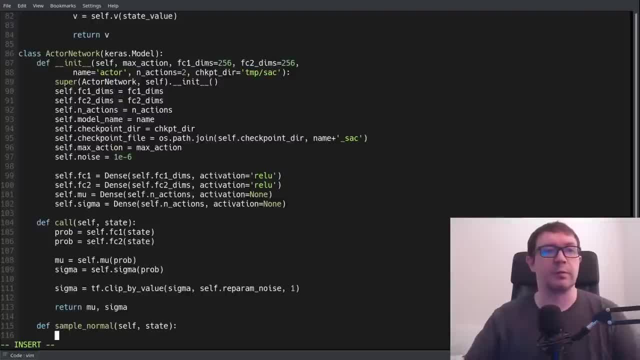 PyTorch has a very simple function called rsample that does basically the reparameterization for you. You can implement the code yourself if you really want to be a completionist about it, but I'm not bothering here because I do get good results without it. 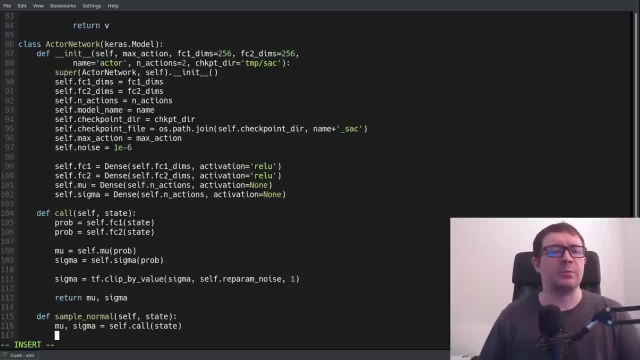 That's kind of like with the DDPG paper, where they use the Ornstein-Ullenbeck noise And then people that implemented that later kind of threw it away because they're like, wait a second, this is unnecessary complication. That kind of seems to be the case here. 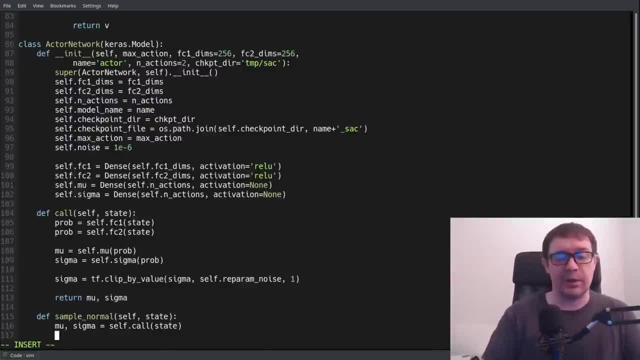 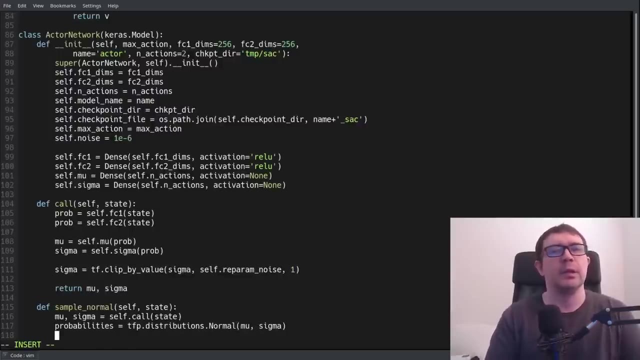 where it works without it and is an unnecessary complication. But I mean, I could always be wrong, but I do get solid results without it. So here we're going to go ahead and instantiate our normal distribution defined by mu sigma, and our action is going to be- our actions are going to be- a sample. 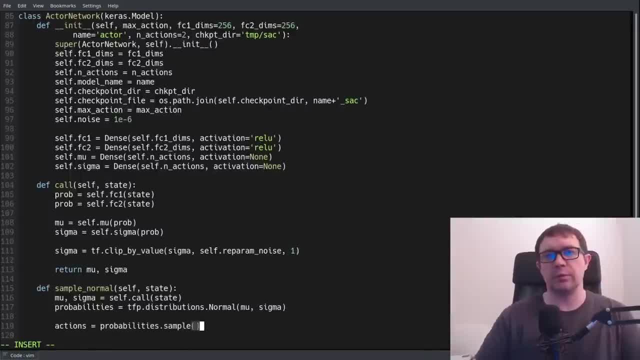 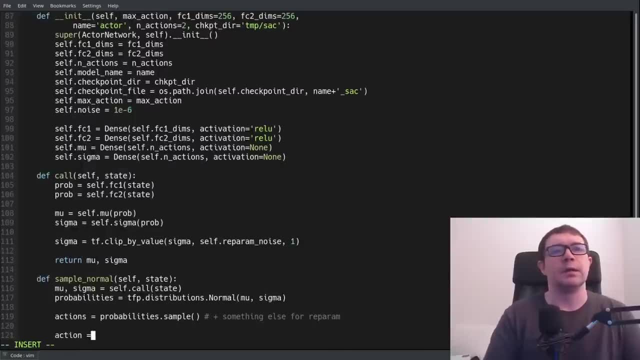 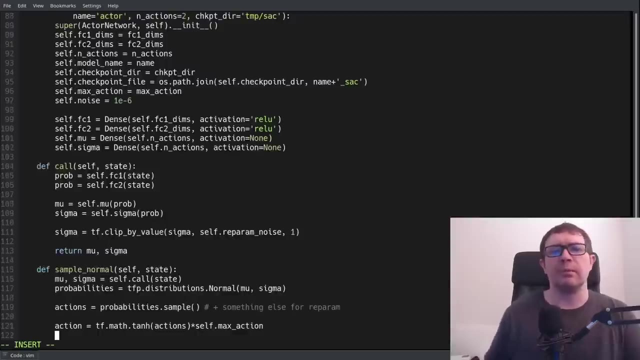 probabilities dot sample. if you want to do the reparameterization, you'd reparameterize it there and the action is math, tan, hyperbolic times, max action. that max action takes care of the fact that our environment may have max actions outside of the bounds plus or minus one, which are, of course, the bounds. 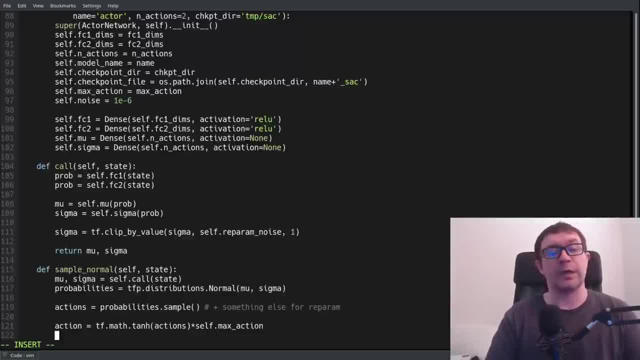 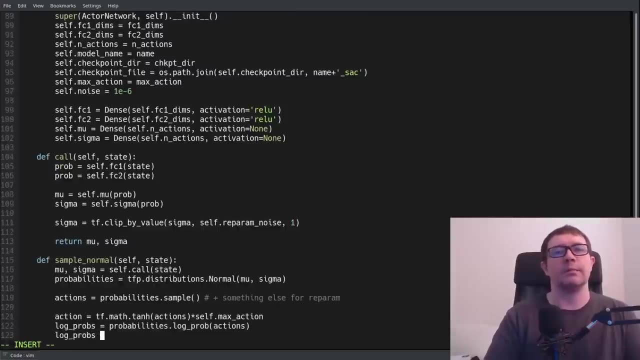 of the tan hyperbolic function. so you want to not arbitrarily cut off half of your action space. if you don't have to a log probes its probabilities, will it stop log prob of actions and then go ahead and subtract off math log 1 minus tf dot math dot power. 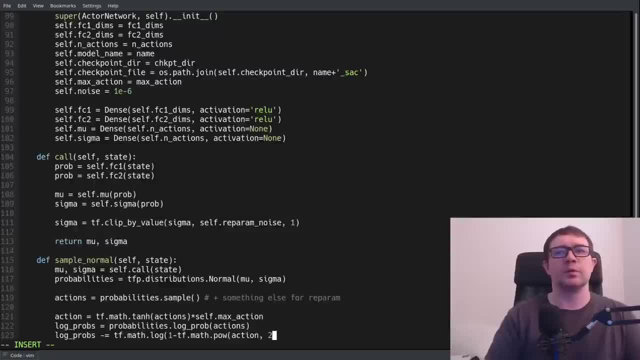 excuse me, action. so we're going to square the action plus self dot reprogram called it noise, didn't I self dot noise? and so then I had to change it here as well, don't I? yeah, self dot noise plus self dot noise. do I have the right number of parentheses here? yes, I do, and 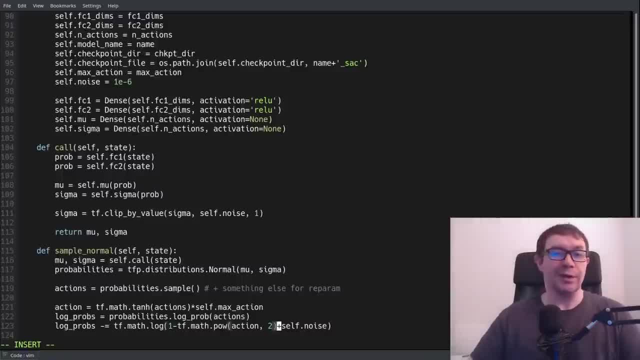 so since you have a logarithmic function here, you don't want to take the log of zero. that is oftentimes not advisable, so I just add in some really small number to make sure we're taking the log of something finite. so then we're gonna go. 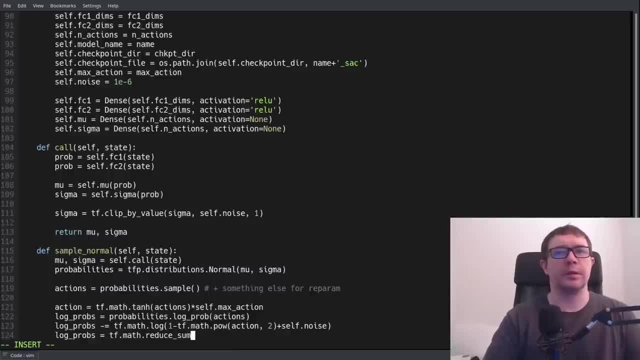 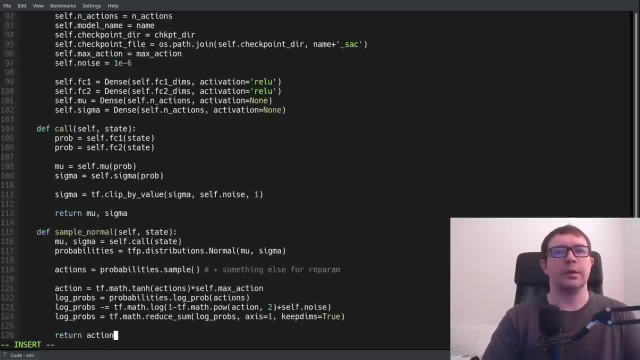 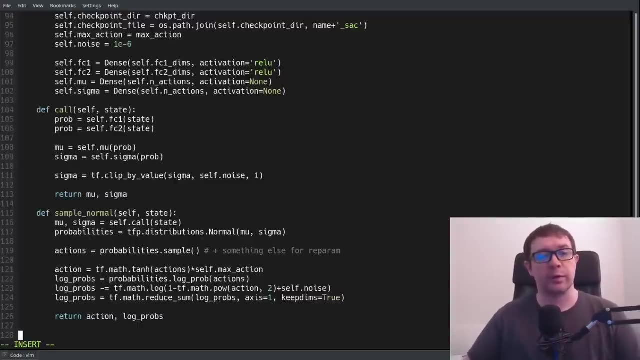 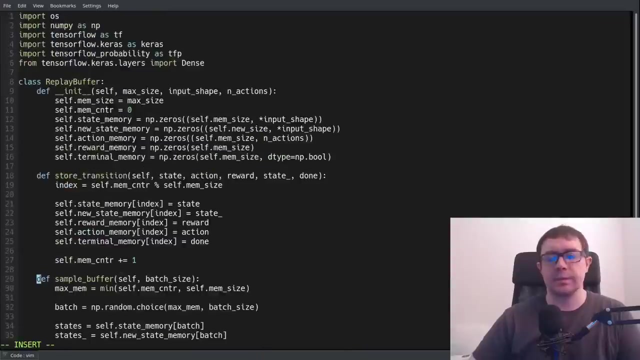 ahead and do a reduce sum on that log one, keep them true and return the action and log props. so that wraps up the networks portion of our code. now we have to handle the agent class, which will tie everything all together. so of course, again we have to come back up to the top. 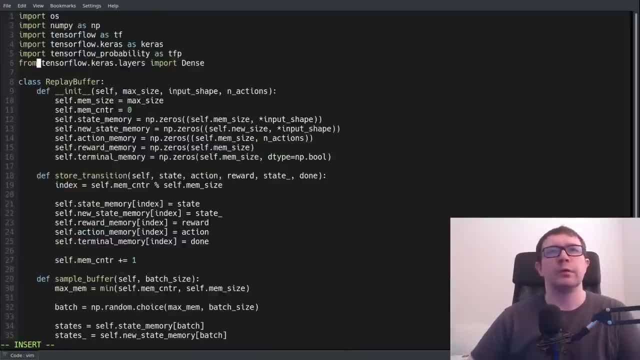 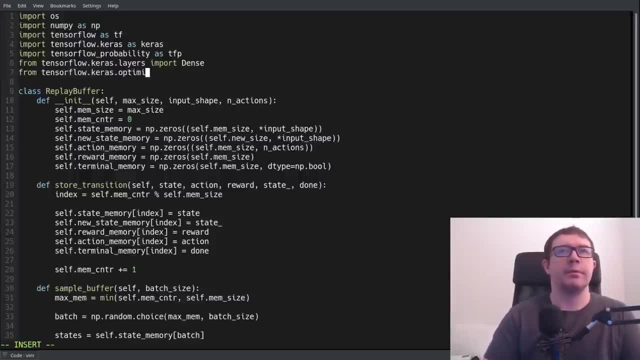 and add in some imports. we're going to need our optimizer. so we'll say, from tensorflow keras optimizers, import Adam, and I think that's the only other import we will need. and then we come back down here, we have our훈 until we know what we're gonna actually need. so then we go ahead and go counter to our veya family first, and then we'll go 10 to 10 after we прирaw dist. 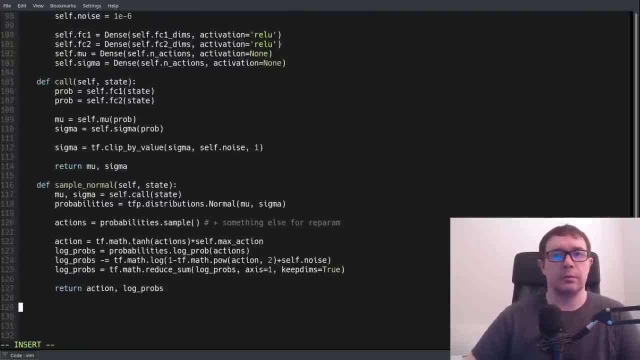 here and start our agent class, which derives from nothing. our initializer is going to take a number of learning rates. now we're going to use two separate learning rates. you could, in principle, use three: one for the critic, one for the actor, one for the value network. in this case, we're going to use one single. 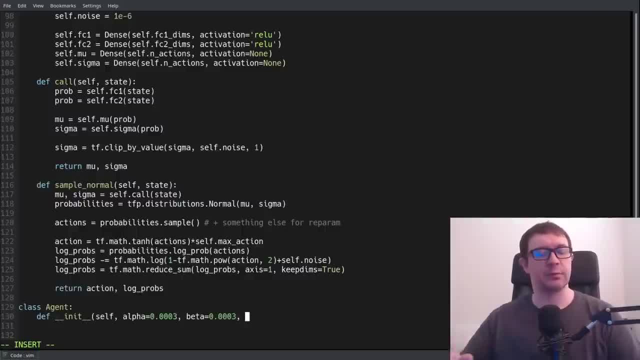 learning rate for the actor and then the same. the beta learning rate will be for the value and critic networks input dims something like eight. that's just the default for the lunar lander. it's the only default I know at the top of my head. we're going to want to pass in the environment to get some useful. 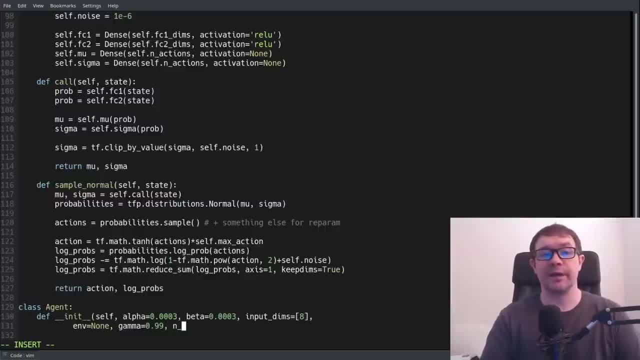 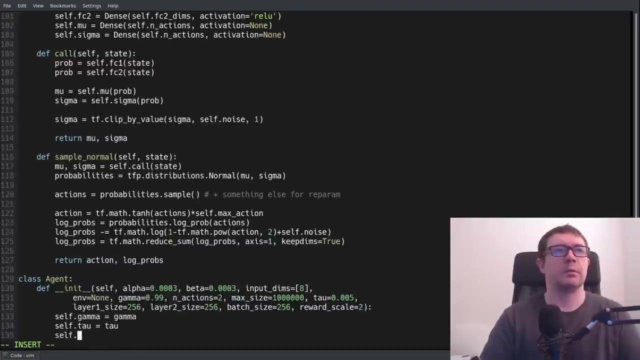 information from it. a gamma, the discount factor for our update equation. max size for our memory. a million transitions. default value of tau: 0, 0.005. layer 1 size. layer 2: size 256. batch size default 256 and a reward scale default of 2. let's go ahead and start saving a replay buffer. max size. 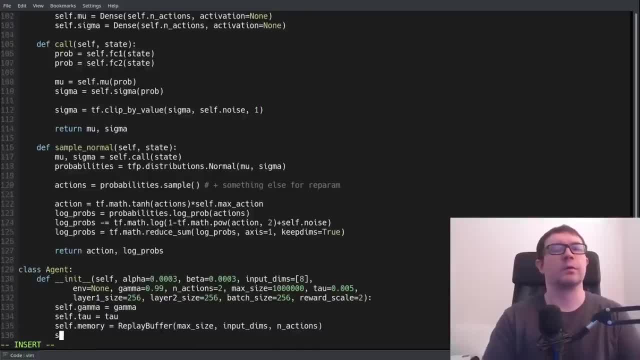 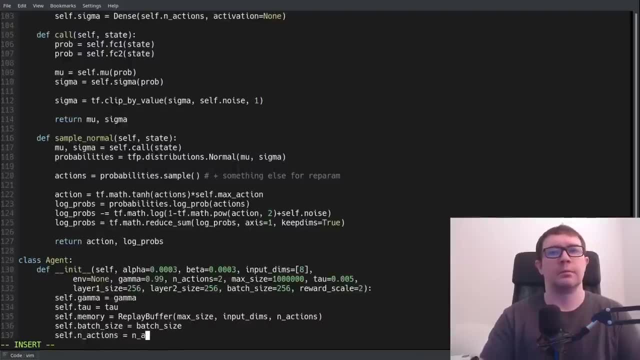 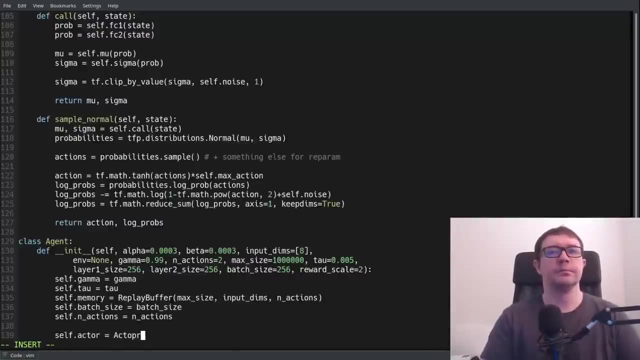 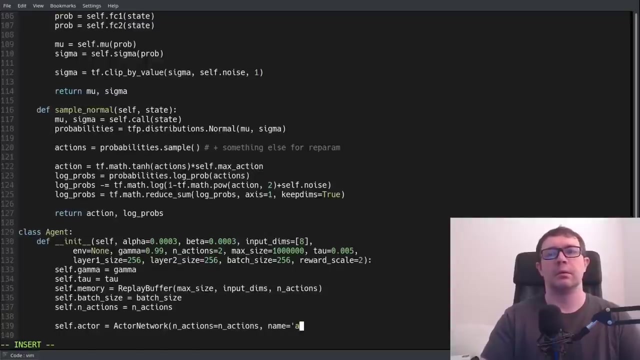 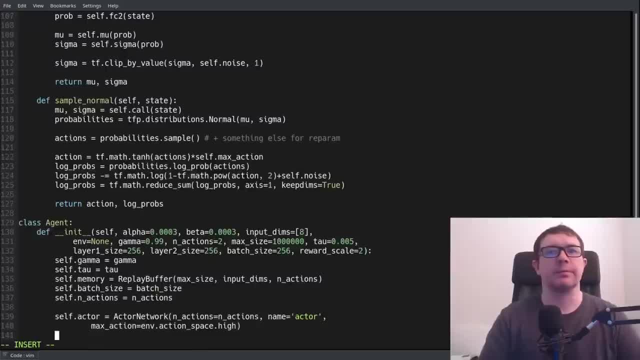 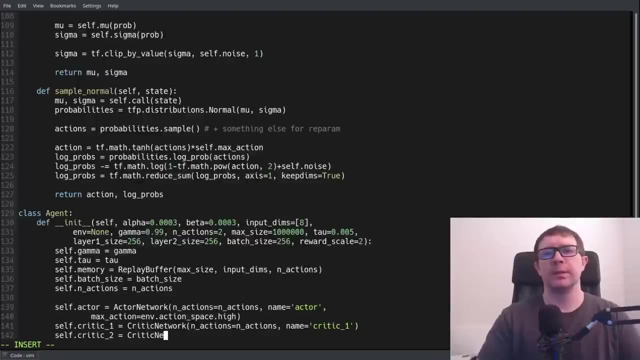 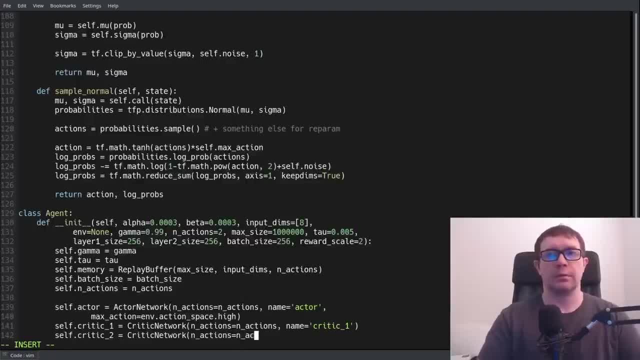 second critic and these are, you know, identical in terms of their definitions. identical in terms of their definitions, identical in terms of their definitions, except for the name. because, again, when- except for the name, because, again, when, except for the name, because, again, when we save files, we want to save separate. 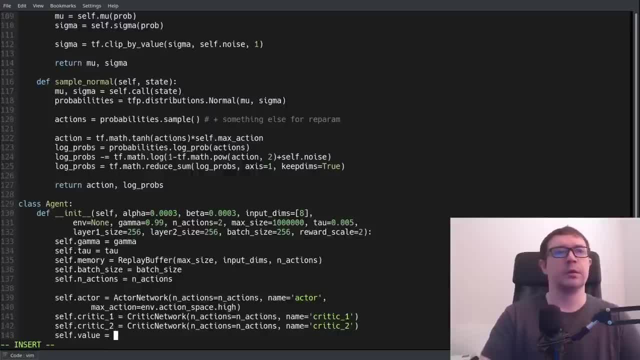 we save files. we want to save separate. we save files. we want to save separate files for both critics, otherwise we're files for both critics, otherwise we're files for both critics, otherwise we're going to get a mess value network and going to get a mess value network and 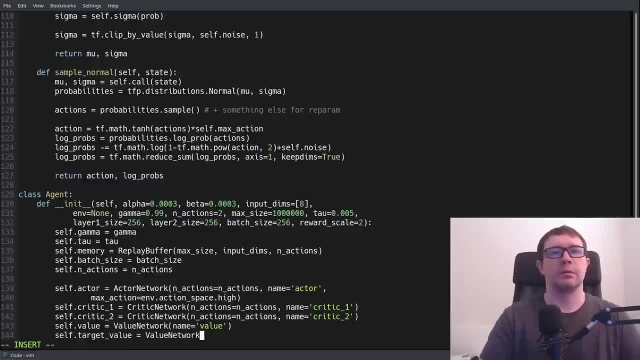 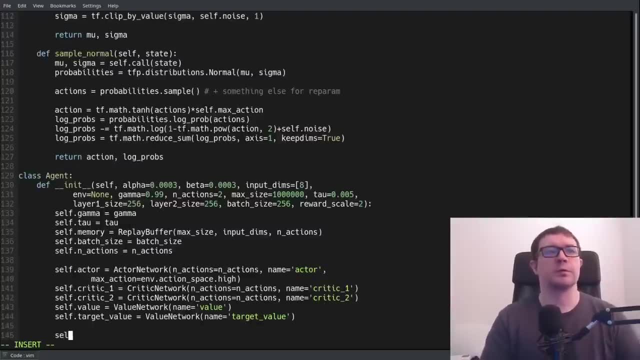 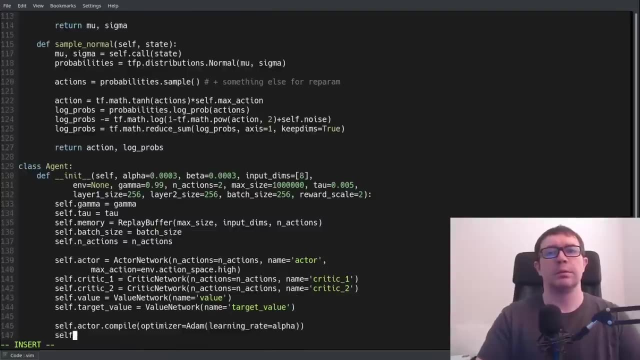 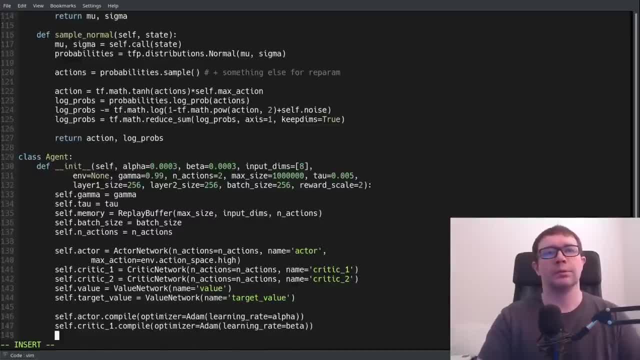 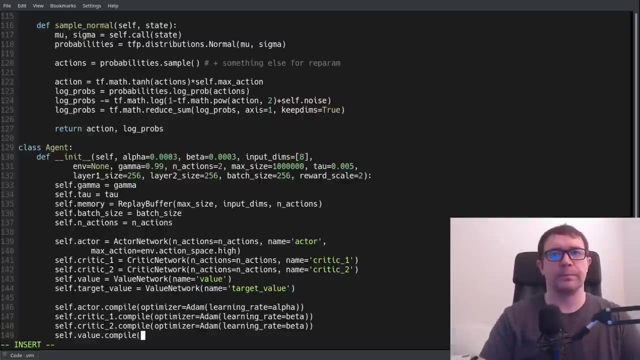 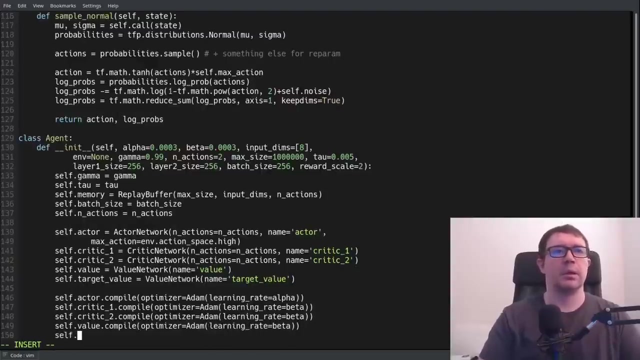 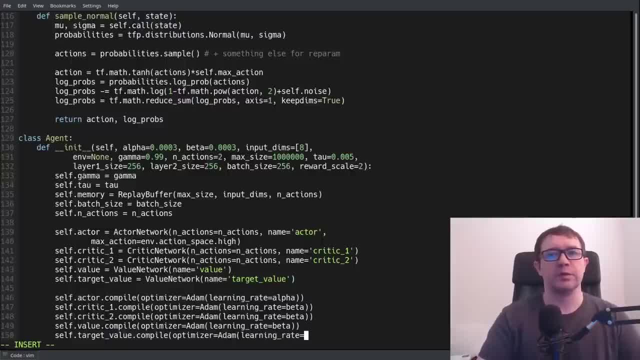 any optimization. we just copy weights using any optimization. we just copy weights using our soft update rule. but it is part our soft update rule. but it is part our soft update rule. but it is part of a. it's just part of the framework that we of a. it's just part of the framework that we. 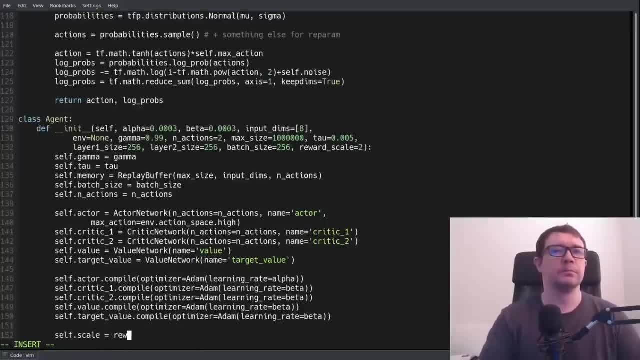 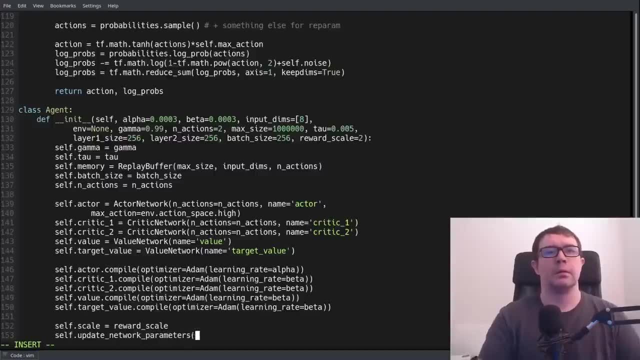 of a. it's just part of the framework that we have to compile the model. before we have to compile the model, before we have to compile the model, before we can use it, our scale factor and our initial can use it. our scale factor and our initial can use it. our scale factor and our initial update network parameters where. 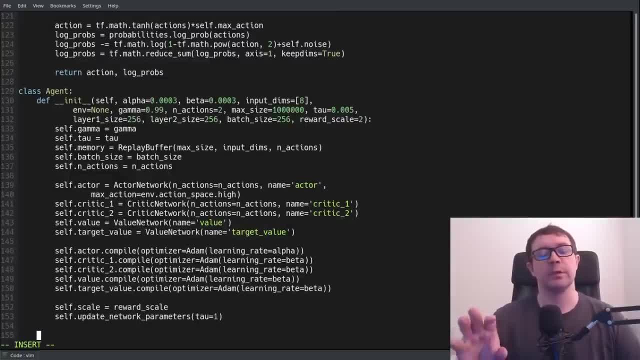 update network parameters. where update network parameters? where we're going to do a hard copy of the, we're going to do a hard copy of the, we're going to do a hard copy of the parameters from the online network to parameters from the online network to parameters from the online network to the target value network. the first: 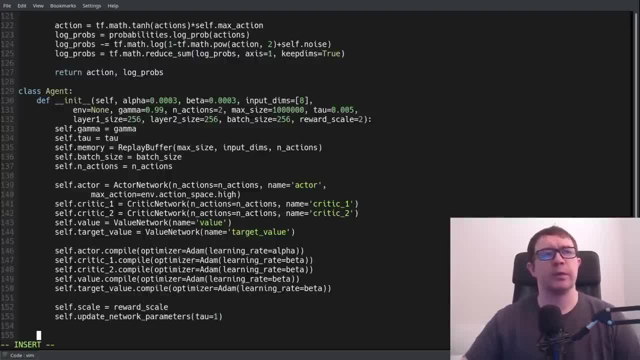 the target value network. the first, the target value network. the first function I want to handle is the choose function. I want to handle is the choose function. I want to handle is the choose action function. then we'll get to the action function, then we'll get to the. 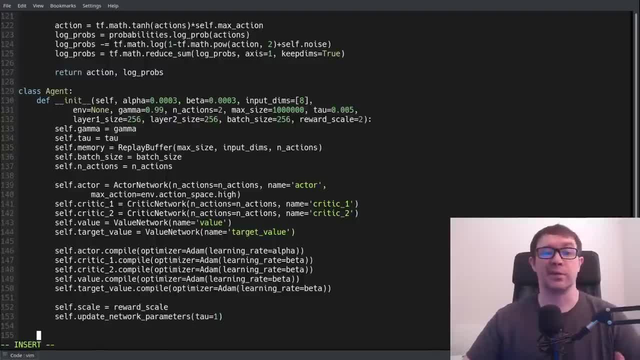 action function. then we'll get to the remember function, the update network remember function, the update network remember function, the update network parameters and our save model parameters and our save model parameters and our save model parameters. finally we'll get to the parameters. finally, we'll get to the. 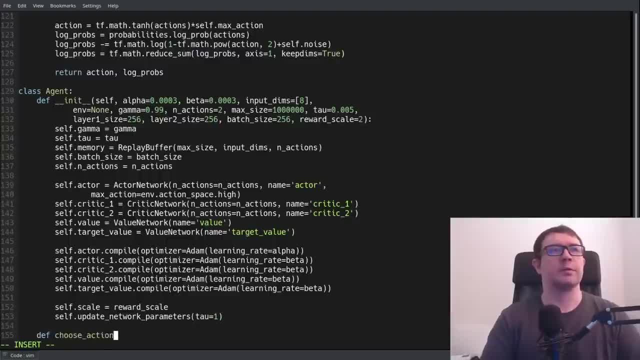 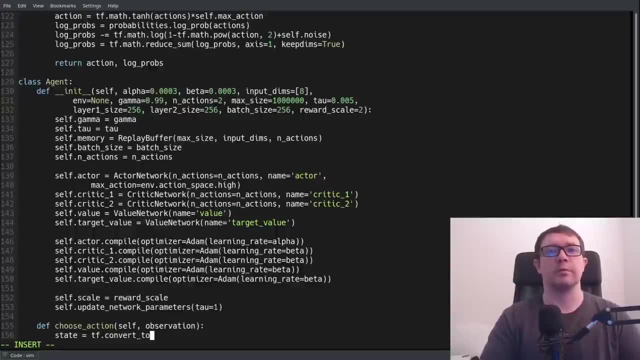 parameters. finally, we'll get to the learn function. we'll save the best for learn function. we'll save the best for learn function. we'll save the best for last. so we want to convert our state last. so we want to convert our state last. so we want to convert our state, our observation, to a tensor and the 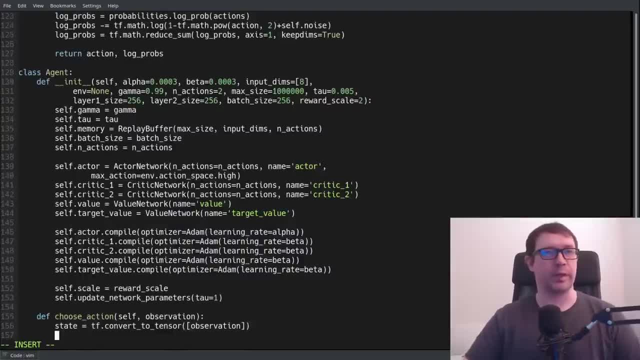 our observation to a tensor and the our observation to a tensor and the neural network expects that we will have neural network expects that we will have neural network expects that we will have a batch dimension. so we have to do that: a batch dimension. so we have to do that. 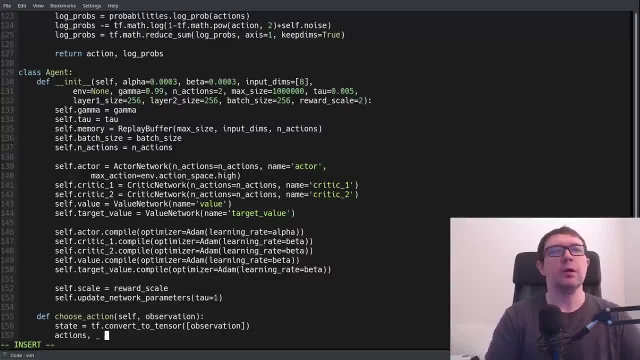 a batch dimension. so we have to do that. we have to add an extra dimension to get. we have to add an extra dimension to get. we have to add an extra dimension to get our batch. we want to get the actions we, our batch. we want to get the actions we. 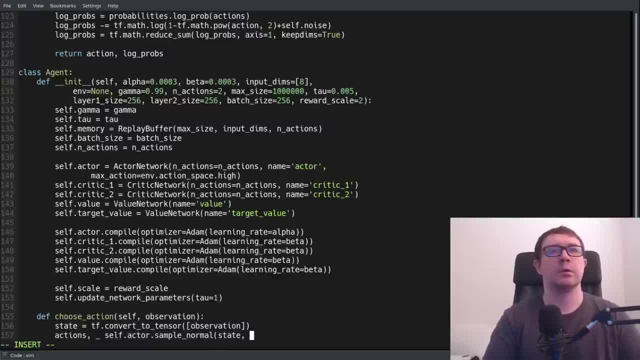 our batch. we want to get the actions. we don't really care about the log problems, don't really care about the log problems. don't really care about the log problems at this stage, and then we just go ahead at this stage, and then we just go ahead. 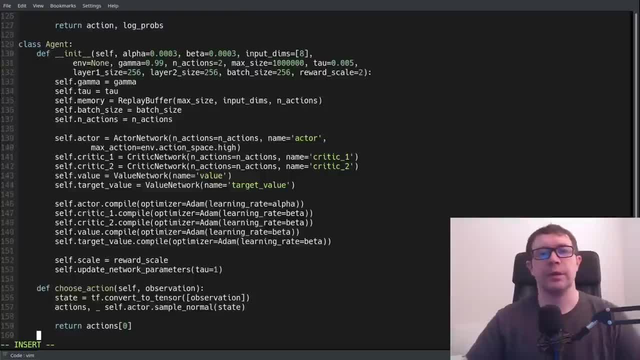 at this stage, and then we just go ahead and return actions zero because the and return actions zero because the and return actions zero because the tensor, I believe, is the output and we tensor, I believe, is the output and we tensor, I believe, is the output and we want to return a numpy array because the 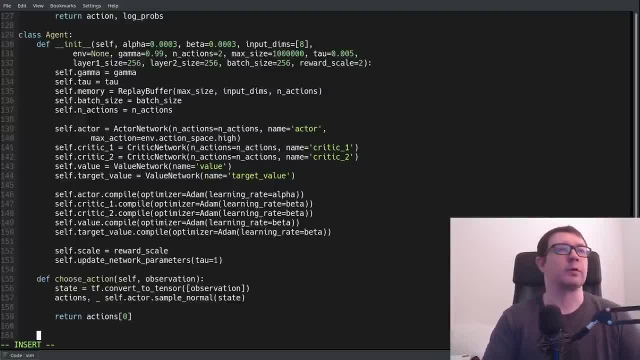 want to return a numpy array. because the want to return a numpy array? because the environment doesn't accept the tensor environment doesn't accept the tensor environment doesn't accept the tensor flow tensor as input to the step flow tensor as input to the step flow tensor as input to the step function. so this is a simple interstate. 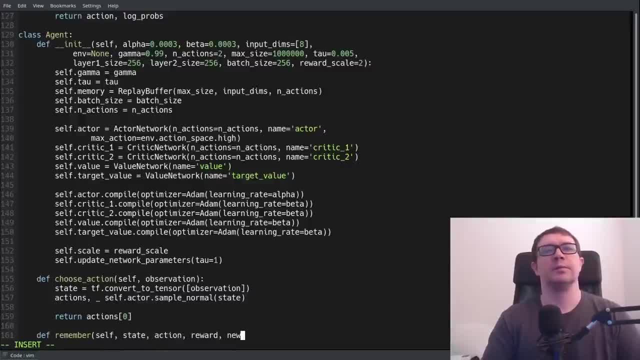 function. so this is a simple interstate function. so this is a simple interstate interface function between the agent and interface function between the agent and interface function between the agent and its memory. and this is necessary- its memory, and this is necessary, its memory. and this is necessary because you don't want to directly. 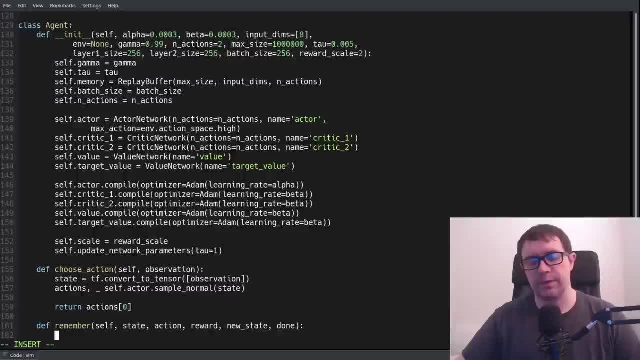 because you don't want to directly, because you don't want to directly access the values of the memory class. access the values of the memory class. access the values of the memory class from the agent class. it's just bad- from the agent class. it's just bad. 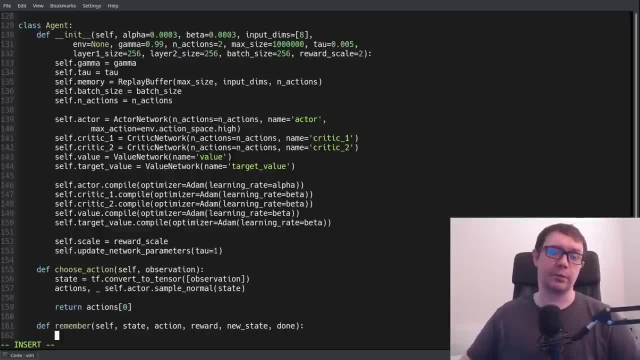 from the agent class. it's just bad software design. you don't want to go software design. you don't want to go software design. you don't want to go overriding parameters of one class with overriding parameters of one class with overriding parameters of one class with another. you want to have an interface. another. you want to have an interface another. you want to have an interface function that handles all that for you. function that handles all that for you. function that handles all that for you. that where you use one function to call, that, where you use one function to call. 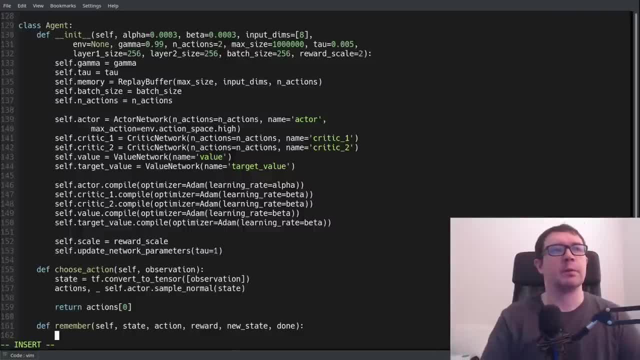 that where you use one function to call another, let's just clean software design another. let's just clean software design another. let's just clean software design. always keep that in mind. that takes a. always keep that in mind. that takes a. always keep that in mind. that takes a state action, reward new state and it. state action reward new state and it state action reward new state. and it looks kind of silly, we could get away. looks kind of silly, we could get away. looks kind of silly, we could get away with it in this context, because we're with it in this context, because we're. 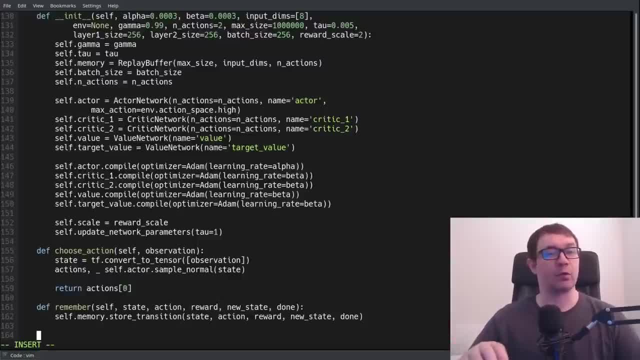 with it in this context, because we're not going to be building on this, not going to be building on this, not going to be building on this code base later, but I always find it code base later, but I always find it code base later. but I always find it important to use strong and consistent. 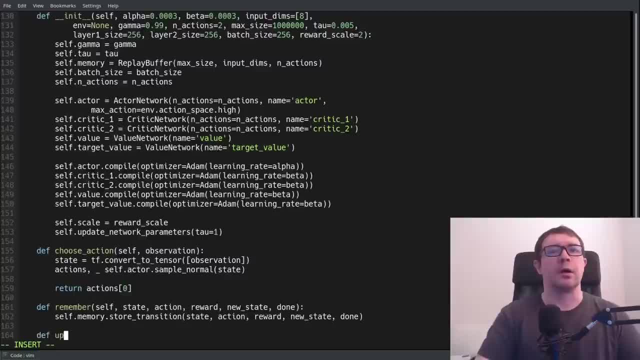 important to use strong and consistent. important to use strong and consistent software design principles wherever software design principles wherever software design principles. wherever possible, our update network parameters possible, our update network parameters possible, our update network parameters function. it's pretty straightforward so function. it's pretty straightforward so. 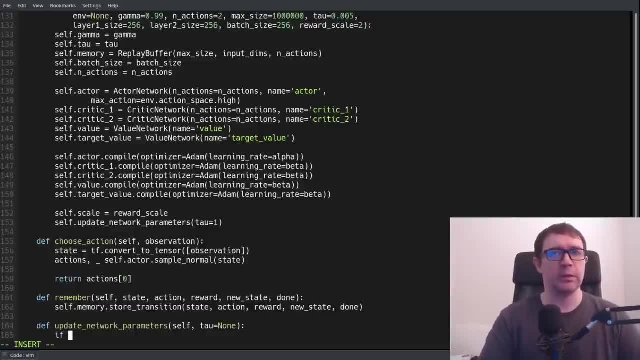 function. it's pretty straightforward. so we're gonna pass in a towel which is a. we're gonna pass in a towel which is a. we're gonna pass in a towel which is a default value of none. so if tout is none, default value of none. so if tout is none. 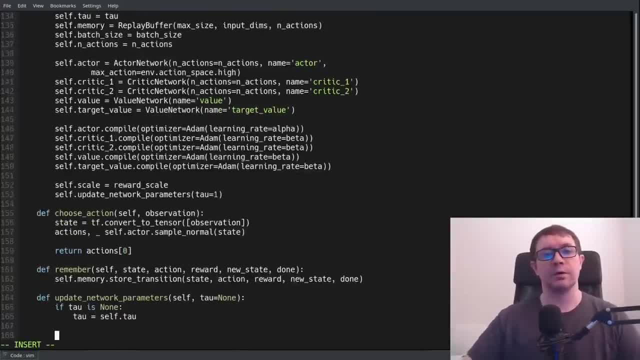 default value of none. so if tout is none, then we want to go ahead and use our, then we want to go ahead and use our. then we want to go ahead and use our default value for towel, and this has to default value for towel, and this has to. 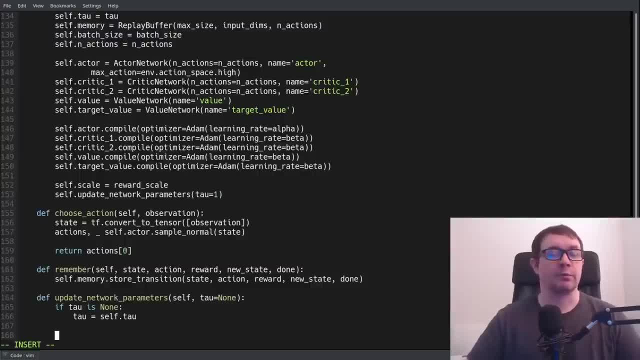 default value for towel. and this has to do with the fact that up here on line 153, do with the fact that up here on line 153, do with the fact that up here on line 153, we're calling update network parameters, we're calling update network parameters. 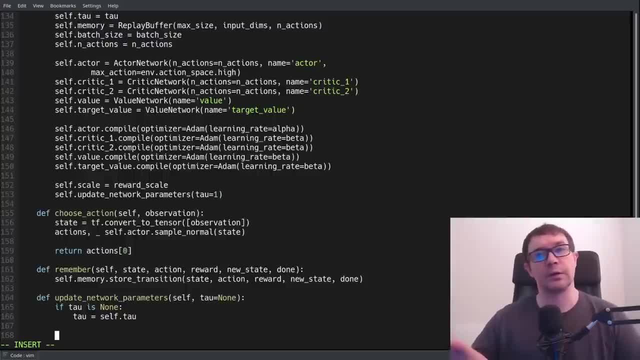 we're calling update network parameters. of the value of tau equals one to. of the value of tau equals one to. of the value of tau equals one to facilitate the hard network of hard, facilitate the hard network of hard, facilitate the hard network of hard network, weight copy. so we're basically 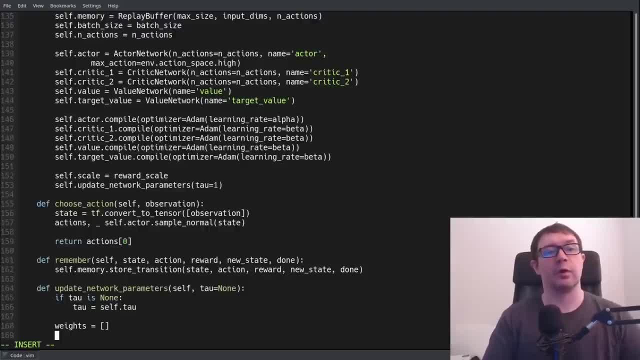 network weight copy. so we're basically network weight copy. so we're basically gonna just go ahead and iterate over our gonna just go ahead and iterate over our. gonna just go ahead and iterate over our network weights. do the calculation network weights? do the calculation network weights? do the calculation? append those to a list and then upload. 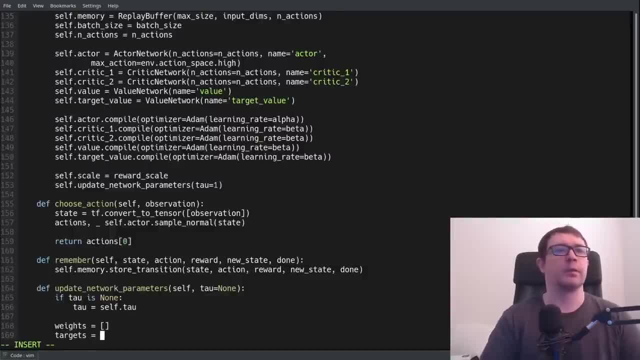 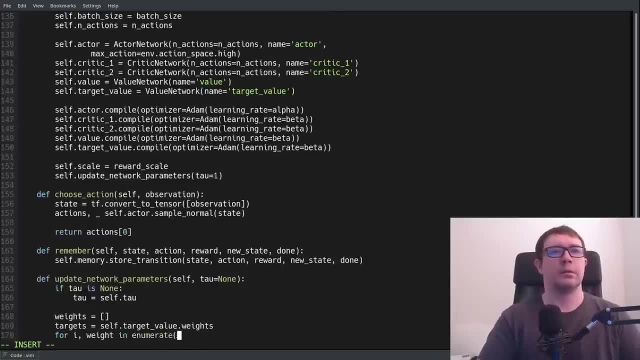 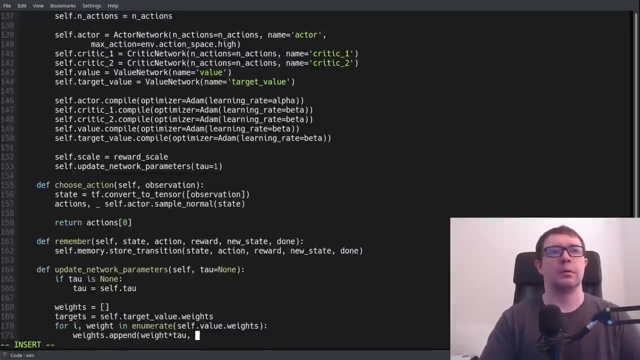 append those to a list and then upload. append those to a list and then upload that list to our value target by your that list, to our value target by your that list, to our value target by your network network network network weight times, tau plus targets times one. 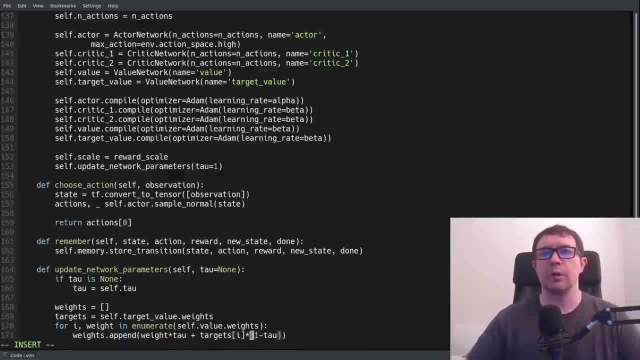 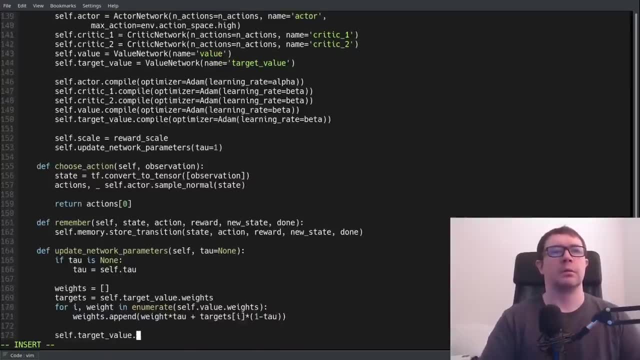 weight times tau plus targets: times one. weight times tau plus targets times one minus tau. minus tau minus tau. i have one too many parentheses there. i have one too many parentheses there. i have one too many parentheses there. that looks right. set weights and that is it for our update. 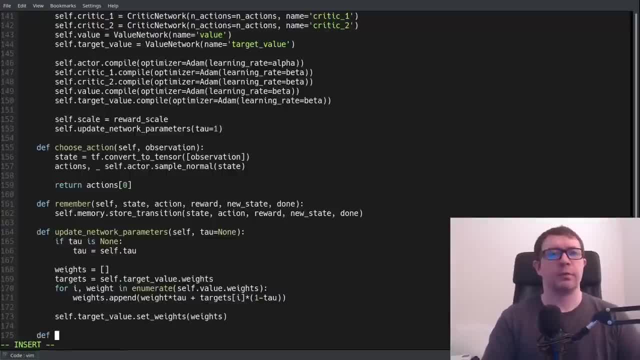 set weights. and that is it for our update set weights. and that is it for our update network parameters. network parameters, network parameters- pretty straightforward. next, we have two- pretty straightforward. next we have two: pretty straightforward. next, we have two bookkeeping functions to save our bookkeeping functions, to save our. 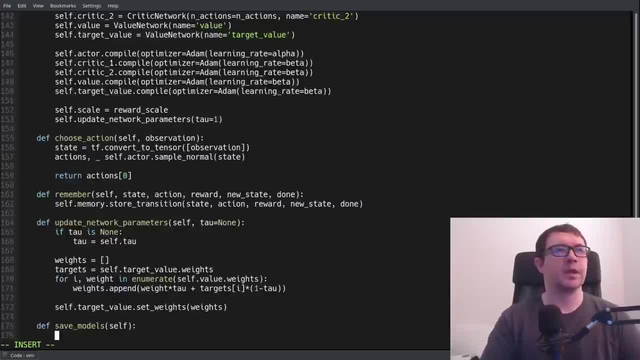 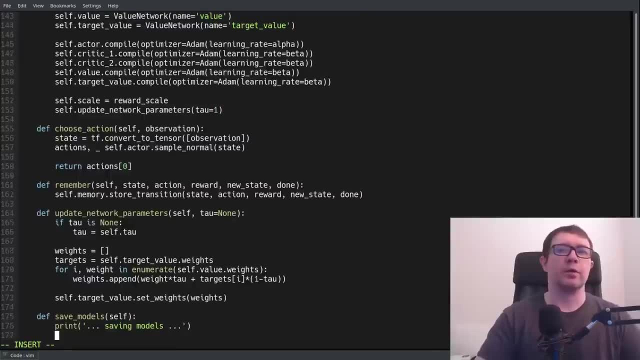 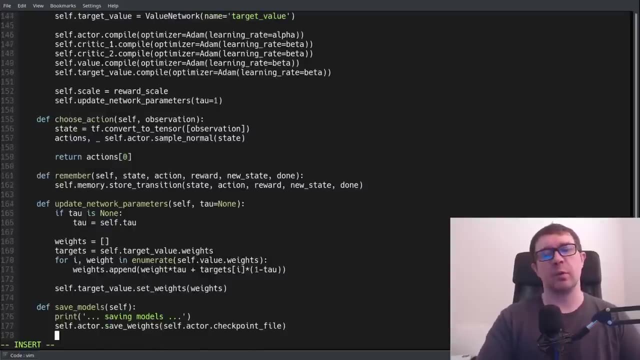 bookkeeping functions to save our models, models, models, those don't take any inputs. those don't take any inputs. those don't take any inputs. surveying, surveying, surveying. that is not useful information. so we just want to save the weights to. so we just want to save the weights to 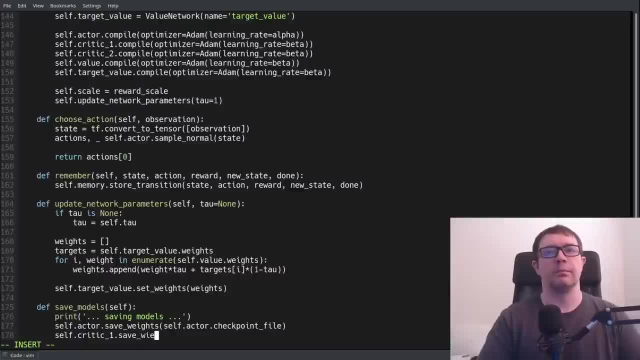 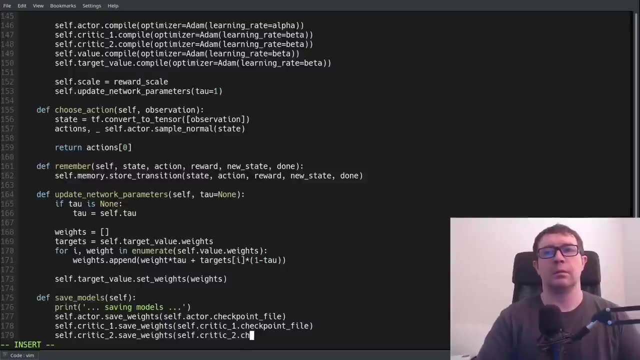 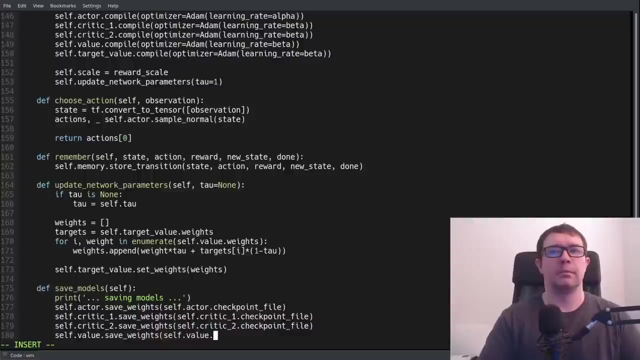 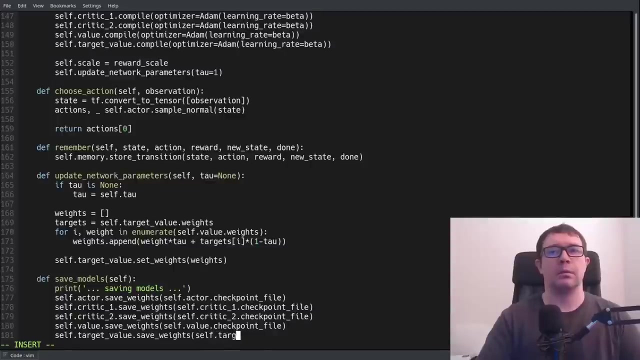 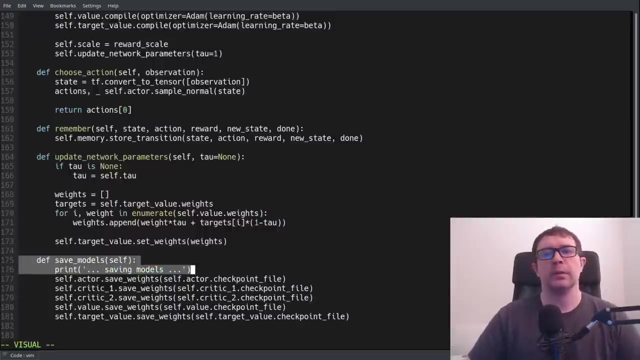 so we just want to save the weights to the checkpoint file. check pint, i'll take a pint that sounds check pint, i'll take a pint that sounds check pint, i'll take a pint. that sounds pretty good, pretty good, pretty good. and then the load models function. 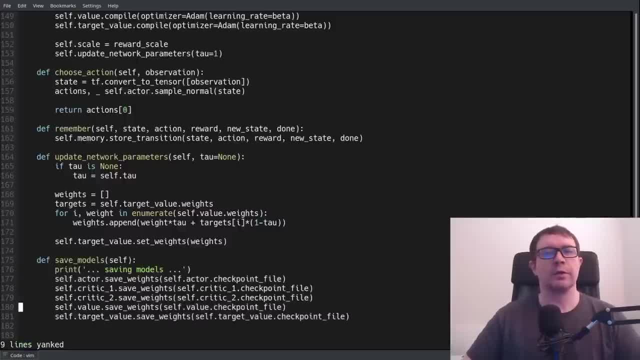 and then the load models function. and then the load models function is basically the inverse, is basically the inverse, is basically the inverse. so i'm just going to go ahead, and so i'm just going to go ahead, and so i'm just going to go ahead and yank and paste and then make sure to 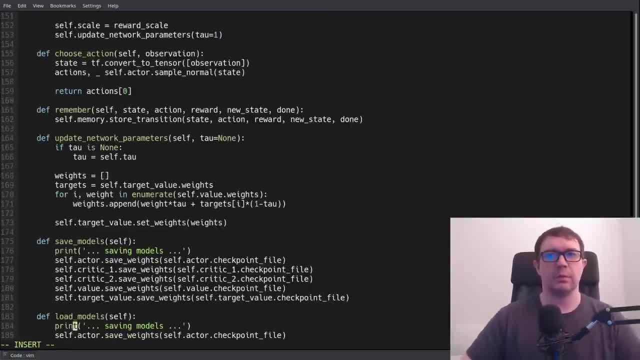 yank and paste and then make sure to yank and paste and then make sure to change save to load. so that way we don't do anything wonky. so that way we don't do anything wonky. so that way we don't do anything. wonky actor dot save weights. we want to change. 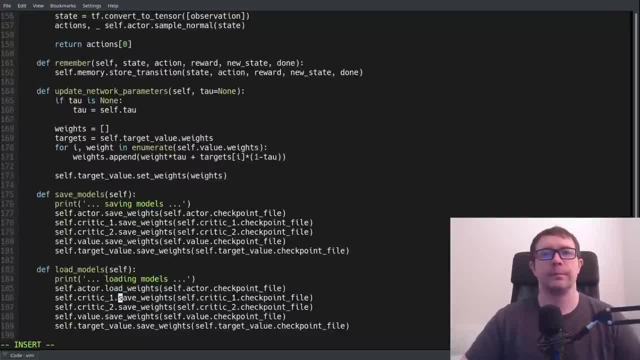 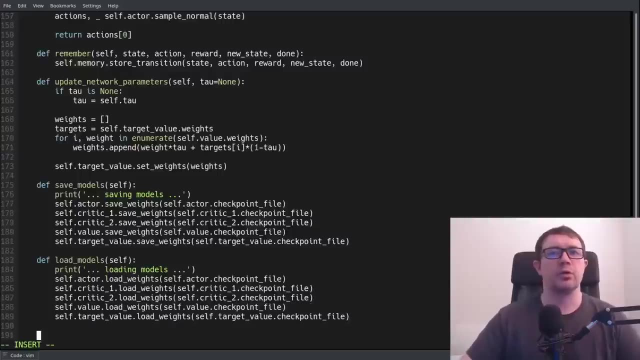 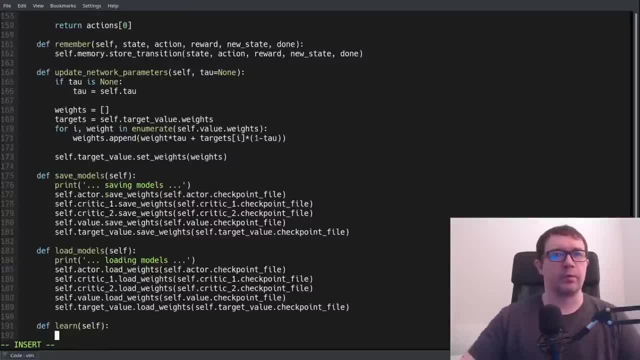 check point files. check point files. okay, now we come to the hard part of the okay. now we come to the hard part of the okay. now we come to the hard part of the problem: the learn function problem, the learn function problem, the learn function. now we've got a kitty cat joining us. 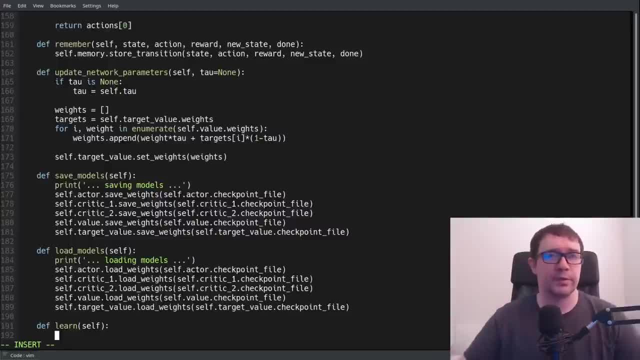 now we've got a kitty cat joining us. now we've got a kitty cat joining us. perhaps she will hop up on the desk the. perhaps she will hop up on the desk the. perhaps she will hop up on the desk. the first uh consideration we have, so the 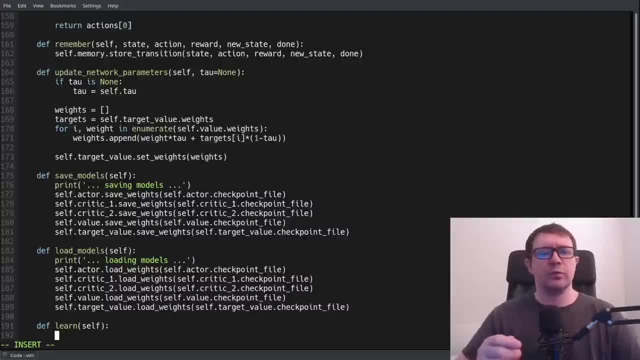 first uh consideration we have. so the first uh consideration we have. so the first consideration we have is first consideration we have is first consideration we have is what we would do, what we do in the event, what we would do what we do in the event, what we would do, what we do in the event that we haven't filled up. 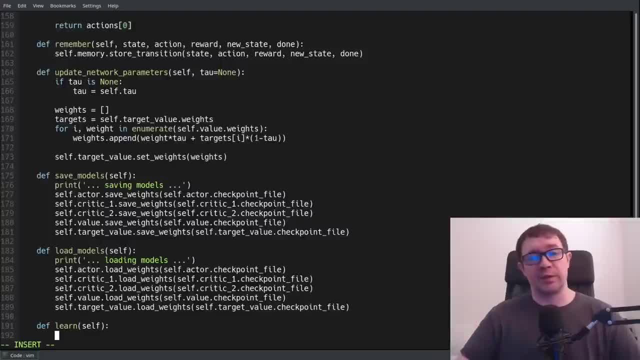 that we haven't filled up, that we haven't filled up enough of our memories to actually load a enough of our memories to actually load a enough of our memories to actually load a batch size of those memories, batch size of those memories, batch size of those memories. and you can do many different things. you 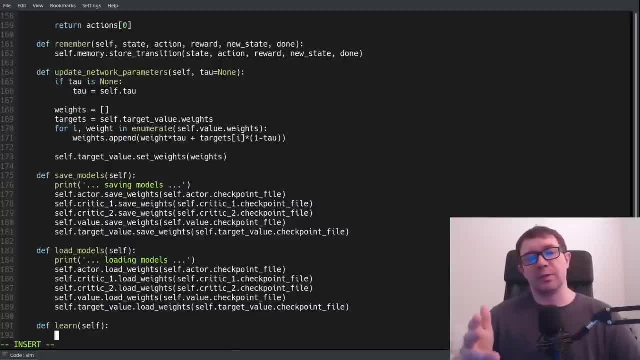 and you can do many different things. you and you can do many different things. you can, can. can play batch size of transitions randomly. play batch size of transitions randomly, play batch size of transitions randomly and store those transitions and then and store those transitions and then and store those transitions and then call your learn function. call your learn function. call your learn function. or, in this case, you can just say hey if i. or, in this case, you can just say hey if i. or, in this case, you can just say hey, if i haven't filled up at least batch size. haven't filled up at least batch size. 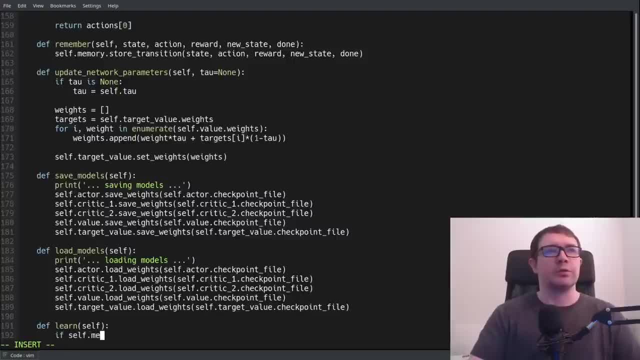 haven't filled up at least batch size of memories. just go ahead and return of memories. just go ahead and return of memories. just go ahead and return. so that's what we're going to do. so that's what we're going to do. so that's what we're going to do, and this is a. this violates my principles. and this is a. this violates my principles and this is a. this violates my principles of good software design. where i'm of good software design, where i'm of good software design, where i'm calling the mem counter of the memory, calling the mem counter of the memory. 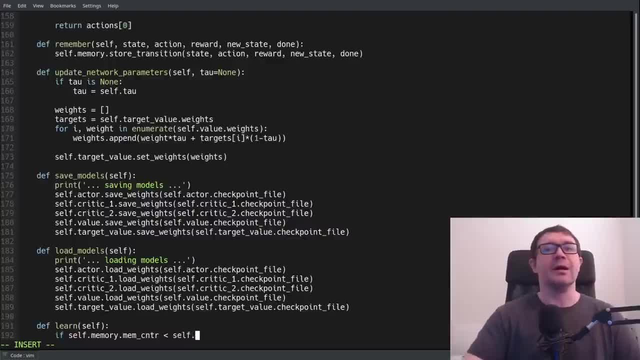 calling the mem counter of the memory class directly here instead of using a class directly here, instead of using a class directly here, instead of using a function to get it. function to get it, function to get it. uh, this is bad design. uh, this is bad design. uh, this is bad design. um. 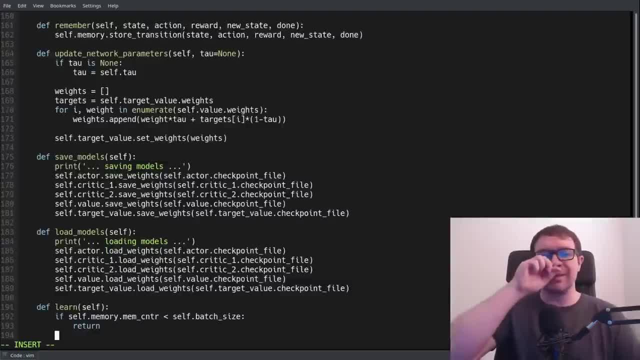 um, um, so don't do this. if you have an option, so don't do this. if you have an option, so don't do this. if you have an option not to, i'm just doing this, not to. i'm just doing this, not to. i'm just doing this, uh, because it's like i said, it's not. uh, because it's like i said, it's not. uh, because it's like i said, it's not going to matter. going to matter, going to matter. it's: this isn't a huge code base, that it's. this isn't a huge code base, that it's. this isn't a huge code base, that we're. 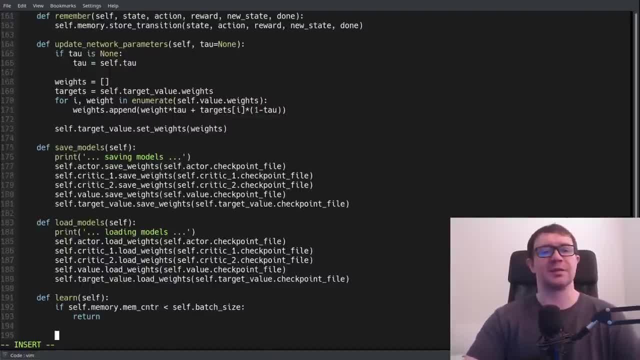 we're. we're going to be building upon later, but just going to be building upon later, but just going to be building upon later. but just know that this isn't consistent with know that this isn't consistent with know that this isn't consistent with what i said earlier. 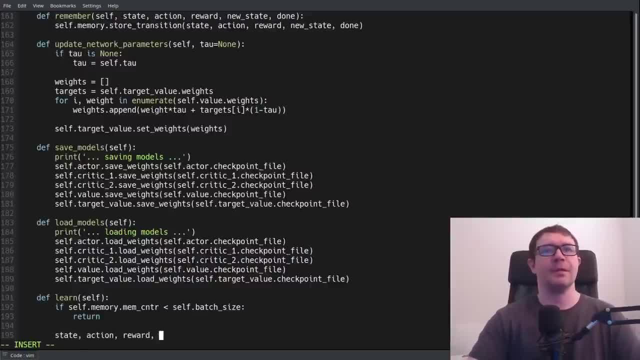 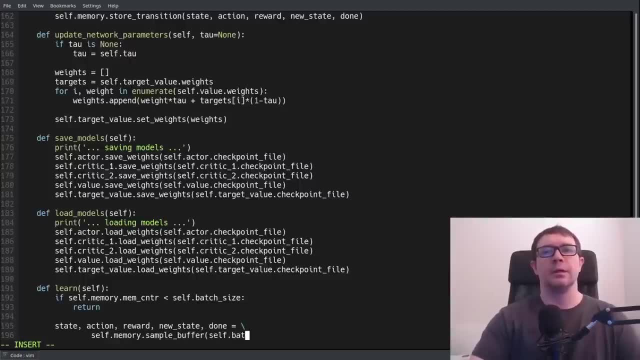 what i said earlier. what i said earlier- i'm kind of backpedaling a little bit. now we have to sample our memory. now we have to sample our memory. now we have to sample our memory. and we got to pass in our batch size. and we got to pass in our batch size. 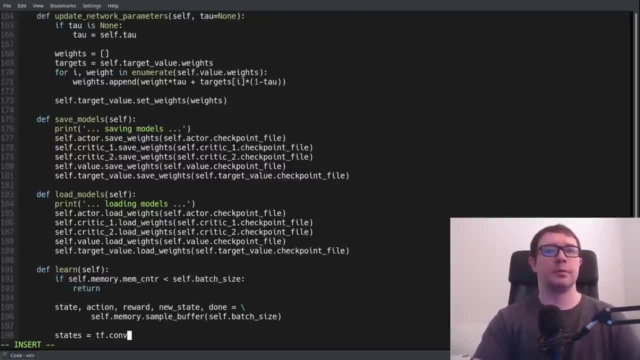 and we got to pass in our batch size, then we want to go ahead and convert, then we want to go ahead and convert, then we want to go ahead and convert those to tensors, and i want to be really consistent with, and i want to be really consistent with 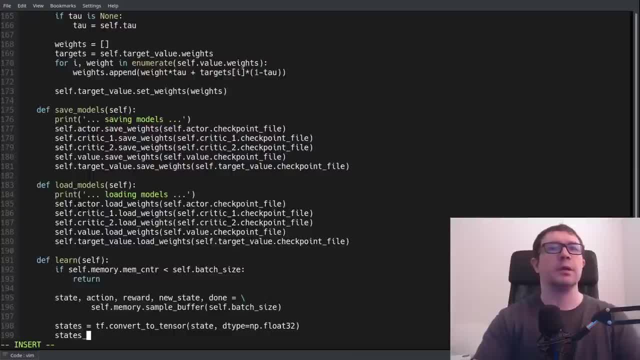 and i want to be really consistent with my data types here, my data types here, my data types here. reason being, reason being, reason being a lot of these frameworks tensorflow and a lot of these frameworks tensorflow and a lot of these frameworks tensorflow and pytorch specifically, pytorch specifically. 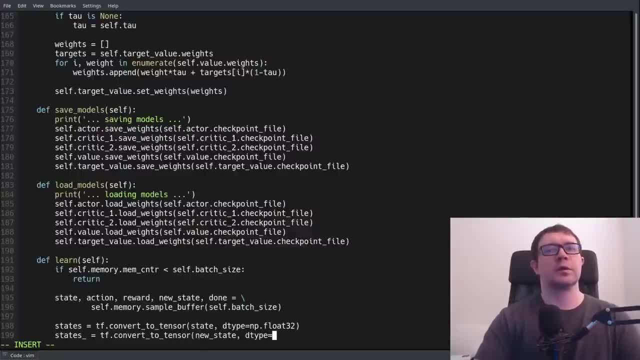 pytorch, specifically: get a little bit finicky when you start get a little bit finicky when you start get a little bit finicky when you start mixing up data types. they don't like to mixing up data types, they don't like to mixing up data types, they don't like to mix. 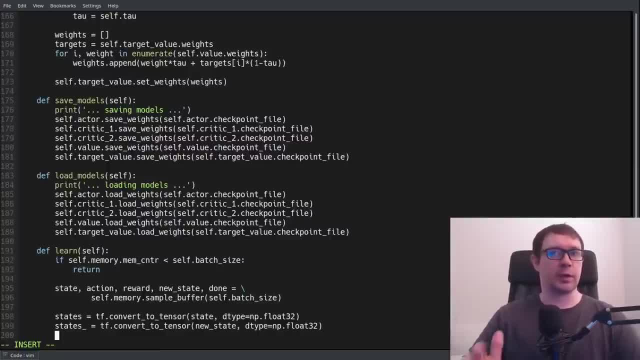 mix, mix, data types and calculations, because that data types and calculations, because that data types and calculations, because that screws up the precision of the, screws up the precision of the, screws up the precision of the calculation, calculation, calculation. they want everything to be, they want. they want everything to be they want. 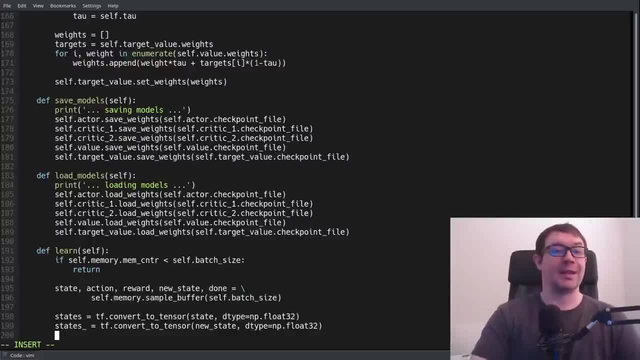 they want everything to be. they want everything to be consistent and explicit, everything to be consistent and explicit. everything to be consistent and explicit, so that you get exactly what you expect, so that you get exactly what you expect. so that you get exactly what you expect because, of course, there is a rather 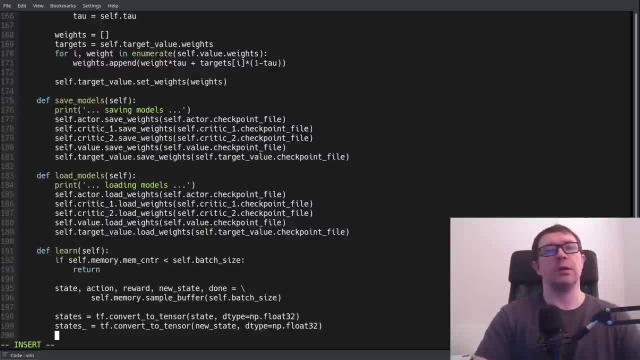 because of course there is a rather, because of course there is a rather significant difference in large, significant difference in large, significant difference in large calculations between floating point 32, calculations between floating point 32, calculations between floating point 32, floating point 64, even floating point 16. 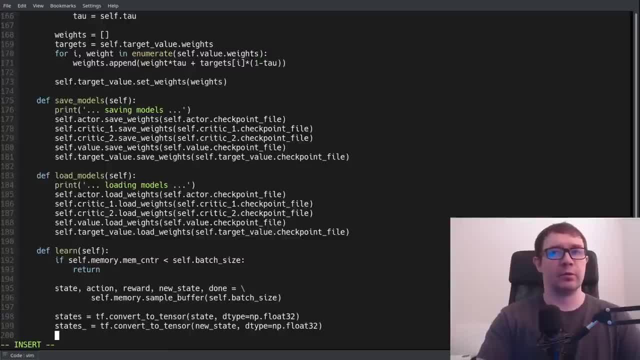 floating point 64. even floating point 16. floating point 64. even floating point 16. calculations, calculations, calculations. so it's very beneficial to go ahead, and so it's very beneficial to go ahead, and so it's very beneficial to go ahead and specify what data type you're using. 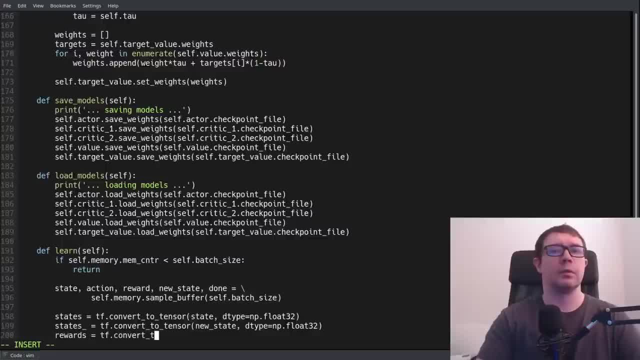 specify what data type you're using. specify what data type you're using. in this case, we use float 32 and we, even in theory, could get away, and we even in theory could get away, and we even in theory could get away with uh, uh, with uh uh. 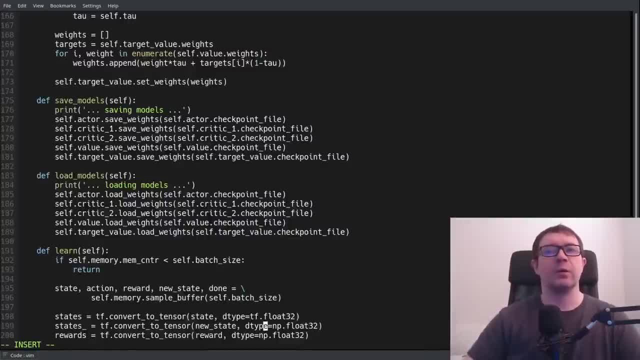 with: uh, uh sorry, these are sorry, these are sorry, these are tf, not np. we could get away with tf, not np. we could get away with tf, not np. we could get away with: uh 16 point, because 16 point precision. uh, 16 point because 16 point precision. 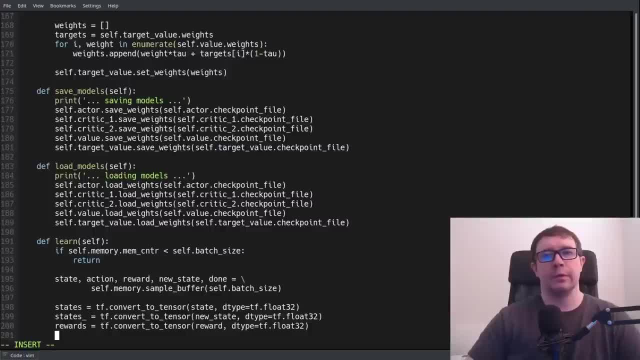 uh, 16 point, because 16 point precision, 16-bit precision. excuse me because we 16-bit precision. excuse me because we 16-bit precision. excuse me because we don't need, don't need, don't need. you know a whole bunch of decimal places. you know a whole bunch of decimal places. 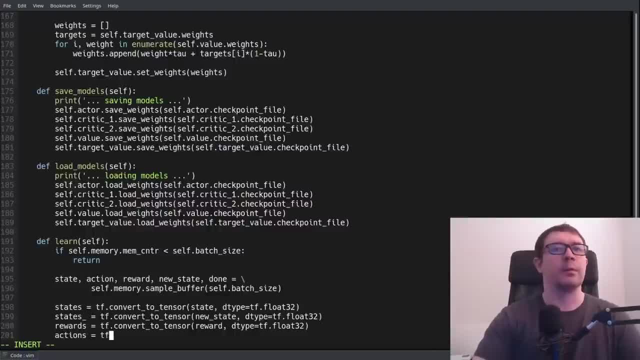 you know a whole bunch of decimal places in our rewards or anything like that in our rewards or anything like that in our rewards, or anything like that, but we'll use 32, but we'll use 32, but we'll use 32 just to be safe. 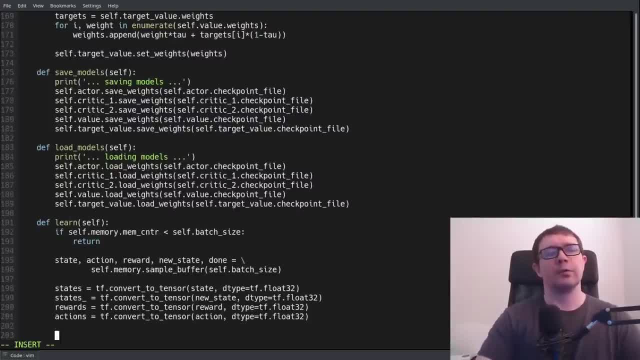 just to be safe, just to be safe. so now we're going to handle the update. so now we're going to handle the update. so now we're going to handle the update. rule for our value network, rule for our value network, rule for our value network. so we need our gradient tape. 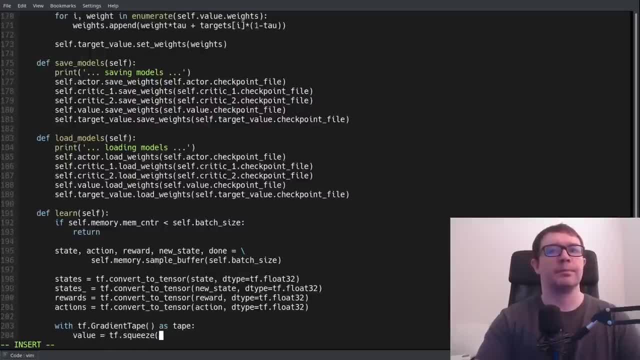 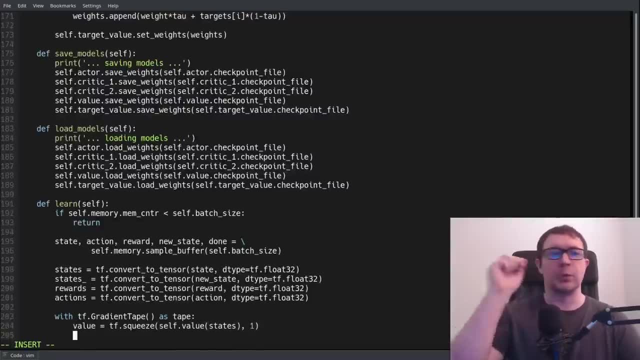 so we're going to pass the state states through our network and state states through our network and state states through our network and then squeeze to get rid of that batch, then squeeze to get rid of that batch, then squeeze to get rid of that batch. dimensionality. 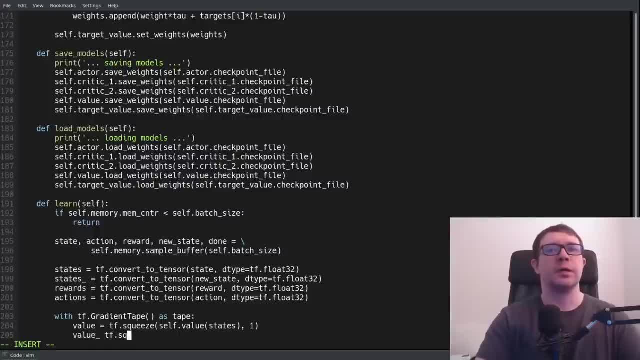 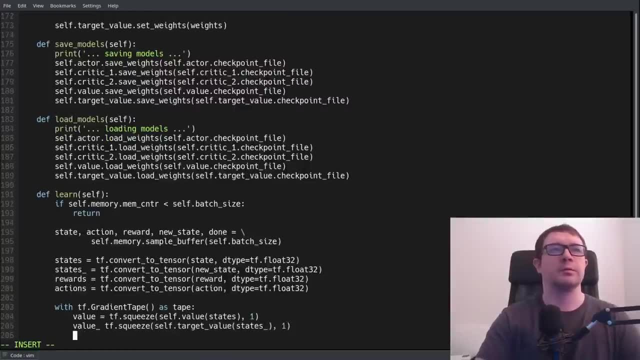 dimensionality, dimensionality, then we're going to do the same thing, then we're going to do the same thing, then we're going to do the same thing with, with, with our new states, our new states, our new states, except we're going to pass through the target value network squeeze again. what are the actions? 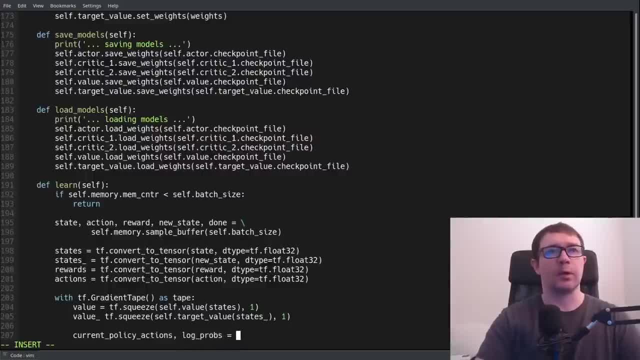 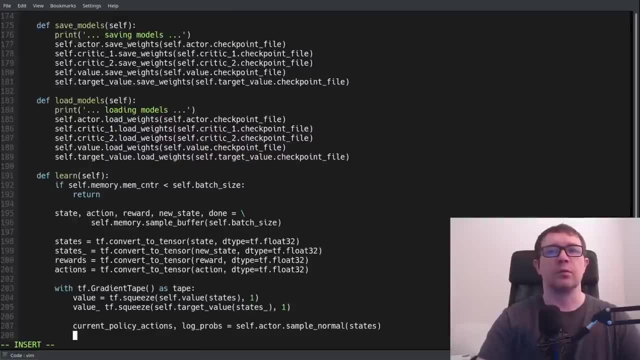 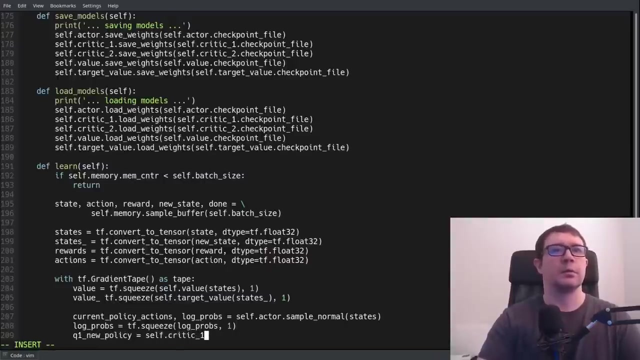 occurring according to our current policy and the log probes. so we're going to sample normal states and we of course don't do any re-parameterization. so then our log probes we have to squeeze, then we get the values according to the new policy critic: one states policy actions. 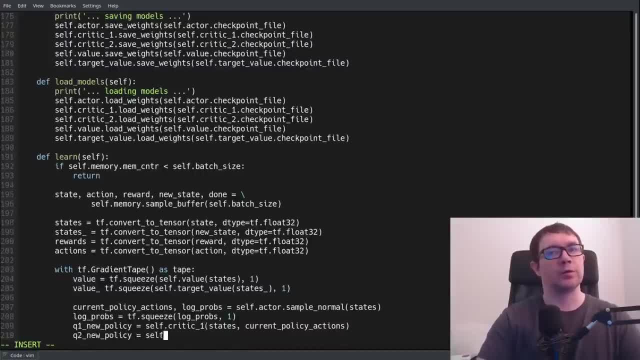 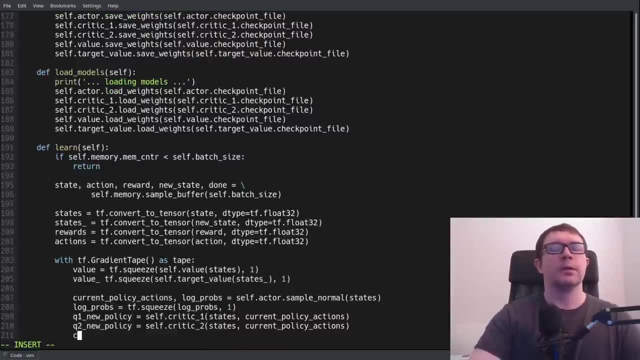 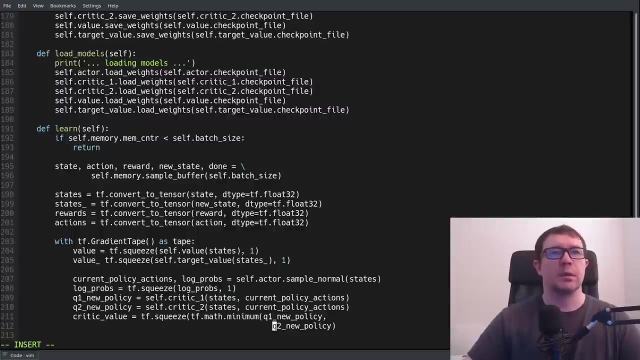 and then the value according to the second critic. then our critic value. not that value: tfsqueeze, tf math minimum between the q1 new policy, q2 new policy, and I'm missing a parentheses there. there we go. now we're gonna squeeze along the first dimension. so then our value. 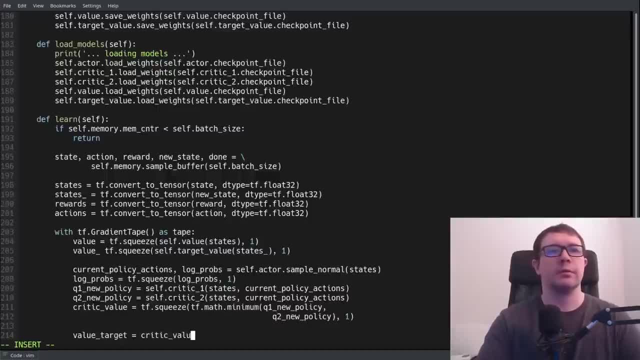 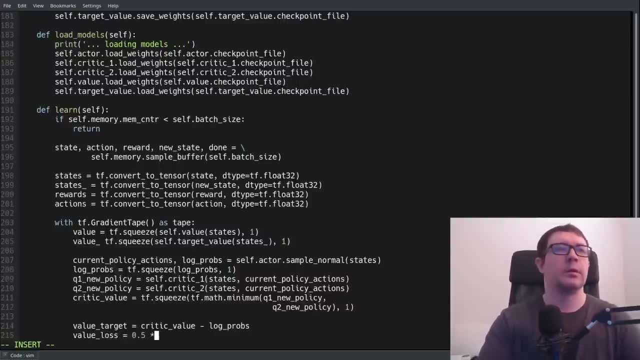 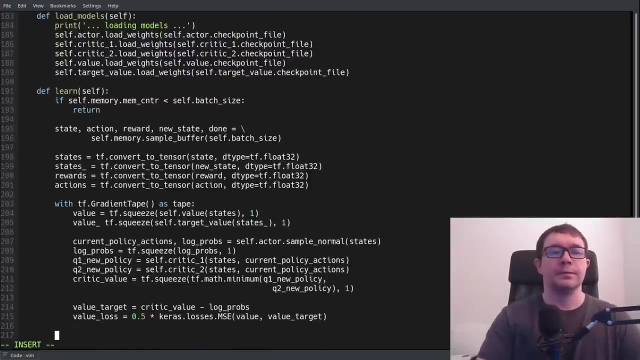 target is going to be our critic by you, minus our log problems. that's from the paper value loss: 1 half Karos losses dot mean squared error between the value and the target. value value target. sorry, sorry, my toddlers rampaging again. so now I'm马他是 rampaging again. 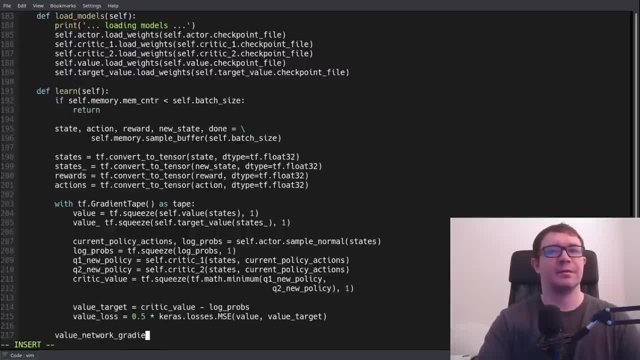 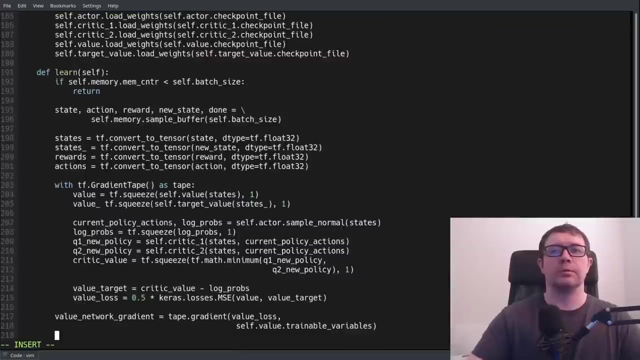 so now we need to calculate our gradient. good grief, I have the cat on my lap as well. that's making it very difficult to type value loss, self dot. value dot- trainable variables- and we can stick that on a new line to be good little programmers. then we have to apply our gradients: optimizer dot- apply gradients. 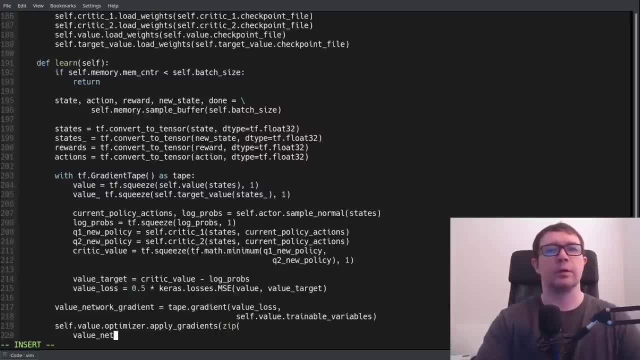 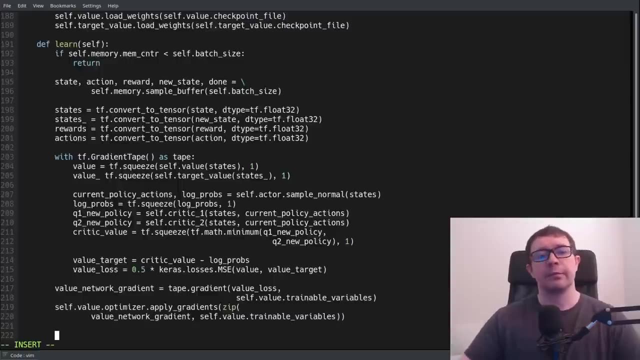 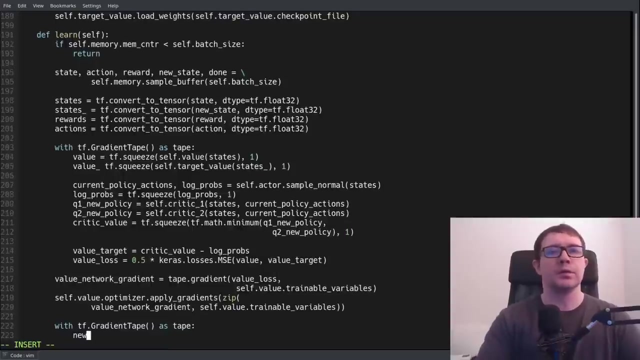 zip value, network gradient value, trainable variables, and this is just how we do: gradient descent using the gradient tape. and so that is it for our value network loss. now we have our actor network and critic networks to worry about. so we need more gradient tapes, so we need our new policy actions and their log probes. we're on a sample. 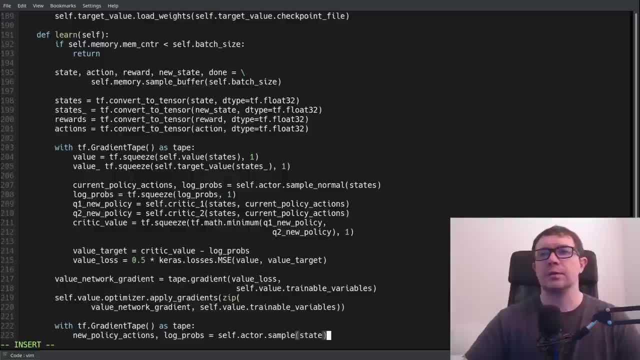 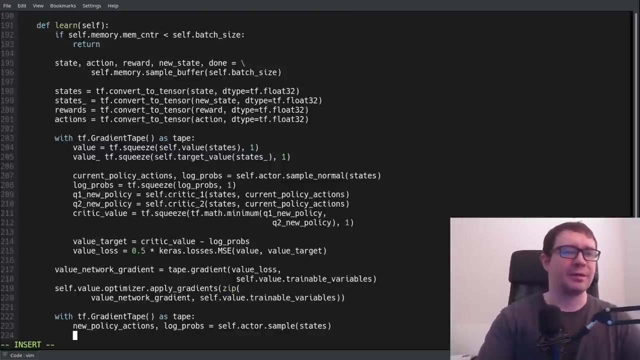 our States. oh, that's interesting. I have- I see that's interesting- in my sheet sheet here. I have the numpy arrays and it works interesting. I'll go ahead and fix that. so let's see if it breaks when I pass in the tensorflow tensors. it shouldn't. I just have a typo in my cheat sheet. so let's go ahead and. 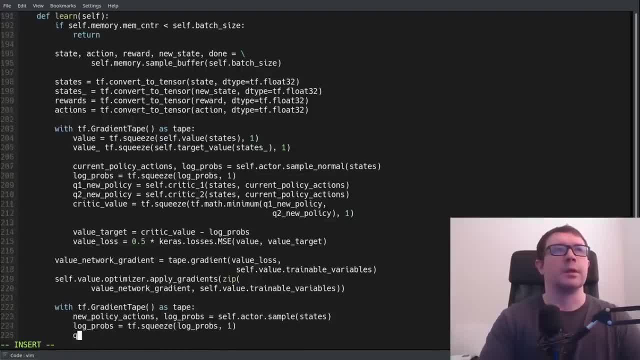 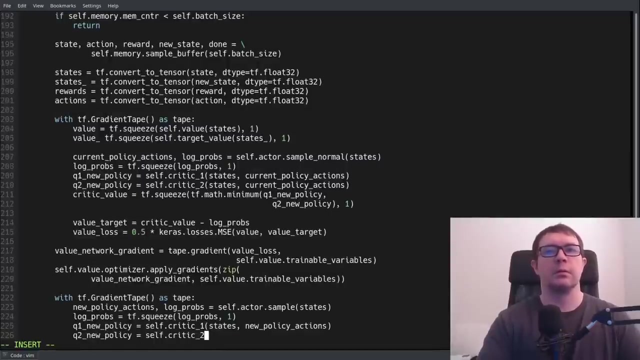 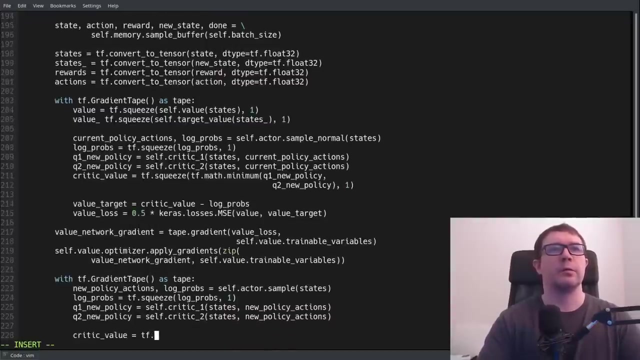 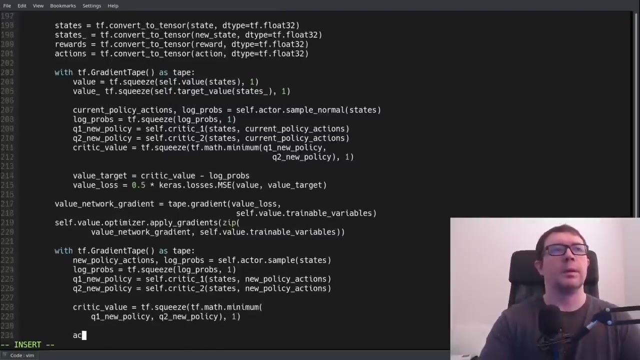 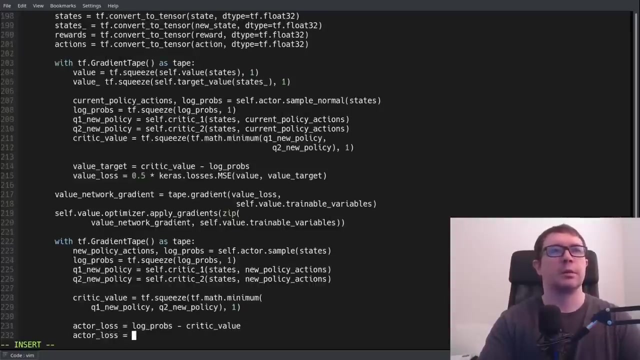 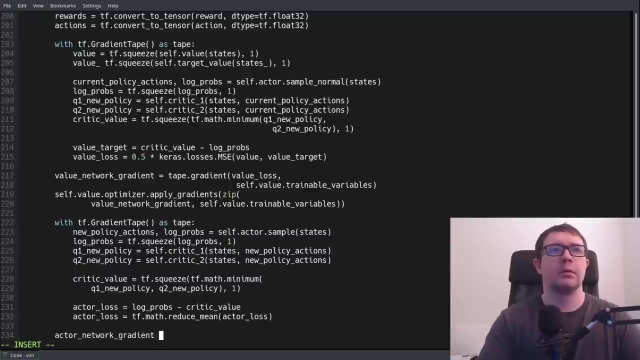 squeeze our log probes and get some new policy values and dot critic one new policy, actions q2 new policy and we have our critic value, squeeze math minimum. you then our actor loss, just the log probes. minus that critic value, actor loss equals math reduce mean actor loss. then we have our actor network gradient tape, gradient after loss. 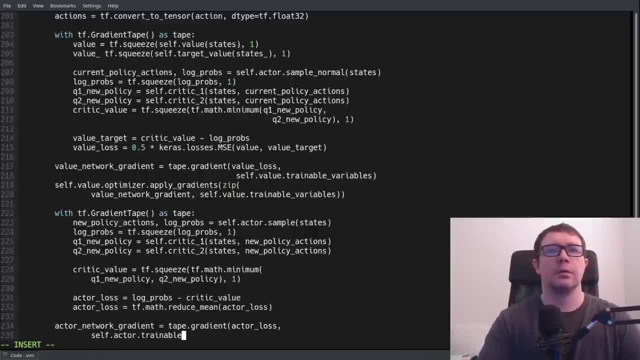 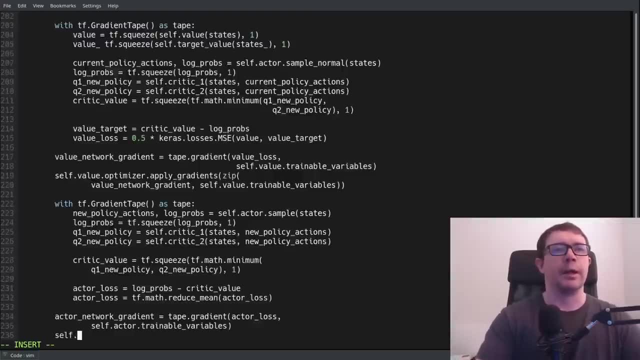 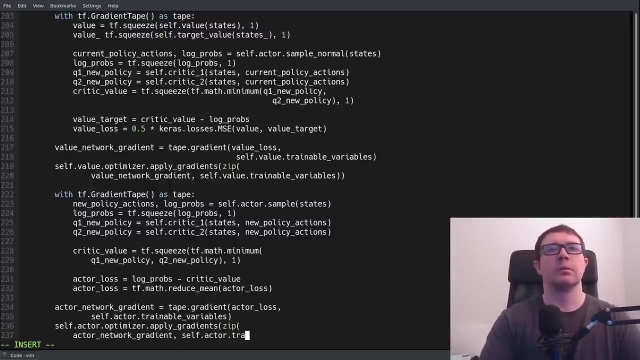 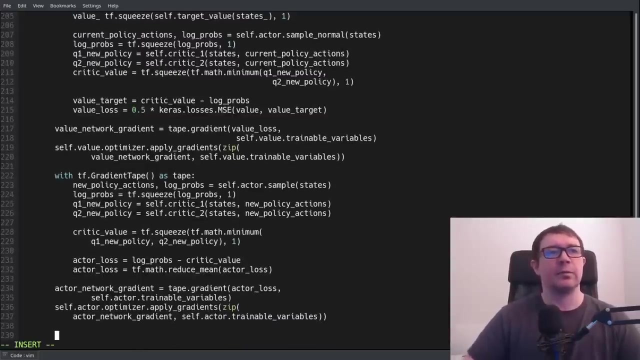 the gradient of our loss with respect to our actor trainable variables. then we want to apply our gradients actor optimizer and of course that expects a zip as input and that handles our actor loss. and then we want to apply our gradients actor optimizer and of course that the gradient of our loss and finally we come to the critic loss. 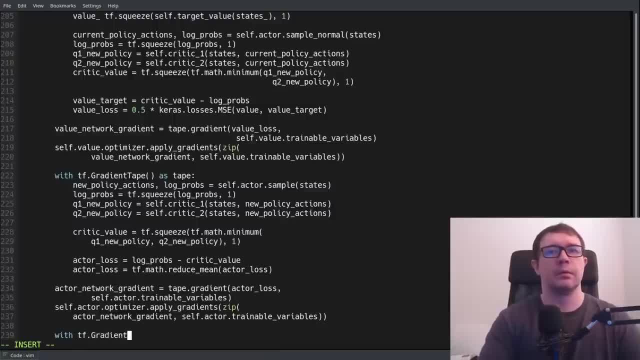 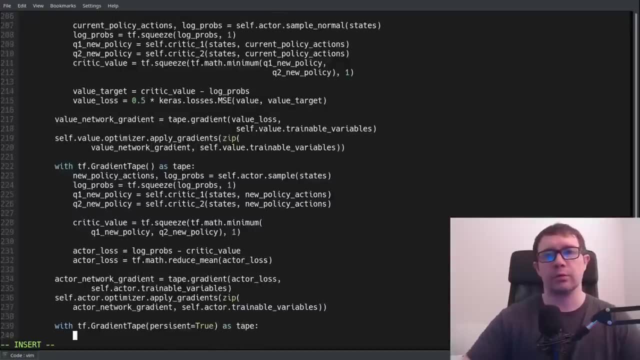 now we have to pass the persistent equal true parameter to our function call, because the loss is going to have two components, so we'll have a critic one and critic two loss if you don't pass the persistent equals true flag. it only keeps track of stuff for the 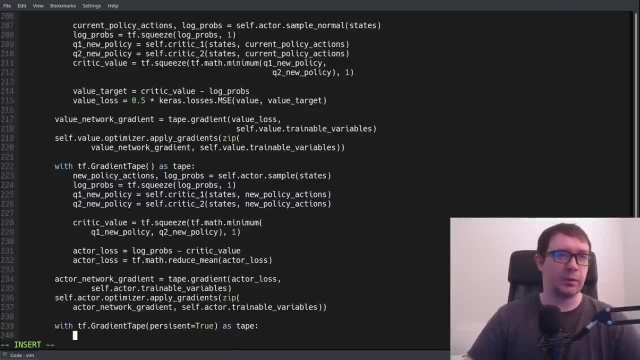 application of a single set of gradients. so you can only do the update to one of your critic networks instead of both. so you tell it to just keep track of the gradients even after it go ahead. have even after it applies gradients one time so you can apply gradients twice. a cute hat is our scale factor and multiplied. 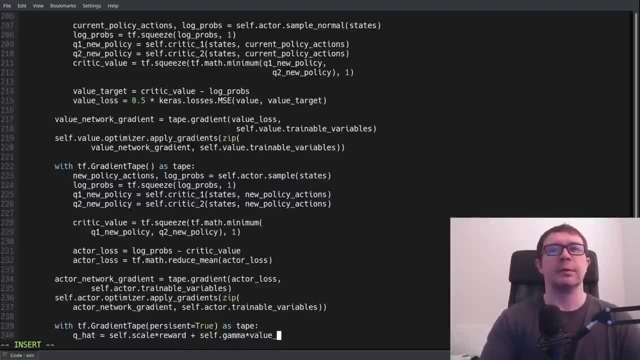 by a reward. that's where the entropy comes in. gamma times value underscore 1, minus done. that is interesting. so this gives me a little bit of pause because, first of all, I know the code works. I've tested this and I haven't accidentally deleted a line. but what gives me pause here is that I have this value. 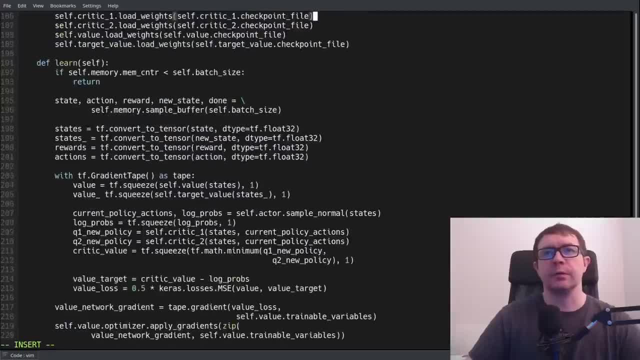 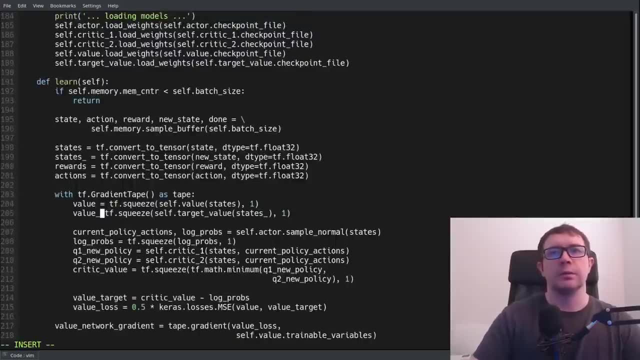 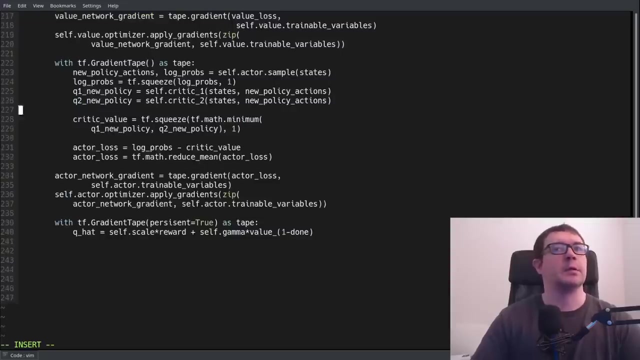 underscore, which is defined up in this other scope. here I'm actually missing a equal sign there that would have triggered an error. so it does work. that's interesting. I didn't know that the context manager shared the scoping of variables. I didn't know that. that is new information to me, so I 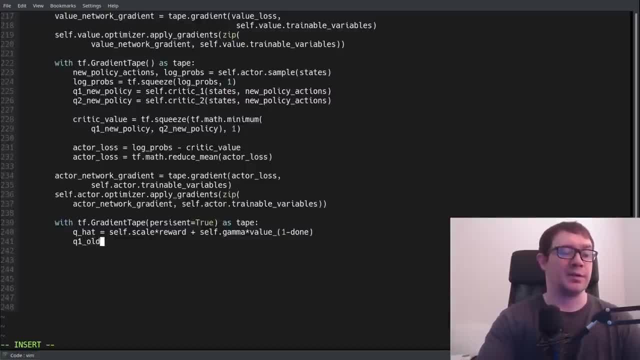 want to go ahead and roll with it for now. if this is suddenly broken and doesn't work, then I will come back and re-edit this and put in the new code. that actually works, of course, but that is new information to me. qui learn stuff even while making content. so we have to get the values according to the overnight. 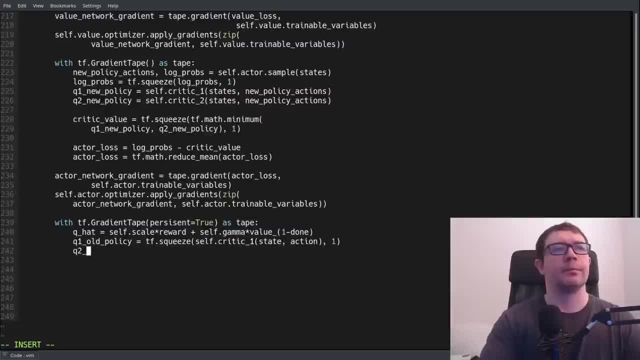 policy. why do I call it old policy? perhaps go ahead and check the github for this. when I upload it. I will probably do some variable name swapping to make things a little bit more logical. if I have to scratch my head while I'm typing out the code here, you're probably 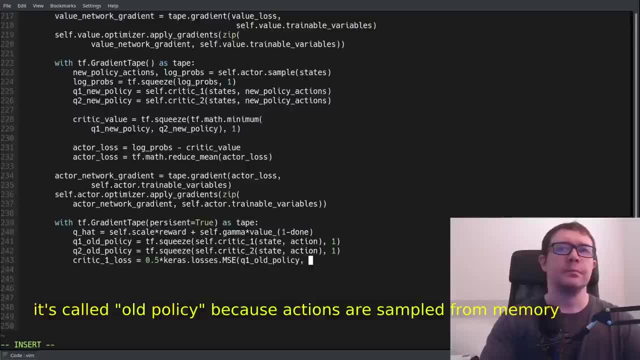 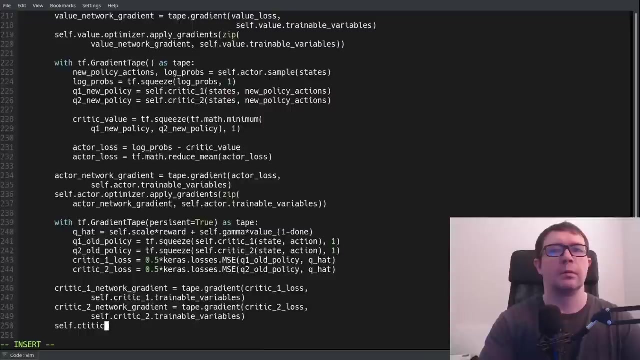 scratching your head watching it. of course, the losses are pretty straightforward. just mean squared error between the q1 and q2 old policies and this Q hat value. then we can go ahead and calculate our gradients: critical network gradient, Q hat value. Alright, there we go. let's see what is the most common error here. 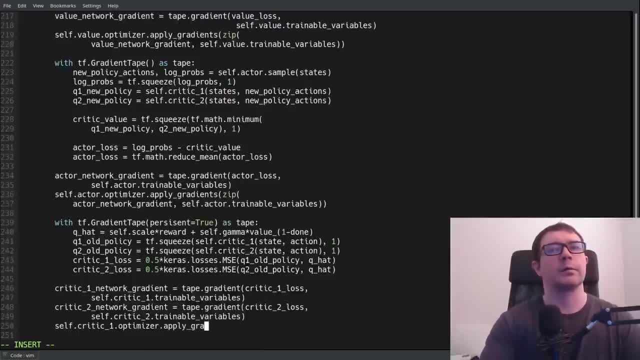 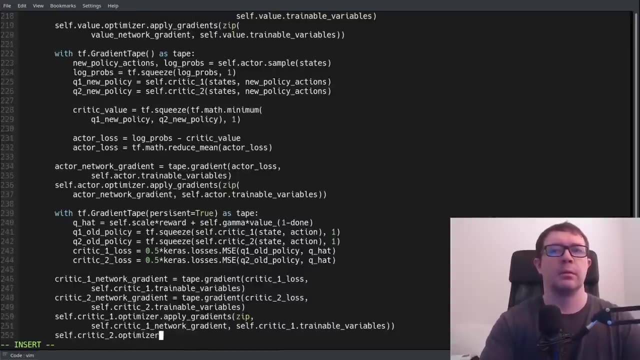 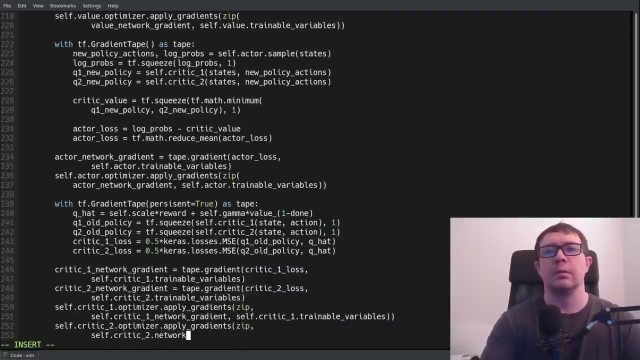 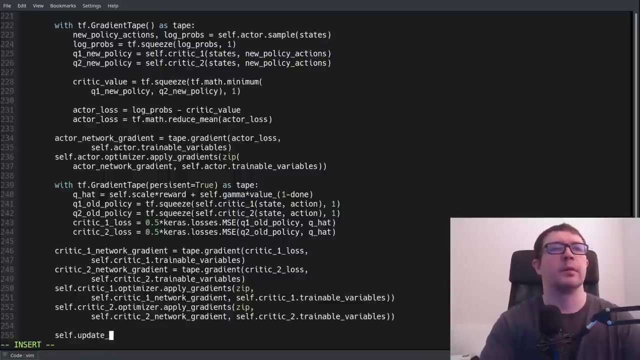 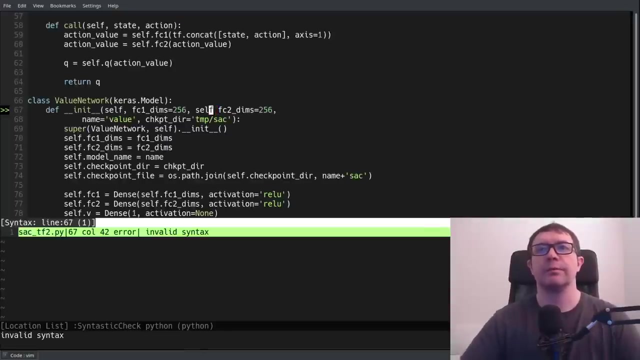 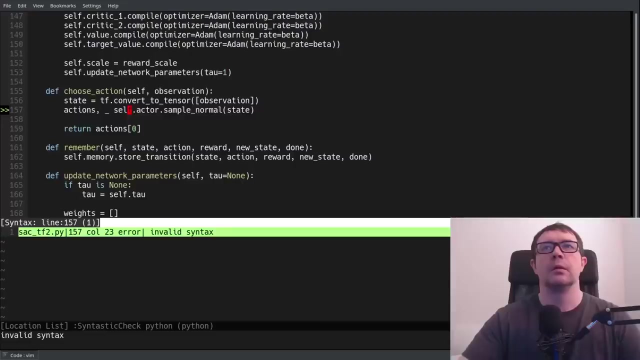 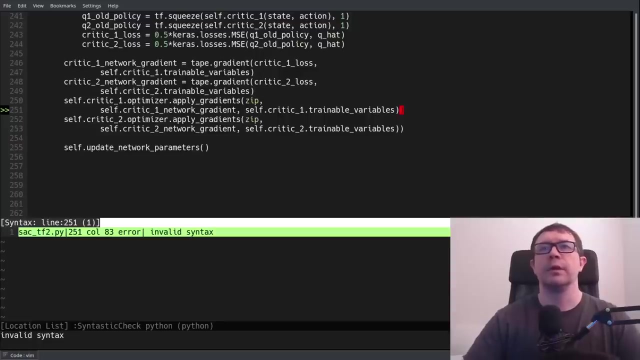 so we want to go ahead and apply our gradients Q, hat value, x. right, there we go. 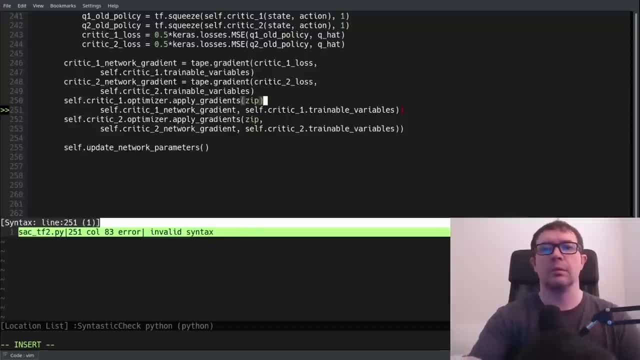 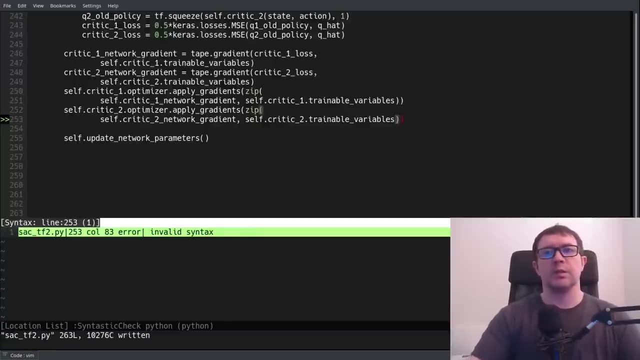 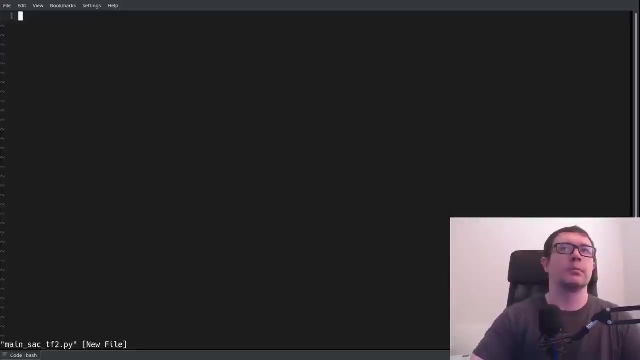 We're going to make our environment inverted: pendulum bullet and v v0.. We need to make our agent. 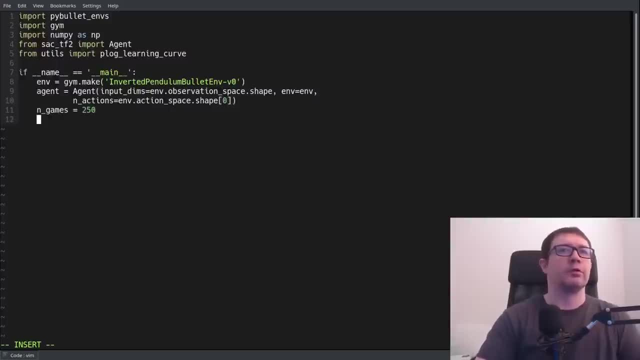 Pass in all of our relevant parameters. We'll play 250 games. Our figure file is just the directory plus the file name. You can condense that into one line if you want, it's not a problem. We say best score and the reward range 0.. 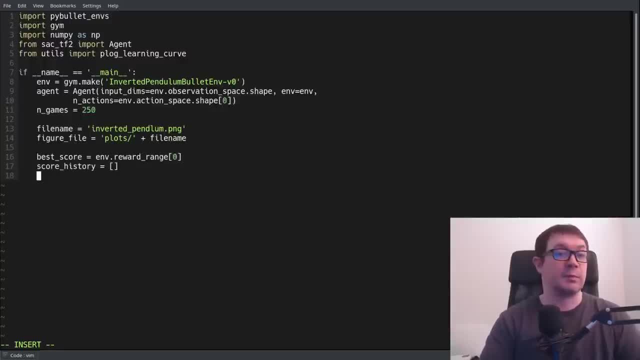 Score history. we want to keep track of the scores the agent receives over time so we can see if it's learning, as well as to plot them later. And a load checkpoint variable which you can set to false if you want to load a checkpoint. 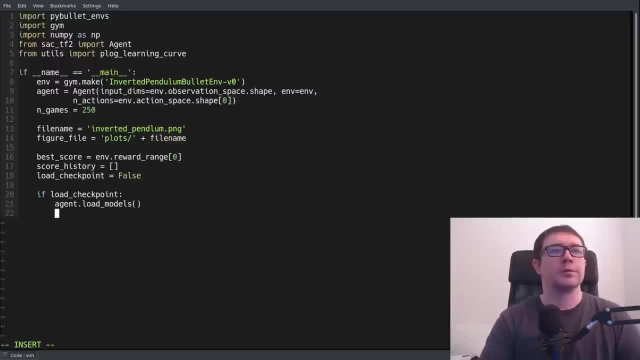 So if we're going to load the checkpoint, I'm going to load your models, And one thing I like to do is set the render mode to human so that way you can see the agent play the game, Because if you're loading a checkpoint, you probably want to. 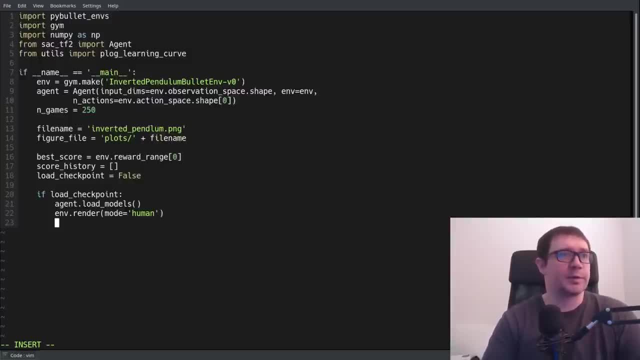 Evaluate the performance, If not just comment out this line. In other words, if you're doing checkpointing so that you can do more training later, then just get rid of that line. No big deal. So let's go ahead and play our games. 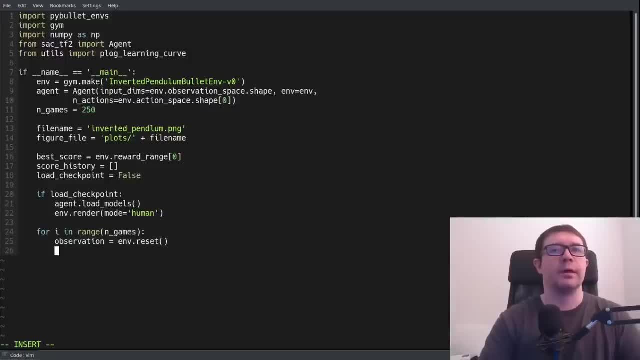 Reset your environment. at the top of every episode, Set your done flag and set your score to zero. Play your episode by choosing an action. Take your action, get the new state reward done and debug info back from the environment. Keep track of your score. 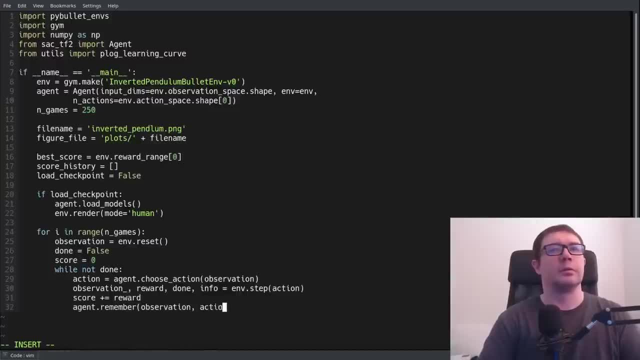 Remember your transition, Not load Checkpoint- Then you want to learn the logic here, being that if you're loading a checkpoint, you're probably evaluating. if it's the case that you're just loading a checkpoint to perform more training later, then you're going to need to put that agent dot learn outside of. 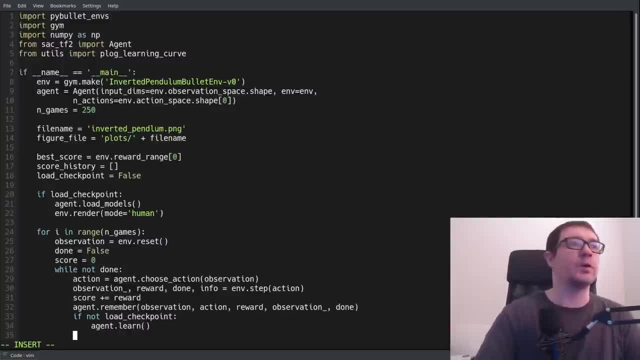 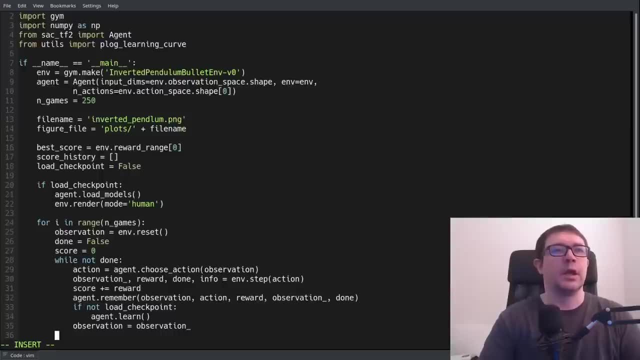 that if statement. Just get rid of the if statement. Okay, So that you're going to do what you actually intend, No matter what. you need to set the current state to the new state And at the end of the episode, you want to append the score to the new state. 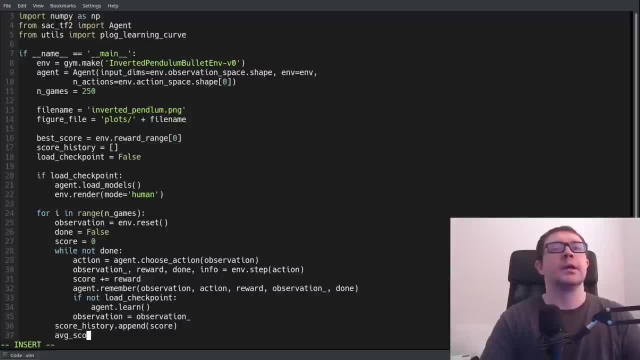 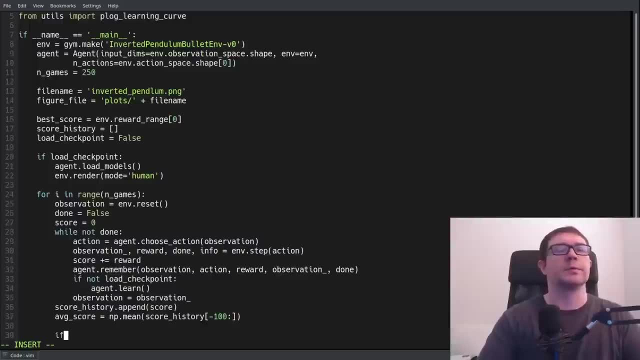 You want to append the score to the new state, So you want to set the score to the score history. Calculate an average of the previous 100 games. If that average score is better than your best score, then set the best score to that. 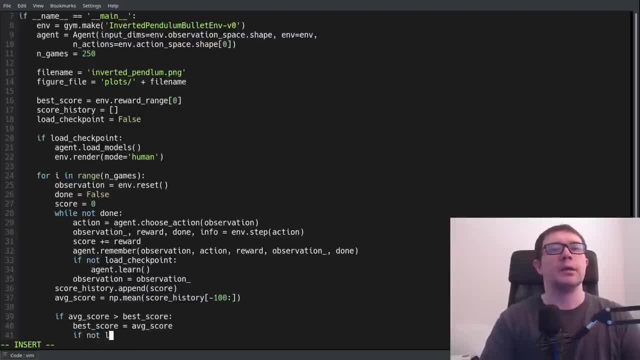 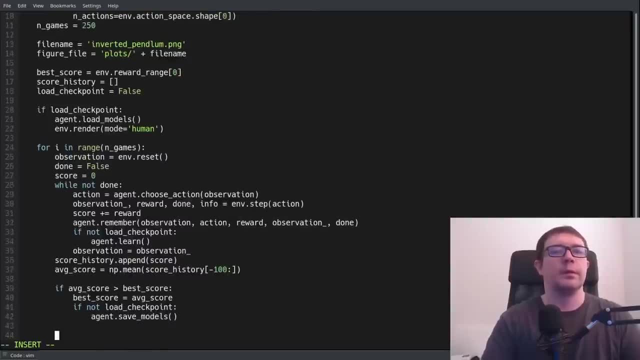 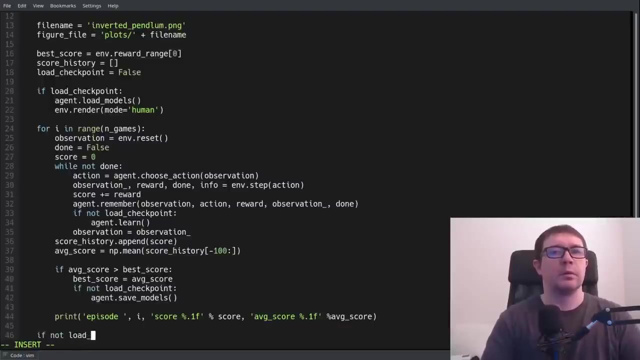 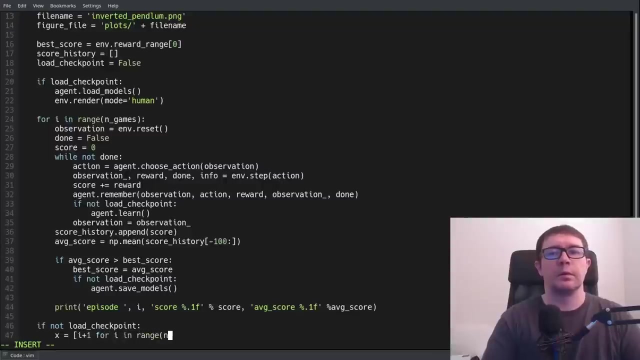 average so that you know you're learning. And again, if not, load checkpoint agent, dot, save models And you want to print episode, The current state, Let's see I score, average, score and then, when all the games are over, go ahead and plot. 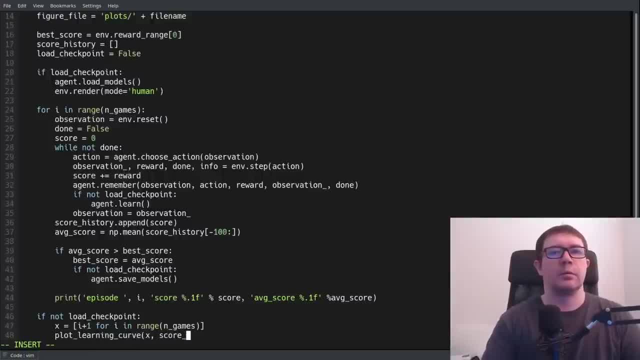 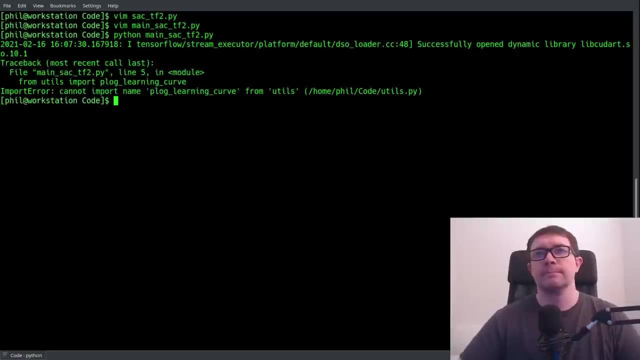 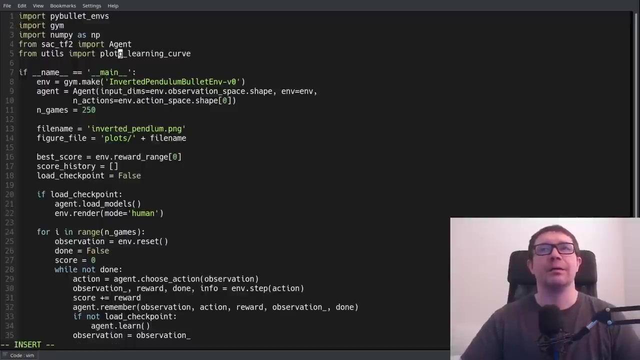 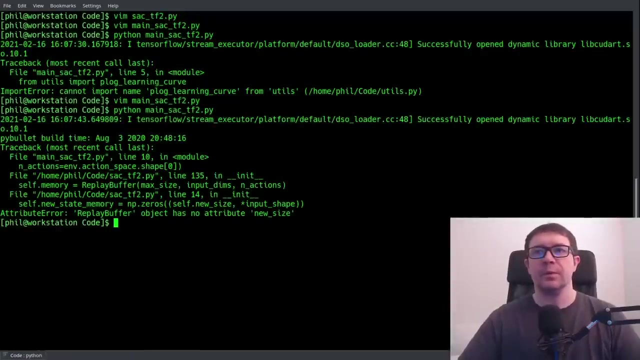 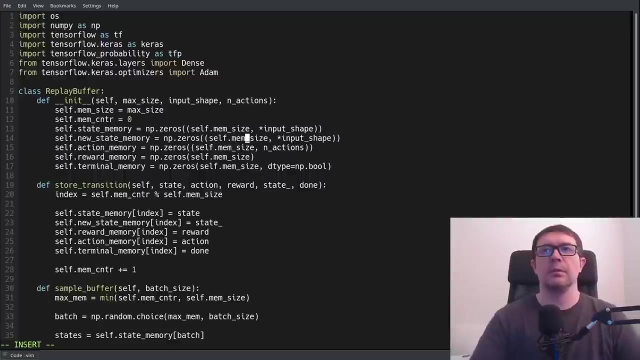 your learning curve. Okay, moment of truth. Let's see how many typos I made. That's easy. Plog Replay buffer has attribute newSize. It should be memSize, selfnewSize. I didn't do that elsewhere. I don't think. 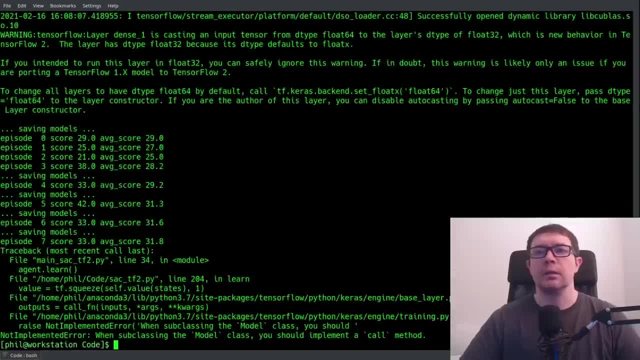 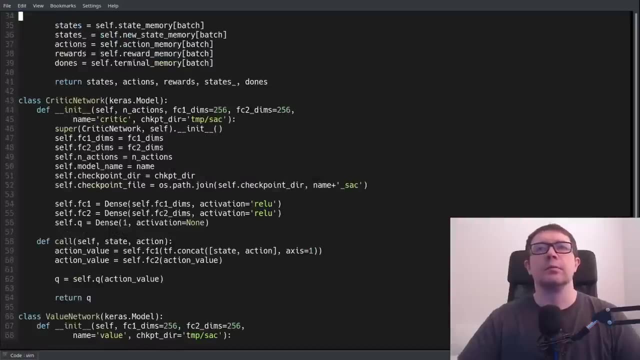 Okay did I not call it call. Okay did I not call it call. Okay did I not call it call. That is interesting. So that is for my value network. Okay, replay buffer critic and value network. 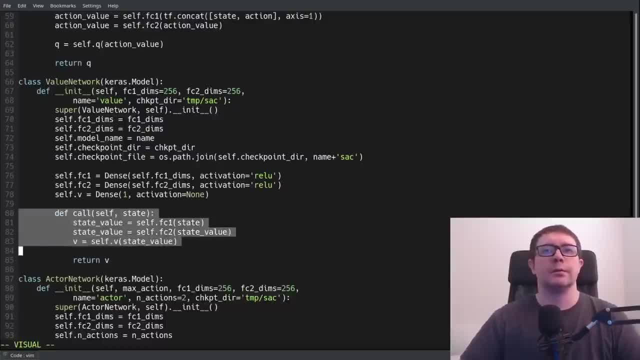 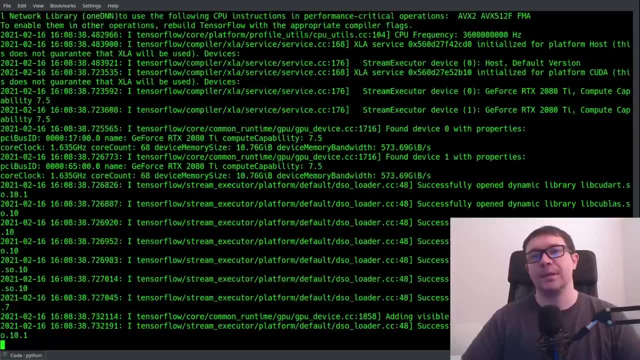 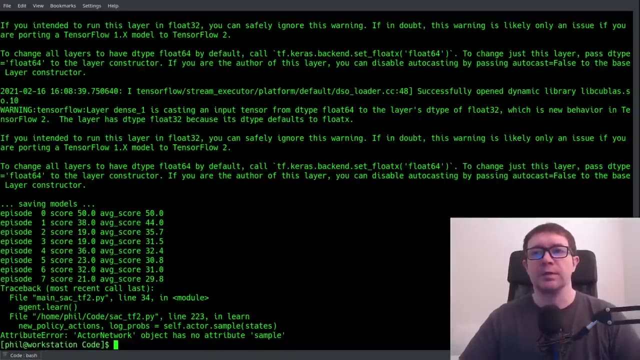 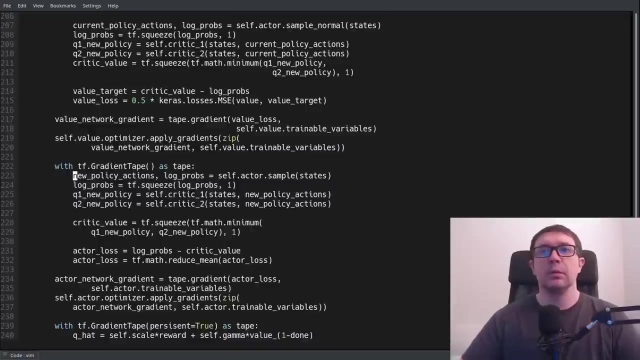 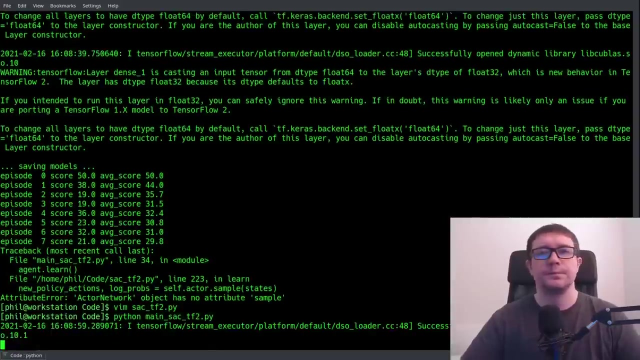 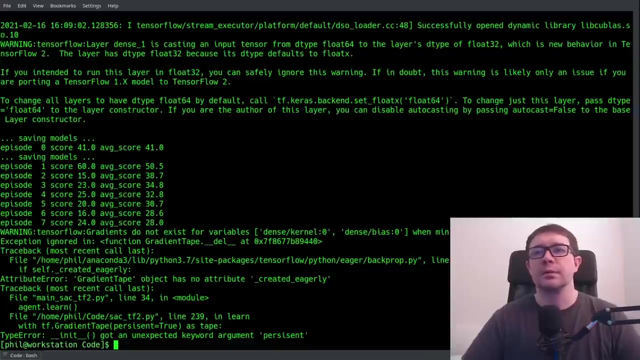 Oh, There we go. Sorry about that. Indentation error Has no attribute sample. That's because it is sample normal. That is in line 223.. Agent does sample normal Persistent Because I forgot a T. That is in line 239.. 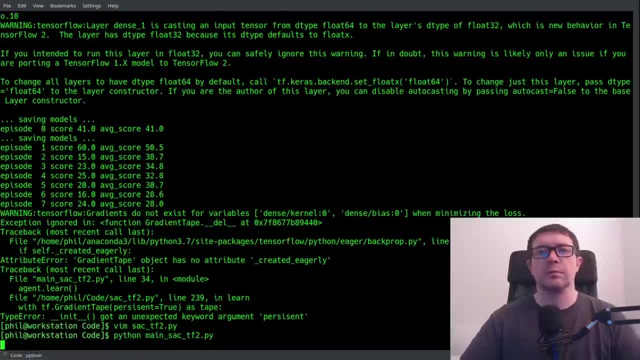 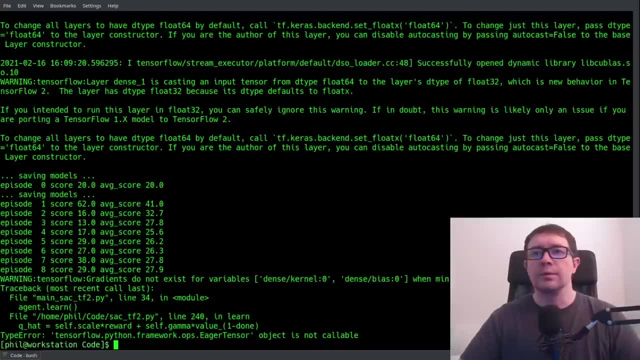 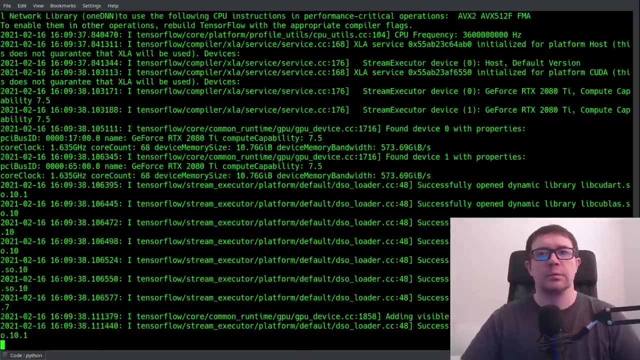 Persistent Equals. true, That's another typo. Perfect Eager ops is not callable. Let's see Selfgamma times value underscore. Oh, I'm missing a multiplication sign. That is in line 240.. Sorry about that, Okay. 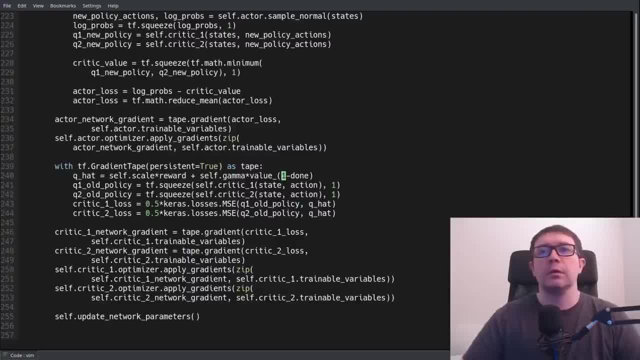 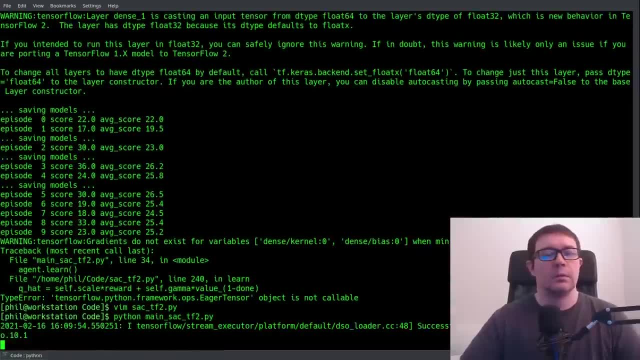 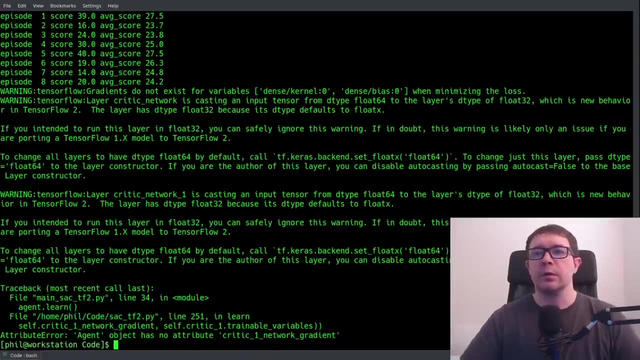 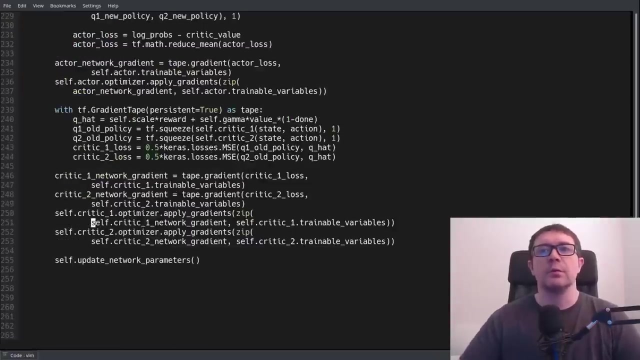 Line 240.. One minus done, Good grief, Critic. one underscore: That is in line 251.. Oh, because it's not. There's no self in there. Okay, Good grief, There is no self there, Yep, Okay. 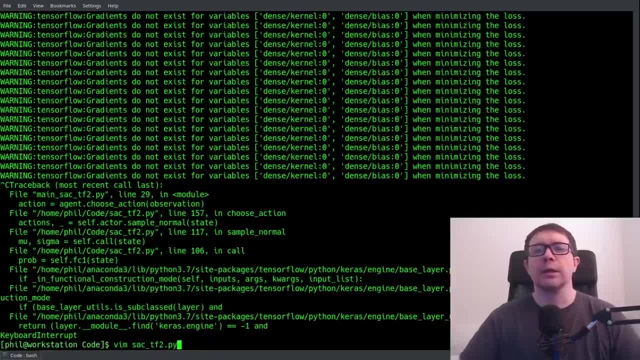 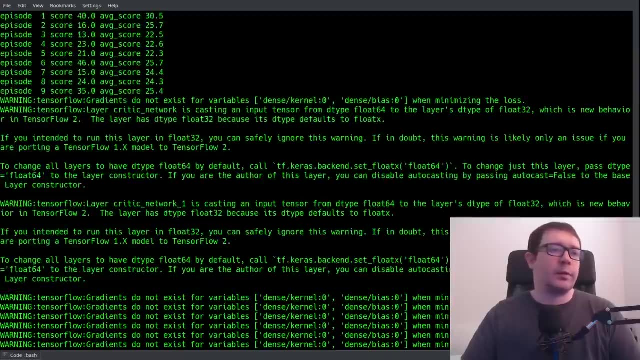 Gradients do not exist for one of my layers. Okay, Okay, It means I have forgotten something. indeed, That's problematic because it doesn't tell me. Well, these warnings here, don't worry about those, Those aren't a problem. 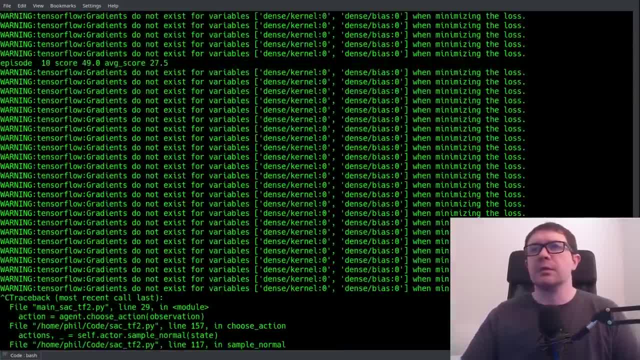 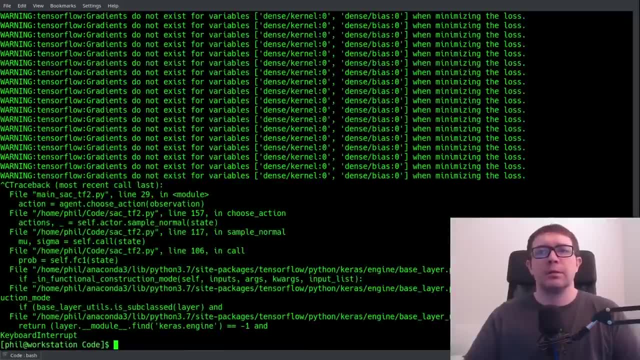 This grading does not exist is in fact a problem. So let me see. I don't even know which network it is talking about there. It doesn't tell me. It says dense kernel zero. So that's probably whichever network I uh made first. 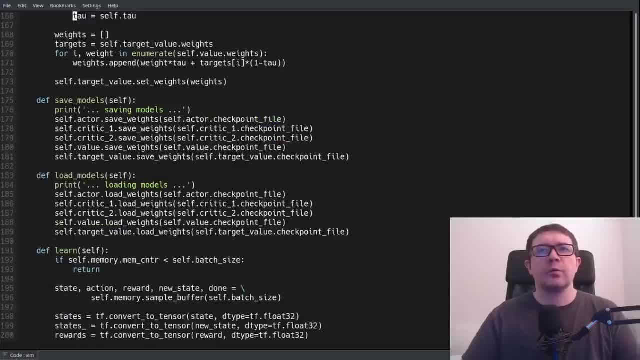 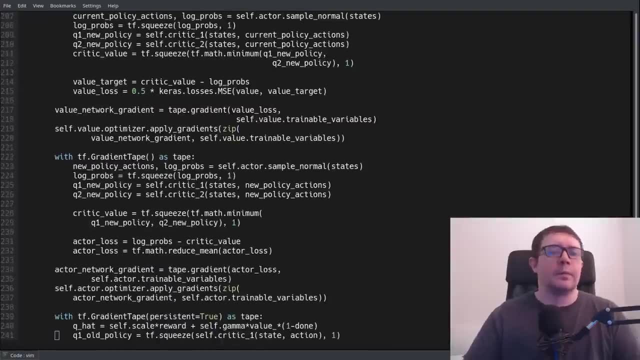 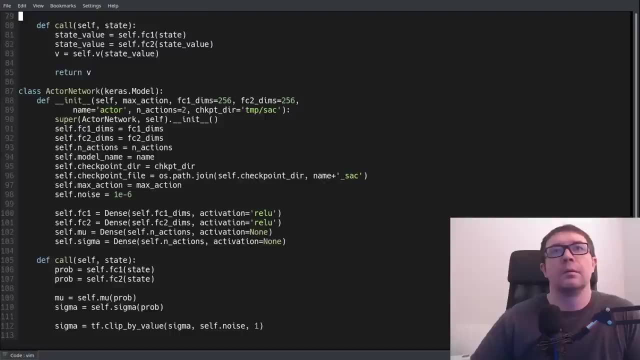 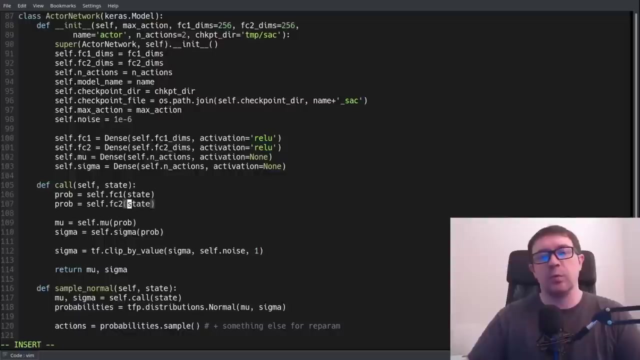 So I instantiate my actor network first. So here is value: actor loss. Hmm, Let's check out our handy dandy cheat sheet here. And so I have located the source of the issue and I will annotate this when I edit the video. But uh, the issue here is that I was passing the state through both the 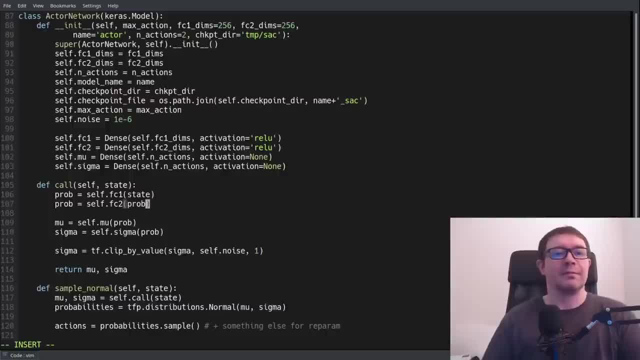 first fully connected and second fully connected layer, instead of allowing the output of the first fully connected layer to feed into the second layer. So, of course, that's how deep neural networks work, and you won't get uh anything useful if you don't um feed things through properly. 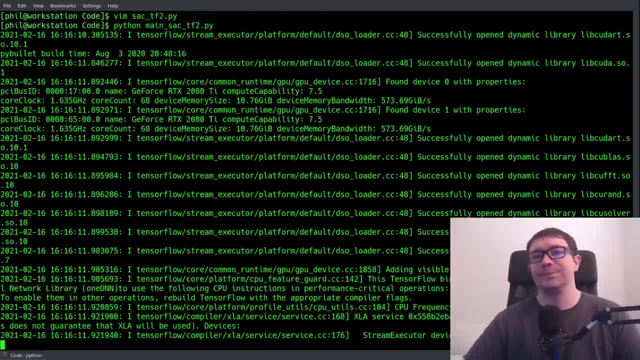 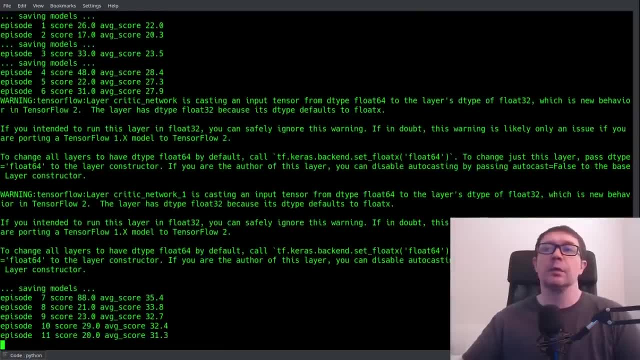 So let's go ahead and try it again. Okay, So now we've got the same warning, and that's not concerning Uh, it just has to do with, uh, the precision, Um. so that's something you can, um, deal with on your own. 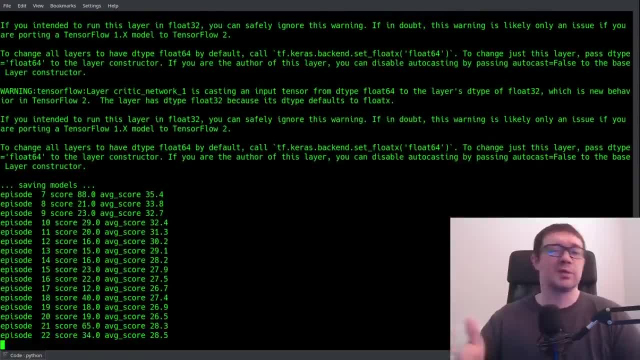 If you want, I'm not going to go changing the backend settings. Uh, I could suppress the warning, but it doesn't really bother me that much, So I'm going to come back in a few minutes and make sure that this is learning. 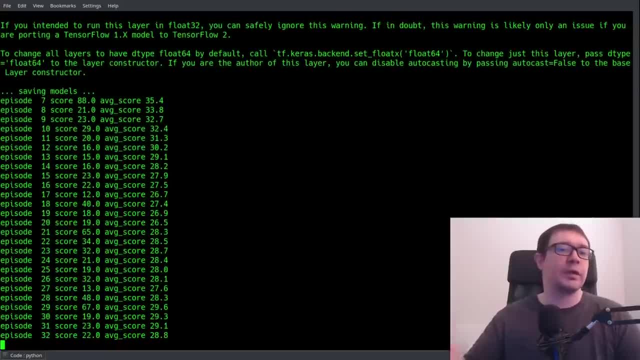 And when I do, I'll go ahead and show you the output of a fully trained network. And if it doesn't learn, then I'm going to go back and debug it And you'll know, because I'll tell you in a few minutes from your perspective. 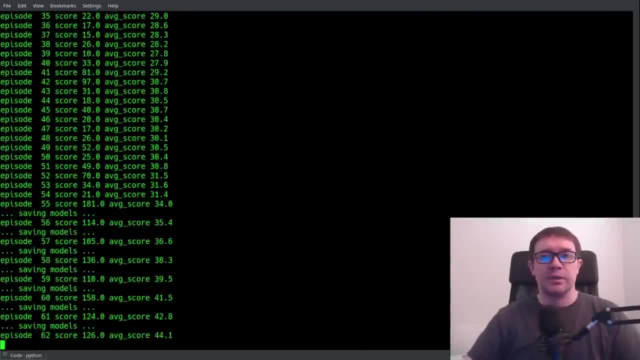 Okay. So here we are, And it's just a few Okay. A few minutes later, by game 60,, we can see that the average score is improving with each episode, meaning that it is in fact learning and it's getting well over a hundred. 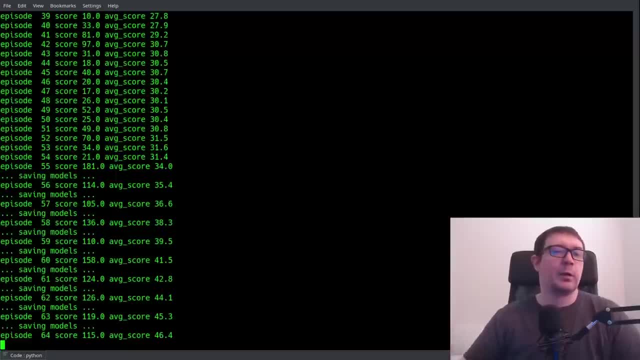 And so I'm going to switch to the other terminal where I have finished running it. I'm not going to wait for it to play all 250 games, Cause it does take quite a while once it gets closer to a thousand steps. So hold on one moment. 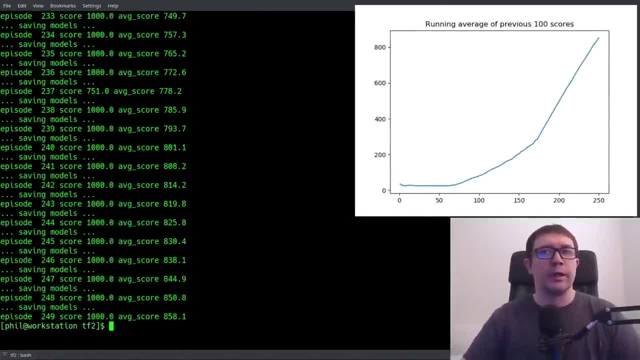 So here is the output of an earlier model I trained- and I'm just checking the other window to make sure it is indeed still learning and it is it's saving models pretty much with every game. So this is an output of a model I ran earlier, where you can see that for the last several games it gets a. 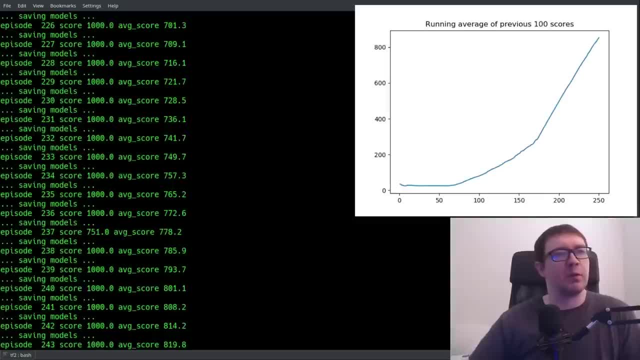 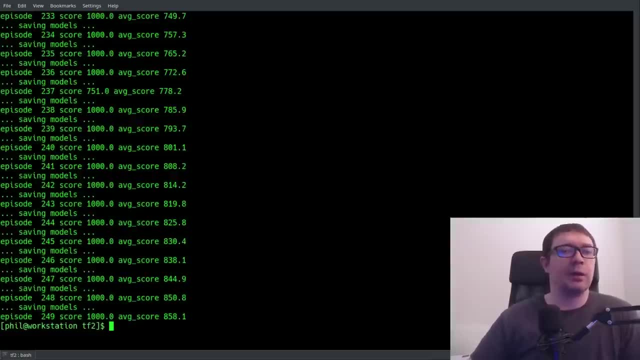 consistent score of a thousand, with a little bit of a low flyer here at seven: 51, still a respectable score. It doesn't have a hundred games of a thousand, So the average score hasn't hit a thousand, but it is trending well up on its way. 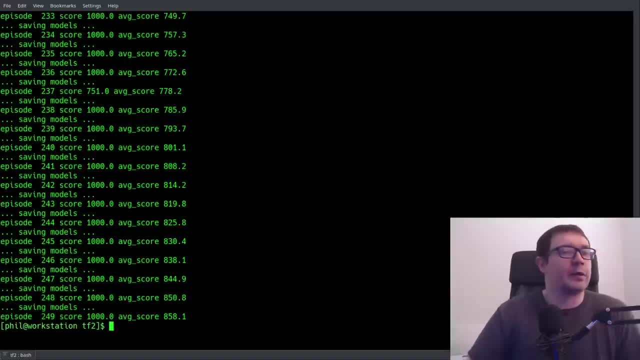 So I consider that to be a fully trained model. If it ran another 50 games, a hundred games, then the average score would be a hundred and we would have beaten the average score. So that is some after critic. in TensorFlow two, I left out the re-parameterization because I don't think it's entirely necessary. 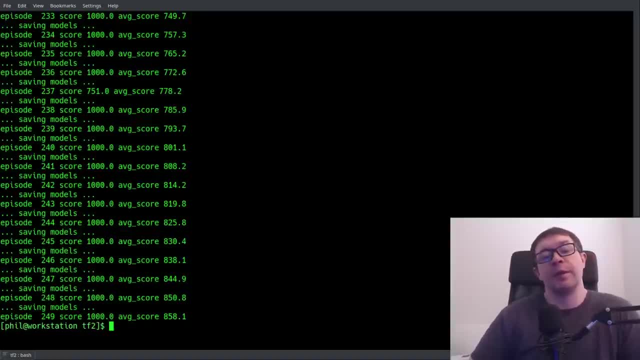 I don't know why it was put in the original paper. I have implemented it in PyTorch. You can see that video If you want to see how that works. it's just passing in a parameter to your sample function And if that parameter is true, then you use the our sample instead of the sample function from your distribution. 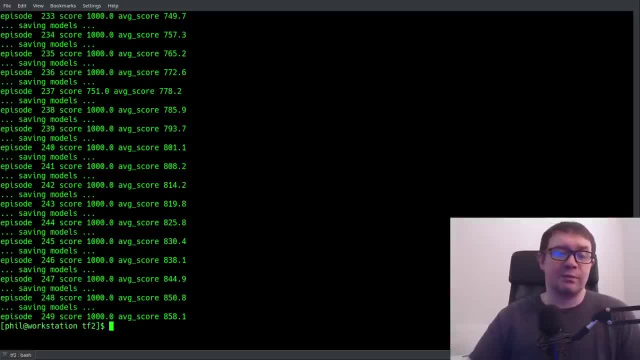 If you want to implement that intensive load, to leave that as an exercise to the viewer. But You would have to do some simple calculation of adding in some spherically sampled noise to it. So that's not. you know, it's not particularly difficult. 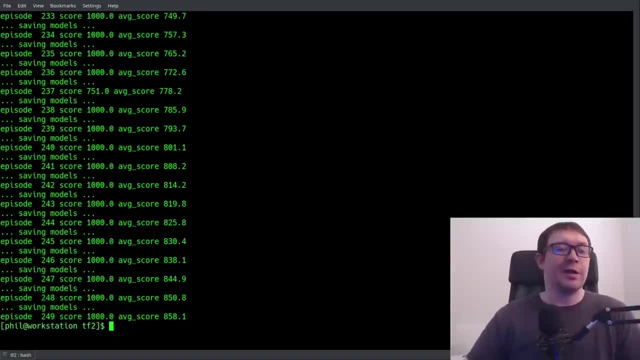 It's just something I didn't want to bother with. So this agent learn that is solved after critic in TensorFlow two, an incredibly powerful algorithm, indeed state of the art. I prefer TD three. I think it tends to perform a little bit better, but this is certainly no slouch in and of itself. 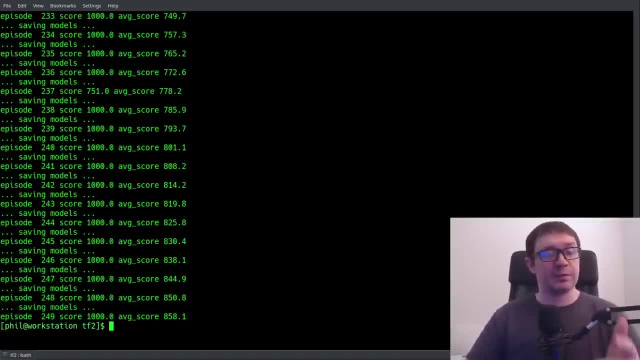 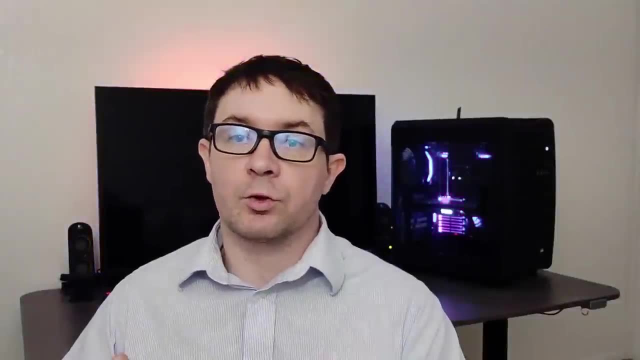 I hope that was helpful. Leave a comment, a question, a subscribe- certainly, if you've made it this far, and I will see you in the next video. If you give me about 45 minutes of your time, I will show you how to code a fully functional asynchronous advantage, actor, critic, agent in the PyTorch framework. 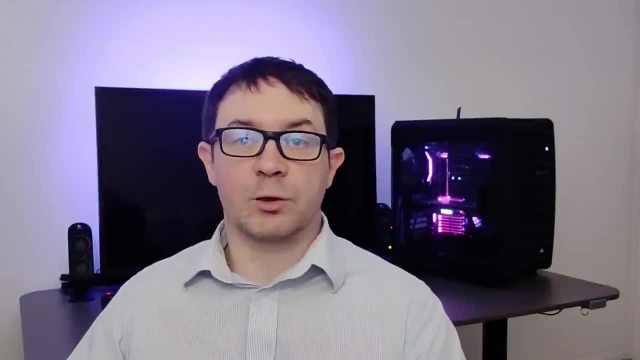 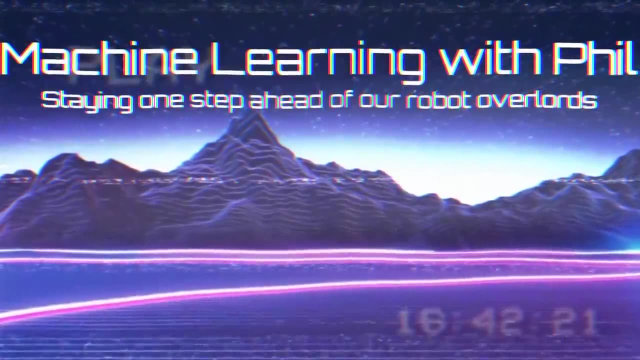 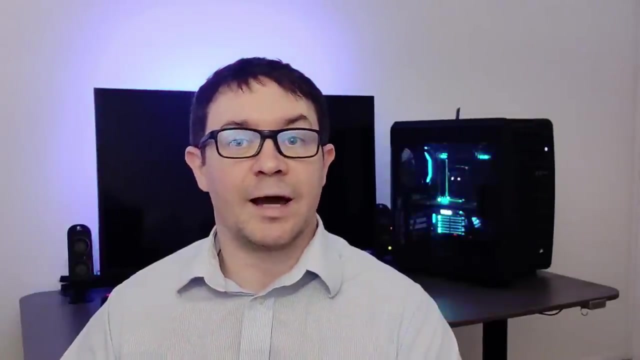 Starting from scratch. we're going to have about 10 to 15 minutes of lecture, followed by an about 30 minute interactive coding tutorial. Let's get started Really quick. If you're the type of person that likes to read content, I have an associated blog post where I'm going to go into much more detail. 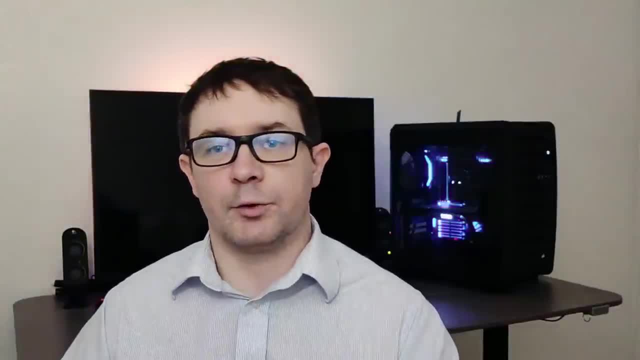 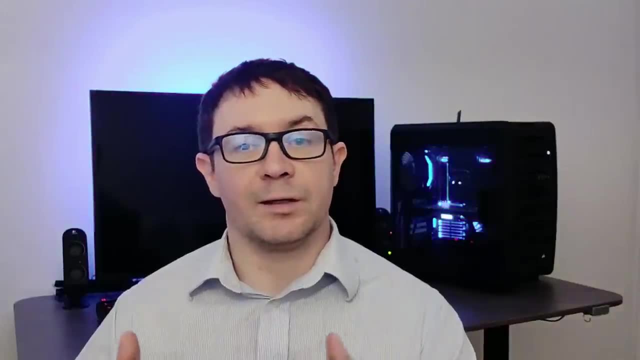 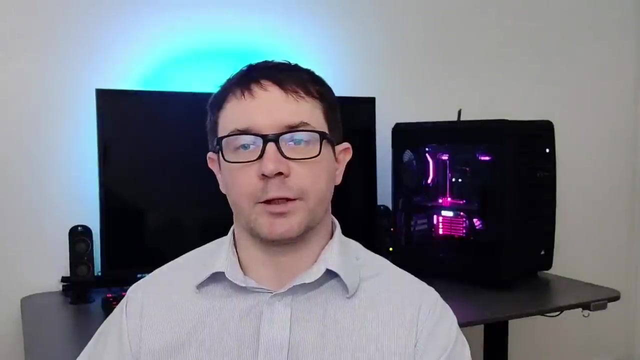 Check the link in the description. Deep reinforcement learning really exploded in 2015 with the development of the deep Q learning algorithm. One of the main innovations in this algorithm that helped it to achieve such popularity is the use of a replay buffer. The replay buffer solves a very fundamental problem in deep reinforcement learning. 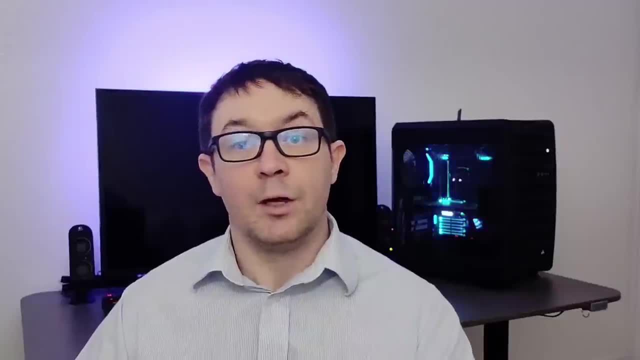 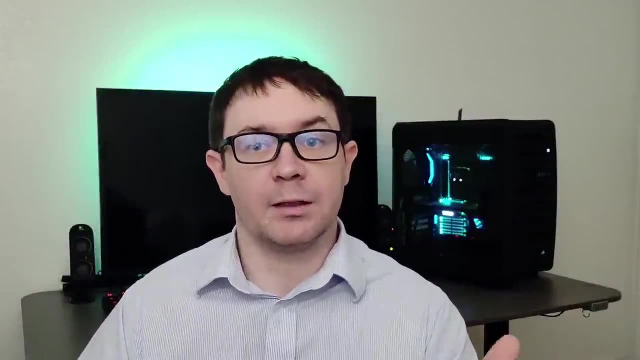 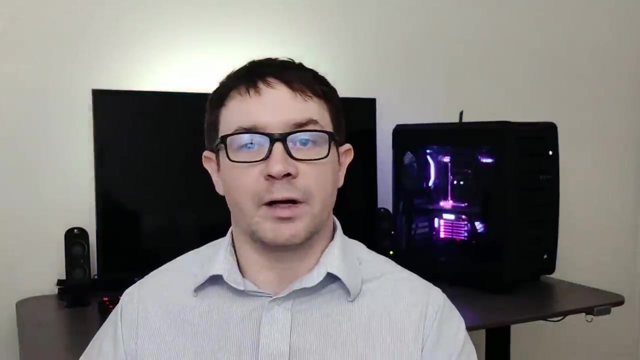 And that problem is that neural networks tend to produce garbage output when their inputs are correlated. What could be more correlated than an agent playing a game where each time step depends on the one taken immediately before it? These Correlations cause the agent to exhibit very strange behaviors, where it will know how to play the game and suddenly forget when it encounters some new set of states that it's never seen before. 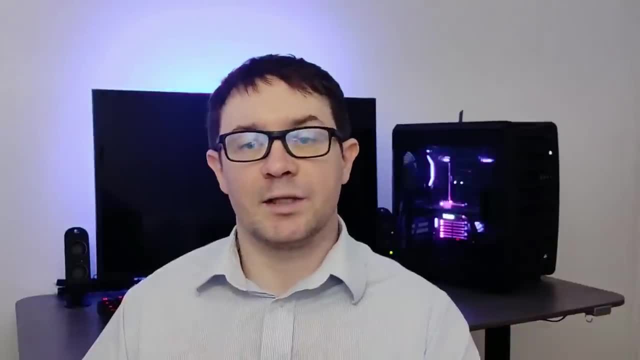 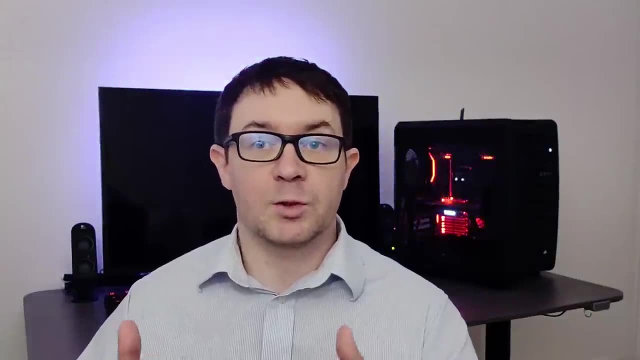 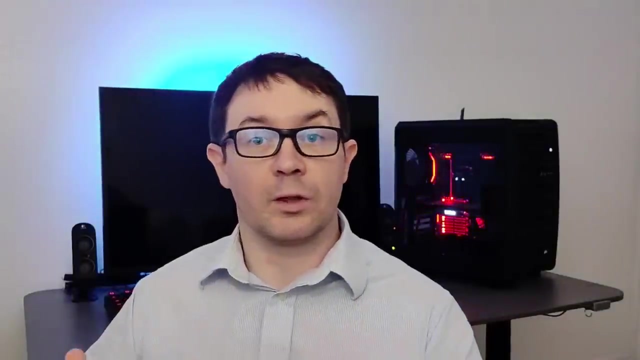 The neural network really isn't able to generalize from previously seen states to unseen states due to the complexity of the parameter space of the underlying problems. The replay buffer fixes this problem by allowing the agent to randomly sample agents from many, many different episodes. This guarantees that those time steps taken are totally uncorrelated. 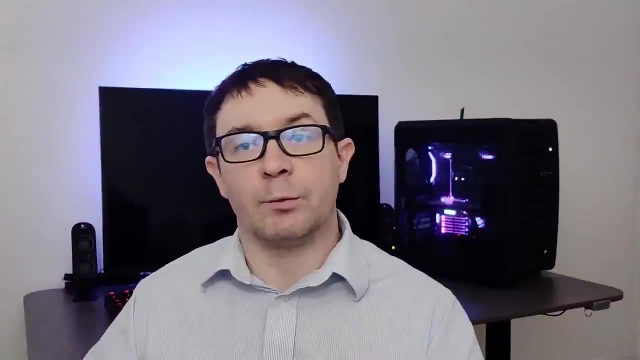 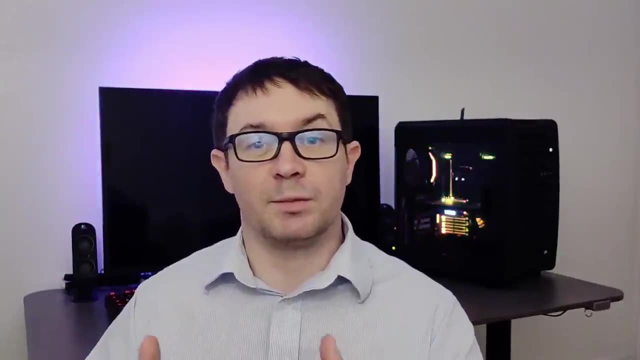 And so the agent gets a broad sampling and parameter space And is therefore able to learn a more robust policy with respect to new inputs. As I've shown before on this channel, problems arise when you attempt to simply bolt on a replay buffer onto the actor critic algorithm. 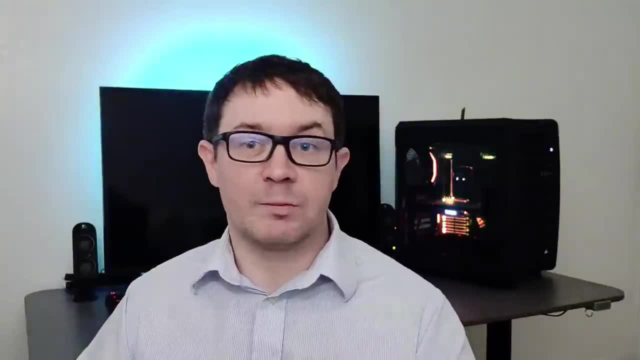 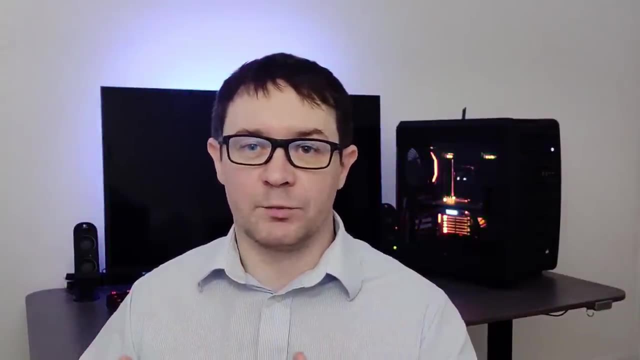 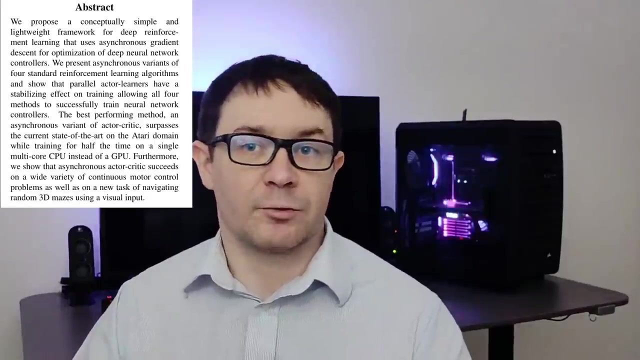 It doesn't really seem to work, And in fact, it's not very robust after critic methods in particular suffer from being especially brittle, And so adding on a replay buffer really doesn't help to address that problem. In 2016,, a group of researchers managed to solve this problem using something called asynchronous deep 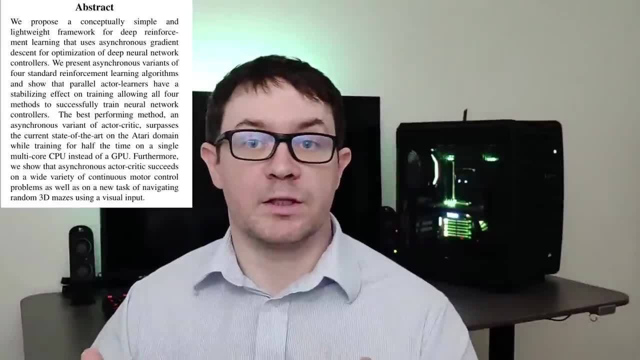 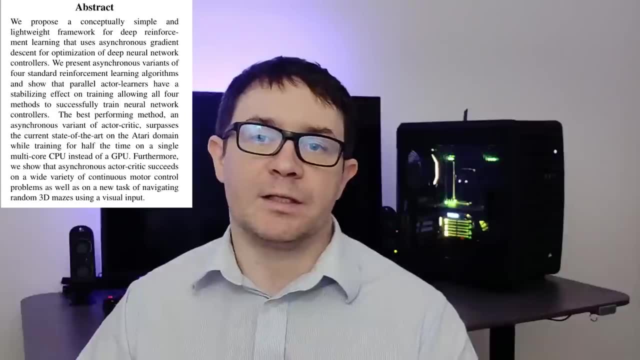 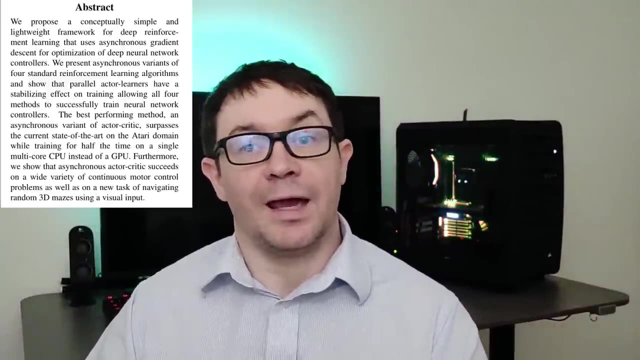 Reinforcement learning. It's a totally different paradigm for approaching the deep reinforcement learning problem And in fact the technology can be applied to a wide variety of algorithms. In the original paper they detail solutions for deep Q learning and step Sarsa- excuse me- and step Q learning, as well as Sarsa and actor critic methods as well. 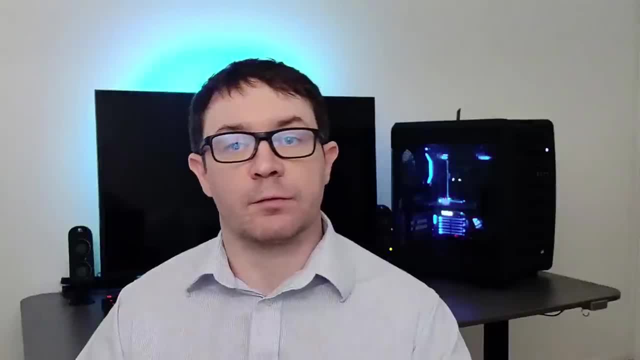 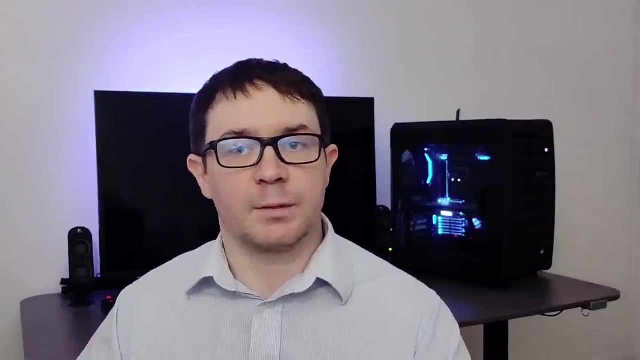 So what is this big innovation? Well, instead of having a replay buffer, we're going to allow a large number of agents to play independently on totally separate and self-contained environments. Each These environments will live on a CPU thread, in contrast to a GPU for most deep Q learning applications. 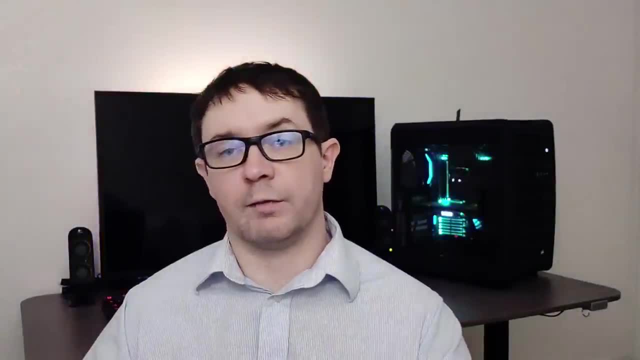 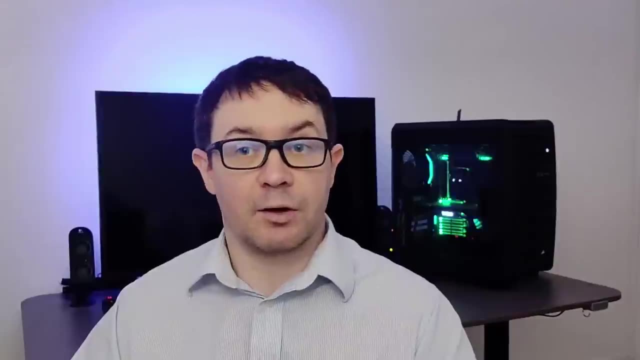 This has the additional benefit that if we don't use a replay buffer, we don't have to store a million transitions, which for trivial environments really doesn't matter. But if you're dealing with something like, say, the Atari library, a million transitions can take up a significant amount of Ram, which can be a limiting factor for enthusiasts. 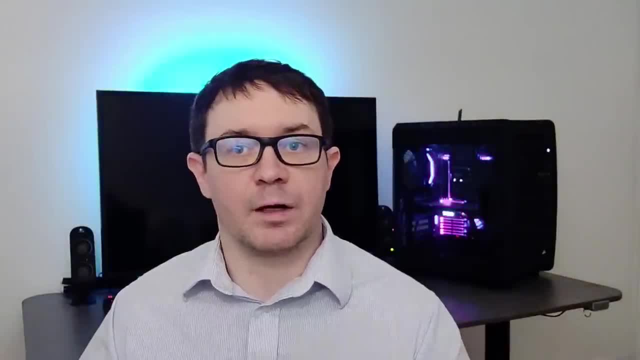 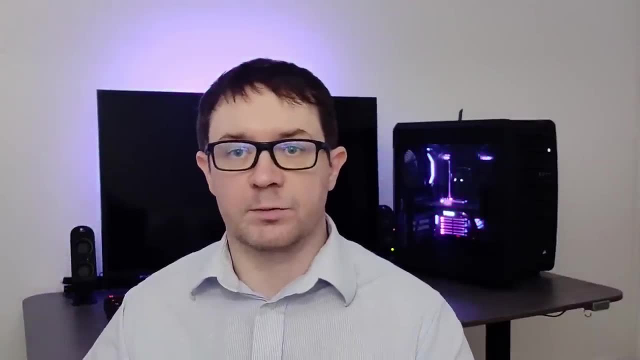 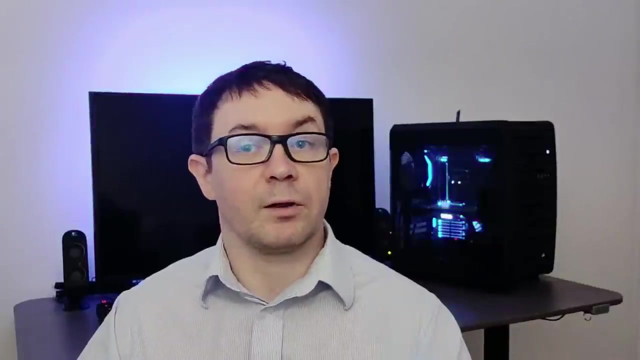 So having the agent play a bunch of different games in parallel on separate environments, only keeping track of a small number of transitions vastly reduces the memory footprint required for deep reinforcement learning. So in what sense exactly is this algorithm asynchronous? What this means exactly in this context is that we're going to have a large number of parallel CPU threads with agents playing in their own environments. 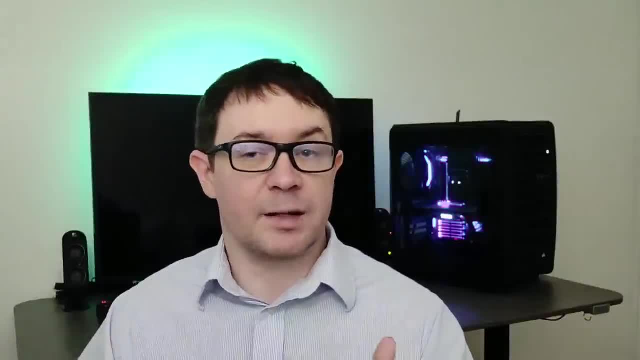 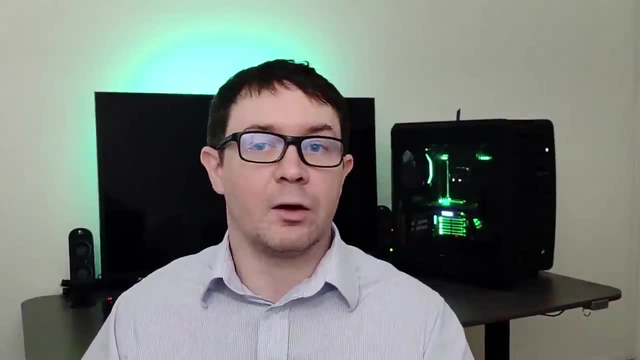 They're going to be acting at the same time, but at various times they're going to be deciding what to do, as well as updating their deep neural network parameters, And so we're not going to have any one agent sitting around waiting on another agent to finish playing the game to update its own set of deep neural network. 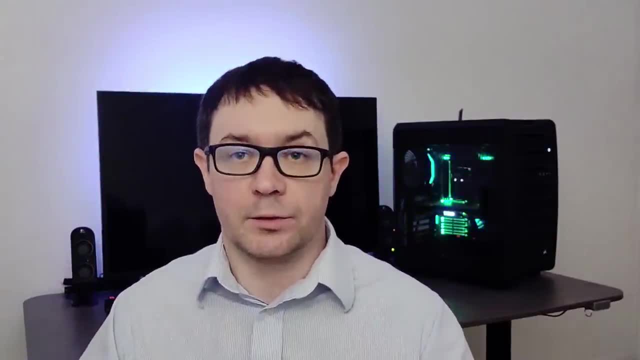 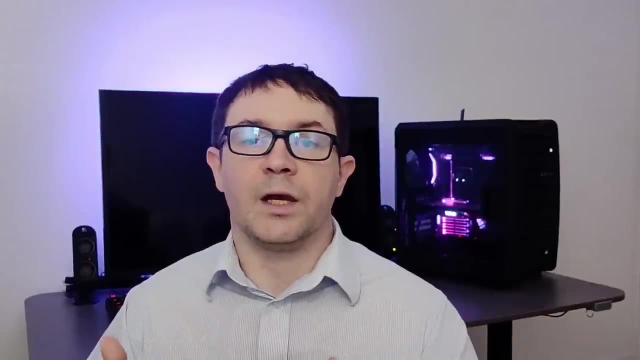 parameters, Okay, Okay, Each one will be totally independent and learning on its own. Now, we're not going to be simply throwing away the learning from each agent after it finishes the episode. Rather, we're going to be updating the network parameters of some global optimizer as well as some global actor critic agent. 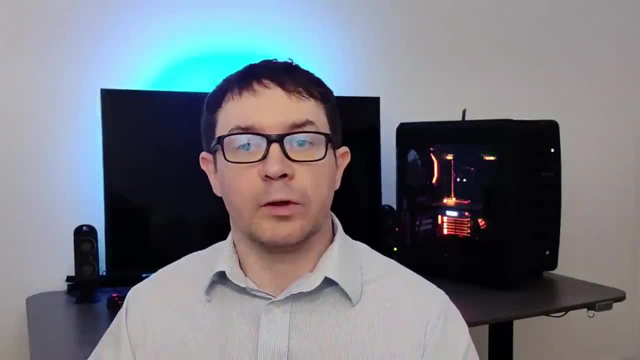 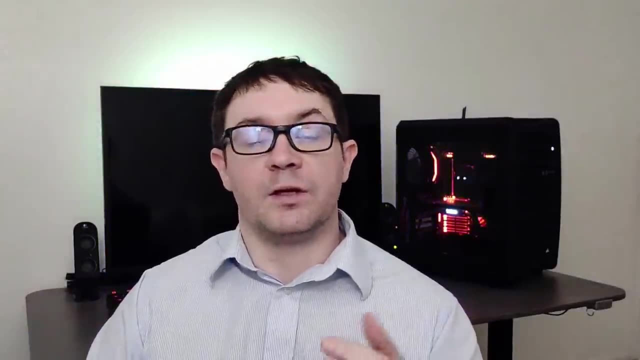 So you have one actor, critic agent that sits atop all of the others and the local agents that do all the learning by interacting with their environments. So what is the advantage? part of A3C. So the advantage essentially means what is the relative advantage of one stage. 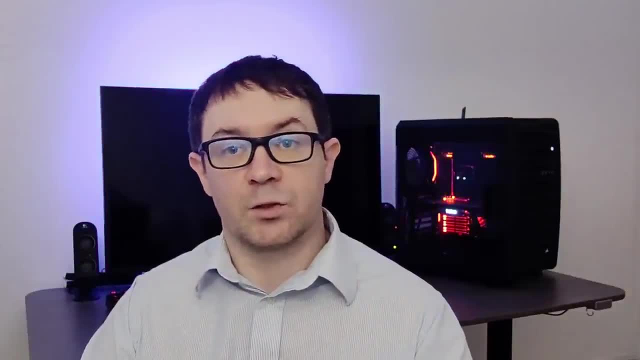 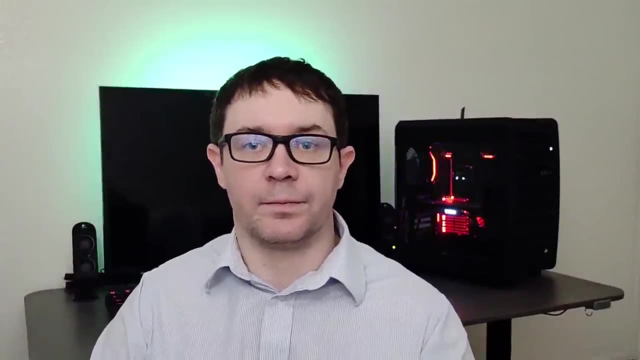 So the advantage is that you can take a state over another. It stands to reason that an agent can maximize its total score over time by seeking out those states which are most advantageous or have the highest expected future return. The paper gives a relatively straightforward calculation for this. 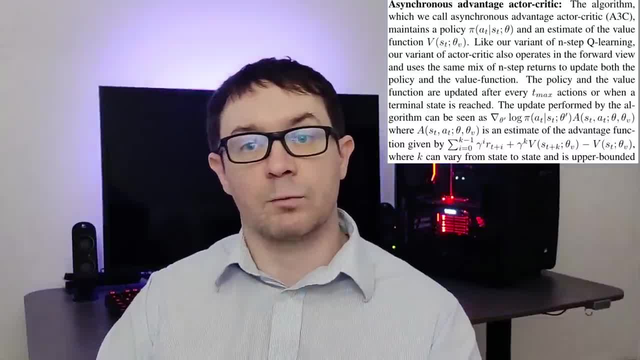 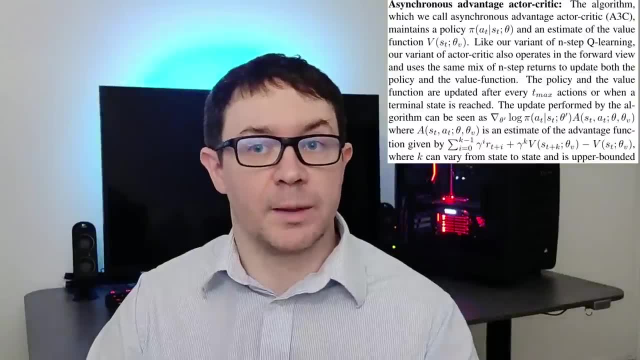 All we have to do is take the discounted sum of the rewards received over some fixed length trajectory and then add on an appropriately discounted value estimate for the final state the agent saw in that trajectory. Please note that this could be some fixed number, like, say, five steps. 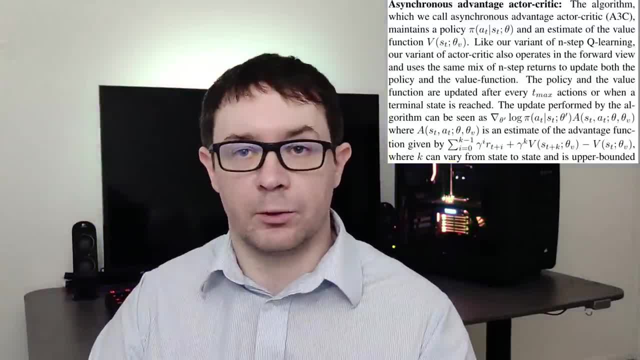 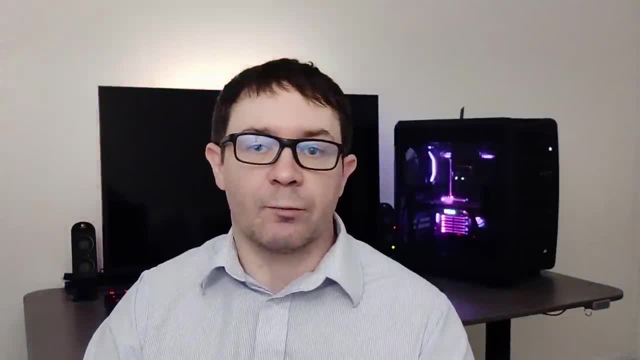 This could be three steps. if the agent encountered a terminal state along the way, We're then going to go ahead and subtract off the agent's estimate of the value of whatever current time step it's in in the trajectory. So that way we're always taking the value of the next state minus the current state. 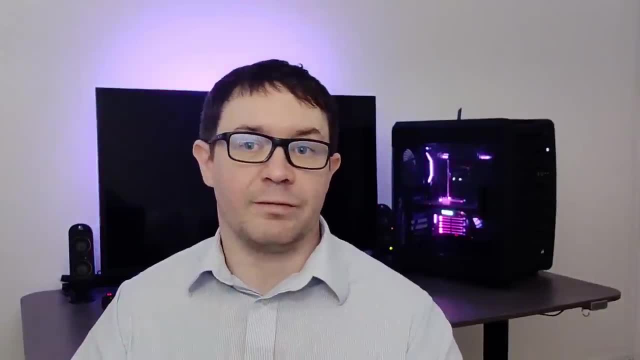 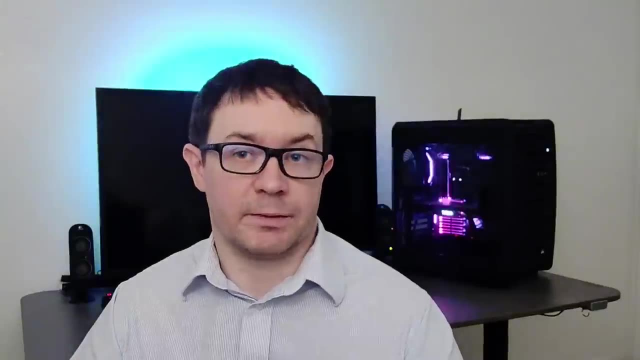 That's what gives us the relative advantage. So what does the actor critic portion of A3C mean Specifically? this refers to a class of algorithms that use two separate neural networks to do two separate things. So the actor network is responsible for telling the agent how to act. 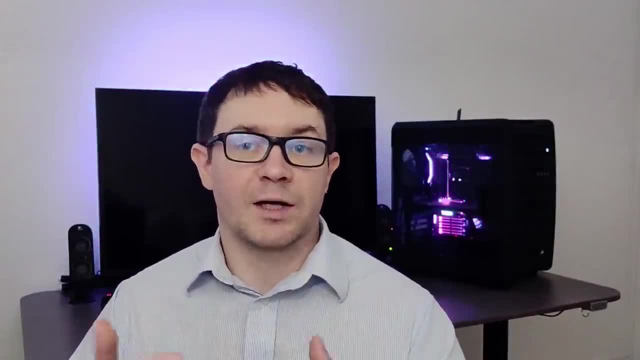 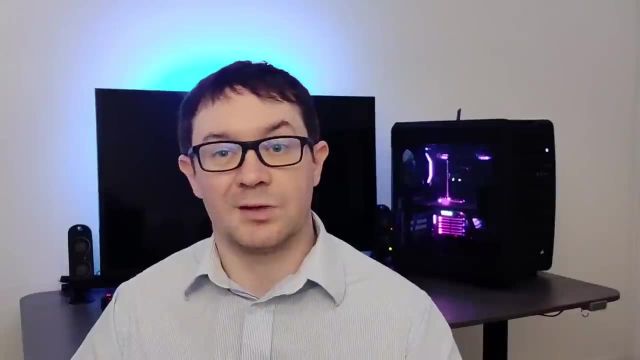 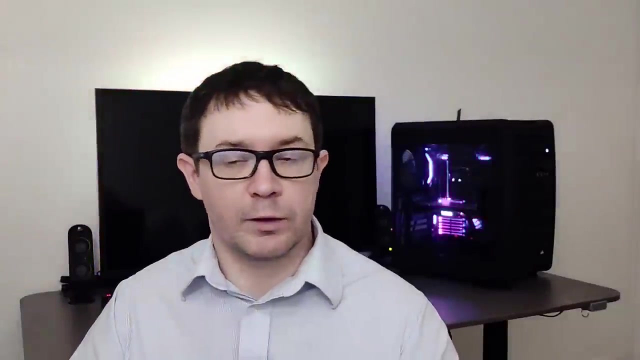 Kind of like this Kind of a clever name. right, It does this by approximating a mathematical function known as the policy. The policy is just the probability of selecting any of the available actions for the agent, given it's in some state, And so for a discrete action space, it's going to be a relative probability of selecting one action over another. 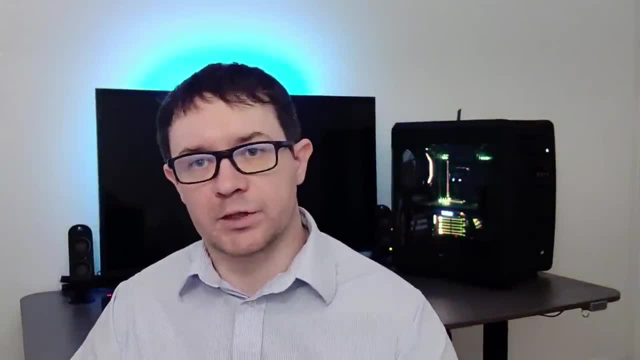 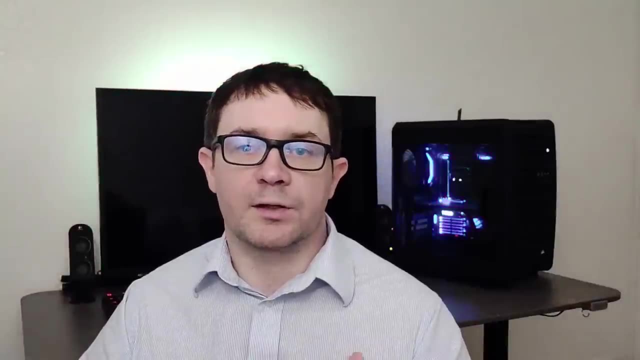 So in our cart poll it's going to be say, 60% move left, 40% move right, so on and so forth. We're going to facilitate this by having two separate networks. The actor network will take a state or set of states as input. 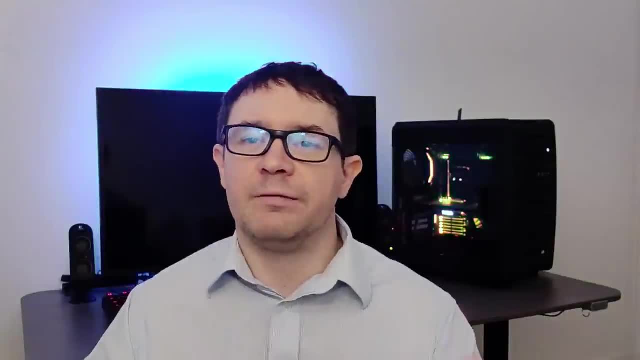 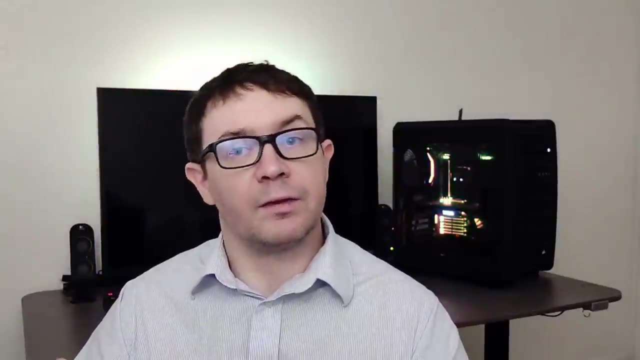 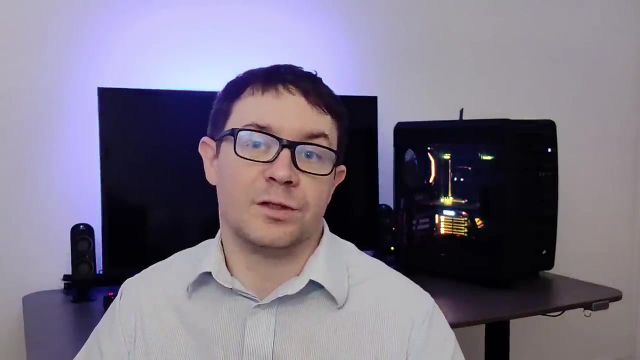 And output a softmax probability distribution that we're going to be feeding into a categorical distribution from the PyTorch framework. We can then sample that categorical distribution to get the actual action for our agent And we can also use that to calculate the log of the probability of selecting that action according to the distribution. probability distribution. 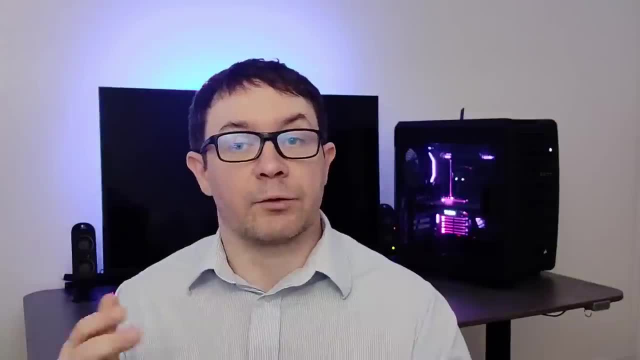 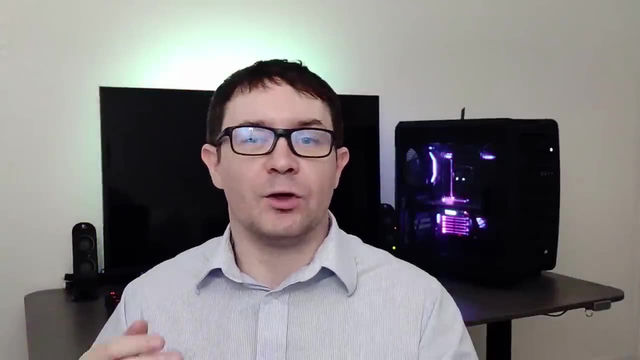 And we will use that for the update rule for our actor. Now the critic has a little bit of a different role. The critic essentially criticizes what the agent, the actor, did. It said: you know that action you took gave us a pretty lousy state that doesn't have a very large expected future return. 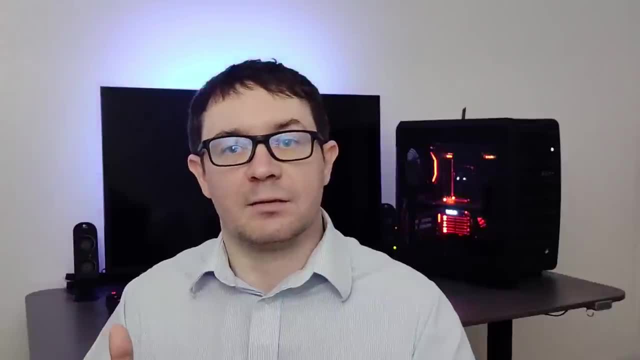 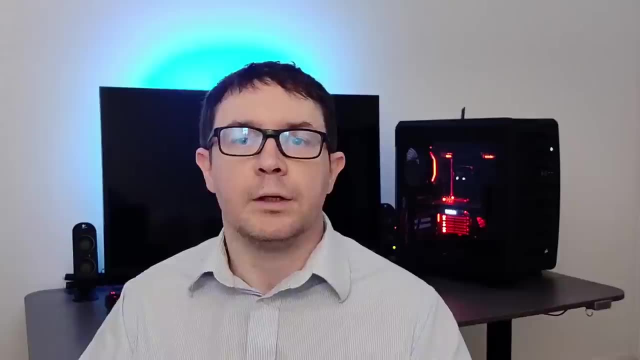 And so we shouldn't really try to take that action, given that state, any other time that we encounter it. So the critic essentially criticizes what the actor does And the two kind of play off of each other to access more and more advantageous states over time. 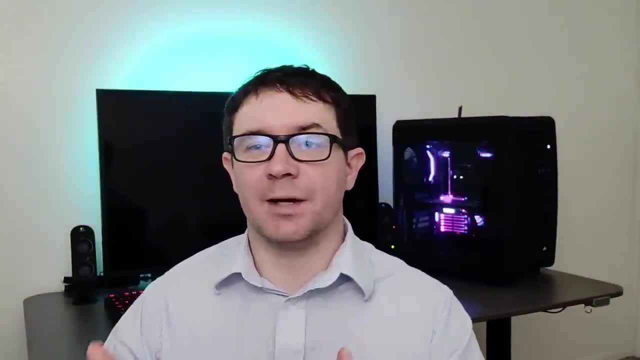 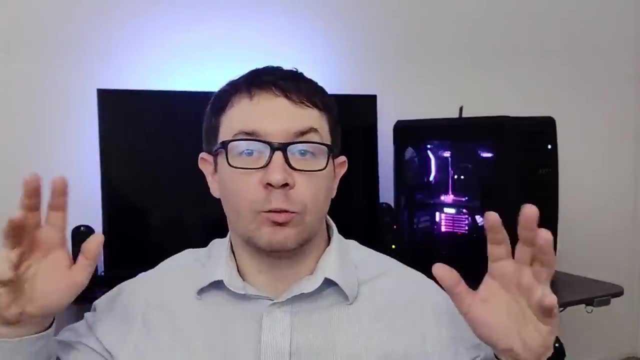 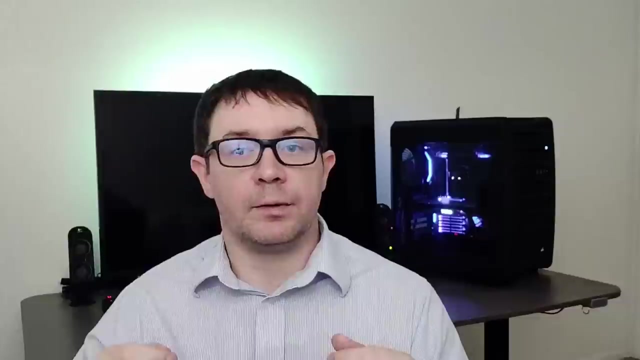 Before we go ahead and talk about the specifics of each class, let's get some idea of the general structure and flow of the program. The basic idea is that we're going to have something like this: We're going to have some global optimizer and global actor critic agent that sits on top that keeps track of everything the local agents learn in their own individual threads. 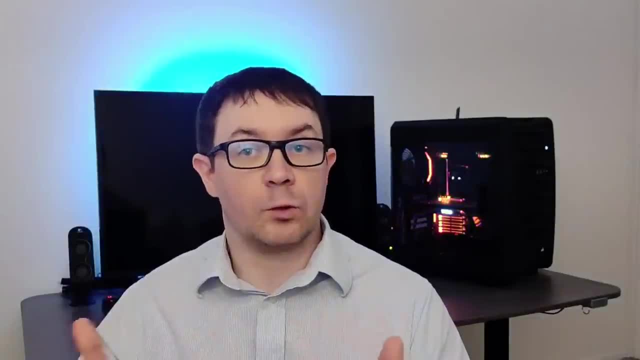 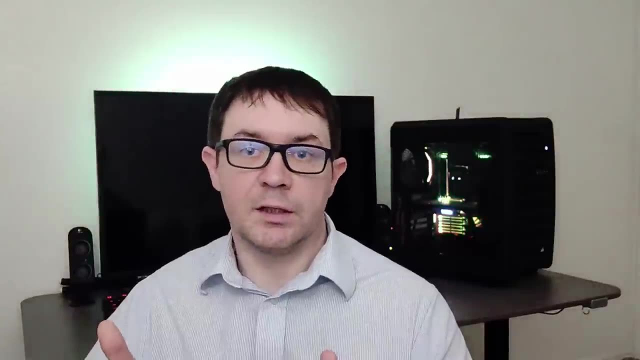 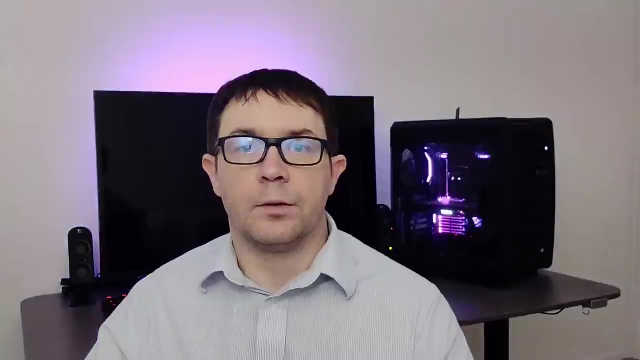 Each agent will get its own specific thread where it can interact with its own totally distinct and separate environment. The agent will play either some fixed number of time steps or until it encounters a terminal state, at which point it will perform the loss calculation to do the gradient descent on the global optimizer. 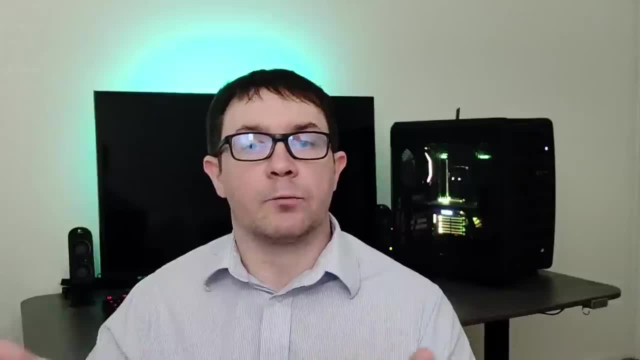 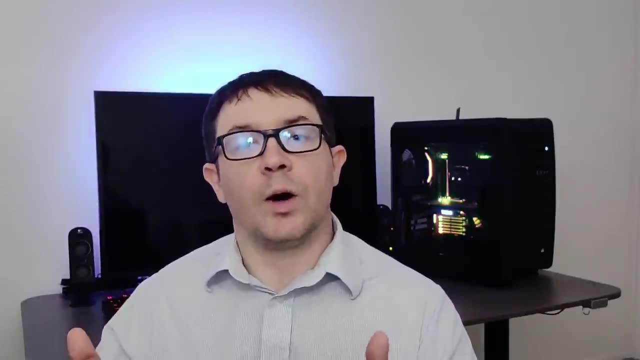 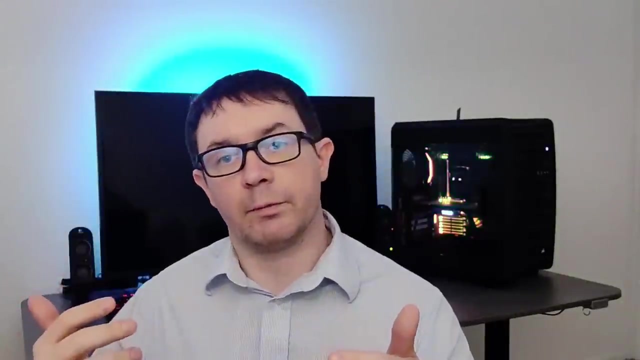 Once it calculates those gradients, it's going to upload it to the global optimizer And then redownload the parameters from that global optimizer. Now keep in mind each agent is going to be doing this asynchronously, So while one agent is performing its loss calculations, another agent may have already finished that loss calculation and updated the global optimizer. 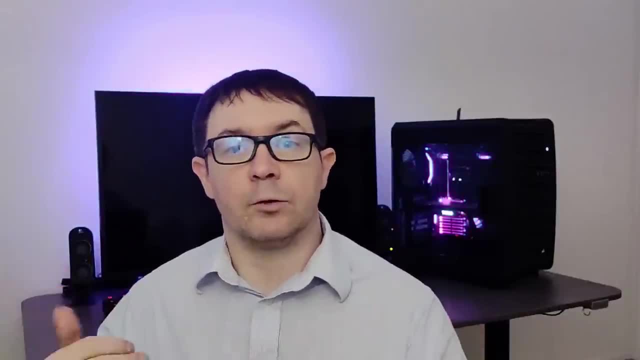 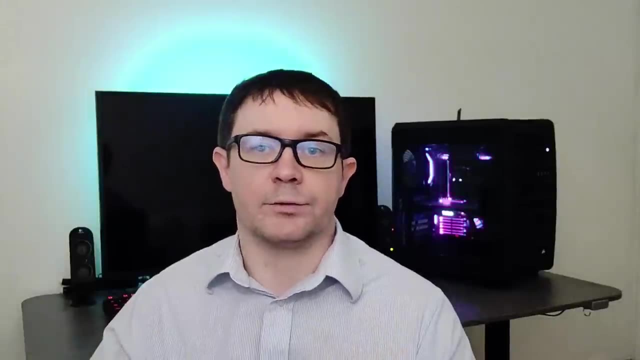 That's why, right after calculating the gradients, we want to go ahead and download the global parameters from the global actor critic, So that way we make sure we are always operating with the most up-to-date parameters After each time the agent performs an update to its deep neural network. 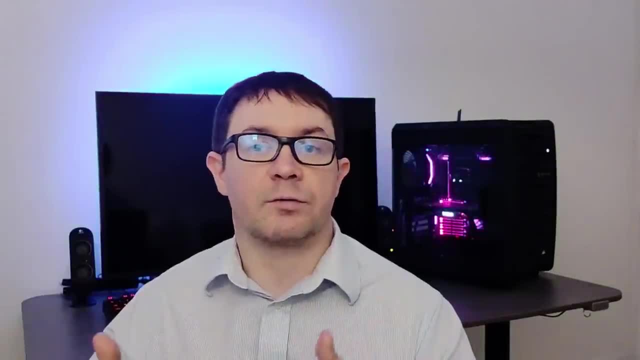 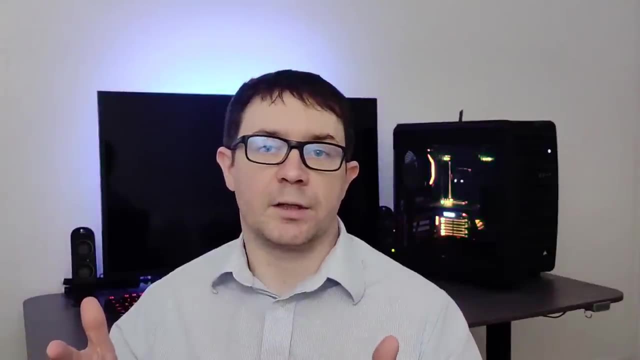 we're going to want to go ahead and zero out its memory so that it can start fresh for another sequence of five or until it encounters a terminal state number of steps. So now let's talk implementation details. We're going to have a few separate, distinct classes for this. 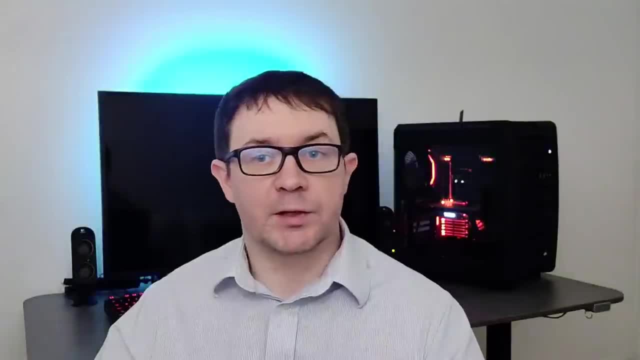 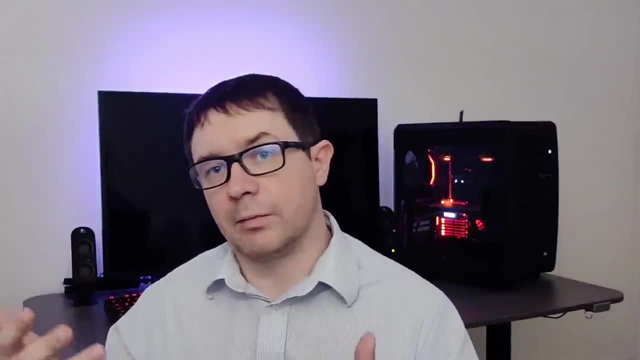 The first of which is going to be overriding the atom optimizer from the base PyTorch package. So we're going to have a shared atom class that derives from the base TorchOptimAtom class, And this will have the simple functionality of telling PyTorch that we want to share the parameters. 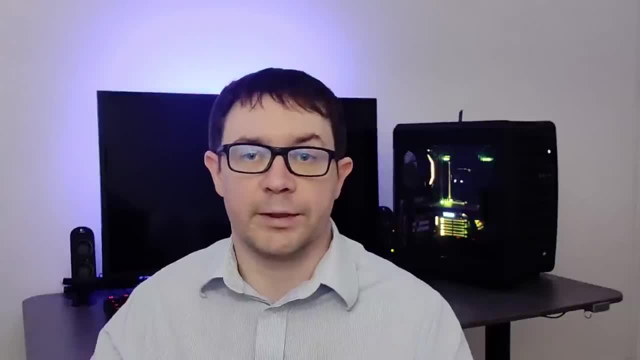 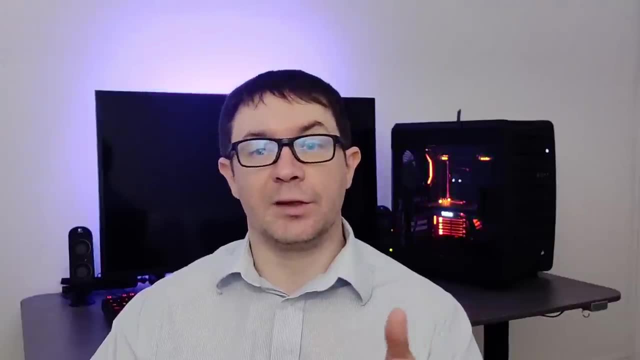 of a global optimizer among a pool of threads. It's only going to be a few lines long and it's much easier than it sounds, And I'll show you how to do it in code. Our next class will be the actor critic network. 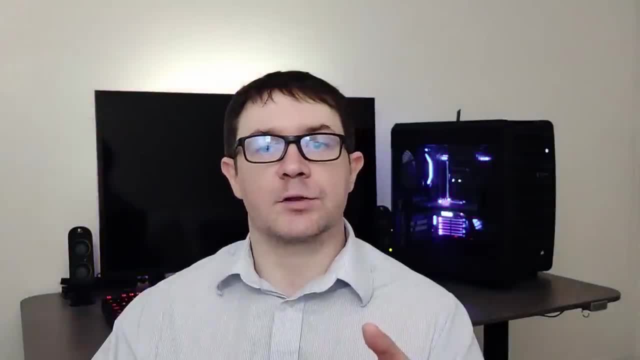 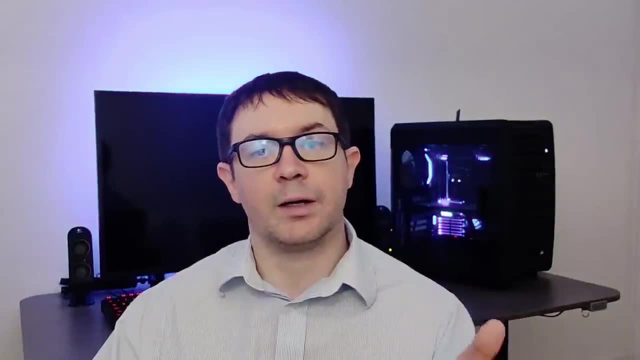 Now, typically we would use shared input layers between an actor and a critic, where we simply have one input layer and two outputs corresponding to the probability distribution pi and the value network v. But in this case we're going to host two totally separate, distinct networks within one class. 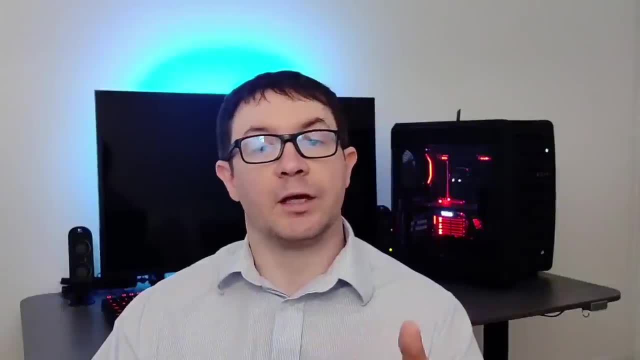 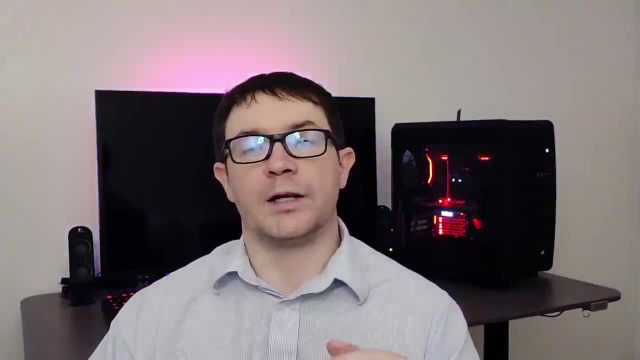 It's a relatively simple problem- The carpool- And so we're going to be able to get away with this. The reason I'm doing it this way is because I, frankly, could not get shared input layers to work with the PyTorch multiprocessing framework. 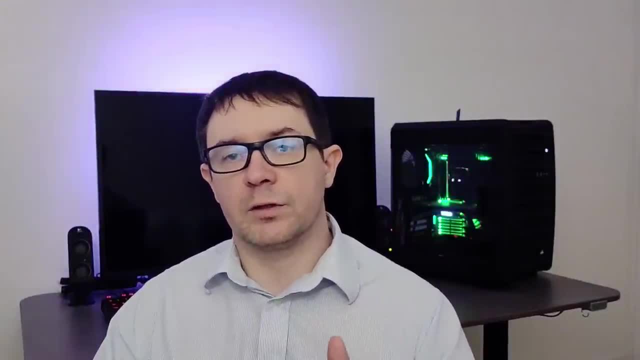 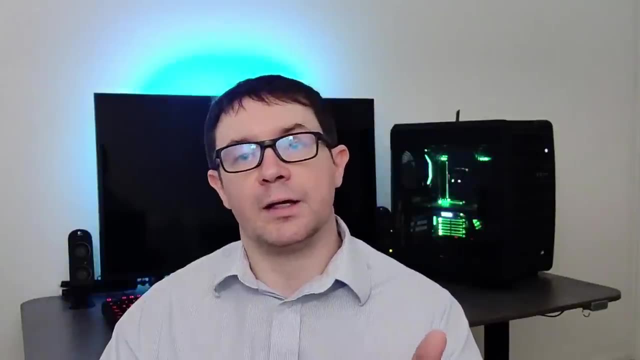 Our agent will also have a memory which we're just going to use simple lists for that. We're going to append states, actions and rewards to those lists and then go ahead and set those lists back to empty lists when we need to clear the agent's memory. 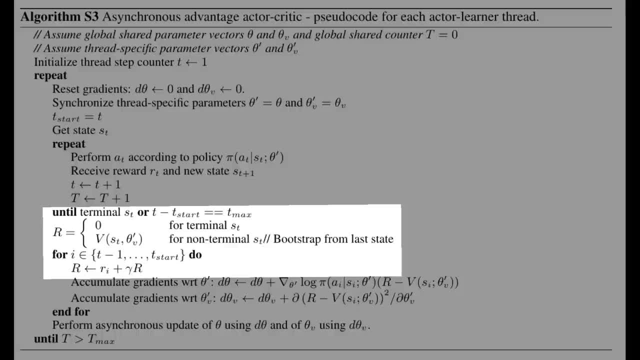 We're going to have a function for calculating the returns, where we're going to use the calculation according to the algorithm presented within the paper. So the idea is that we're going to start at the terminal step or the final step in the trajectory. If that step is terminal, the r or the return gets set to zero. 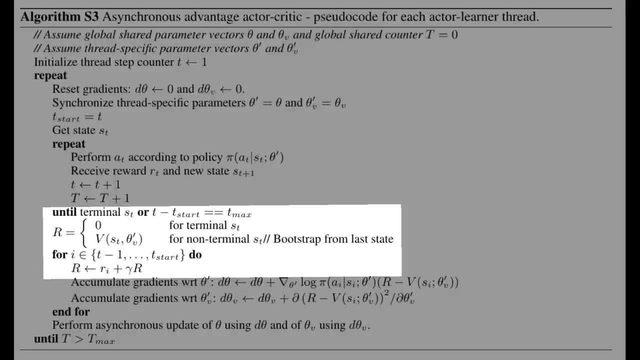 If it's not, it gets set to the current estimate of the value of that particular state. Then we're going to work backward from the t minus one time step all the way to the beginning And we're going to update r as r sub i plus gamma times the previous value of r. 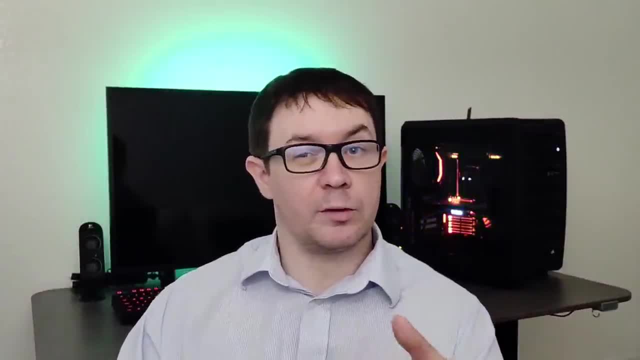 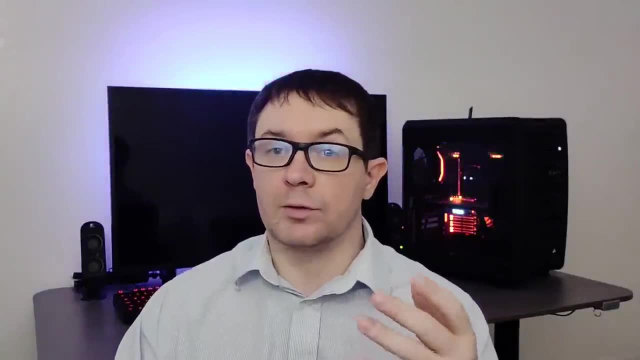 Now I'm going to do a calculation in the video of the coding portion to show you that these two are equivalent, meaning this calculation as well as the earlier advantage description I gave you. I'm going to make sure that you understand that those are actually equivalent. 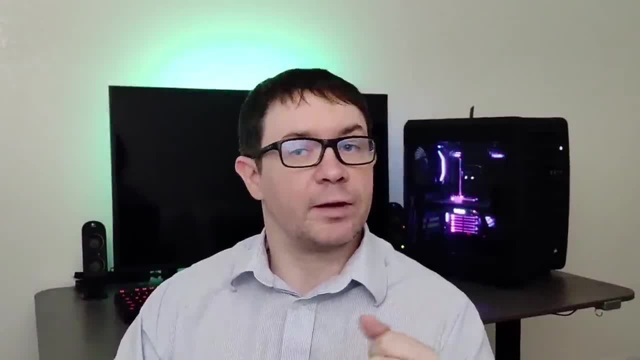 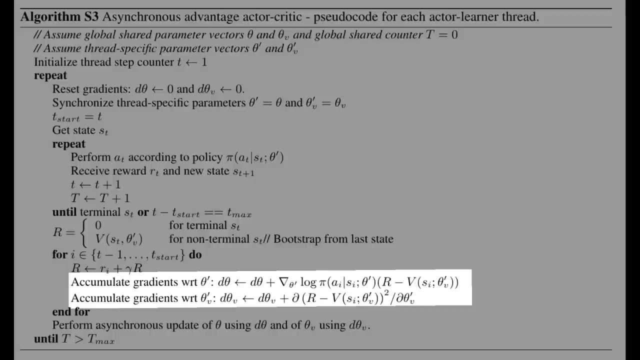 And it's just a few lines of mathematics, so it's not really that difficult and I've taken the liberty of doing it for you. Then we're going to be calculating the loss functions, and these will be done according to the loss functions given in the paper. 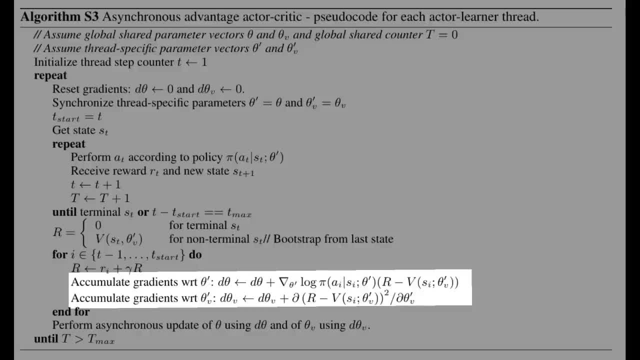 So for our critic, we're going to be taking the delta between those returns and the values and taking the mean squared error. For our actor, we're going to be taking the log prob of the policy and multiplying it by the advantage, and with a negative one factor thrown in there as well. 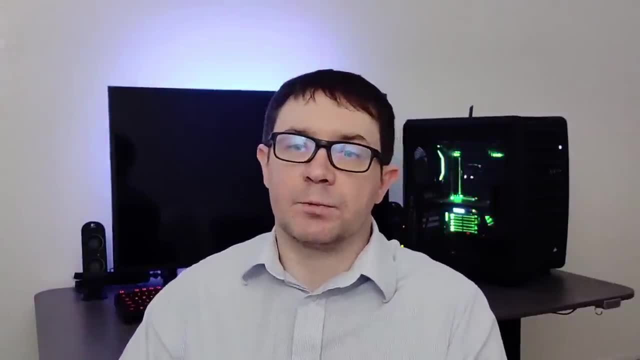 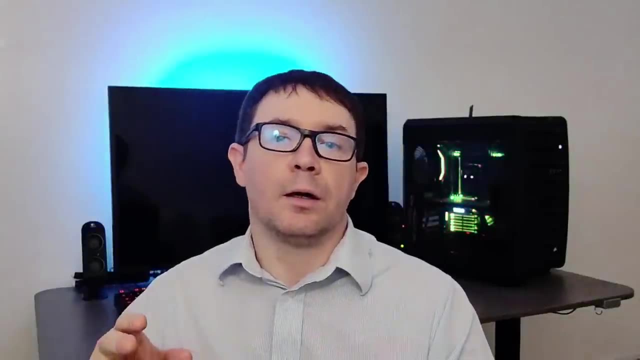 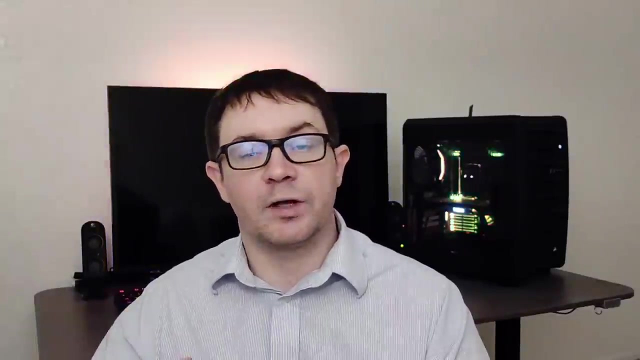 Now that's a really cool way of calculating the loss for the actor, because it has a pretty neat property. So when we multiply the advantage by the log of the probability, what we're actually doing is weighting probabilities according to the advantage they produce. So actions that produce a high advantage are going to get naturally weighted higher and higher over time. 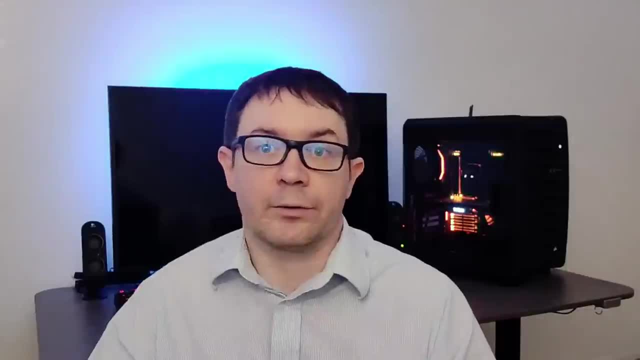 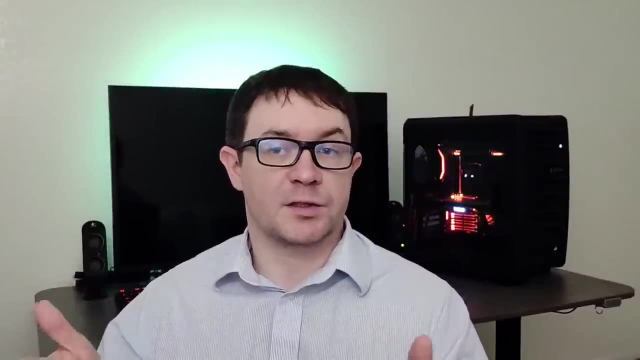 And so we're going to naturally evolve that. We're going to evolve our policy towards being better over time, which is precisely what we want, right? Our final class will be the agent class, and this will derive from the multiprocessing process subclass. 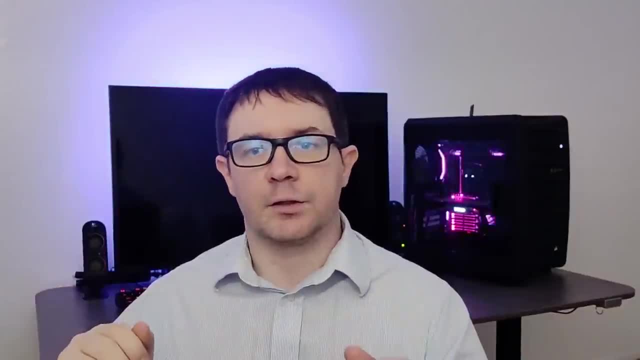 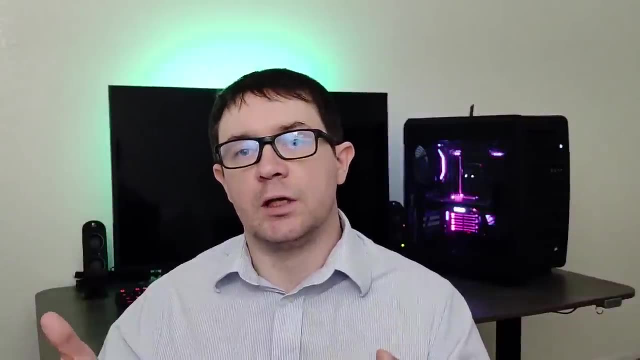 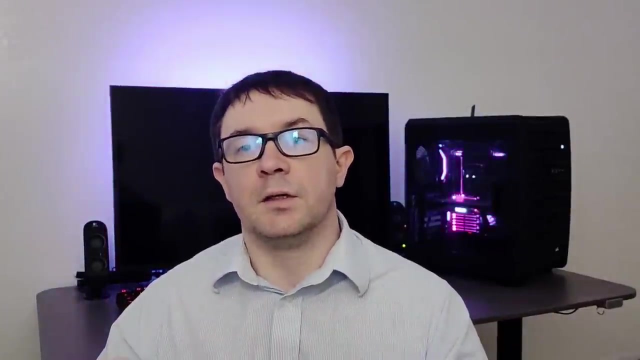 So here's where all of the real main type functionality is going to happen. So we're going to be passing in our global optimizer as well as our global actor critic agent instantiating 16,, in the case of 16 threads for a CPU, local critics with 16 separate environments. 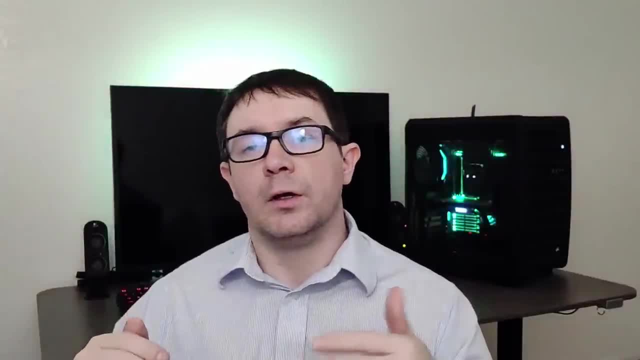 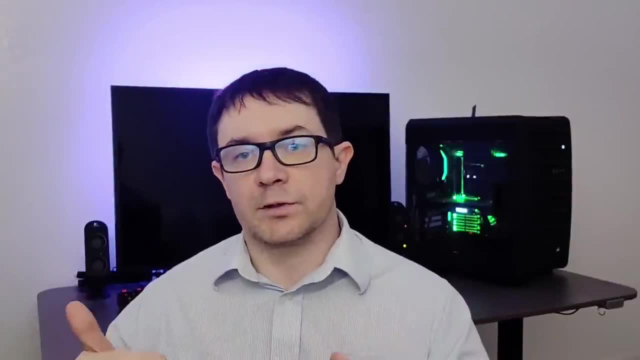 And each one of those is going to have two separate loops where it's going to go up until the number of episodes that we dictate and it's going to play each episode As I described earlier. within each episode it's going to play some fixed sequence, number of steps. 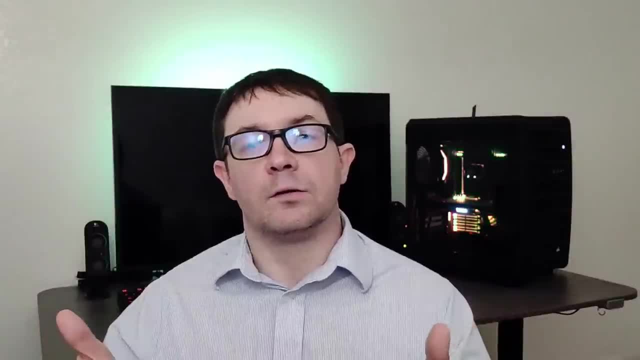 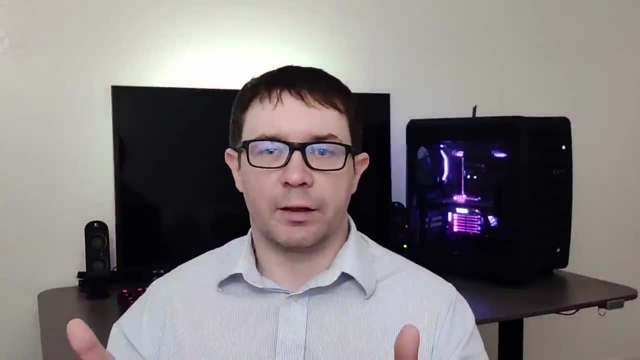 and then it is going to perform some update to the global optimizer and then download the parameters from the global actor critic agent. Our main loop is basically going to set everything up. We're going to go ahead and define all of our parameters, create our global actor critic. 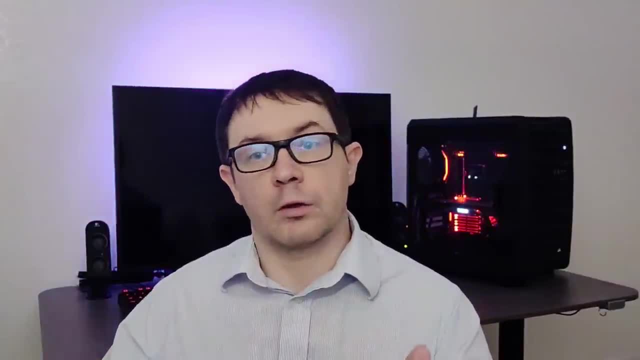 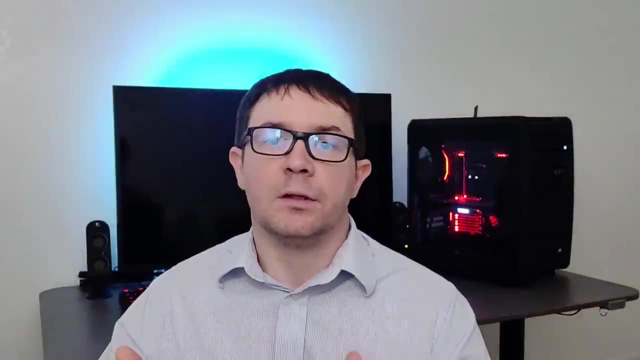 our global optimizer and tell PyTorch that we want to share the memory for our global actor critic agent. And then we're going to make a list of workers or agents, and then we're going to go ahead and send each of those a start command as well as a join command. 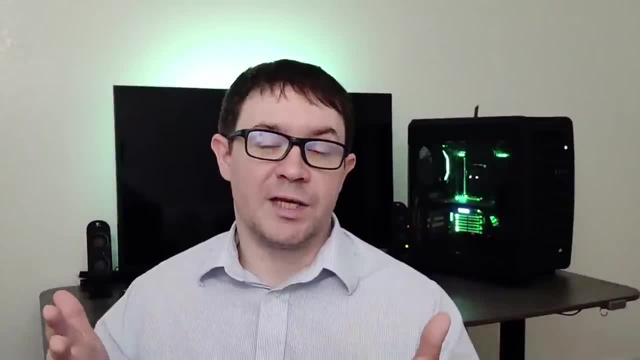 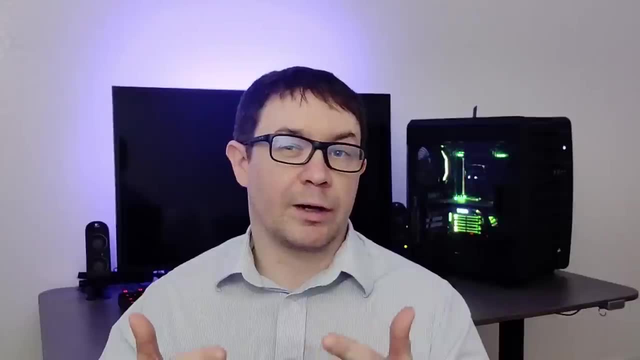 so that we can get everything rocking and rolling. So what are some critiques of this algorithm overall? Well, one is that it is exceptionally brittle. Most actor critic methods require a fair amount of hyper-parameter tuning, and this one is no exception. I tried to use the lunar landing system. 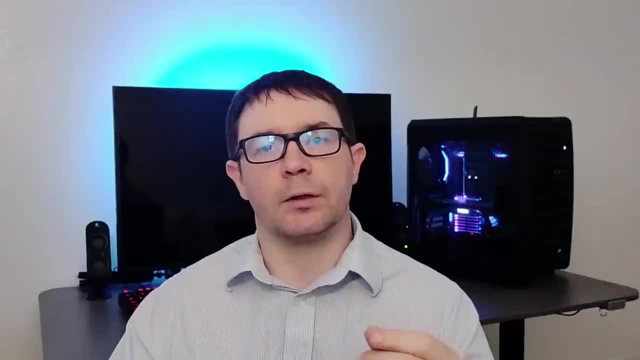 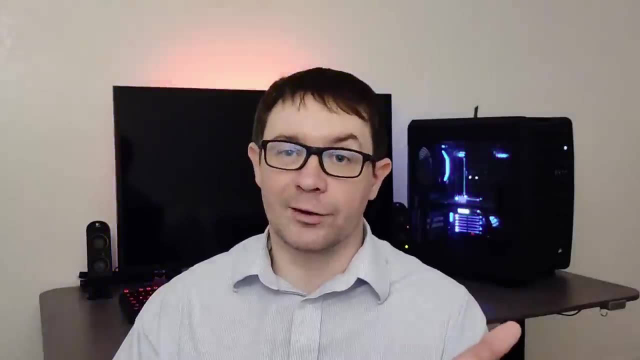 which is a standard environment, but couldn't really get a good set of parameters to make it run effectively and get a consistent score of 200 or above or, heck, even a consistent score of over 100.. I would have called that good enough for YouTube. 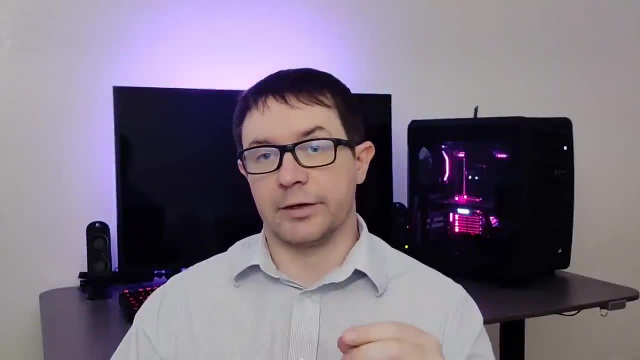 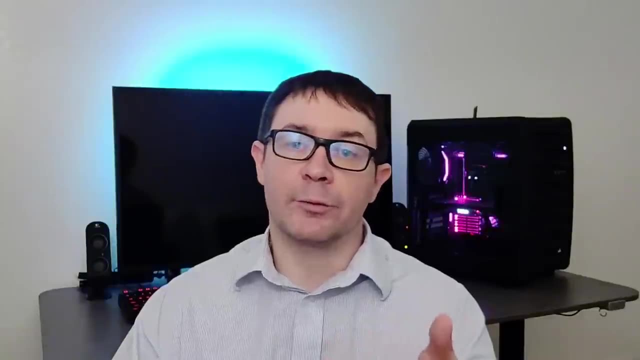 Another one is that there is a significant amount of run-to-run variation, so it's highly sensitive to initial parameters. You can solve this by setting global seeds for the random number generators, so that you're getting consistent random numbers over time and so you're going to know exactly how you're starting. 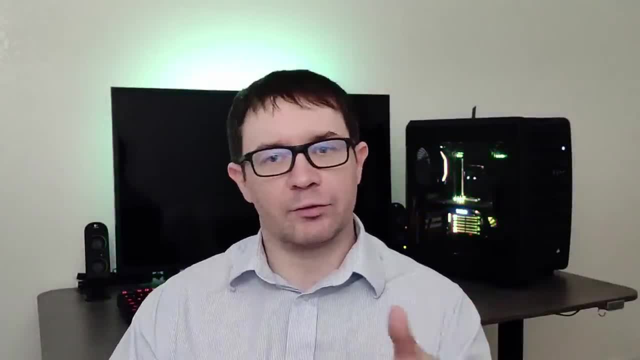 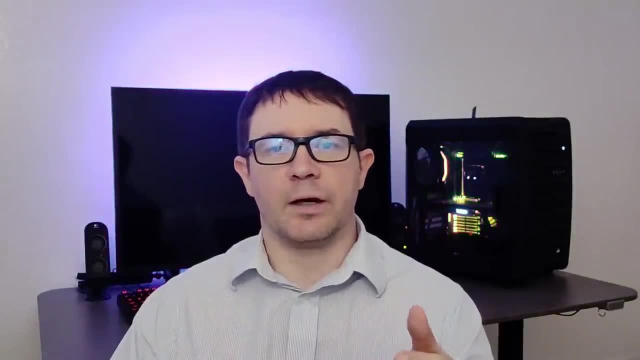 But to me it's a little bit kind of like cheating, so I don't do it in this video, but it is something to take note of, And in the original paper I think they do something like 50 different runs of each evaluation. 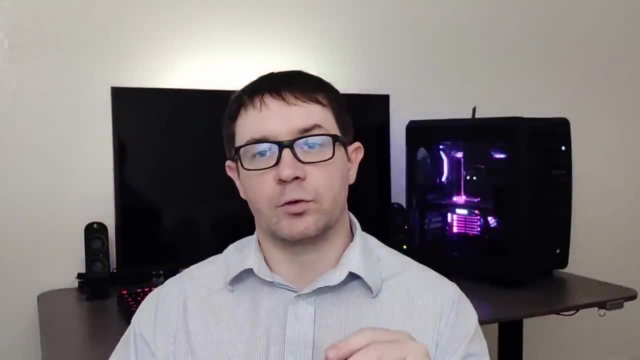 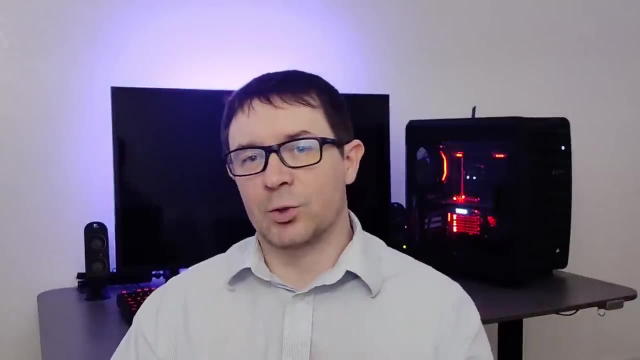 some large number to get a pretty solid distribution of scores, and that is, I think, because of the high degree of run-to-run variation. Okay, I have lectured at you enough. Again, if you like to read written content, I have a link in the description to a blog post. 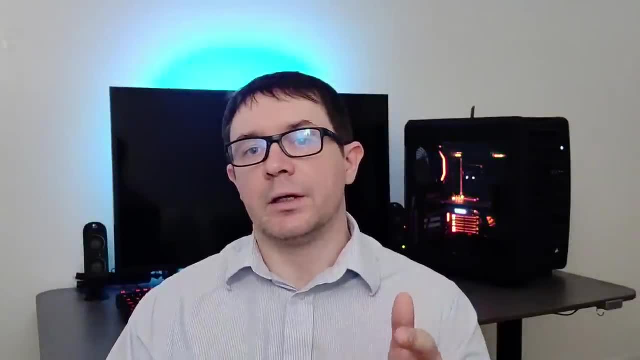 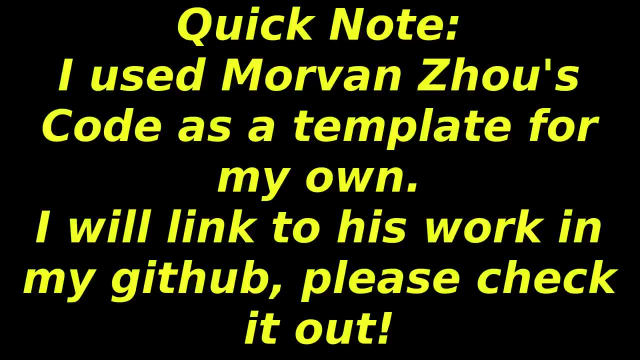 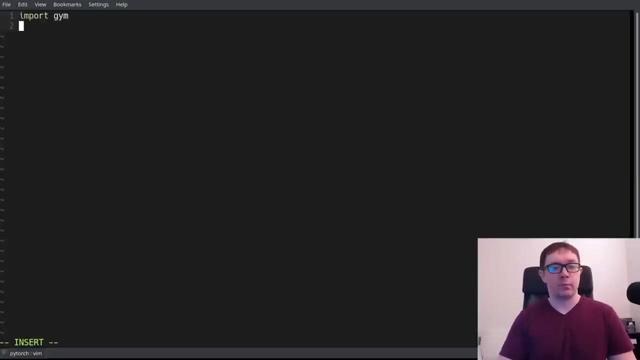 where I talk about this in a little bit more detail. But nonetheless, let's go ahead and jump right into the coding tutorial. Let's go ahead and start with our imports. We will need Jim for our environment. We'll need our base Torch package. 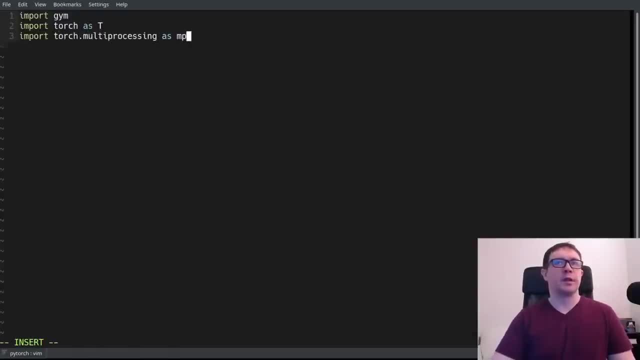 We'll need Torch multiprocessing to handle all the multiprocessing type stuff. We will need Torch NN to handle our layers. We'll need NN functional to handle our activation functions And we're going to need our distribution as well, And in this case we're going to need a categorical distribution. 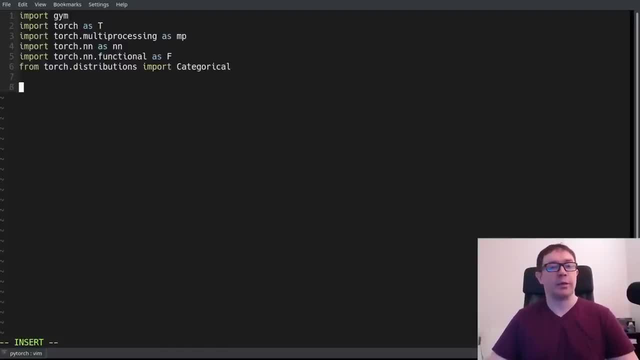 All this does is takes a probability output from a deep neural network, maps it to a distribution so that you can do some actual sampling to get the real actions for your agent. Now I'm going to show you how to do that. Now I want to start with the shared atom class. 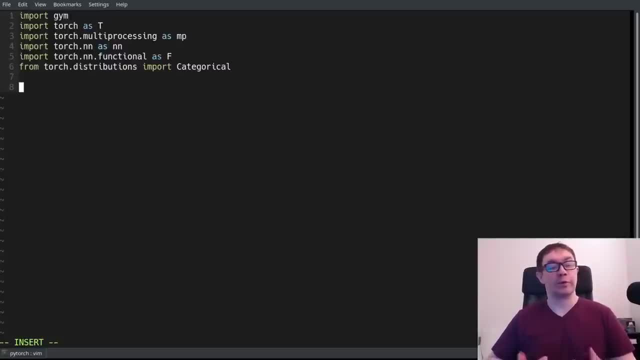 This will handle the fact that we are going to be sharing a single optimizer among all of our different agents that interact with separate environments. All we're going to do here is call the base atom initializer and then iterate over the parameters in our parameter groups. 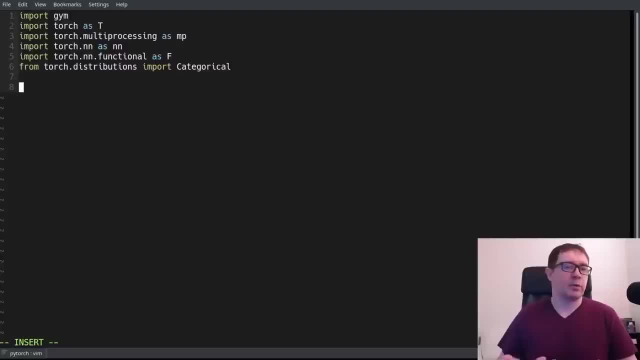 setting the steps exponential average and exponential average squared to zeros effectively and then telling it to share those parameters amongst the different pools in our multi-threading pool, And this will derive from the base atom class. Our default values are going to be, I believe, identical to the defaults for the atom class. 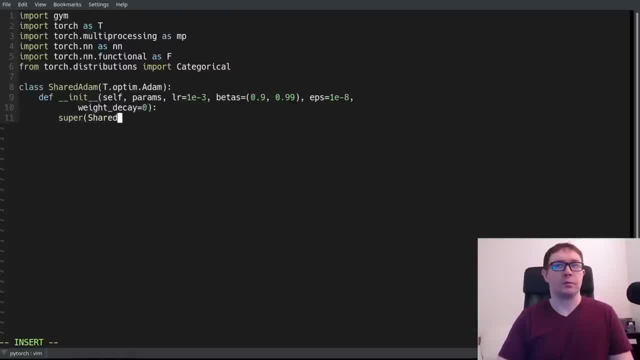 And then we want to call our super constructor. And then we want to call our super constructor. Now we're going to handle setting our initial values. Now we're going to handle setting our initial values. So I can just basically start from the base atom. 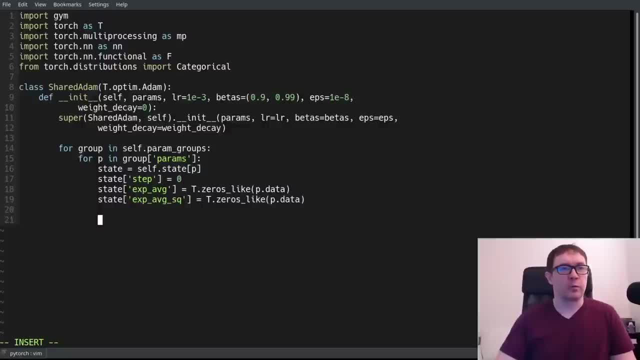 And then we're going to tell TorchApply, we want to share the memory for our parameters, for our gradient descent, and note the presence of the underscore at the end of memory there. Okay, that is it for the shared atom, pretty straightforward. Next up, we want to. 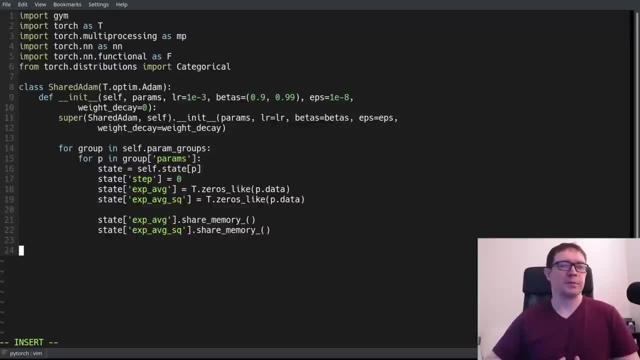 handle the actor critic network, which will also encapsulate a lot of the functionality I would typically put into an agent class because of my understanding of the design principles of object-oriented software programming. In this case, I have to shimmy a few things around because the agent class is. 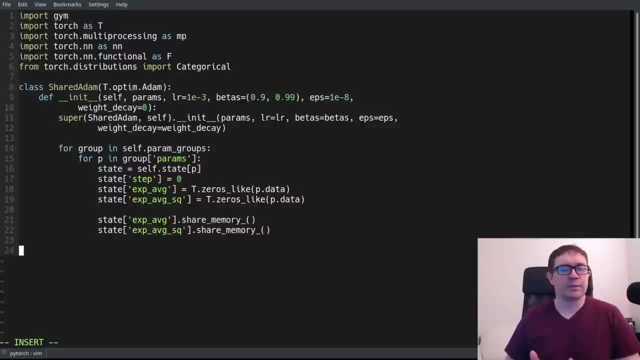 going to handle the multi-processing elements of our problem, and so it doesn't really make sense to stick this, like the choose action memory functionality, in the agent class. so we're gonna stick it in the network class. It's not a huge deal, it's just a departure from. 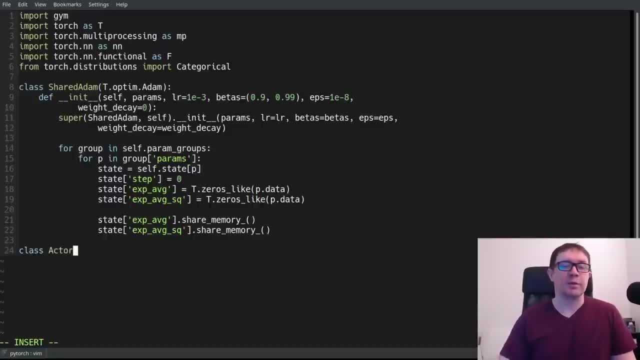 how I normally do things, and certainly not everybody does things the same way I do. So our initializer takes input dims from our environment, number of actions from our agent and a default value for gamma of 0.99.. We also have to save our gamma, and the next thing we want to handle is writing. 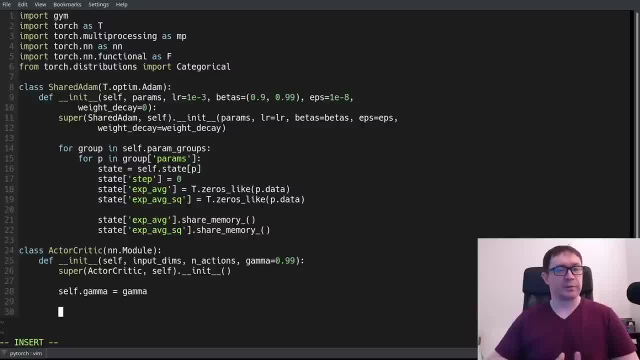 our actual deep neural network. Now, this is also a little bit different than the way I normally do things. Normally, I would have a shared input layer that branches out into a policy and a value network as two separate outputs with that shared input layer. When I tried to do that, I found that the software 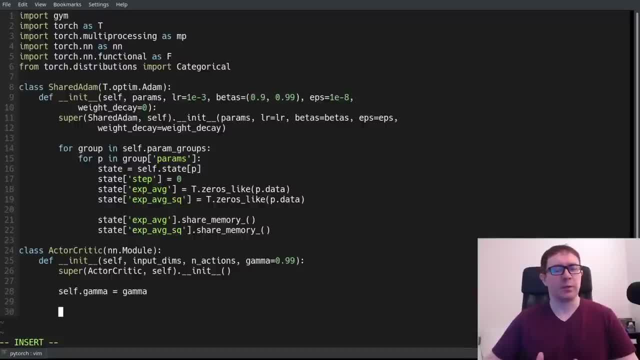 doesn't actually run. it doesn't handle the threading aspect very well in that that case, when you have shared input layers from a deep neural network. I don't know exactly why that is. If you know, please leave a comment down below, because I'd be very curious to hear. 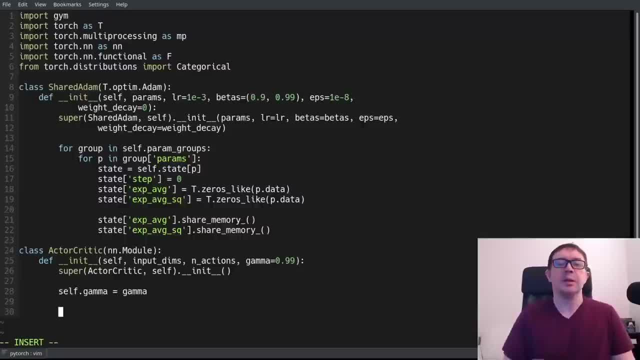 the explanation. It's simply what I found out through my own experimentation. So we're going to have two separate inputs- one for the policy and one for the value network- as well as two separate outputs, So they're effectively two distinct networks within one single class. 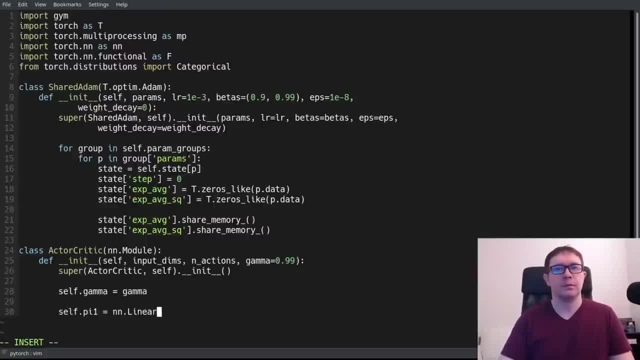 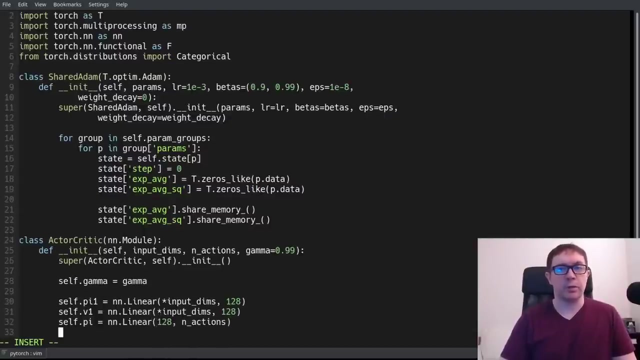 And we're only going to be using 128 neurons here, not a very large network, And our output will take those 128 hidden neurons and convert it into the number of actions, And our value function will take likewise the 128 hidden neurons into the number of values And we're going to have a number of actions. 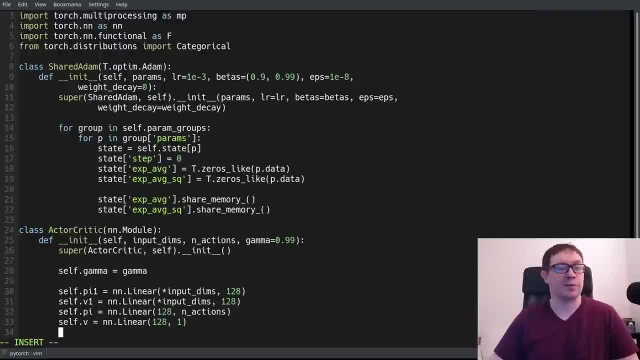 And we're going to have a very large network and our output will take those 128 hidden neurons, 28 hidden layers, hidden elements, and convert it to a single value. or if you pass in a batch of states, a batch of values, the agent also- excuse me, the- 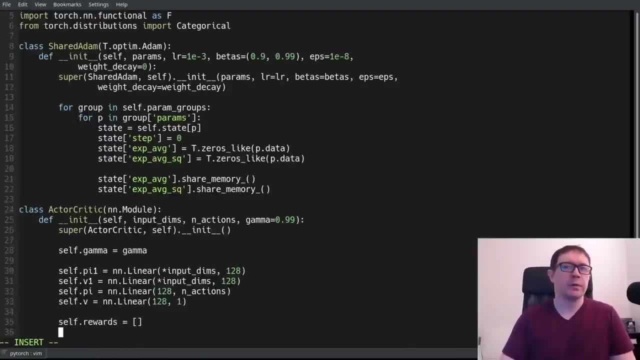 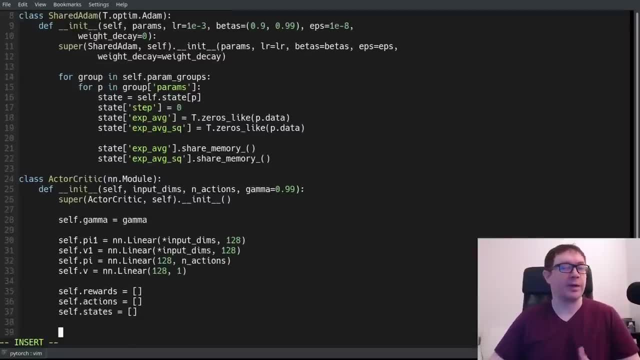 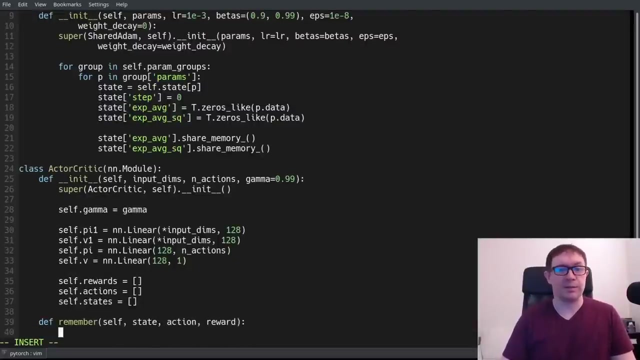 network also has some basic memory. so rewards, actions and states, these we will handle just by appending stuff to a list and then, and each time we call the learning function, we're going to want to reset that memory. so let's go ahead and handle that functionality first. so the remember just appends a state action. 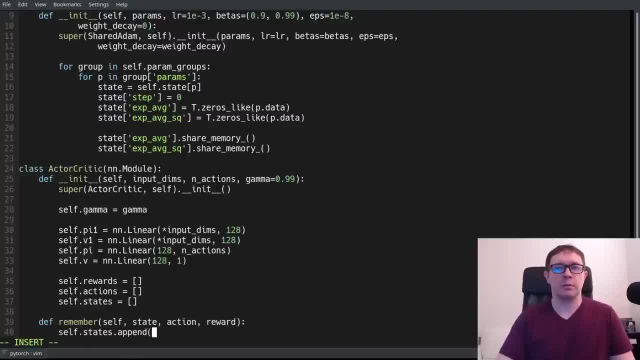 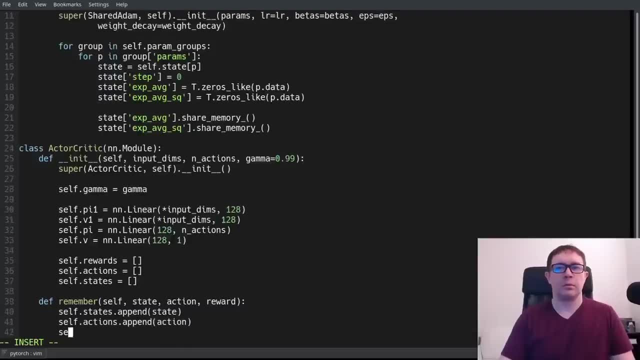 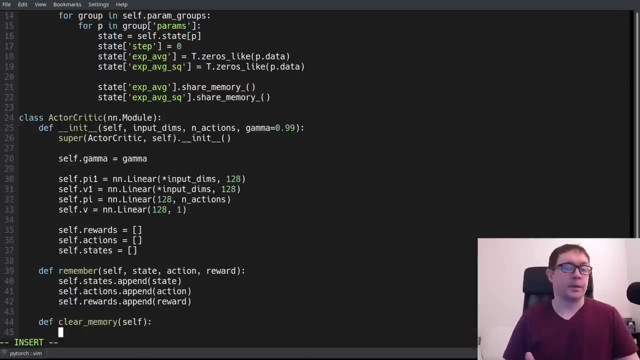 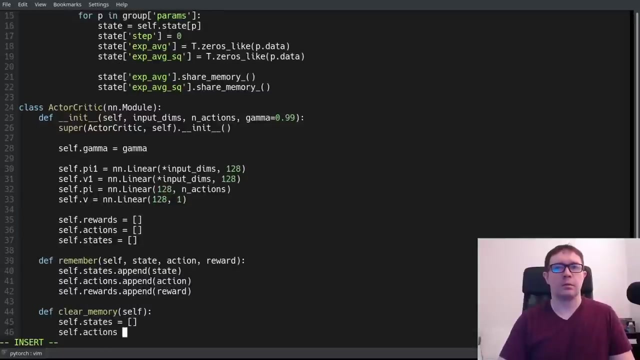 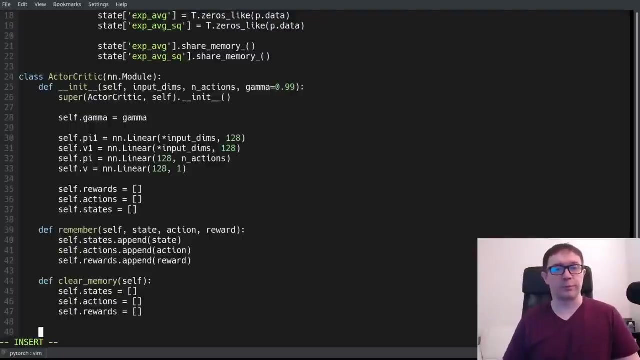 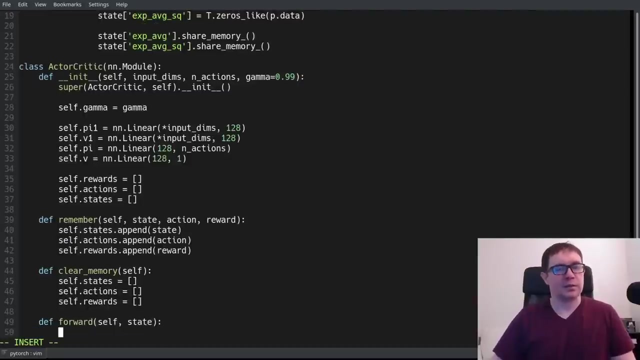 reward to the relevant list and a clear memory function just zeroes out all those lists- pretty straightforward. next we have our feed forward function that takes a state as input. so we're gonna pass that state through our first input layer for our policy and perform a value activation on that and do something similar for 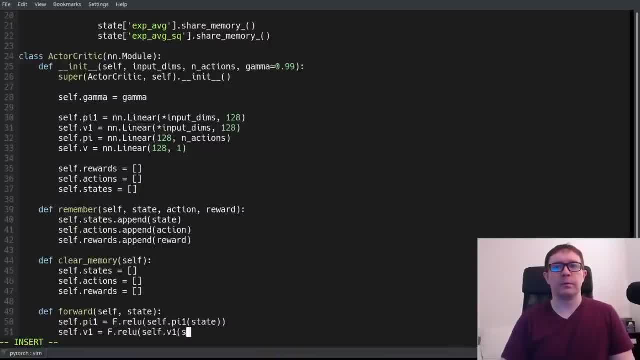 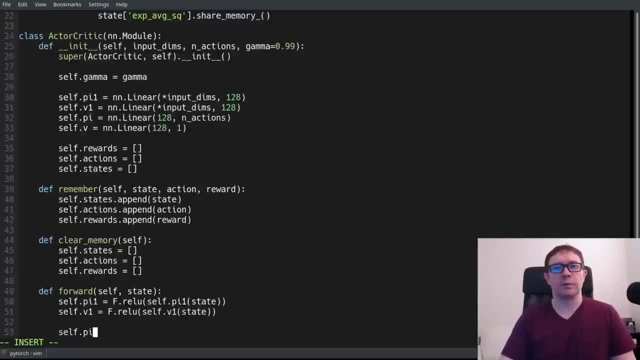 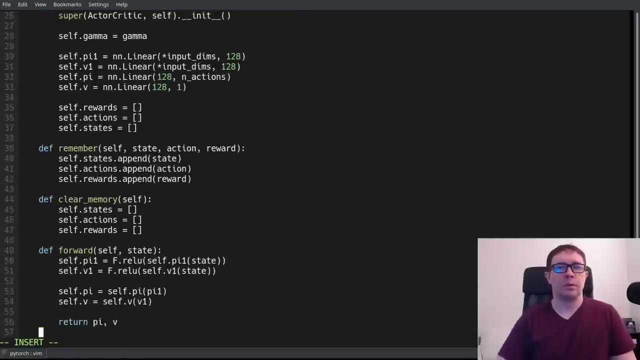 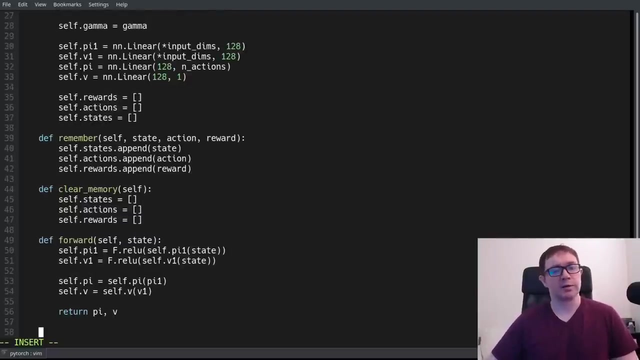 the value input layer, and the outputs of those two are going to be passed to the rel, to the relevant policy and value outputs, and then we just return PI and V. pretty straightforward yet again. next we're gonna have our function to calculate the returns from our sequence of steps, so this will only take a single. 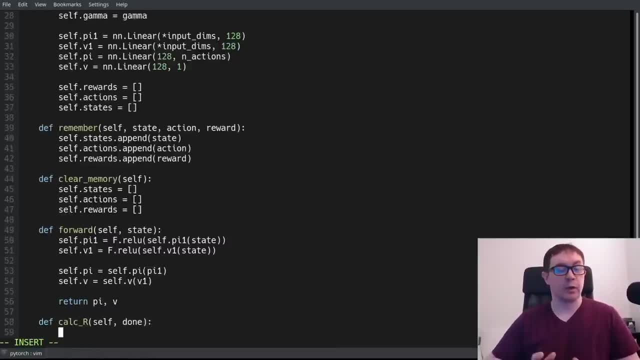 input and then we're going to have our function to calculate the returns from our sequence of steps. so this will only take a single input in the. that will be the terminal flag. recall that the return for the terminal step is identically zero, so we need the terminal flag or the done flag to accommodate that. 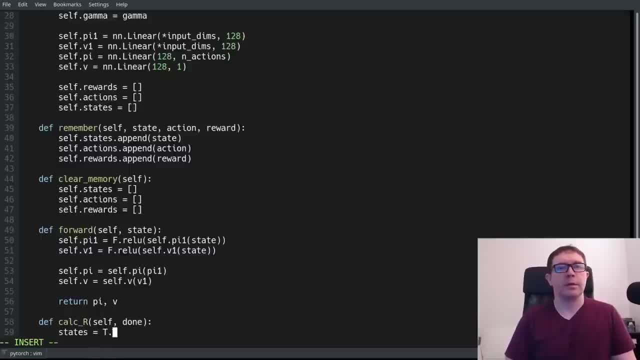 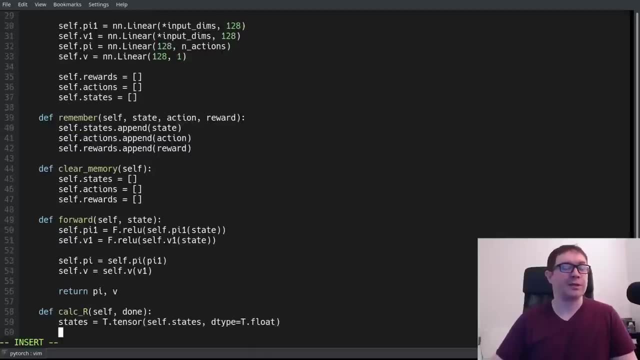 so we want to go ahead and convert the states from our memory to a torch tensor of T dot float data type, because it is a little particular about the data type. you don't want to pass it in double. it gives you an error, so best to take care. 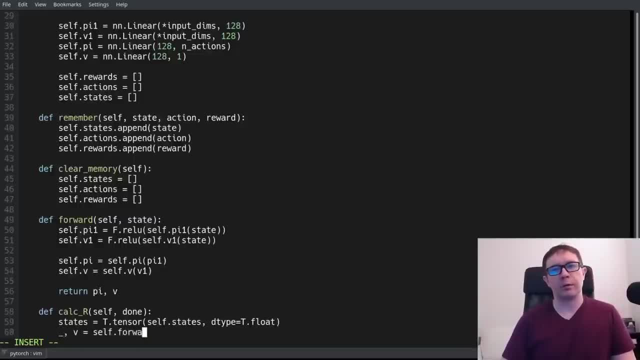 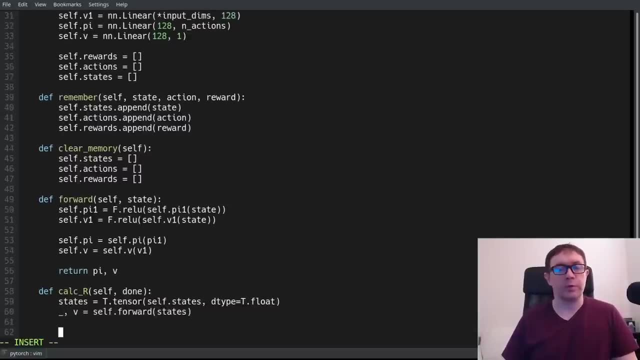 of it. now we're gonna go ahead and pass that through our neural network and we're not going to be concerned with the policy output at this stage. we just want to know what the value evaluations the critic has for that set of states. so our return is going to be- is going to start out as the 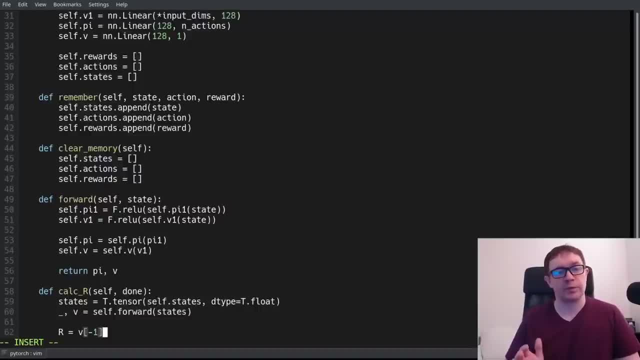 last element of that list, so the terminal step, or the last step in the sequence of steps, and we're gonna multiply that by 1 minus and done so that if the episode is over 1 minus int is done, so that if the episode is over one minus int is done. 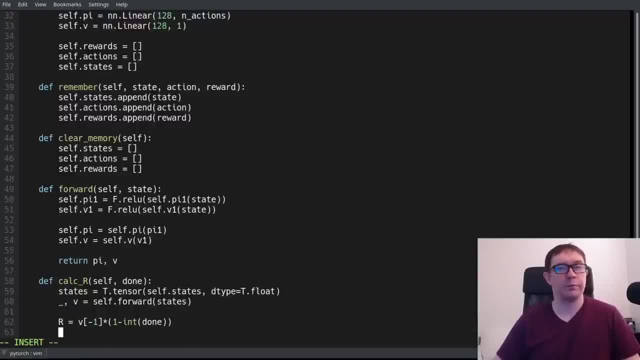 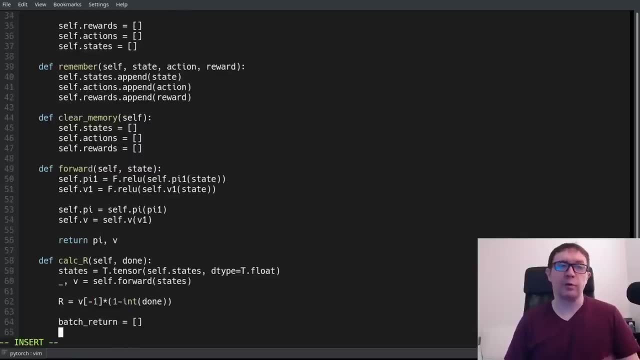 one minus int is done, is done is zero. so you're multiplying by zero, you get zero. pretty handy way of handling that. then we're going to handle the calculation of the returns at all the other time steps. so we're going to go ahead and iterate over the reversed memory and say that our return is the 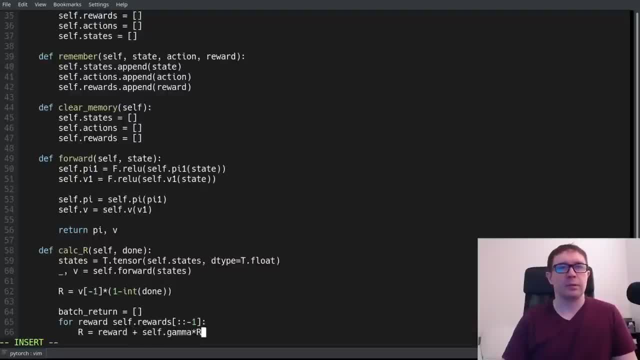 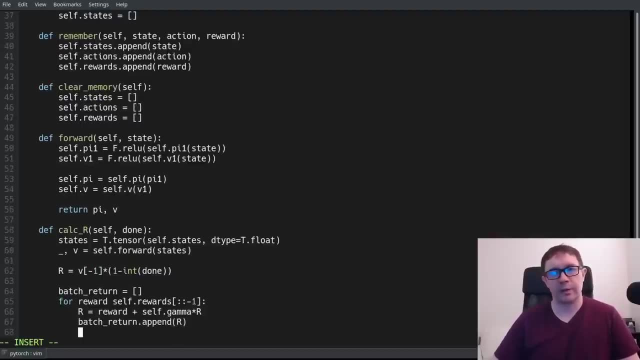 at that time, step plus gamma times r, and then just return, excuse me, append that return to the list of batch returns and then finally, at the end, you want to go ahead and reverse that list again. so that's in the same order in which you encounter the states. this calculation reverses it because 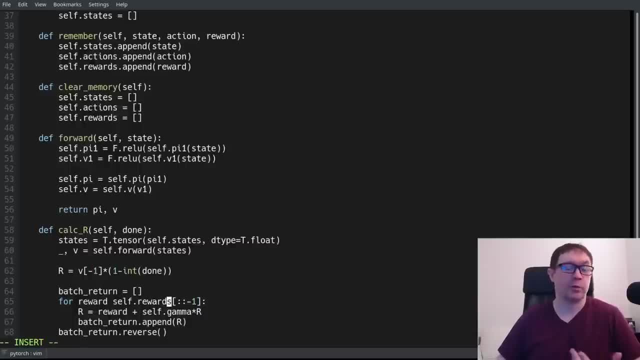 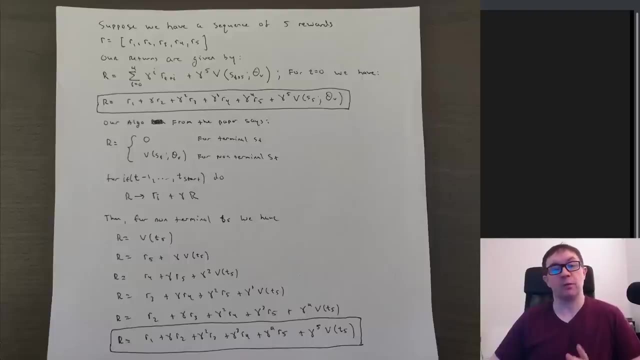 you're starting at the end, when you know the value of the final state, or at least the estimate of the according to the critic, and then reversing it to get it back in order for passing it into our loss calculation function. Now, this may be a strange form to you. If you write it out by hand, maybe I can show you something here where. 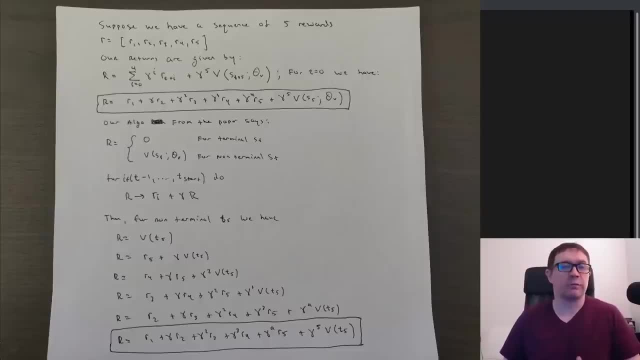 I did it for you. If you write it out by hand, this particular chunk of code, you can see that it's identical to what they tell you. the calculation is in the paper. So yeah, you can do that exercise on your own to convince yourself, or I can just show it to you so that I can convince you of it. 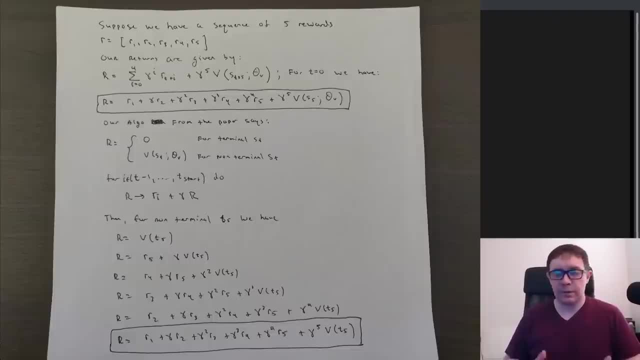 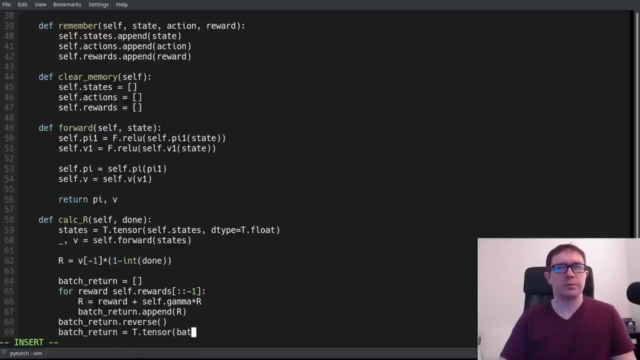 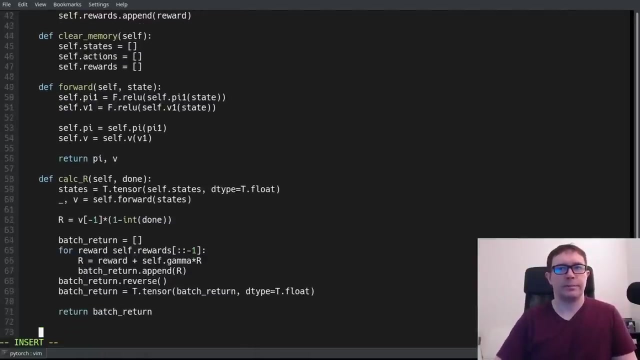 But this is indeed the return calculation from the paper. Everything is as it should be, And then I want to convert that to a tensor and return it. Next we have to handle the calculation of our loss function, And this again is only a single input: the terminal flag from the environment. 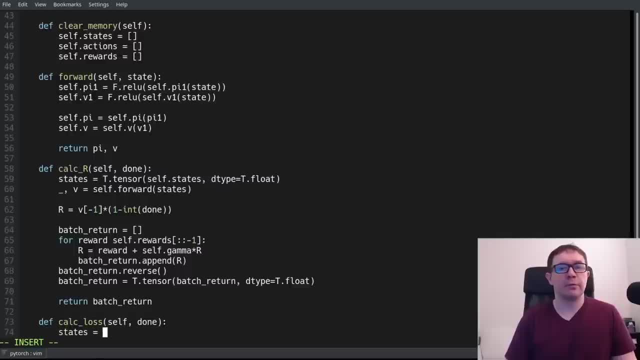 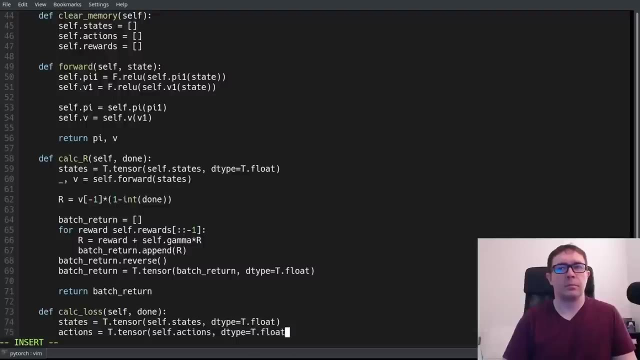 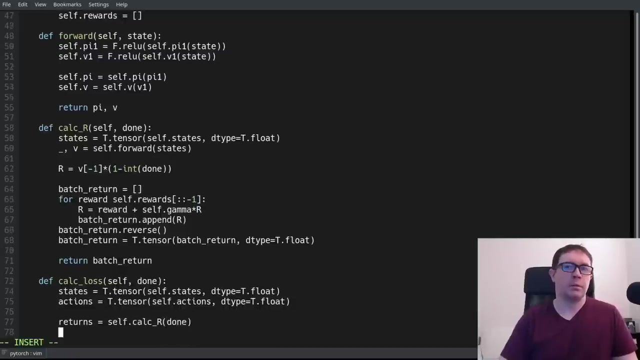 We're going to go ahead and get the value- excuse me, the tensor- representations of our states and actions right at the beginning, And then we're going to go ahead and calculate our returns And then we're going to perform the update, So we're going to be passing the states through. 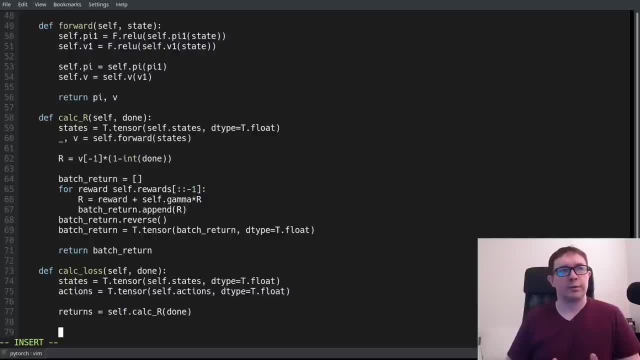 our actor critic network to get the new values as well as then a distribution according to the current values of our deep neural network. We're going to use that distribution to get the log probes of the actions the agent actually took at the time it took them, And then we're going to 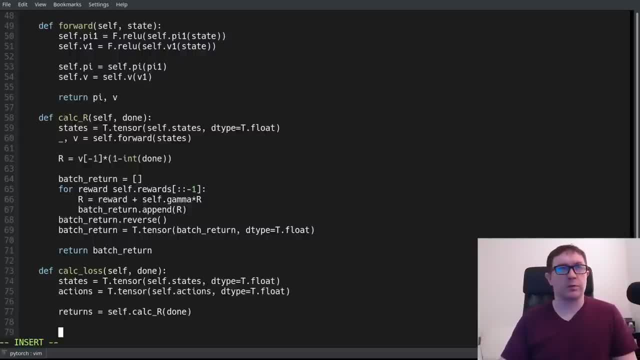 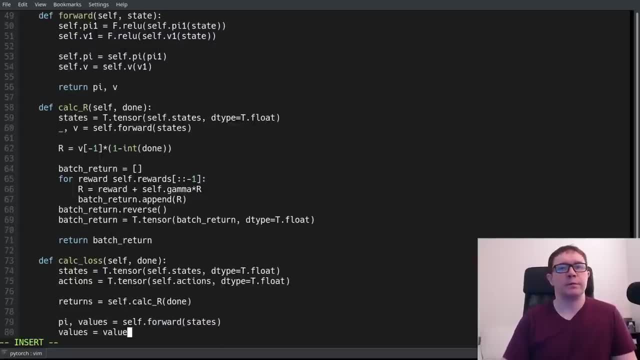 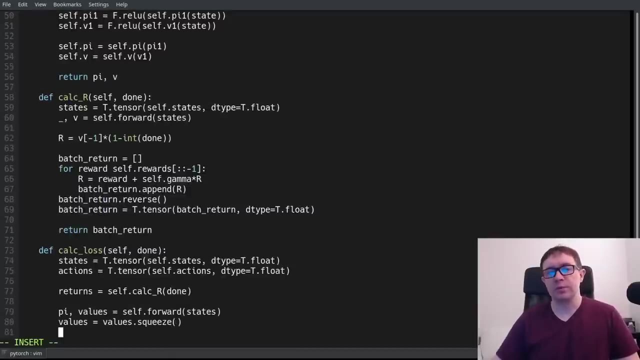 use those quantities for our loss functions. So we're going to use the values valuessqueeze. Now, this squeeze is very important. If you don't squeeze here, it won't trigger an error, but it will give you the wrong answer. 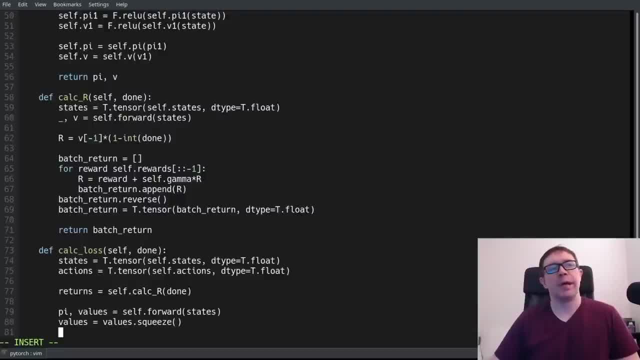 The reason it will do that is because the actor loss and the critic loss, I believe, will come out as a shape of five by five, And that is not the shape we want. We want something in the case of five time steps. T max equals five. 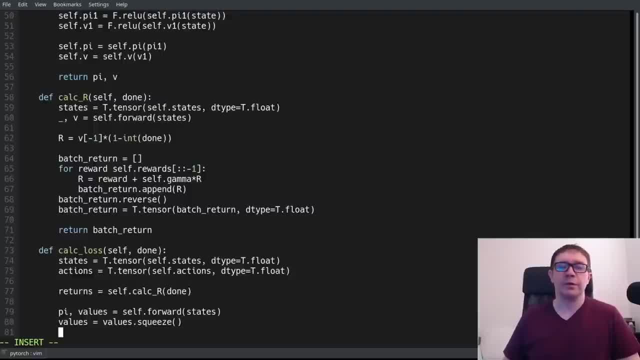 So it'll give you a five by five matrix instead of a five element vector. So you have to perform the squeeze here to get the five by one output of the deep neural network into something that is just five: a list of five elements or a vector of five elements instead of five by one. 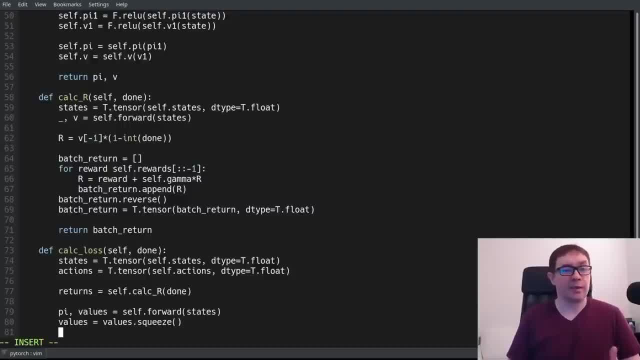 So definitely need that squeeze. If you don't believe me, by all means erase the line or comment it out and print out the shapes of things to the terminal. I always recommend doing that. It's a good way of solidifying your understanding of how all this stuff works. 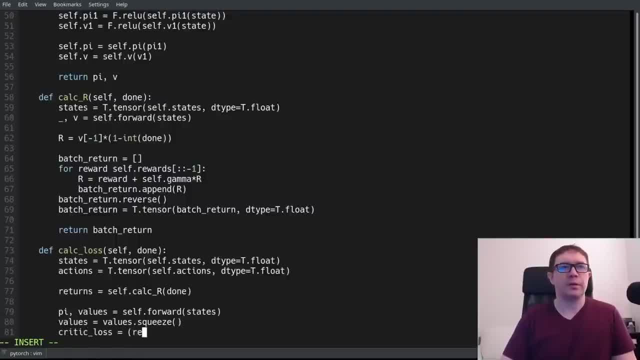 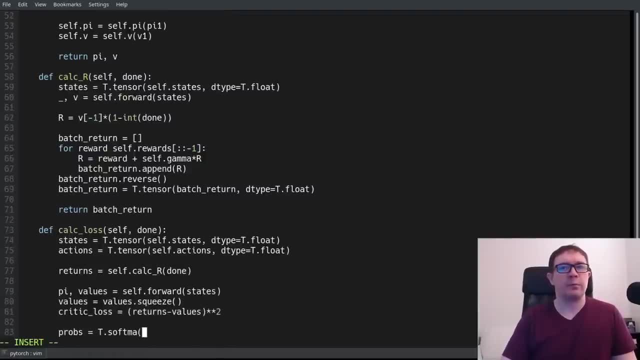 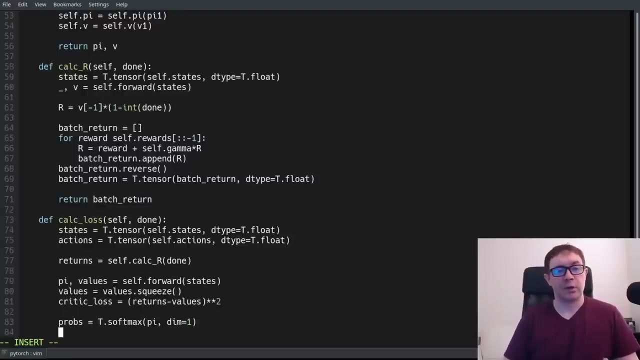 So then our critic loss is just the returns minus values squared. Pretty straightforward. So now let's go ahead and say that we want the softmax, activation of our output, And that has a property that of course, the softmax guarantees That every action has a finite value and that the probabilities add up to one, as all probability distributions distributions should. 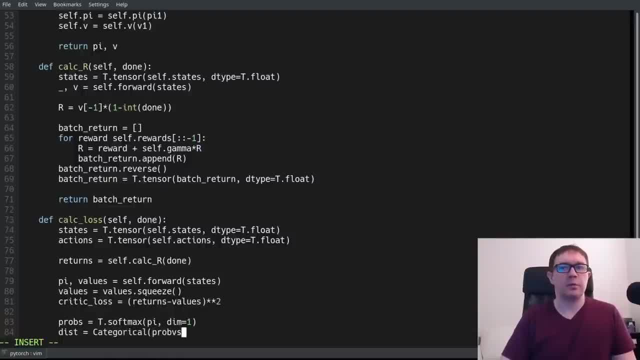 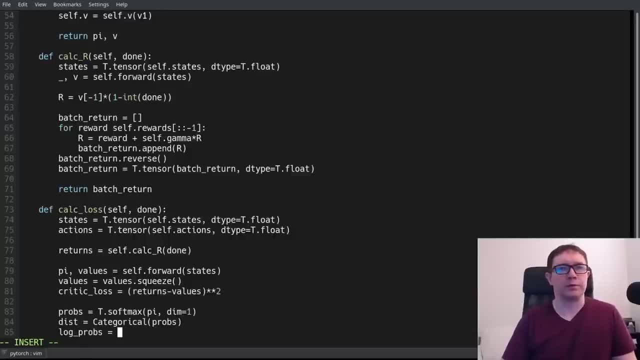 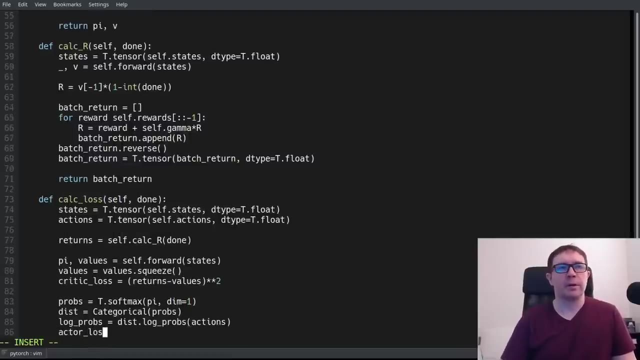 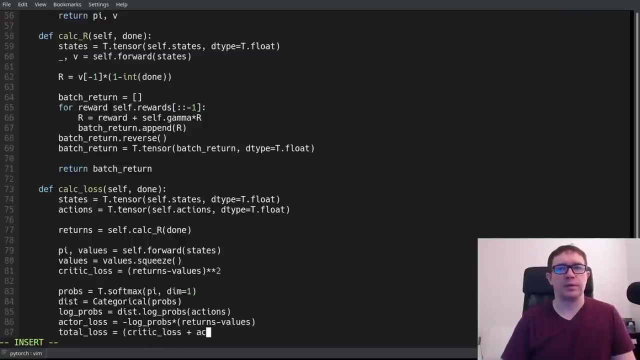 So then we use that output to create a categorical distribution and calculate the log probability distribution of our actions actually taken. Then our actor loss minus log Probs times the quantity returns minus values, That's from the paper, And then our total loss is just critic loss plus actor loss dot mean. 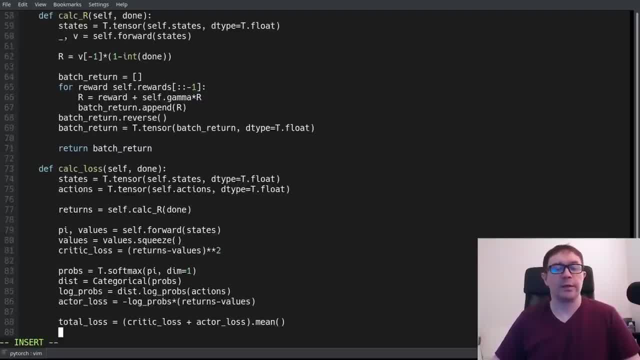 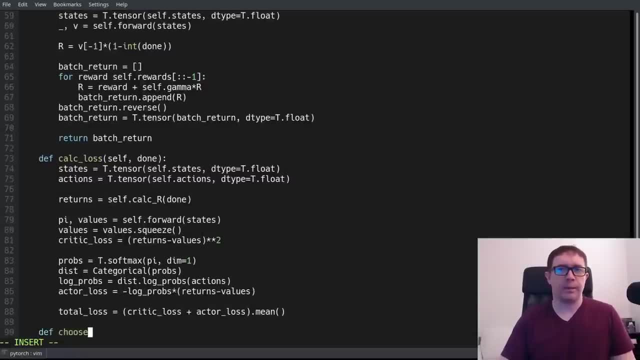 We have to sum the two together because of the way that the back propagation is handled by PyTorch. And of course I did forget to choose action function. But that Is not a big deal, We'll just go ahead and handle that now. 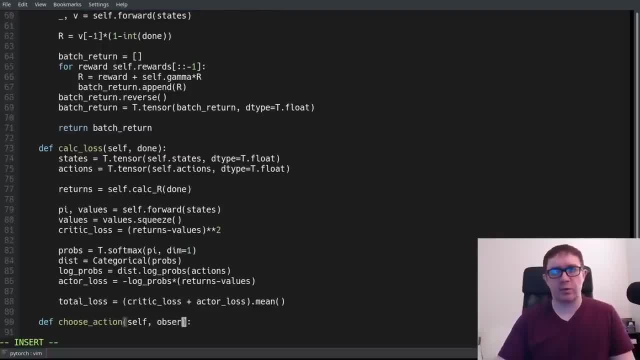 So that will take. We're going to call it observation as input, Because we're going to be passing on the raw observation from our environment, And so we have to convert that to a tensor right off the bat And we have to add a batch dimension to that. 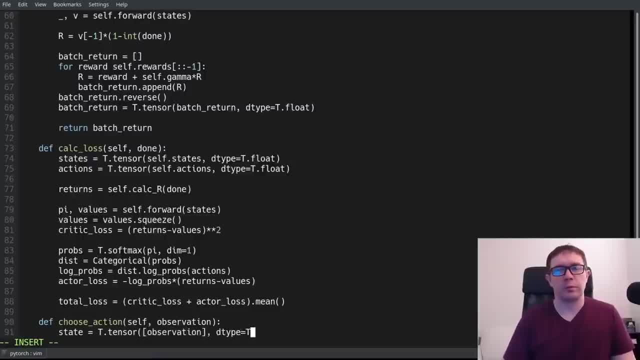 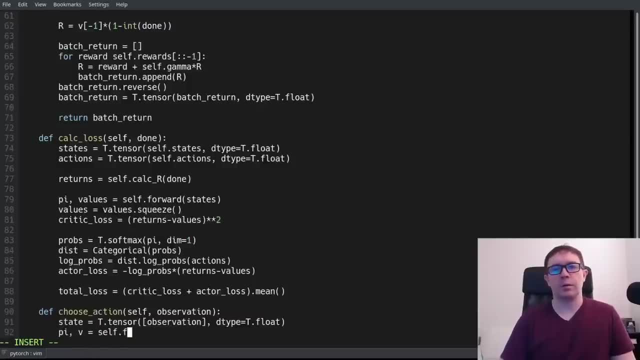 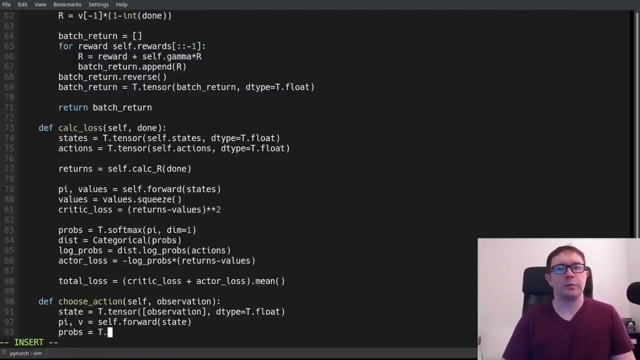 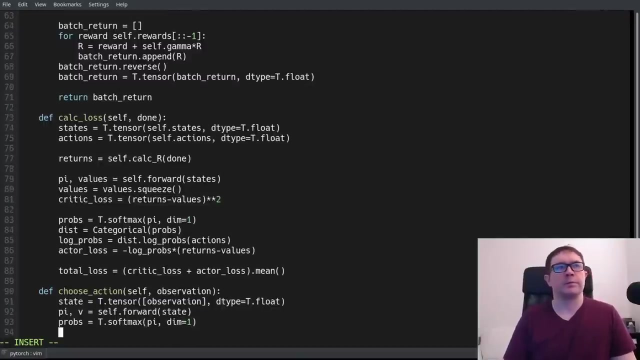 For compatibility with the inputs of our deep neural network And we're going to call it a D type of float. We pass that Through our neural network, Get our policy and value function out. Perform a softmax activation on our policy along the first dimension. 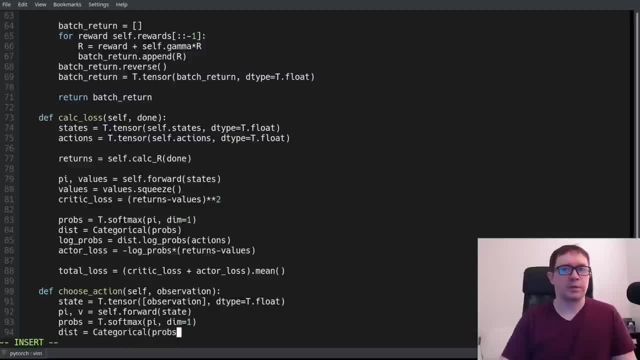 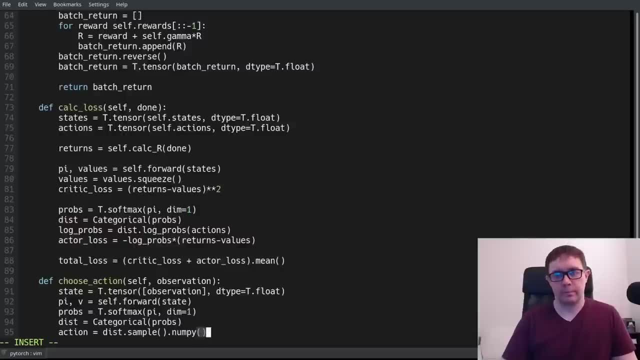 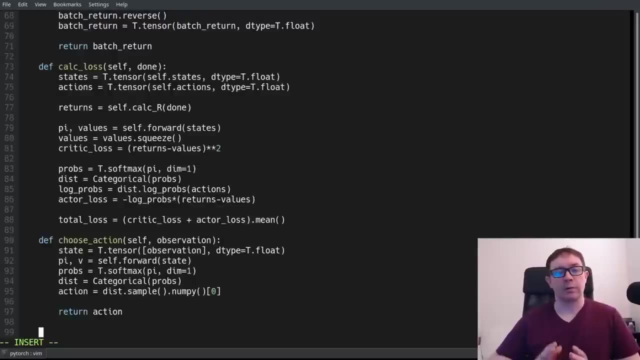 Then we're going to create our distribution based on those probabilities and sample it And convert it to a NumPy quantity, Take the zeroth element And return it. So that is it for our actor network class. It encapsulates most of the functionality I would associate with the agent. 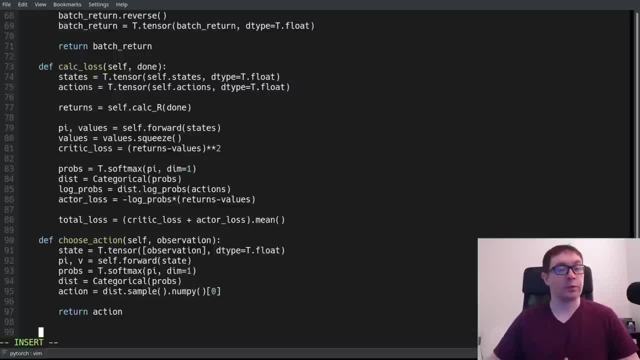 But it does everything we're going to need each of the independent actors within their own thread to do. Now we're going to move on to the agent class that is going to handle our multiprocessing functionality. So I'm going to call this agent. You will sometimes see it referred to as worker. 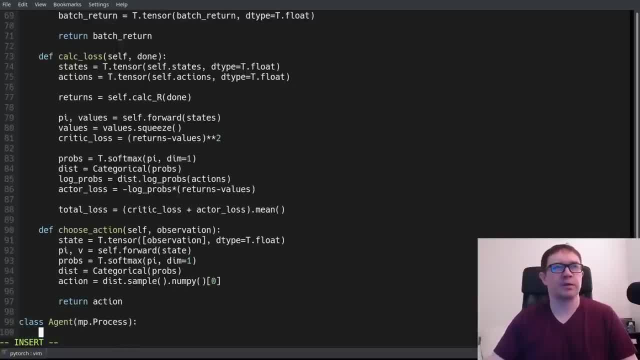 And that is a fine name. That is kind of precisely what it is. I'm just using agent. to be consistent with My previous nomenclature, It has to derive from the npprocess class, So we get some access to some goodies there. 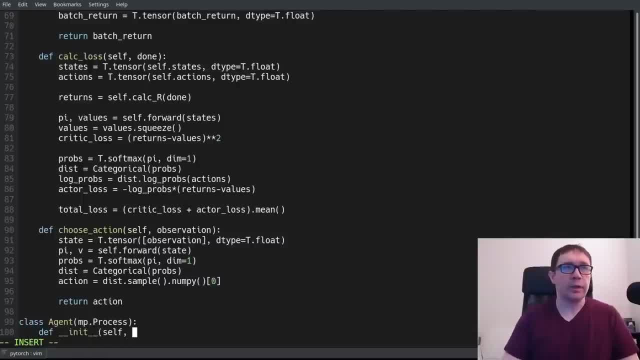 So we will need our global actor critic. That is what is going to handle the functionality of keeping track of all the learning from all of our environment specific agents. The optimizer That is going to be the shared atom optimizer that we wrote earlier. Input. 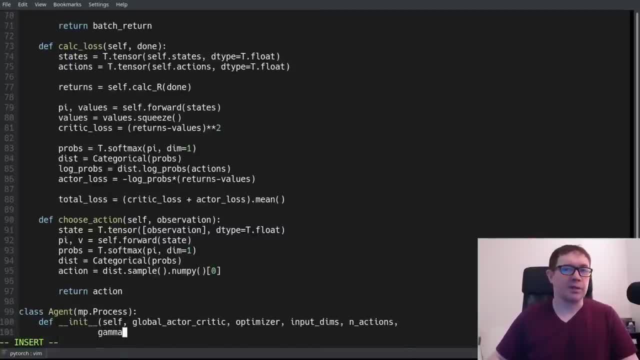 Dims Number of actions. Gamma, In case you want to use something other than 0.99.. A learning rate, A name to keep track of each of the workers from our multiprocessing, The global episode index. So this will keep track of the total number of episodes run by all of our agents. 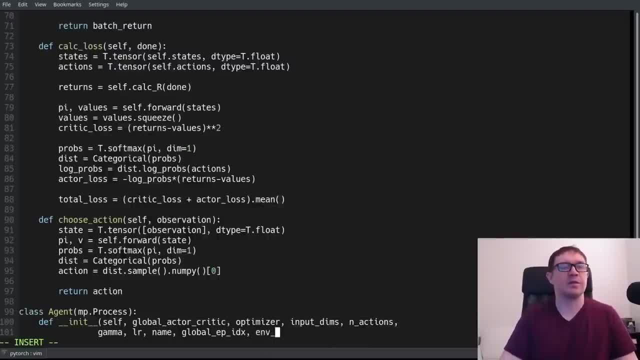 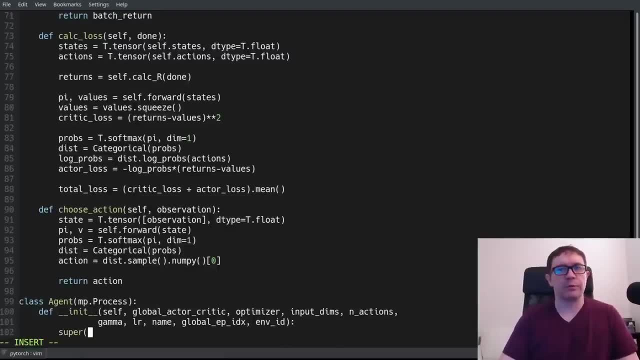 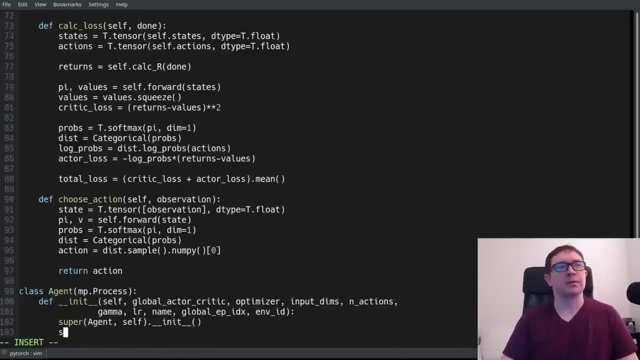 It's not as easy of a concept as it may seem, because you're doing asynchronous processing As well as An environment ID. So the first thing I'm going to do is call our super constructor And go ahead and start saving stuff. So our local actor critic is just going to be our new actor critic with inputs, of input. 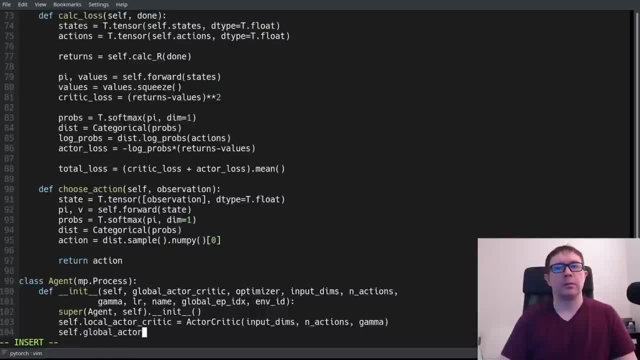 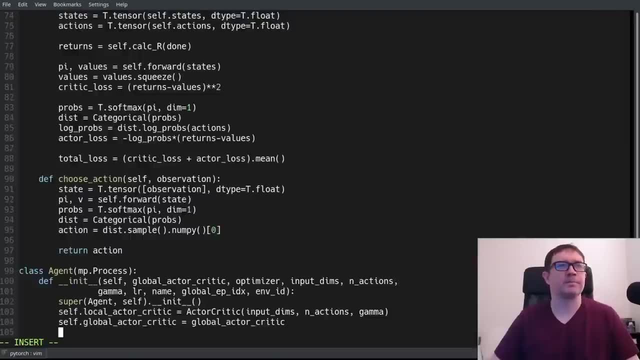 Dims, Number of actions And gamma. You want to save our global actor critic So that we can update its parameters. We're going to have a name for each worker in its own independent thread And that's just going to be. 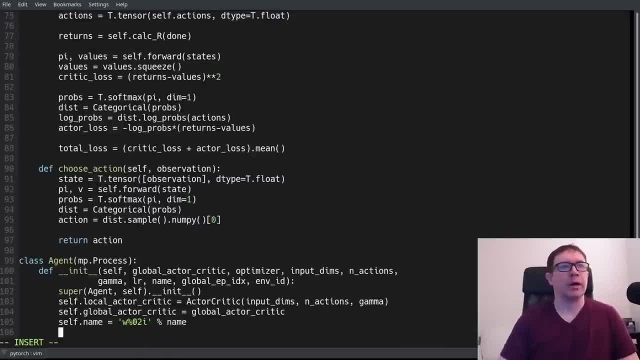 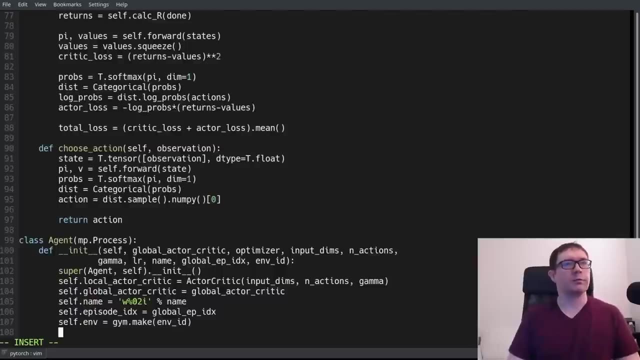 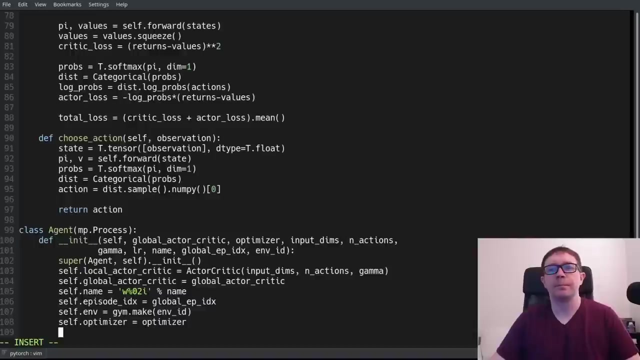 Just worker number name And then we'll have an episode index. Global episode ID X- Our environment. So environment ID is a string here That is included. Clear Um And our optimizer. I spell that correctly? Yes, I believe I did. 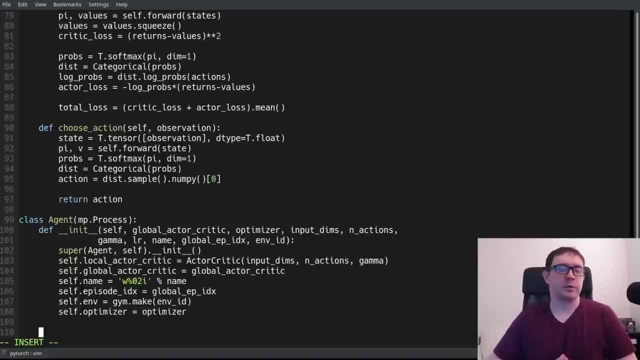 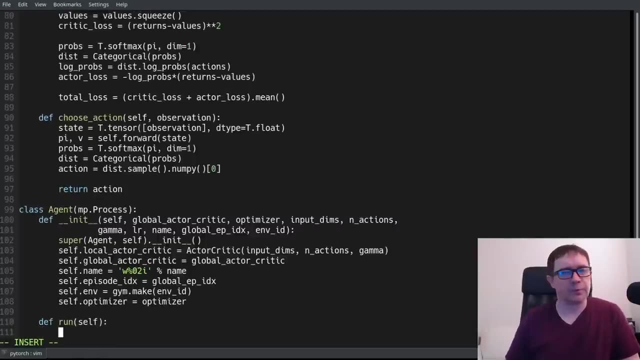 So we have to define a very specific function so that stuff actually works, And that function is the run function. This gets called behind the scenes by the worker dot start function that we're going to handle in the main loop. But this handles effectively all the main loop type functionality of our problems. 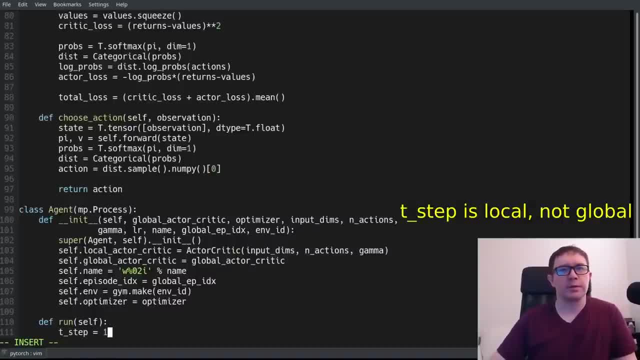 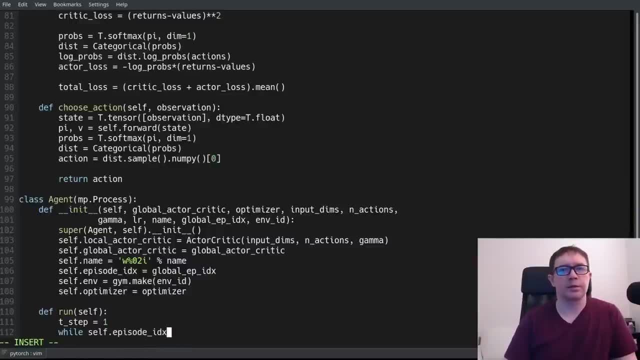 So our global time step is going to get set to one, while our episode IDX dot value. So episode IDX is a global parameter from the multiprocessing class and that we want to get the value by using the dot value dereference, And while that's less the number of games, some global variable we're going to define. 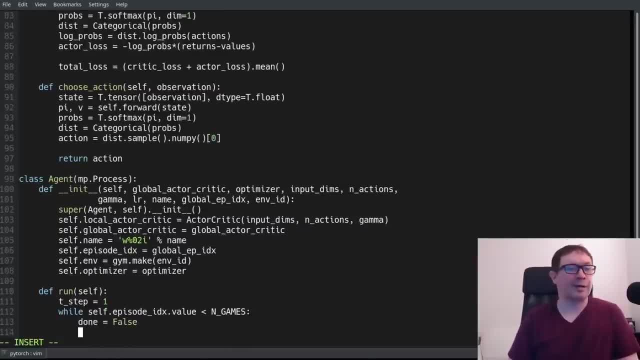 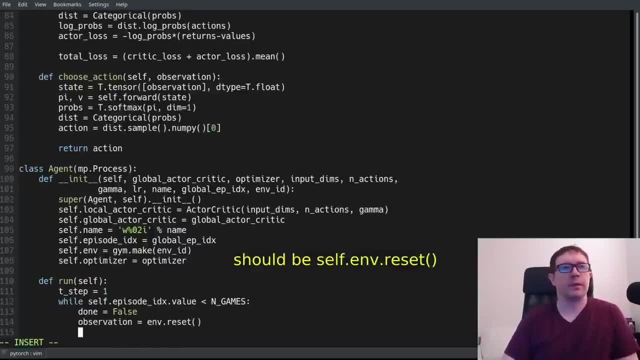 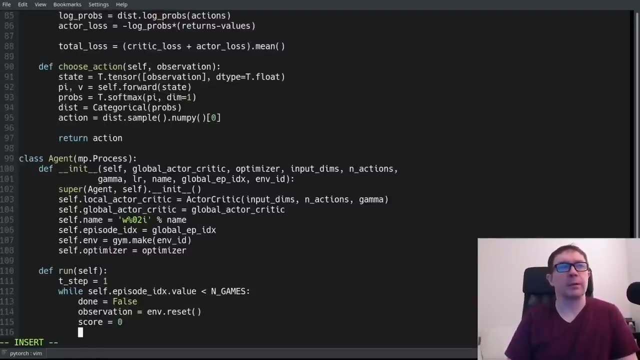 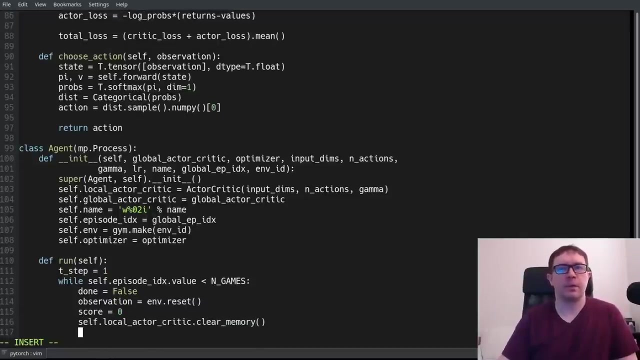 Um Uh. in other words, while we have not completed all of our games, set your terminal flag to false, reset your environment and set the score to zero, and go ahead and clear the agent's memory at the top of every episode And then, while you're not done so, go ahead and play your sequence of episodes. 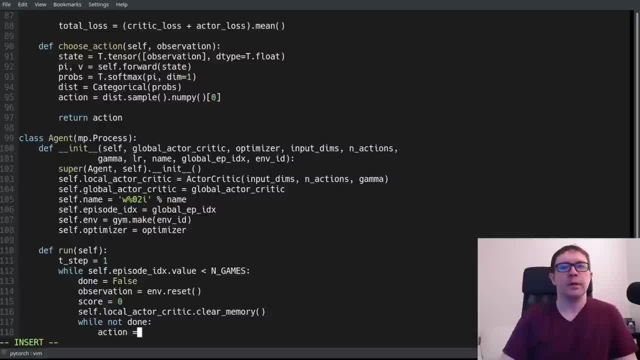 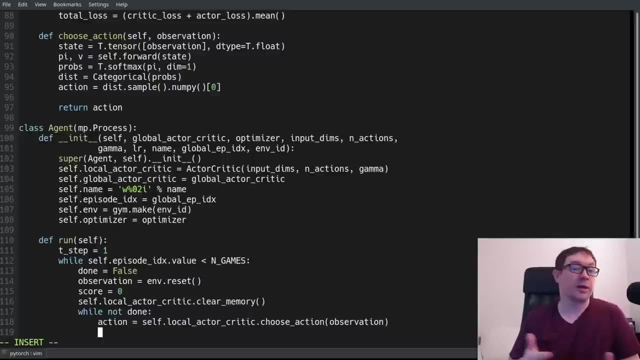 I'm sorry. Sequence of steps. Sequence of steps within an episode, The action is chosen by your local actor critic, So you're going to pass the observation into each local actor critic. So each of the 16, in this case threads- will get its own local actor critic and that'll synchronize to the global. 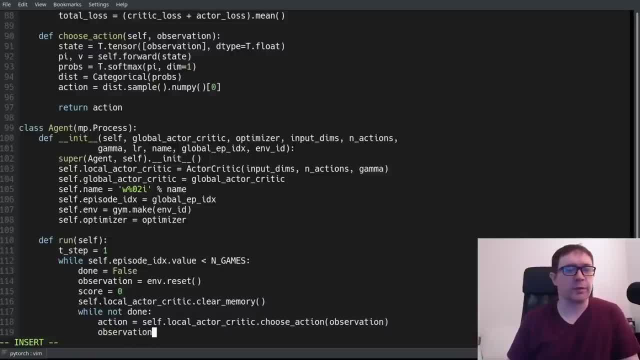 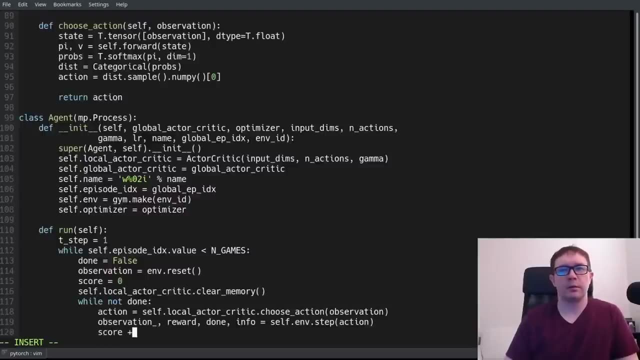 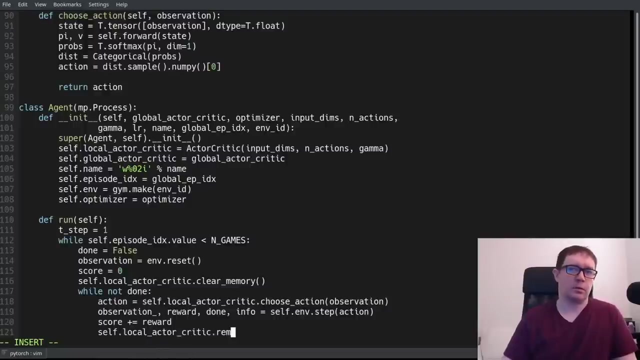 But you never actually use the global network directly to do things like choosing actions. So get the new state reward done And debug info back from your environment. Keep track of the reward received as part of the total score. Remember that observation, action and reward. 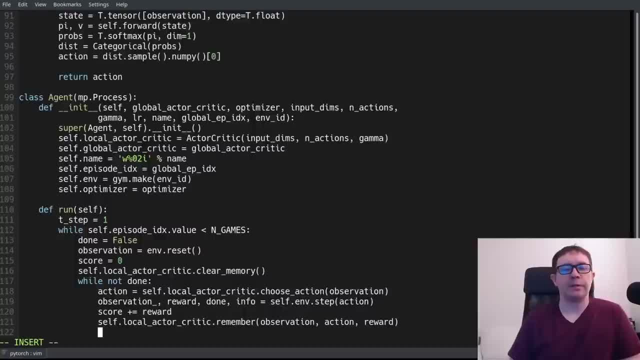 Then we have to say: if the number of steps, If the number of steps Modulus the maximum number of steps, is zero, In other words, if it is every, if it is every fifth time step or we have finished the episode with that last time step, 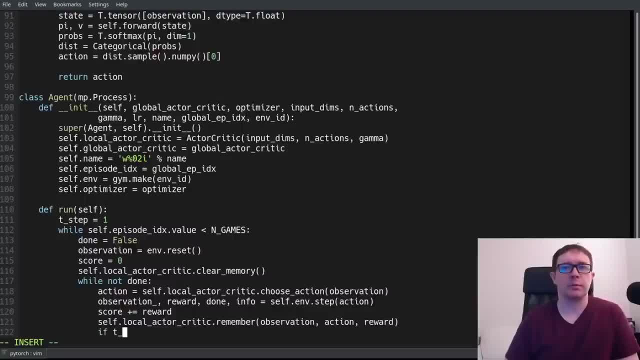 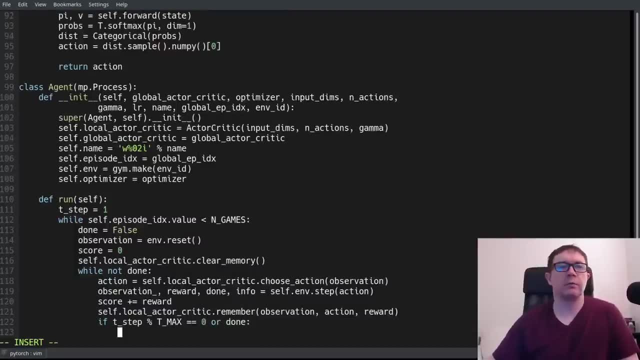 Then we're going to go ahead and perform our learning step, Modulus T max. We're done. Then we're going to go ahead and handle the learning functionality. So we'll say: loss equals local actor Critic, dot, calc, dot, calc, loss. of course we need the most recent terminal flag as the parameter for that function. 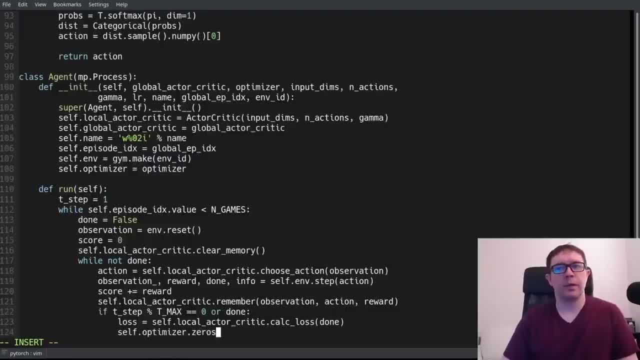 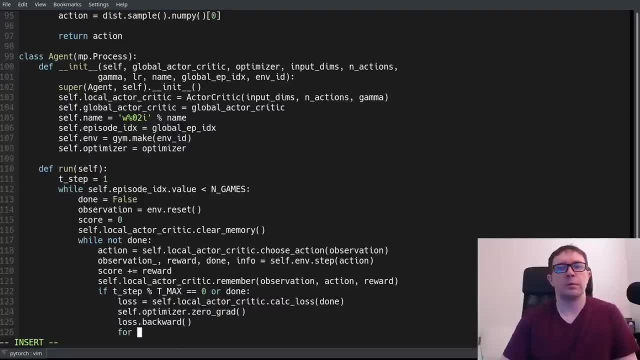 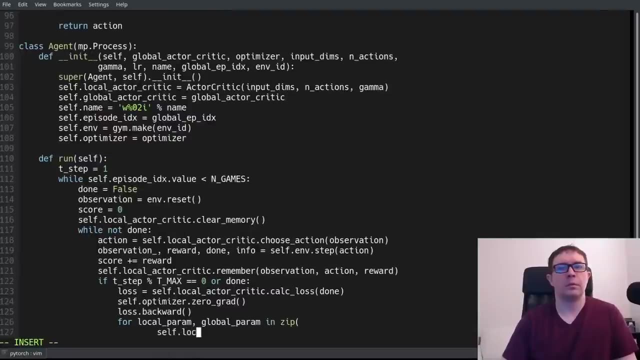 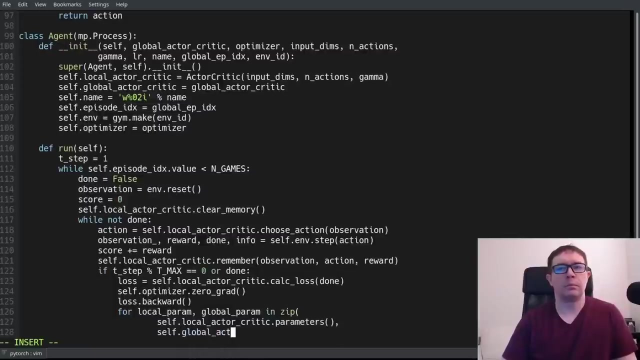 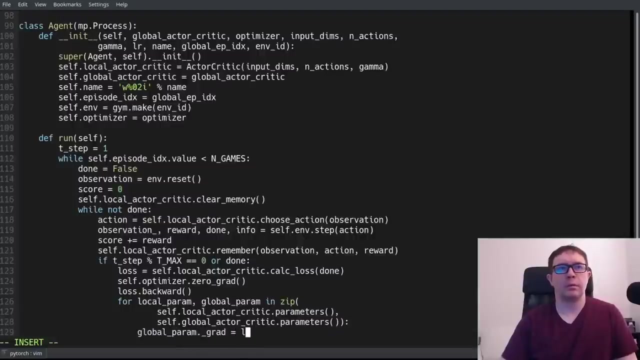 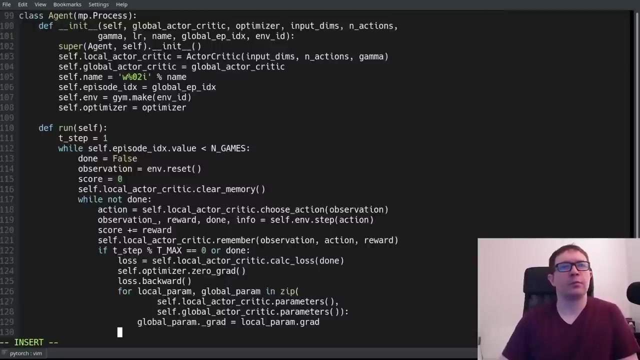 the argument: go ahead and zero your gradient and back propagate your loss. so we're going to set the parameter for the global gradient to the local agent's gradient at this step and then, after doing that, we can tell our optimizer to step, and then we can go. 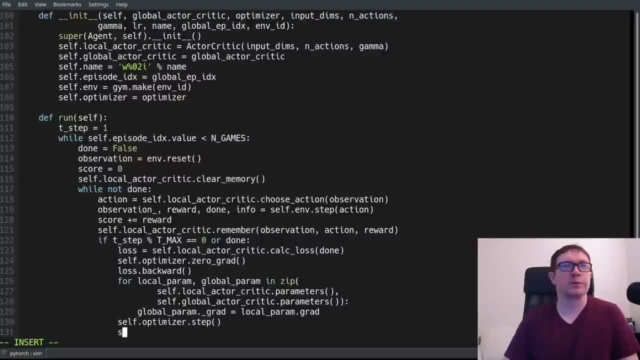 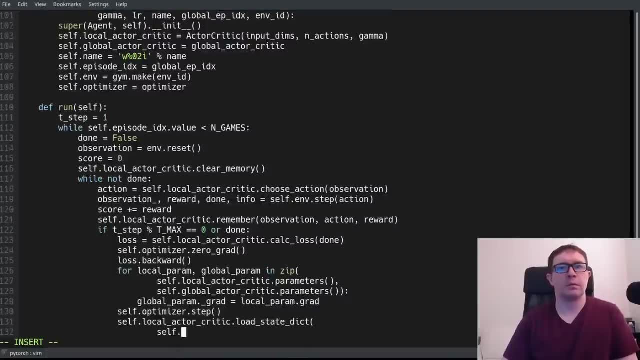 ahead and set the parameter for the global gradient to the local agent's gradient at this step and synchronize our networks. and we do that by loading the state dictionary from our global actor critic to our local one. and then we want to go ahead and clear the memory. 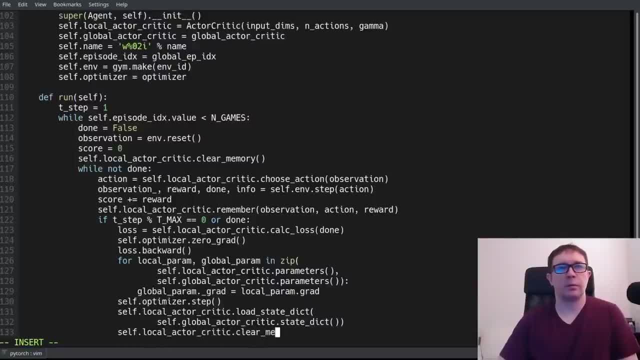 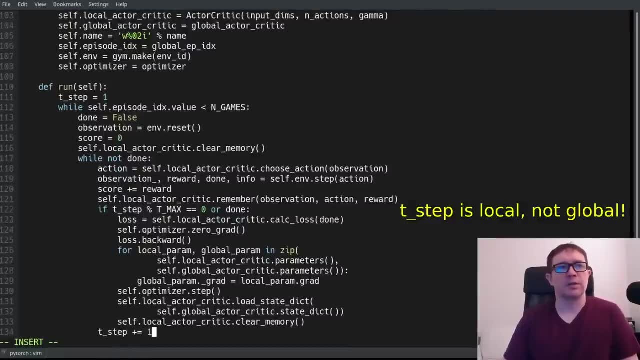 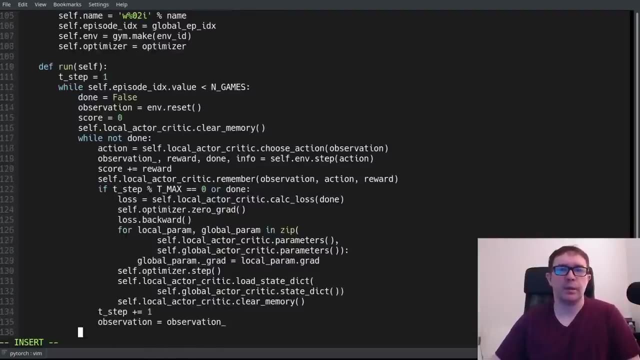 after each learning step and then tell the algorithm and then tell the algorithm and then tell the algorithm to increment t step by one, the global time step, and set the current state to the new state. then at the end of every episode we have to handle the the fact. 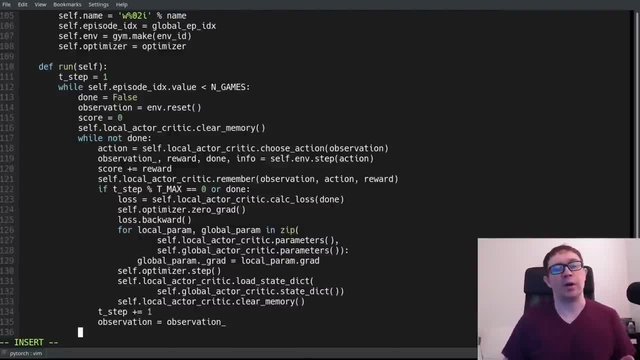 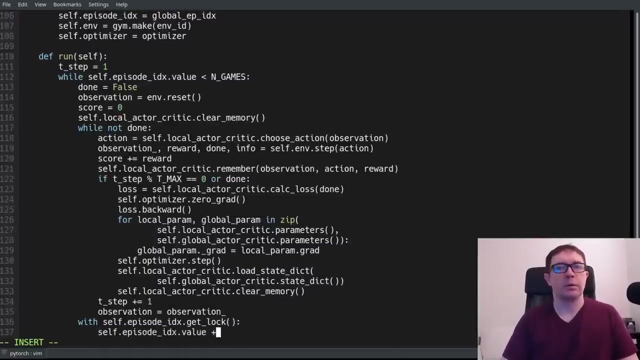 that we may have finished an episode from another agent while one, Fred, was running, because this is running asynchronous, asynchronously. so we say with self duck global, sorry, self episode ID X get lock. so we want to make sure that no other thread is trying to access that variable right now. and if we 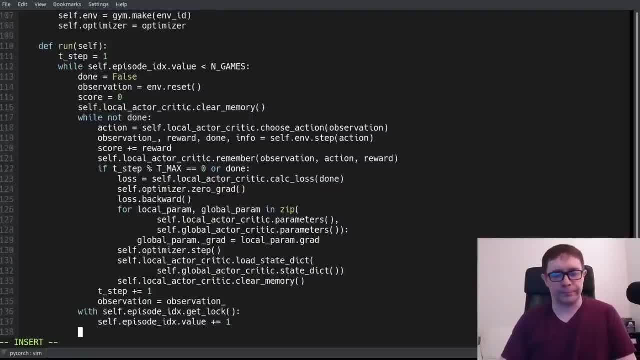 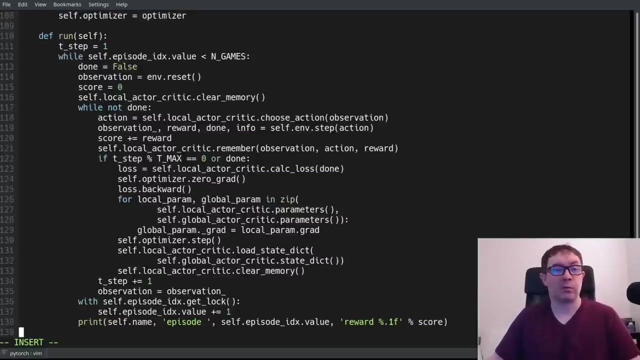 can go ahead and increment that episode value by one. then we do the usual print the debug stuff to the terminal. we're gonna print out the name of the worker, the episode, episode IDX value and the reward, the total score from the episode. that is it for our agent class. so this is relatively straightforward. all we're. 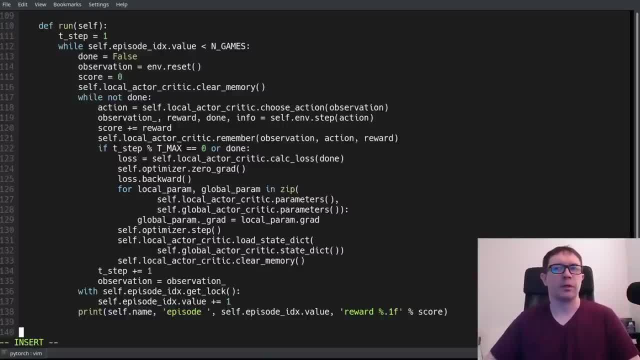 doing is now handling the fact that we have our local parameter, our local agent that chooses actions. we're going to perform the gradient descent optimizer update using the gradients calculated by the actions of that agent and then upload that to our global network so that every, every agent. 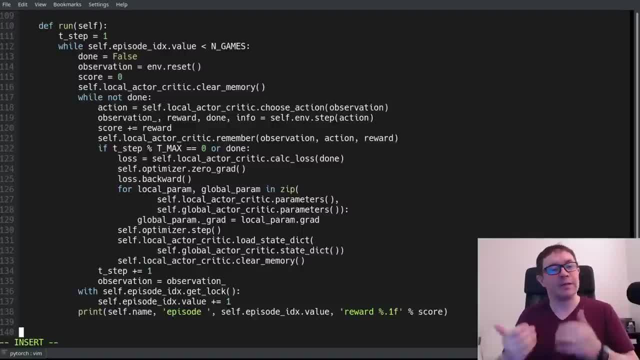 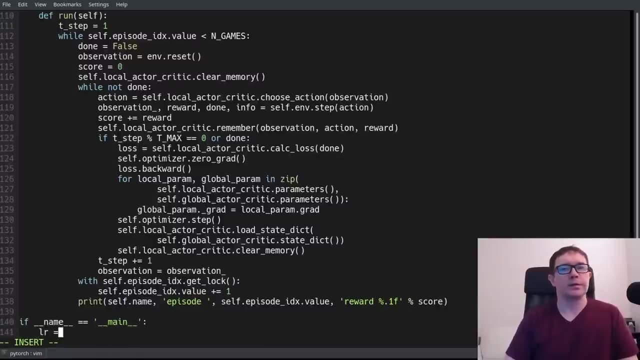 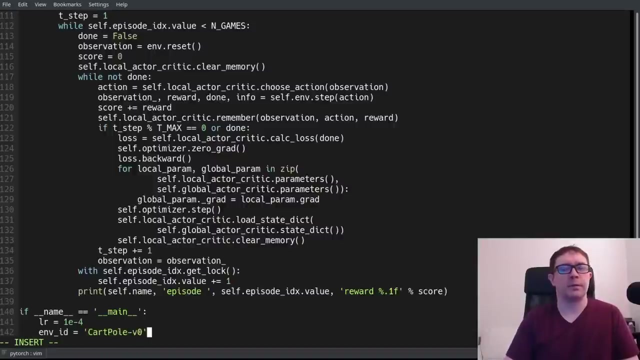 uploads its learnings to the global network, and then we're going to go ahead and download that from our global network as well, so that we make each agent in its own thread better over time. now we have our main loop and we're going to do some stuff like declaring our learning rate, our environment, ID cart. 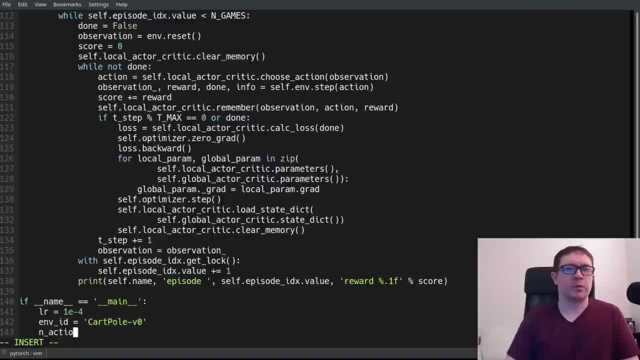 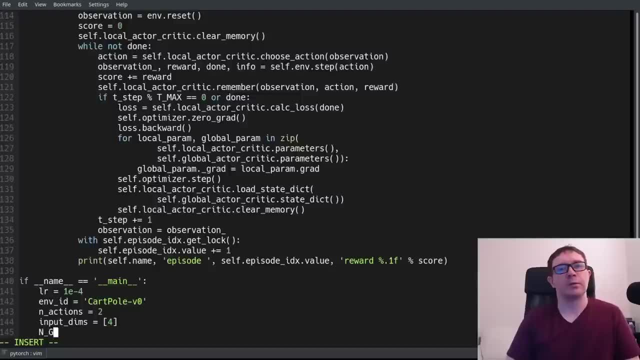 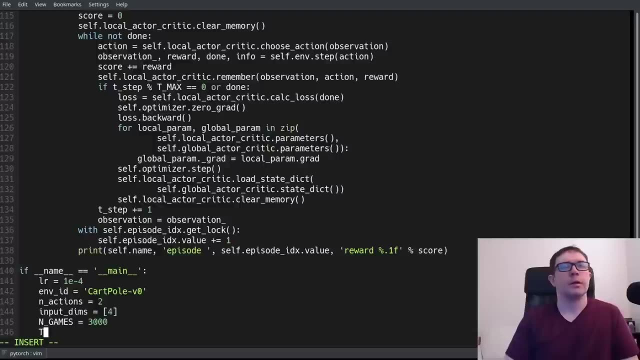 pole v0. number of actions for that environment is just two. left and right input dims. it's just a four vector. we'll say number of games: five thousand. you know we can actually get away with three thousand, I believe. team max every five steps. that comes from the paper: a global. 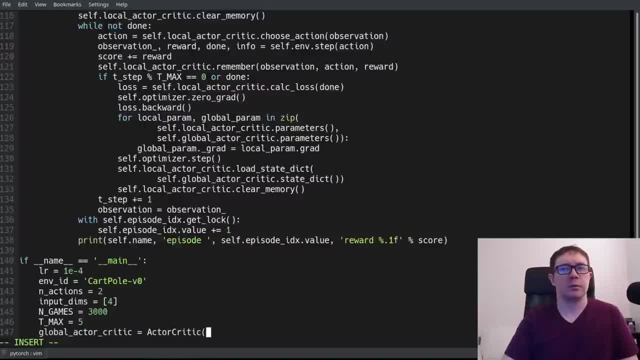 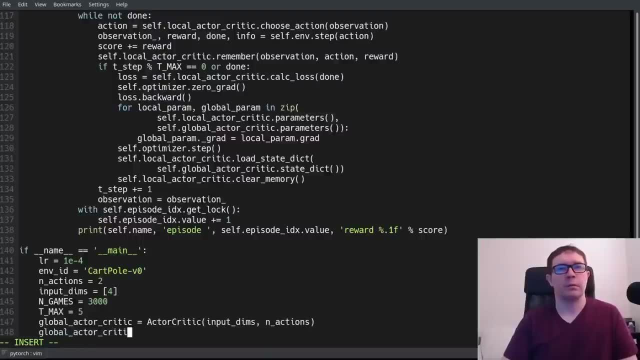 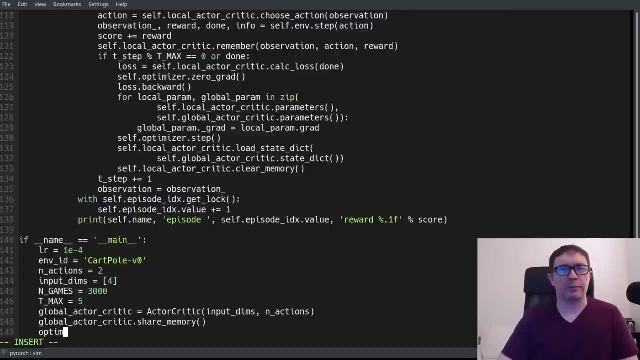 actor critic gets initialized here and that takes into dims and number of actions. you want to tell that global actor critic object that we want to share its memory. then we have our optimizer. what are we going to be optimizing and sharing the parameters of our global actor critic network learning? 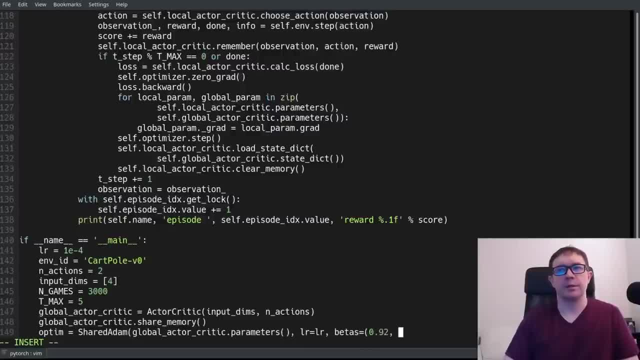 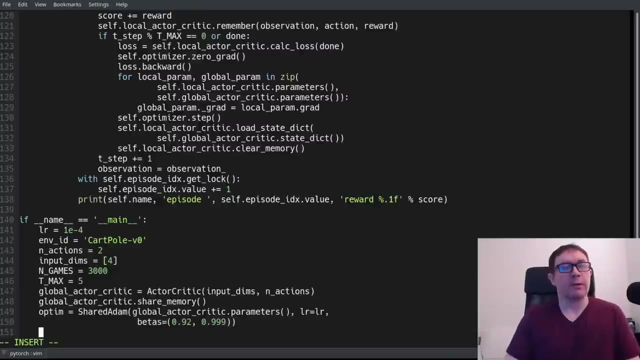 rate defined by learning rate and betas: zero point nine, two, zero nine, nine, nine. I get that from more Van Joe's stuff. I haven't experimented with that too much. a little bit of cargo, cargo called programming here. I apologize for that. now we have our global episode and that is just going to be a value of type I. that means unsigned. 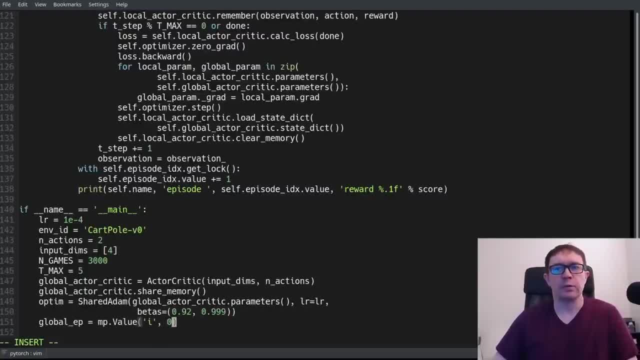 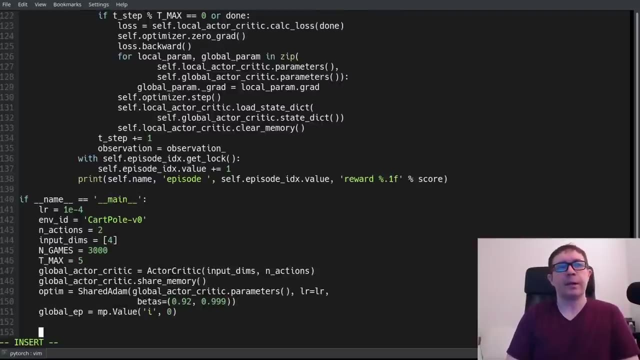 integer doesn't mean I as an account or variable. you could also have D for a double if you wanted to keep track of all the values that we're going to be doing, like a score or something like that. I just means unsigned integer or no. it's a. it's a sign in the term, so it could be negative as well as positive now. 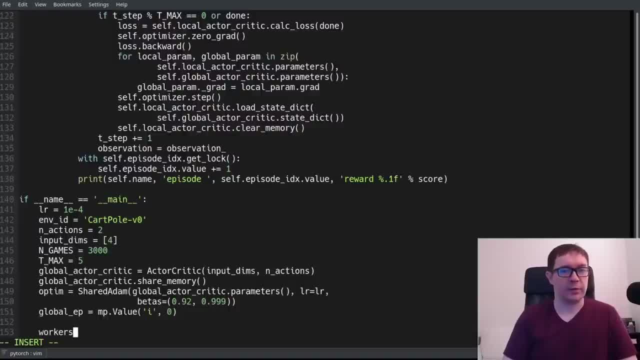 we have to create a list of workers and that's going to be a list of our agents, and this is what's. this is the construct that we're going to use to handle the starting and running of our specific threads. so that's an agent we have to. pass in our global actor critic or optimizer. so now we can see here that we have a step by step mount. we're going to go ahead and call all our parameters. we're going to say to our agent: now we have a step by step mount so that we make. 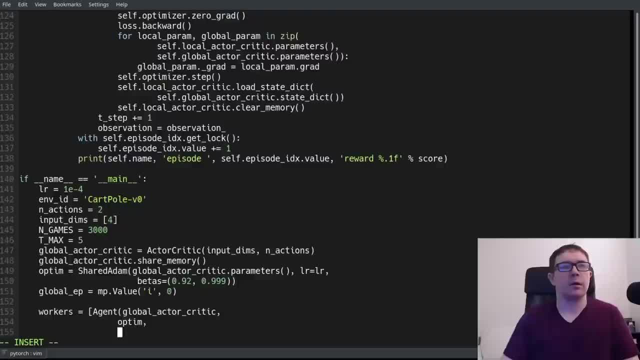 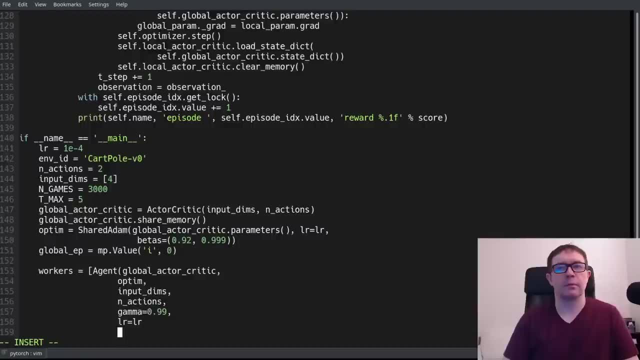 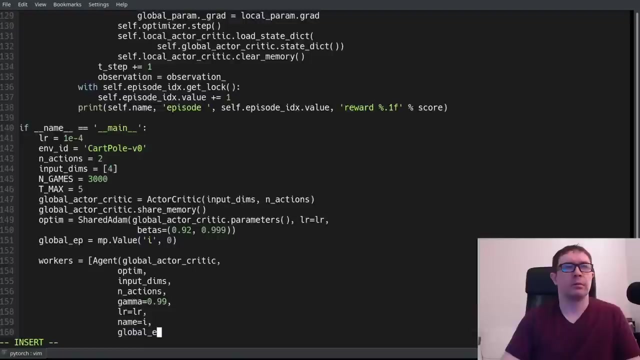 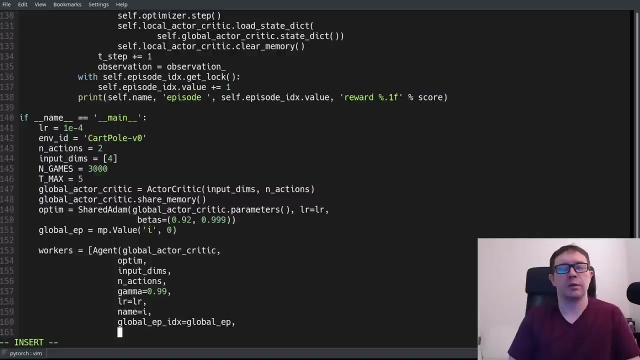 optimizer, our input dims, number of actions, a gamma learning rate. it's helpful to use commas. our name is just going to be the. the name is just going to be the I in our list comprehension. our global episode ID X is going to be that global EP variable we just defined and we're gonna pass in our environment. 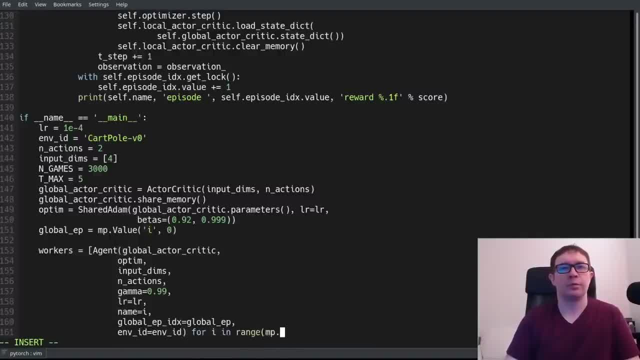 ID or I in range multiprocessing CPU count. now I haven't noticed a huge difference in running this with different numbers, so something other than CPU count. in the range I have 16 threads. if I tell it 8, it still uses all 16, so I'm probably missing something here. I could do a deeper. 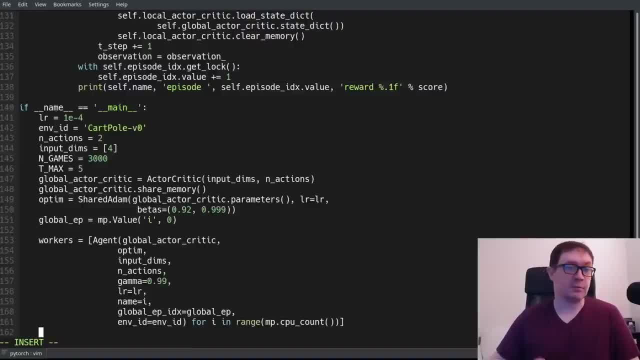 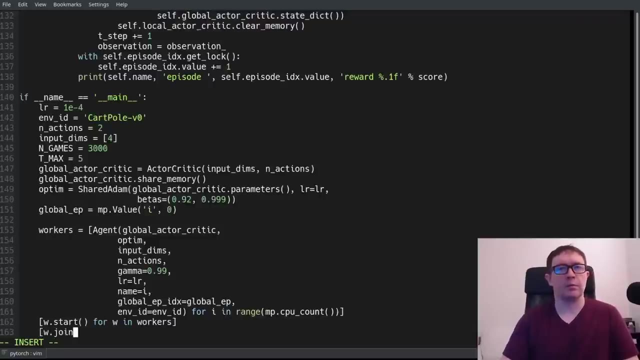 document, dive into the documentation to figure it out, but for the purposes of the video I'm just gonna go ahead and roll with it. so now we want to go ahead and start all of our workers and then go ahead and do our join operation. okay, so now, moment of. 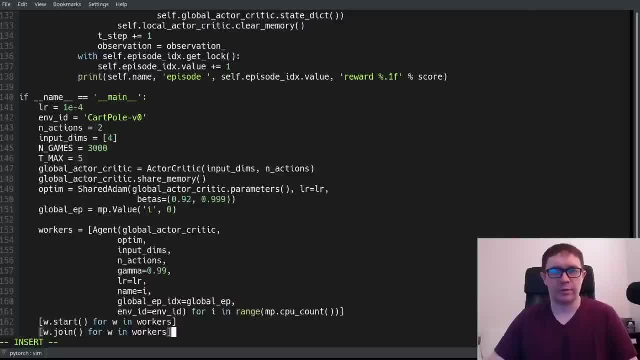 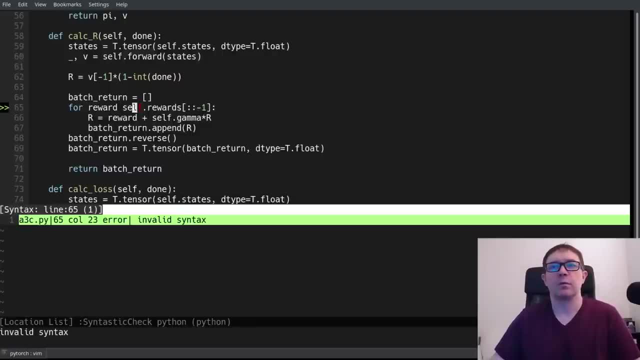 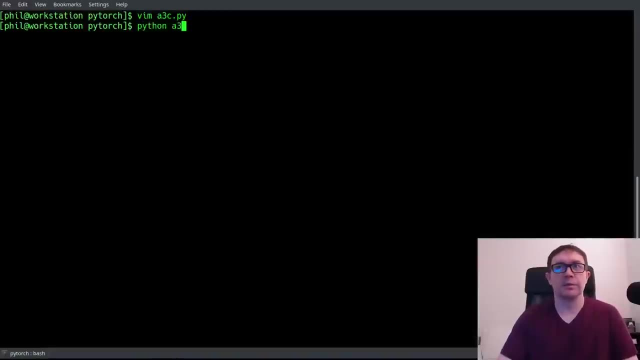 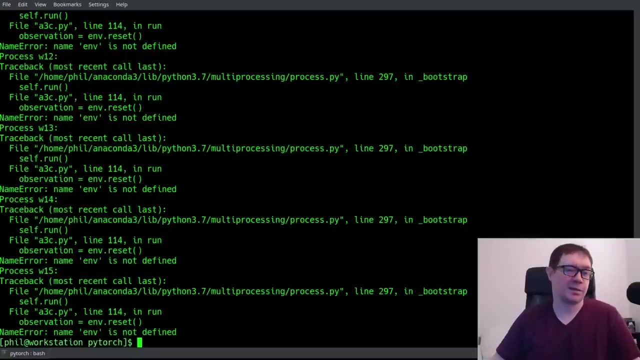 truth. I want to find out how many typos I made in the recording of this. let's go ahead and do it right now. let's go ahead and find out how many. I'm sure there are a lot for a lot of these, but that's pretty much. all I'm going to do is I'm going to build my new. program here, and let's do that for this program here, and then first thing I'm going to do is I'm going to abort it, so let's do that, and then, after I supervised our task, let's see how many bits we have. that's, that is actually a recursive troublemaker, okay, so four figures. so we're gonna take that. operations and经ony are asking us to put their timeline down. a district quickly, a couple other things. in many cases, obviously, exactly what we're after is going to lay about what do you have an internal database for? through the day that we're moving forward and try to pull. 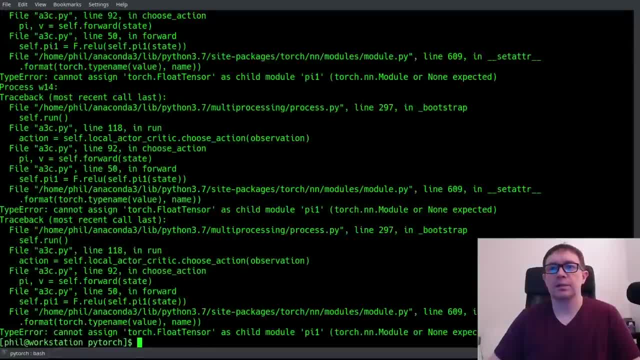 through that. two different values, just cut out, and maybe those are going to popula free. know, know, glory for sure got a digital bachelor class is going to do just that. once again. cannot assign torch float tensor as child module, pi one torch nn module or none expected, so that. 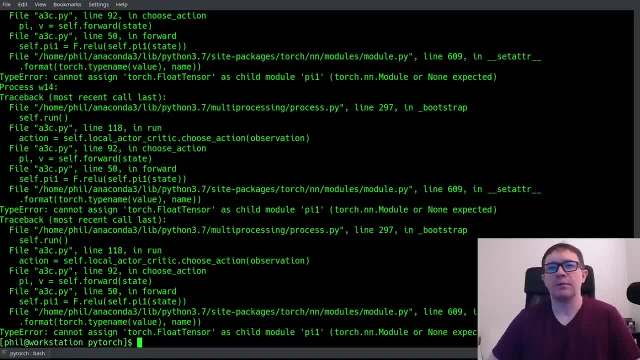 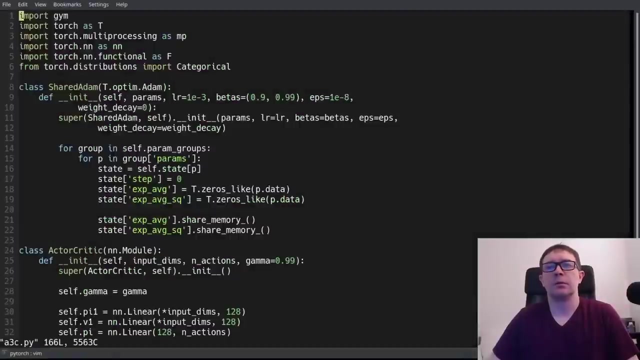 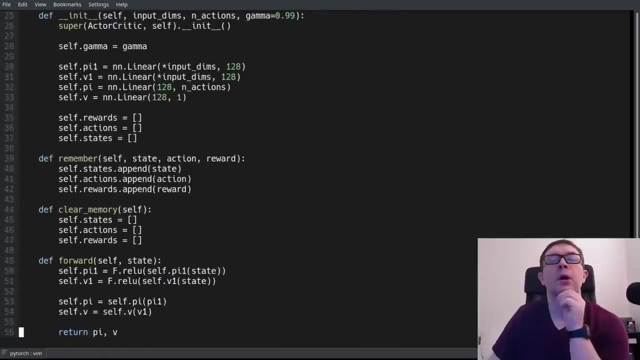 is when i handle the feed forward in our choose action function. oh, this is an interesting one. i haven't encountered this before. let's take a look. cannot assign as child module pi one. oh, that's because interesting. oh, of course. yeah, obviously i don't want that self here. i'll have to annotate that when i am. 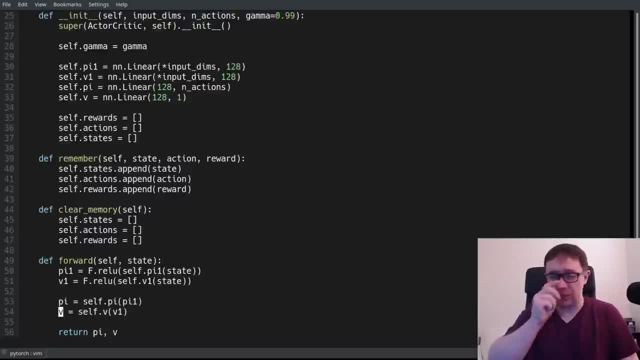 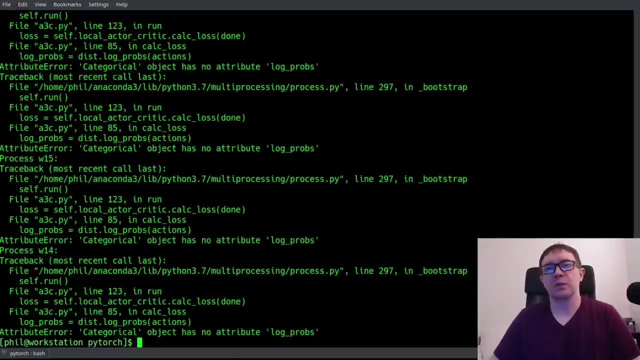 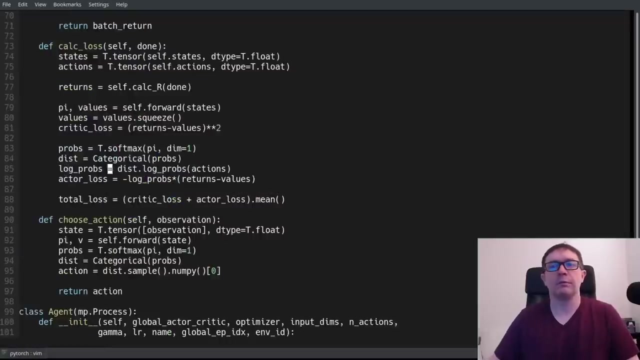 editing the video. uh, that is obviously going to be problematic. so you'll probably have seen that already that i put in a no self dot in there. okay, that's the beauty of doing things for that. oh, it's because it's log prob, not log probs. that's in 85 log prob. i hope i remember all these. 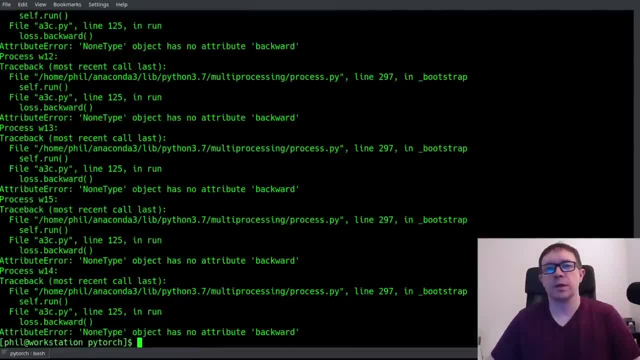 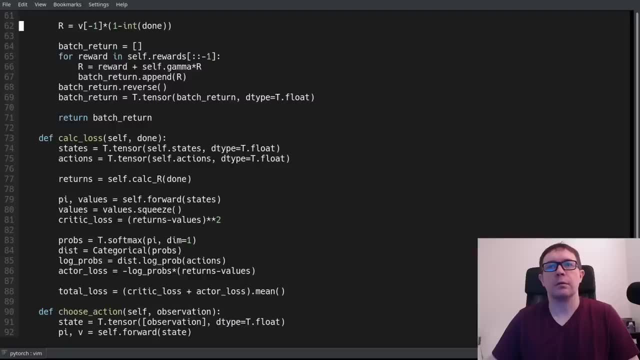 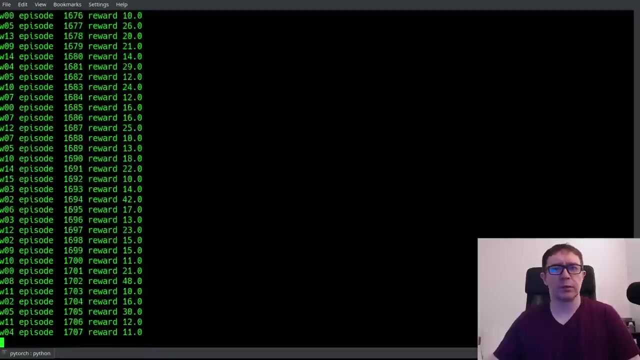 this none type object has no attribute backward. i probably forgot to return my loss. yeah, that's right there we go all right. now it's running. hopefully it's still going to record, even though it is running across all of our threads. looks like we're still good now. you see that executed really really fast. 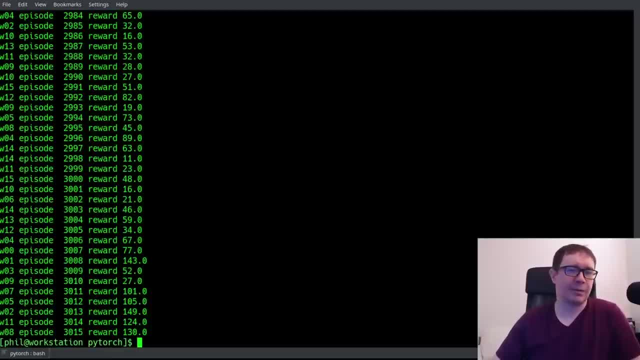 um, it was so fast i didn't even have time to get up the thread count, the resource monitor to show you guys, uh, but you can see here that it achieves a non-negligible score. so that indicates some learning is going on. now let's go ahead and run it again and you can see now this time. 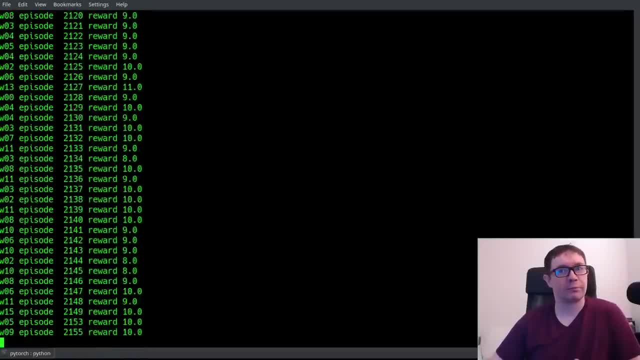 it's not doing any learning at all. so there is a significant amount of run to run variation. so i'll let it run and finish and we'll try one more time and maybe we'll get lucky and it will actually approach a score of 200. 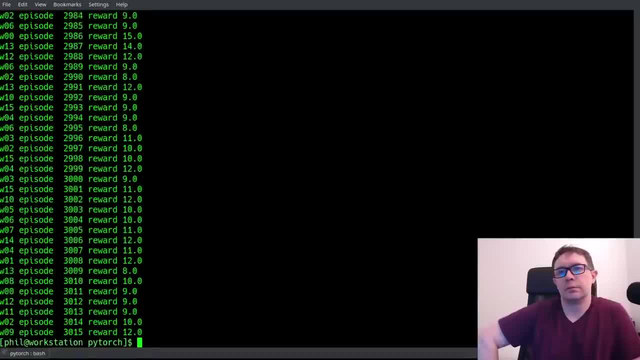 now that's one of my big criticisms of this algorithm is that there is a significant amount of run to run variation and it is pretty brittle with respect to some other algorithms that came later. basically, the main advantage here is that it's asynchronous and this paradigm can be employed. 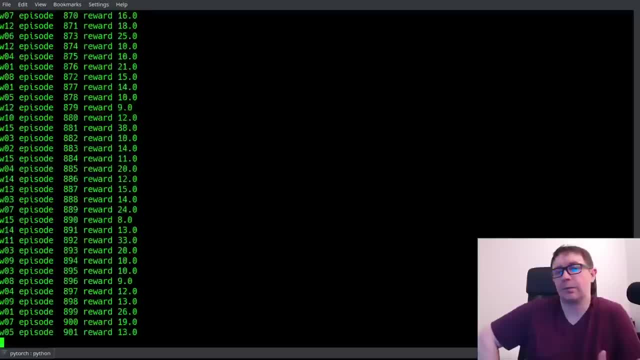 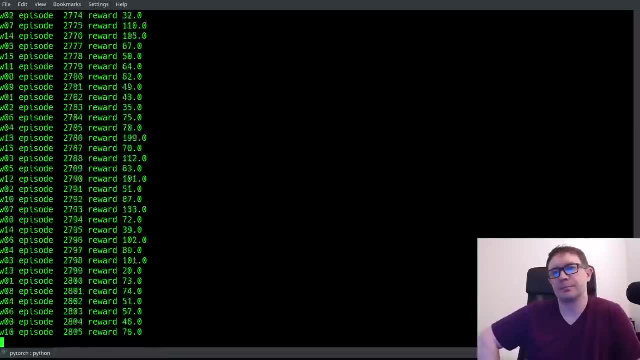 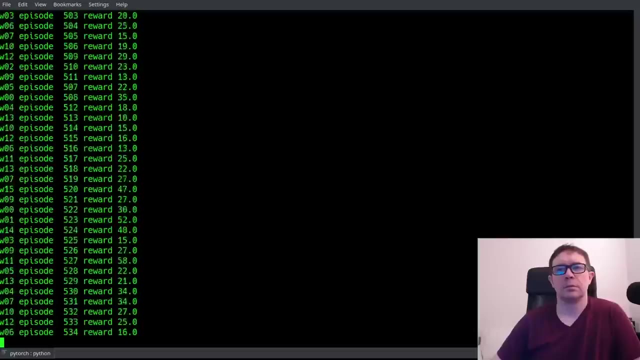 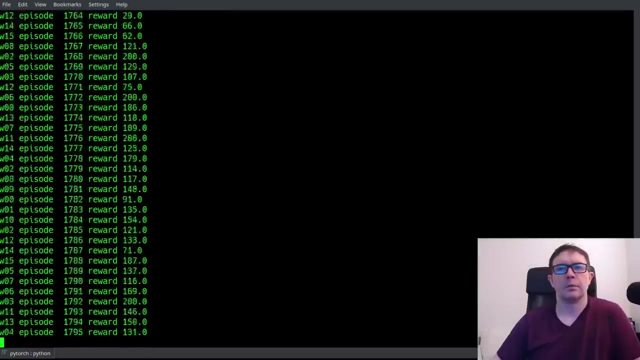 on many different types of algorithms. as you read in the paper, you know it can be applied to deep learning as well as uh n-step learn, uh sarsa, stuff like that. okay, so it's getting a little closer. okay, so it's getting a little closer. 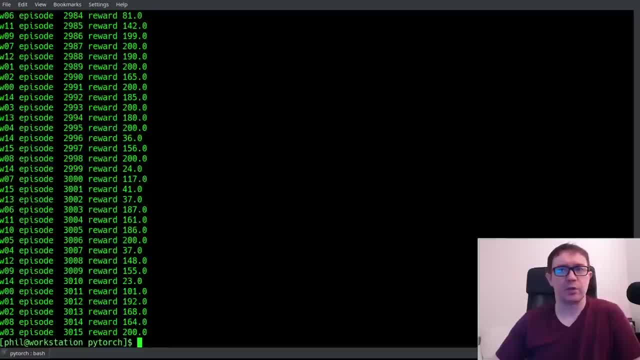 okay, so this one took a little bit longer because the episodes actually achieve scores of 200, which is the max. uh, not every thread manages to be a winner. not all of us can be winners in life. that's a nice little microcosm of the universe, uh, but you can see that for the most part, uh, some of the 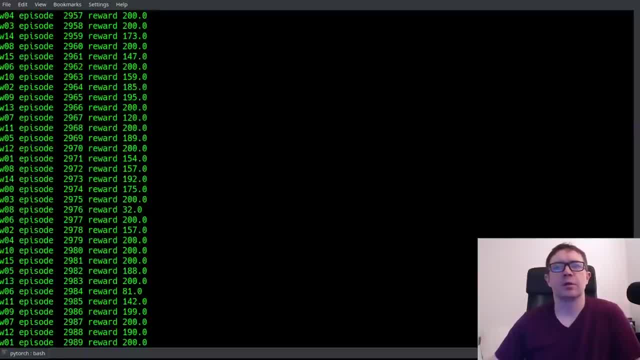 workers. actually, i wonder if there's consistency amongst so worker 11, not uh 200, and if i scan down here another, worker 11, 142, 161, 161, interesting. so, uh, you do get uh actual learning across your agents. uh, it's just not super consistent. 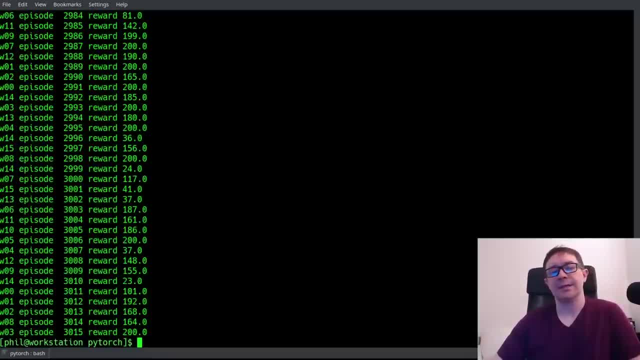 and that is my biggest criticism of this algorithm is that it has a high degree of render and variation, as you can see. uh, but it's still pretty good. it's an interesting take on deep reinforcement learning and, uh, i i do enjoy the algorithm. it's just not what i would categorize as the top two or three. 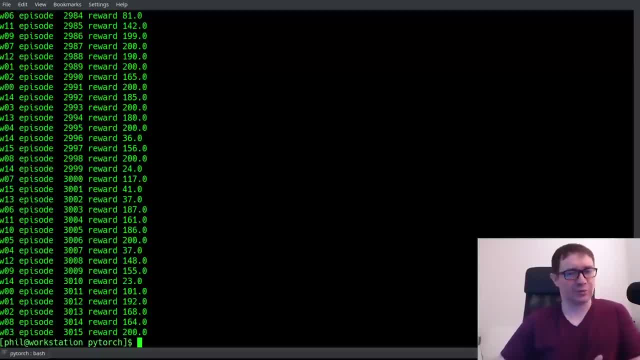 algorithm in actor critic methods. i hope this was illustrative for you. i hope you found it very helpful. if you have made it this far, please consider subscribing. leave a like, a comment down below, and i'll see you in the next video. 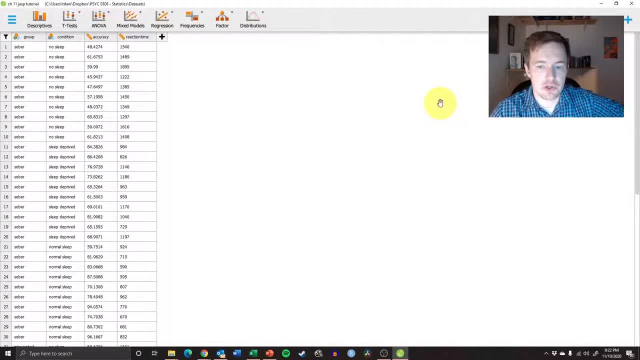 Hey everybody and welcome to another JASP tutorial. What I want to do in this video is walk you through how to do a one-way ANOVA. So just a quick little bit about the data set that I have here. I have a data set where I have two different factors. 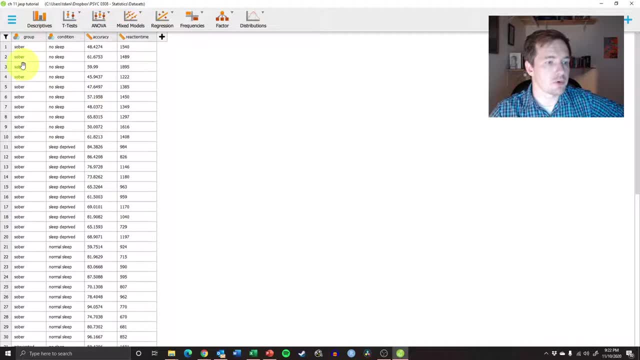 I have group and I have condition. So group being sober and intoxicated, condition being no sleep, sleep deprived or normal sleep, And so each group had people in these three conditions, So subgroups, And then we also had two dependent variables: 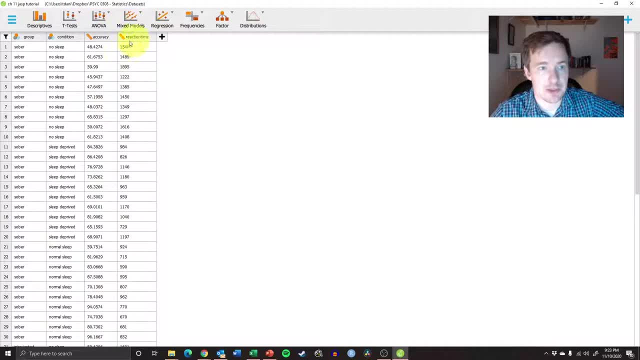 Accuracy on a memory test and reaction time measured in milliseconds on a memory test. So I am interested in: how can I analyze this? How can I make sense of it? I can't use t-tests for this. So what you want to do is you want to run up to ANOVA. You want to click on ANOVA, not surprisingly.